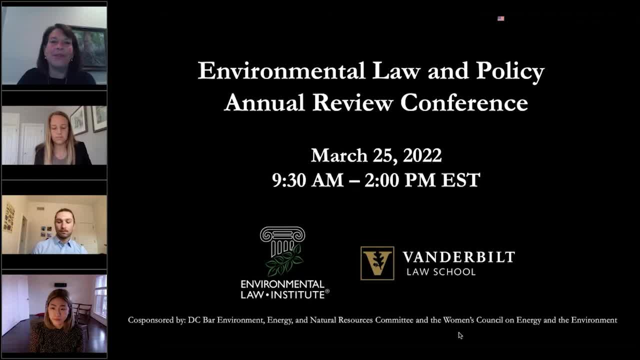 We're also very pleased again this year to welcome our co-sponsors for the conference: the DC Bar Environment, Energy and Natural Resources Committee and the Women's Council on Energy and the Environment. So it has been 14 years, which is incredible, that Environmental 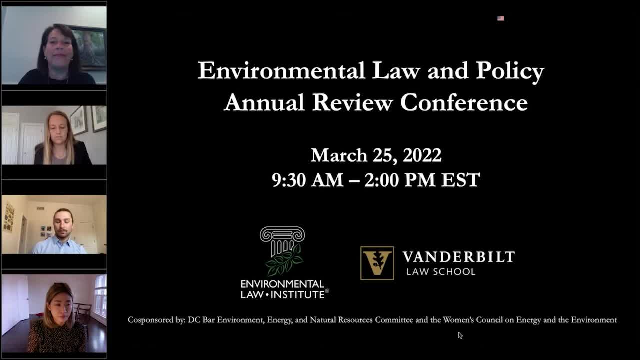 Law Institute has been able to do this And I just want to say we particularly appreciate the work that the Institute and Vanderbilt Law School have collaborated on this effort, in which law students work to identify some of the most important ideas from the legal academic literature each year and bring them to policymakers and practitioners. We could 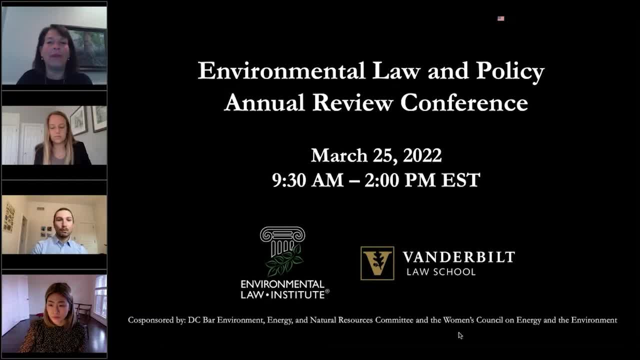 not do this without the help of our stellar committee of public and private sector leaders, our advisory committee, And I think Heather has a slide just to show who those wonderful individuals are. They're also listed on our webpage, As you may know. the articles that 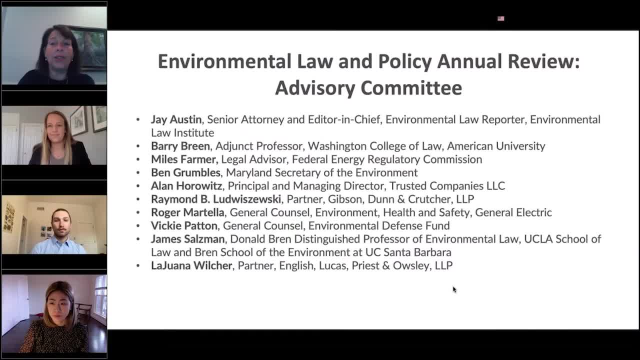 we select each year to discuss at this conference are also published in shortened form with commentaries in the Environmental Law Reporter each August, And I want to just say a special thank you to the ELR team for making this all work, So particularly Jay Austin, Rachel. 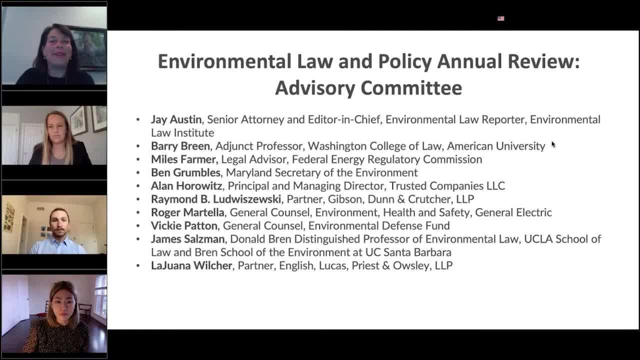 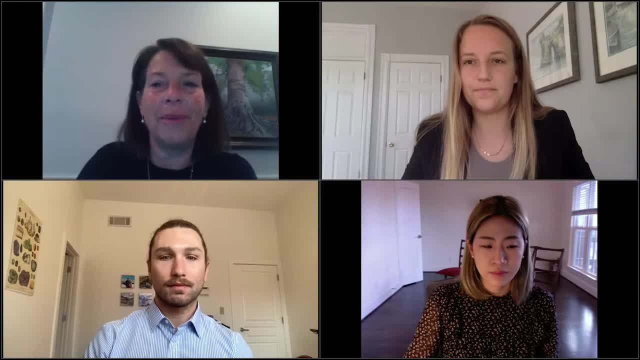 Jean-Baptiste and Bill Stroh, You're going to learn more about the process we use to select articles in just a minute from our wonderful third-year Vanderbilt Law students. But now I want to turn it over to Mike Vandenberg, who's actually here in the room with me. 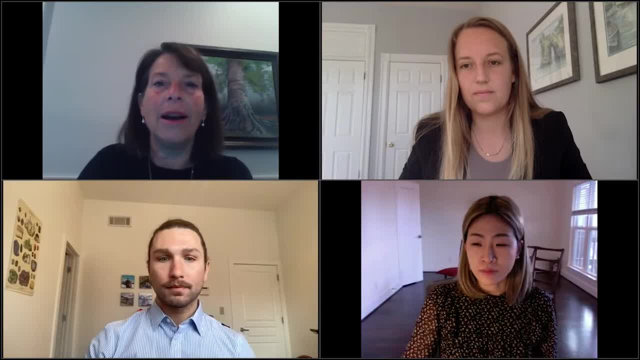 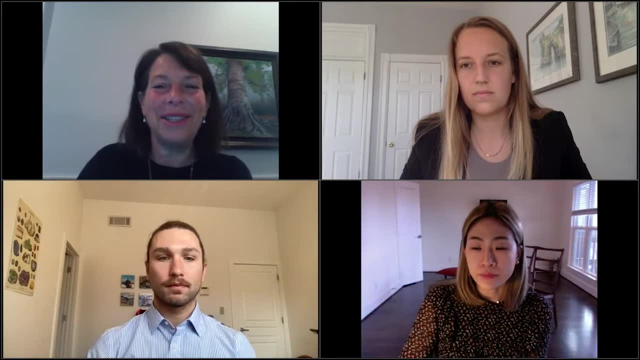 to talk about what we're trying to achieve with ELPAR. Mike is a chaired professor at Vanderbilt University Law School and director of the Climate Change Research Network. He's also my co-instructor for the ELPAR course at Vanderbilt and also a close family member, So I'm going. 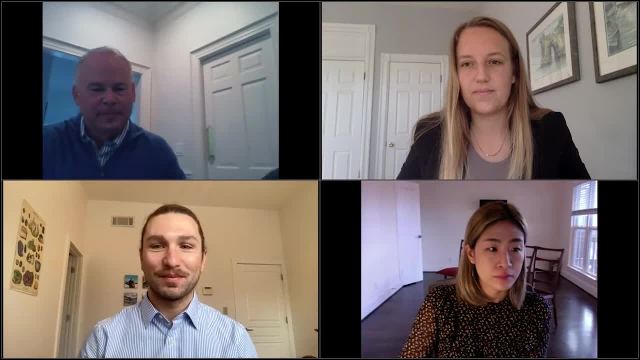 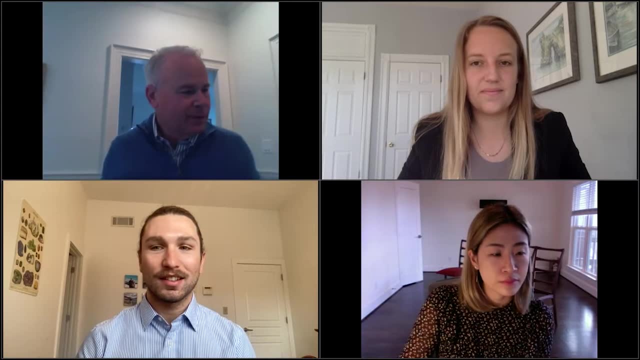 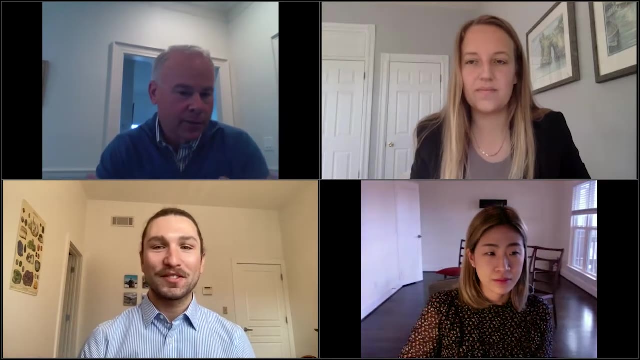 to hand this over to Mike Great Close family member- I love that- Also known sometimes as husband. So I'm going to hand this over to Mike. So let me just describe, if I may, for a moment what we're trying. 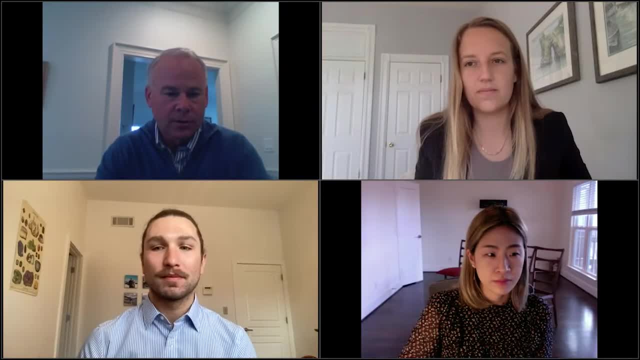 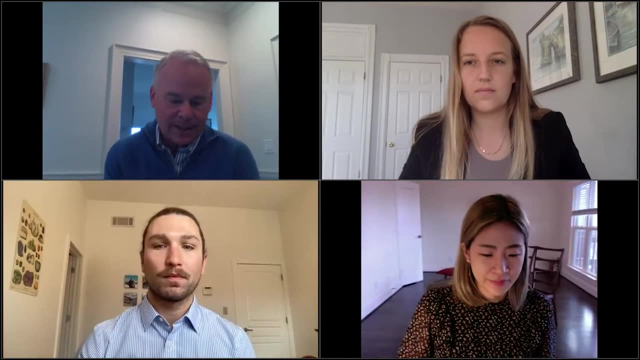 to accomplish and welcome everyone on behalf of Vanderbilt University Law School. This is a wonderful collaboration with the Environmental Law Institute. We're really lucky to be able to do this. We're trying to do several very basic things here. The first is to provide 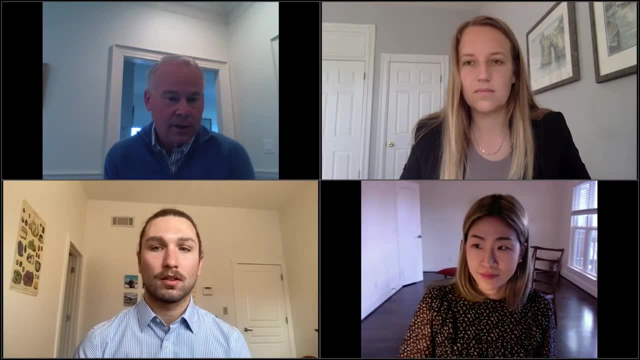 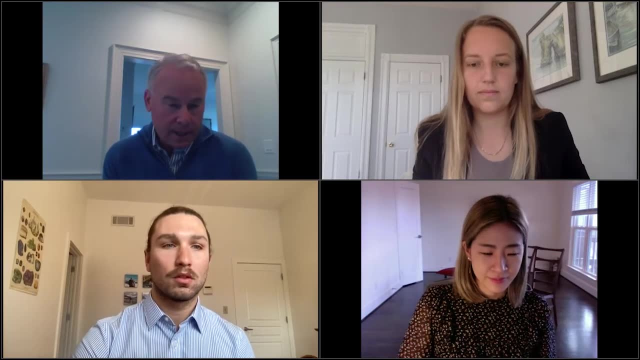 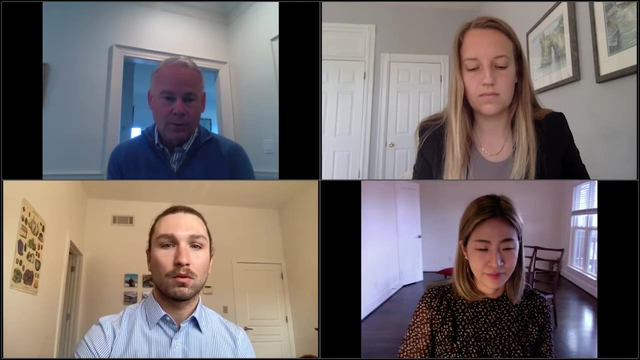 an exceptional educational experience for our students, whether it is selecting articles from among the three to five hundred published every year and arguing about which are the best policy ideas, to presenting programs like the one we have today, to organizing and managing what is effectively both a class and an organization. All those things we 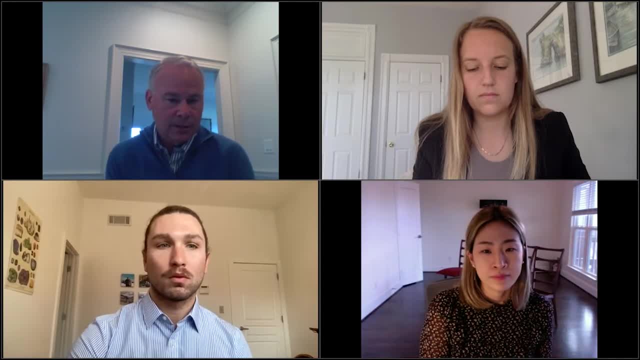 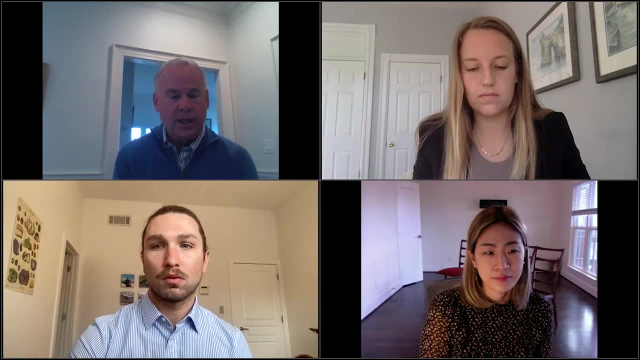 hope, provide a truly exceptional educational experience, And that's really goal number one in many ways. The second is one that may be a little less obvious, and that is that we are trying to encourage academics not to just invent a can opener every time they need to open a can. 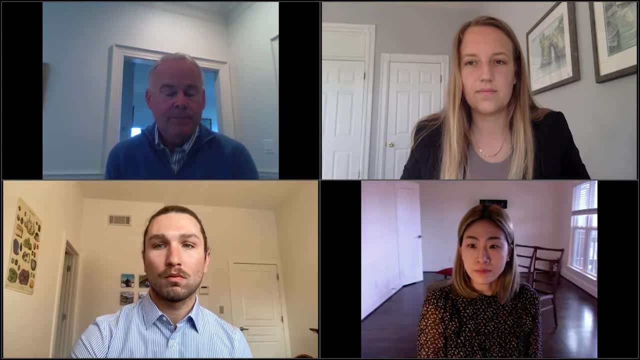 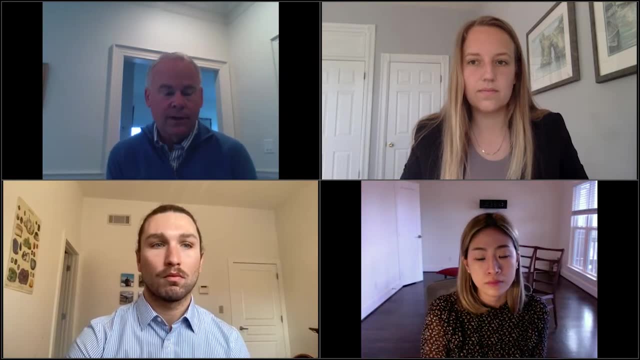 And that's essentially the incentives that we all have in the academy. Stick with the theory. Don't get bogged down in the feasibility of your ideas, And on some level that may make a lot of sense. We want to all develop new theoretical approaches to problems. The 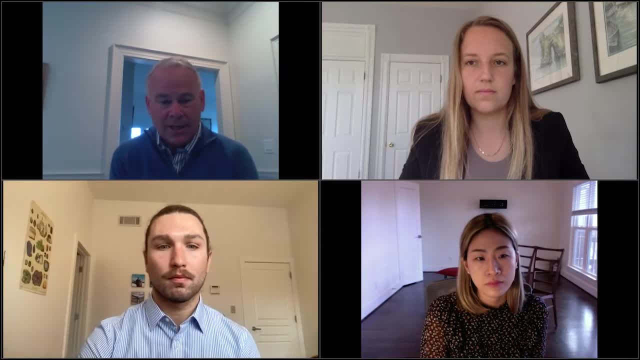 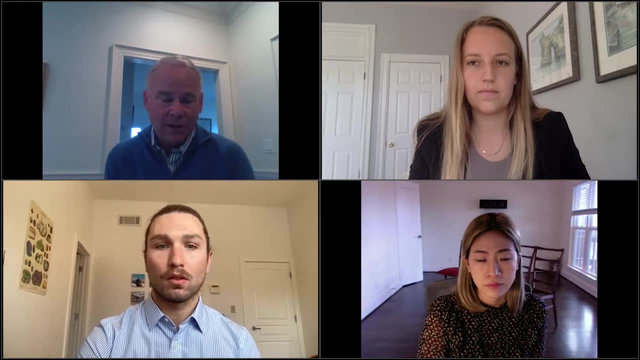 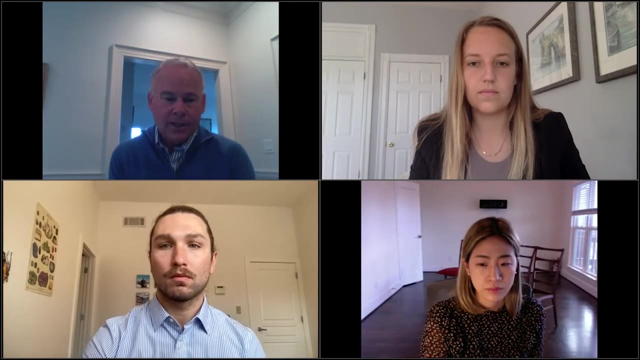 challenge is that your theory can be very weak if you don't test your theory against the feasibility of different policy implications. So our goal here is to find those articles that take that very difficult step of examining and proposing feasible policy options. And we're doing it not just because we want to identify those options, but because we want 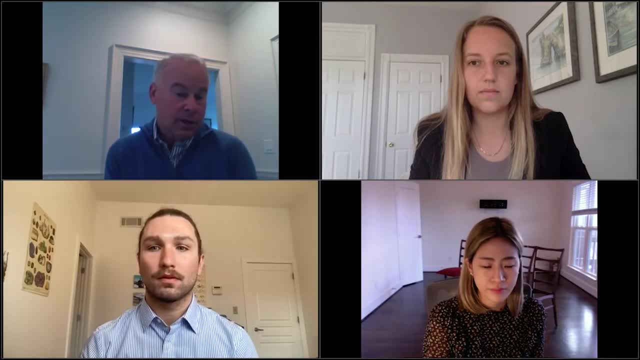 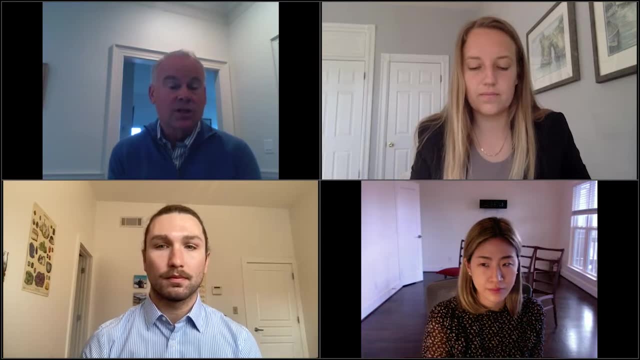 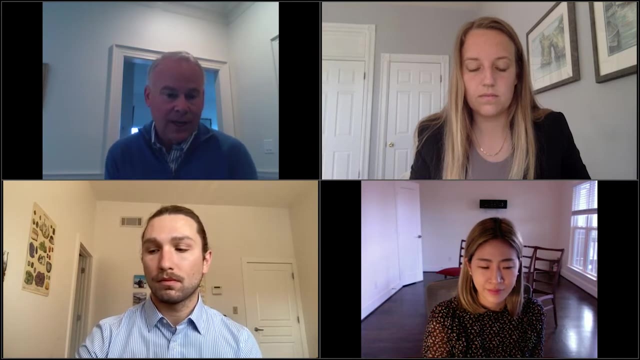 to improve the quality of academic scholarship by forcing or inducing, encouraging, encouraging: encouraging academics to really wrestle with the hard questions that feasibility presents to theory, not just to feasibility itself. And then, lastly, and the principal focus of today's event, 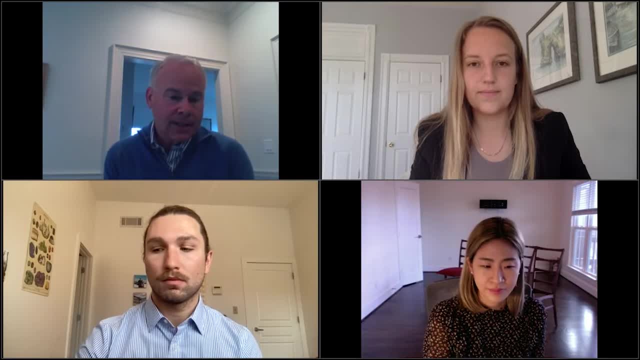 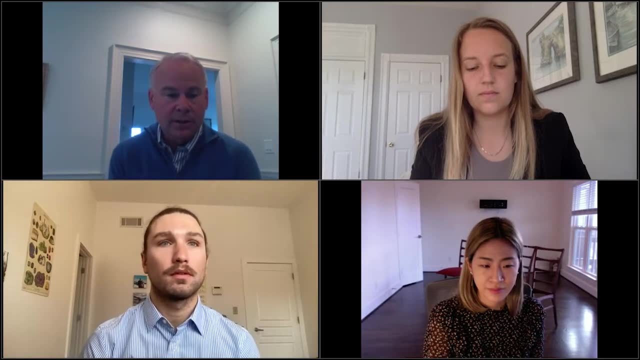 is that we're hoping to move ideas from the academic world into the policy world. Linda and I both served in the Clinton administration. We both were following the legal literature at the time and almost none of it was relevant to the kind of work we did day to day, because it tended 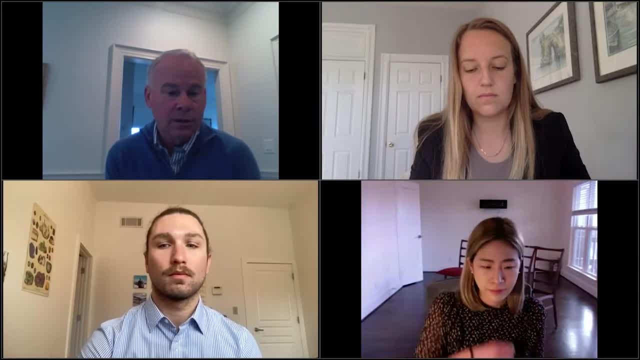 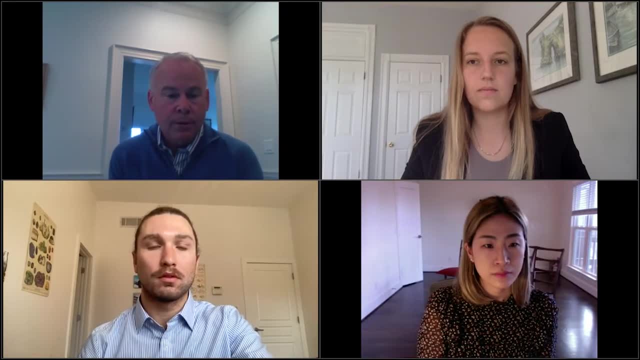 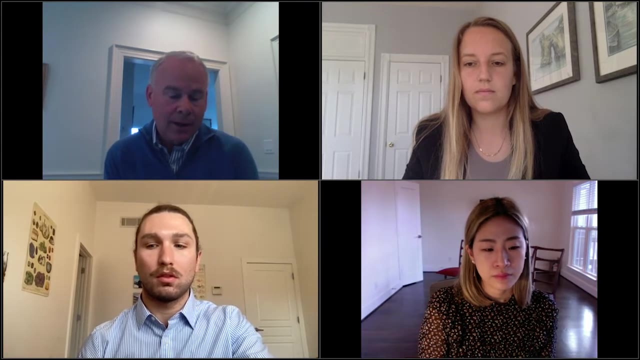 to be too dense, too many footnotes, really hard to move into quick thinking for people who are under lots of pressure to develop new ideas. So the idea here with our program is to help us produce a forum in which we can move ideas in a way that are easily digestible into the policy world and 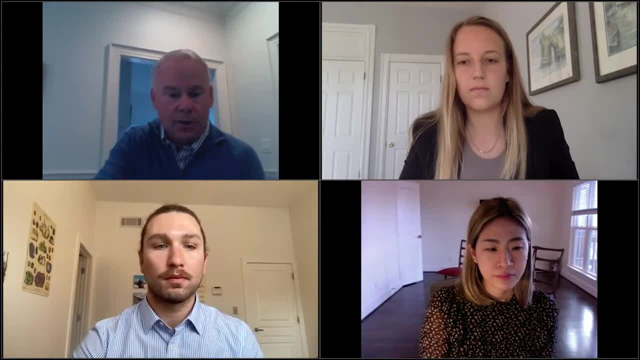 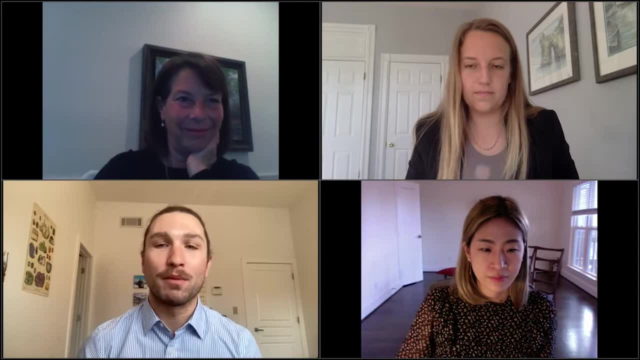 we hope that's what will occur today. So back to you, Back to Bruce, Bruce, on to you, Bruce. All right, thank you, Professor Vandenberg. Good morning and welcome everyone. My name is Bruce Johnson and I'm the professor at the University of Michigan. I'm a professor at the University of 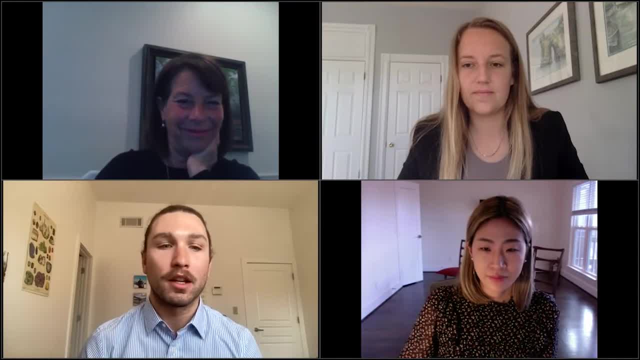 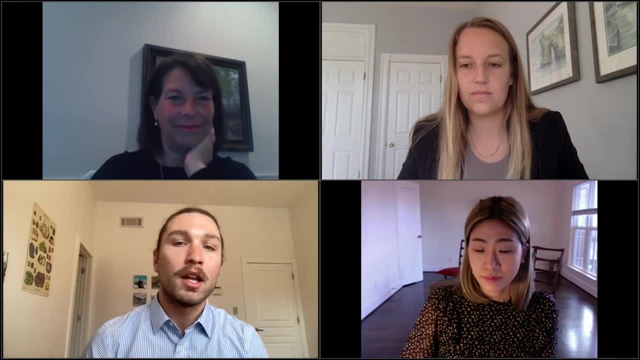 Michigan, and I have the true honor of being the editor in chief of the 2021-2022 edition of the Environmental Law and Policy Annual Review, or, as we like to affectionately call it, LPAR. I want to quickly acknowledge the hard work of our 22 student members. 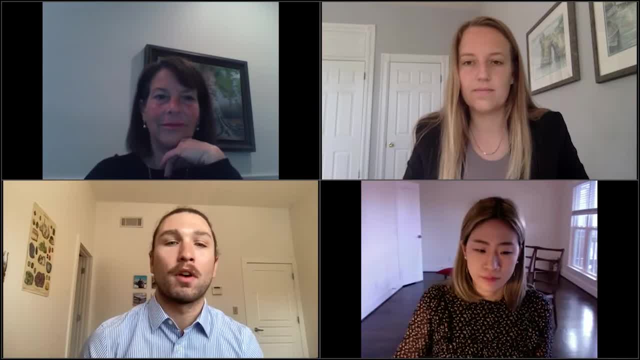 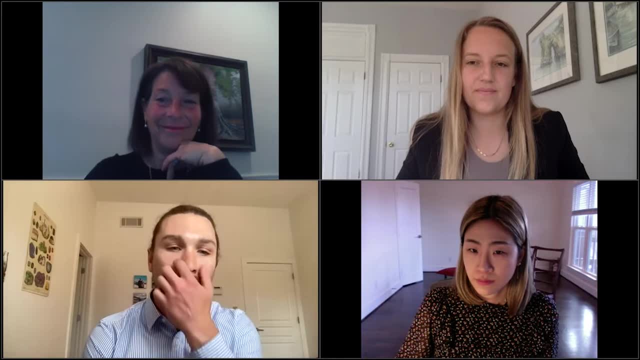 as well as Professor Bragan Vandenberg and Heather Lewicki, who have all become my good friends throughout this arduous but incredibly worthwhile process. We also owe a big thank you to our advisory committee, Vanderbilt Law School and ELI for making this all possible. 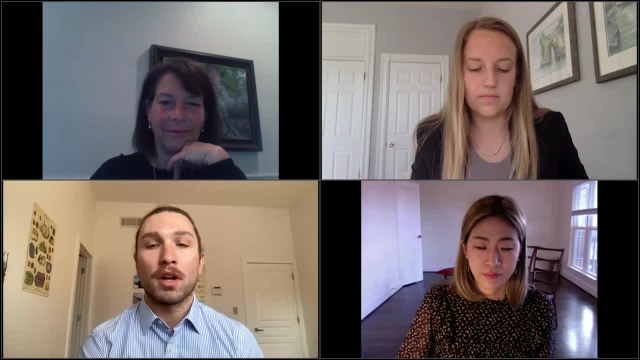 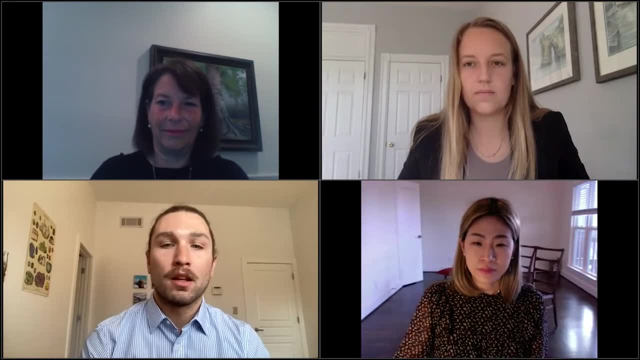 So now I'm going to go ahead and explain LPAR's article selection process, which JE will later get into a little more detail, and how we have gotten to this exciting point that we're at today. So, as the professors indicated, LPAR seeks to publish the best. 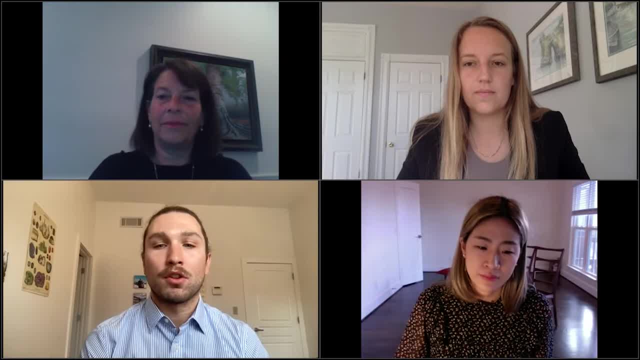 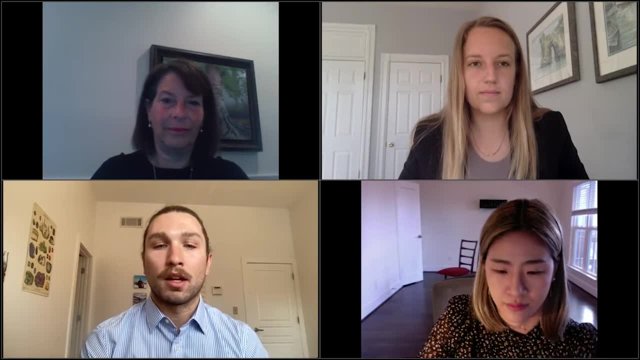 environmental law and policy articles published each year which are addressing pressing environmental issues. LPAR is a joint publication by Vanderbilt Law School and the Environmental Law Institute. There's also a class here at Vanderbilt made up of 20 to 22 law students each. 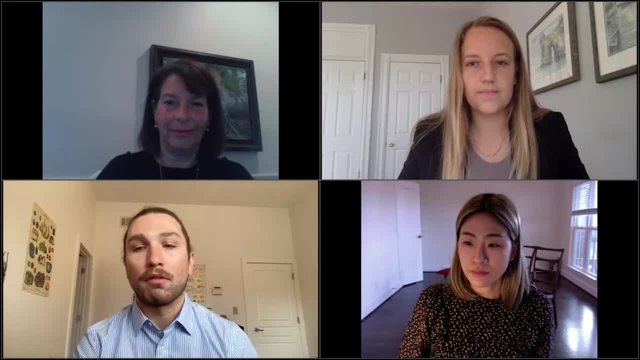 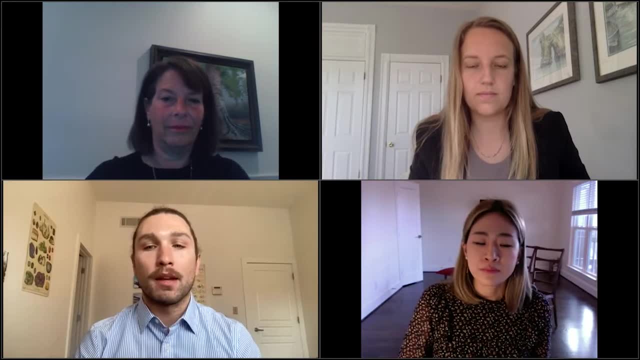 year 2L and 3L members who actually had to participate in a write-on competition to become members. Our selection process for articles follows a series of major steps. We begin by logging every article published in the Law Review of Schools ranked in the US News Top 100, as well as a variety. 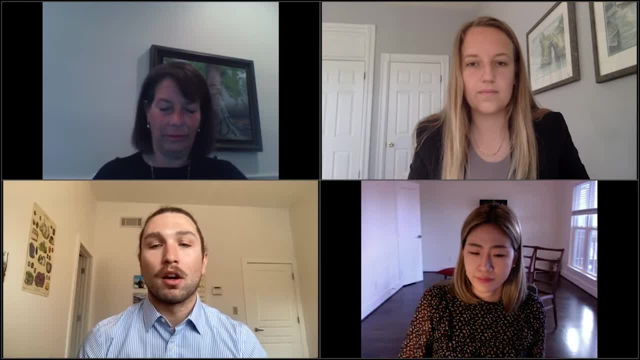 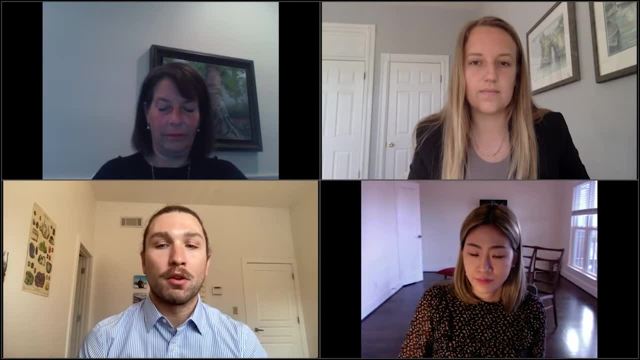 of environmental law-specific journals looking for articles that use the word environment, usually around 500 articles per year. We then screen these articles down to about 150 to 200, which discuss the environment in a meaningful way. We then screen these articles down to about 150 to 200, which discuss the environment in a meaningful way. 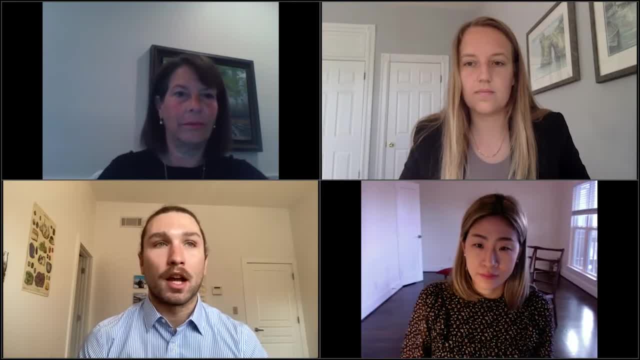 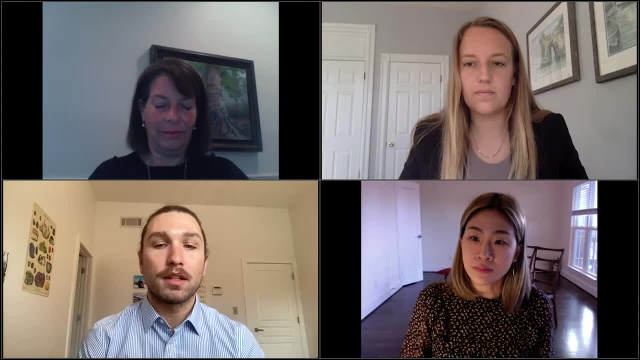 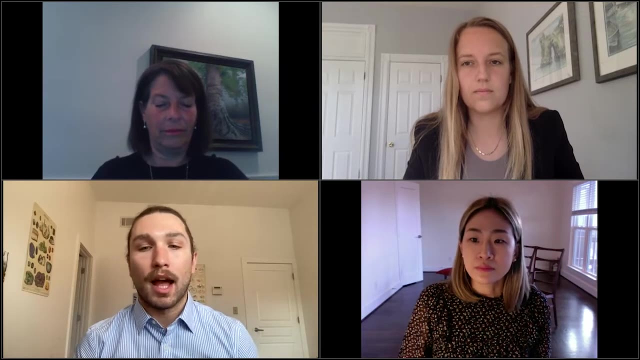 way and relevant within our context, not just like the political environment. After evaluating these articles based on our four major categories of persuasiveness, creativity, impact and feasibility, two students each summarize the articles, which we will then discuss as a class, with the guidance of professors Bregan and Vandenberg. 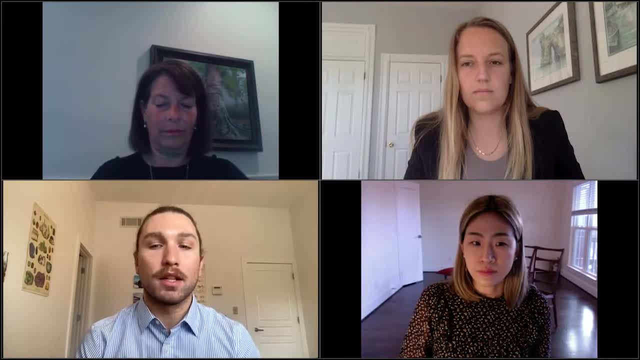 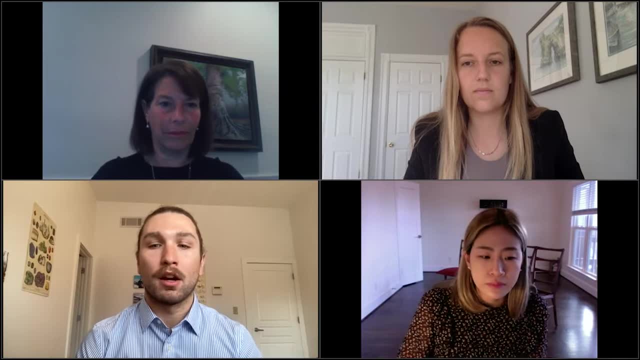 Over the course of two semesters, the students and professors collectively settle on a top 20 list of the most exciting and innovative environmental law and policy articles which we'd like to highlight in our LPAR August edition. With our top 20 selected, we then consult our expert advisory committee. in reaching 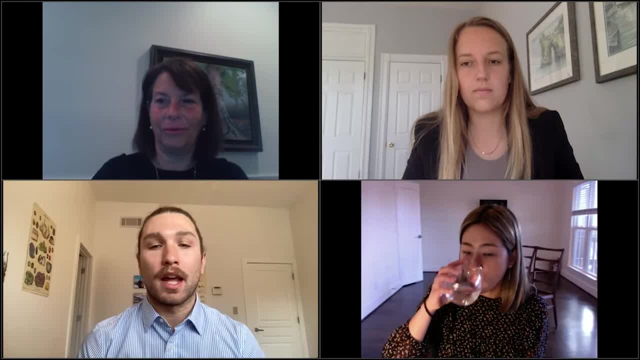 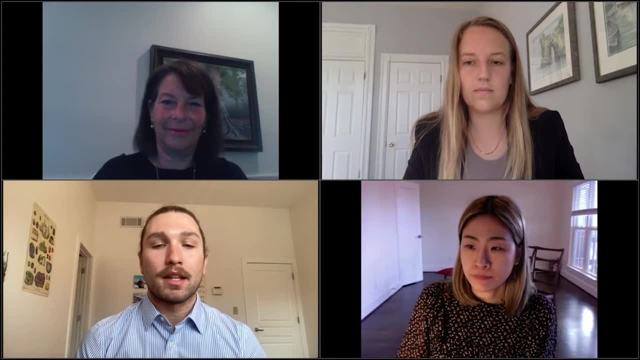 a top three to five, which is published in a condensed version in the August edition of ELR. We also list the top 20 in that edition, each with a big idea sentence that explains the crux of the article and its policy proposal. 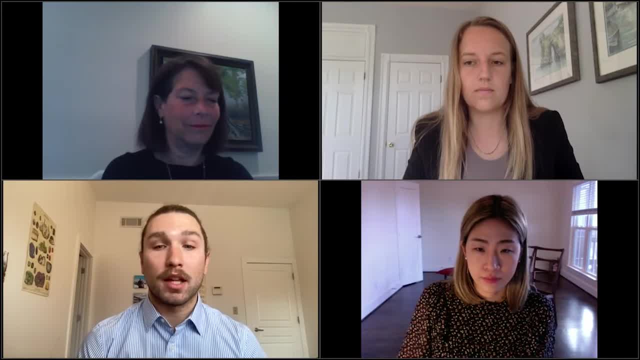 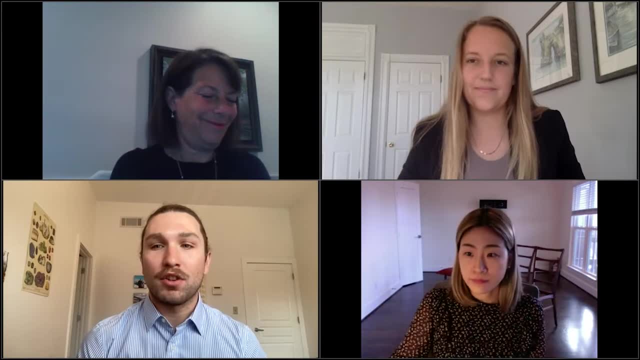 This year we evaluated 172 articles And selected four to include in our publication, three of which will be highlighted in today's conference. Hope you guys enjoy. Let's pass it off to Jaehee. now to get into some of the numbers. 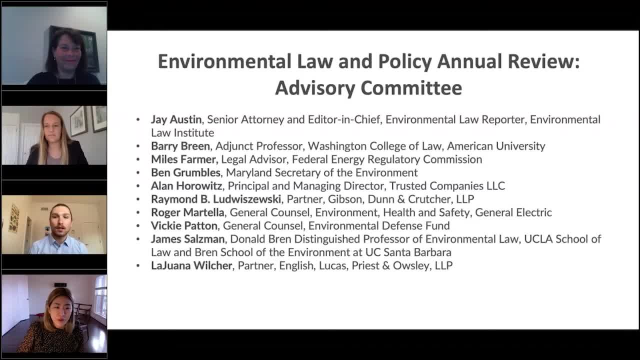 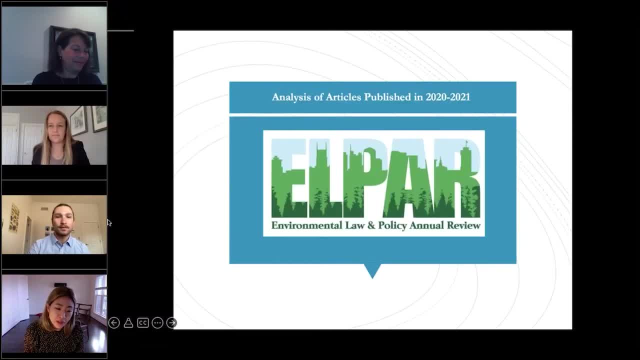 Jaehee Kim. Good morning. My name is Jaehee Kim and I'm a third year law student at Vanderbilt Law School, and I've had the honor of serving as the development editor of LPAR this year. So As part of my role on the journal, I keep track of the data and trends in environmental. 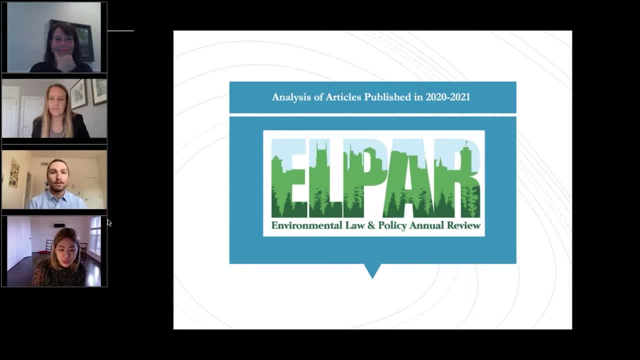 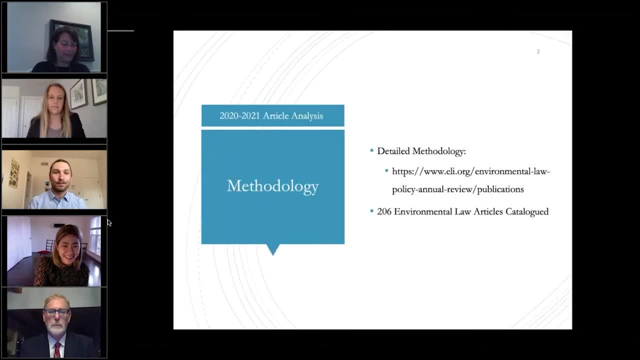 law scholarship. This morning, I'd like to give you a brief snapshot of the environmental publication data we have reported this year. Next slide. So, as Bruce described, we have an established methodology for evaluating environmental articles and collecting data, And if you are more interested in having a detailed look at this process, be sure to 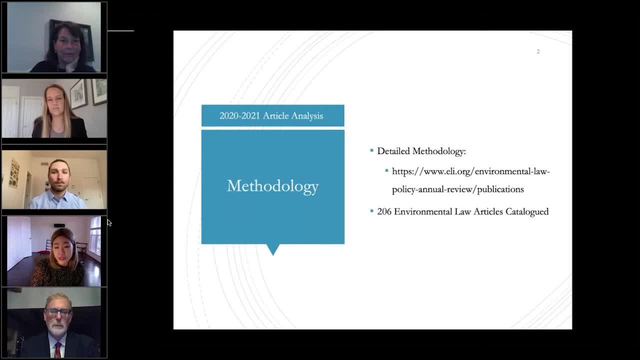 click on that link. The full information on our methodology can be found at this link on the ELI website. So this past year we analyzed 206 environmental law articles. When members read through an article to assess whether it's an environmental article, they 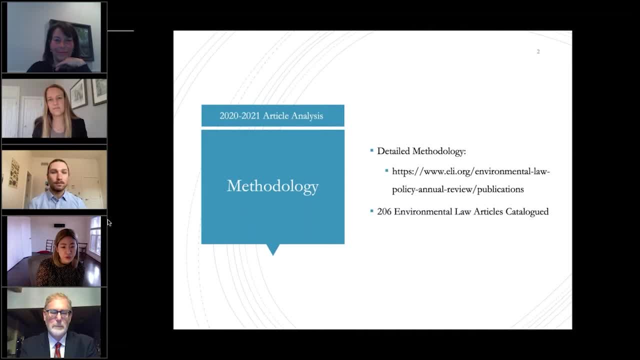 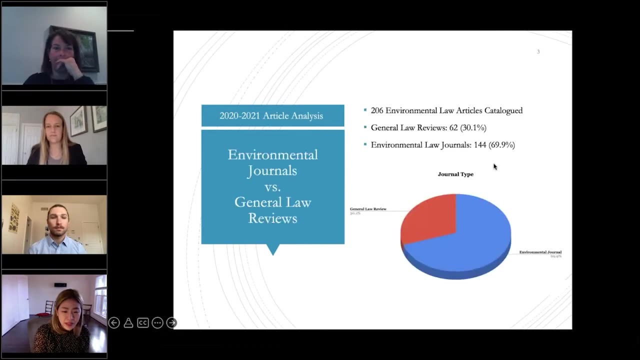 consider whether environmental law and policy are a substantial focus of the article and whether environmental topics were given more than an incidental treatment and were included in the article Next slide. Of these 206 environmental law articles, 62 came from general law reviews and 144 came. 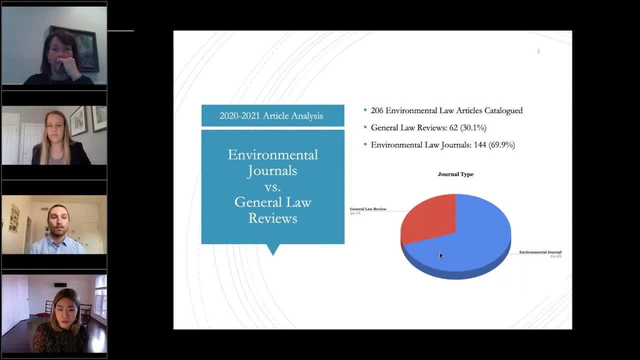 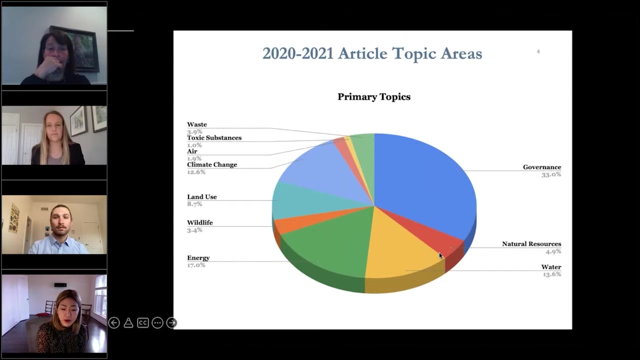 from environmental law journals. We define environmental law journals as US-based specialty journals listed in the environmental and land use law subject area. The most recent rankings compiled by the Washington and Lee University School of Law Next slide. So LCAR members classify all the articles into 10 topic categories, which are set out: 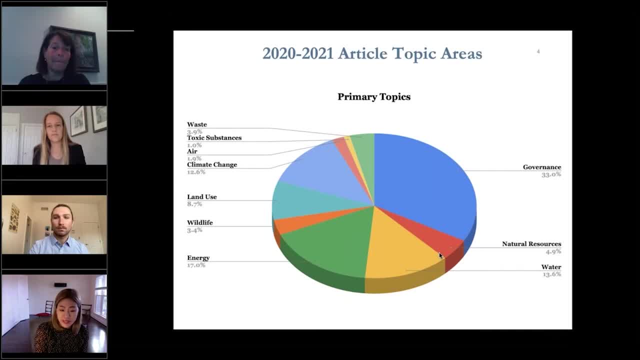 by the Environmental Law Reporter. Subject Matter Index. These topics include air, climate change, energy governance, land use, natural resources, toxic nitrogen and pollution substances, waste water and wildlife. Articles receive a primary topic and also a secondary topic. 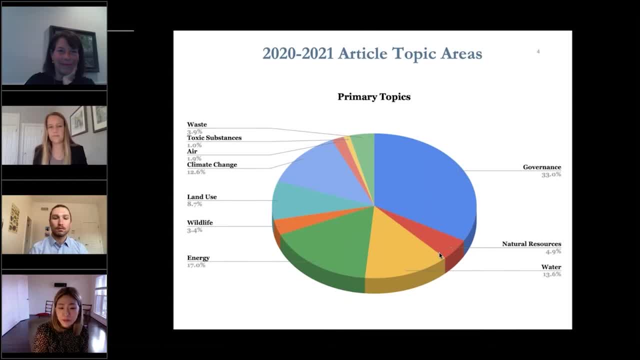 if that's applicable. So the environmental articles published from August 2020 to July 2021 included 68 governance articles, 35 energy articles, 28 water articles, 26 climate change articles, 18 land use articles, 10 natural resource articles, 8 waste articles, 7 wildlife articles. 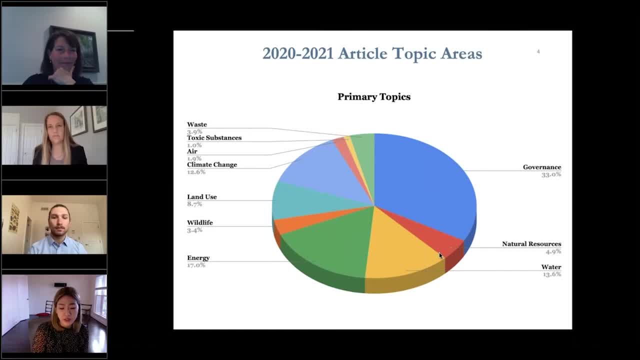 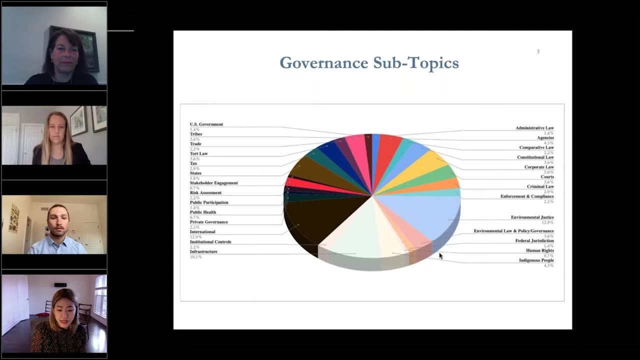 4 air articles and 2 toxic substance articles, And you can see each grouped by percentages in this chart Next slide. We also gathered data about articles subtopics, mainly because the governance category casts a very wide net With 36 different subcategories. So these are all the subtopics per percentage Next slide. 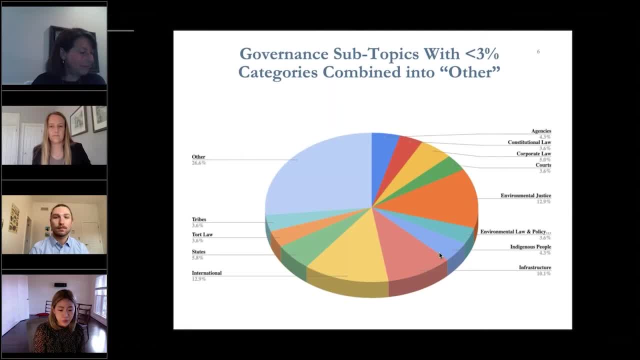 We grouped all of the categories that were under 3% and grouped them into other in this pie chart for ease of understanding. This chart tracks the exact same data, and the most common topics within governance articles were environmental justice tied with international law, and they were followed by infrastructure, then corporate law and state government. 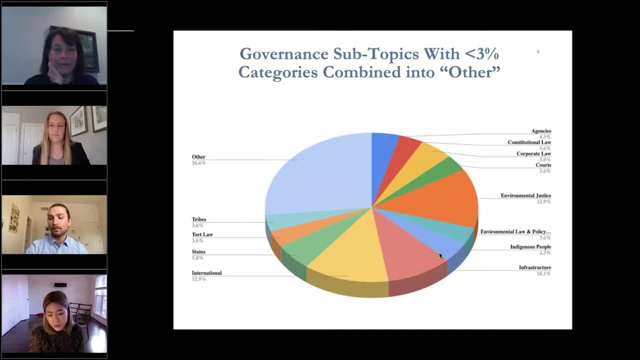 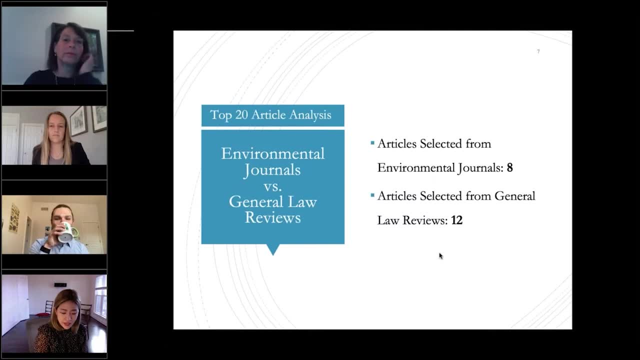 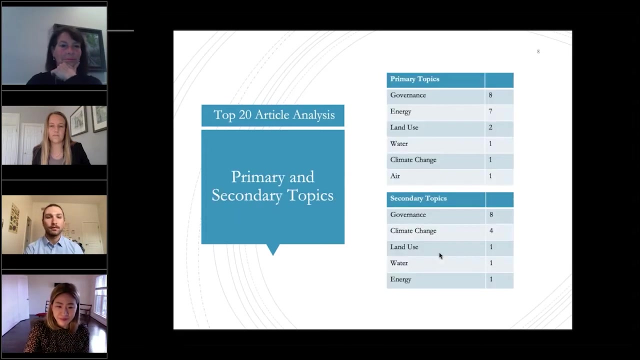 then agencies and indigenous people, both came in sixth place. Next slide: Out of our top 20 articles chosen for 2020 to 2021, eight articles were from environmental journals and 12 were from general law reviews. Next slide: So within the top 20, we had a range of primary topics, with the most common being governance and 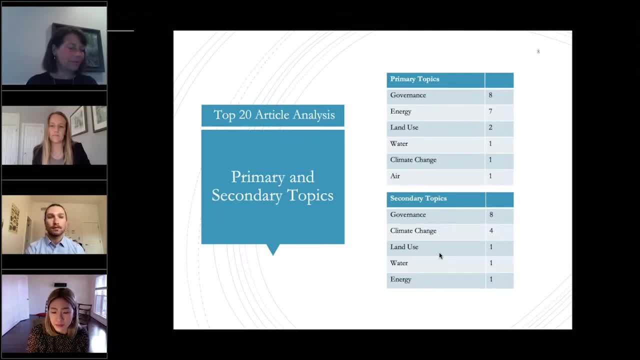 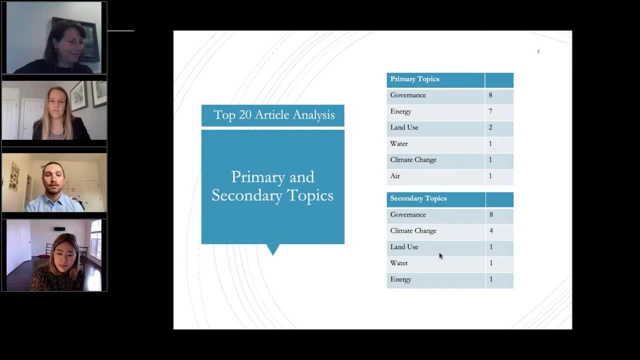 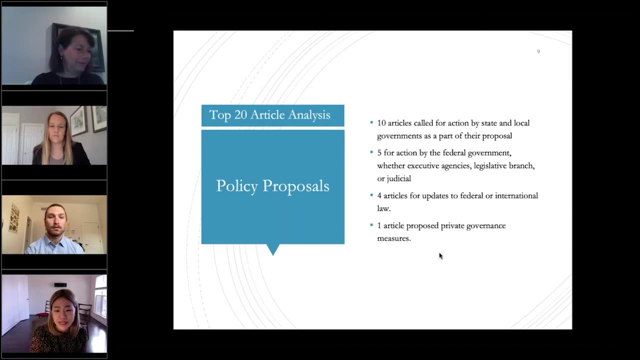 climate change. You can see the secondary topics below, although not every article had a secondary topic. Next slide In our top 20,. 10 articles called for action by state and local governments as part of their proposal and five called for action by either: 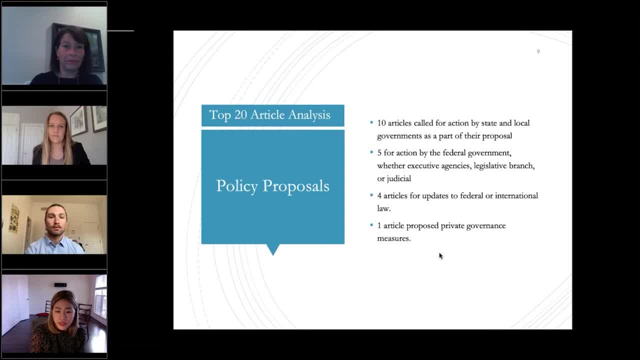 federal executive agencies or judicial actors. Four articles called for updates to federal or international law and one article proposed private governance measures. We had a great pool of articles to choose from this year and we are excited to discuss some of them today, And with that I will hand it back to Linda Great. Thank you, Bruce and Jaehee- Terrific. 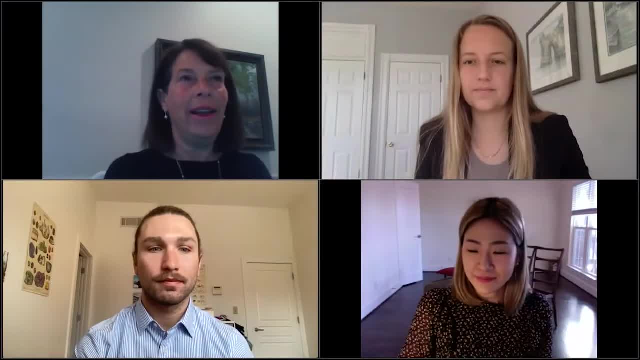 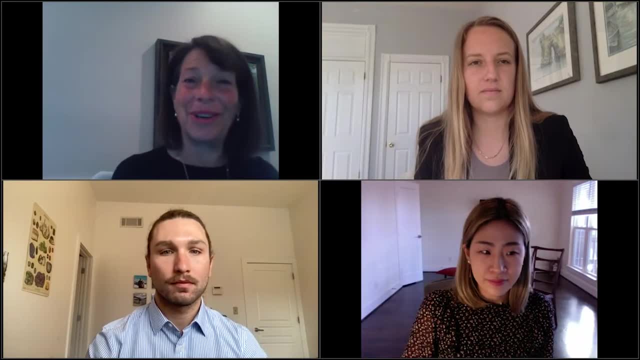 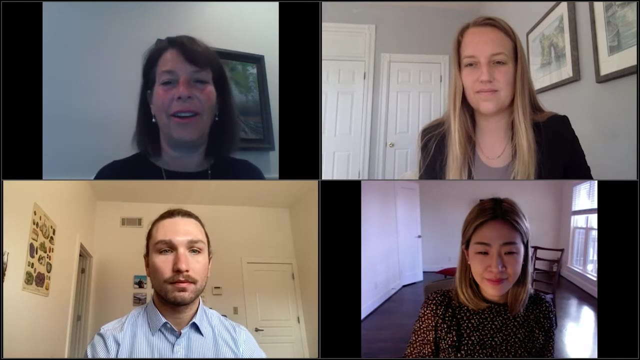 job. I always find it really interesting to see how the topics change over time. As you might imagine, when we started this 14 years ago, we didn't have any climate change articles or energy articles, So it's just interesting to watch how the trends evolve. I want to say a special thank you. 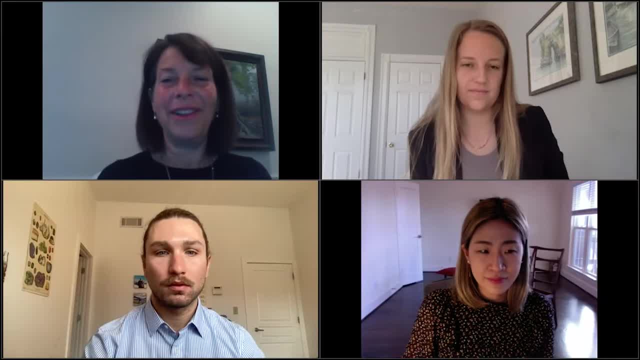 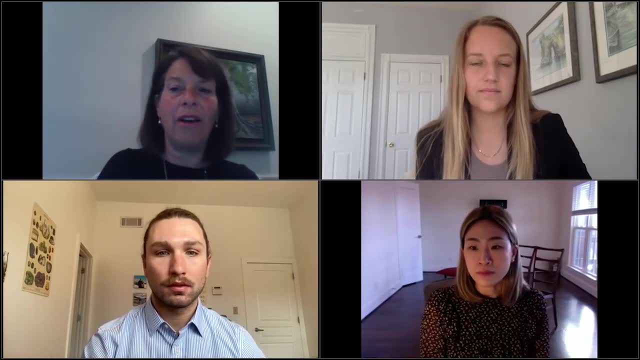 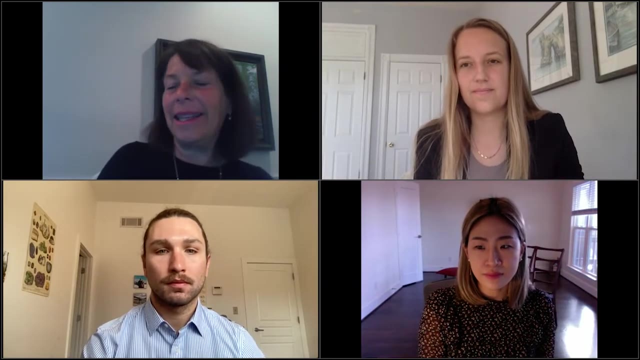 before I forget, to the LPAR students in Nashville who are listening to this today. The class really did a terrific job this year of picking a great group of articles And also I want to thank Heather Ludeke, our All Star Research Associate, for her incredible work on LPAR for the 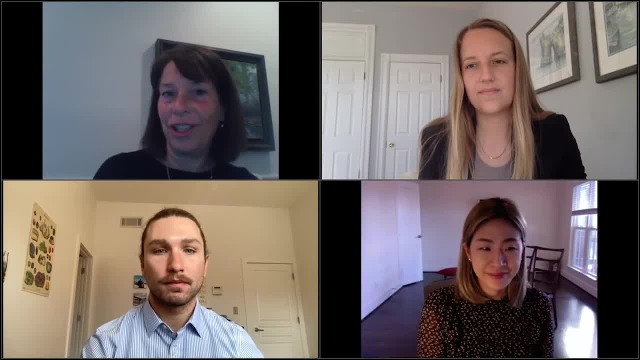 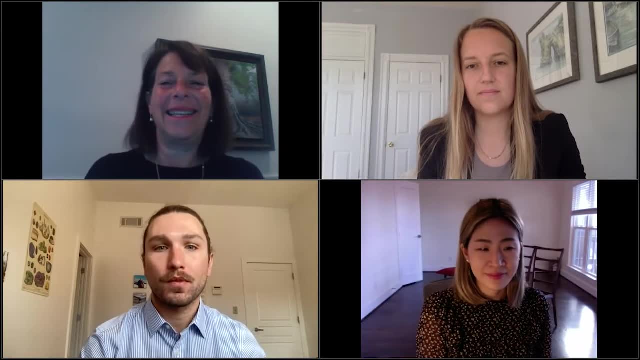 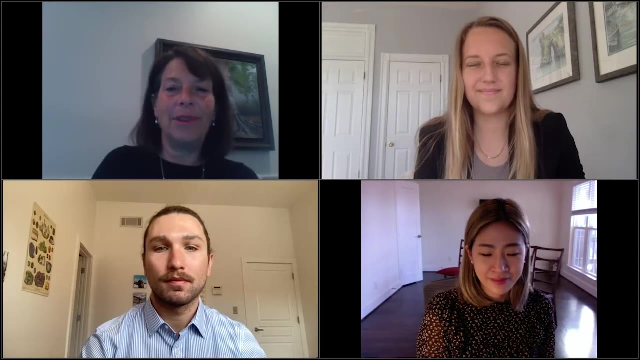 past two years, and Colin Gibson-Tansel, who is managing the technology for us today, As he knows, we could not do this without him, And Victoria Dorward at Vanderbilt, who is just instrumental to our LPAR work. So my job today is to move us along as smoothly. 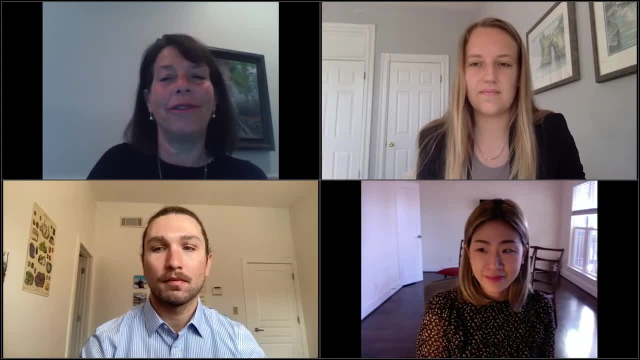 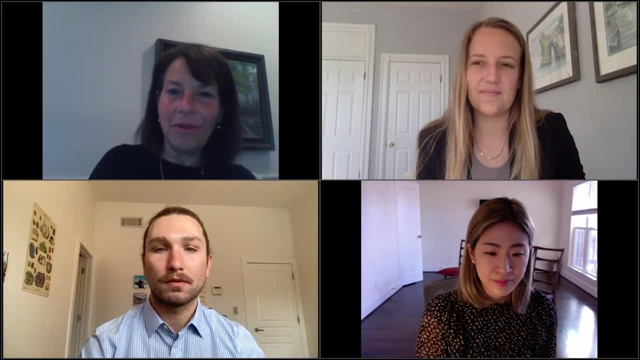 as possible, and also deliberately, so we make sure we aren't talking over each other, which go to the point that Heather does not like, and to try to just keep us running on time. So the way this is going to work is that the Vanderbilt Student Article Editor will introduce the panel and then 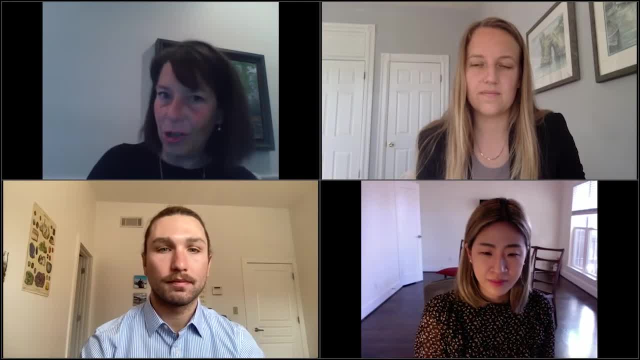 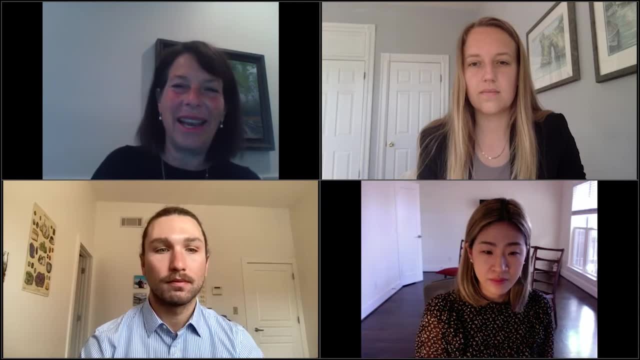 the professor, or professors, will present the article for about 15 minutes, Then each panelist will comment for about 10, and then we'll give the professors a chance to respond to what they've heard from the expert commenters. And that's always, I think, a really interesting aspect of 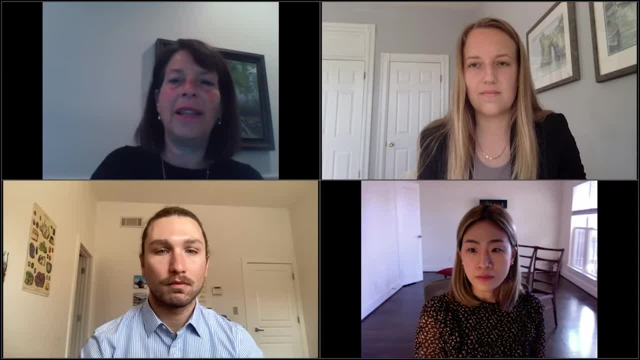 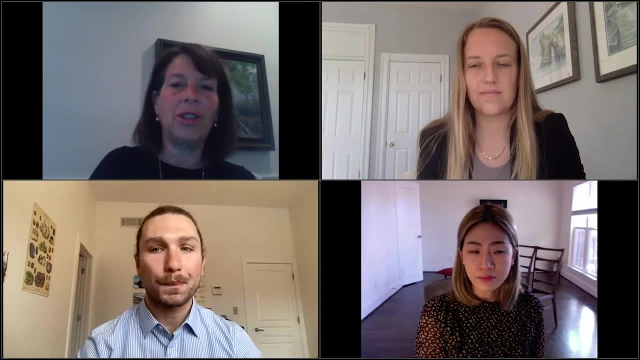 this And then the student editor will kick off the you know Q&A with a question, and then we'll take questions from the audience and continue discussion among the panelists. We strongly encourage you to ask your questions as they arise during the panels. Don't wait till the very end. Use the question box in GoToWebinar. 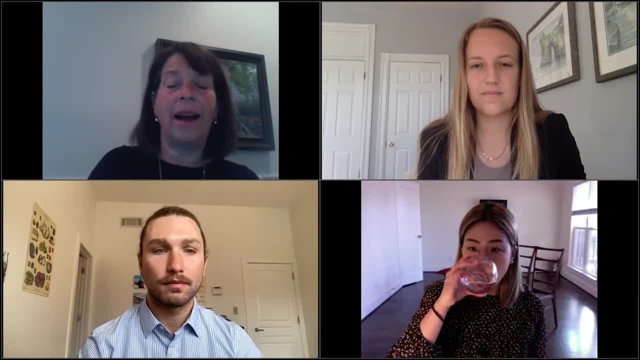 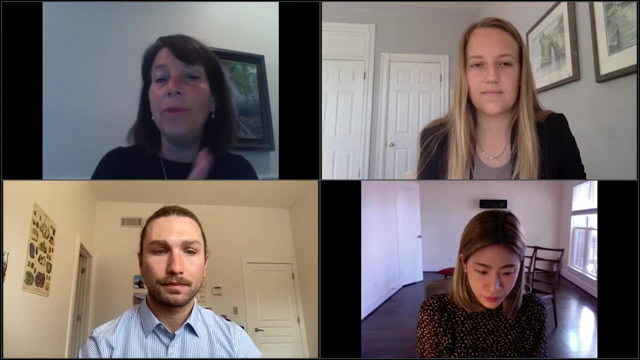 and I'll post as many of your questions as I can during the Q&A section. And just a word about technology and, most importantly, patience. As we change panels we apparently cannot mute the audio, So unfortunately you will hear us testing the tech for each new panel. So if you have any, 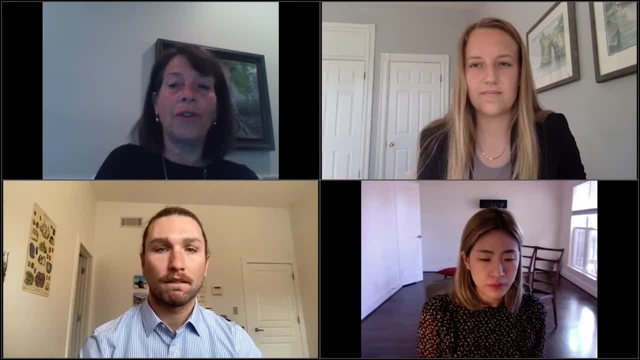 questions, please feel free to put them in the Q&A box And we will be posting them in the Q&A section as well. While the conference is on a 10 minute break, Of course, you're free to come and go throughout the panels today. just to re-enter the webinar, Just use the same link you used this. 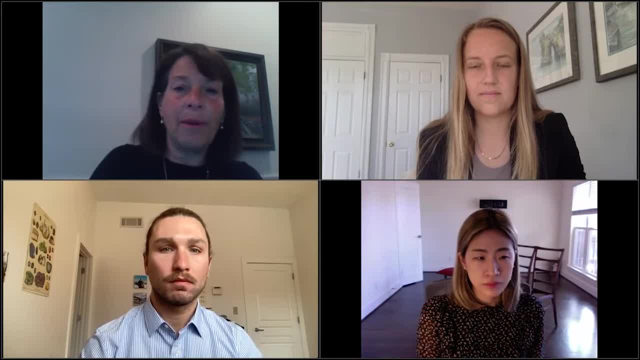 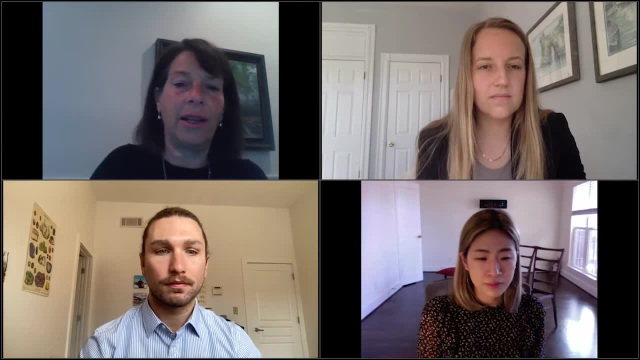 morning and all attendees are muted. If you have any problems or questions, feel free to put them in the GoToWebinar question box. Those will only go to the conference organizers and Heather or Colin can help you out. We always get this question. so I want to say that the slides from 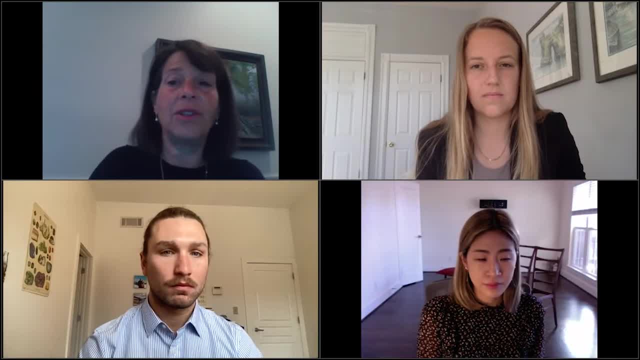 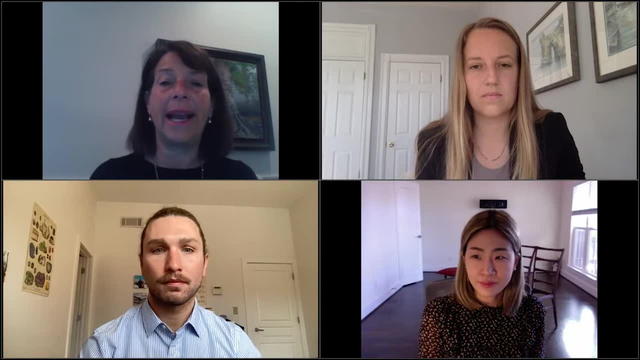 the presentations today, as well as the recording of today's conference, will be posted on the LPAR website after the conference within a few days, as well as the speaker bios. And the schedule for today is available on the ELI events page where you register. But I'll remind everybody as we move. 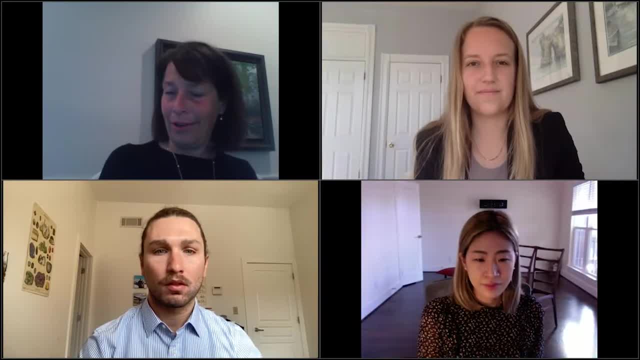 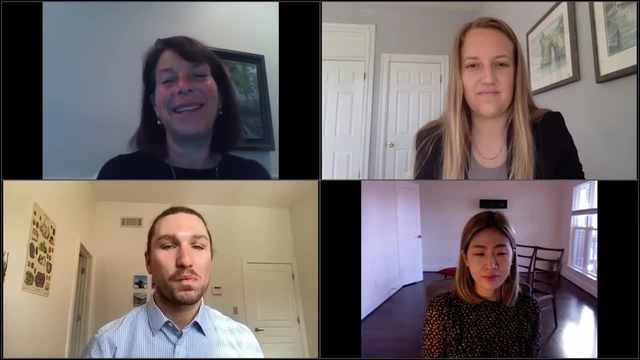 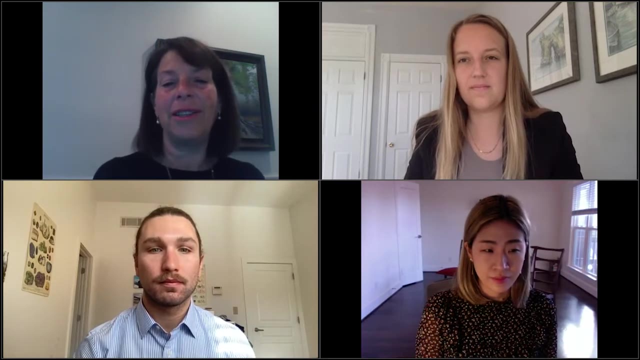 forward. which panel is next? Lastly- and I never used to say this 14 years ago- we will be tweeting during the conference, So please feel free to engage with us on social media. on Twitter it's ELIorg, So I am going to hand it over now to Vanderbilt third-year law student Izzy. 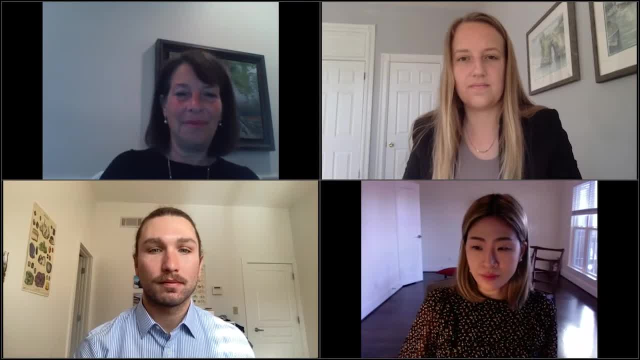 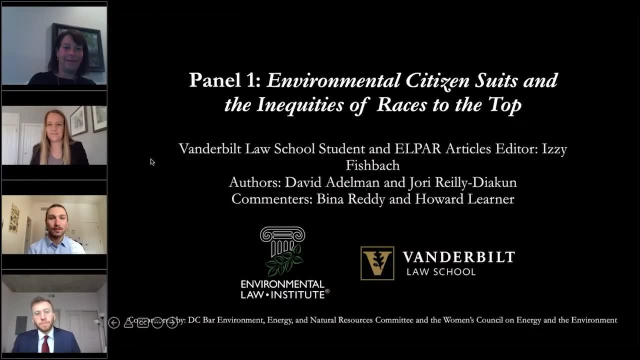 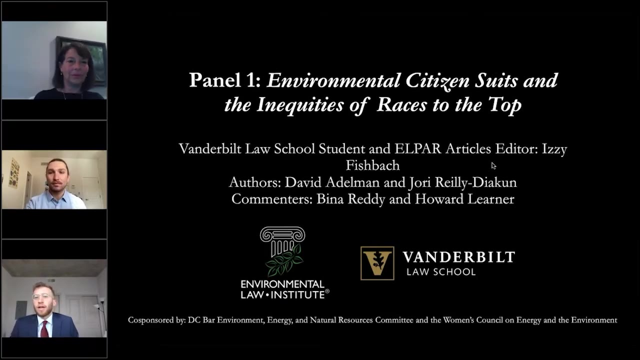 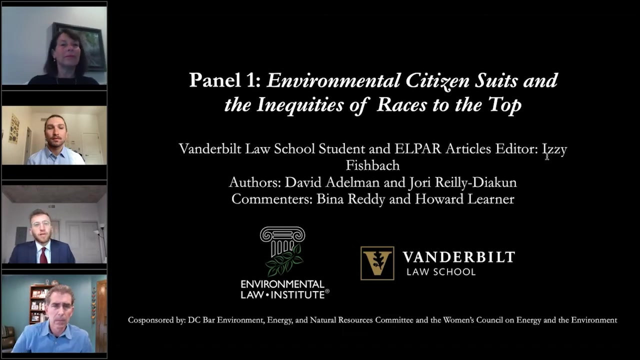 Fischbach to introduce our wonderful first panel, Izzy. Hi everyone, Good morning. My name is Izzy Fischbach, I'm a third-year law student at Vanderbilt Law School and I am the LPAR article editor for our article, which is Environmental Citizensuits and the Inequities of Races to the Top. 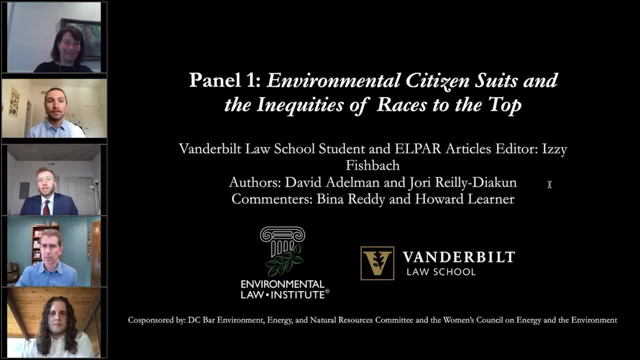 authored by David E Edelman and Jory Riley Dyakun. I'll introduce these authors for you and tell you a little bit about them. David Edelman teaches and writes in the areas of environmental law, intellectual property law and climate change policy. 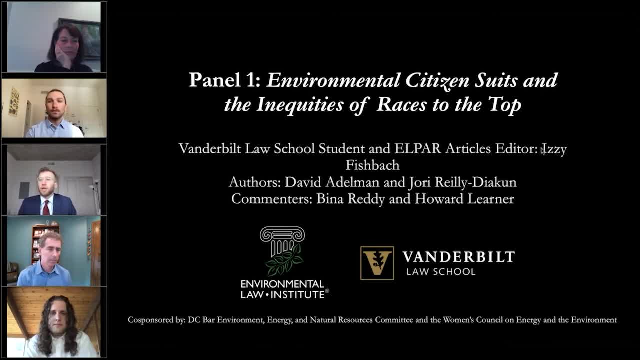 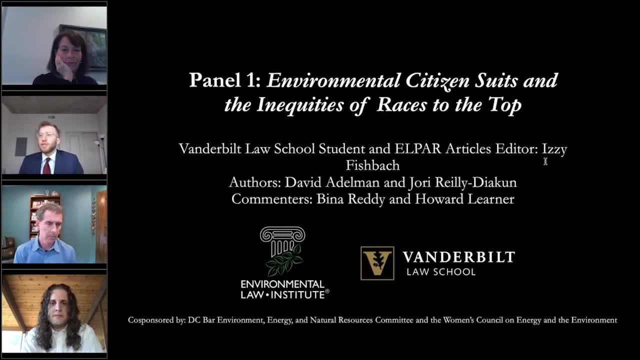 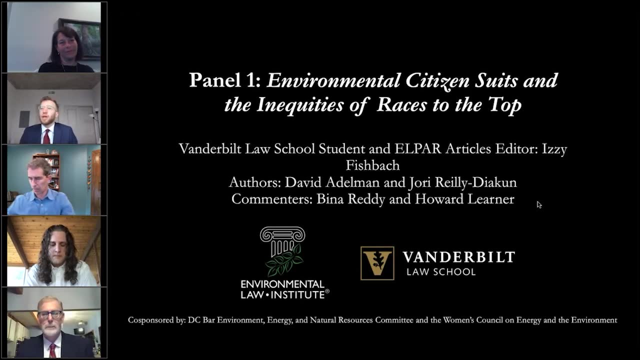 Professor Edelman's research focuses on the many interfaces between law and science. His articles have addressed such topics as the regulatory implications of emerging genomic technologies and the tensions between legal and scientific evidentiary standards. Professor Edelman clerked for the Honorable Samuel Conte of the United States District Court for the Northern District of California. 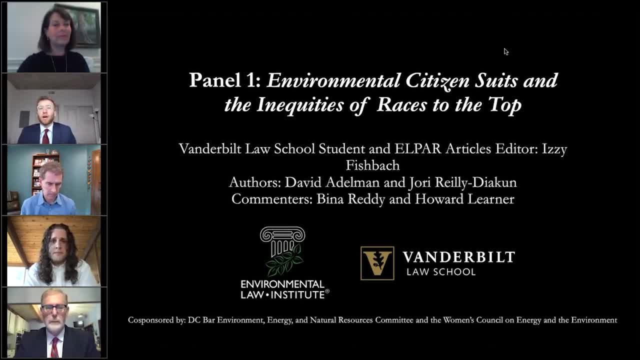 Before entering academia, he was an attorney with the firm Covington & Burling and a senior attorney with the National Resources Defense Council. Prior to joining UT Law, he taught at the University of Arizona Rogers College of Law. Jory Riley Dyakun joined EPA's Office of General Counsel in 2020 as an attorney advisor. 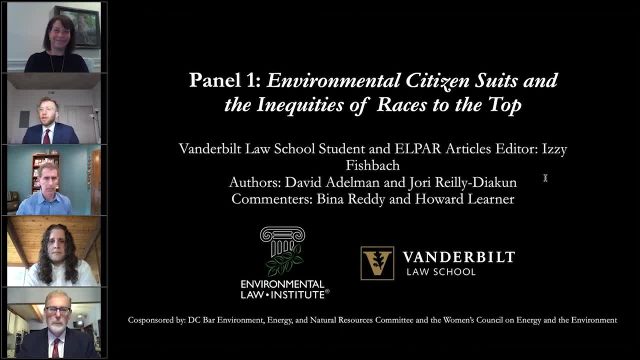 and a senior attorney at the National Resources Defense Council in the Pesticides and Toxic Substances Law Office. Prior to his work at EPA, he worked as a fellow at the University of Texas School of Law. He earned his BS in Physics from the College of William. 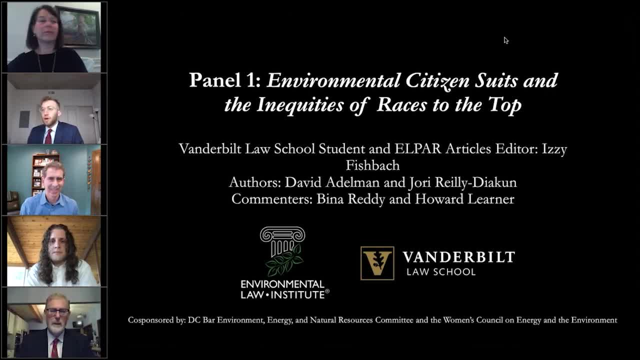 and Mary and his JD from the University of Texas School of Law. We also have two wonderful commenters for you today. Our first commenter is Bina Reddy. Bina is a principal at Beverage and Diamond PC, and Bina co-leads the firm's Toxic Torts and Mass Torts group and has served on the 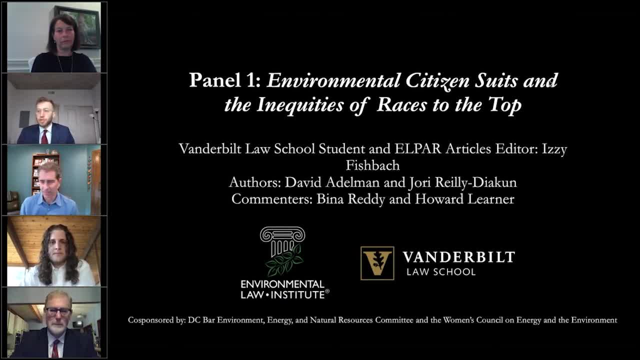 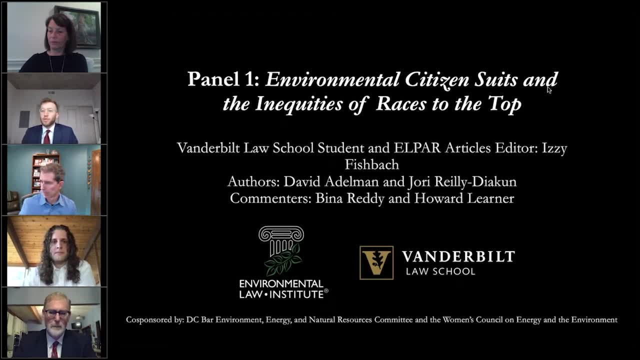 firm's management committee, Bina has devoted a substantial portion of her practice to litigation under federal environmental citizen supervisions. Her experience extends to all major environmental statutes: the Resource Conservation and Recovery Act, Clean Water Act, Clean Air Act and even the 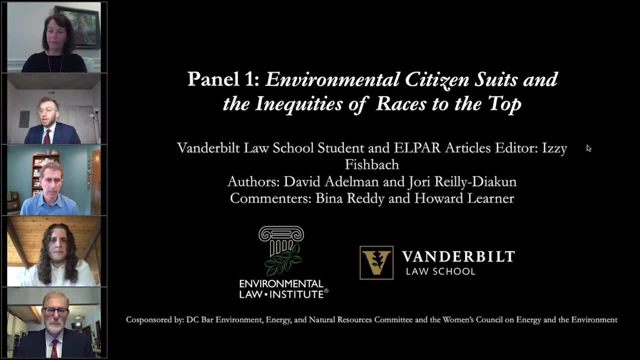 Safe Drinking Water Act. She speaks and publishes on environmental litigation and, in particular, on the subject of novel uses of federal citizen suits. Our other commenter is Howard A Lerner. Howard is an experienced publicist. He is a public interest environmental and energy litigation attorney serving as executive director of the 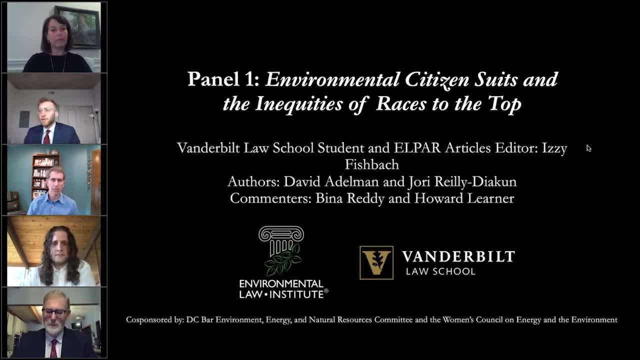 Environmental Law and Policy Center. He is also an adjunct professor at the University of Michigan Law School, teaching advanced seminars on climate change and clean energy law, environmental constitutionalism and sustainable development law. He received his JD from Harvard Law School and 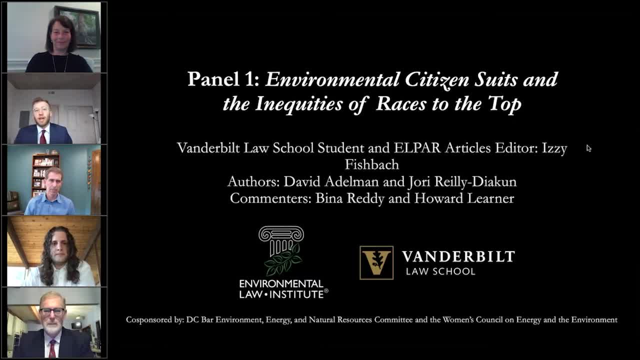 his BA with honors from the University of Michigan And I'll hand it back to Linda. Thank you so much, Bina. Thank you so much. Thank you so much. Professors, over to you to tell us about your article. 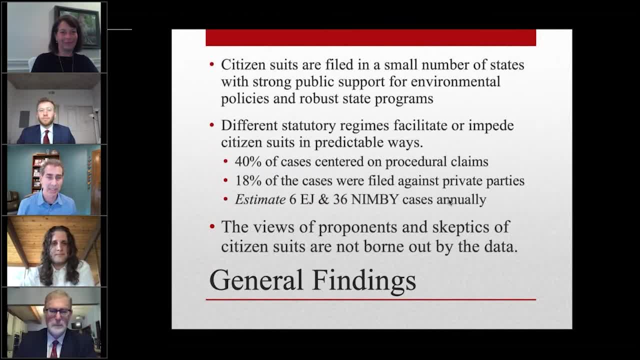 OK, so I'm going to start off. We're going to split the presentation between myself and Jory. I wanted to start off by just thanking everyone associated with the Environmental Law and Policy Annual Review. I have even a greater appreciation for all of the work that goes into that. 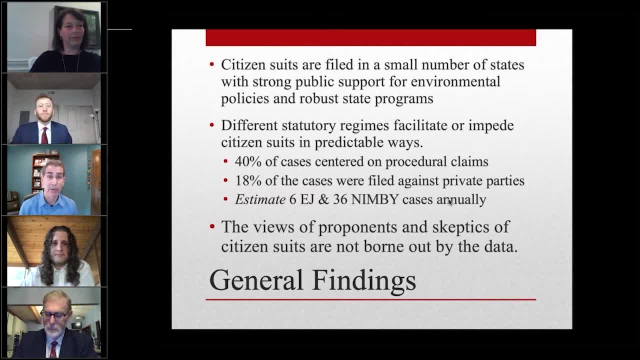 And really we are both grateful to you, Thank you. Thank you, We're so grateful for being selected, having our paper selected this year. I also want to thank Jory. It was a real pleasure working with him, both as a student and after he graduated from UT Law. 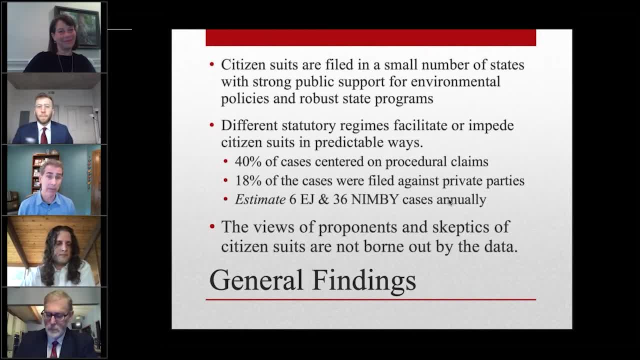 And, like I said, we're going to split things up. I'm going to talk about, or provide just a general overview of our principal findings in the study, and Jory is going to talk about the implications and some of our recommendations. So what I want to do is start off with 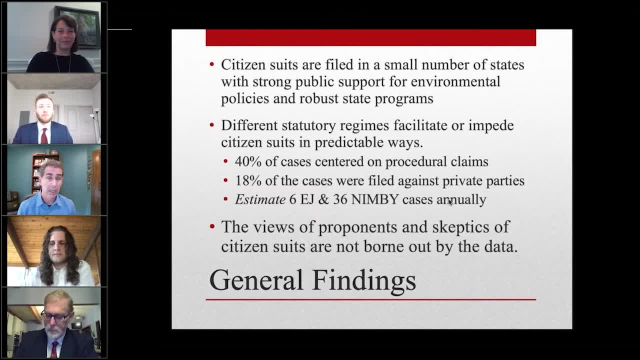 OK, kind of three principal observations At the highest level. what we find is the number of citizen suits filed in a given year is relatively small and that the suits are not evenly distributed geographically around the country. They tend to be principally filed in states where 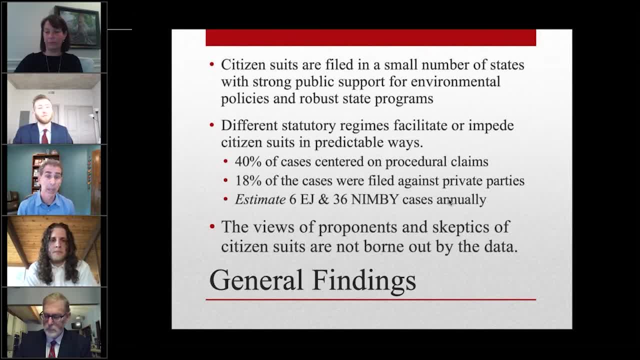 there's strong public support for environmental protection, and state programs are relatively strong. Another point to keep in mind is roughly 50% of the cases are petitions for review and an additional 28% of the cases have the federal government as a defendant in those cases. 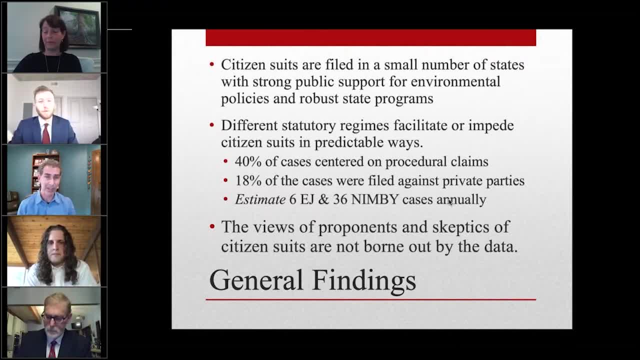 So we've got this distribution of cases that's really uneven geographically, and we've got a heavy emphasis on cases that involve the federal government as opposed to private parties. The other thing that we observe is significant differences across the different environmental statutes, particularly with regard to the balance of petitions for 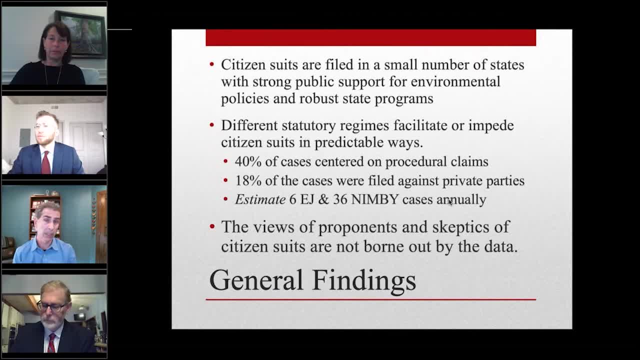 review what we refer to as wholesale litigation versus litigation involving specific federal actions or specific facilities. With regard to the claims, about 40% of the cases center on procedural claims and only about 18% of the cases involve cases against private parties. 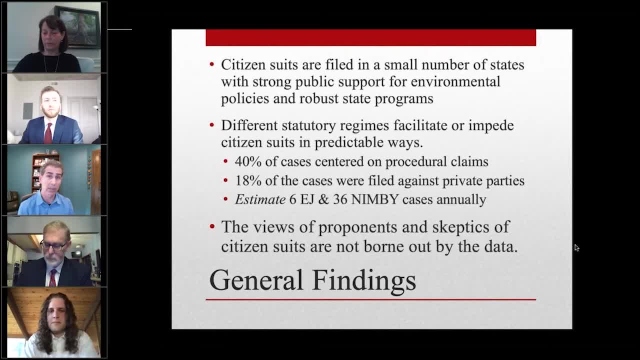 This is particularly important because, as I said, the federal government has a lot of controversy around this type of case and the potential for that to distort or impact federal or state implementation of environmental statutes And a lot of the debate around citizen suits is. 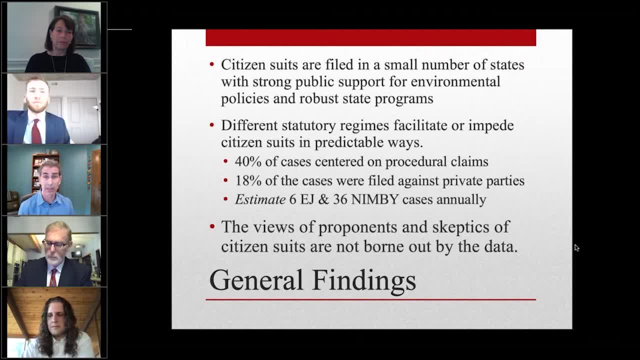 centered on this type of case, and yet it's a relatively minor or small number of cases on an annual basis. One of the things we want to talk about is the importance of the federal government in advice as a team andil particular planning, as well as I would say section 1, the merta of this. 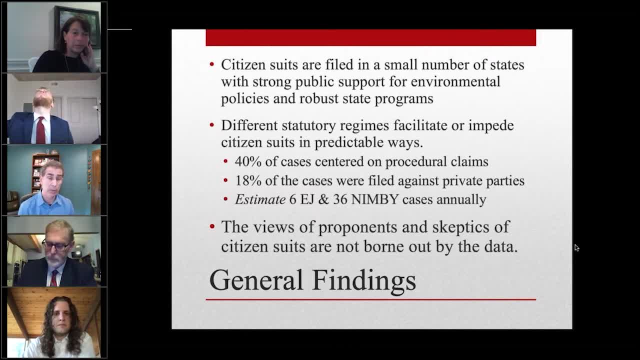 bill Under the federal administration of the vinyl interpretations and the experimental spacecraft assessment process. another important issue is that a number of environmental justice cases include provaive Verbavir. As I said, we potently overlooked a number of environmental issues, notGoodρέca taxes, qua as important for these matters. Now The second thing that I wanted to. look at was specific classes of cases, in part because of their significance, are important. So what we want to do was identified a number of environmental justice cases filed each year and the number of NIMBY cases filed each year. This was something that's not easy to do, both because of the limitations of the 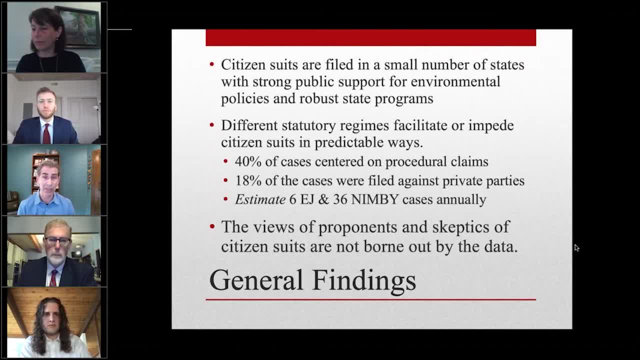 numbers and say that they're subject to significant error, bars or uncertainties, and we've just done the best we can with time and resources we had and the data we had available to us. But in either case, we find that there's a really small number of environmental justice. 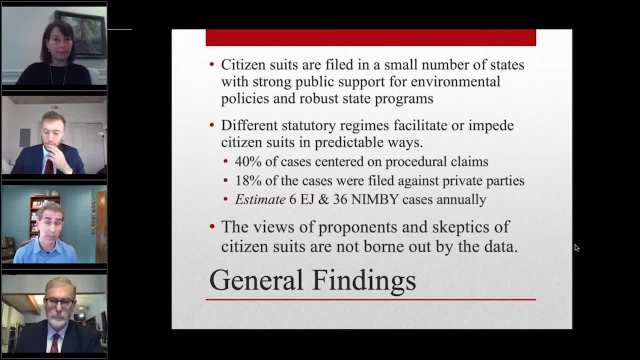 cases filed in a given year and a relatively small number of NIMBY cases are filed in a given year, And even if our numbers are off substantially, even by like a factor of two, I think the numbers are relatively small, suggesting that we could certainly be doing a lot more. 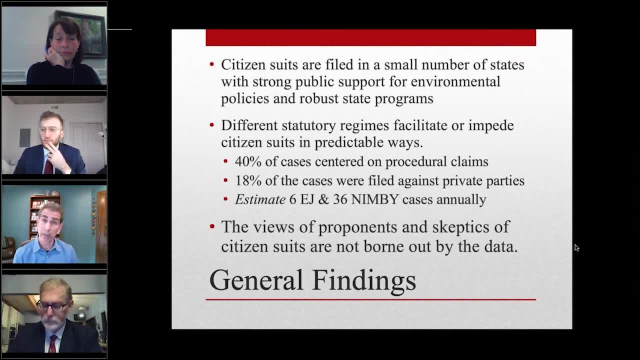 with regard to the EJ cases and also suggesting that, despite the fact that there are a number of really high-profile cases that are sometimes characterized as NIMBY, that's not really representative of the bulk of the cases out there. The third point I want to start with is our data, when you look at them kind of collectively. 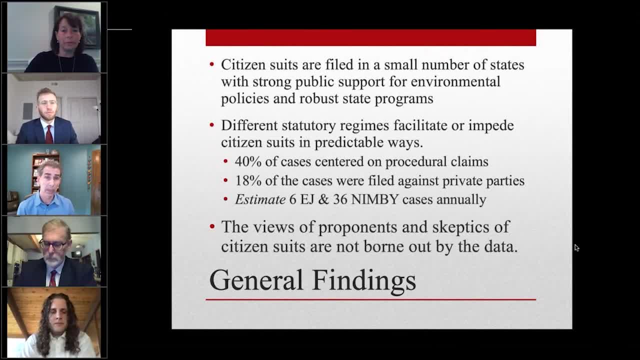 are inconsistent with the sort of conventional views- Pro and bad. That's something that we're really concerned about, And so I would ask our audience to think about that and to think about the context of that and the impact on the data, For example, if the data shows that a government isn't doing the right thing we want to do. 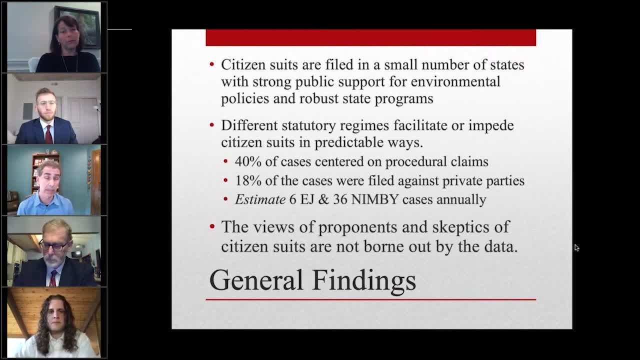 the right thing. But if the data shows that an individual has not done the right thing, it means that the government is not doing the right thing. And if the data shows that you know the individual needs to be protected from things that are not protected, then that means the government is doing something that's really. 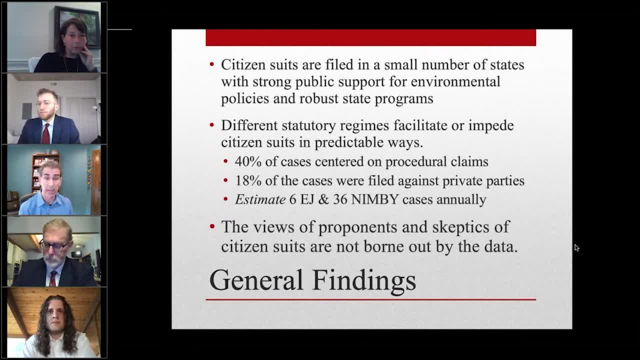 for implementing them, and again, we don't see evidence of that either, and so one of the central things we hope will come out of this case is the importance of understanding how citizen suits operate in practice and therefore how we should be thinking about them. see if I can access good, so this first slide is: 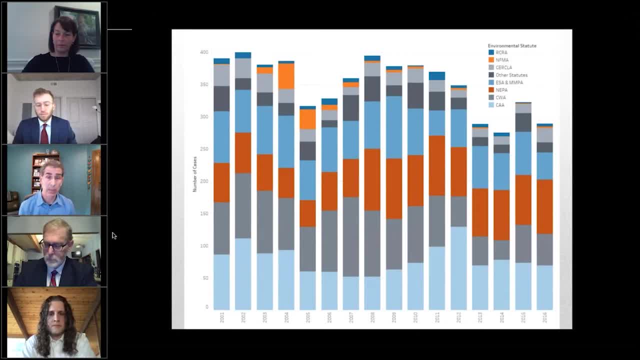 really looking at the aggregate data. we're looking at the number of cases per year. it's broken down by statute. what we see is roughly 80% of the cases are filed under the Clean Air Act, Clean Water Act, NEPA, ESA and MMP a each of. 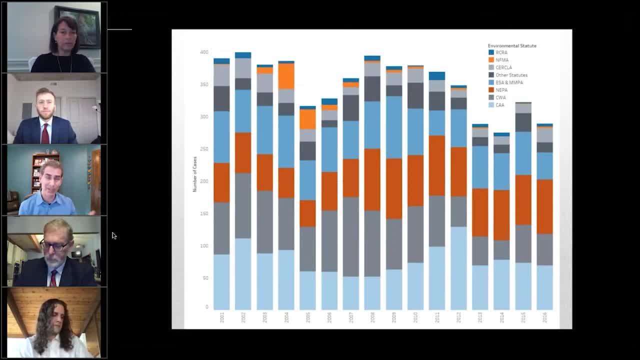 those types of cases or those cases filed under each of those statutes makes up roughly 20% of the cases filed in a given year. overall, the number of cases filed in years about 350 plus or minus 50. it's been pretty stable, although in the last few years there's still a lot of cases filed under the Clean Air Act. 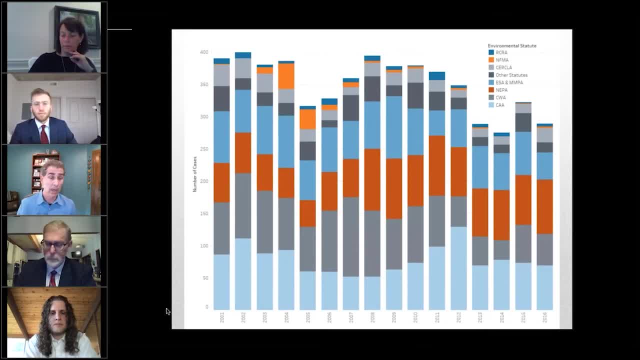 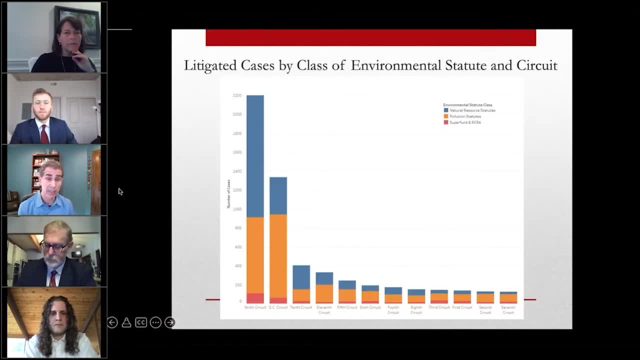 Clean Water Act and the 13th is really down, which is a great example for some indication that the number of clean water act cases was diminishing. one of the most striking findings we have is the geographic distribution of cases. so this is looking at the number of cases by circuit and it's broken down just to 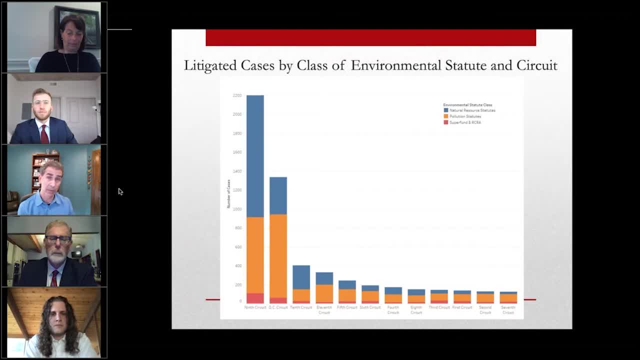 make this, you know, more easy to interpret by the natural resource cases, cases filed on the pollution statutes and cases style filed under super fund and RCRA. we might expect there to be a large cases in the DC circuit, both because most of the federal agencies are based in Washington DC. 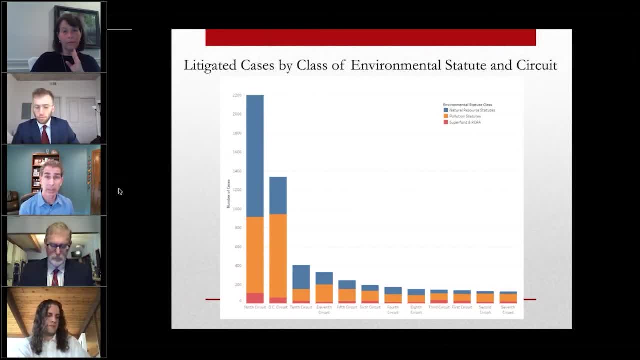 and because of the unique status of the DC circuit itself, particularly with regard to Clean Air Act cases. You also might expect there to be a significant number of cases in the Ninth Circuit, particularly because about 60% of public lands are located in the states that are. 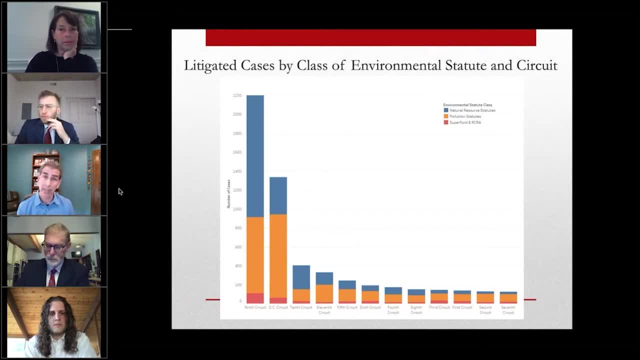 encompassed by the Ninth Circuit. But we even think, taking that into account, the number of natural resource cases is pretty striking. even with that factored into your analysis- and we'll sort of illustrate why a little bit more rigorously later on. But particularly with regard 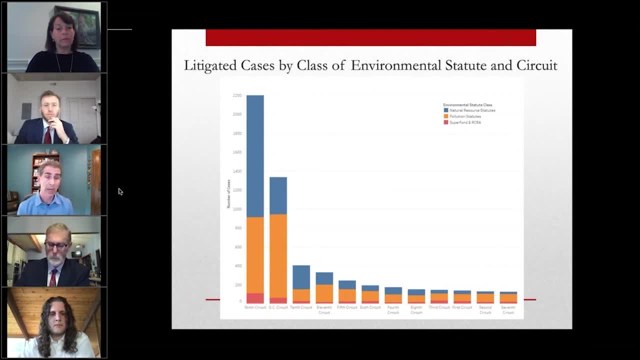 to the cases under the pollution statutes. it's actually surprising to see so many in the Ninth Circuit, both because a number of the states have relatively low population, low urbanization and relatively low industrialization, especially relative to states like Texas or Louisiana. 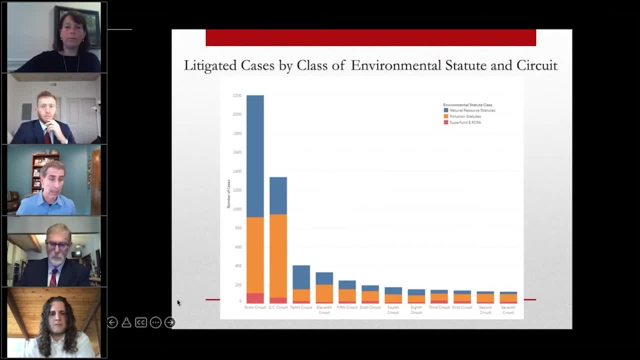 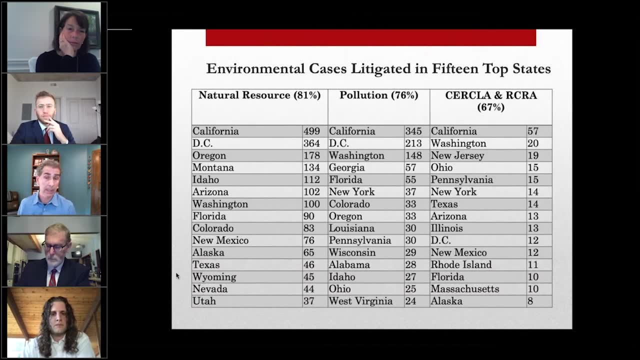 So we see this kind of geographic imbalance in the distribution of cases. We see that same geographic skew mirrored at the state level. so California kind of exists in a category all to itself. If we look at the natural resource law cases, we see this interesting. 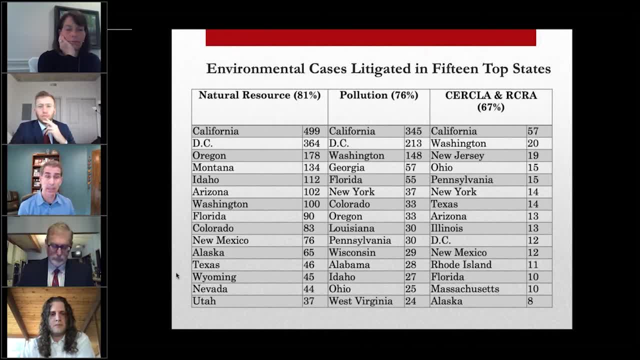 divergence between states like Oregon, Montana and Idaho in the Ninth Circuit versus states like Colorado and New Mexico In the Tenth Circuit, in terms of the relative number of cases, which again is suggesting that the cases aren't simply tracking, for example, the amount of federal land in a particular state. 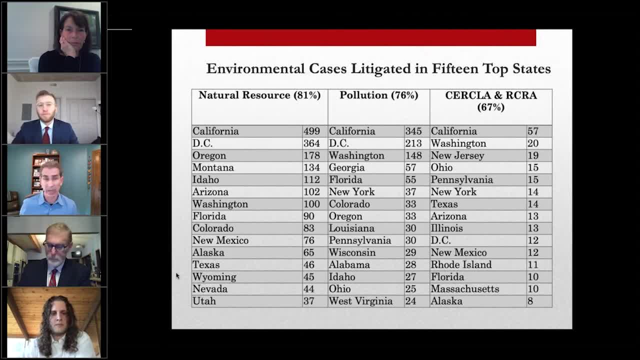 that there's form issues that seem to be an important factor with regard to where cases are filed, With regard to the pollution statutes. a state like Washington, which is so dominant, relative again to states like Texas or Louisiana, I think, is also a 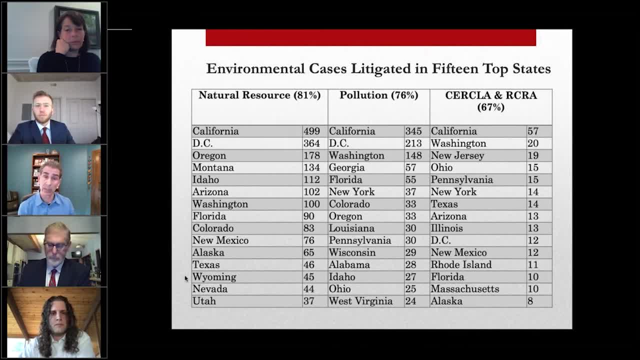 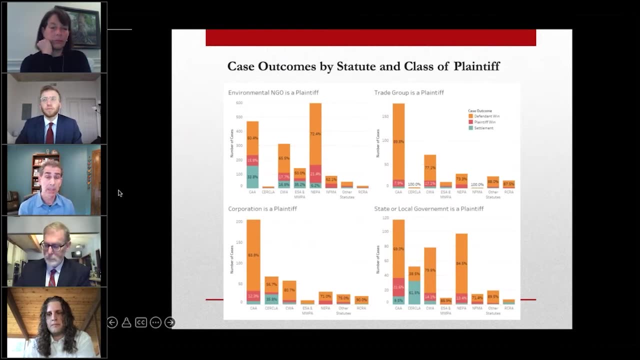 really striking and suggesting that numbers or maybe concerns about implementation of environmental statutes isn't really the driver with regard to where cases are filed. When we look at case outcomes, this is looking at how the rates at which different classes of plaintiffs prevail in environmental lawsuits, So the percent in which defendants win. 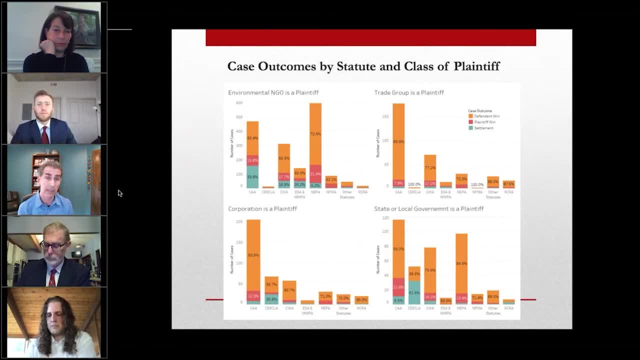 the percent in which plaintiffs win, the percent in which we have settlements by different classes of plaintiffs, so environmental trade groups, corporations, state and local governments. And there are really just two observations I want to make here. The first is that we find 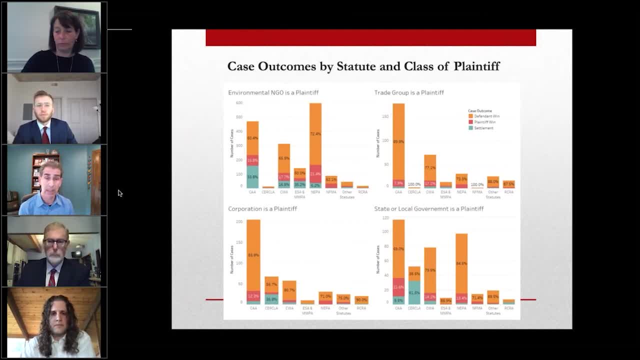 that environmental organizations prevail consistently at higher rates than the other classes of plaintiffs. And the second thing is that we see quite a significant difference in the rates at which plaintiffs prevail across the different statutes. So, for example, with the environmental NGOs, they prevail at substantially lower rates in cases under the National Environmental 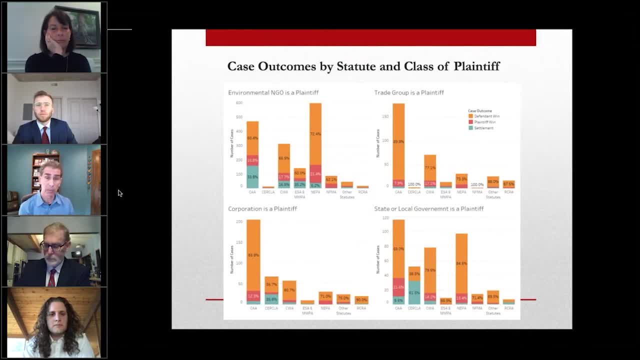 Policy Act, They still prevail at rates that are comparable to or greater than those of the other classes of plaintiffs, and so one thing that comes out of this is we find the data, or at least suggestive of that, environmental groups are at least as selective or more selective than the other classes. 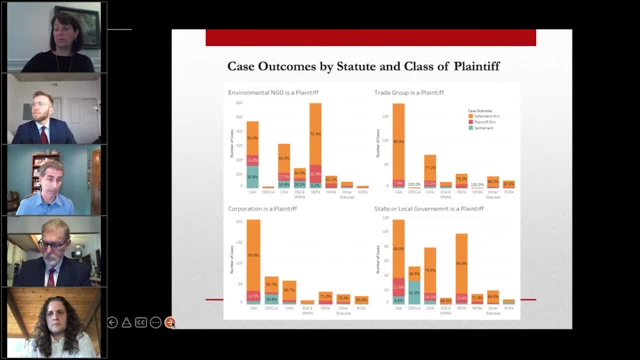 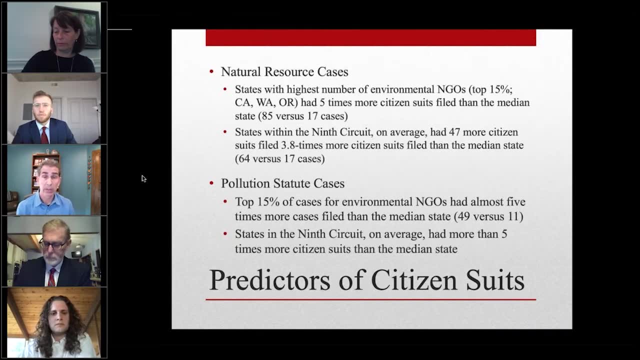 of plaintiffs, And that's really important to see, because the more you look at the data you see, the more you're going to see that the rates are less, less, less selective. So when we look at the rates at which plaintiffs are at a lower rate, the more we see that the rates are less selective. 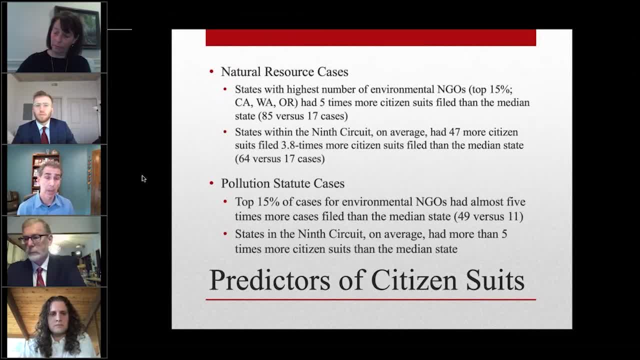 then, the more we see that they are at higher rates, more likely to prevail in terms of the other classes of plaintiffs. So we want to try to make sure that the rates are at a higher rate and that the rates are more selective. So that's the first thing that we want to do in this case. 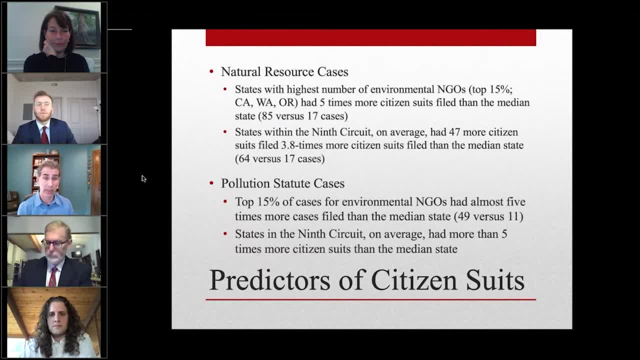 So, again, this is just a little bit of a summary of what we have seen so far. as the regard to the amount of federal land in the state and with regard to the pollution statutes, with regard to the number of permanent facilities, We basically see two explanatory variables dominating our regression analysis. 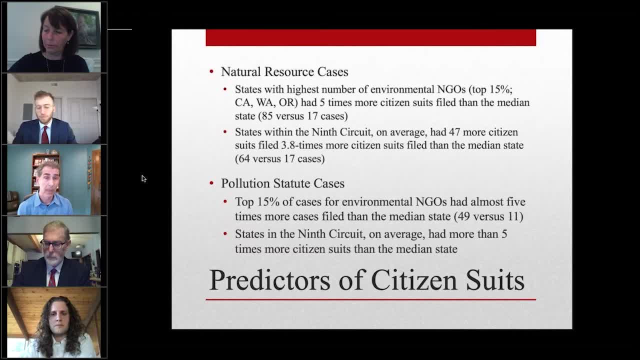 The first is the number of environmental NGOs in the states, And although this is a crude proxy, we view it as indicative at least of the public support for environmental protection in a state. And the second is whether a state falls within the Ninth Circuit or not. 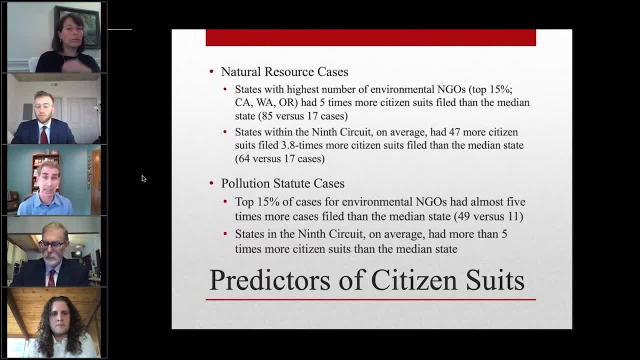 And sort of tracking the patterns in the descriptive statistics that we've already observed In both cases, and for both natural resource cases and pollution cases, we find them as really powerful predictors of where cases are going to be filed, And so what we're finding is where there's strong support for environmental protection. 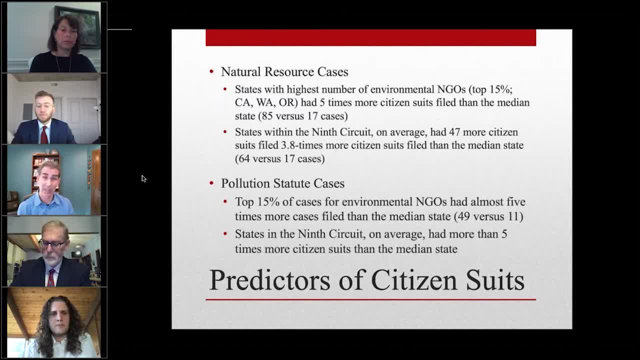 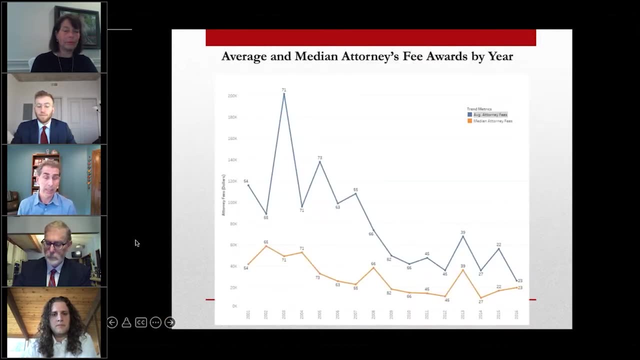 cases are being filed there, Where a state is in the Ninth Circuit, which seems to be suggesting. a significant factor in where a case is filed is the forum It's driving where cases are located geographically across the country. The last thing I'm going to talk about, really briefly, is attorney fee awards. 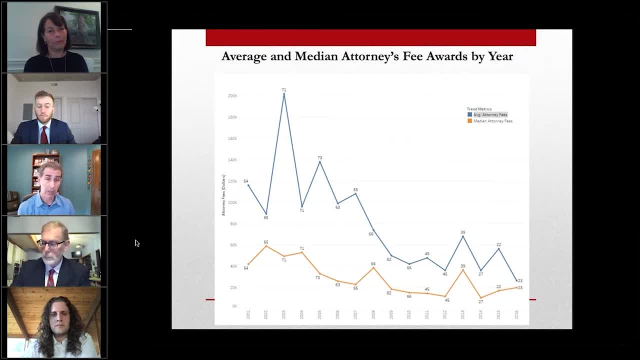 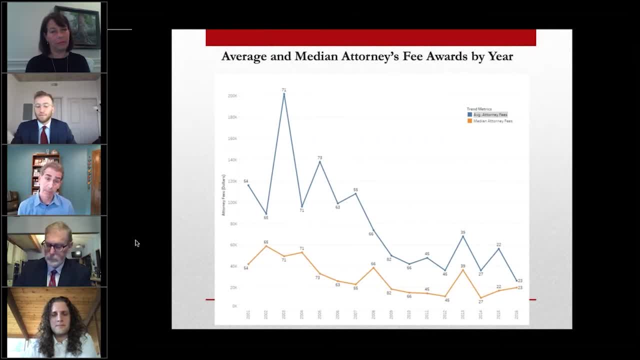 The relative general trends are what matter most here, And so what we observe is, in terms of absolute amounts, attorneys' fees granted are relatively modest. Probably the median is the most important statistical variable here, given the skew in the data. so maybe $40,000 or $50,000 in attorneys' fees early on, but that's also. 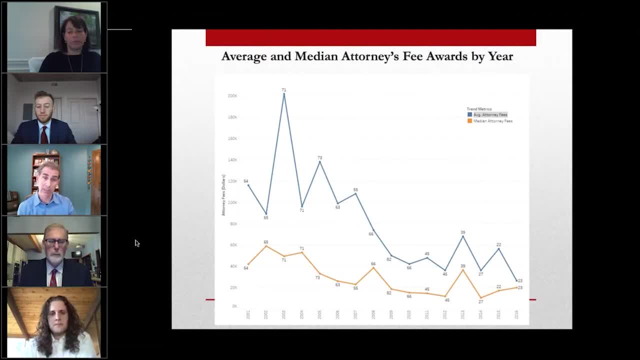 declining over time. So we not only observe relatively modest amounts of attorneys' fees granted. there's a relative low percentage of cases in which attorney's fees are granted- roughly 15% overall, or a little less than 40% of the cases in which plaintiffs prevail- And then it's also declining over time. 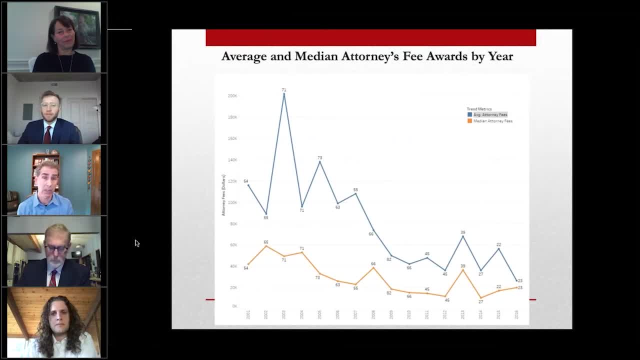 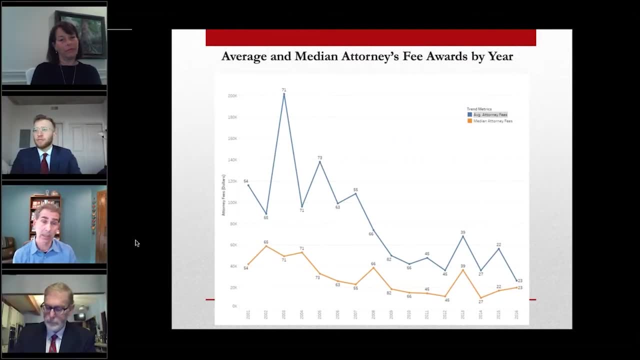 And so again, one of the controversies over citizen suits is claims that one reason that they're filed is to obtain attorney's fees. We just think the amounts and the percentages and cases in which they're granted really are compelling evidence against that. those sorts of 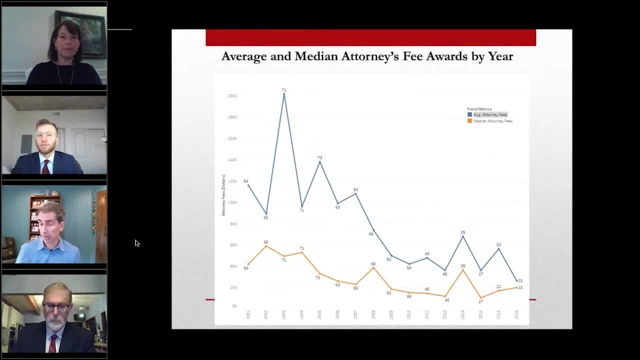 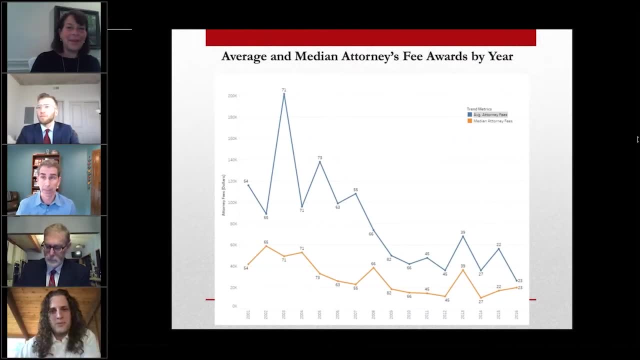 claims with regard to citizen suits. So I'm going to stop there and then turn it over to Joy to talk about the implications and our recommendations in the paper, And I just want to remind everyone that the slides will be available on the ELI website. 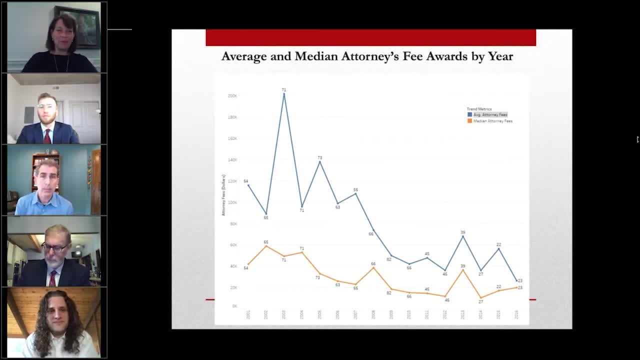 I think this is fascinating data And also remind everyone to mute. I love when dogs can join the webinar, but it would be great if we can mute when we're not speaking, And hopefully no dogs will sit off mine, so I apologize in advance. I'm going to take 30. 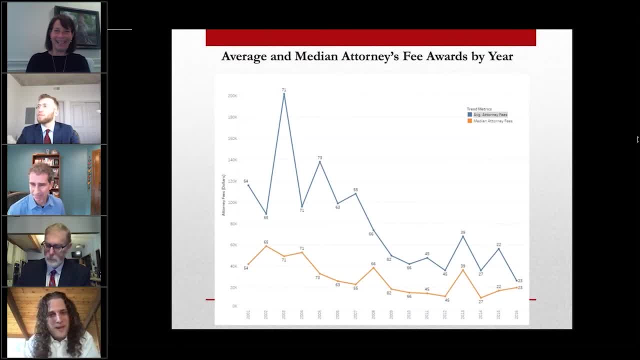 seconds out. I'm going to take 30 seconds out, in front of a very limited time here, to disclaim that I'm here today in my personal capacity. I had the pleasure to work with David on this project before I joined EPA, So everything that I say today is my opinion, mine alone, and not that of the United States. 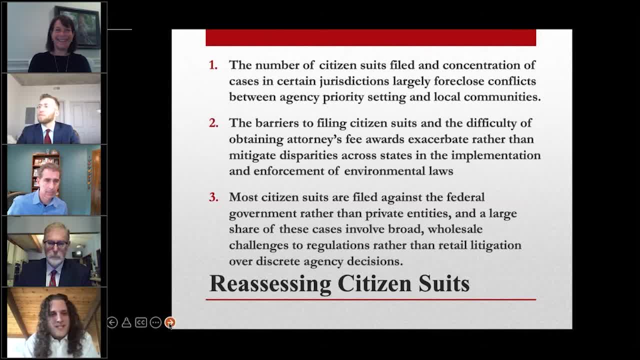 government or necessarily representative of the use of EPA. That all being said, I'm going to go ahead and quickly jump into a little bit of our reassessment of citizen suits. So, based on the data that David presented- and he's touched on a few of these themes already- we kind of took 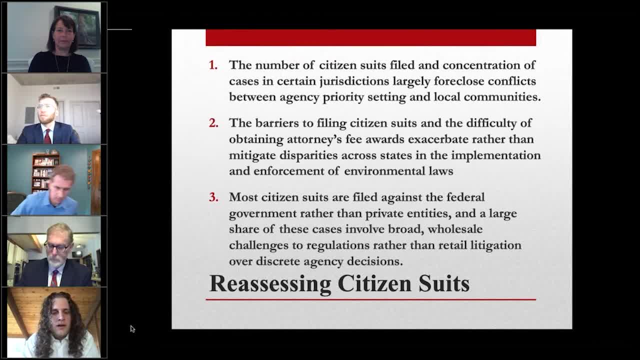 three key takeaways about the commentary that has existed on the threats and promises of citizen suits. The first is that the number of citizen suits that are filed and the concentration of cases in certain jurisdictions largely forecloses critics' critique that citizen suits will conflict with agency. 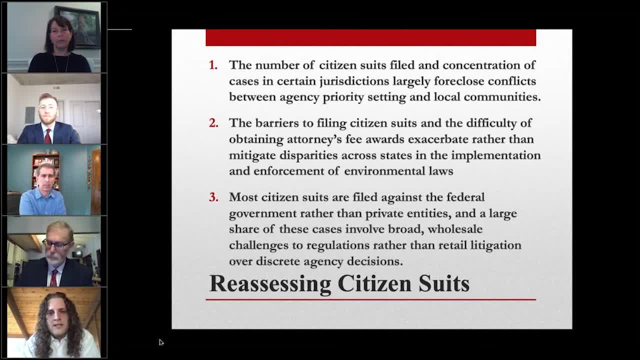 priority setting and the preference for local communities. This is kind of tied, as David mentioned earlier, to the modest number of citizen suits that are filed and the clustering of those citizen suits. The second major takeaway is that the barriers to filing citizen suits and the 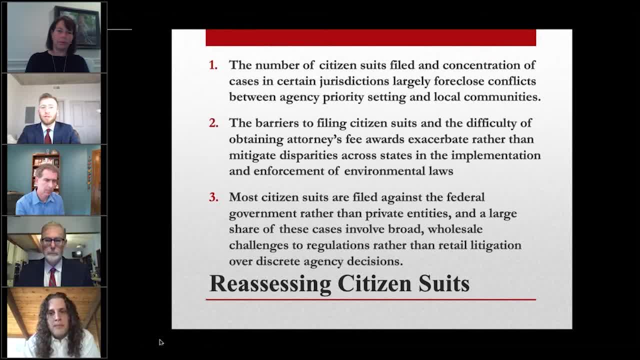 difficulty of obtaining attorney's fees awards may exacerbate rather than mitigate, as proponents posit, the disparities between states in implementing and enforcing the environmental laws. This is kind of the core of where our paper's title came from, and our theory here is based on the data that we're 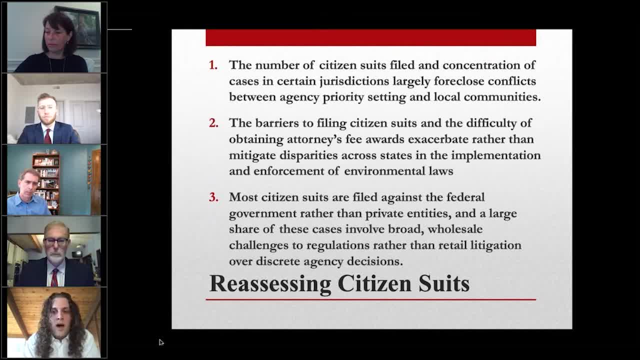 seeing is, the progressions do not show a significant connection between the rigor of enforcement in a particular state and where third party citizen suits are filed. Rather, it seems to be that there's parochial behavior on the part of the litigants. The last of our major takeaways is that most 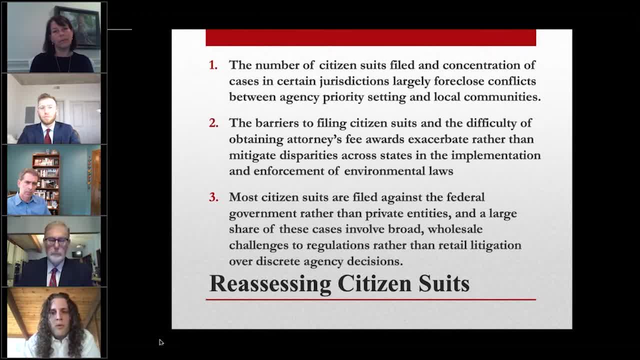 citizen suits focus on the federal government, not private entities, and may involve what one might consider broader actions like regulation, rather than retail challenges to discreet agency decisions or actions, And this does tend to be heavily tied to the structure of the statute. On one end is the CAA. 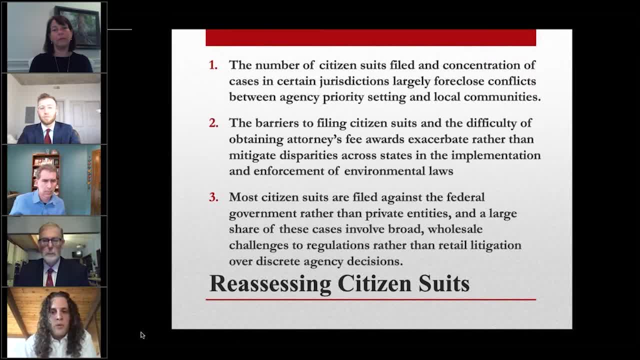 which is overwhelmingly a wholesale statute, as David mentioned. On the other end would be NEPA, which is overwhelmingly retail, and everything else being kind of in the middle ground. David, can you advance the slide please? So just to put this a little bit in perspective. 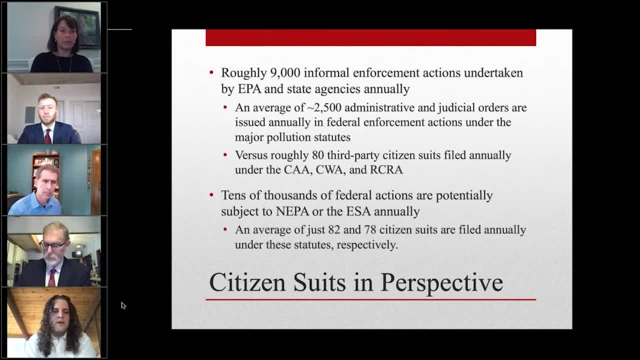 we wanted to draw out something that's a little bit buried in our paper and I'm going to leave the work on the slide. I just wanted our audience to allow me to read what's on the slide, but I'm going to focus on the particular example of the CWA. So during our 16-year sample period, 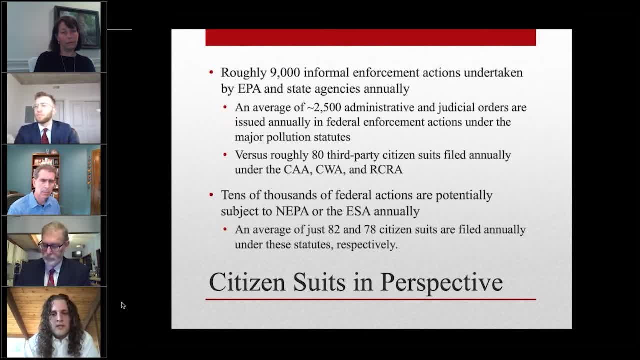 for the cases, there were roughly 19,000 facilities that were permitted to discharge pollutants And, during the 16-year period, as I said, there were between 10,000 and 11,000 federal or state enforcement actions. Despite this, citizens filed more citizen suits in any other area. 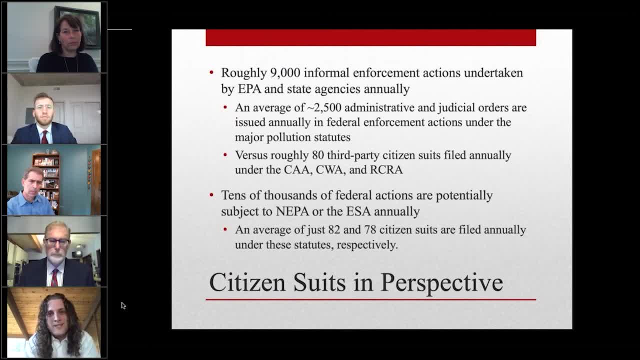 that were directed at private entities in this particular subcontinent, and this was a lot of work. In other regards category of cases, there were only 160 cases filed by citizens, And that accounts for just about 2% of the total activity of the federal government in that same timeframe. So the federal 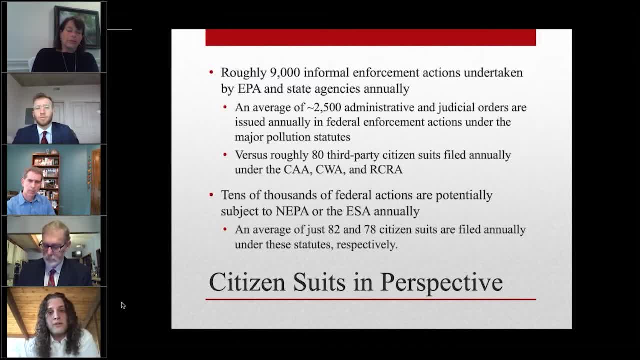 activity really is dwarfing it. And so, even if by a couple orders of magnitude, so even if the impact of an individual citizen suit is greater than the impact of an individual enforcement action by the federal government or the state government, the sheer volume of federal and 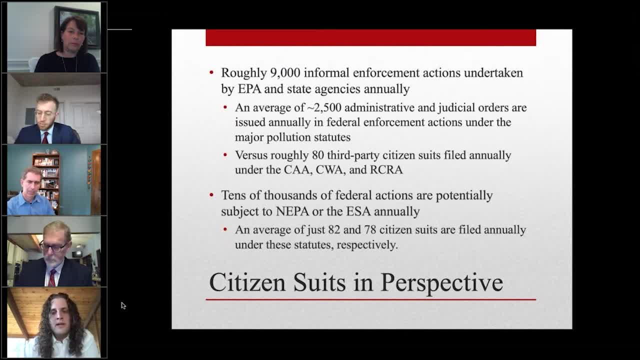 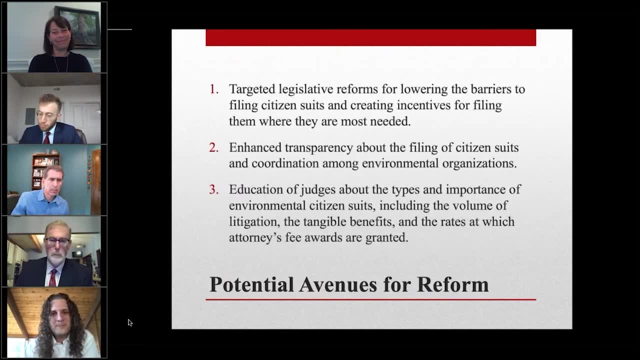 state activity is significantly outweighing that of the individual actors in the citizen suit provisions, And I'm going to be sensitive to time, so let's go ahead and go to the last slide here. So, based on our findings, we kind of put forward three key takeaways that might be. 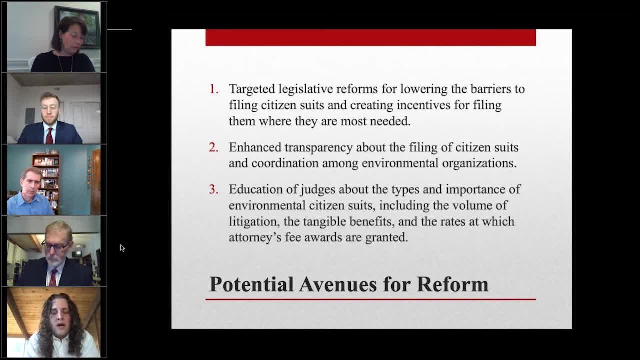 potential avenues for reform. We were primarily focused on reforms that could be considered to be practical or things that would be trying to exist within the existing climate of both federal and state government, And so we were primarily focused on reforms that could be potentially beneficial in the context of politics and the conversation around citizens suits today. 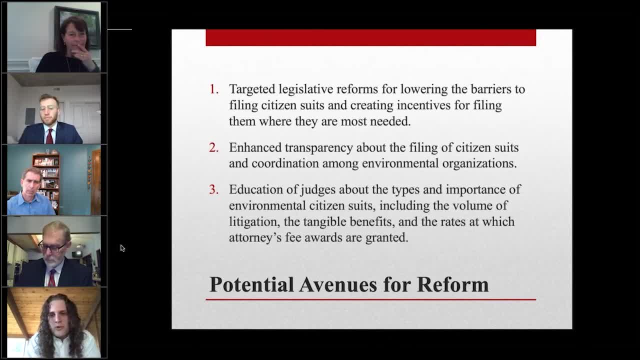 These are by no means exhaustive and certainly additional data could provide additional creative thoughts, But our key takeaways were that we wanted to push for targeted reform in the legislation context to lower the barriers to filing citizens suits and to create incentives for filing them. 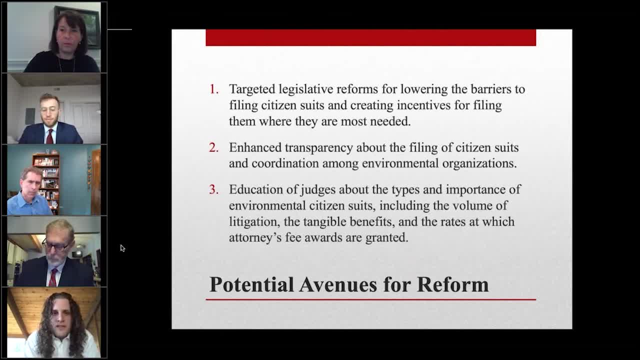 where they're most needed. David's going to talk a little bit more about this, I think, in the next slide, But I'm going to go ahead and move on for now from that one and talk a bit about enhancing transparency in the state of power. 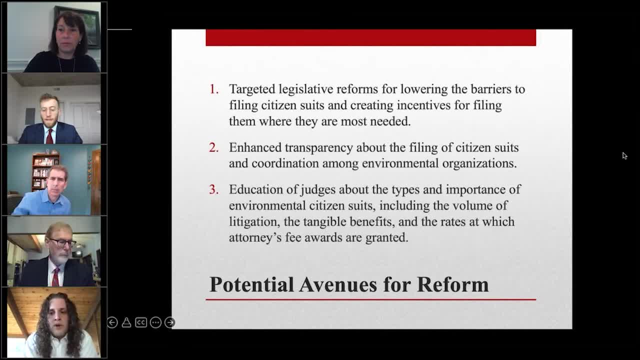 Okay, thank you of the filing of citizen suits and improving coordination among environmental organizations, which was our second key reform. Here we thought about using the existing infrastructure for reporting citizen suits to provide a mechanism by which we can improve the information gathering. that would allow both organizations themselves to better coordinate and conserve their resources. 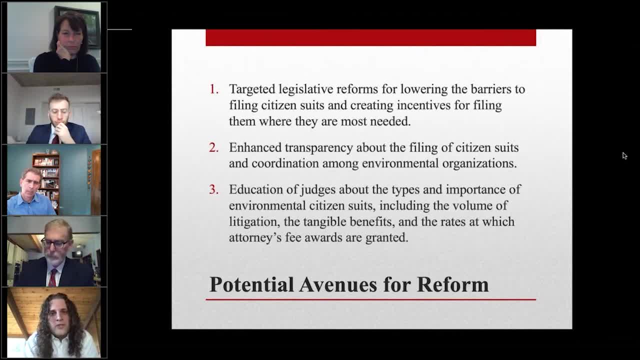 and also to allow us to better understand and dispel some of the myths that are around citizen suits, to allow us to hopefully allow them, to calibrate them to actually serve the goals that they were intended to serve. The last major area that we want to talk a little bit about is 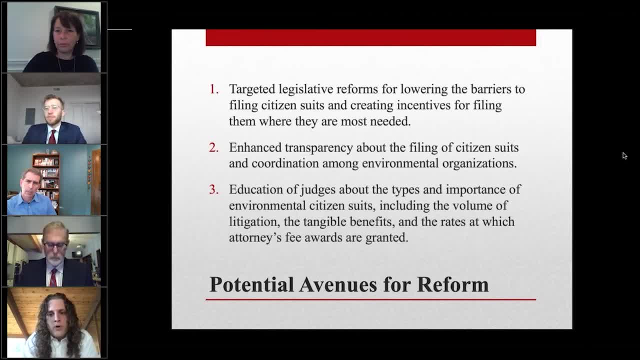 providing education to judges, And the importance here is that data suggests that many judges, because of the concentration in particular areas and forums, many judges, only have episodic exposure to environmental litigation And so, to the extent that they do and the intense polarization around many cases, they're not going to be able to do that, And so we're going to. 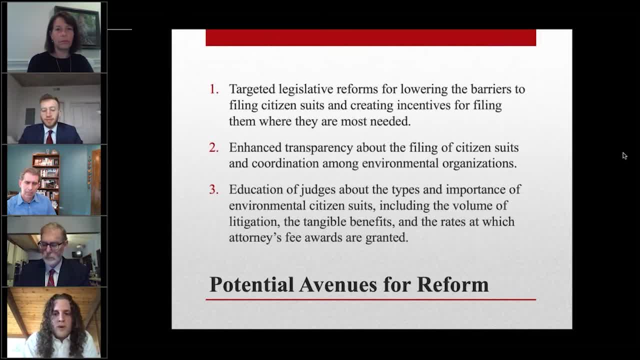 particularly citizen suit cases. This reform is directed at providing judges with the empirical context for how citizen suits operate and the important role that they could and may serve within the environmental law infrastructure, while combating any preconceptions that they might develop based on their limited exposure and the popular commentary around them. So I'm 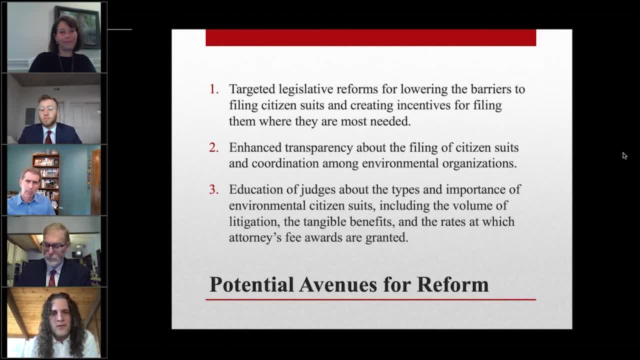 going to pass this back to David just to cover the last piece, and then we should be able to wrap it. Yeah, actually, I think what we should do. why don't we stop there, and maybe in the next few minutes we'll talk about some of the things that we've been talking about? 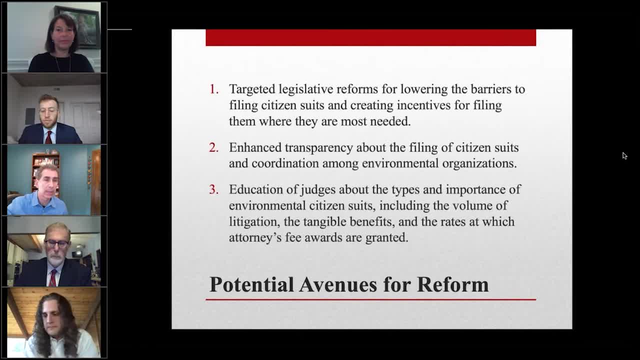 And then maybe in the Q&A we can talk about the some of the recommendations in a little bit greater detail or in response to some of the questions that are raised, just to keep on time. Well, that's not. that sounds great. And please reminder to everyone: send your questions in, We've. 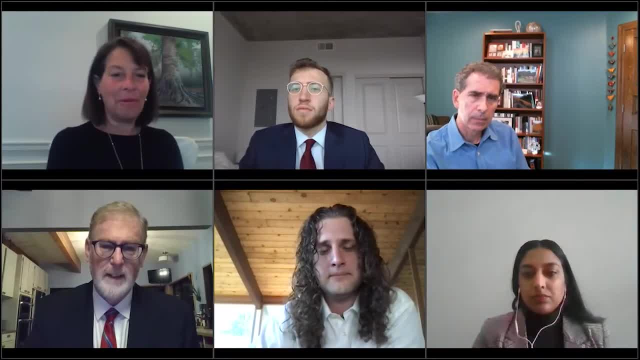 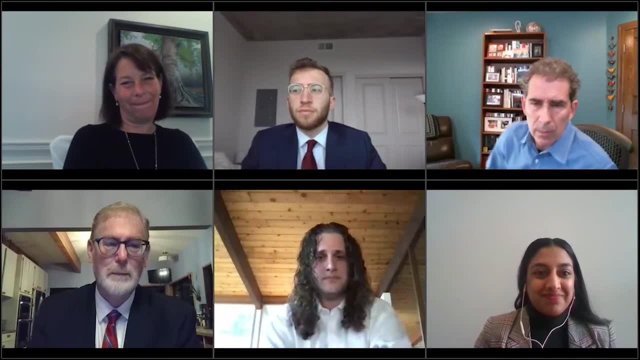 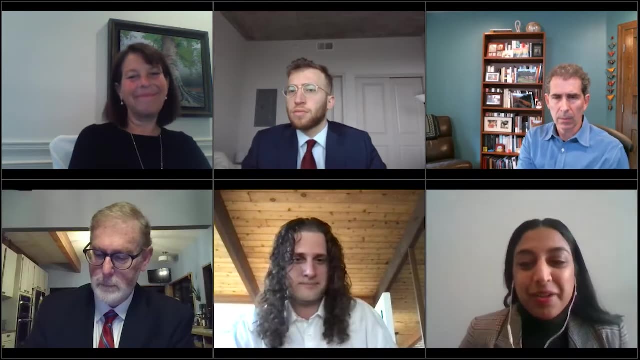 gotten a few, but we would like to get more, And I think we'll hand it over to our first commenter, Ms Revy. All right, I hope everyone can hear me. Thank you all. It's a real pleasure to be here. My name is Bina Reddy. 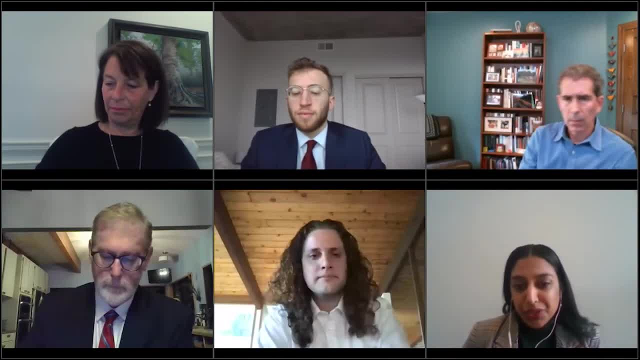 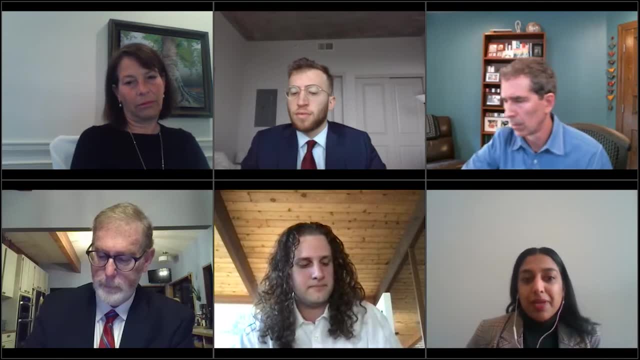 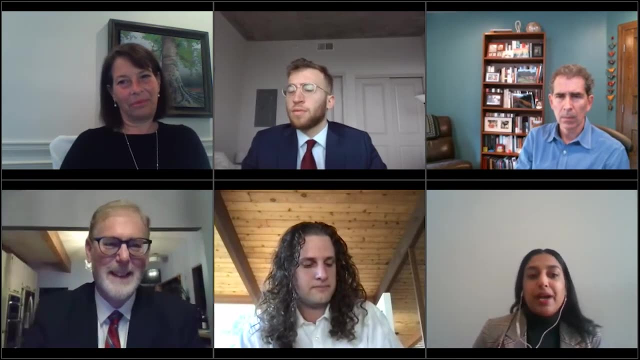 And, as mentioned, I am a private practitioner And my practice actually is primarily the defense of citizen suits. And you know, I'll start off by saying that. you know, I'll confess I've wondered many times to myself about, you know I practice in this space And what are the actual numbers? 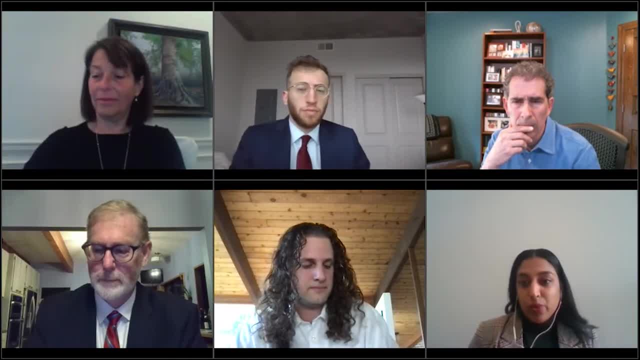 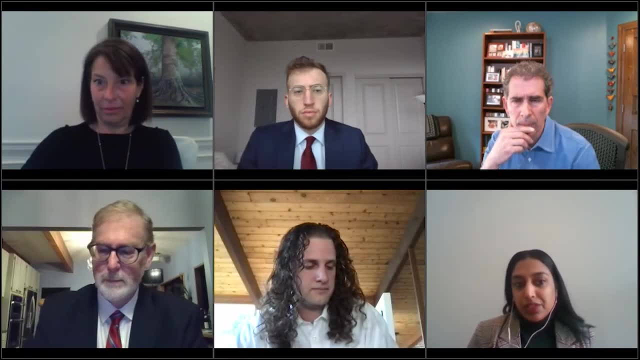 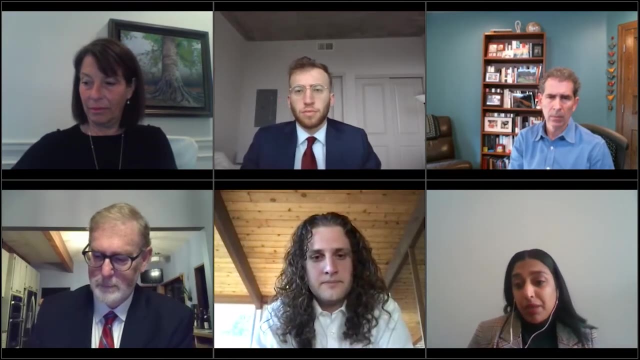 or trends that are associated with citizen suits, because from where I sit it is just really difficult to tell, And so it is. it's really interesting to me to be involved in this conversation that is around an empirical analysis of these suits And another thing that may be. 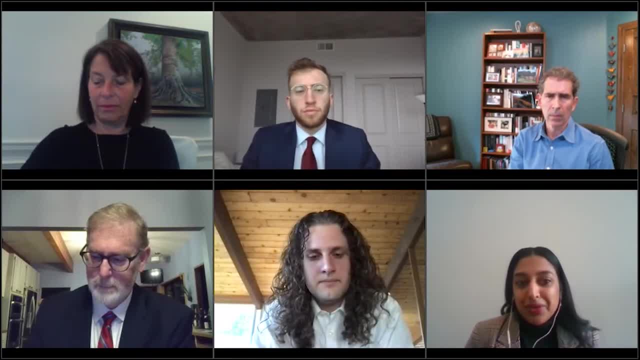 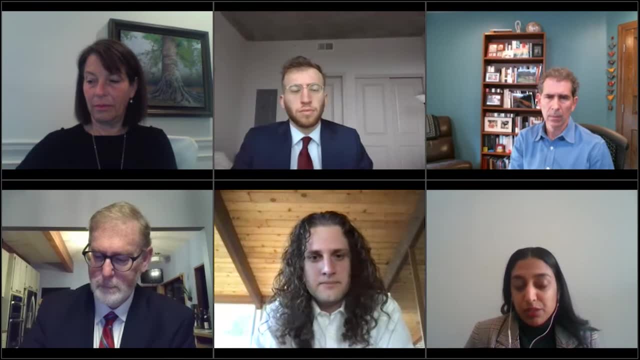 evident but is worth underscoring, I think, from my bio, is that I live in the world of retail suits. I live in the world of the private suits against against private entities, but not exclusively, as I'll get to later. And, and you know, this is, this is basically almost been. 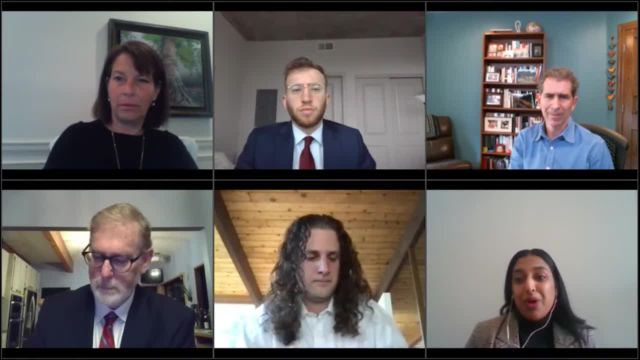 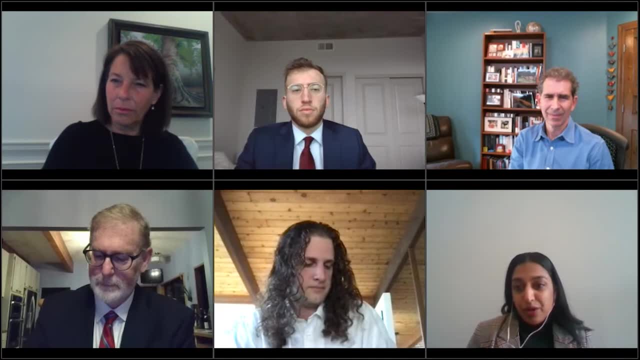 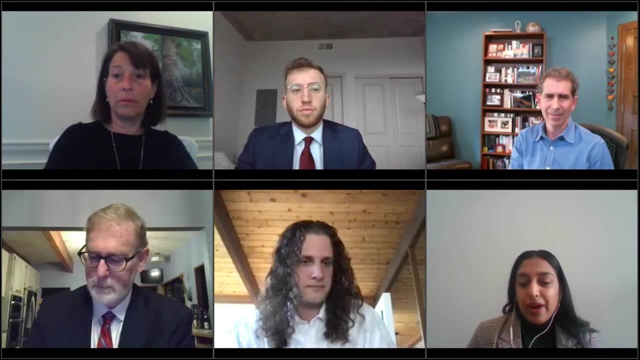 full time for me And so my comments are going to represent that perspective And I that that means that they're sort of necessarily anecdotal And I hope that you know my experience as a private practitioner is helpful to the group to sort of shed light where I can on, you know the 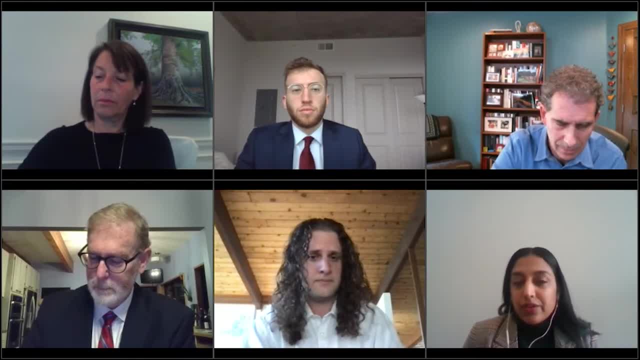 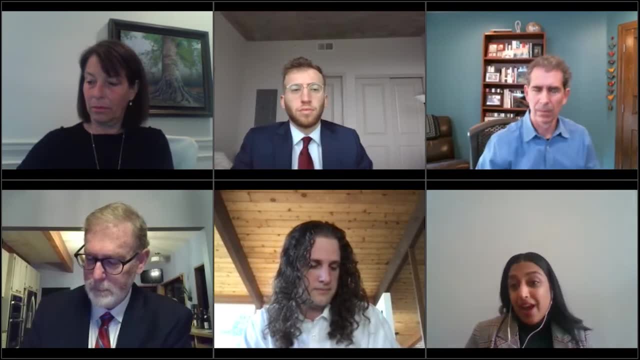 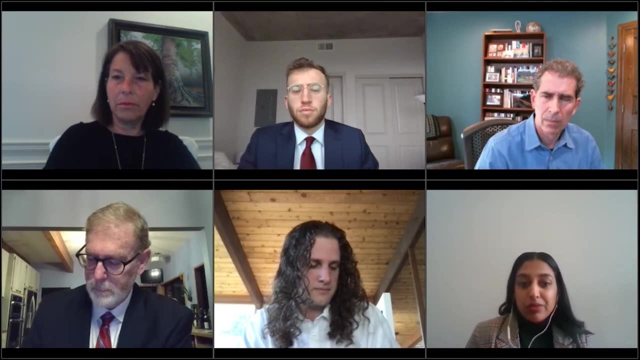 the disparities that are that are discussed in the article, And I guess I'll also. I want to be the first to acknowledge that. you know, I recognize that the private suits do take on this disproportionately large profile, right in light of the relatively small numbers that these suits 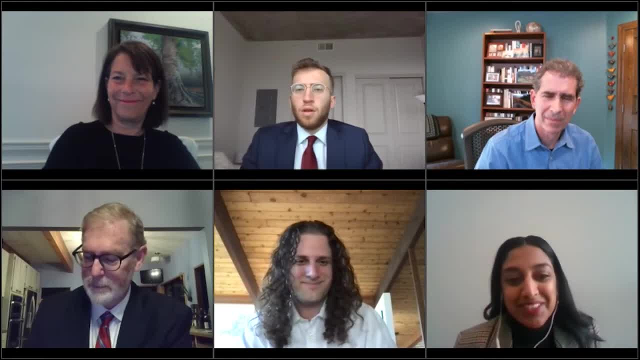 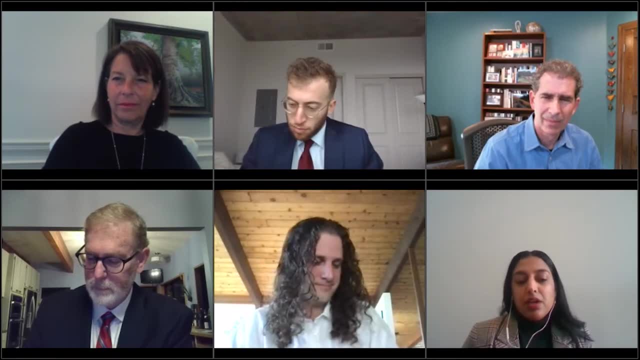 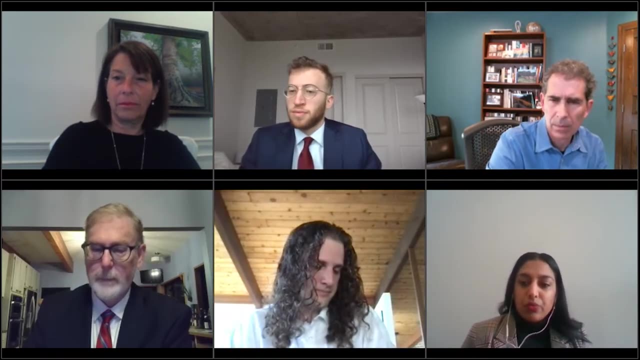 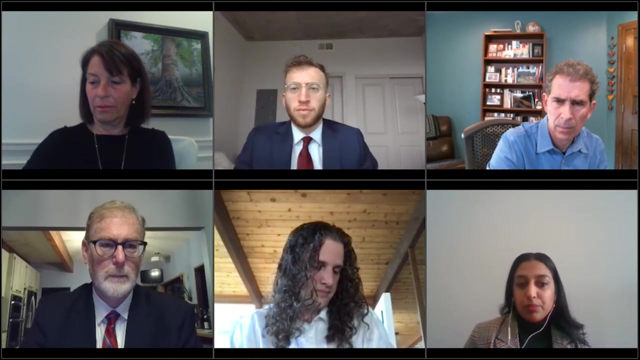 represent. But having said that, let me talk about the private suits, And one of the points that I took away from the article at a general level is that the retail suits, the private suits, don't really significantly advance the ball in terms of having the effect of raising or leveling the bar in terms of enforcement And 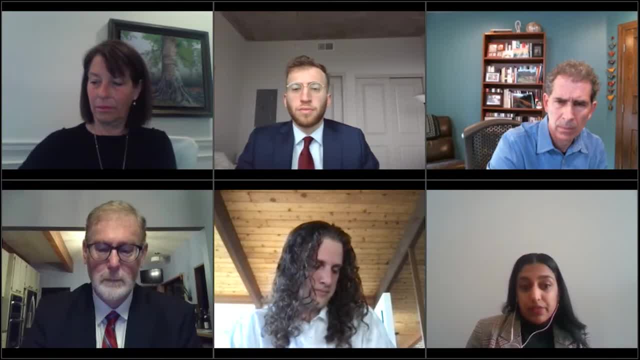 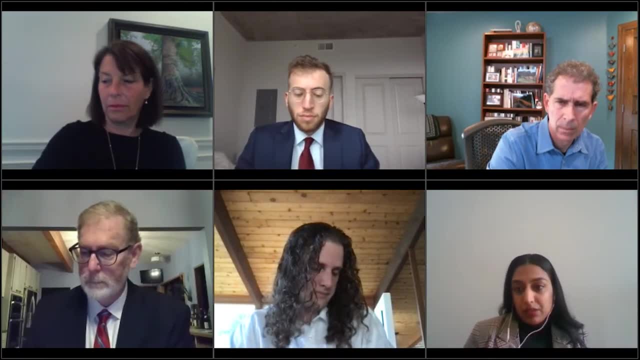 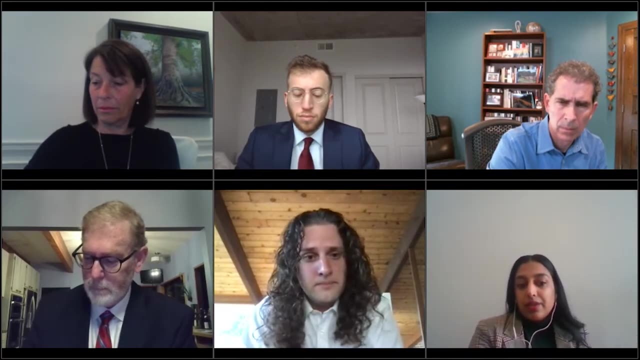 that's because they tend to be dominated by the site specific permit challenges. So the impact of that kind of enforcement is going to be inherently limited. it's going to be limited to okay it be informed at this particular location or facility, and so that's going to be of a limited. 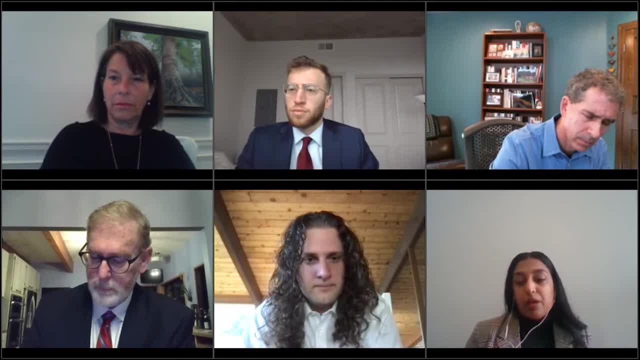 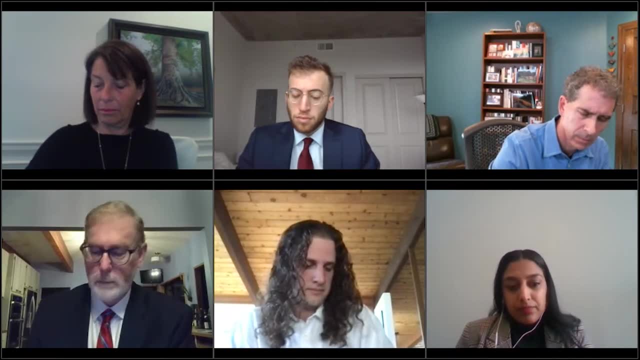 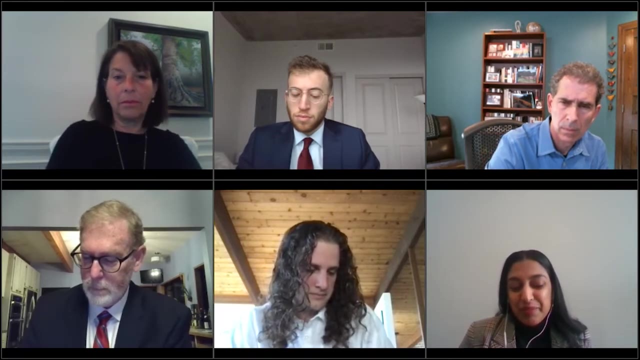 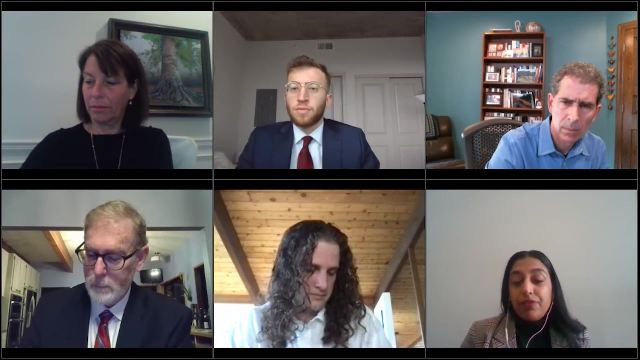 impact in it best neutral in terms of moving that bar in in enforcement. and I just want to offer that you know, as a you know full-time, for many years practitioner defending citizen suits, the suits that I defend don't fit well in that profile. the private: the private suits that I defend don't don't fit well. 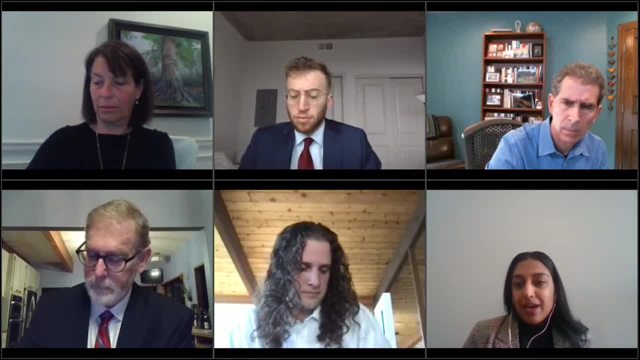 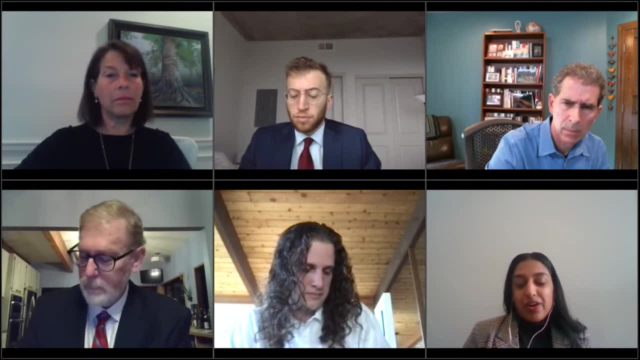 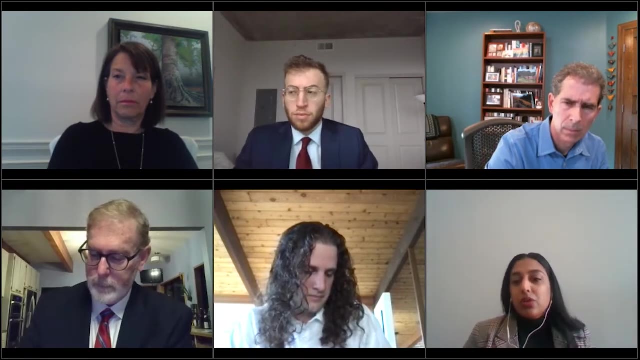 they are rarely about the numerical limits in a permit. they are not okay. this is your discharge threshold and you have exceeded it, and here's the citizen suit that you are defending, so I don't think that that will be a good suit. those are always going to be claims, but they really exist, mostly on the. 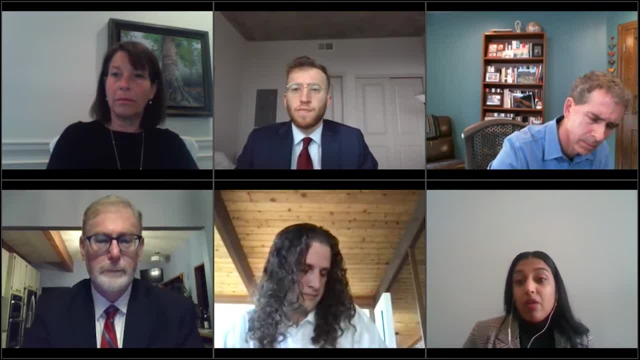 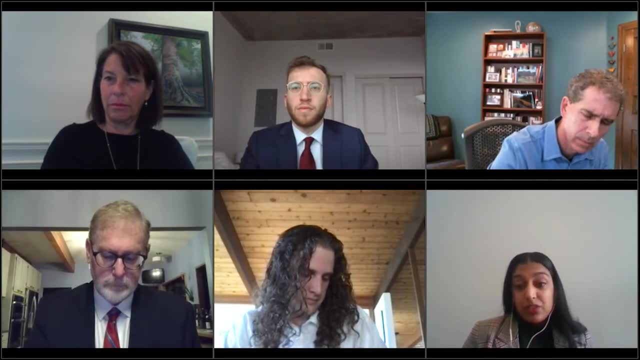 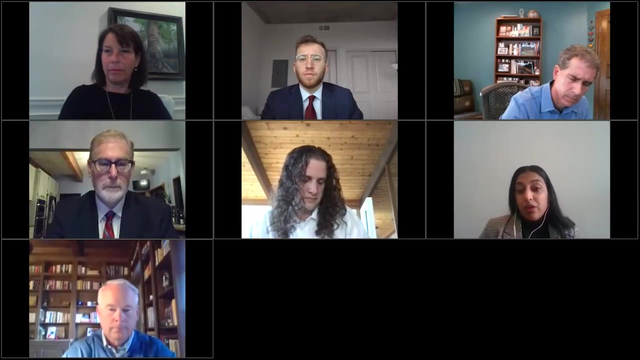 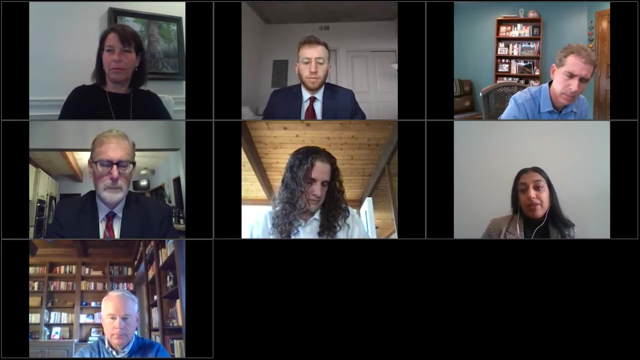 margins, at least in my experience, and and the heart of the cases that I've defended now for for many years- and I really can't overstate this, this is this is true consistently for me over a fairly long period- is that the heart of the cases are about narrative, qualitative terms in permits and these 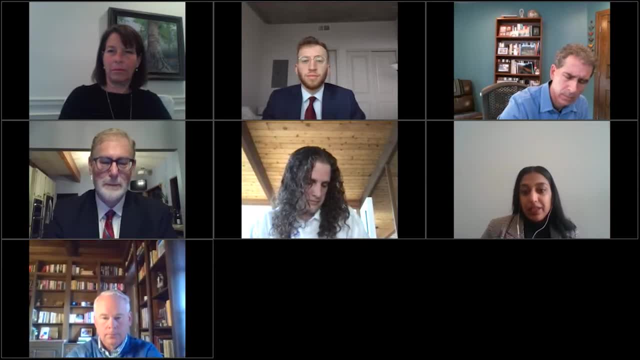 are. these are terms that exist in basically every permit, and I'm going to walk through a couple examples to sort of make this a little bit more concrete. but again, you know they are, they are about terms that are that are, you know, going to be subject to interpretation. they're not, they're not numerical. 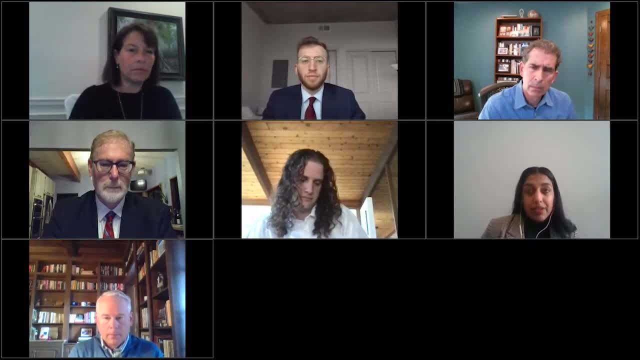 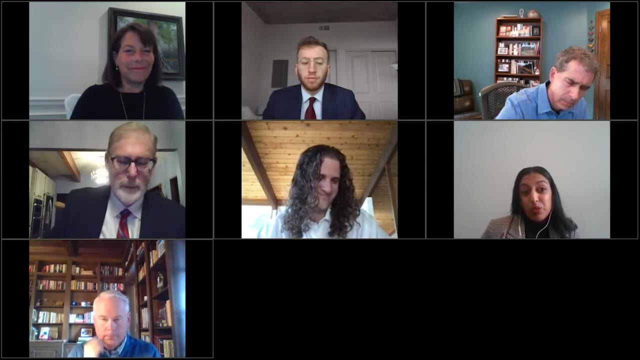 they're not easy to interpret. they're not easy to interpret, they're not easy to call, kind of a ball and strike, and often these are, surprisingly, questions of first impression. sometimes the statute of the regulation will have a definition. the definition will often be circular, and there there will. there will just. 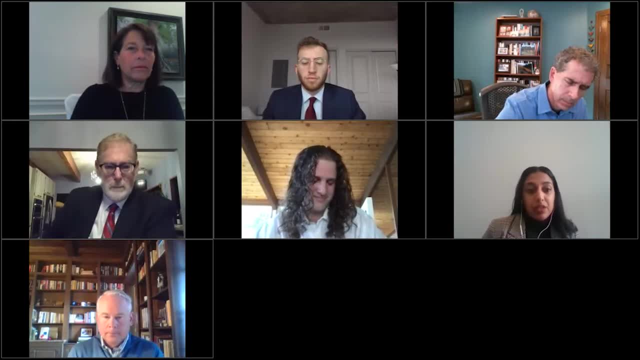 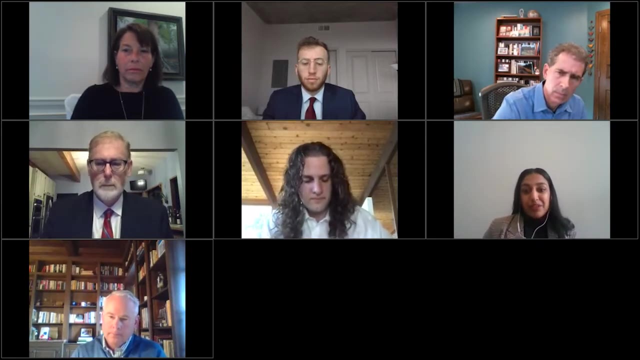 simply be almost no interpretation of what some of these terms mean, and I think it's. while, again, the retail private suits represent this small slide, and so I would, I would, and I would弄e it, I would posit that the impact of these suits can be very large and and and do in fact raise the bar. one of the 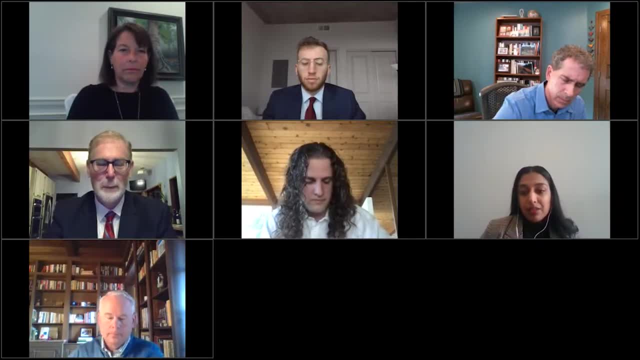 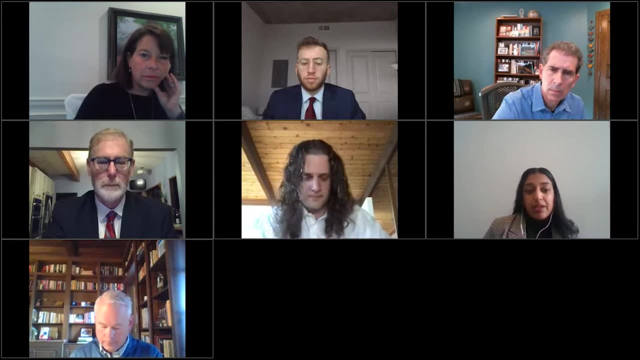 most high-profile examples of those that probably many in this audience are familiar with is the Formosa plastic suit in in Texas. that was a clean water act suit filed in 2019. I think- and then I'm likely thinking that's like the last in the audience- were the four most plastic suits that were in Texas. that was. 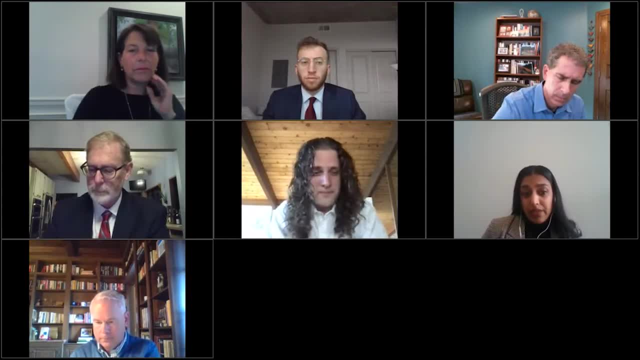 that was a clean water act suit, filed in 2019, I think, and that's exactly the. that's exactly the answer that I would. I would, I would argue that that's exactly that involved qualitative standards in a Clean Water Act permit And specifically so this is a case. 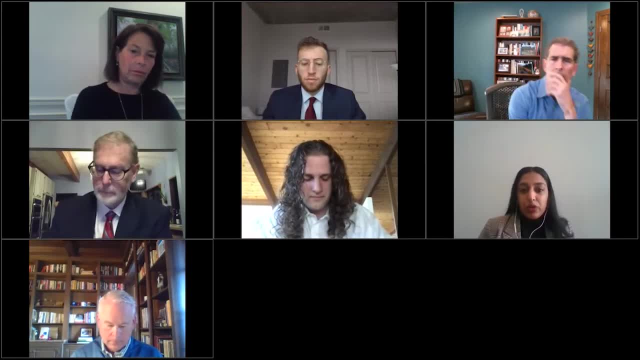 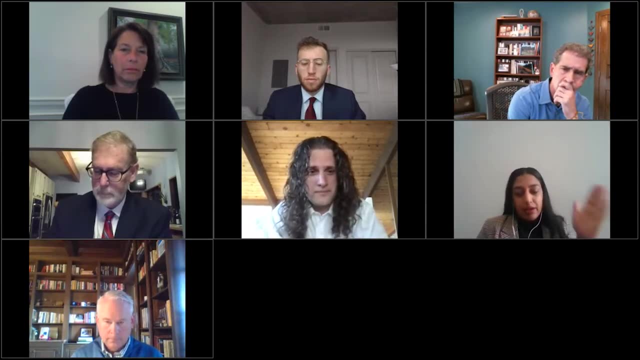 and there's several of these that have been filed around the country involving the discharge of these fairly small plastic pellets into waterways that are a byproduct of the production process, And the permits here forbid discharges of floating solids, of floating solids in quote, other than trace amounts. 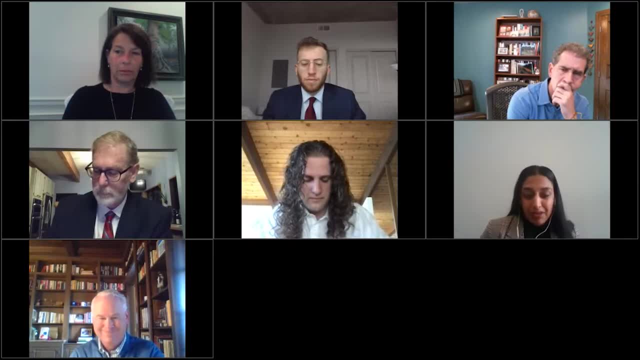 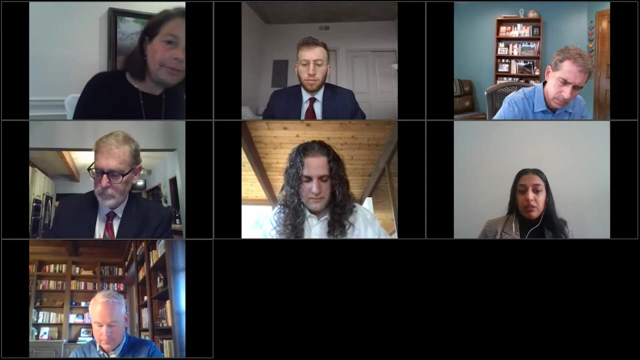 So the case was okay. what does trace amounts mean? right, And in that case the plaintiffs introduced into evidence hundreds of bags of waste that were collected downstream of this particular facility. The judge there determined that trace meant very small or fairly discernible, and concluded that the plaintiffs 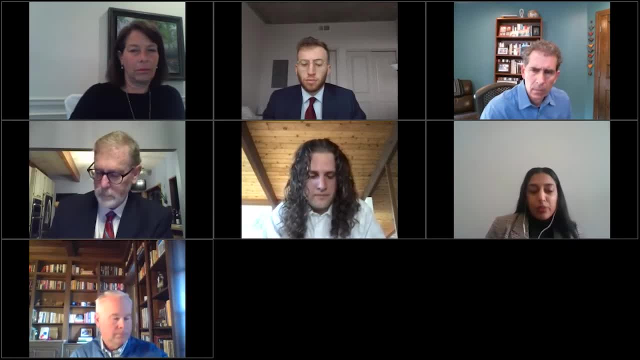 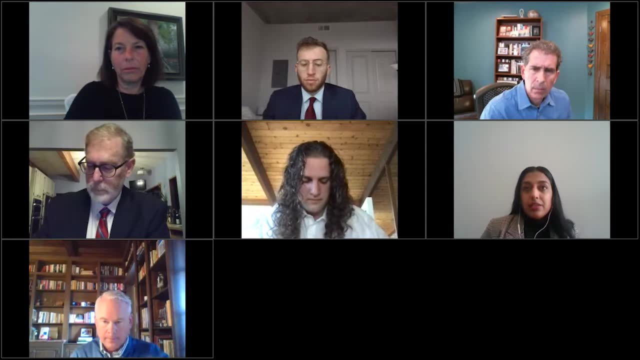 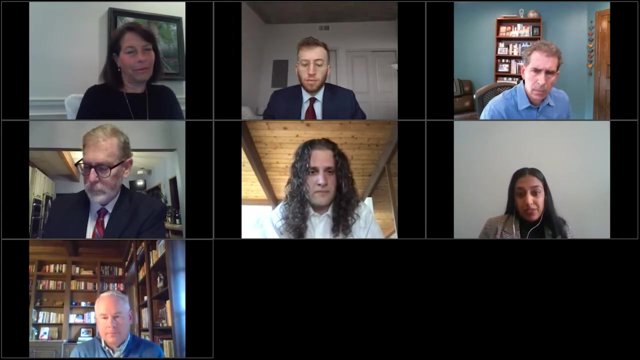 had provided sufficient evidence to meet this threshold and there was a violation of this language other than in trace amounts. And you can draw a pretty straight line from that newly defined standard in a permit that exists in everybody's general permit to an immediate action on the part of state agencies. 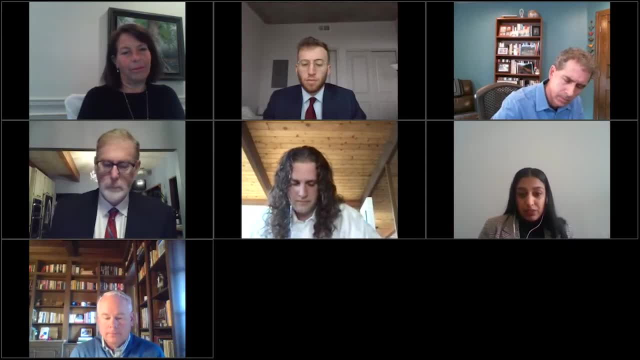 where, for at least the state agency in Texas- this is TCEQ- announced a clarification of its enforcement of this term and they have started to rewrite all the general permits to interpret this in other than trace amounts to mean zero Right. so the impact of that is, I mean, 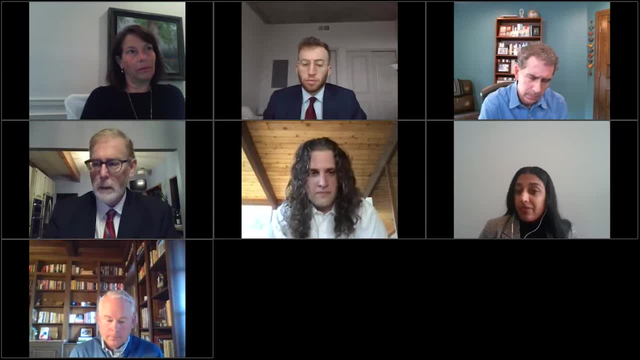 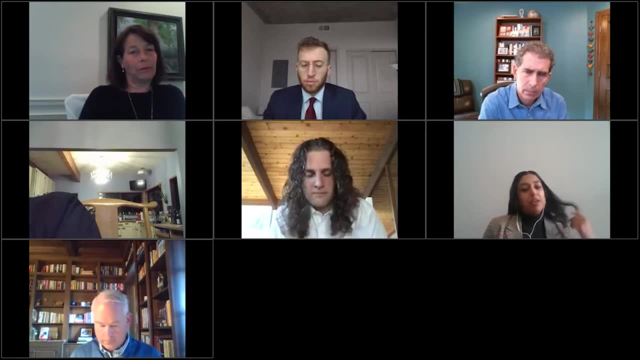 there's hundreds of dischargers in Texas that have that language in their permit And whether you sit on the side of the fence that thinks that's good or bad. it's just simply a fact That that is a raising of the bar via one interpretation. 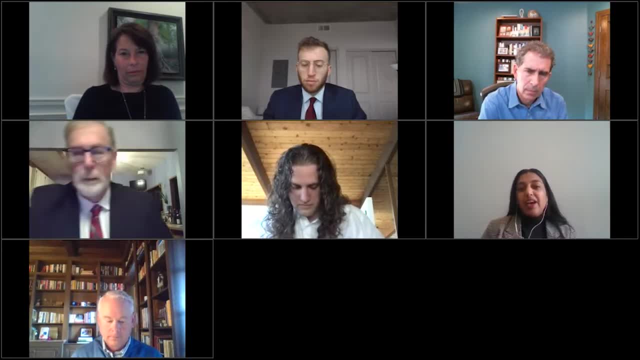 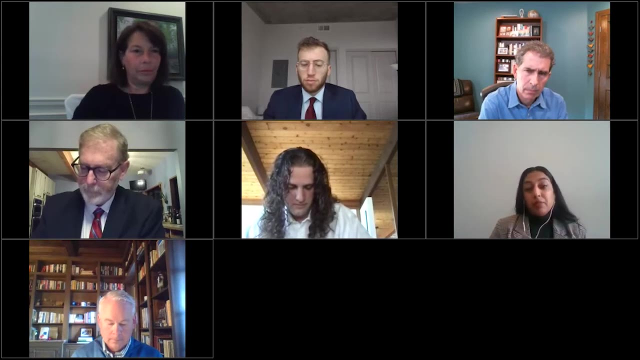 by one district judge, And so I think it's hard to capture those sort of examples in looking at the data that you all very admirably put together from the DOJ database. But I do think it's worth flagging that in my experience, this is the litigation. 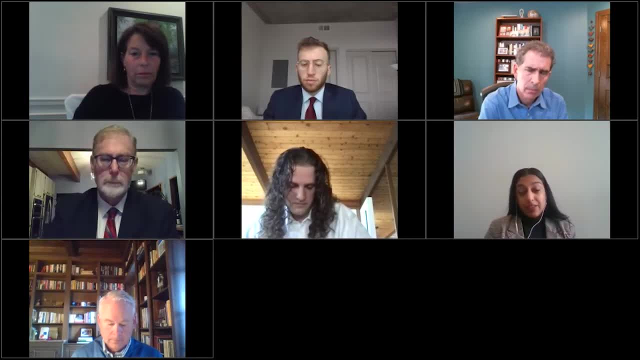 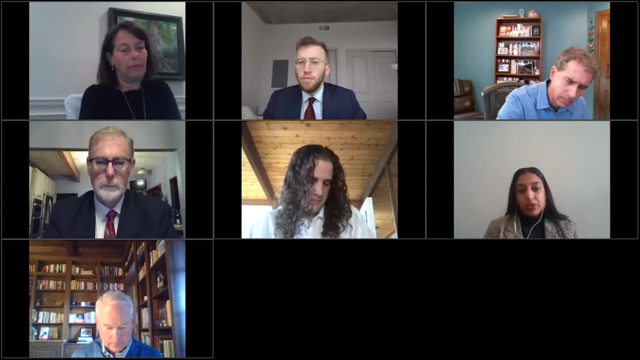 This is the litigation that I am seeing and that many are seeing, and at least I perceive there to be an uptick in it, And I'll just quickly touch a couple more examples in different statutes. So that was the Clean Water Act And we actually saw that resolution on the merits there. 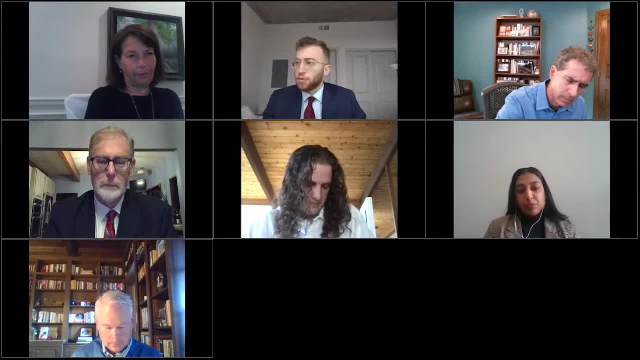 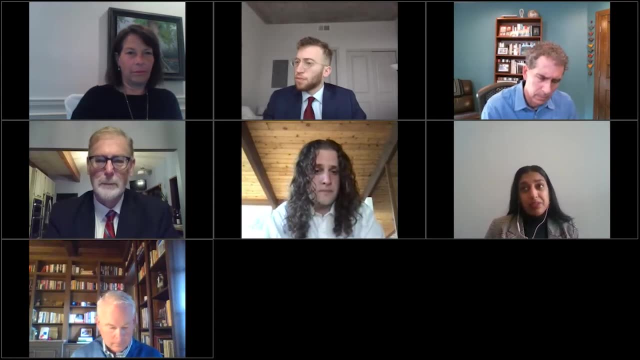 The next two were not resolved on the merits but pose the same sort of issues. Then the second one. the second example is under the Safe Drinking Water Act, which is it's rarely litigated in a citizen suit context. There's a lot of complexity there. 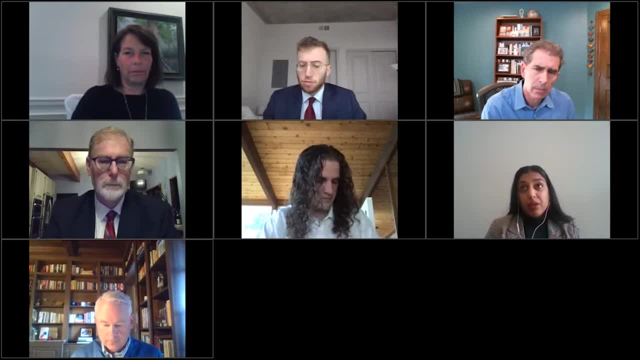 And I was involved in a Safe Drinking Water Act suit where really the question, the real central question in the case, was: what does the word optimization mean in the lead and copper rule? And I'll just kind of cut straight to the point that that term for 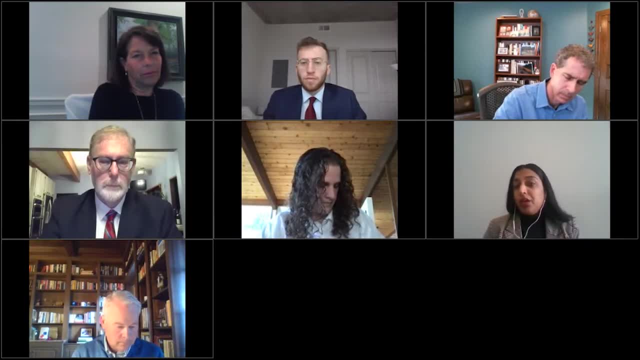 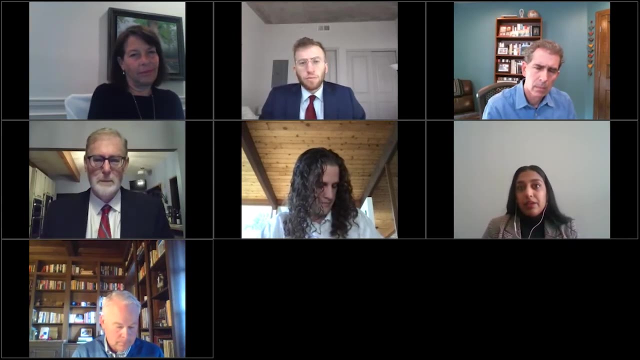 purposes of controlling lead in drinking water applies to literally every drinking water provider right, And so the impact of that decision is massive, both just in terms of the regulatory impact- I mean the compliance impact- and also there's huge financial impacts with having to tweak how you treat drinking water. 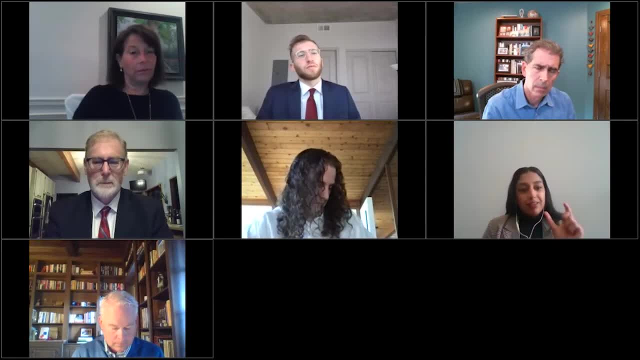 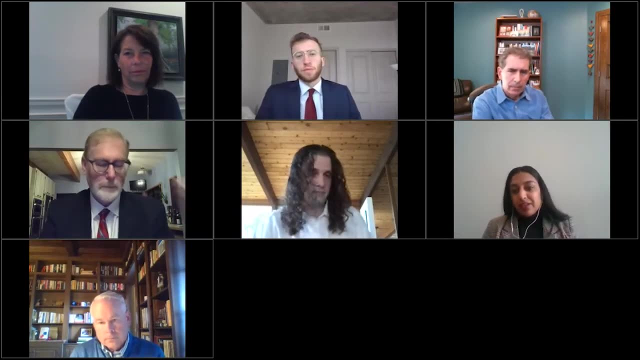 Those are gonna require major changes. So again, what does optimization mean? That's a kind of question, And similarly with trace amounts. those are not issues that are gonna be decided on a motion to dismiss. These cases are gonna go some distance, right. 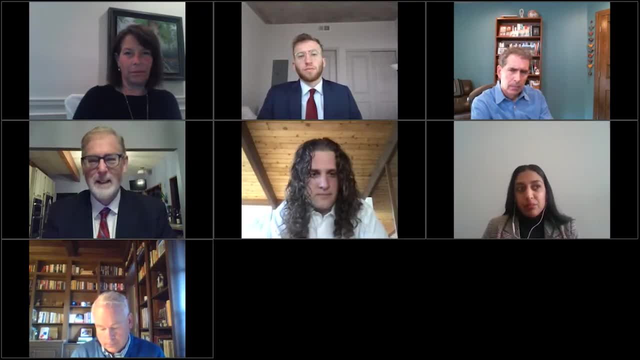 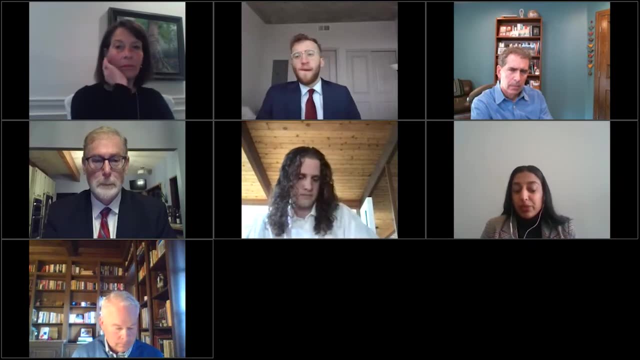 And you will potentially get a ruling at some point on that- and they can have the kinds of impacts we saw with Formosa. The last one I'll mention, because I think it's a really interesting one, is under the Clean Air Act and a term that I'm sure everybody 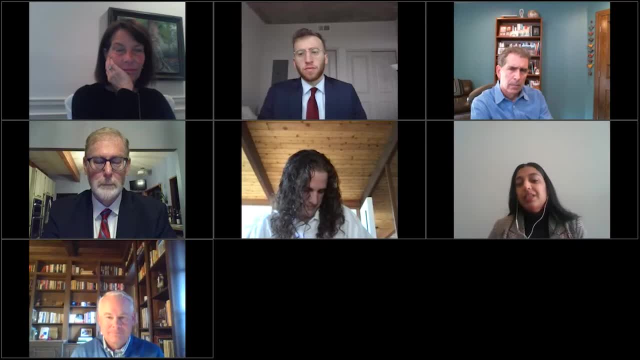 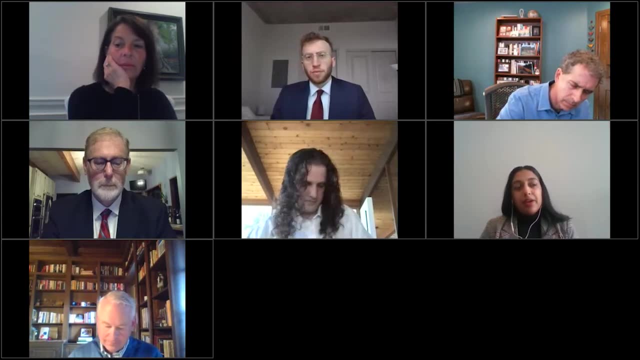 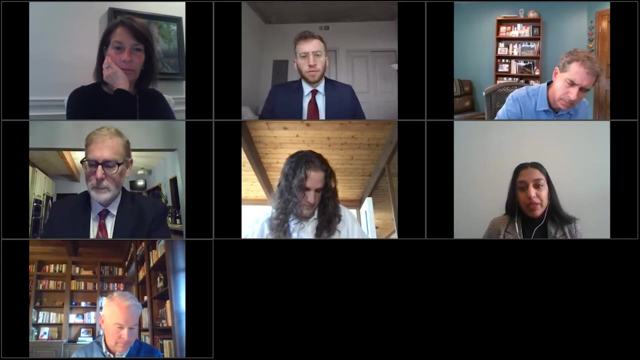 has crossed paths with is nuisance. A lot of Clean Air Act state implementation plans incorporate a nuisance provision, And so I was involved in a case. again there were on the margins questions about: did you exceed this limit? Did you exceed that limit? 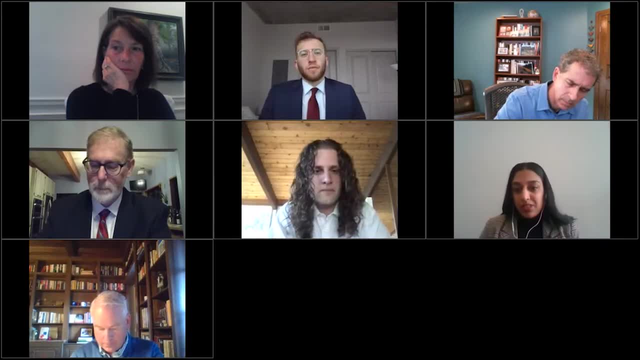 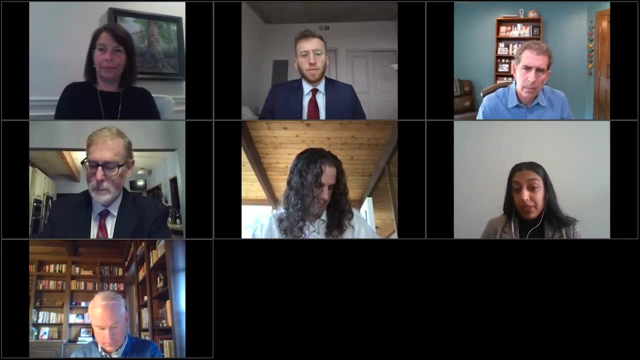 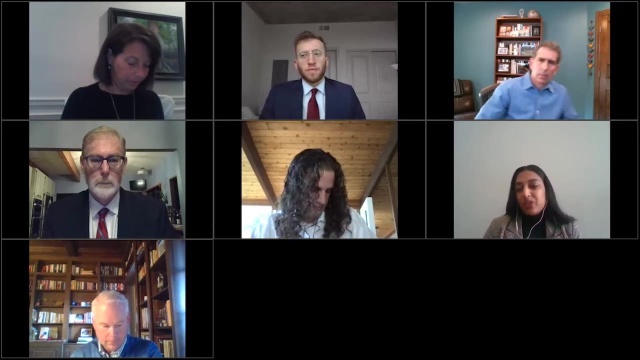 But the real question was: what does nuisance mean in the context of a Clean Air Act permit that has sweeping implications and also is interesting from an academic perspective, because that traditionally is somewhat of a subjective inquiry. but regulation is supposed to be uniform, shouldn't vary all that much. 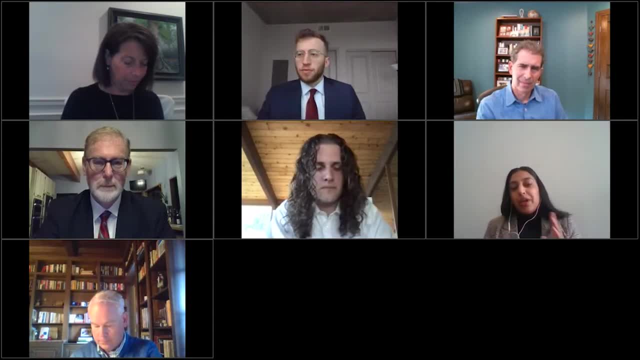 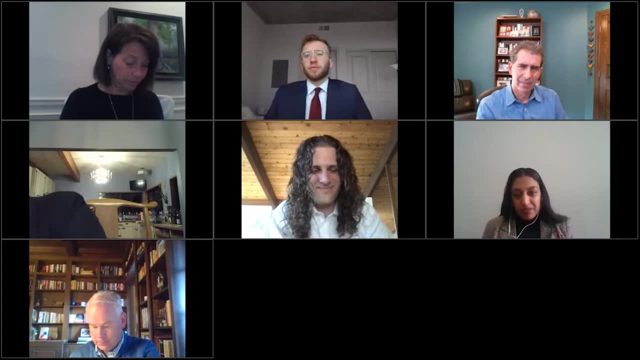 So I think I just wanna shine a little bit of a light on the litigation around narrative, qualitative terms and the role that it plays, And I think that's one of the things that I think is important. I think that's one of the things that I think is important. 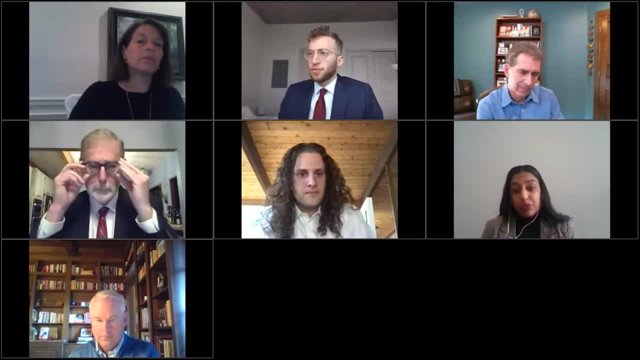 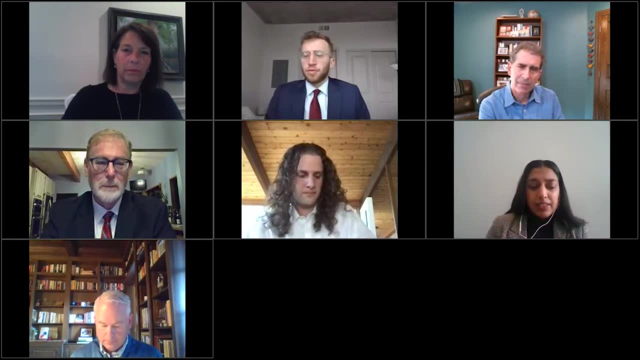 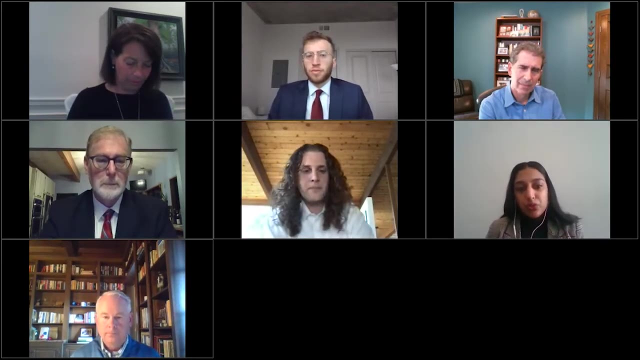 they play and what I see as real potential for raising that bar in terms of enforcement. The second point I want to make also comes from my experience and it relates to the questions about whether citizen suits do or do not really align with local prerogatives. right, What? 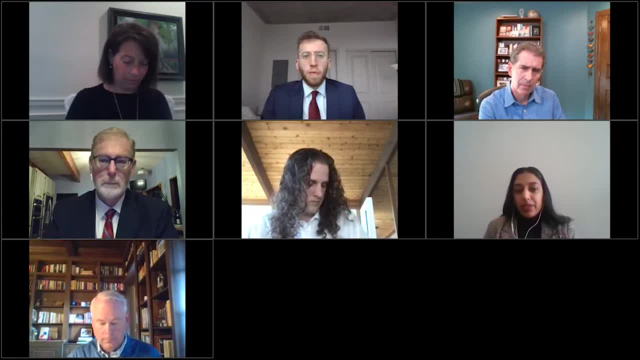 do local communities want and are these citizen suits really consistent with that? And I think the answer to that question is obviously it depends, And the answers are. those are incredibly complex questions, but in that vein I'd like to offer sort of a caution on relying 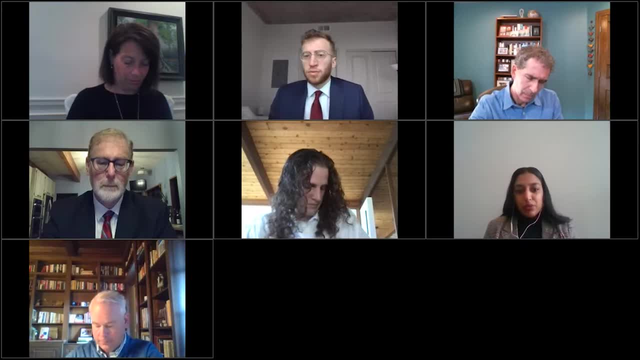 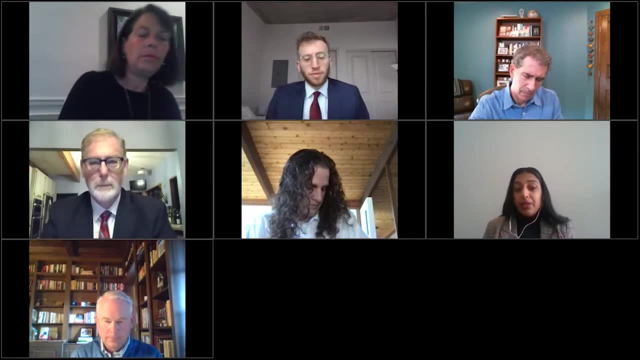 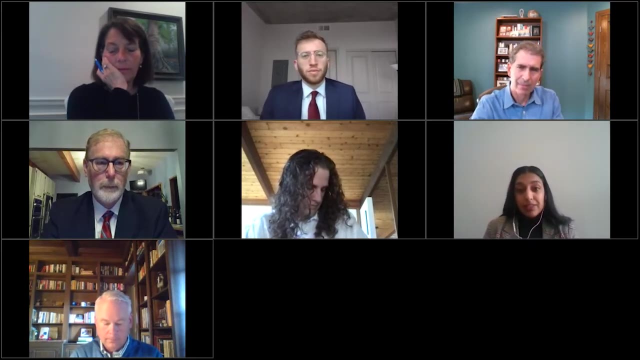 too much on statewide metrics as a proxy for local viewpoints because, at least in my experience, local views on environmental issues can vary dramatically Even across a single city, and they will reflect nuances and local politics. It is amazing what's really happening at the on the street level, And my thoughts on this are informed. 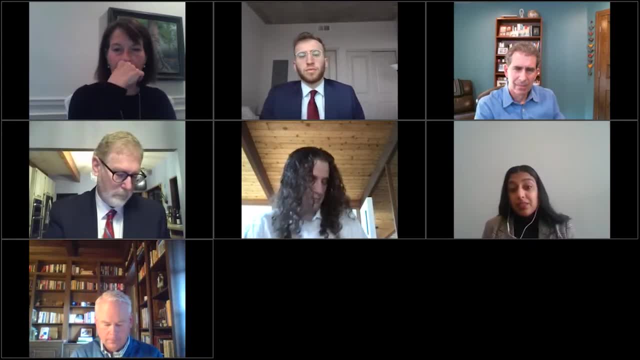 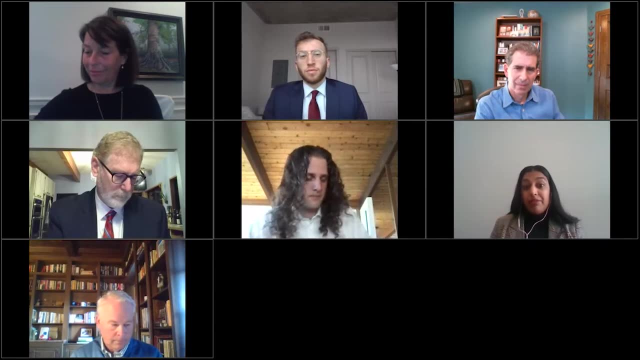 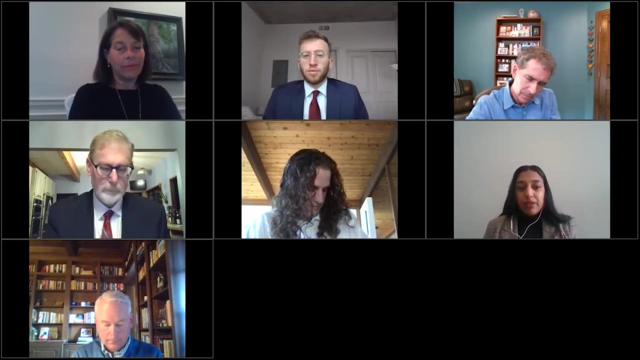 in large part by my experience defending municipalities and citizen suits when they are the regulated entity, because they're the issues of local views are often very sharp and easier to see. And that makes sense If you think about it, because citizen suits are often going to involve a claim for injunctive relief and major injunctive measures can have 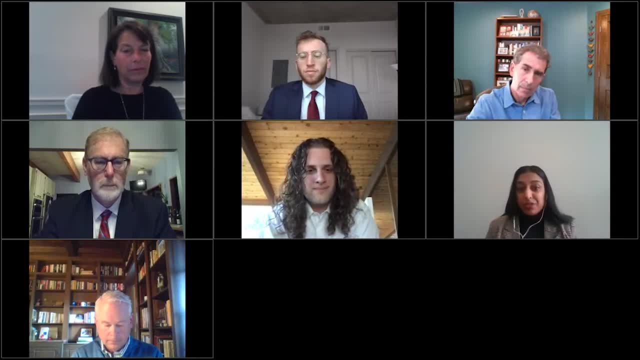 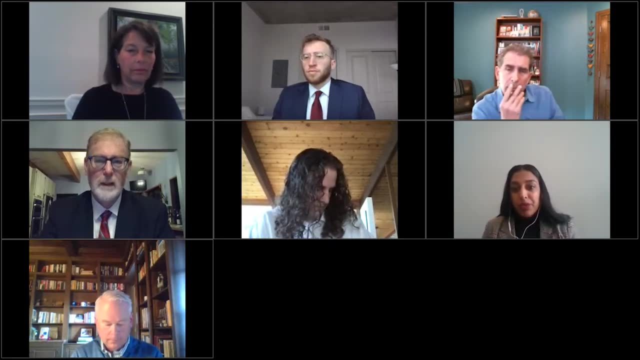 extremely high price tags, especially if you're talking about changes to municipal infrastructure, And so the rubber really hits the road there when you're talking about well, what does the local community want? Because the cost of that injunctive relief is ultimately going to be paid by. 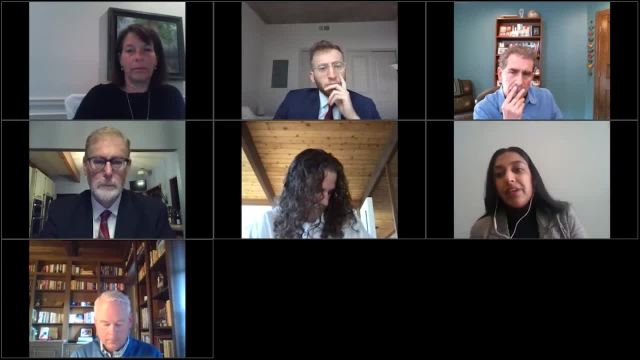 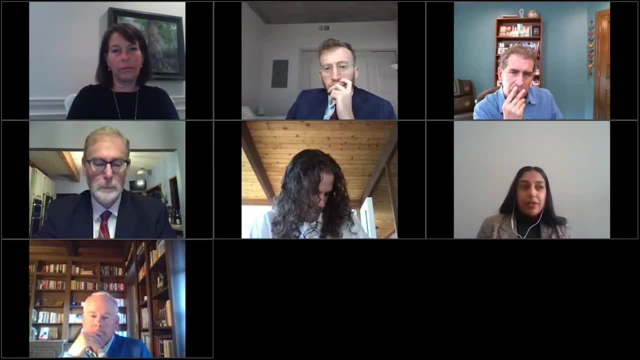 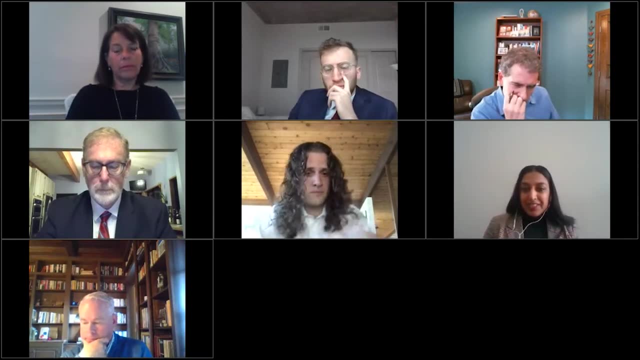 questions there that I just say, you know, I just want to offer- I know that it's difficult and we have to work with the data that we have- But I, you know, like I said, this is kind of anecdotal, but it's been true, in my experience at least, that it's very, very 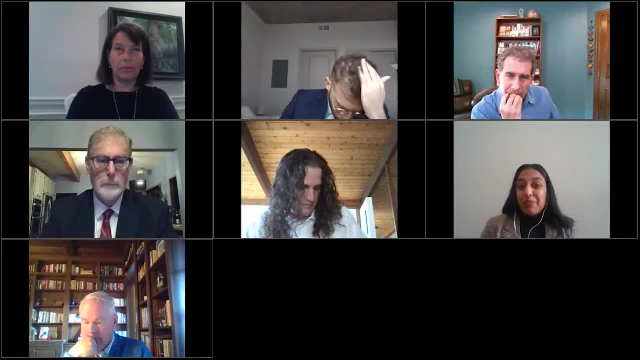 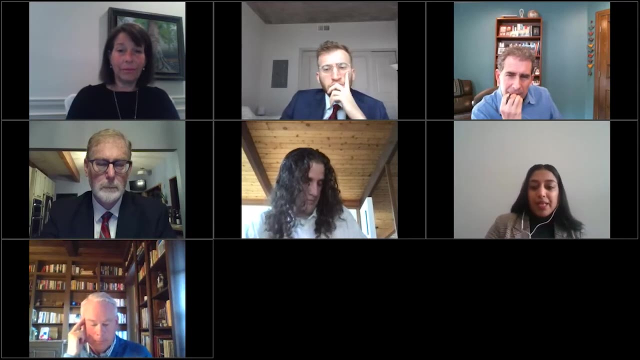 hard to capture local politics and while the impact of one city council race on your litigation can, you can feel it And and and how it reverberates through through the voices of the community. My last point- and I think I'm probably get bumping up against the end of my time- is on: 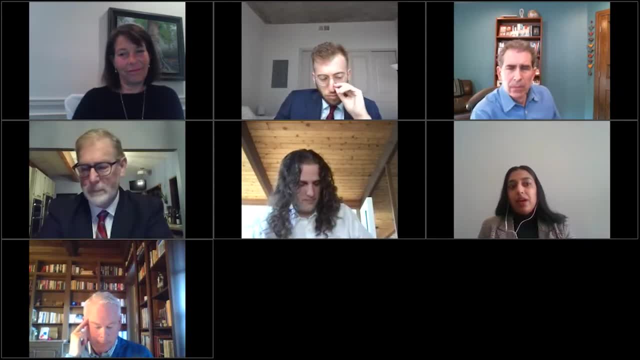 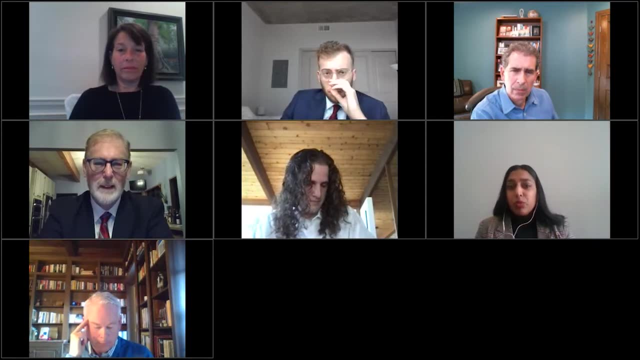 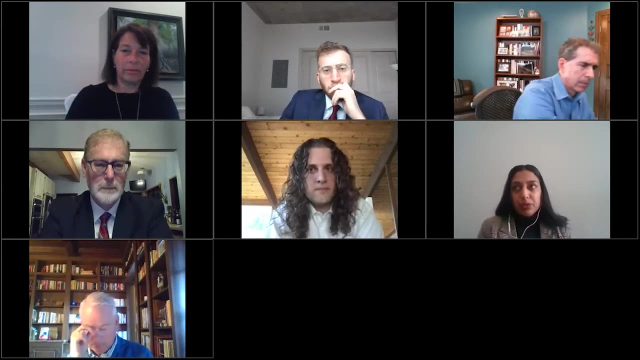 you know. so the ultimate question of how do we, how do we, how do we rectify this gap, How do we make this more balanced in terms of where these suits are being filed? And I have, you know, one comment, and then it sort of flows into maybe a question, And 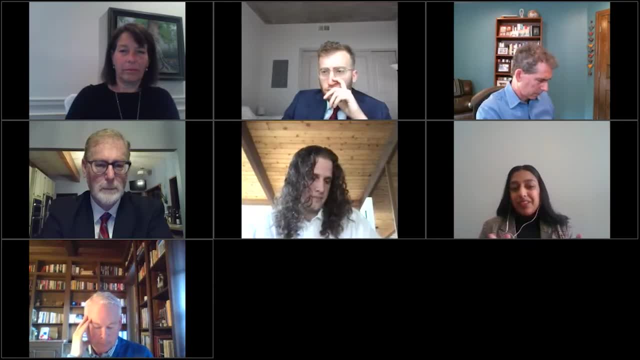 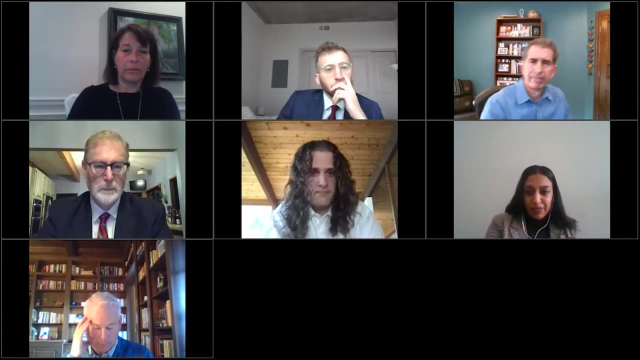 the comment is that, in my view, none of even the easy cases are not easy. You don't have a whole lot of attorneys walking around who are raising their hands to file citizen suits. They are complex, You know. you have to put out, you have to expend some funds and you 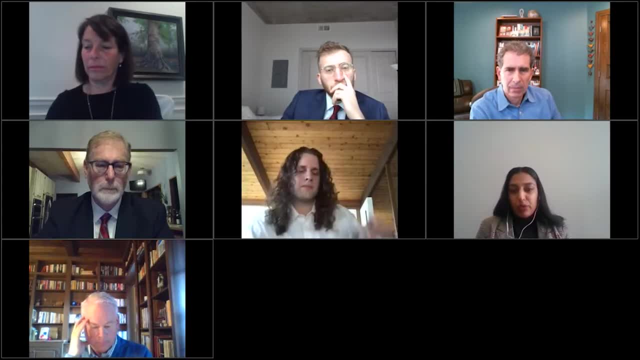 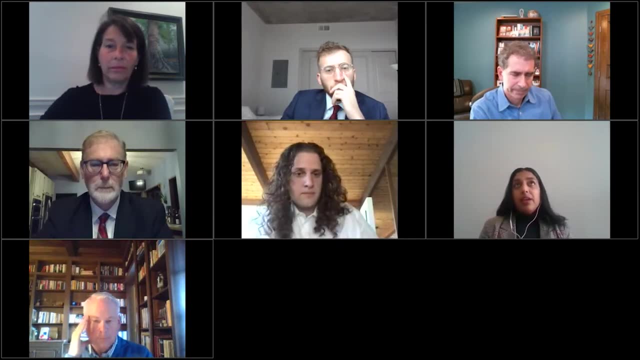 don't know, as we've discussed, whether whether you recoup that in the form of getting your attorney's fees back And the the technical and legal issues can be very arcane. And so I think you know, even if you're talking about one of those sort of simple suits where you have the 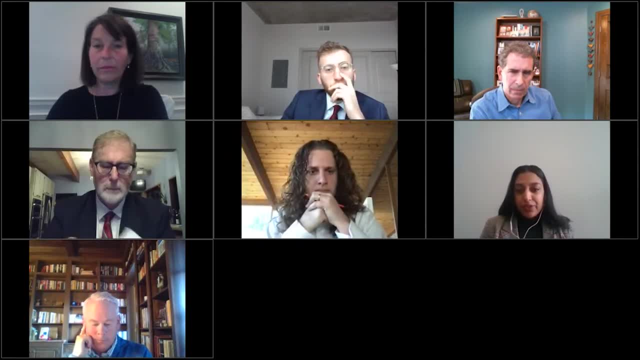 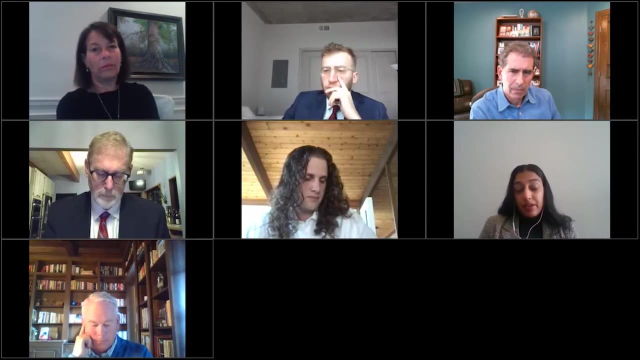 publicly available data on. you know, okay, here's your, here's your exceedance open and shut case. It never works out that way And that it's always been interesting to me that you know with the national environmental organizations. I think that 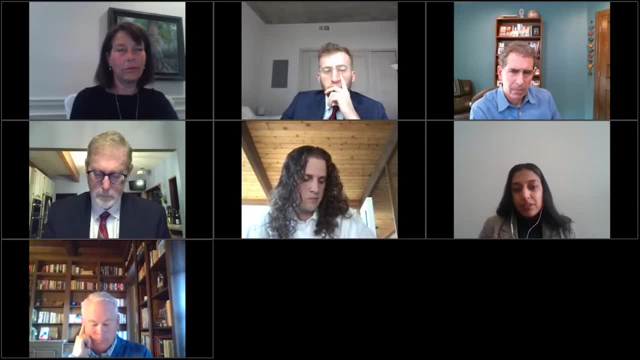 I have to suspect, at least in part, they have the success rates that they do because they are repeat players. They know how to do this. They have, they come to the table with, with a really knowledge that's hard to find other places and they have local chapters. 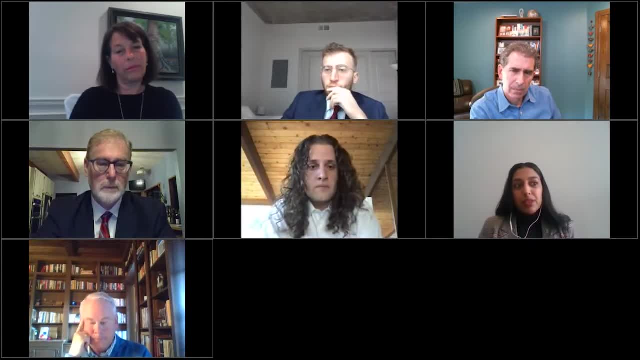 And I always wonder- you know you talked about coordination among the groups- Why, if it's not flowing to the local chapters in a meaningful way, why not? And I, I, I will say I, I don't really know whether it is or isn't. 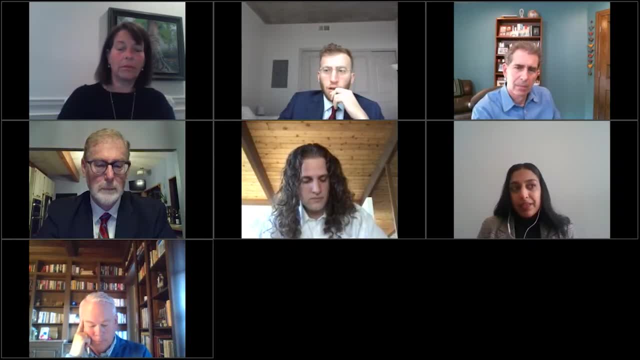 or the dynamics of how that works. But it always strikes me that, at the end of the day, the locations of where the suits are filed are right there, a decision of the, of the plaintiffs, And, and these organizations have have so much institutional knowledge, It seems to me that they 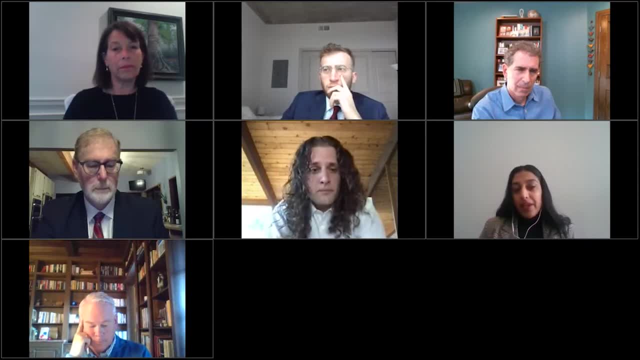 are a good place to start, particularly where they have these footprints. you know, and they're, they're a great place to start, particularly where they have these footprints throughout, throughout the country. So you know, I think that that is it for my comments. I look forward. 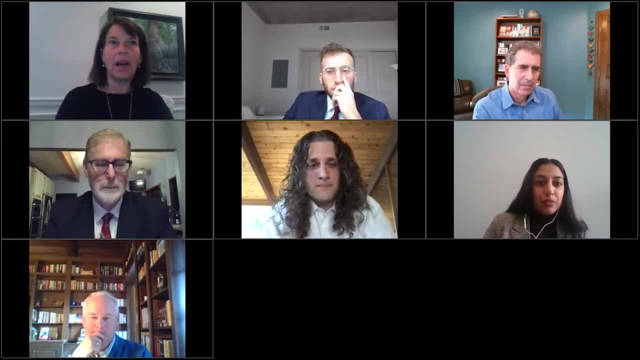 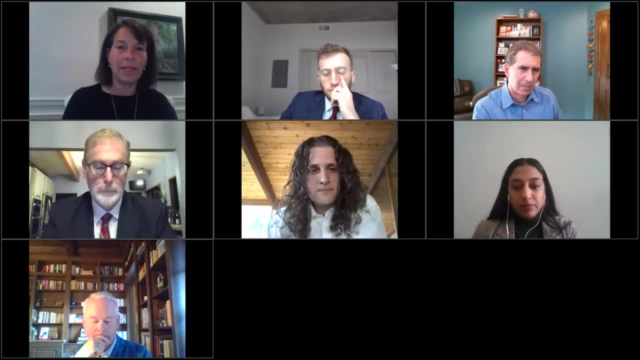 to any questions and I'm going to pass it back to Linda Bina. thank you so much. It's really it's really interesting to hear from your perspective, And I was particularly interested in your observations about the local dynamic, because I do a lot. 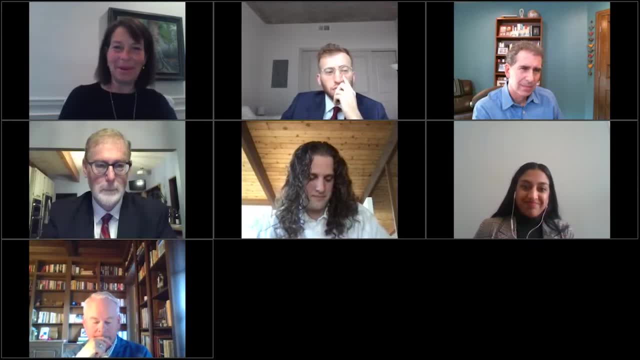 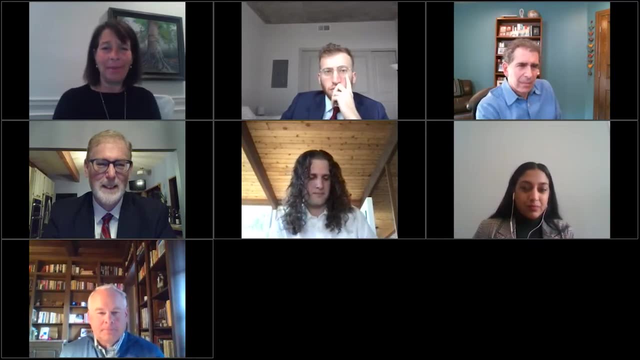 of work here in Nashville at the local level will want to engage with some of your remarks. but we're going to now turn to our second um expert commenter, who i think gets some kind of gold star or something, because i believe he is coming to us. 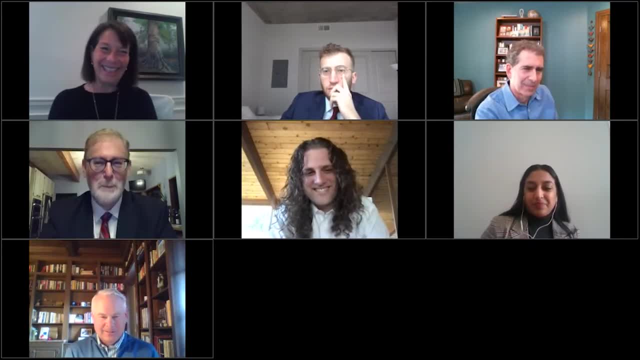 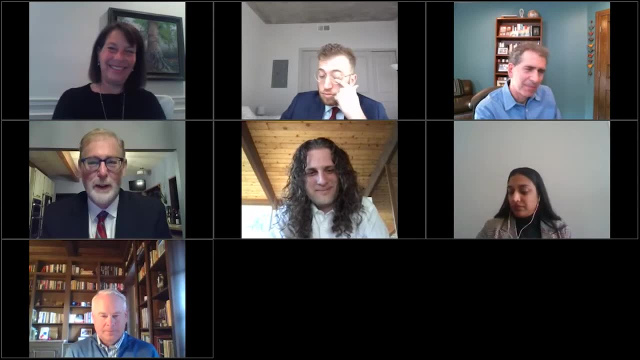 from hawaii. is that correct, howard? i am thank you for being here over to you all right. thank you, linda, and thank you for all those at eli and at the law school who organized the el part forum. bravo, and thank you to the authors for a well put together and provocative paper. it's timely. 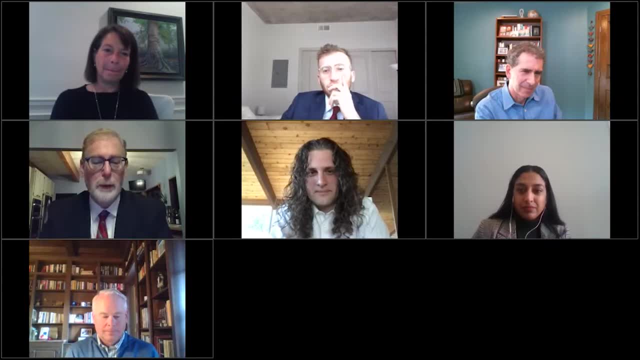 and i really do look forward to reading the final article, which i think will be helpful. in the field. the empirical analysis is helpful, but let me bring you some good news in two regions of the country, excuse me, the midwest and the southeast- which aren't always 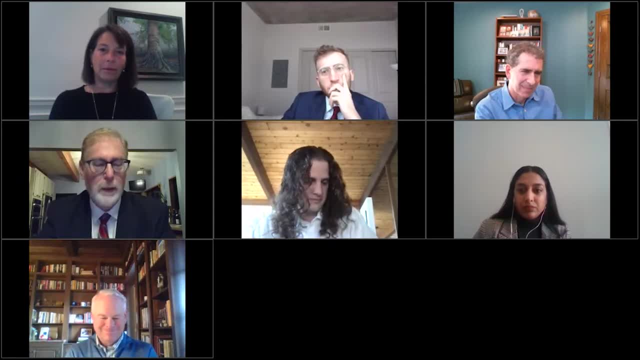 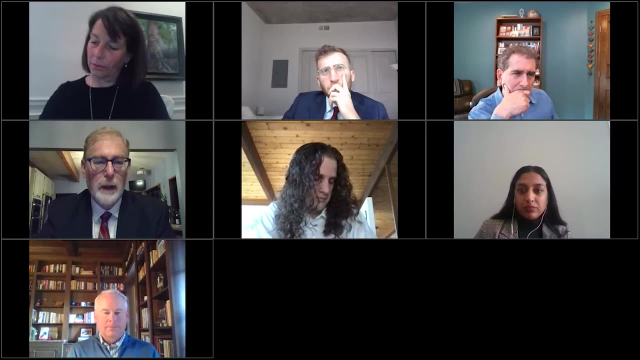 viewed as having especially vigorous state-level enforcement or strong environmental programs. there are a significant number of big deal substantive citizen suits being filed- uh prevailing that involve both actions against private parties and actions against government. okay, these are cases that are retail, but they have high leverage value. 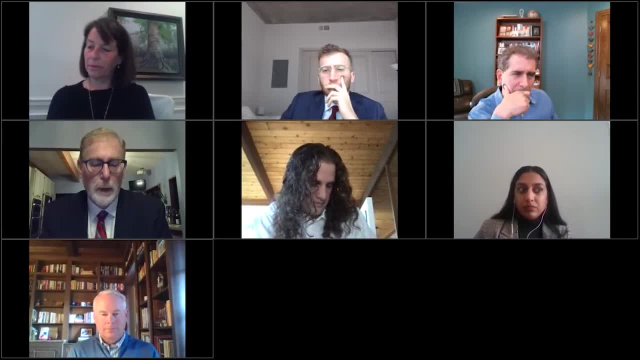 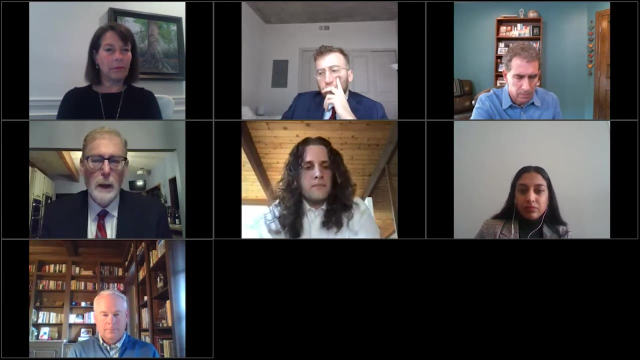 when it comes in the midwest, to clean water and protecting the great lakesapena was talking about local views. These are 80 to 90% plus public issues When you look at what the public views are in places like Toledo, Ohio, Northwest Indiana, Chicago, most of Illinois and so forth. when it comes to the Clean Water Act, when it comes to protecting the Great Lakes, these are not just bipartisan issues, these are nonpartisan issues. 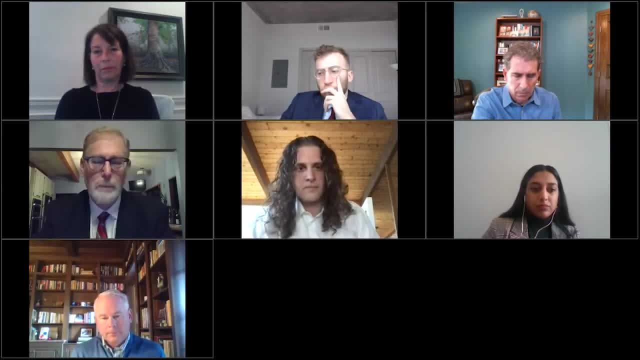 And that's reflected by the congressional delegation in which both Republicans and Democrats have strongly supported protecting the Great Lakes. Okay, so why are all these cases happening? And I'll describe a little bit about what's happening in Indiana, Ohio, Illinois, Wisconsin, Michigan, Minnesota. 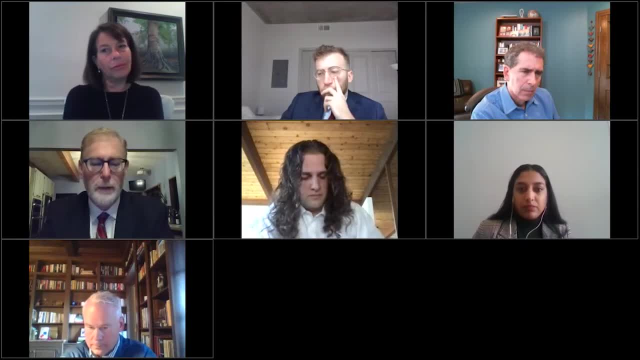 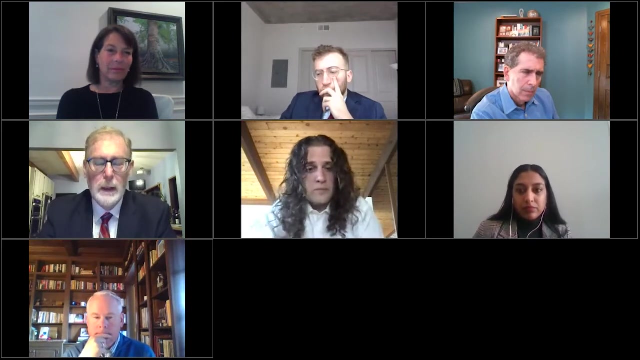 In both regions, the Midwest and the Southeast, there are sophisticated public interest environmental legalists. There are a number of legal advocacy groups that have the legal capacity, strong enough financial base, attorneys who know how to bring these sorts of citizen suits. In the Midwest it's the Environmental Law and Policy Center, but also our good colleagues at Midwest Environmental Advocates, Earthjustice, the Sierra Club and others. 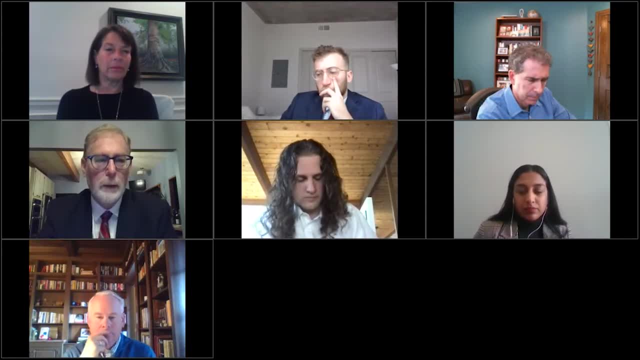 In the Southeast it's the Southern Environmental Law Center and a number of other groups. So when you have a set of groups that bring legal sophistication, reasonably strong financial basis so they can take on a case involving a citizen suit, and folks who are talented at doing public interest litigation, you then have the situation to do the sorts of cases that I'll talk about right now. 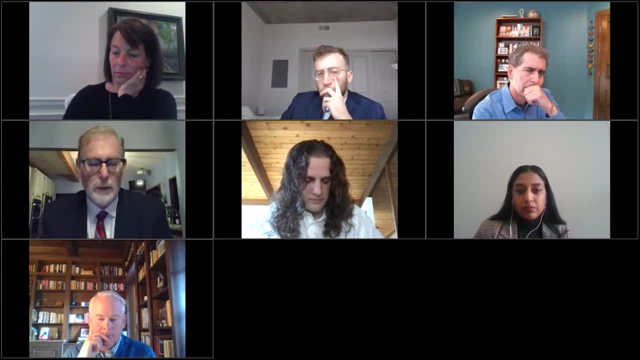 And there is indeed sort of a self-regulating component to this. We are looking at cases that raise the bar. We are looking at cases that raise the bar. We are looking at cases that have leverage value. We can't do everything at the Environmental Law and Policy Center. 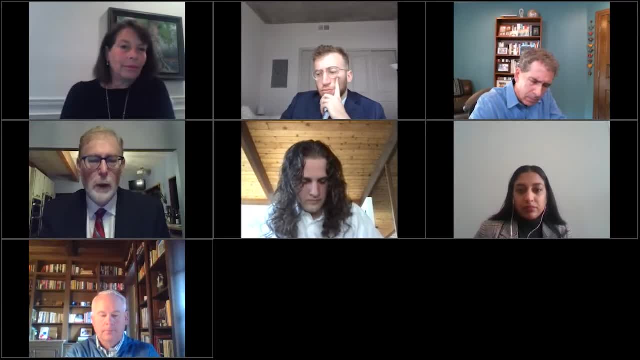 So one of the questions is always: is this a one-off case or does this case raise the bar for others? And one piece of that is one of my former board chairs who is the managing partner of a big law firm, put it: look, my clients want to know that if they do things right, and their competitor isn't that. if the federal government in a certain administration, 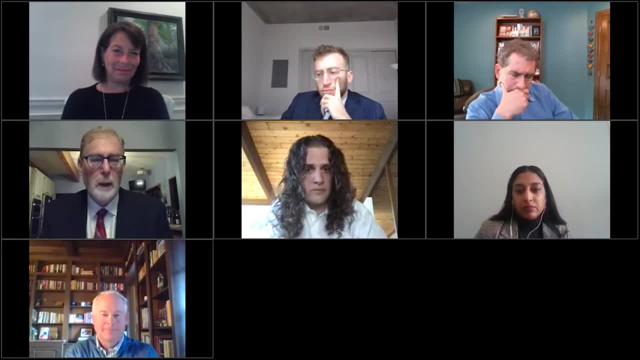 isn't coming after them, that there'll be a group like the Environmental Law and Policy Center or Earthjustice or the Southern Environmental Law Center who does it, because otherwise they're at a competitive disadvantage and they don't want to be in that situation. 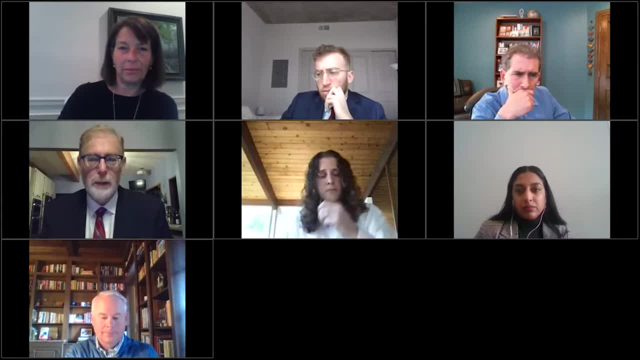 In terms of leverage. no general counsel, no CEO of an industrial polluter wants to be seen on the front page of the newspaper being labeled as a major polluter of the Great Lakes. I mean, that's just nobody. Nobody wants that. 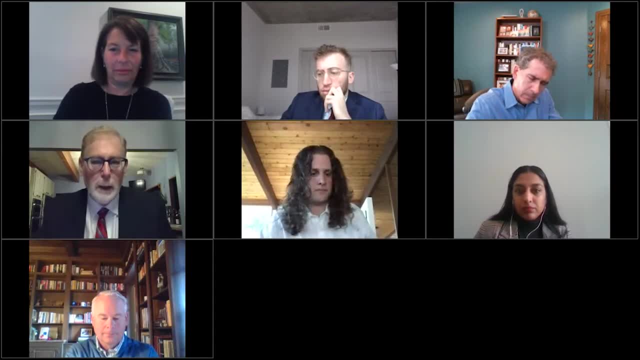 And that is some leverage and that's part of the game. That's part of how do you play effective citizen suits. So let's look at some of the current litigation on our docket- and I'm not going to go through all of it, but I'll give you some examples. 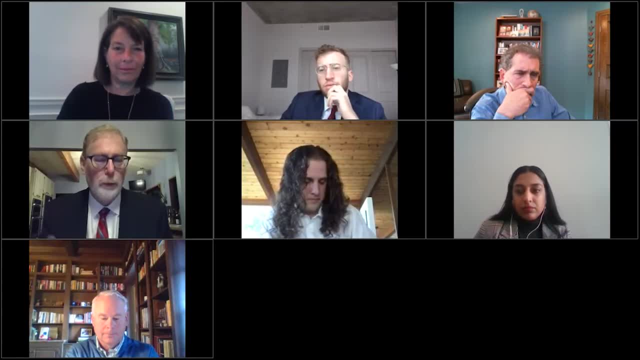 Indiana, not a state that is well known for strong environmental programs or enforcement. I don't have a reason to take a shot at Indiana. There's some very good people there, but it wouldn't come to most people's top of the list. 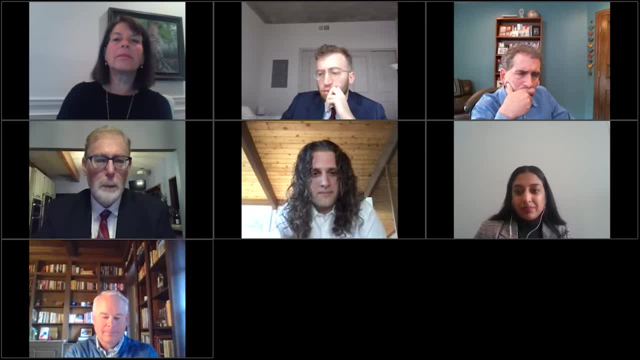 When they say: here are the strong programs. The Environmental Law and Policy Center and the Hoosier Environmental Council brought a Clean Water Act citizen enforcement suit in the US District Court for the Northern District of Indiana involving ArcelorMittal, now Cleveland Cliffs. ammonia and cyanide pollution of the Little Calumet River that went into Lake Michigan. 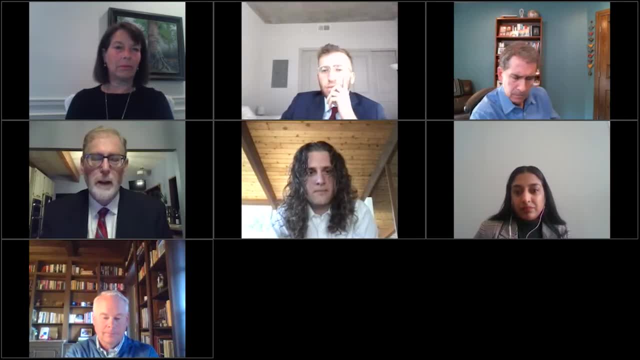 The company didn't say publicly what happened when it did 72.. 2 hours when dead fish- 3000 dead fish- started showing up in the East Arm of the Little Calumet River and Lake Michigan, people knew something was going on. 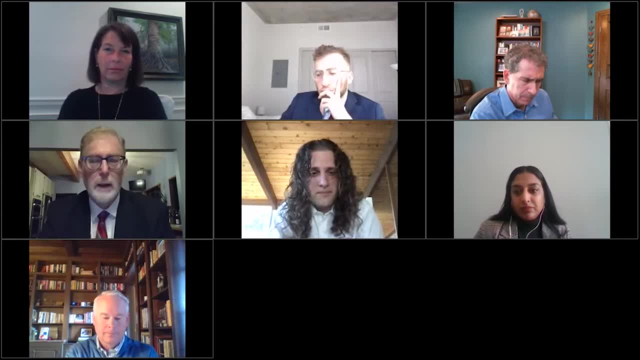 They finally acknowledged there was ammonia and cyanide that got into the waterway, that were spilled out. First aspect of bringing a citizen suit: You can file a 60 day notice letter, which is required under Clean Water Act, Clean Air Act and so forth. 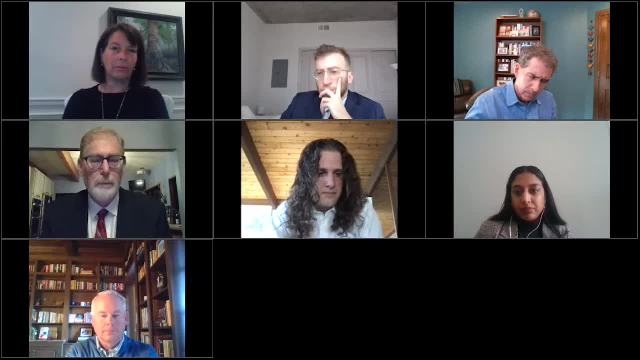 But you need to spend some time Negotiating with the state attorney general, the state EPA and the federal authorities, because otherwise you're in the risk of, at day 59, the federal and state government step up and bring their own enforcement action. 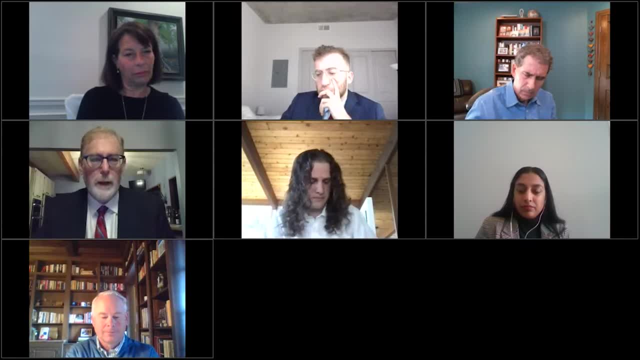 Now, that's not bad. We want the federal and state governments to do a very good job of enforcement, but we also want to make sure that if they're going to do it and over file, that they really do it. Well, okay, so that's a negotiation. It's a matter of making sure that if there is over filing, it's really going to be vigorous and effective enforcement And it for whatever reason. the federal or state government aren't going to do that. You want to make sure that they get out of the way so that the citizen suit can be brought. 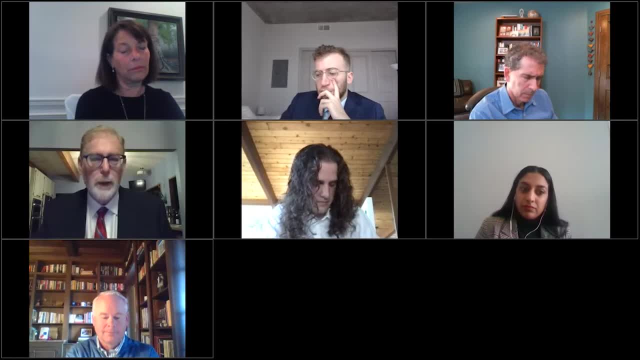 So the best situation is the federal and state governments do it and do it well. But if they don't, that's the role of citizen suits under the Clean Air Act and Clean Water Act And the other environmental law. So we're going to make sure that we're doing that. Okay, Thank you. Thank you, statutes. you've got to work that within the 60-day period. um, you know, just without going chapter and verse in that lawsuit, plaintiffs, citizens groups brought that lawsuit. it was on the front pages of the newspapers. turned out that there were a lot of permit violations. 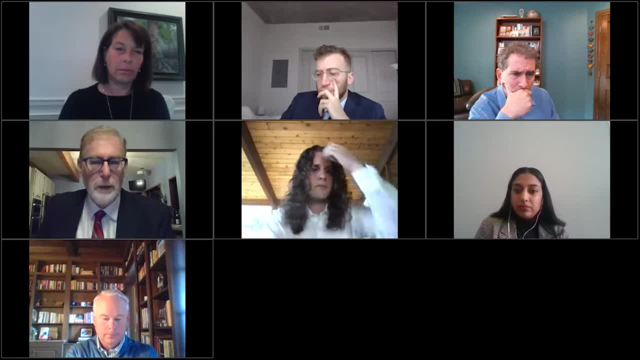 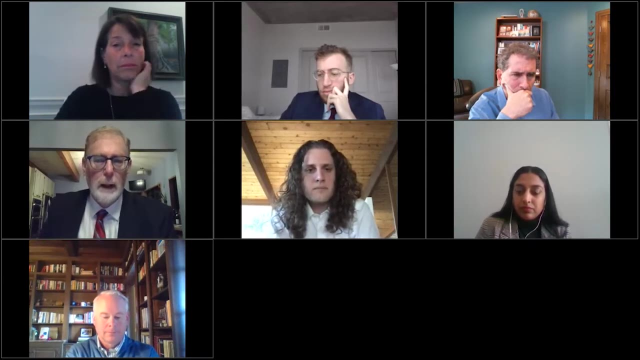 we believe they were significant. the defendants believe they were less significant. two years into the litigation, the federal and state governments decided to step up and move forward. there's now a consent decree that's been filed, more than three million dollars of civil penalties, some additional environmental programs, including 127 acres of land that will eventually 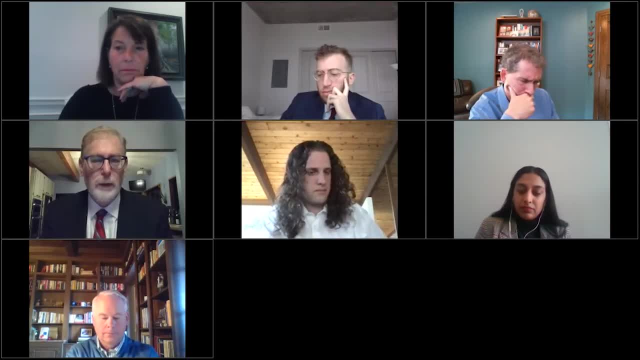 be donated through a land trust to expand the indiana dunes national park. a series of provisions involving injunctive relief by which cleveland cliffs has to fix their steel mill, improve the conditions, better equipment that are, operating facilities and so forth, and protocols and there. 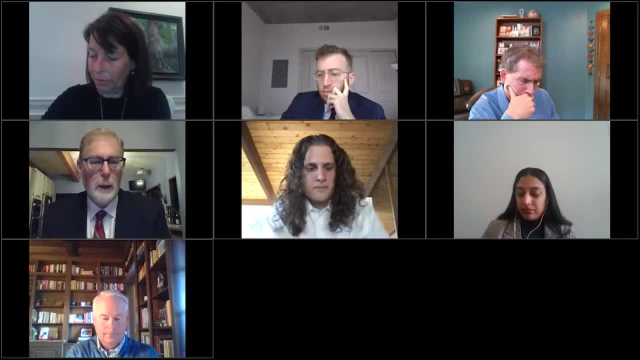 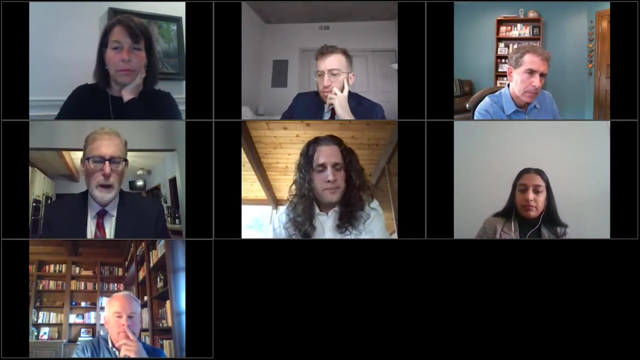 is almost a million dollars of attorney's fees going to the environmental law and policy center is having brought the citizen suit action. so i mean this is a big deal case. it has retail value in the context you're talking about, but huge leverage value in terms of every other industrial. 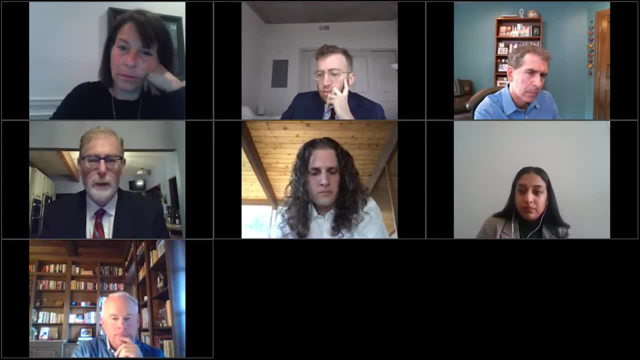 facility along the lake michigan shoreline looks at this and says we don't want to be in this position. so that's the leverage you get out of it, not just for one huge steel mill but for the others along the way who look at and say, yeah, we better make sure. 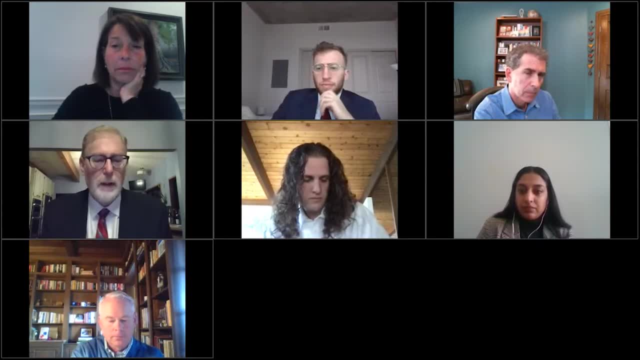 that we're doing things right. it's not just indiana. we have clean water action suits involving the federal government and agricultural interests involving nutrient runoff pollution into western lake erie that's led to severe toxic algae blooms every summer. that's about as substantive as you. 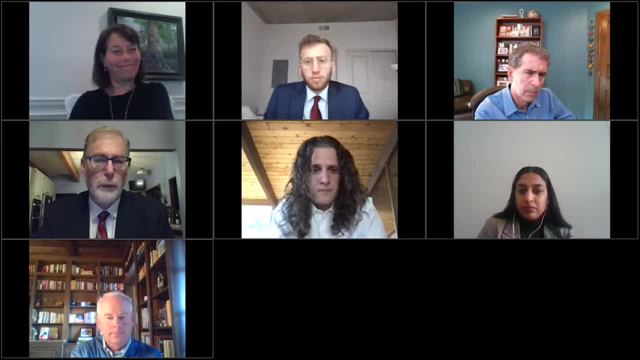 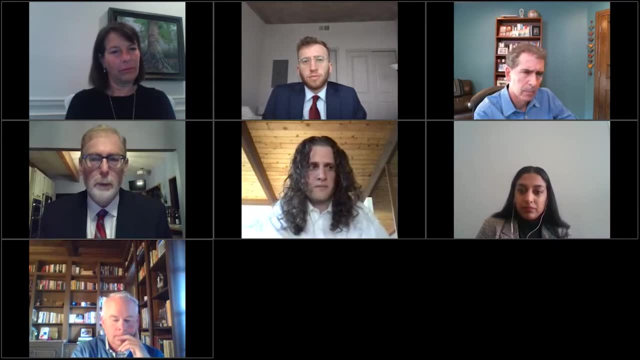 can get. lake erie is sadly the poster child for severe recurring toxic algae blooms. this litigation which we brought is designed to help clean that up. over time we've won some pretty significant victories. we're moving forward at this point into a potential consent decree with the state of ohio and the federal government clean air act in. 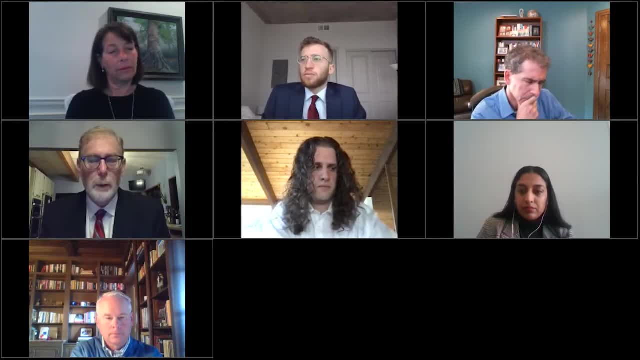 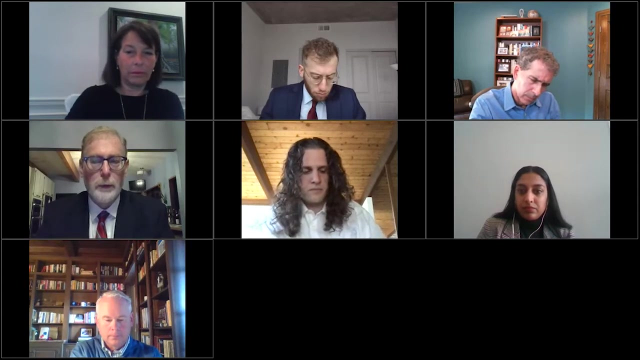 addition to the consent of the president of the state of ohio and the federal government, the state has a number of Jake wisconsin involving the laws designed to protect national wildlife refuges and nepa clean air act enforcement suits in illinois against vistra in peoria for its old edwards coal plant. 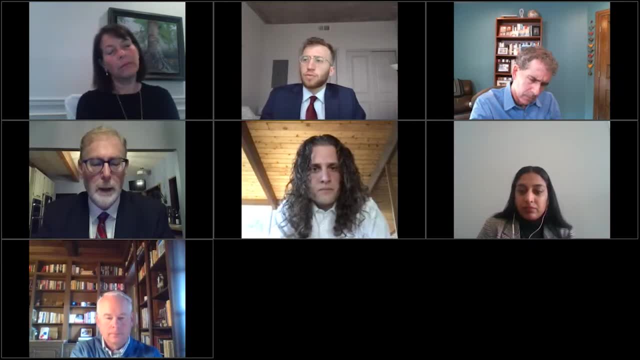 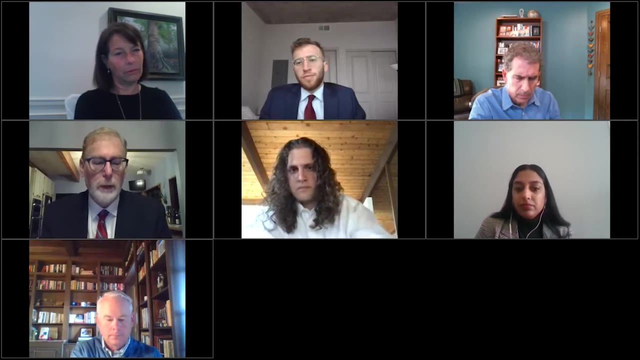 violating opacity standards, too much particulates being admitted into the air. suits in michigan as well. um, an ozone action in the dc circuit, because that's where it needs to go. these are all substantive. they're a mix of private parties and governmental defendants. they are all in most cases. 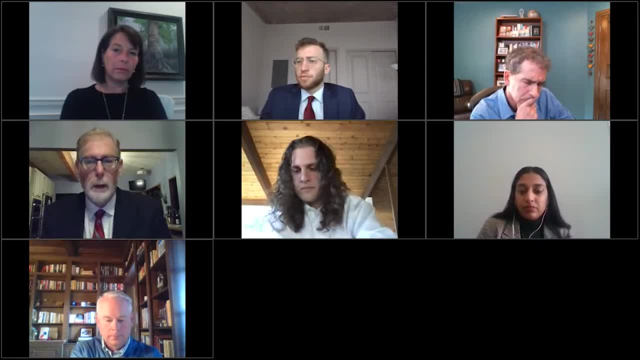 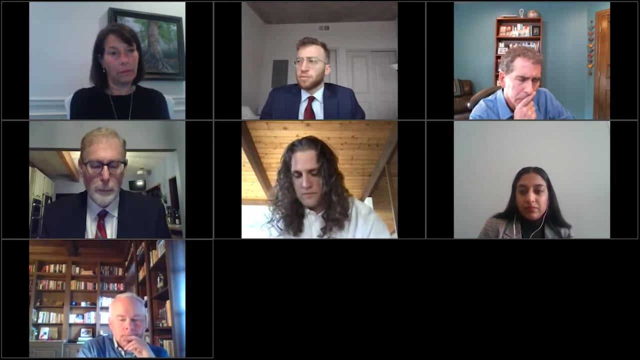 very publicly visible, which increases the wholesale leverage value beyond the retail and leads to other defendants and other corporate counsels saying: uh-oh, are we going to have this problem at our plant, whether it's air pollution, water pollution or other things involved. importance in terms of the role. 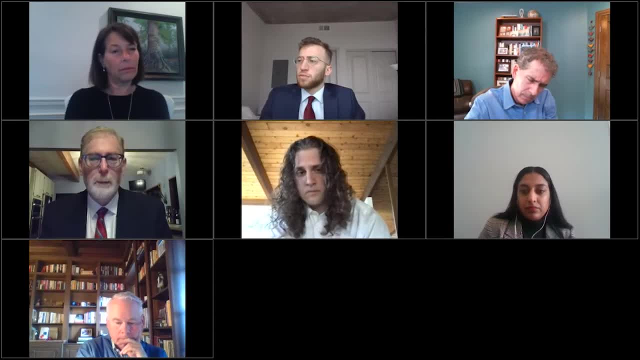 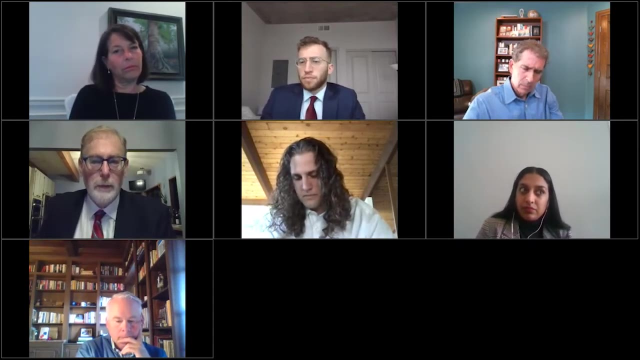 of the federal government, as we all know, sometimes we have epas and dojs who are vigorous in enforcement, and other times less so. as i said before, we want federal and state governments to be tough, bare, effective enforcers, but when they're not or when they just can't take. 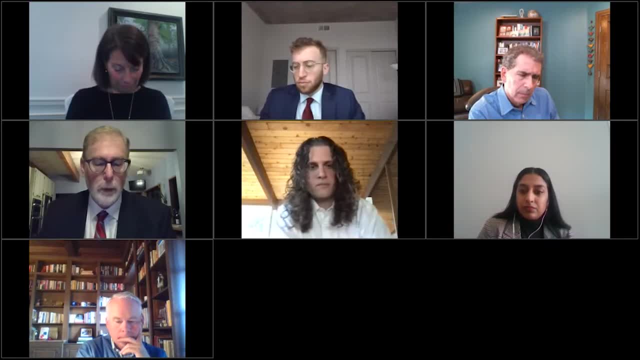 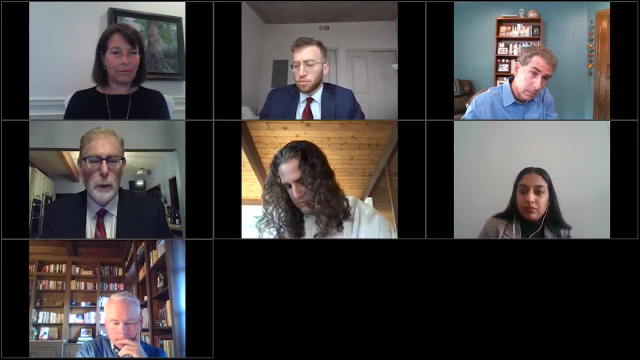 on a particular matter. citizen suits are extraordinarily important. so some factors you might look at as you move, david and jory, to finalizing your article. first of all, think about you know. on the numbers, how do you value what i'll call some of the bigger cases that have a lot of leverage, uh, versus what i'll call deadline cases that are filed? 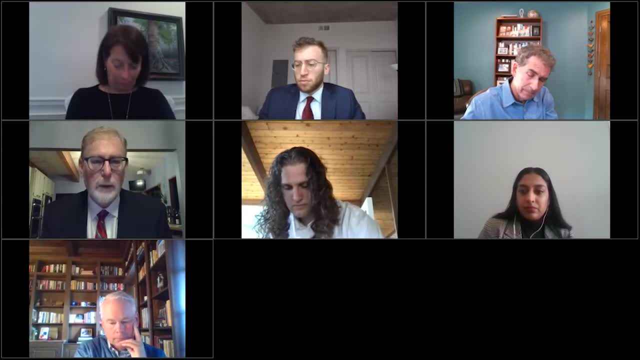 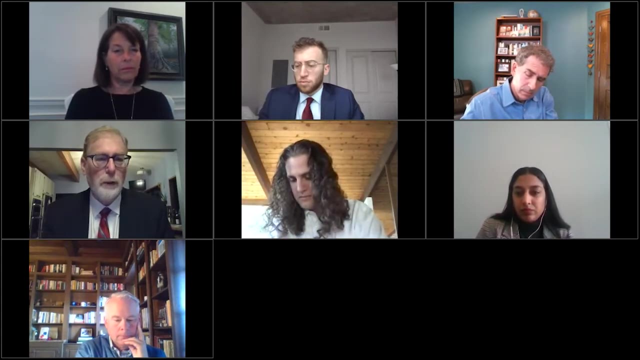 that are much more um, tactical, uh, in terms of moving something forward. i don't know quite how you do that based on the data you have. let's recognize that there is a difference there. secondly, look to the resource question of who has the capacity to bring. 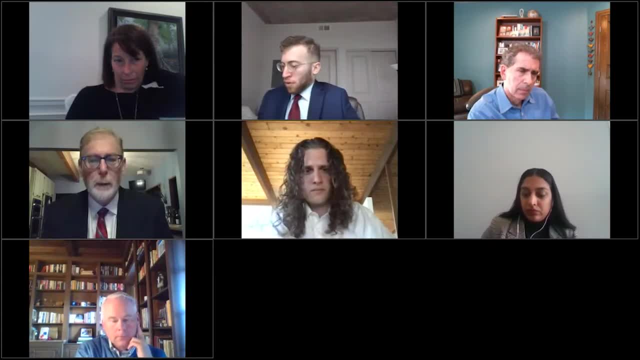 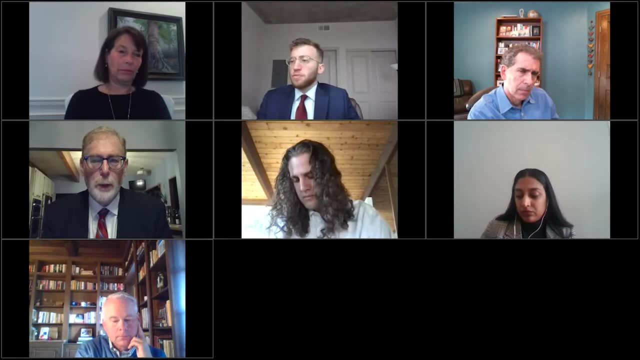 effective citizen suits of the substantive types you're talking about, involving private parties as well as governmental defendants. that tends to be places where you either have offices of the national environmental groups, such as in california, or places like the southeast or the midwest where you have groups like the southern environmental law center, the. 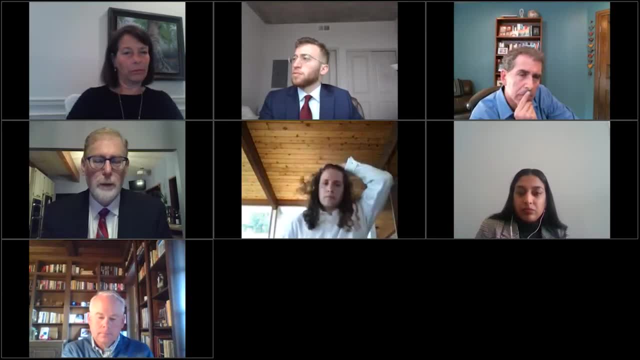 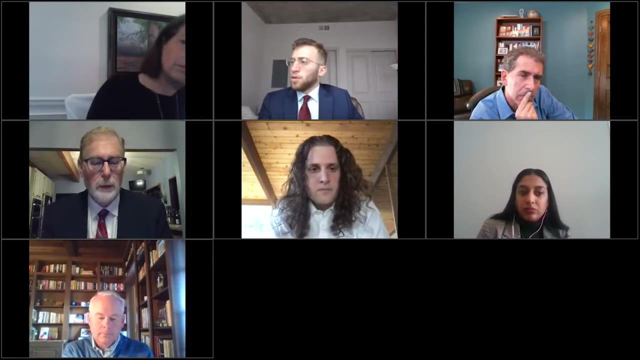 environmental law and policy center and groups like earth justice or edf um having an office, or good state groups like the great lakes environmental law center or the midwest environmental advocates or local chapters in sierra club that have had a litigation history, and those groups have to have a solid enough financial base. 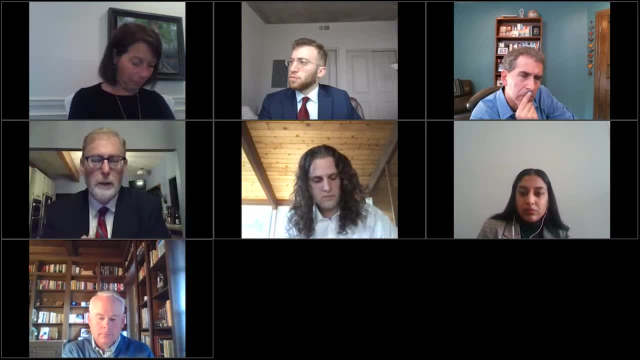 to be able to bring these people into the workforce so that they can bring these lawsuits, because nobody can look at this as attorney's fees alone are going to wind up supporting this work going forward. attorney's fees are mana from heaven. we don't budget them going forward, we look at them. 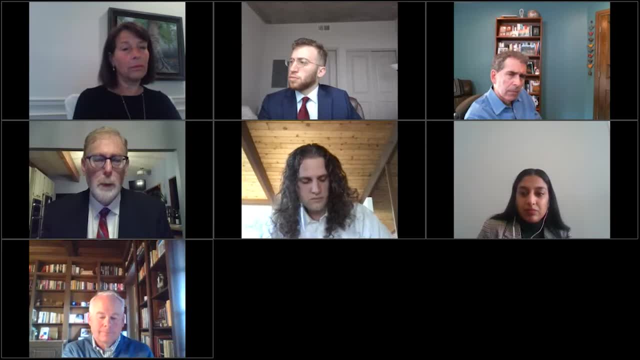 as being an important part of our strategy. but when we get fees, it's episodic. it's somewhat unpredictable what year we're going to get them opposed in court, sometimes not. Sometimes judges look at them as being entirely justifiable. Sometimes judges have a lot of questions about it. There's a question of what rate is used and 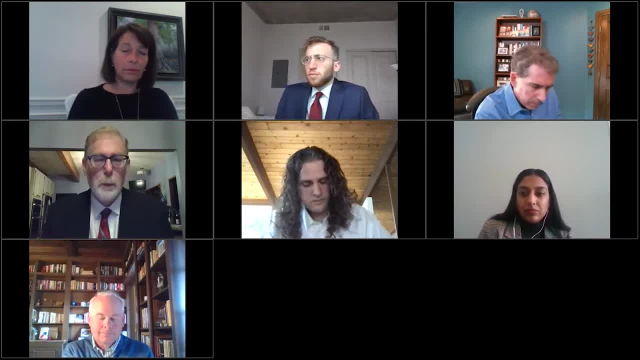 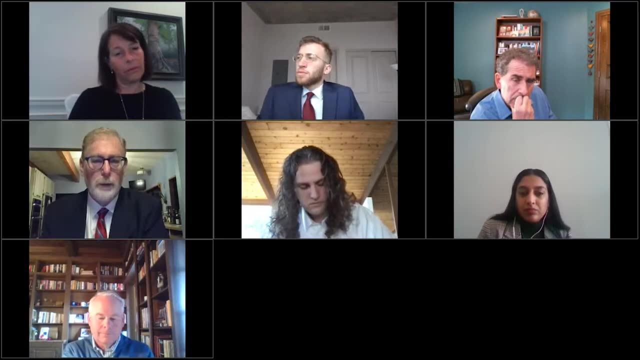 so forth, how many hours versus how long you litigate it. Your points about ways of reforming to make more predictable attorney's fees award I think are important to your analysis, Because when you have the attorney's fees award, that really does provide some incentive. 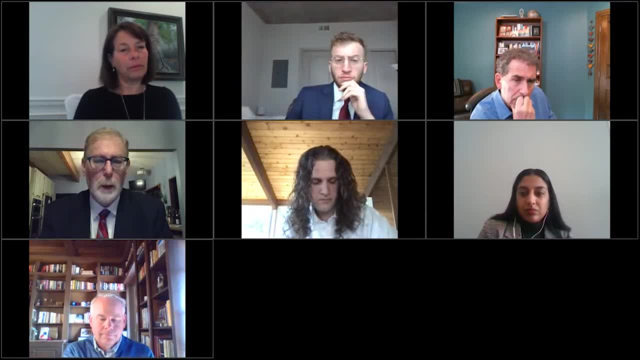 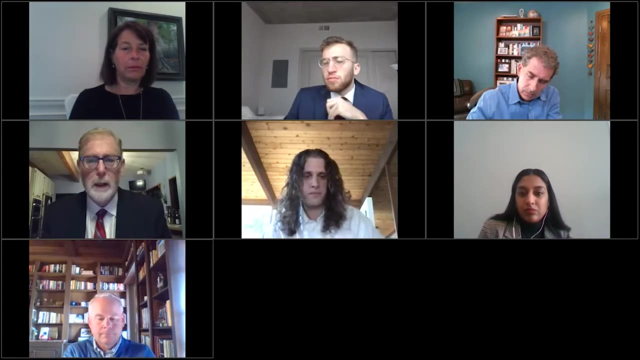 for both public interest law organizations and private parties to bring citizen suits, knowing that they have a meaningful possibility of serious attorney's fees being awarded. That shouldn't become as difficult as it sometimes is, and it shouldn't necessarily become the ancillary litigation that it occasionally becomes. 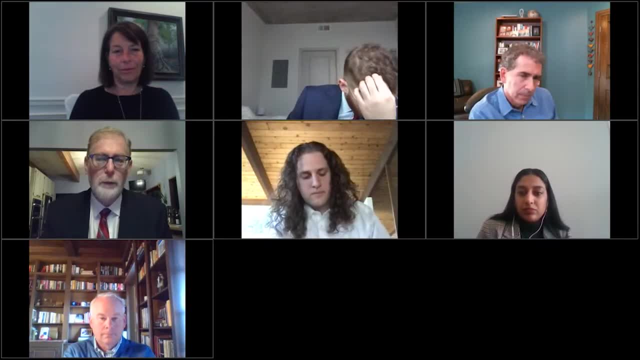 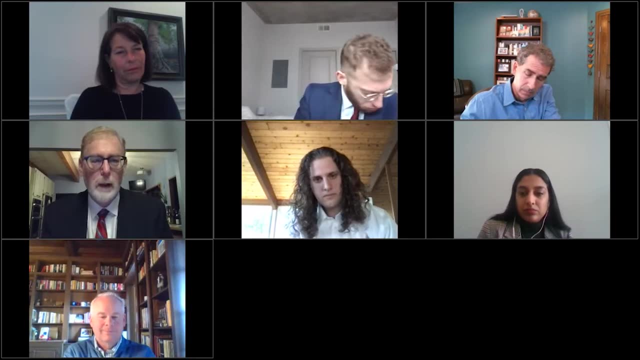 You're. When we get attorney's fees, we're entitled to, if you will, fees on fees. if we need to battle the attorney's fees, Frankly I prefer not to go in that direction. We do it when we need to. 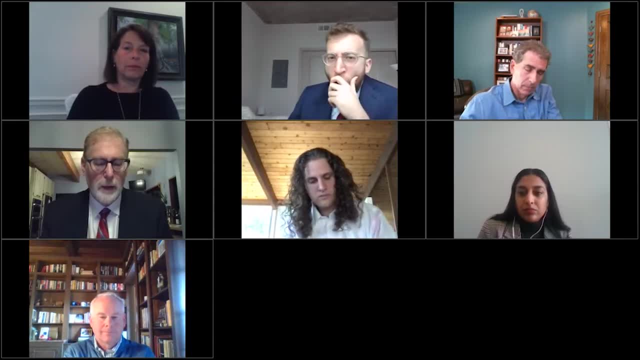 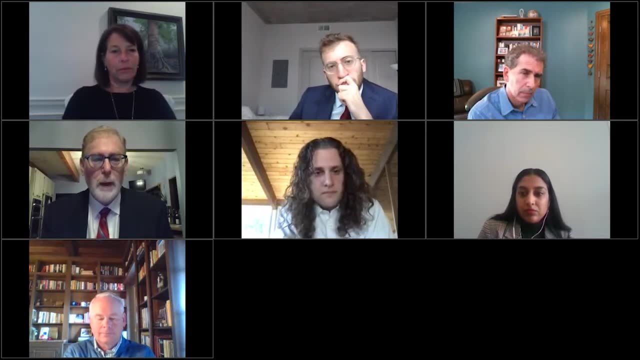 but we ought to be able to find a way of resolving it without having ancillary fees on fees battles. But in short, citizen suits are important, We all recognize it. And they're especially important where you have, for whatever combination of reasons, in particular years, particular administrations. 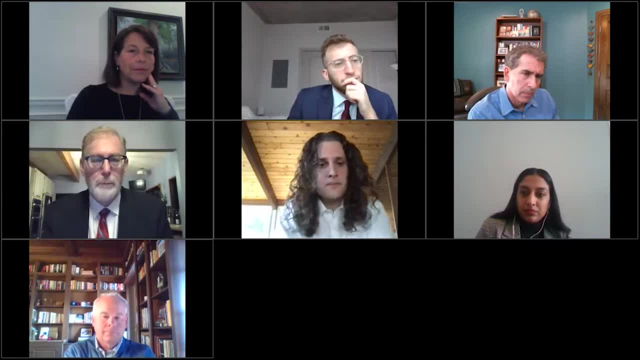 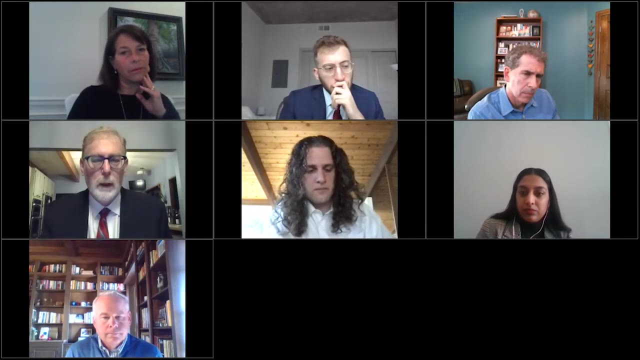 either federal governments or state governments that aren't stepping up when it comes to tough but fair and vigorous enforcement. We need to make it work better, But I think the system, in some places perhaps, is a little bit more aggressive in terms of qualitative impacts. 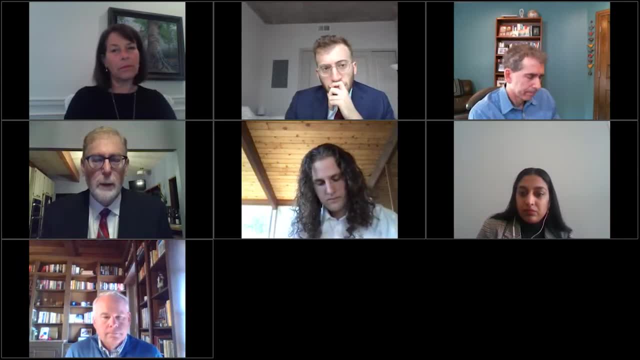 substantively than some of the numbers you have may indicate in terms of numbers of suits, And I get it from your analysis that because the DC Circuit is where so many cases need to be filed, of course the numbers will be higher there. 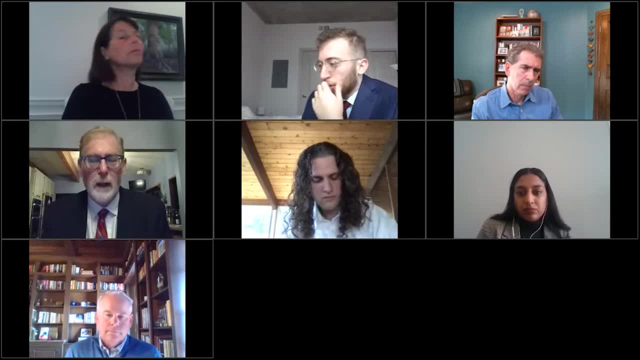 And the Ninth Circuit in some ways is something of a special case. I'd encourage you to look at- if you take out the Ninth and DC Circuit, what are the differences that you're seeing between the other circuits that seem to be relatively flat in your graph. 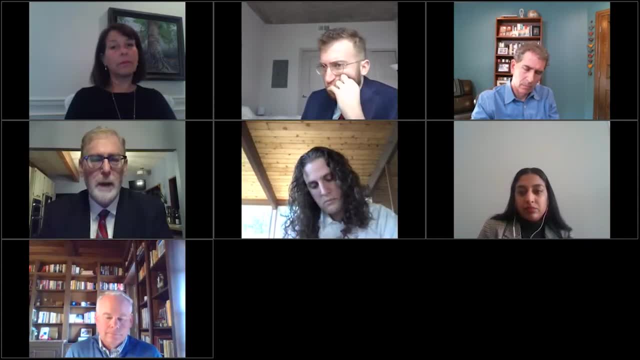 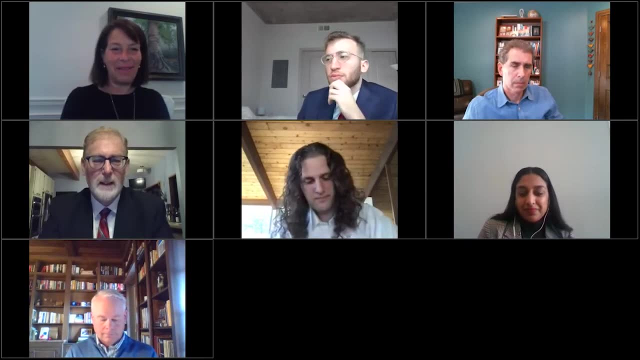 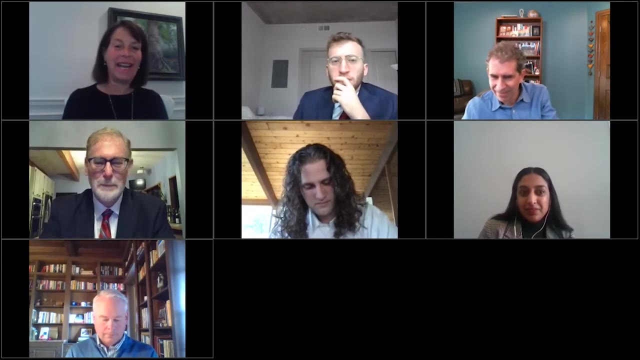 Are some of them more or less in what types of suits? But thank you for your work on the paper and thank you to you. And thank you for taking the time from a vacation in Hawaii to join us. Really interesting to hear your on-the-grounds take on the data. We have some great questions coming in, but I do want 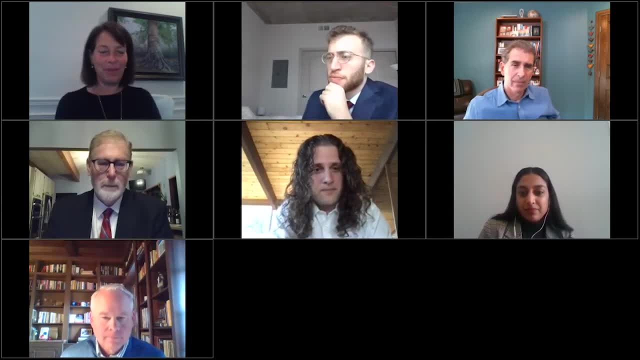 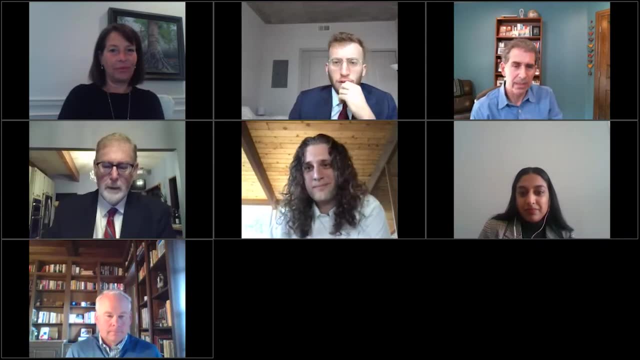 to give the authors a chance to respond to what they've heard, So I'm going to hand it back to them to comment on the comments. Okay, great, So I'll, Jerry, I'll just respond to a few things and then we'll get back to you, Thank you. 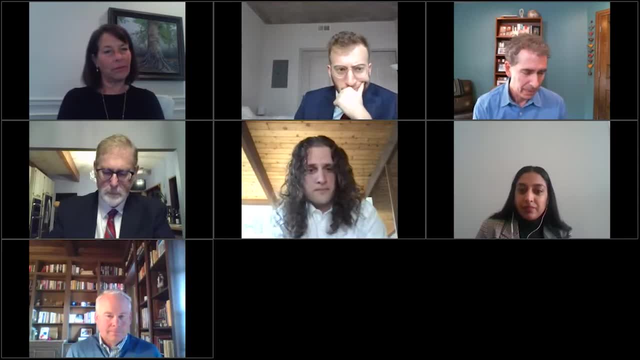 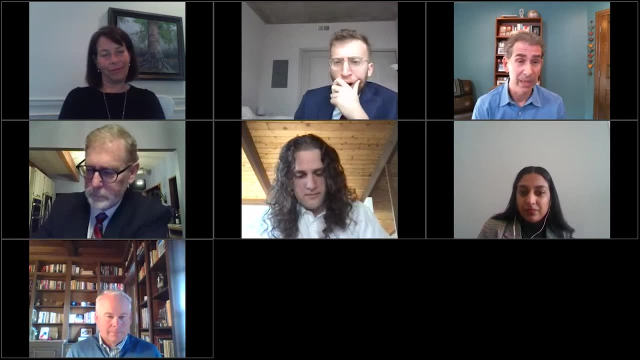 And then you should weigh in as well. First of all, these are really really valuable, incredibly helpful comments that both of you have made, and really appreciate them. I think one of the hardest things in doing this type of empirical work is, you know, raised by 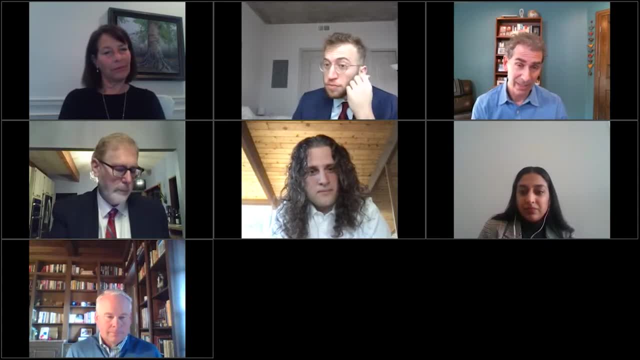 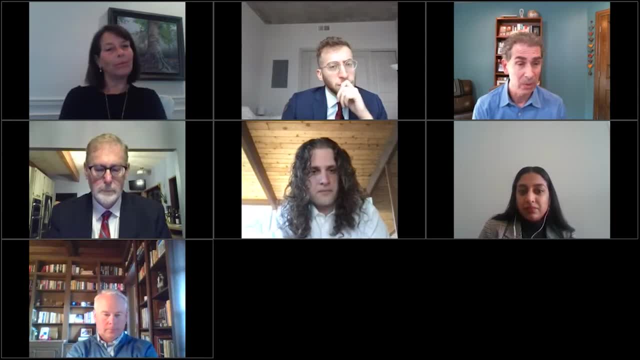 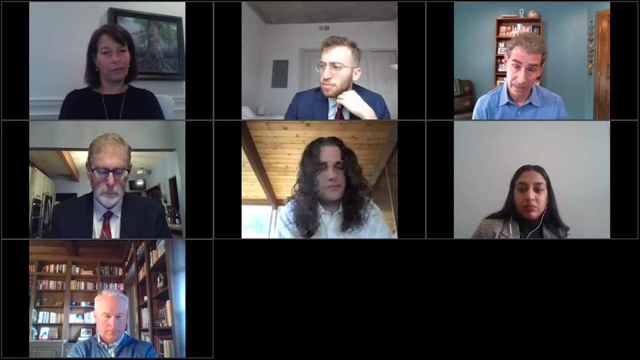 if we wanted to go back to the data, you might be able to categorize cases in a more nuanced way. that would capture the nature of the claims that are being made. For example, if it was an interpretive question, that would have broad implications that would apply to many different 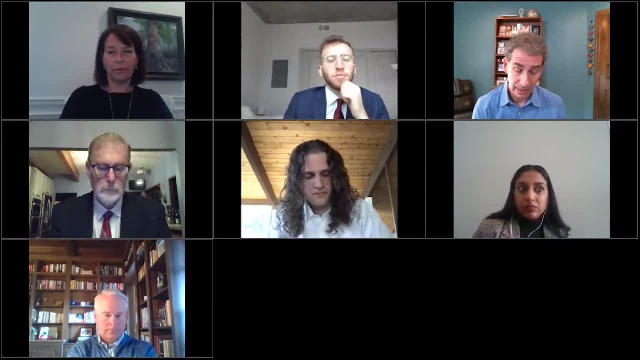 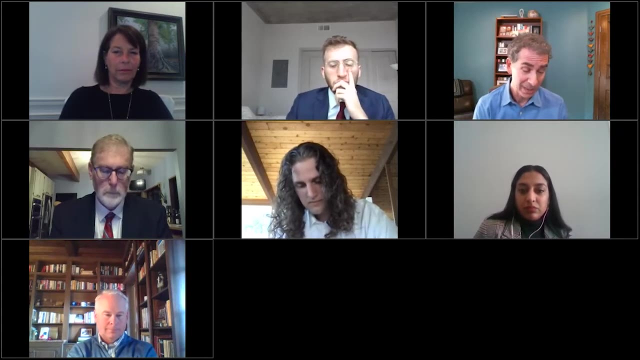 facilities that we might try and weigh that or at least categorize it differently than sort of narrow cases involving specific violations of a standard and a permit. And so I guess more than anything I want to sort of cop to. yeah, that's a very hard thing to do And in some ways I think 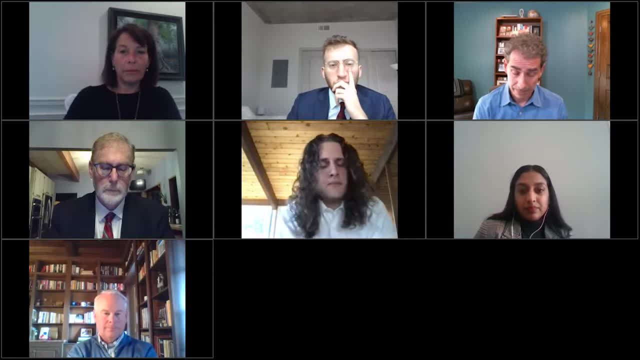 you guys have given us some ideas about how we might, we might think about that. One question I sort of had was if there was some way that when you have kind of impact litigation like this that comes down that observably alters the behavior of other entities, And if there were some. 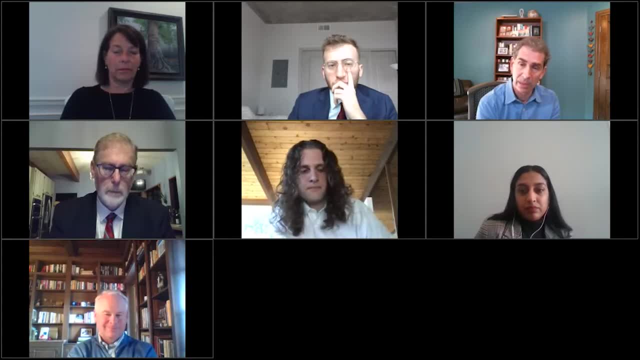 way for us to obtain that information. that would also be a way for us to sort of you know, look or value or weigh the impact of a specific case. I don't think it would be easy to do at all And I guess the question is how visible or how, whether you could. 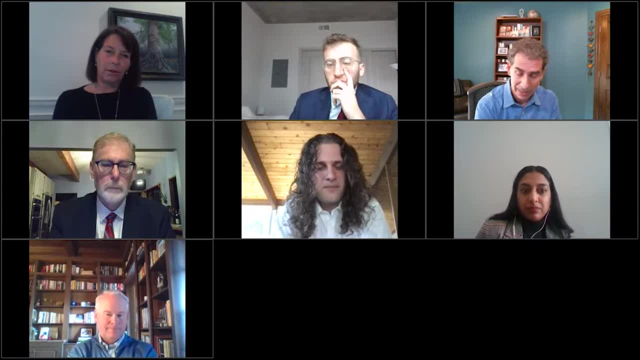 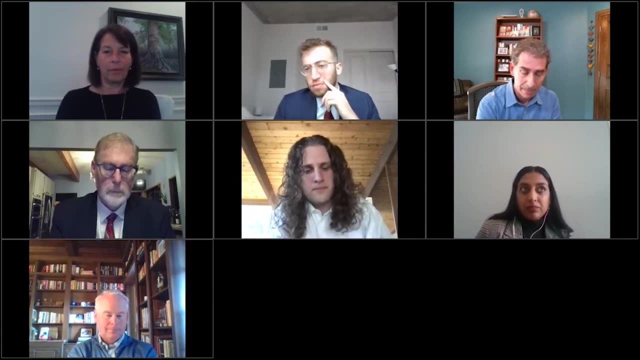 quantify that in any kind of meaningful way. But that was like one thing that came up for both of the comments that you guys made. So you know, I really you know it's interesting to me. So in part, what you're sort of arguing is the dichotomy that we're drawing between kind of wholesale 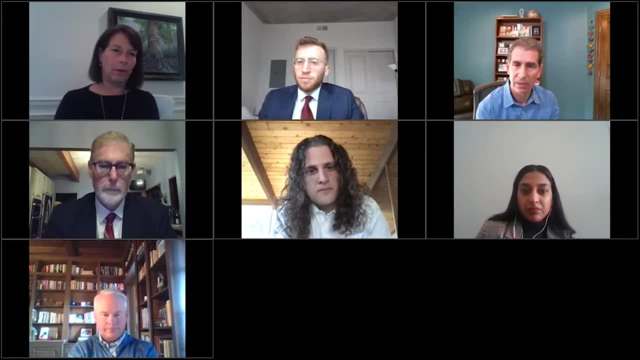 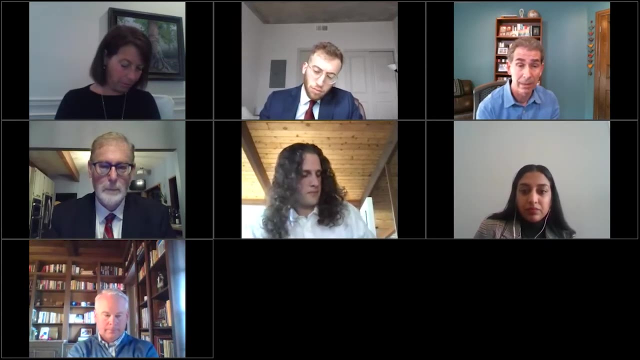 litigation and retail litigation is somewhat false dichotomy, because the costs associated with bringing these cases almost invariably one significant leverage, And so it's not going to be something, a case that is going to be be rare for it to be delimited to a specific facility, for example, just because the you know, Howard, I think 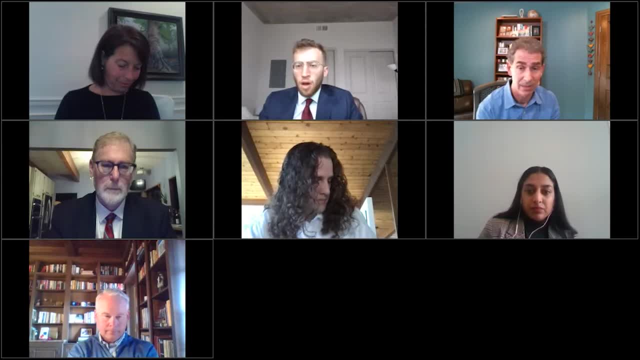 you've alluded to this, to the leverage isn't there, given the cost of of undertaking these disputes? And again I that makes sense to me And in some ways it sort of shows you guys are highlighting, I think, more precisely than we do in the case, just how important leverage is. we see that reflected. 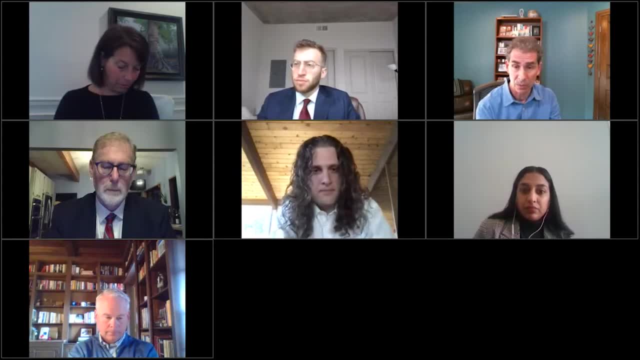 in the balance between you know what we're referring to as wholesale versus retail cases And you're saying: actually the balance is even skewed more towards wholesale, like litigation, because leverage is so important and resources are so constrained. And so in some ways, I think 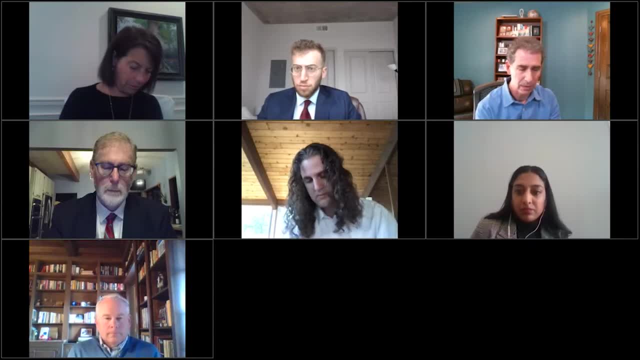 that's a nice, more maybe nuanced way that you're suggesting that we should understand even the more retail litigation, but in some respects it's sort of consistent with the story that we're, that we're telling. With regard to alignment with local views, Again, I hope that. 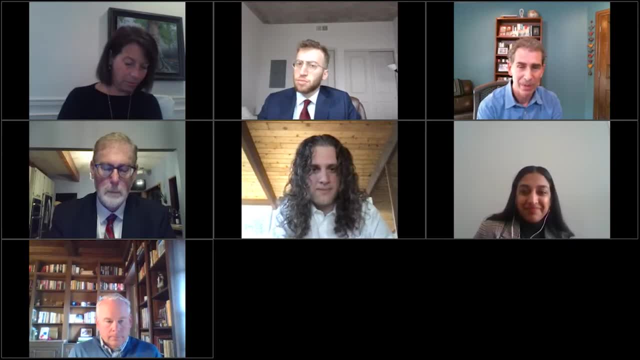 we were reasonably qualified in the sort of the limited data that we had available to us And- and I guess all I can say is I hear you and we certainly didn't want to open, overstate that point- I think maybe at a really broad level we're seeing, you know, cases being 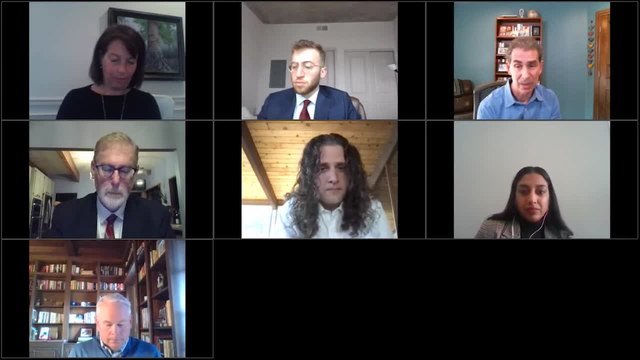 more consistently brought, certainly in states that have reputations for having kind of more robust implementation of environmental regulations and policies. I think that's fair. But the sort of more local differences and conflicts, I think that's really interesting And again it would be. 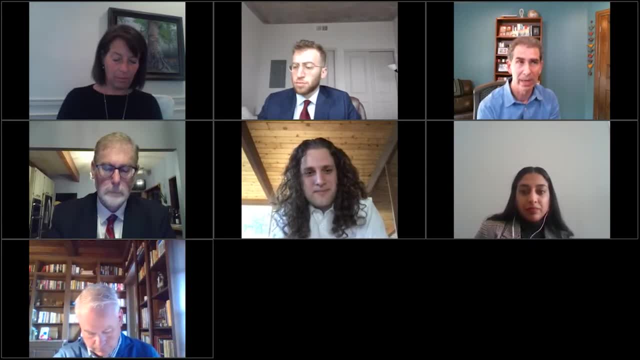 interesting to think about whether there would be some way in which we could capture that More systematically in, in even trying to do an empirical study of it. Why don't I stop there? And, Jori, why don't you? Why don't you weigh in, cuz, I think. 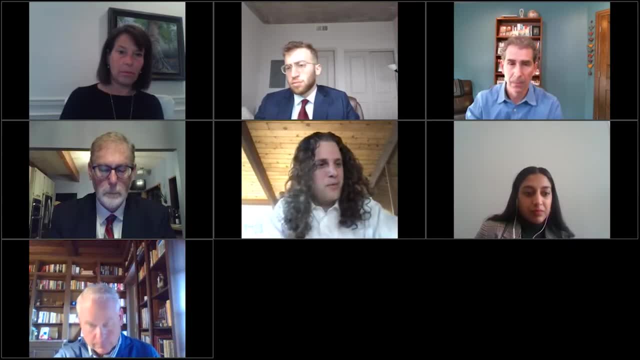 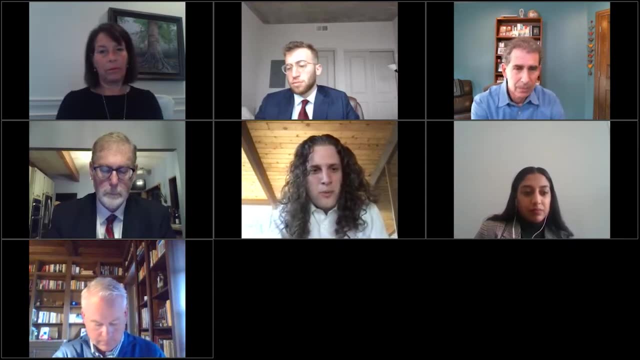 yeah. so I want to quickly give a little bit of a peek behind the the curtain, as it were, on how we thought about the question being that you raised on dealing with what does it mean to be aligned with local interests? Because I thought that you made a really great point And I 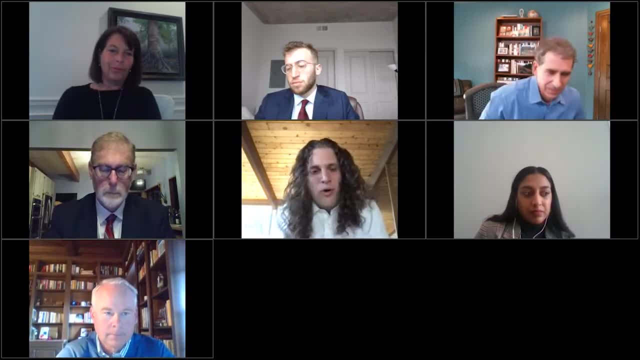 might. so one of the most challenging pieces of your presentation is this question, which I think pieces of all of the types of categorization, when you get right down to dealing with these from the initial point that David was raising about: how do we develop a metric for understanding? 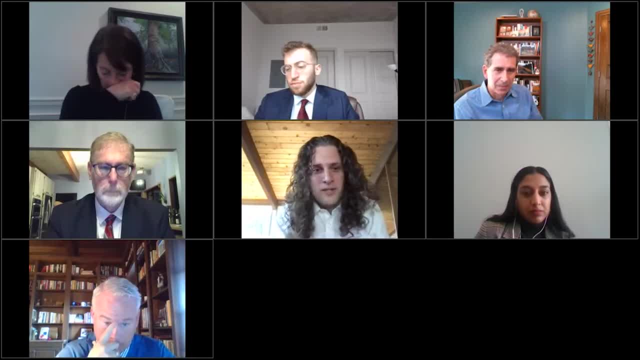 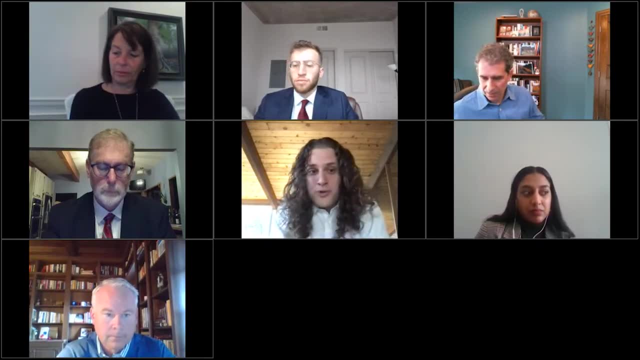 what is the relative merit or impact of a particular piece of litigation in the grand scheme versus what is a less impactful piece of litigation, and also developing these metrics for how to judge or ascertain, kind of even a basic understanding of what is a local preference or 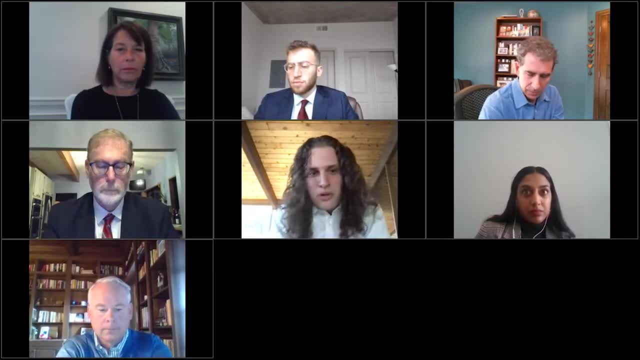 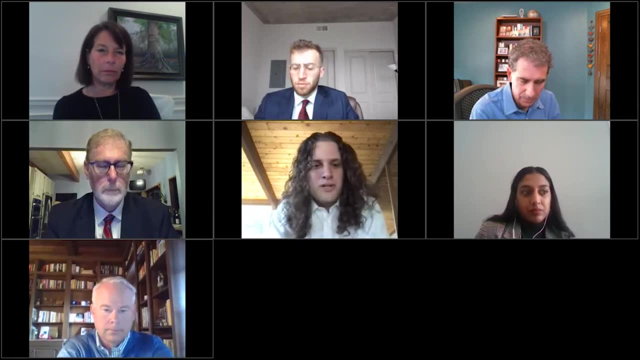 what is in some way aligned with the parochial interest of an organization. And, to Howard your point, I think we did spend a bit of time trying to think about where are these organizations that have the resources to conduct these litigations situated, and it is a very challenging. 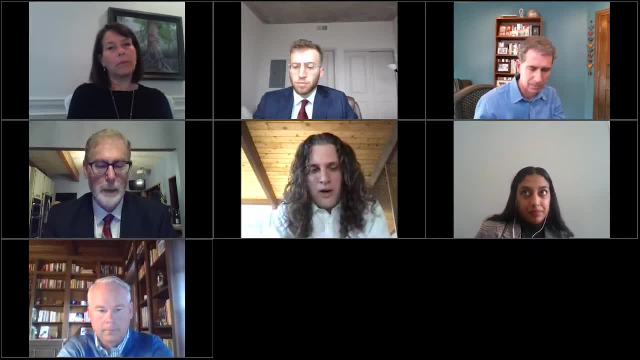 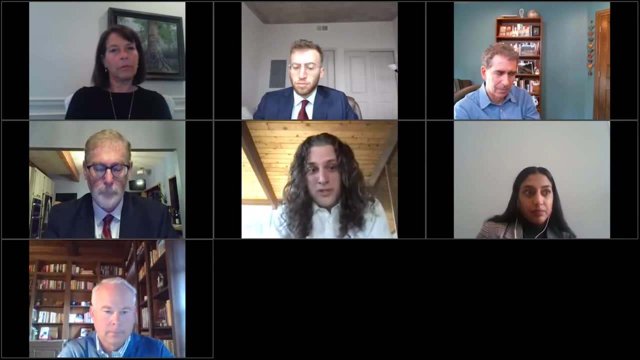 thing to find any kind of data on this. So you're left in a lot of ways, with kind of more aggregated data. Oftentimes you're resource limited, So for us at least it would have been. I think you probably could ascertain. 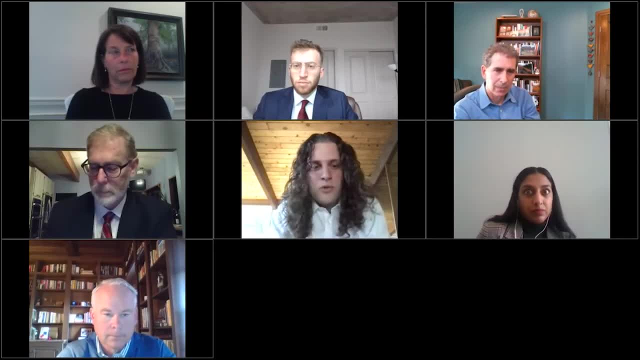 for example, some political data you can fracture down all the way to census districts or voting districts or whatnot. So we could probably look to that. if somebody had enough resources to really dig in and try to do an analysis, to fracture it down into the pieces, I do think there might be. 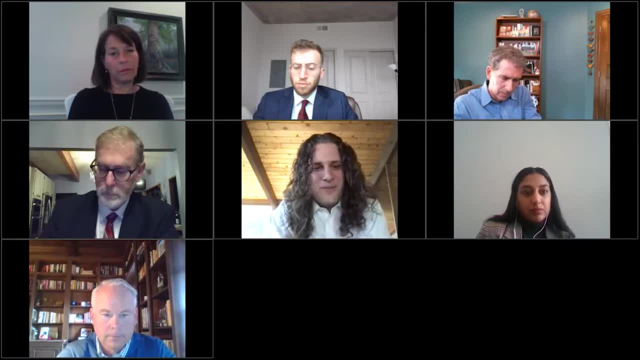 some data there. I would be very interested to see if, in a subsequent analysis, somebody could come up with a metric that better kind of fixes it, because we did spend a significant amount of time when we were initially drafting it batting back and forth around lots of different ideas about what kinds of data that is. 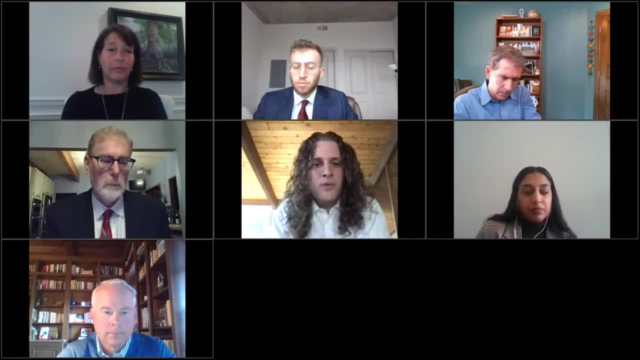 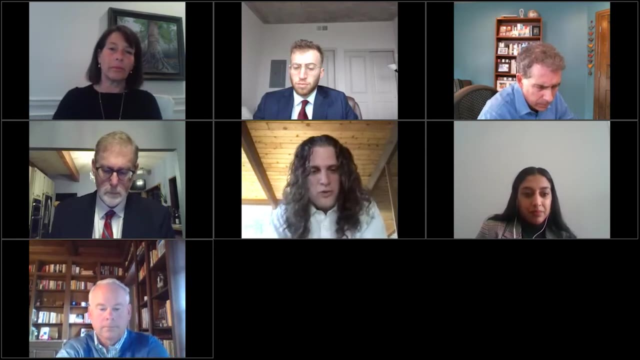 available might be a good proxy for either the particular local support a NGO might have or the particular local support that might exist for the type of environmental litigation that was being done. So just putting that out there as the first piece- And I do think a lot of this highlights a lot of the comments- highlight one of, I think, the central. 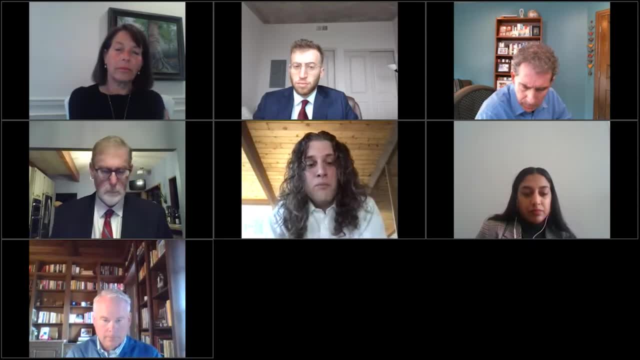 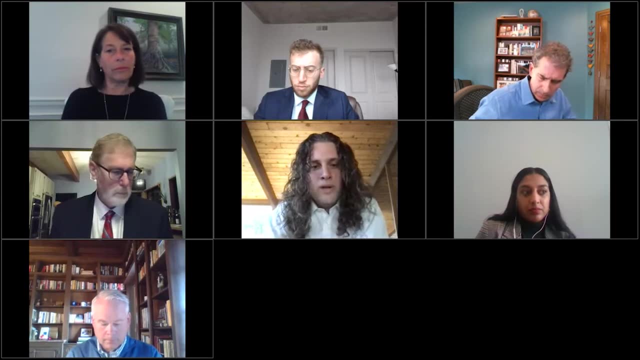 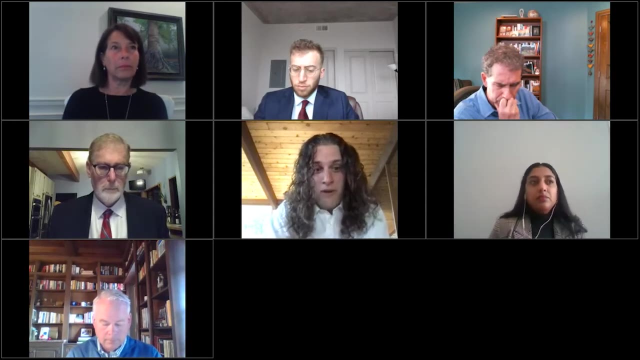 pieces. that is underpinning one of our big takeaways is that more data would be very helpful. More data to understand how and why we litigate the way that we do and how and why we choose the cases that we do and where they end up being filed is of great value. to kind of understand whether or 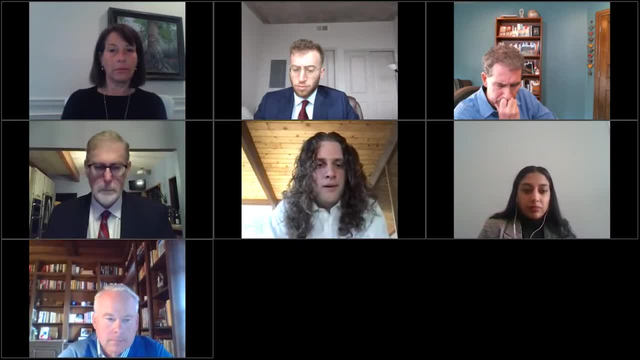 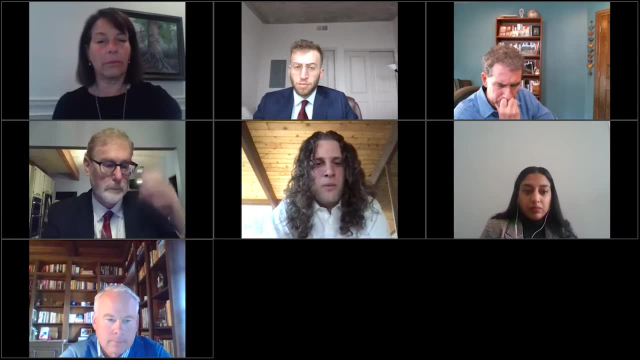 not citizen suits are valid, Whether or not citizen suits are fulfilling their promise of the basic kind of basic functions that we understand them to mean. And so I think, in a lot of ways, as David was alluding, our metrics are, you know, limited very much by the 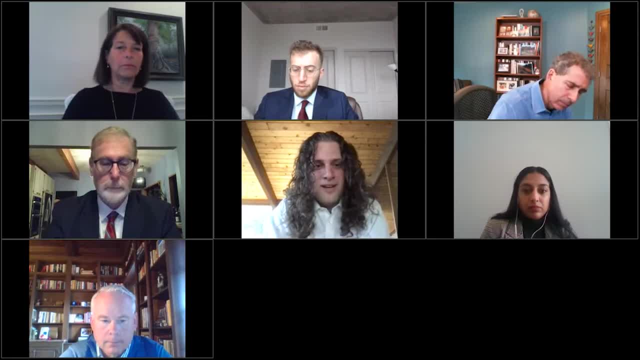 data And so, to the extent that there is additional data that we can, as a community of attorneys and community of environmentally interest aligned people, develop more data that would allow us to better understand how it's going on and why it's going on. it would go a long way to helping build a better framework to understand. 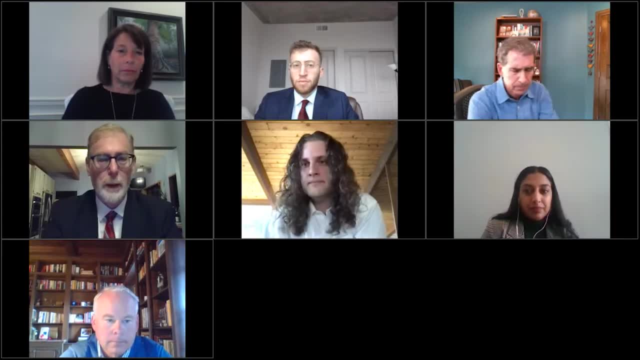 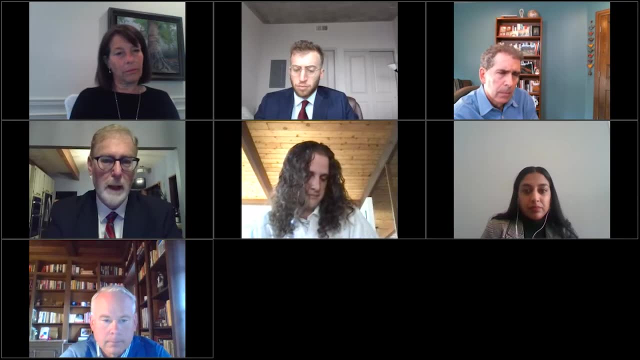 whether or not we need and how to reform it. You know, Jory and David, there's a fair amount of polling data, particularly on water issues around the Midwest and Great Lakes, done by some of the top pollsters in the country. 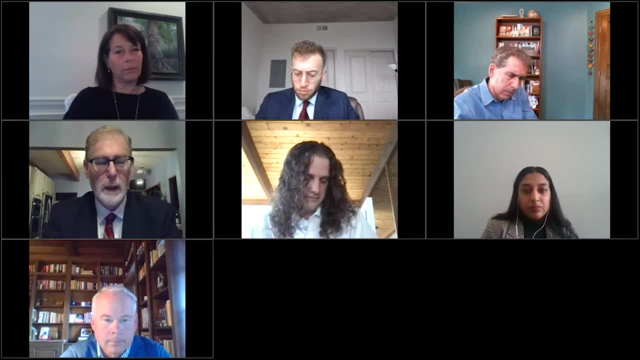 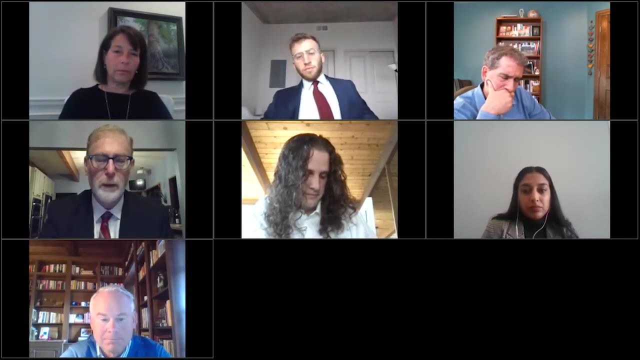 I'll send it your way. I think we'll give you some of the empirical data you need And it basically is showing you know, protecting clean water, protecting Lake Erie, for example. This is an 80% public issue and it's an 80% issue when people are asked if it winds up costing more in terms of wastewater treatment facilities. 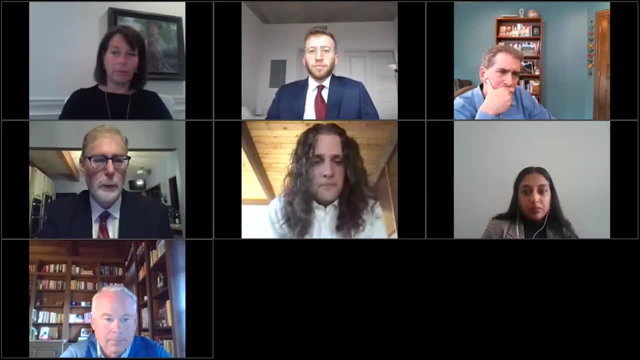 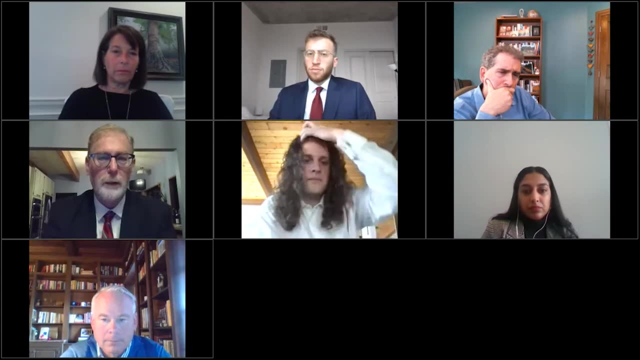 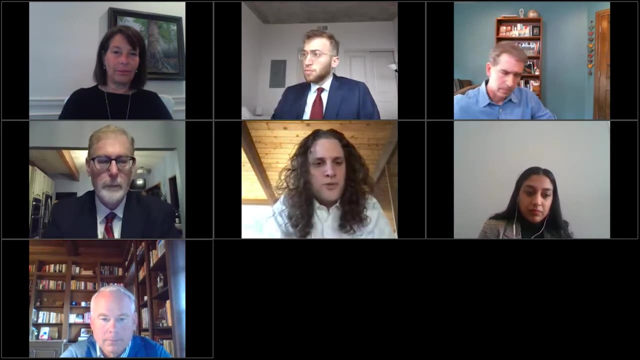 Are you willing to pay it? It's just not a close issue. Polling was done, among other people, by Ann Selzer, who's one of the top pollsters in the country. I'll send it your way. So one thing I do want to note on the concept of looking into the particular litigations. that would be very valuable. 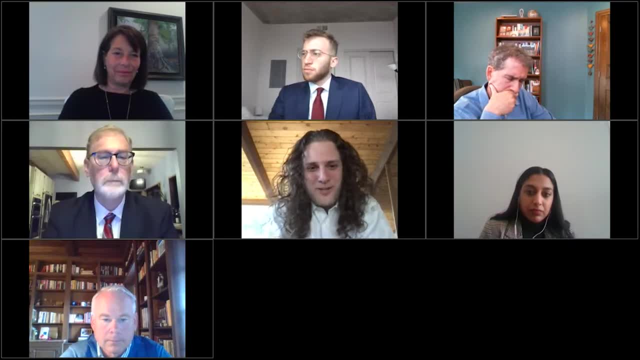 So I spent a fair amount of time During this project going in and trying to categorize all of these cases and with one case it's fine. You open up the complaint and you take a quick look and you, you know, peek at what exactly is being argued within the context. what are the statutes, et cetera. 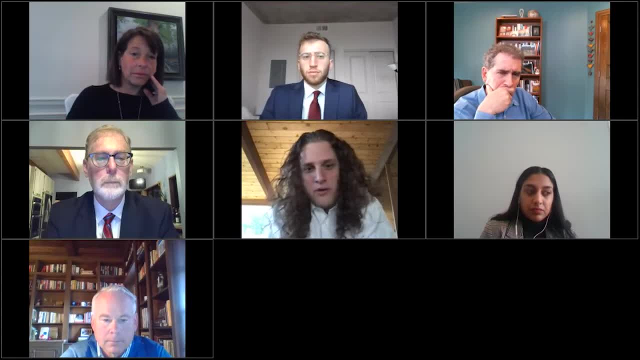 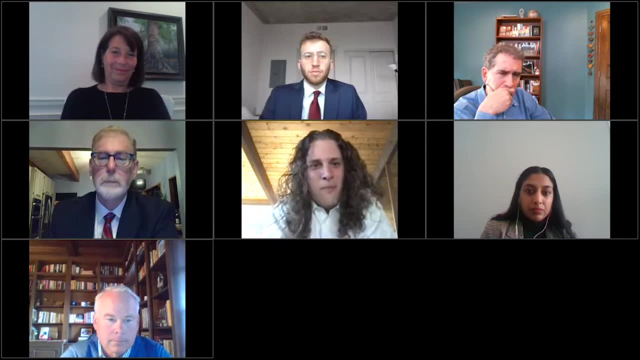 And with 20 cases it's fine, but resource intensive. And with 150 cases it's fine, but more resource intensive. And with 10,000 cases it's next to impossible for one person to do it. So part of the other thing that is underpinning a lot of this too, that would be great if additional. 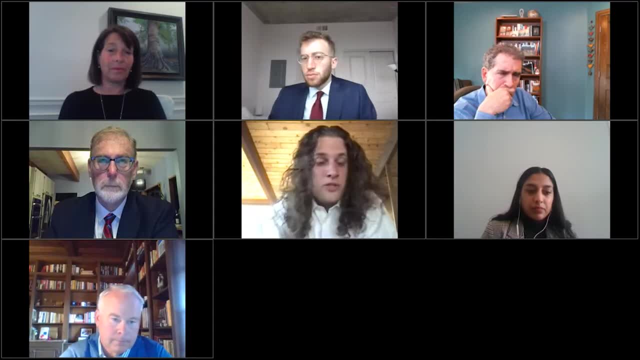 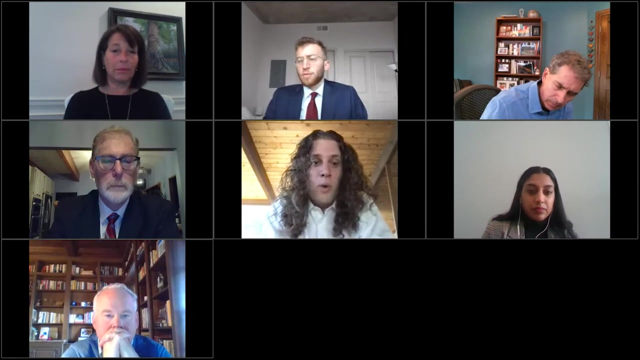 people who are looking into right or research in this area wanted to undertake is to try to help us develop as a- you know, a community. what exactly is in some of these cases- because it's very hard to get down, I think to the nuts and bolts even of sometimes what? what is the central issue that's driving this case outside of the of the particular claims that are being raised when you're looking at it in a big aggregate? 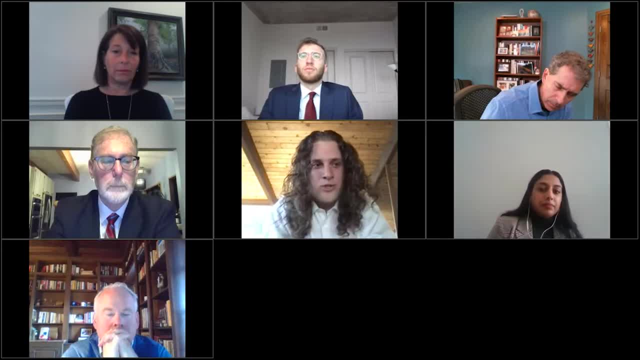 And when you're looking at many, many, many cases, And then I guess the last thing I'll throw on there too is is that I I think it's important to note that we did have to pull. there are some cases that have such such mass impact that we did have to remove them from parts of the data set. 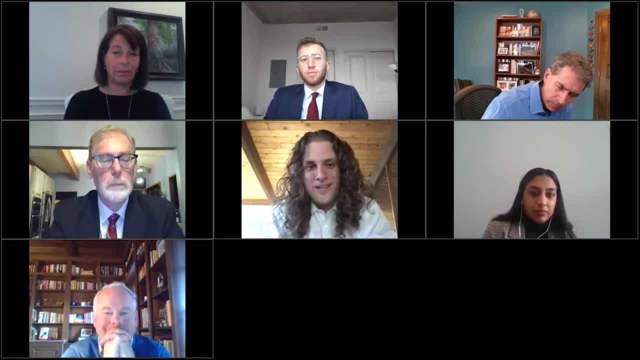 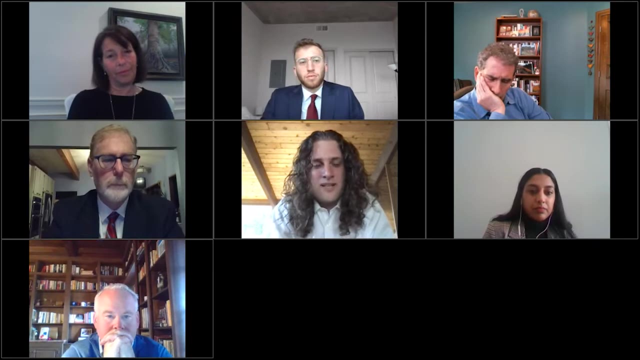 The good examples of these are the, the Volkswagen cases, the, the MDL in Louisiana on the Deepwater Horizon. There are some things that also have these huge impacts, that are really kind of linked locations that you can see Even in The aggregation of the data set to the extent that they might obscure everything else. 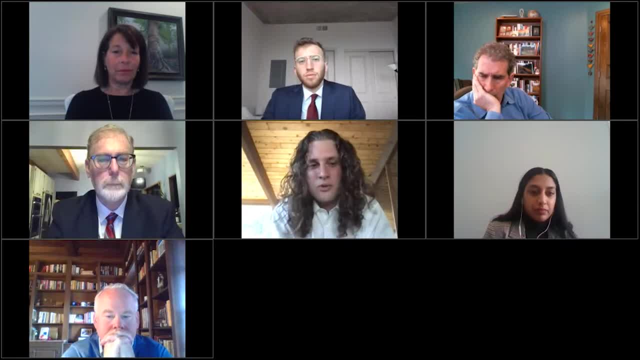 And so that kind of I think how it goes to your point about one of the things that might be interesting, I agree, to look at would be to take the ninth and the DC out and see if we can discern about local trends. All right, 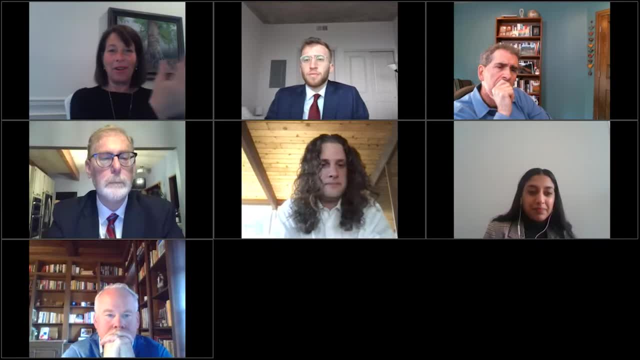 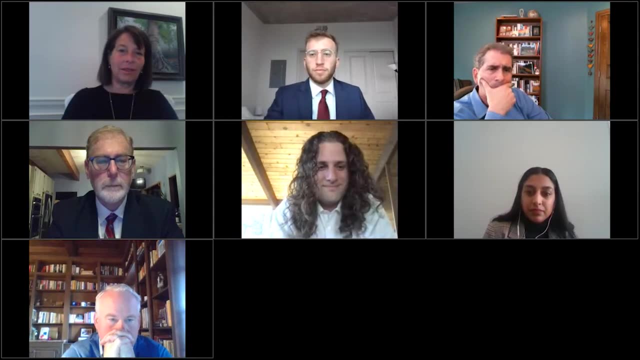 I want to make sure we get that. We have a lot of great questions and we're going to have our Vanderbilt law student kick it off with a first question and then we'll go to more audience questions. Thank you, Linda Um. 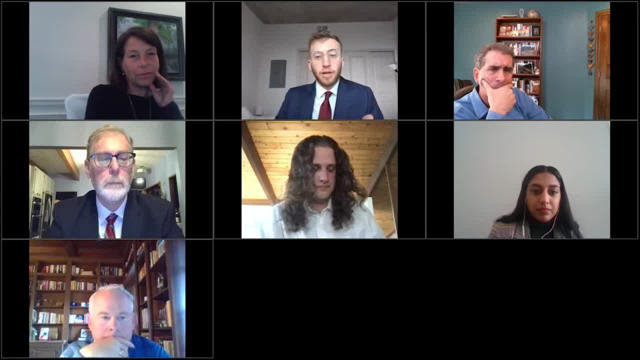 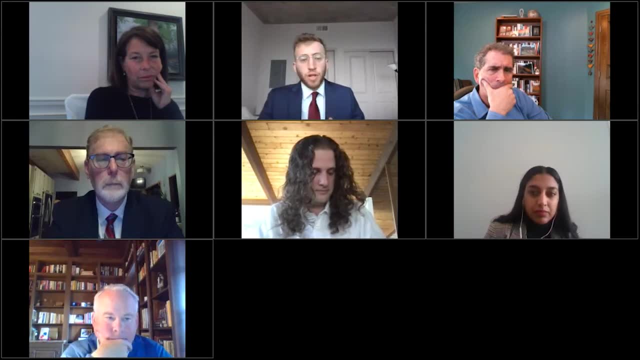 So this question is for the authors, all the commenters, anybody who has some insight on it. My question is fairly basic but I think important. in your opinion, which environmental statute? you know the, the, the largest environmental statutes, the clean water act, things of that nature- which statute? 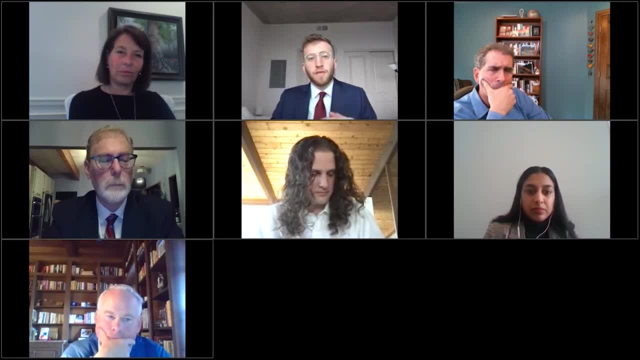 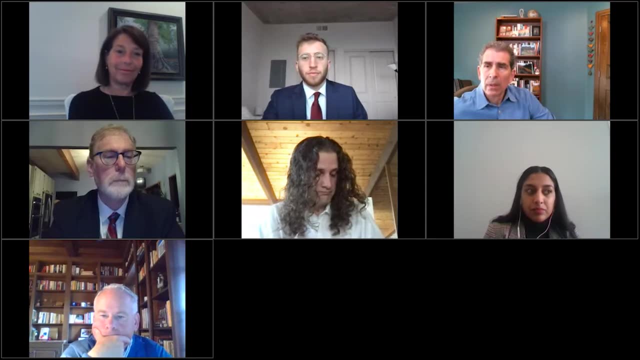 Could and would most benefit from an aggressive, from an aggressive increase in litigation aimed at the statutes enforcement. So, um you know, I I just have a rough intuition and maybe you know, and Howard will have a different sense of things. 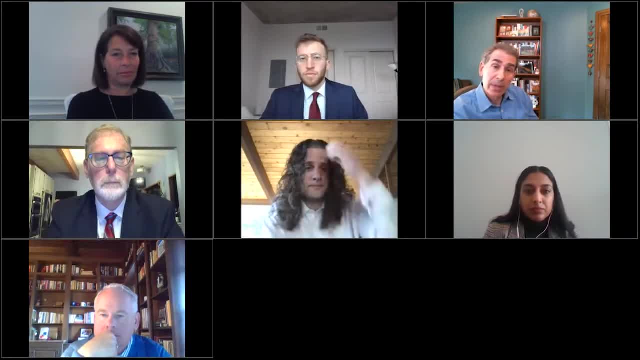 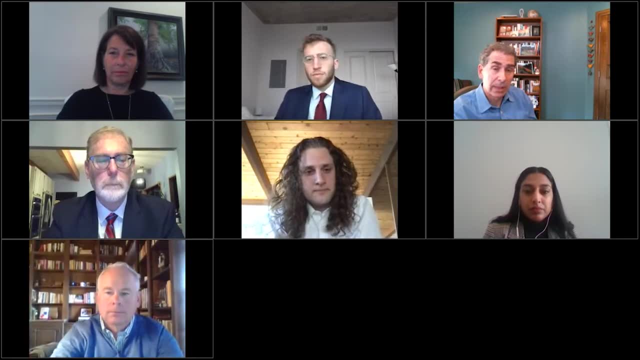 Um, you know, there's relatively little if we're, if we're thinking about it from an enforcement perspective, which is sort of the way you framed it- the relatively few cases filed under the clean air act, in part because the complexity of those cases. 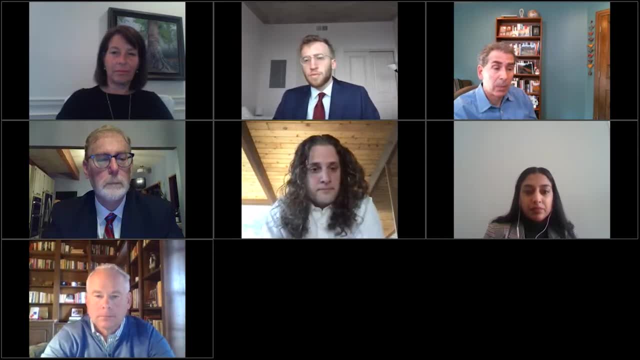 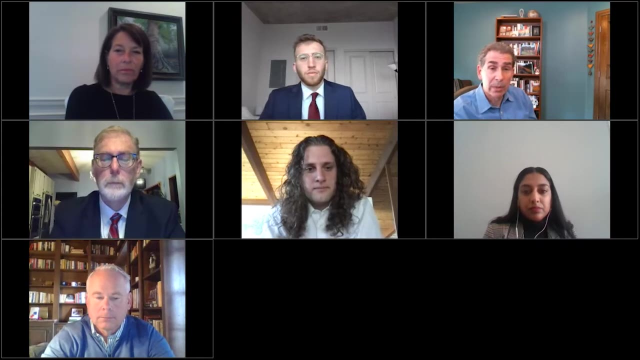 Um, and so anything that would Provide Um, you know, provide more値, Luis pos, I would say that, actually, the lack of of of져 that would would um, provide more recent resources or incentives, particularly under that statue, I think would be valuable. 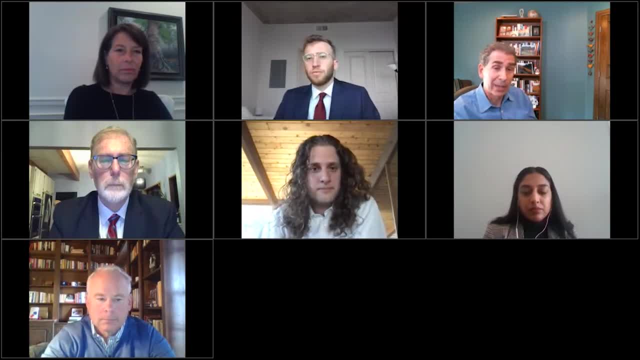 The Clean Water Act, Um, because of the reporting requirements and the relative and I'd want to emphasize relative ease of brain. those sorts of cases. I would see a much higher volume of cases Valuable Um. the Clean Water Act, uma, the reporting requirements in the relative and I and want to emphasize relative ease of three. those sorts of cases. we see a much higher volume of cases there. 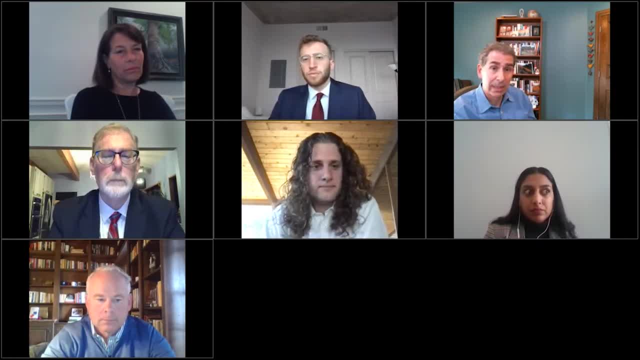 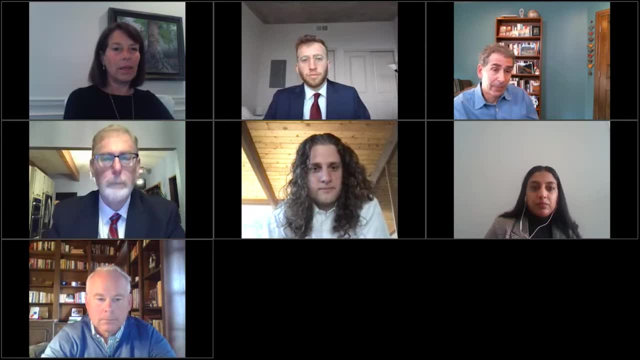 if there's any place where you'd like to see more litigation- or it seems like there's relatively little litigation- that would be the statute that I would point to. Does anyone else want to jump in on that? I was going to mold it quickly and I was going to also suggest the Clean Air Act. 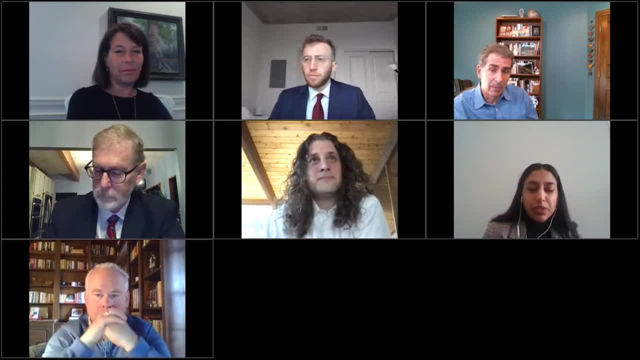 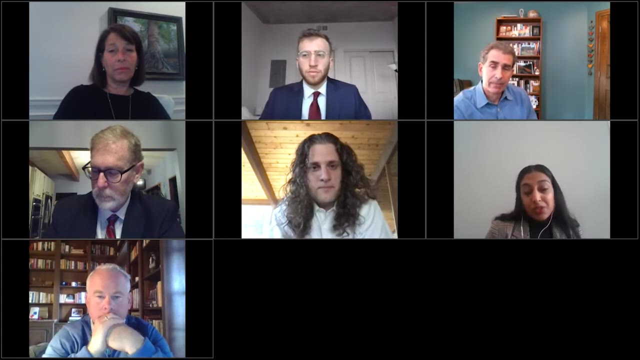 I guess not so much. I mean in addition to the enforcement reason, but also just in terms of the impact of that pollution right on communities. It's just inherently right. it's bigger, it reaches more. And I'll just add that I think there's really interesting things going on. 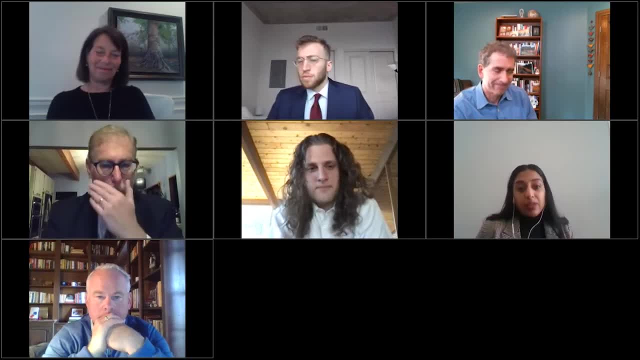 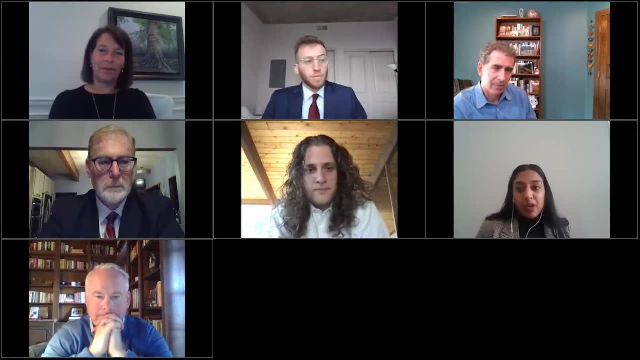 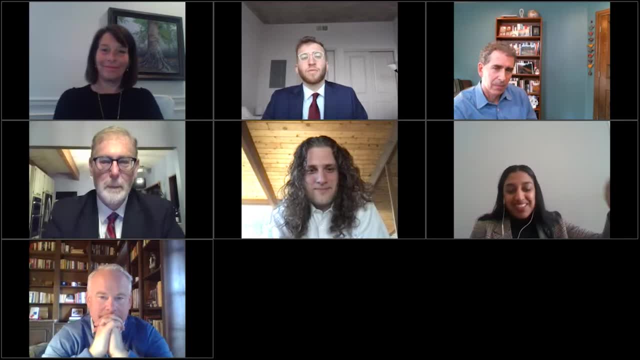 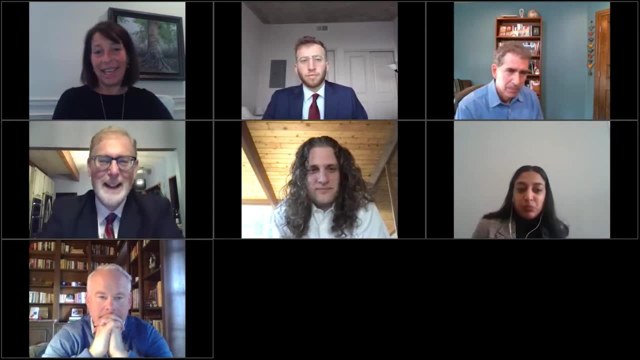 I want to flag. that's kind of right there, It's there, It's right, it's maybe happened or just about to happen, I think. in the air context That's interesting because that was one of the first questions I wanted to pose- was 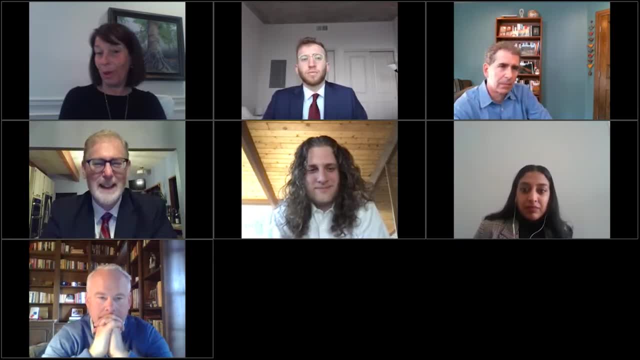 I think about citizen scientists and what role they may start to play in these cases and if they are ready. And one of the people asked: you know what are the Dover considerations? Let me address that one a little bit, because at the Environmental Law and Policy Center we actually 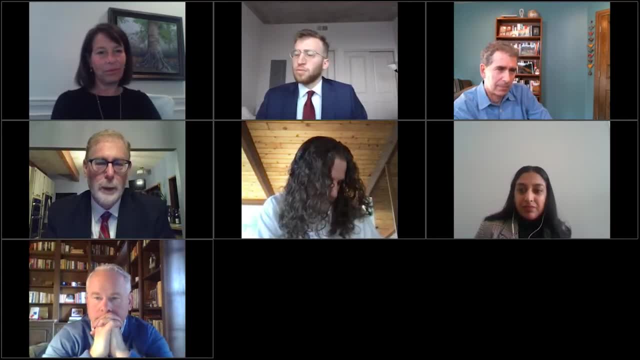 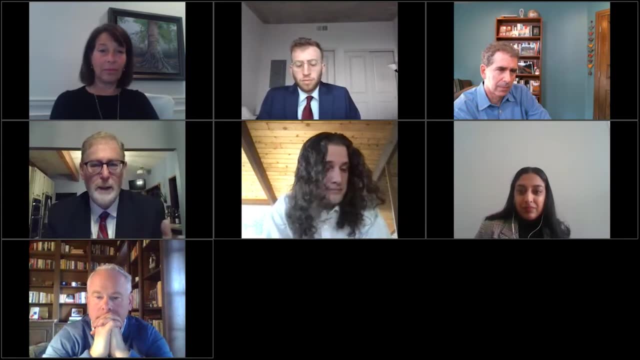 run the largest clean air air quality monitoring citizen science project in the country. We have more than 100 air quality monitors. They're handheld, They're about the size of of two cell phones put together And we work with community groups around Chicago and now Milwaukee. 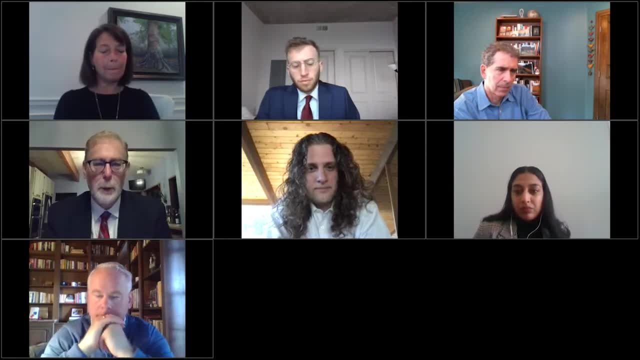 to gather the data. The data is uploaded, It's put onto maps and you get a very good idea where particulate pollution is especially high There. there are Dover issues, as you're pointing out, Linda. This is citizen data. It's important indicative data. It's not necessarily yet ready. 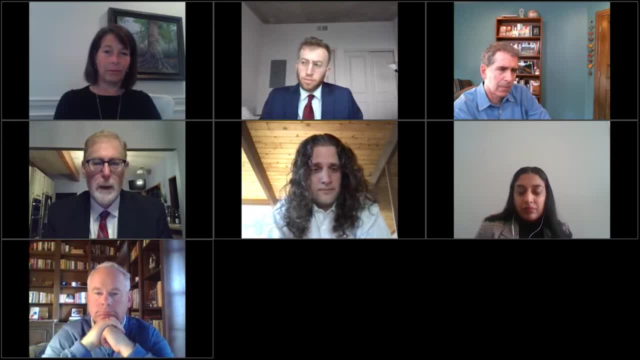 for prime time in terms of, you know, federal standard enforcement data, but it gives you a pretty good picture of what's going on. Keep in mind, from a methodological standpoint, David and Jory, the clean air cases, and I agree. 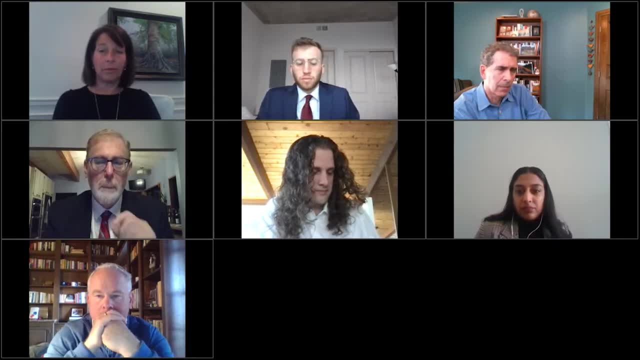 with you. they're very important in terms of citizen suits. Many of them will actually show up in the DC circuit, not in the local circuits. So, for example, if you think that two counties in Indiana and two counties in Illinois ought to be re-designated in terms of ozone non-attainment. 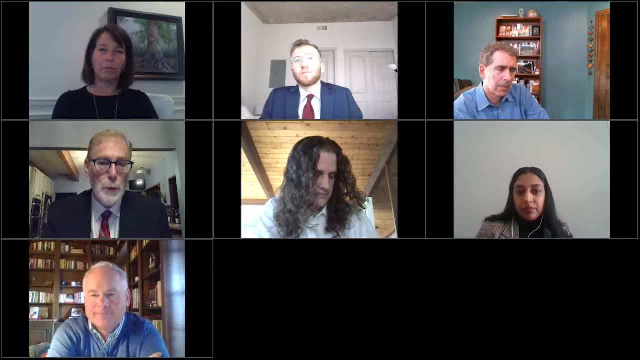 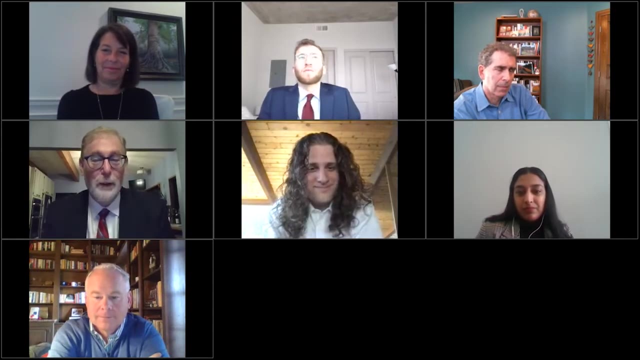 that action gets brought in the DC circuit. It doesn't get brought usually in the local district court or in the local circuit. So from a methodological standpoint for your paper, that that's a matter of you know. the choice of forum is those clean air cases often go. 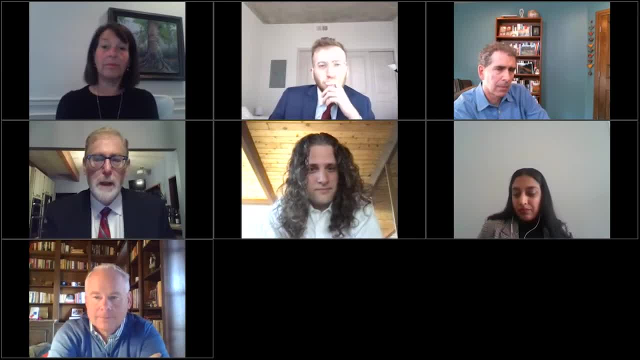 to the DC circuit because they involve decisions being made by US EPA at a national level but, as a practical matter, their decisions being made at the regional level by EPA, with the state EPA, but the actual action comes out of Washington. so you're going to the DC circuit. So that, let me just flag that methodological problem. 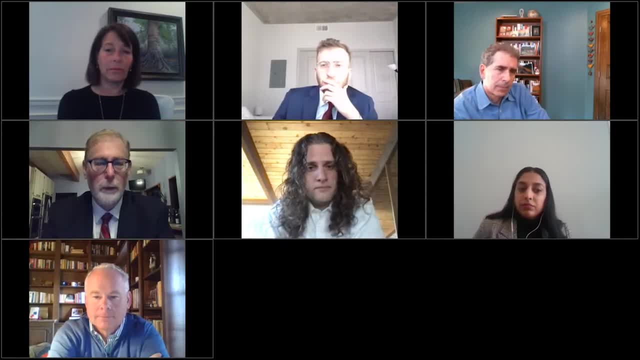 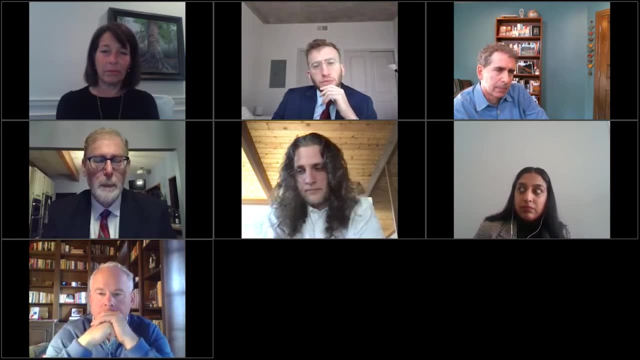 Clean Air Act is certainly one where more vigorous citizen enforcement is not only desirable, it's necessary. A lot of this turns a course on the peculiarities and the. I don't mean that let me say particularities more so than peculiarities. 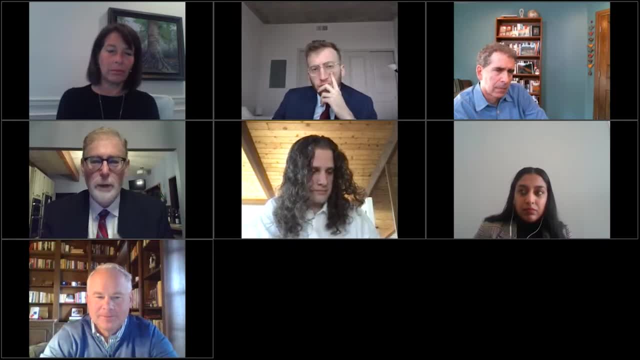 Sometimes at a state EPA there's just a crack team of people who've been working on clean air issues for the last 15 years who are terrific, and they stayed at the agency. The water division, perhaps, is not as strong. Other places it's the opposite. Some places there's some terrific staff. 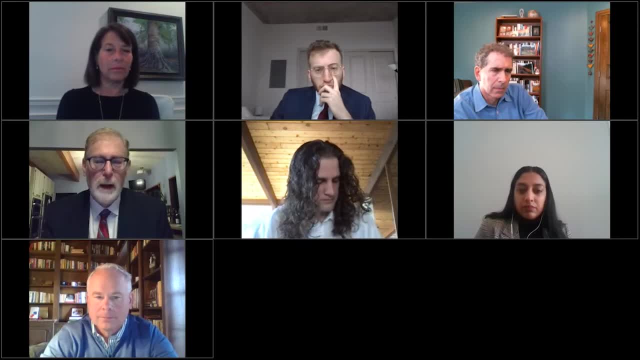 who know RCRA really well. Some places there's some terrific staff who know RCRA really well. Some places there's some terrific staff who know RCRA really well and do a great job of it. Other places, RCRA is underutilized and provides an opportunity for what you're discussing Ditto with the 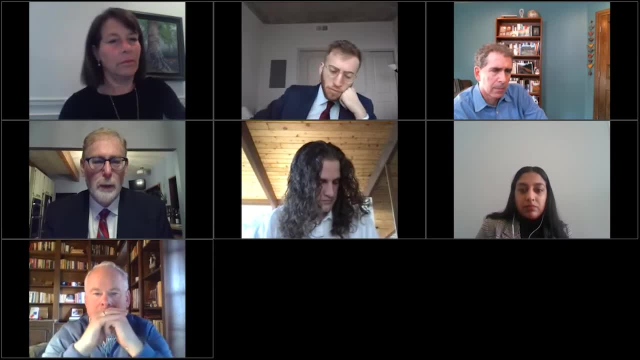 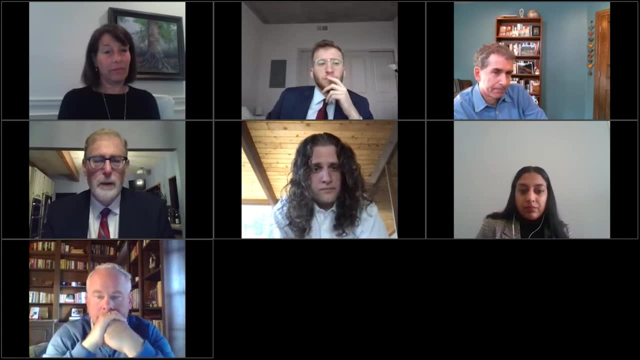 regional, the EPA regions. You know you've had a lot of retirements at EPA during the Trump administration. It may well be that the division that deals with RCRA has been gutted, but the people who are dealing with clean air have stayed, or vice versa. So you really have to look at what. 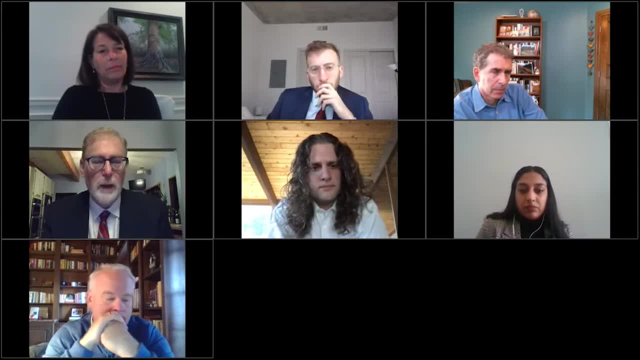 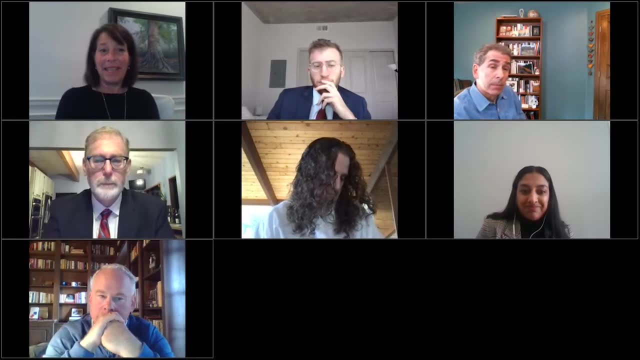 what's going on with the particular state EPAs and what's going on at the particular regional offices. So we have so many great questions. I was going to say could I just throw out a couple others and maybe we'll like do this like Jeopardy. Whoever answers first, we'll try to do a quick. 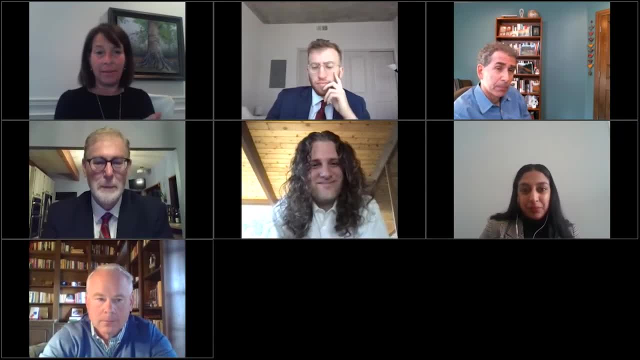 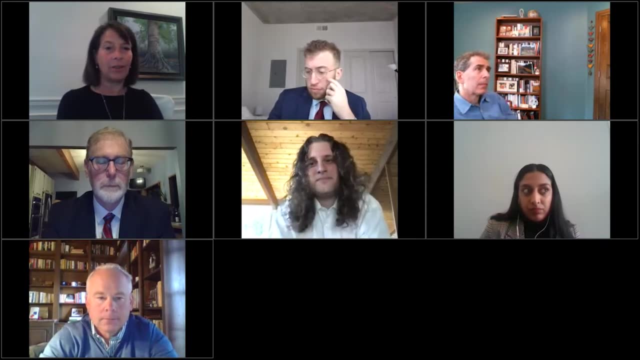 answer and get to a few of them- We have several- about PFAS substances and whether there's an uptick in cases trying to address PFAS substances under Clean Water Act or RCRA. Anyone want to address that one? Yeah, so we. that's outside our empirical data set for this one here. A lot of the PFAS stuff I do know. 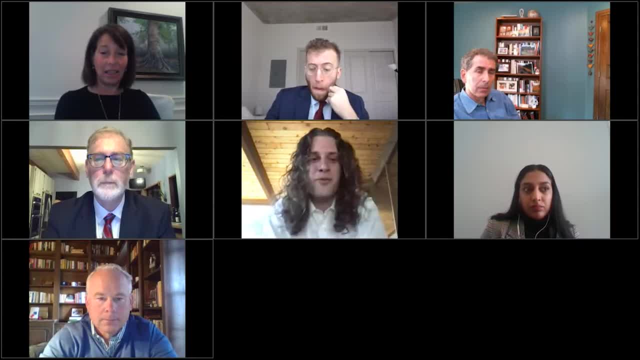 that there is just from. I can just say as an empirical matter that there is a upcoming toxics uptick. If we were to redo this study that covers now, there would be a lot more on toxics than there was during the standpoint period that we looked at in our paper. Great, great We have. 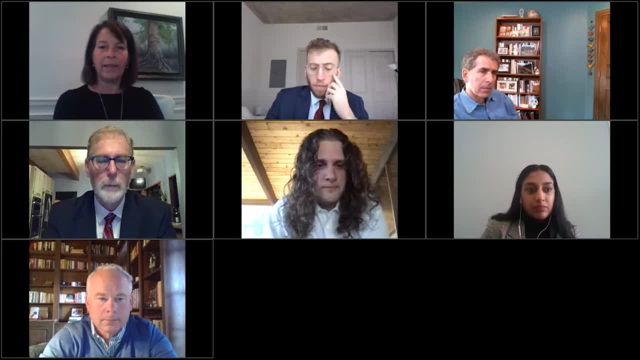 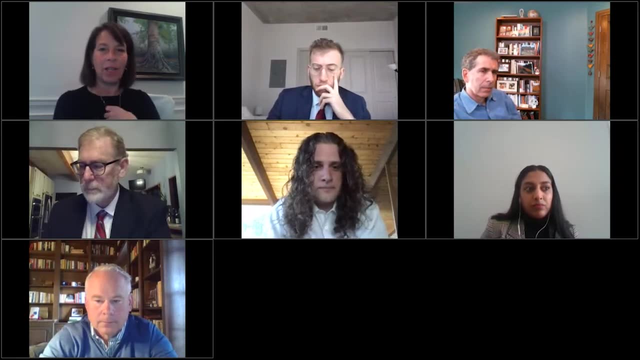 several questions about attorney's fees and why it's so difficult. You know what's leading to the increase in attorney's fees. And another question about whether there's been legislative action at the state level on attorney's fees that could impact us. Anyone want to jump in? 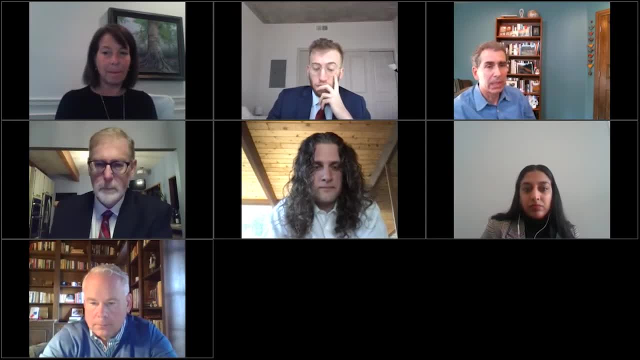 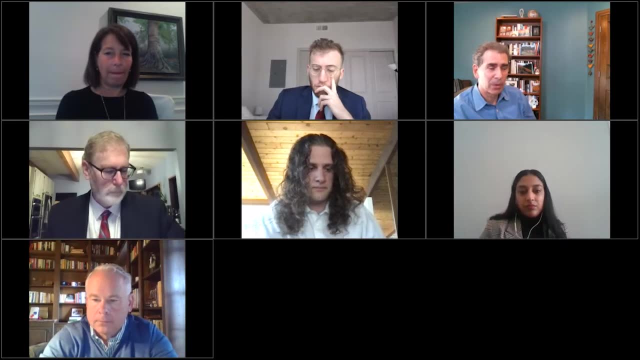 I mean, maybe the- maybe Howard will know this better- We just we spoke to people anecdotally and the impression that we got from those discussions was DOJ, in particular, was often opposing attorney's fees pretty aggressively And then just 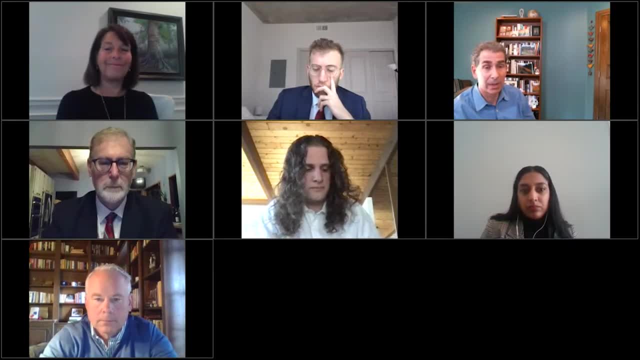 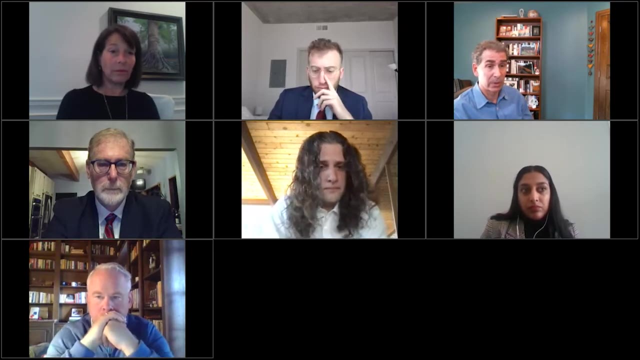 a general pattern of judges being over time less and less willing to grant attorney's fees or more skeptical about them. But that's not anything systematic. We've got kind of broad numbers that we showed you. That's more anecdotal, talking to environmental litigators mostly, really. 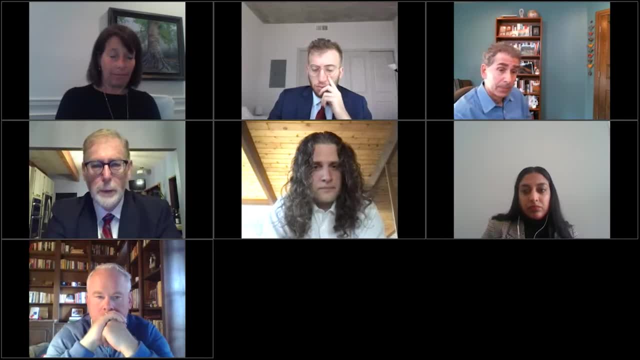 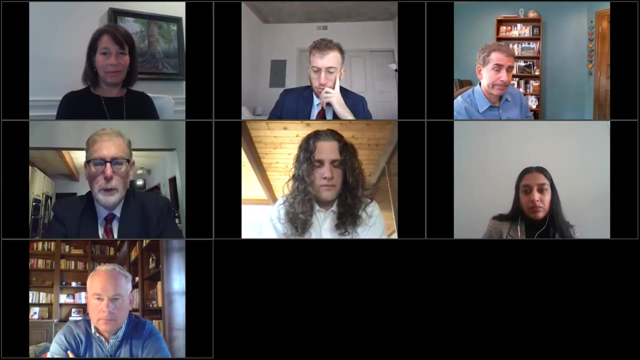 from environmental NGOs. You know, David, I think that's a fair observation And, frankly, it turns out that the federal administration, the Trump administration, the Department of Justice, was pretty vigorous in terms of challenging and pushing back and trying to limit attorney's fees. 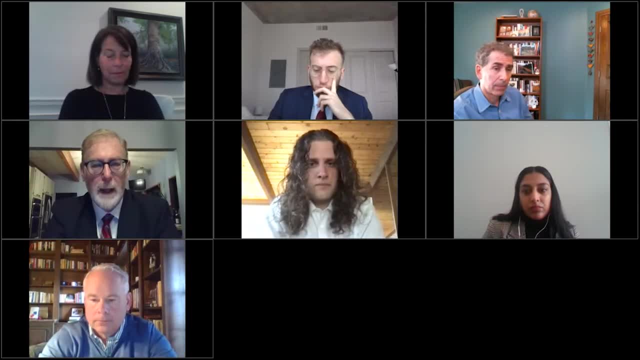 We hope that you know, with Todd Kim coming in at ENRD and the current Department of Justice people coming in at EPA and so forth, that there's going to be a different view And that's not going to be, that DOJ isn't going to do its job. 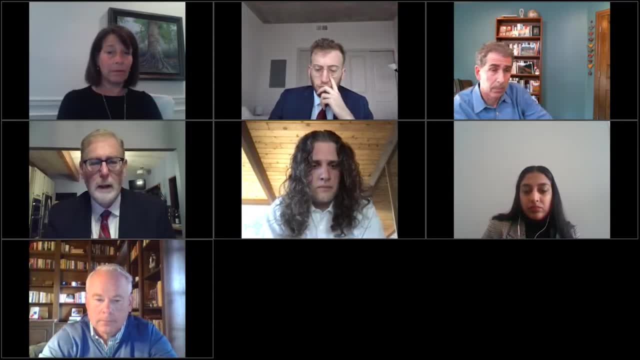 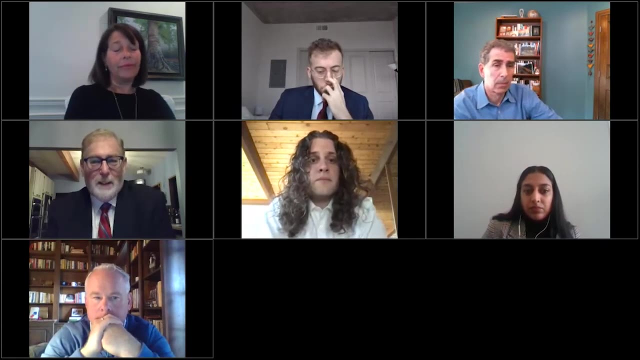 The DOJ job is to protect the taxpayers. We get that, But hopefully there'll be a little bit of a different take on what are appropriate attorney's fees from the new Biden administration than there was during the Trump administration. Let me just say it that simply. 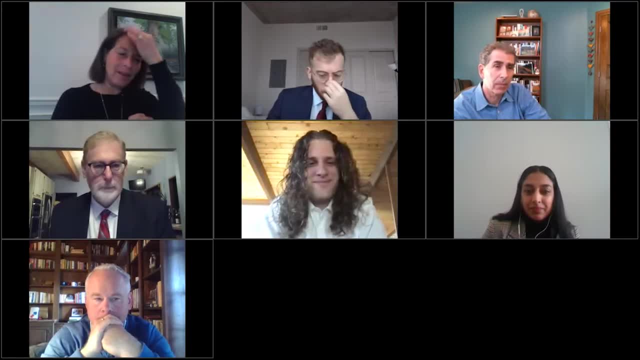 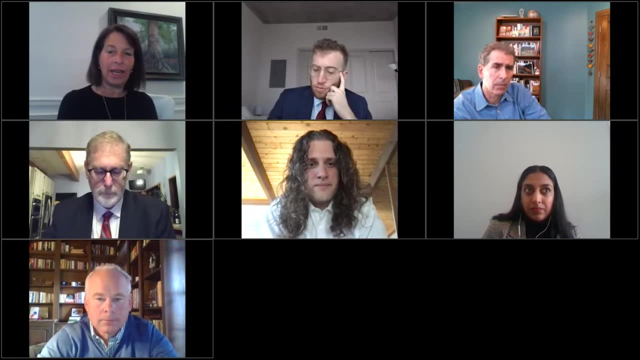 I'm going to ask one. I'm going to let us go over just a little bit because the question came in. That was something we talked about a lot in our class discussion about your article, And the question relates to judicial education Being really important and asking the authors for a little more detail on how they would propose to. 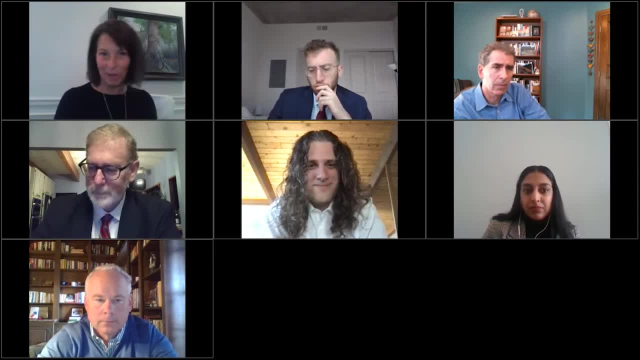 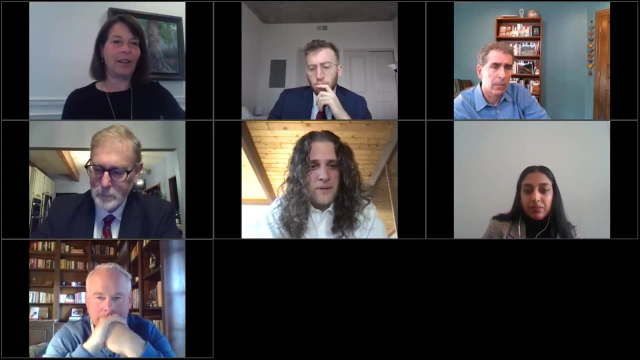 accomplish that, And I'll just do a disclaimer. Of course Environment Law Institute does some judicial training, But what other? what thoughts did you have on this? And we'll close with that. I don't want to go too far over. 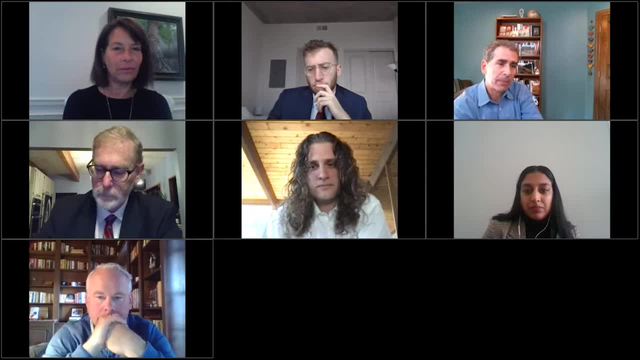 So I'll start And again, Joy, you can weigh in. You know, I think part of the sense is that there are high profile cases, let's say some of the challenges to national law enforcement. There's a lot of high profile cases, let's say some of the challenges to national law enforcement. 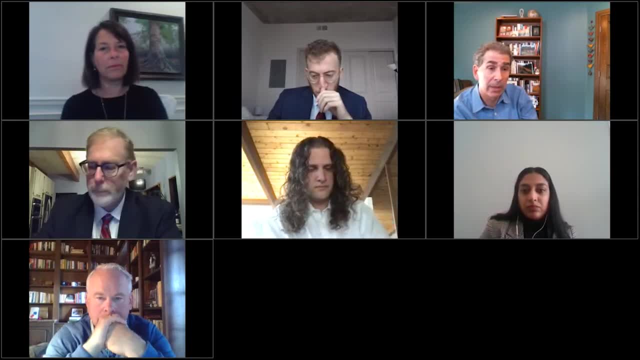 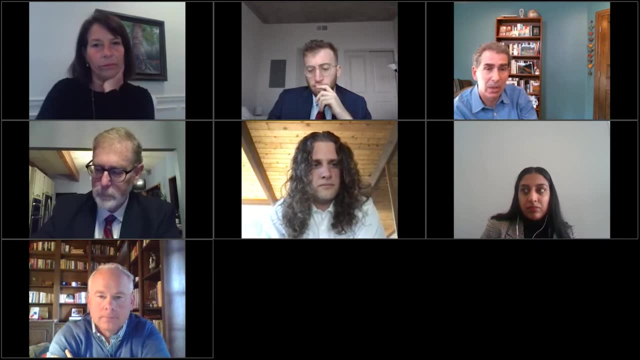 There's a lot of high profile cases, let's say some of the challenges to national law enforcement, And at the same time there are those that are really especially critical for for the health of the people of Los Angeles. So they get really big. 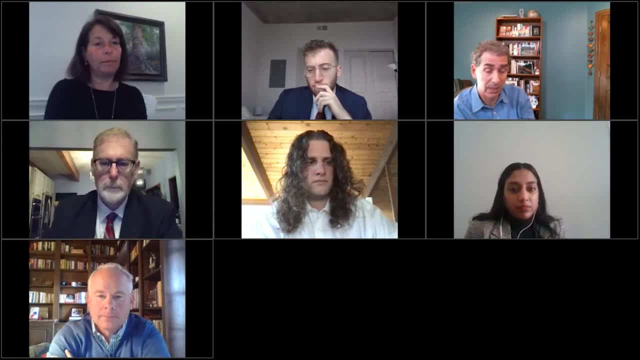 attention And our suggestions that citizen suits are brought much, much more widely than they actually are. in fact, They are getting an enormous amount of attention And are suggestive that citizen suits are brought much, much more widely, of the nature of citizen suits, how frequently they're filed, what their impacts are. 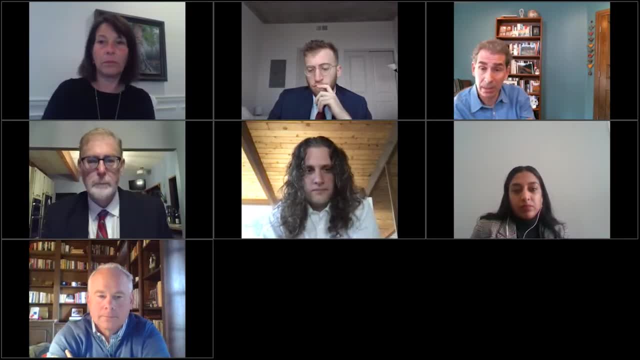 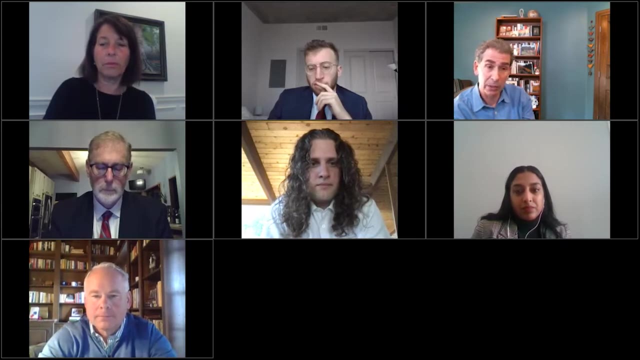 these questions about alignments with community values and some of the complexities around them as well, rather than judicial perception being driven by the most high profile salient cases, which we really do not believe are representative of actually how the pattern of litigation легally greets. Thank you again, David, and I think you know. 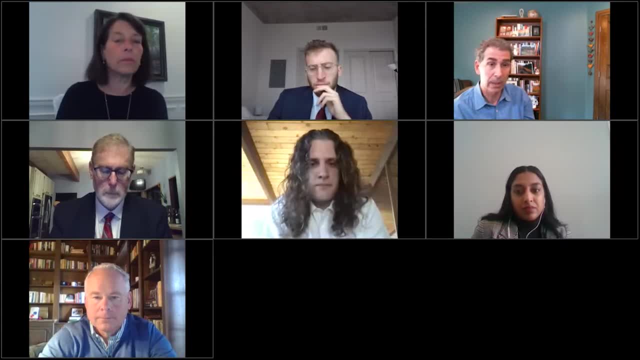 when you think about theboldness of litigation out there. So that's sort of you know, basically drawing on these results as well as any other results that we could draw on, It would be wonderful actually to do something where you have attorneys that are both bringing 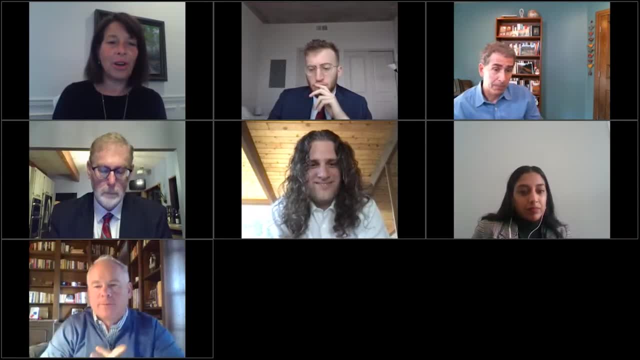 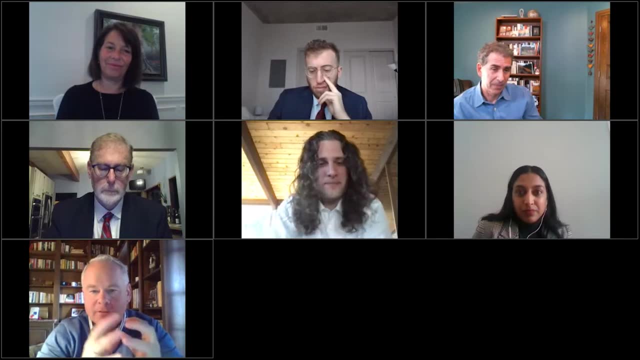 these cases and also defending them, to discuss them as well. I think that would be a really valuable thing to do, David, one of the things that would be fascinating about what are the ways to communicate with those judges who might have a skewed sense of this. It 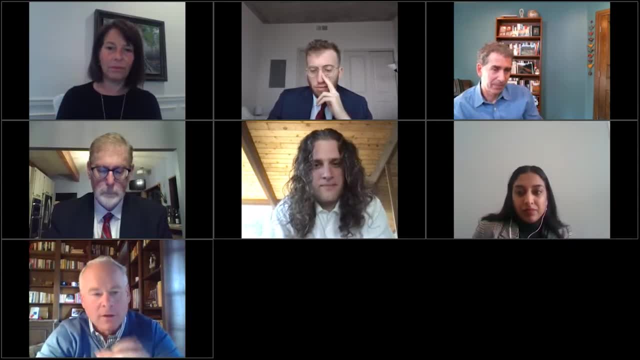 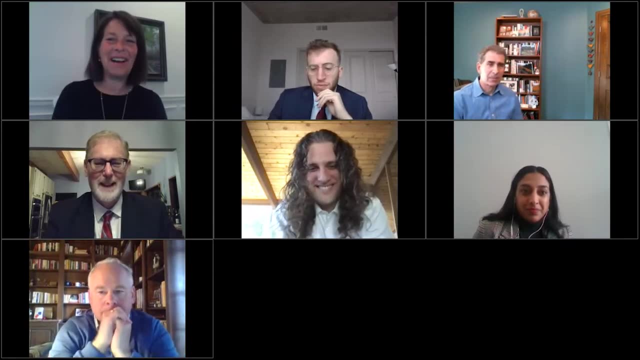 may not be a traditional approach, but I think that's a fascinating thing. This has been a wonderful discussion. I'll pass it back to Linda because I know we're running out of time. Really helpful, I know It's so many great questions. I hate to cut this off, but we are going to thank 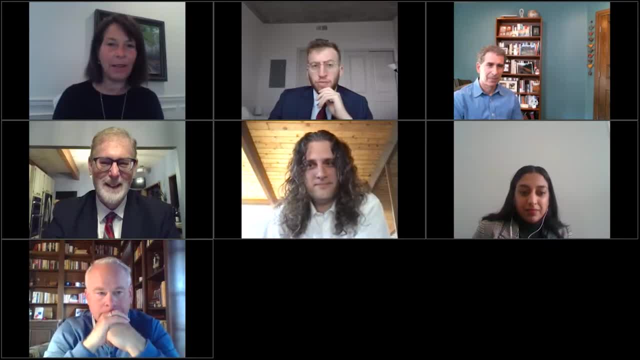 you for an absolutely terrific panel. Thank you, Thank you. There'd be a ton of applause if we were in person. We're going to take a few minute break here, during which time the audio will be live, as I mentioned. So we're going to be testing the tech for the next setup. We hope you will join us. 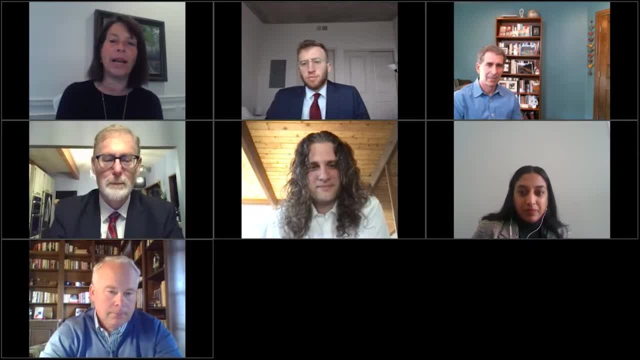 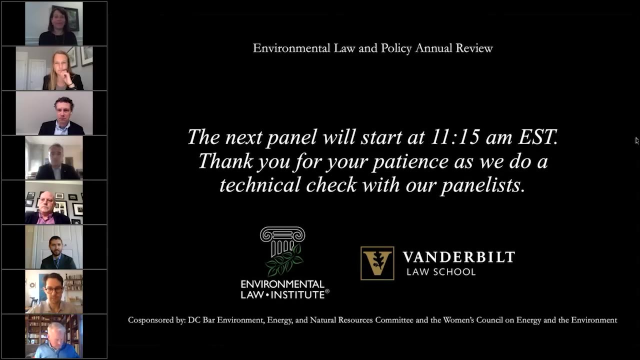 for the rest of the panels. Up next is the discussion of the article Caremark and ESG- Perfect Together, And we will reconvene in about 14 minutes. Thank you again to our wonderful panel, Thank you, Thank you, All right, we're going to get started. Welcome back to our second panel. 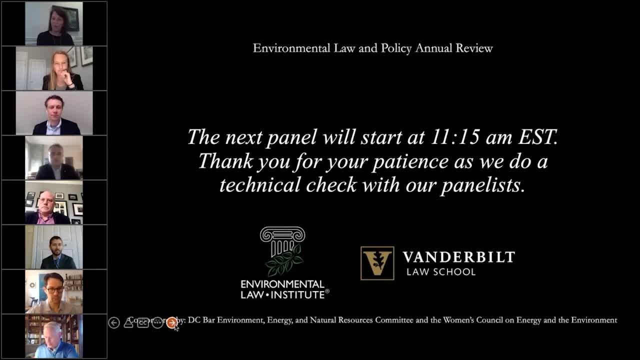 and we are ready to jump. We're going to jump right in, but I am going to remind you all in the audience to send your questions in the question box on the GoToWebinar. We want to get them as we move along and not wait. 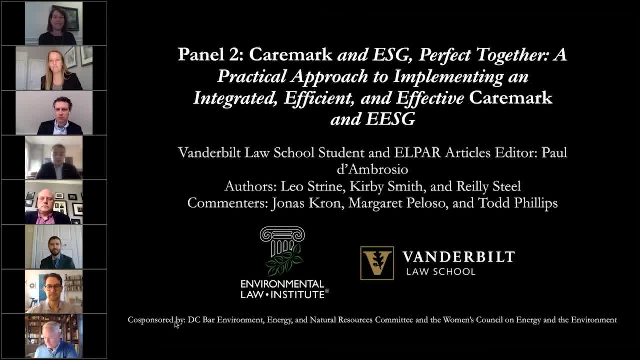 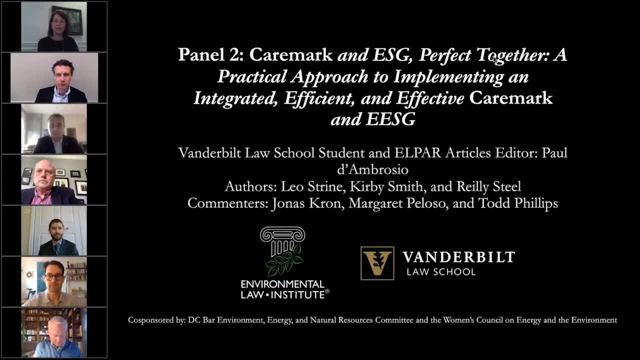 until the very end. Also a reminder that the slides we're using today will be available on the ELI LPAR website, So I am going to hand it over to third-year law student Paul D'Ambrosio, to introduce our speakers: Paul. 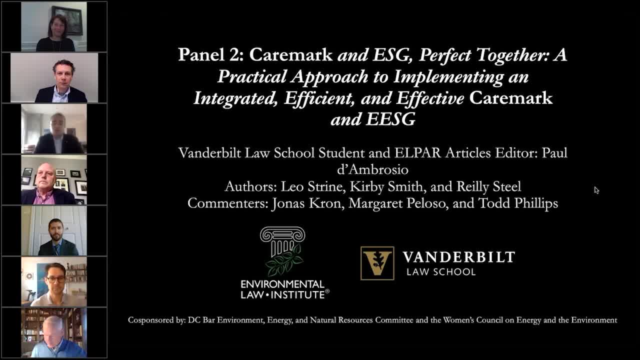 Hello everyone. My name is Paul D'Ambrosio, I am a 3L at Vanderbilt Law School and an articles editor for ELPAR, And I'm here to introduce our second article: Caremark and ESG- Perfect Together. 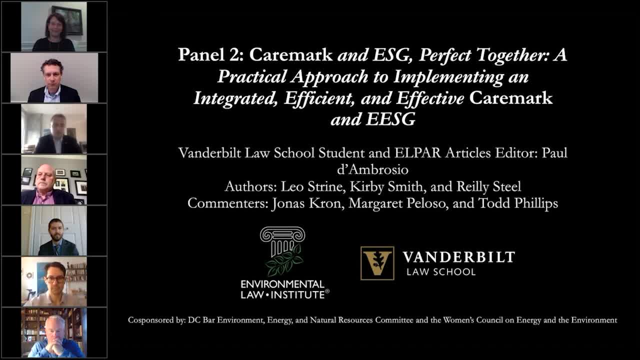 by Leo Strine, Kirby Smith and Riley Steele. Leo Strine is a graduate of University of Pennsylvania Carey School of Law and is currently the Michael L Wachter Distinguished Fellow at Penn Law School, as well as the Ira M Milstein Distinguished Senior Fellow. 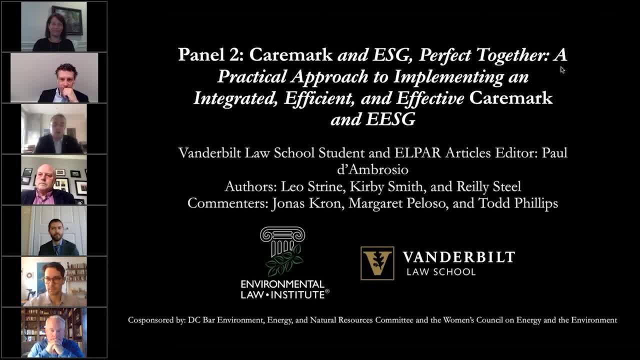 at the Milstein Center at Columbia Law School, a senior fellow at Harvard's Program on Corporate Governance, a Henry Crown Fellow at the Aspen Institute, and is also of counsel at Wachtel, Lipton, Rosen and Katz. But he is most famous for his work as the Chancellor of Delaware and the 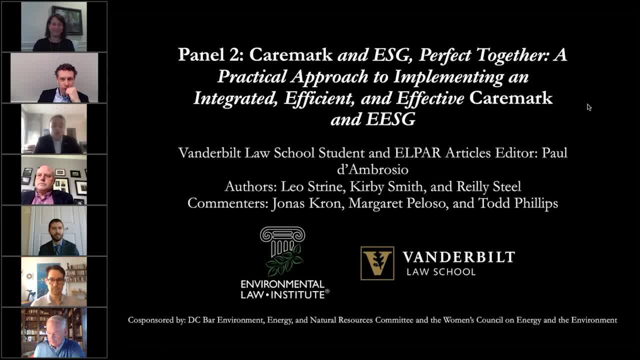 Chief Justice of the Delaware Supreme Court, where he wrote countless landmark corporate law opinions that are staples in every law student's corporation's casebook, including my personal favorite, the MFW shareholders litigation. Riley Steele is a PhD student in the Department of Politics at Princeton University. 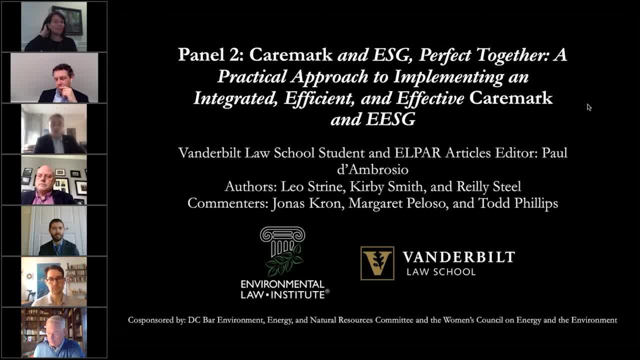 a graduate of Columbia Law School. He was previously an associate at Cravath Swain and Moore and served as a Milstein Fellow for the United States Senate Committee on Banking, Housing and Urban Affairs, And he clerked for Chief Justice Strine a couple years ago. 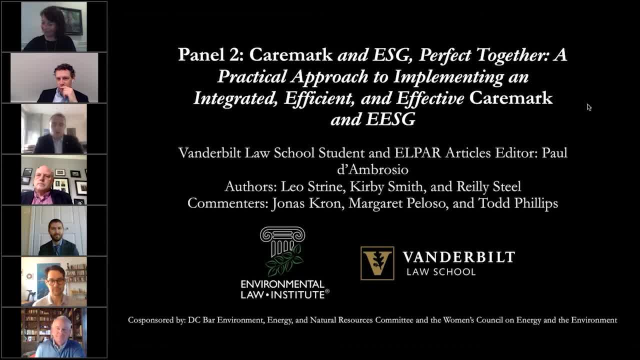 Unfortunately, our third author on this paper, Kirby Smith, cannot be here today, but he is a member of Bridgeport Partners, which is a private investment firm with a long-term, value-oriented approach to investing across public and private markets. He's a graduate of University of Chicago. 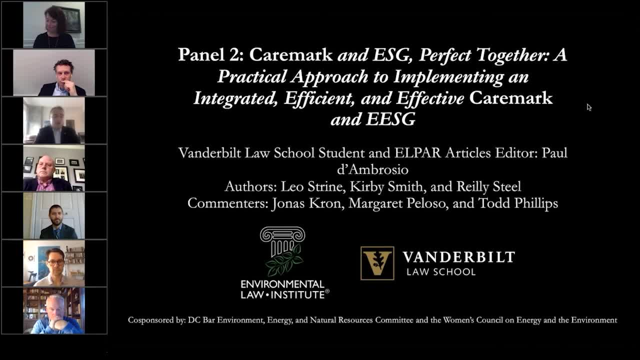 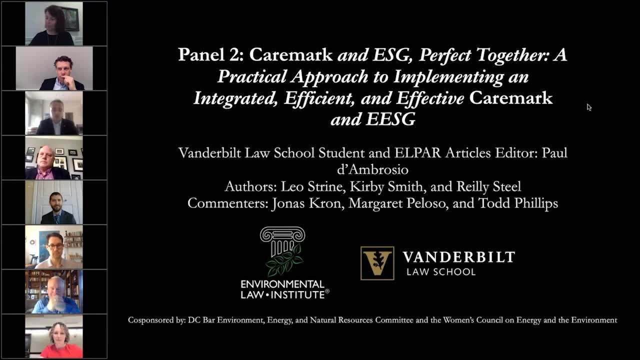 Law School, previously worked as an associate at Wachtel, served as a law clerk to Judge Andrew Hurwitz on the Ninth Circuit and also clerked for Chief Justice Strine. I believe he was a co-clerk with Riley. For this article we also have, unfortunately, only two esteemed panelists. 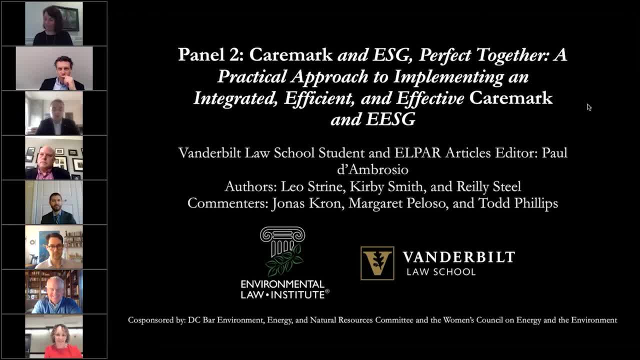 Now a third one could not be here, But they are Jonas Cron, Todd Phillips and, unfortunately, Margaret Filoso cannot be here today. Paul Maggie's just joined us, so we can add you back into the pile. Sorry, I was looking at my notes and 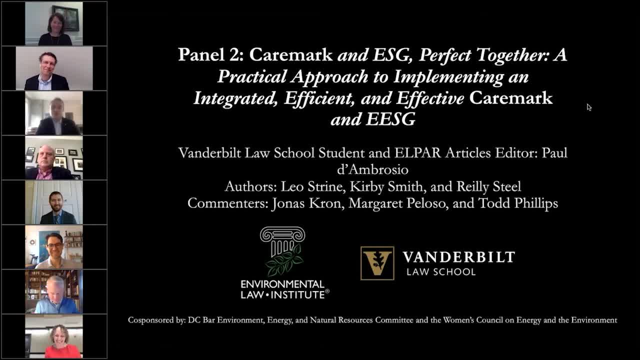 not seeing the camera. Well, welcome, Sorry. All three esteemed panelists are here and they will be introduced in full. Jonas Cron is a graduate of Vermont Law School and is the Chief Advocacy Officer at Trillium Asset Management, an investment firm focused on ESG and responsible. 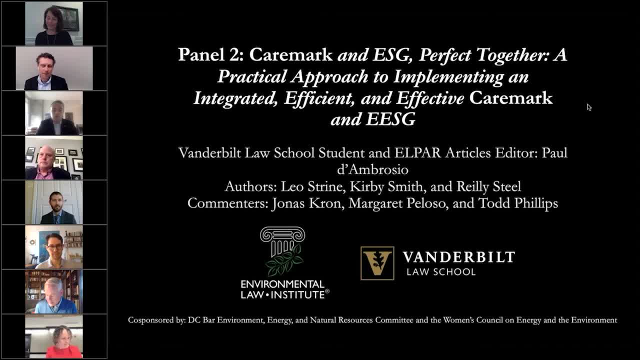 investing. He previously worked as an environmental attorney and a public defender and also serves as the Secretary of the Board for the US Forum for Sustainable and Responsible Investment. Margaret Filoso is a graduate of Stanford Law School and a partner at Finston & Elkins in. 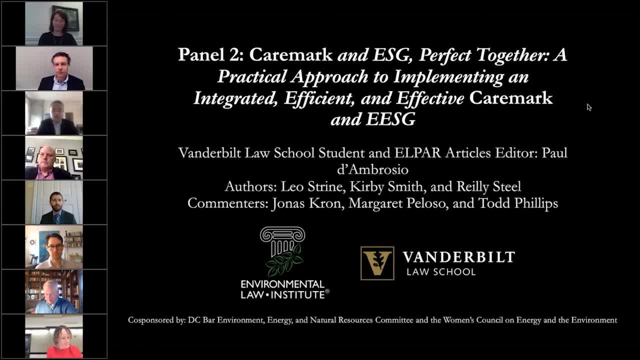 Washington DC. Her practice focuses on climate change risk management and environmental litigation, and she also serves as the Director of the US Department of State for Sustainable and Responsible Investment. She also holds a PhD from Duke and has written extensively on environmental law. 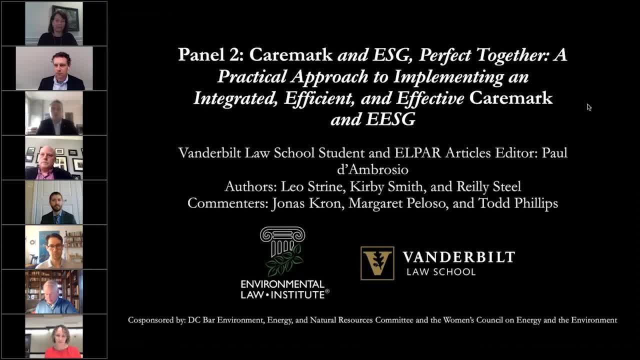 including a book titled Adapting to Rising Sea Levels. Todd Phillips is the Director of Financial, Regulatory and Corporate Governance at the Center for American Progress. A graduate of Michigan Law School, he previously worked as an attorney for the Federal Deposit Insurance Corporation, the Administrative Conference of the United States. 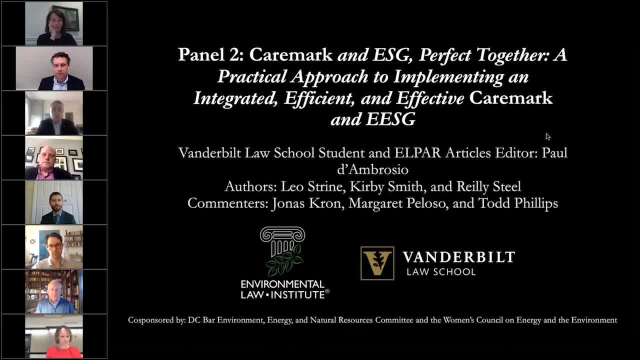 and part of the World Bank. He has also served as a national adviser for the Federal Census Authority and the US House of Representatives. As you can see, we've gathered a group of real underachievers, so we're going to have 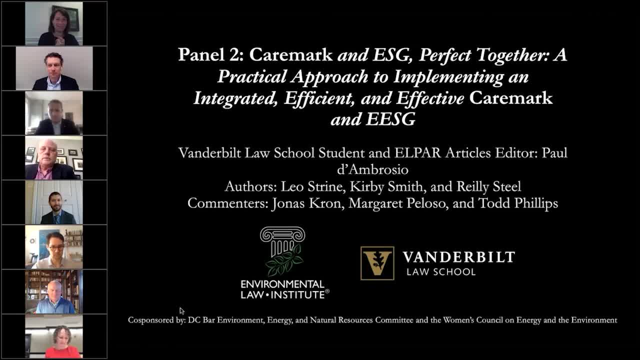 a fantastic discussion. Prof Strine, you can take it off. Thank you, Linda. thank you all for the introduction. I knew it was time to leave the bench and get the demonstration started because, in my opinion, this is the perfect time to leave the bench. 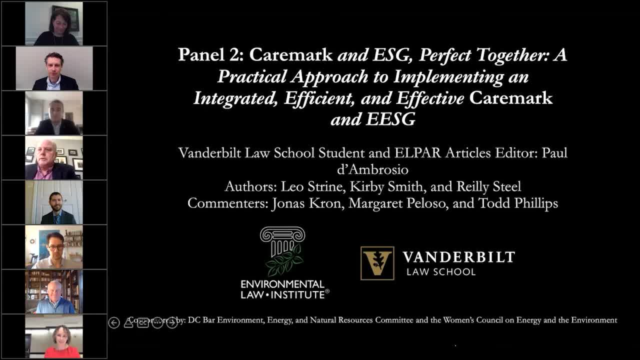 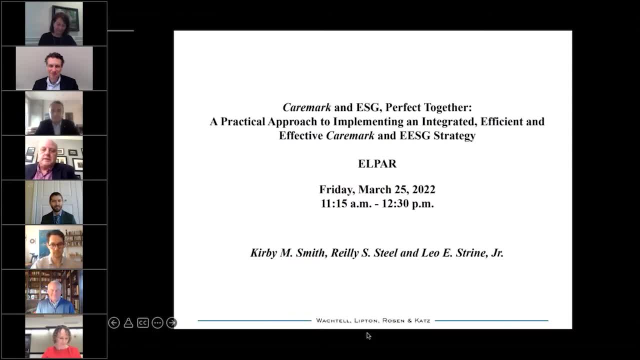 a better year than having Riley Steele and Kirby Smith as my law clerks. So you always want to know when you hit that high watermark, And so it's an honor to be with you all, And I thank the host for putting on such a timely panel. I think it's fair to say I'm going. 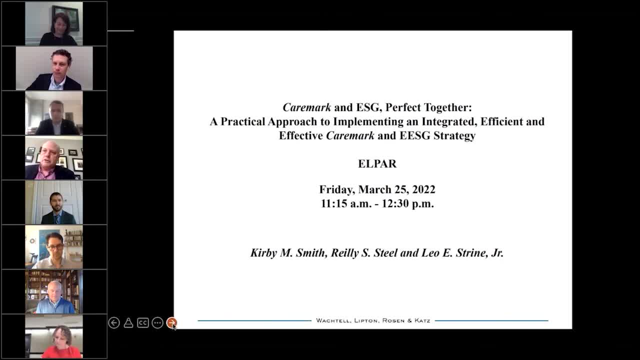 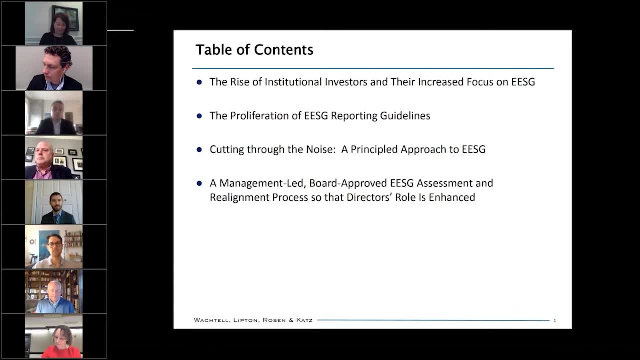 to kick it off. and then I'm going to turn to Riley. We'll probably go a little bit from the general to the particular. We have slides for you all that are really meant for you to take away more than for us to sort of use them. right, Riley, We're not going to put 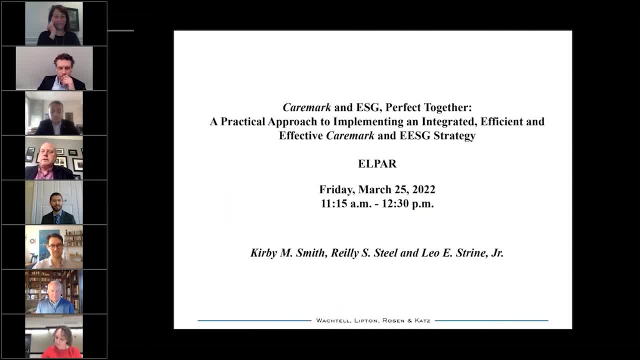 you through it. What we really want to bring to the table today is a way of thinking about these issues that could be helpful to making more progress towards something that we all hope for, which is respect for our environment and particularly addressing what humans have done in terms of carbon. 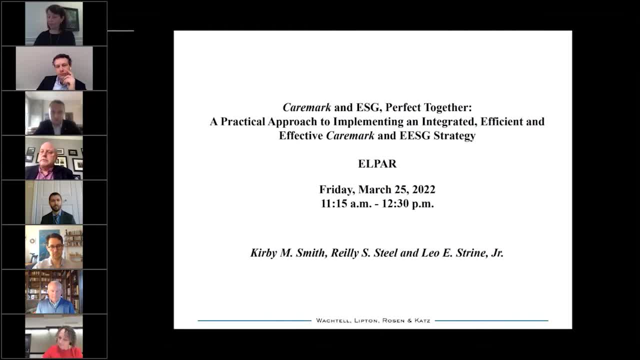 And methane and other emissions and their effect on the Earth's climate. One of the perspectives, I think, that Riley Kirby and I all bring to bear is that, you know, in a perfect world the legitimacy of the republic would be brought to bear to solve most problems. 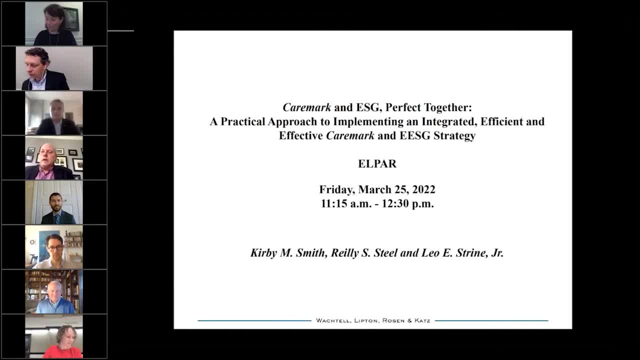 And that is importantly, remains the case. But for a lot of reasons we've written about and talked about in other papers- not just me but also Riley did work on, And so I'm glad that he did work alone on this early in his scholarly career- It's the governmental 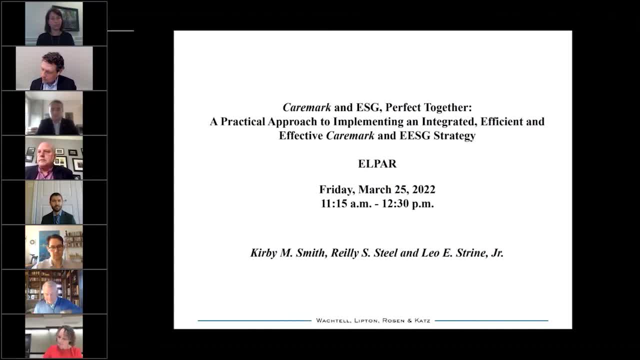 process itself is not adequate to respond to everything And there's increased pressure on business community and the business community to address issues like climate. But there's been a tendency in American public policy on many fronts in the last 25 years to be honestly cheap, opportunistic and of the moment. 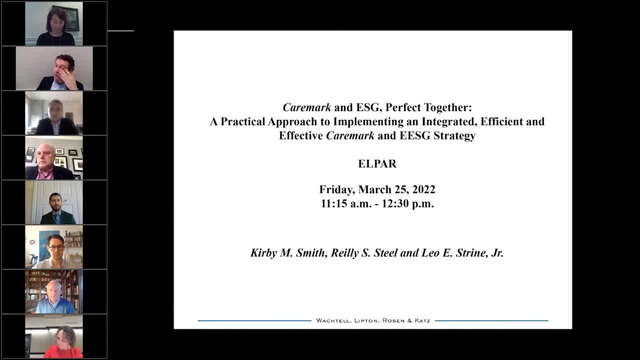 The cooling saucer of our constitution, as Washington put it. the United States Senate is increasingly the most reflexive body, not most reflective. Public policy is not the result of multi-year interdisciplinary efforts by members of the Congress who are more committed to establish statutory regimes and getting them right. It's not that way much anymore. 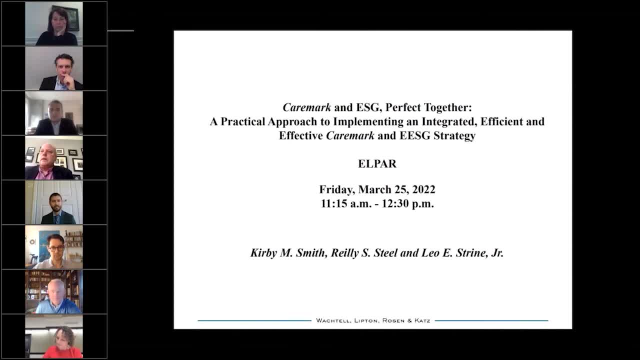 And that's a problem for making progress on this important front. And so business has been put front and center. And but realize, this is just the latest wave, right, ESG. I call it E-S-G because I add an E for employees And I'm going to come back to that in terms of climate, But it used. 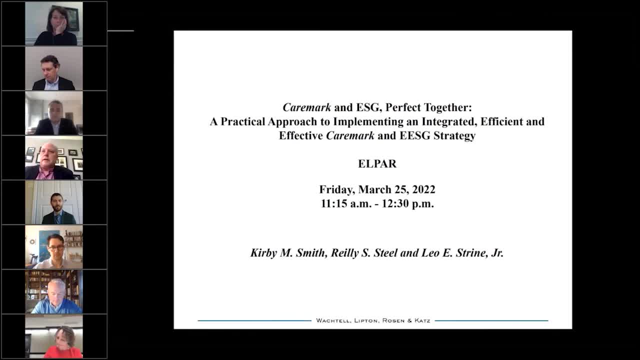 to be called corporate social responsibility. And in between that we had the focus on TSR- total stock return, which has never gone away and will never go away, And companies have been told to manage to the market. Companies have been told to do. 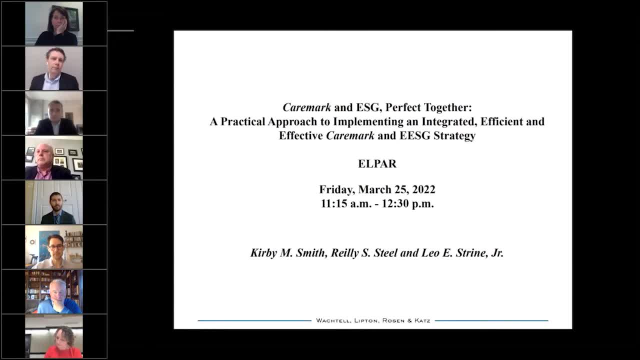 whatever their stockholders want them to do. Companies have been told to have votes on pay every year. that are votes on generalized outrage, And they're now being asked to be make money and be good to other stakeholders, which I always thought was the core mission. 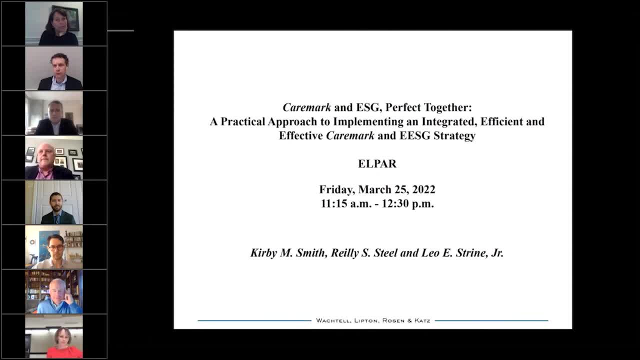 But they're being asked to do all these new things without, frankly, being given much more room to And discretion And to balance interests over the long term and focus on sustainable wealth creation, And part of what we wanted to do in this article, along many dimensions, was to provide a road. 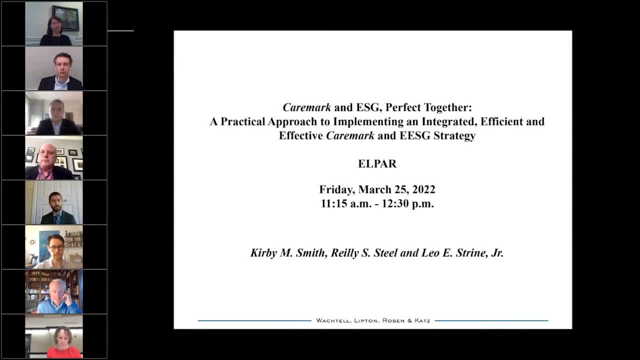 path for companies to think about this and to actually meet these competing demands in an efficient and effective way. And there's not a smooth road, for example, for a company like ExxonMobil to transform itself from an energy producing company that's carbon intensive. 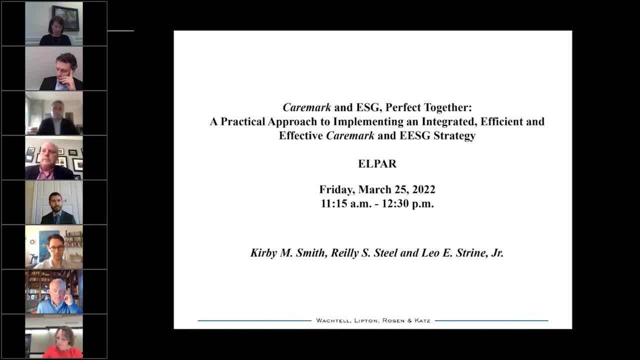 to one that's not, And I've said to my friends that the little engine that did is. will they be there at every meeting? and when the earnings are not smooth to get there, will they be able to do that? And these challenges exist for every company, not just in the environmental front. So what? 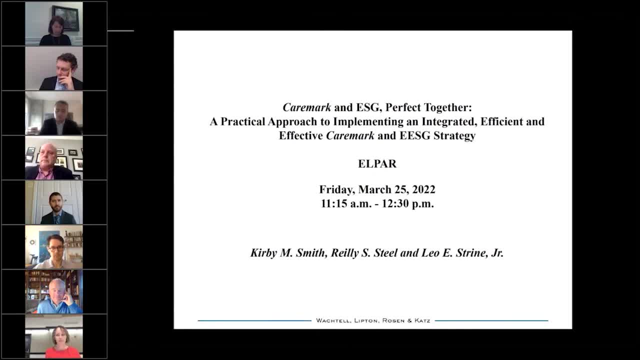 is our key insight. Our key insight is to remind people a little bit about what we do in this country in terms of chartering corporations, which is, whatever the debate about Milton Friedman and all this stuff, The reality is: the first obligation is to be able to do the 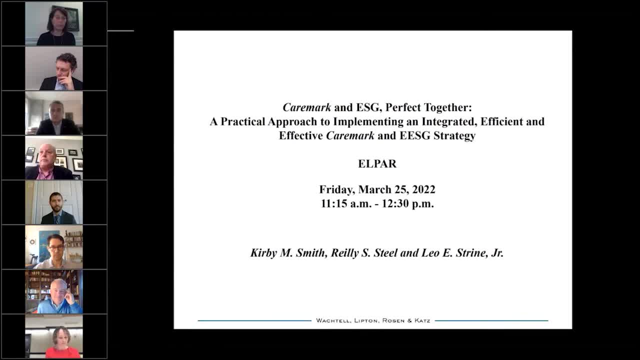 job. The first obligation of a chartered business in United States is to do lawful business, only by lawful means. You can't pursue profit outside the bounds of the law. We also realize, though, that companies are under competitive pressure, and that companies also are under pressure to go beyond the law or to state their values on things, And that's 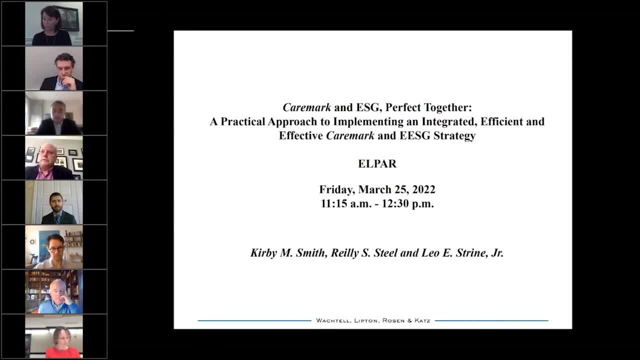 sometimes, when busy people get hit with situational stuff that's not thought out so well. they don't do it so well And what we have perceived is, if you look at the structure of companies and how they address EESG issues, it's not that well thought out And you also have- you often have the environment. 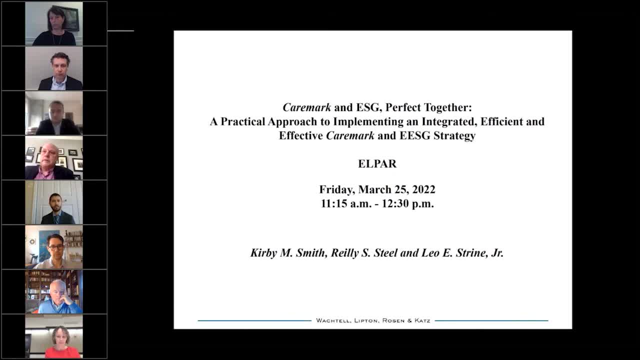 the E for environment done in one place, for sustainability reports and for complying with the core statutes that the company must comply with with a different group of people. We forget that where companies rub up against society is typically where the law rubs up against them, And what we propose is an efficient way of thinking about these things. 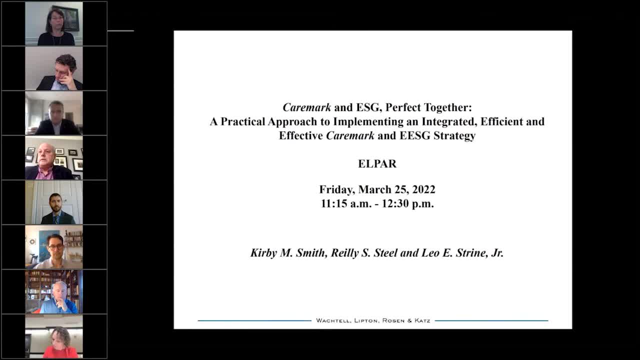 And we base it on evidence. And the reality is that, keeping an eye on the legal bottom line, make sure a company recognizes what society thinks is important, And so it doesn't become a founder's cult of personality where they're good to one stakeholder but don't recognize 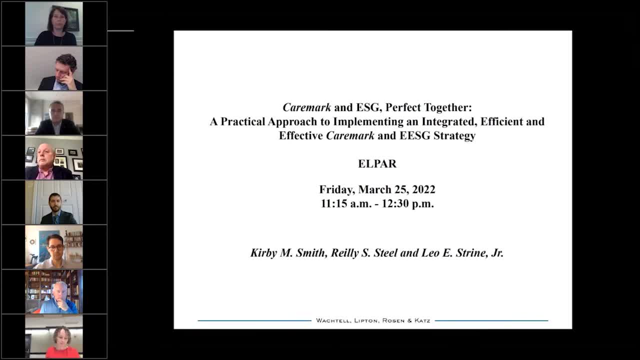 that society expects a broad range of interest And, by the way, that was a profound problem in corporate America. Many people talk very high-mindedly about the environment while not treating their workers particularly well, for example. But the other thing is we know that. 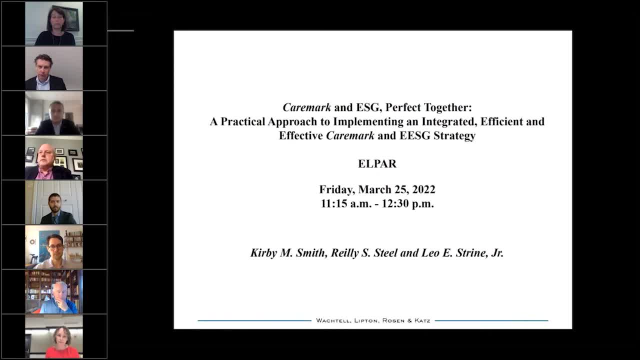 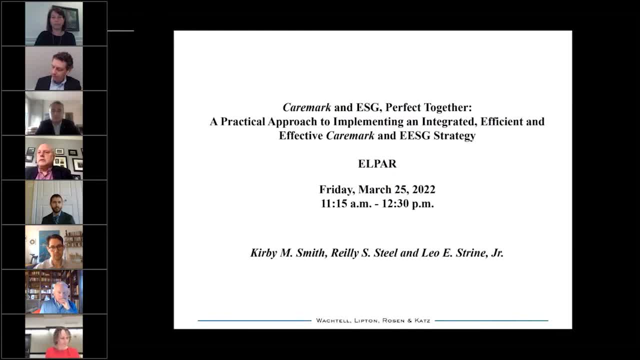 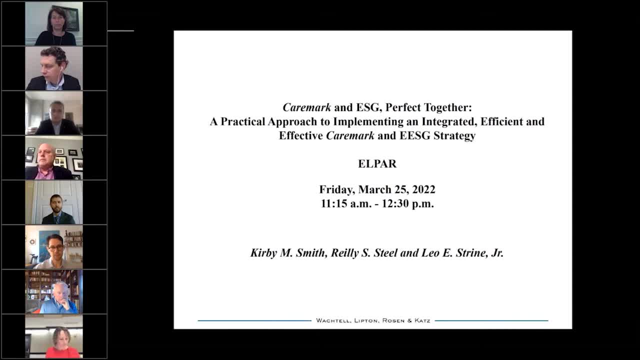 role, how it relates to our society. For many of us that has a real uplifting effect in our willingness to do our part. But we all know that there are grumpier people who will only do something if they have to do it, And so the legal bottom line not only helps you not miss a. 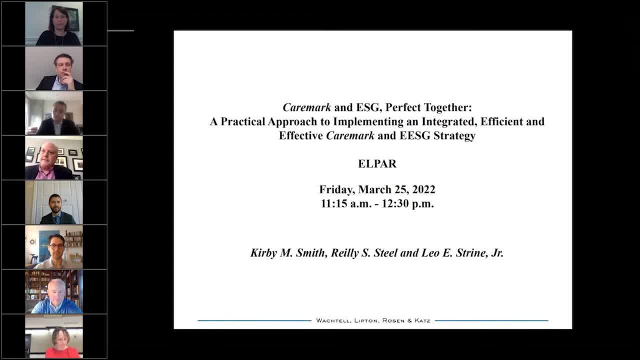 risk. it gives a certain oomph to what you're doing, But these things are not unrelated. And the other thing I think what Riley and I will talk about I'm going to turn it over to him- and some specifics of how corporate America could potentially do better, particularly as 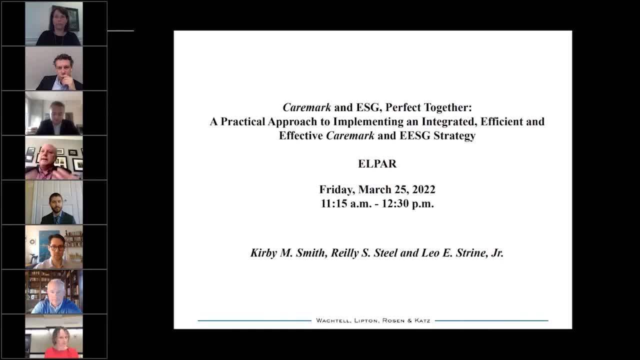 the environment is: you don't have time to do related functions twice, You risk doing them in inconsistent ways, And duplication itself is a cost. Employees are busy, Managers are busy And you want to do things effectively. So if you actually say that, as to our environmental 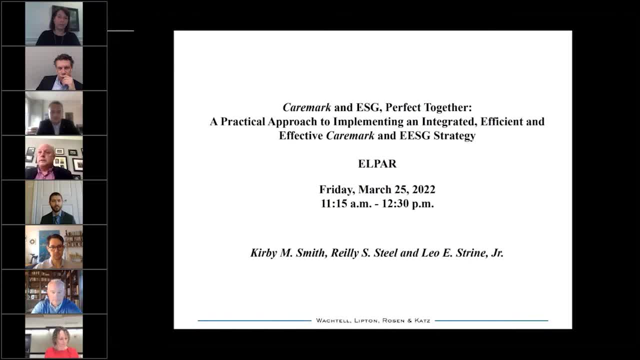 responsibility. we're going to have a focus on, of course, meeting the legal bottom line, And one of the best ways to meet the legal bottom line is to meet the higher goals we have set. We're not asking you to do things twice. We're asking you to do them once and well. We're using all of our 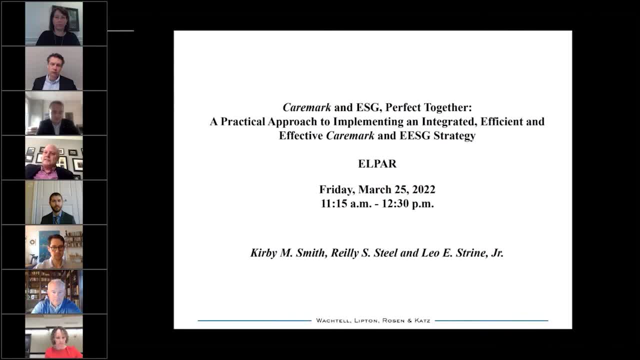 efforts. We're using our disclosure not just as some beard right to hide how bald our head is on time, But we're using all of our efforts to meet the legal bottom line, And one of the best ways to be effective is to work through Dr. 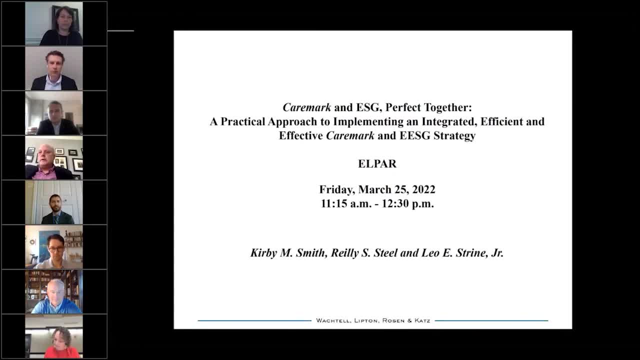 Martin's presentation of짒 existential sehening, And we're going to put it all in an integrated approach, And that's what we're talking about- is a way of thinking that actually is effective, ANd to be effective, you have to beMake. 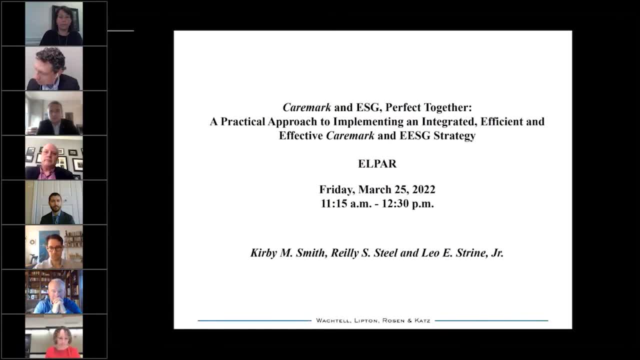 this slide result: a point of F eyes: efficiency through a program or AI. one last policy point, Really just a. one last policy, really just a support, personal privilege. I say you need an E for employees because our, our, our system of market system cannot work in our society, cannot work if the corporate 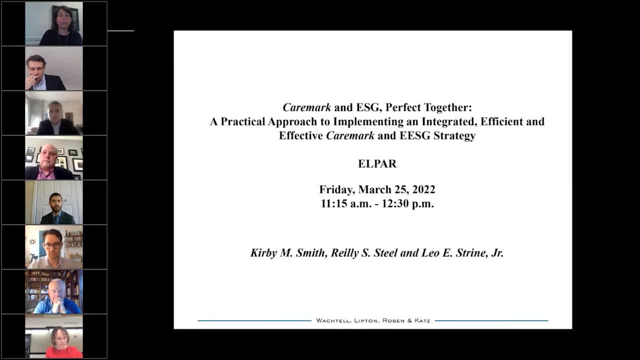 sector is not good to those people most responsible for their success, which is their workers. this is a very climate salient issue. all of us have used carbon-produced energy. all of us have used things to generate methane. we are all responsible for how we got here and the good men and women who work in. 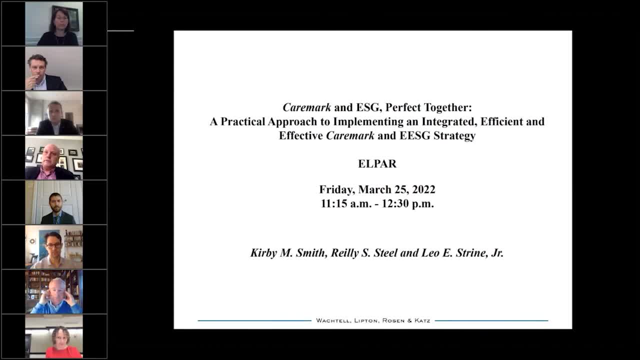 companies in the energy sector should not be demonized. they need to be brought along, and history tells us that if it's a choice between people being able to feed their families and have economic security and things like the environment, it tends that the environment doesn't do so well, and so I'd urge us all to 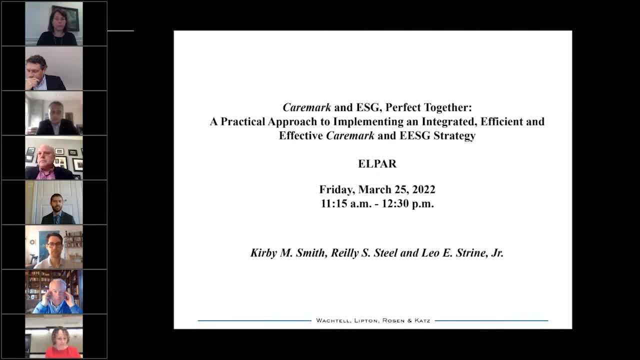 realize that we're as much as that it's a collective responsibility issue, that the way we talk about these things and the concern and consideration we have for the people who face economic dislocation is really important to solving it. and, honestly, these people have huge amounts of talent and experience and are really 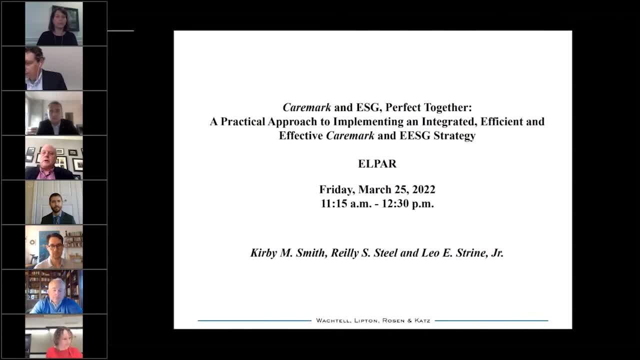 well positioned to help us make that transition. but I think our point is to make money the right way. right, Riley? you got to be good to all your stakeholders and not externalize. you can't just fetishize one. and so I'm going to turn it over my friend Riley. and if I took too much time, Riley, I apologize. 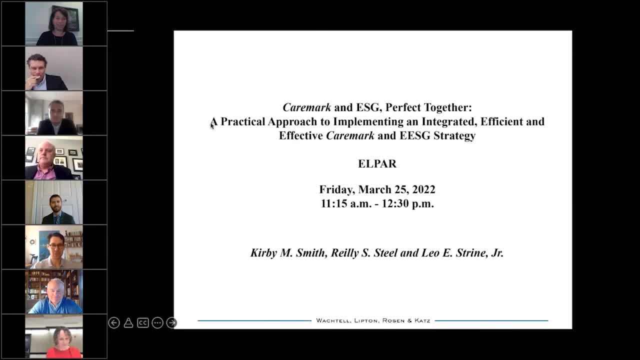 no, no worries at all. chief on thank you. I thank you for having us here. I think we only have a a few more minutes left, so I'm just going to sort of give a broad overview of how you practically implement this thing and if you want more, 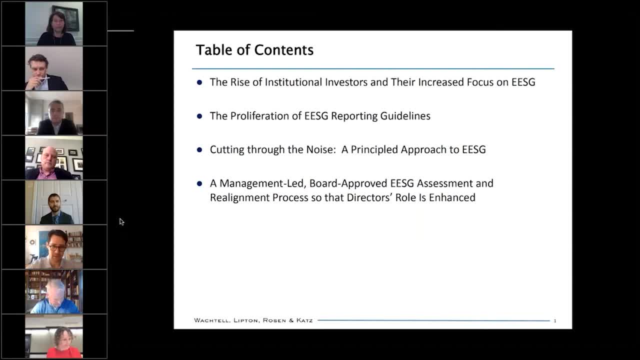 detail you can turn to the slides or the paper itself. in the paper we cover the rights of institutional investors and how they've increased. late focus on esg on. we cover the Karamark case law and how that very much aligns the sorts of cases that are. 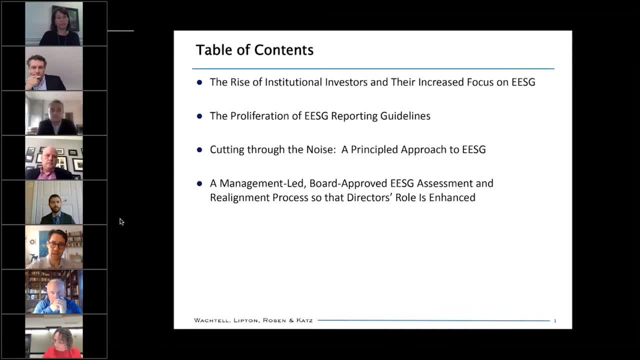 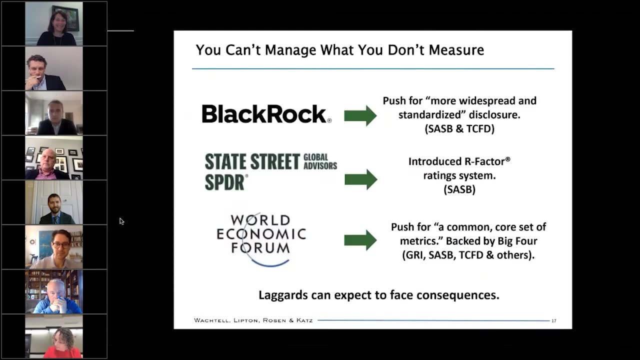 are being brought very much aligns the sorts of concerns that investors have expressed interest in with respect to ESG, but all sort of just slide over that and sort of get to the practical of how you might implement this sort of system. so that's skipping through all these slides here. okay, so our basic solution. 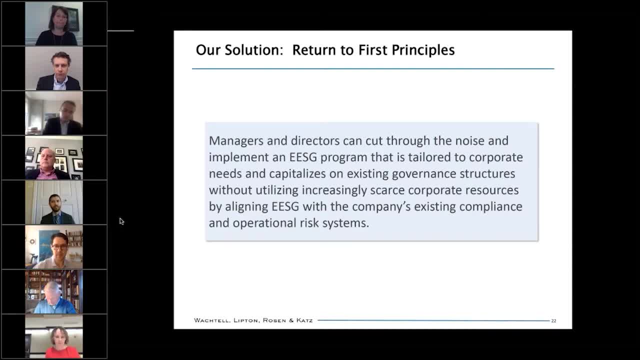 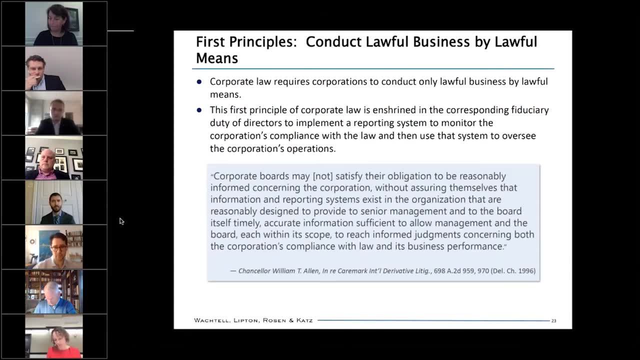 as the chief alluded to, is you return to first principles on as expressed by Karamark? the first obligation of any corporation under Delaware law is to conduct lawful business by lawful means and use that as a sort of starting point for figuring out where your ESG concerns might also lie, because 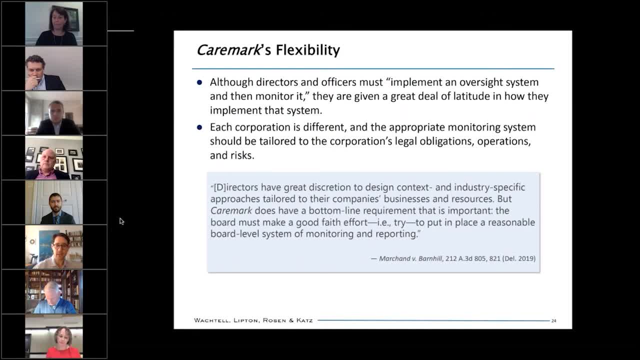 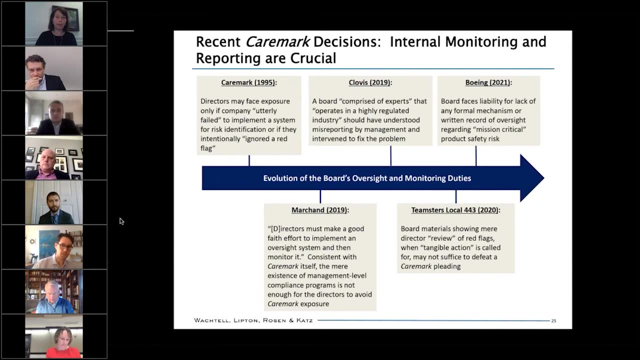 there's a lot of overlap between those two things and under Delaware law, Karamark and the business judgment rule provides you a lot of flexibility about how to manage these sorts of risks, and that can be a useful way for corporations to approach this. so you we 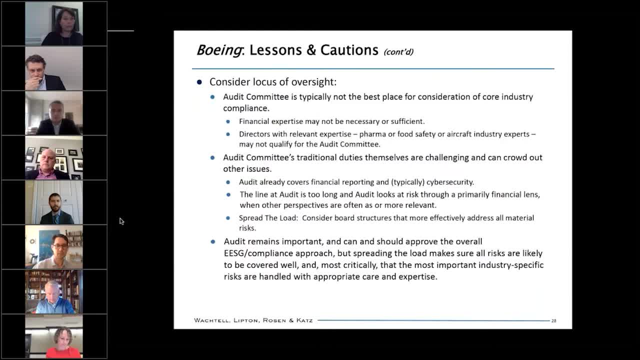 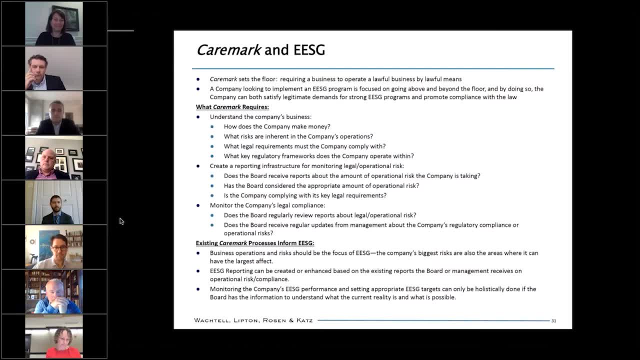 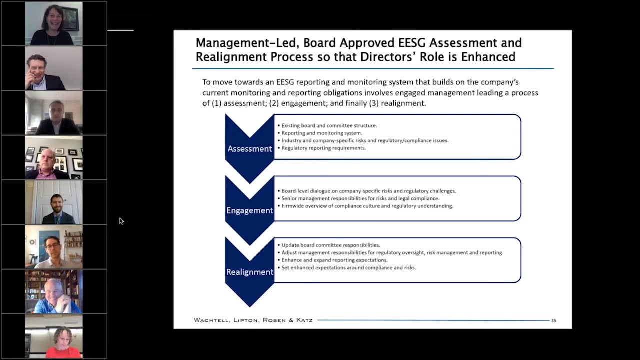 we cover the over the case law here of Karamark in the big example of Boeing, but let's sort of skip over that here on. but on, sorry, there are a lot of slides here. um, the base, the basic way you're going to cover this is: you know, right. 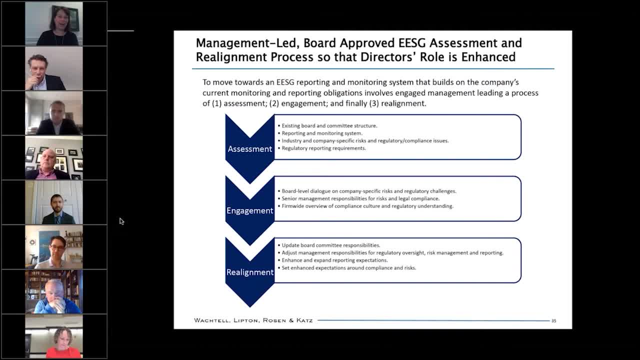 now, boards have oftentimes relied a lot on audit committees for these sorts of functions and we think that's problematic. so we propose integrating these ESG functions into all the board's committees and not just putting in the audit committee, which is already over burdened with compliance work and with 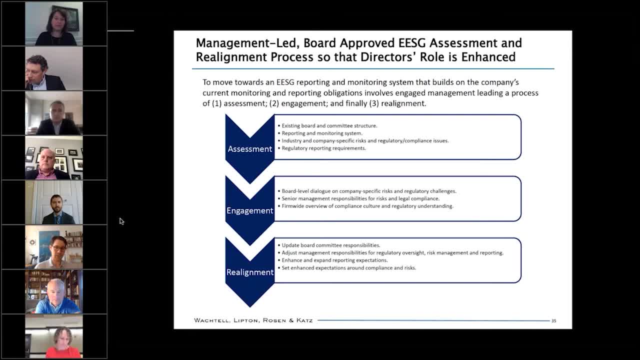 addressing financial concerns, and that's reflecting the composition of this, these committees, as well. so, rather than just lodging everything in the audit committee, we propose that the board, you know, distribute these ESG functions across committees and, in some cases where there might be a sort of mission-critical business risk, that 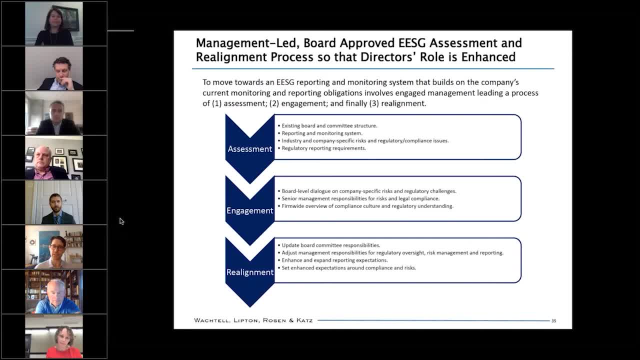 business and legal compliance risk that has the sort of ESG tint to it. it might make sense to have a specialized committee to deal with those sorts of risk and this is reflected pretty clearly in the Karamark case law and landmark Marshall and opinion that the Chief Justice authored, where the company 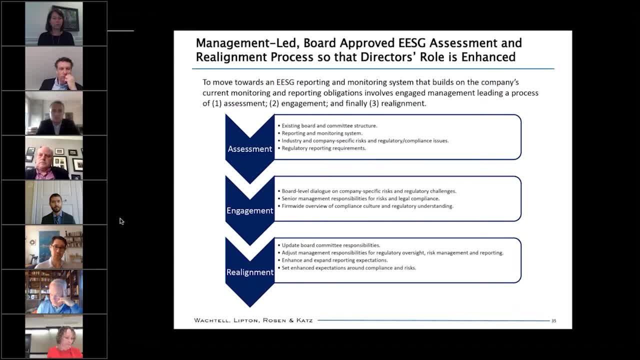 has some pretty serious food safety risks and it didn't have any sort of committee set up to deal with that. had that company had this sort of committee, they might have been able to manage that risk more effectively, both the legal risk and the sort of public relations fallout that ensued as 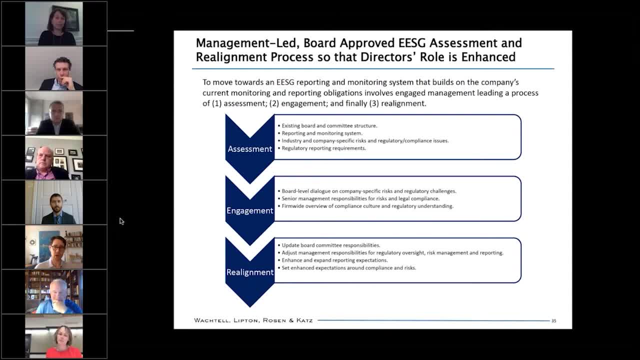 well, this was an ice cream company and they had to recall their products, so that was I was harmful to the bottom line. it hurt their image and and having set up this sort of having these processes in place to start with what it would have helped both manage that legal risk and the sort of ESG risk as well. 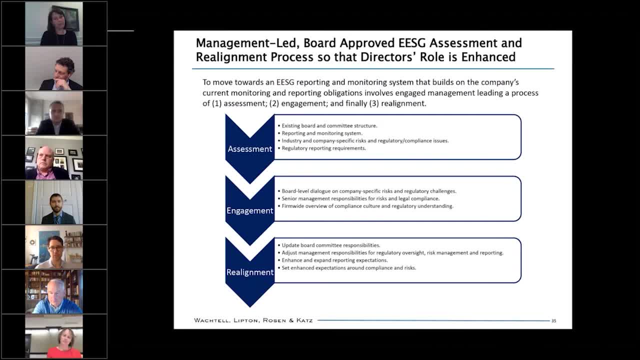 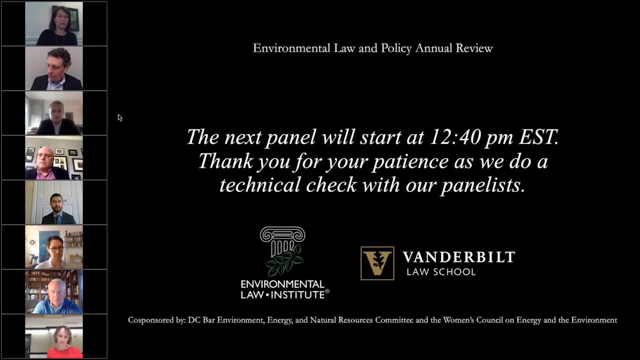 and, and these concerns are heightened even further for public corporations that have public shareholders and have to worry about demands from institutional investors as well. so that's that's the basic idea of it. I think I'll turn it over to our panelists now to sort of address this, and we look forward to your 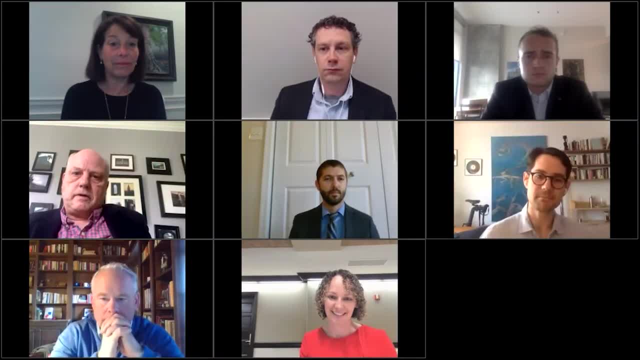 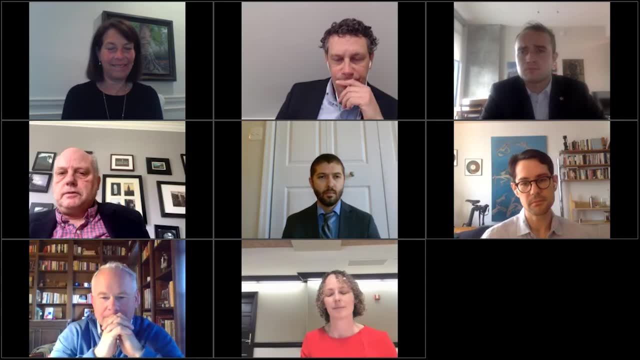 comments, unless if you have anything else you want to add. I think you have, I think we have a minute and a half and let just to put a point on it, in some of these situations you've had companies- and I don't want to pick on names, but a 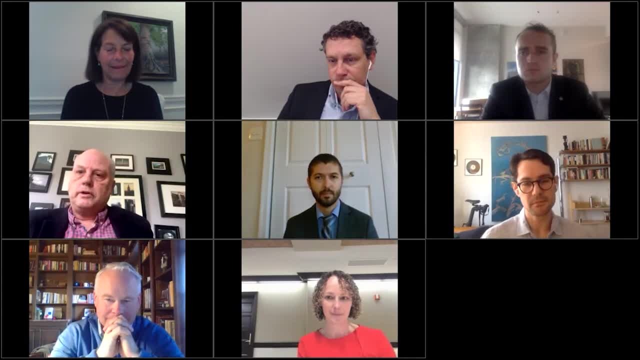 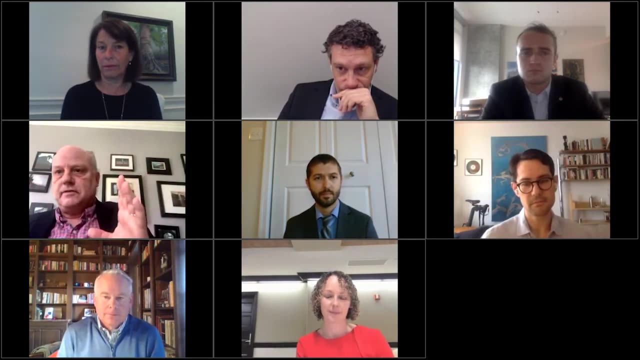 pharmaceutical company right Riley that has no core committee at the board level that deals with the specific industry risk. someone like dr Fauci could probably not serve on an audit committee because he would say: I'm not a financial expert, I'm a health and safety, I'm food safety. I could do a food. 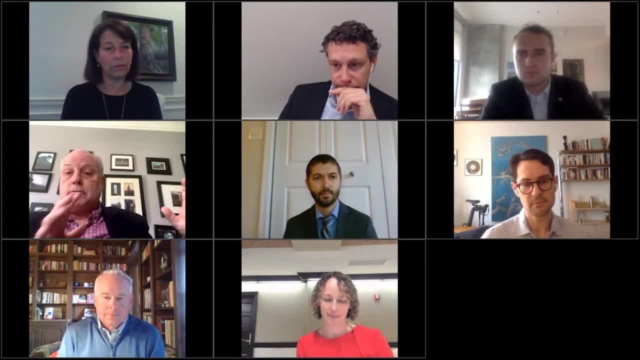 safety committee. I could do a pharmacist committee, but you're gonna put me on audit. and, by the way, every public audit committee has enough to do. and same thing with aircraft safety or other things. and, if you think about the energy transformation right, ExxonMobil, the people who can help with. 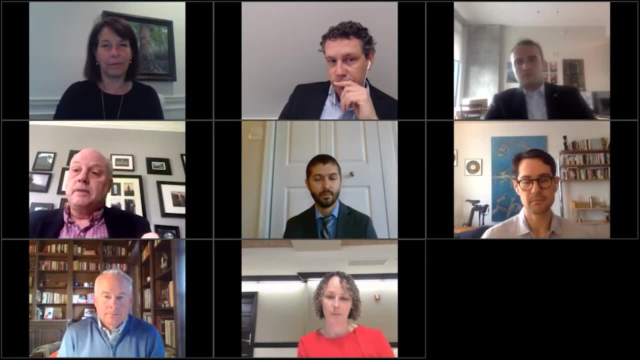 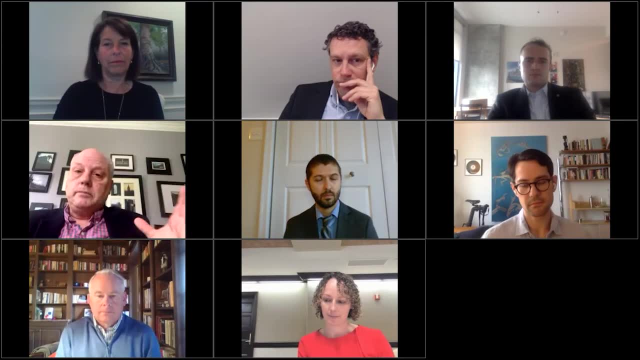 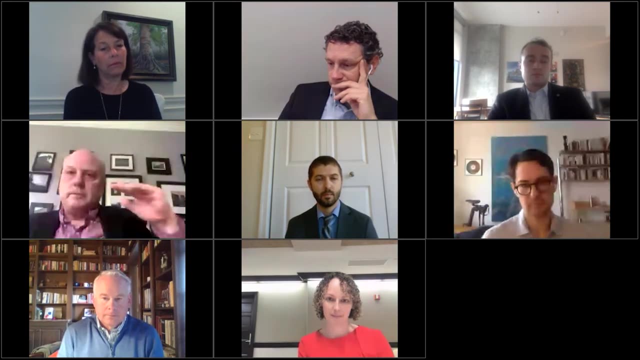 climate. who can help with environmental right? Riley may not be feel really comfortable doing accounting and to give you another example, all the saliency around issues like employee pay or DEI, or me too, a lot of the risk structures that companies actually culminated short of the board and I think what we're 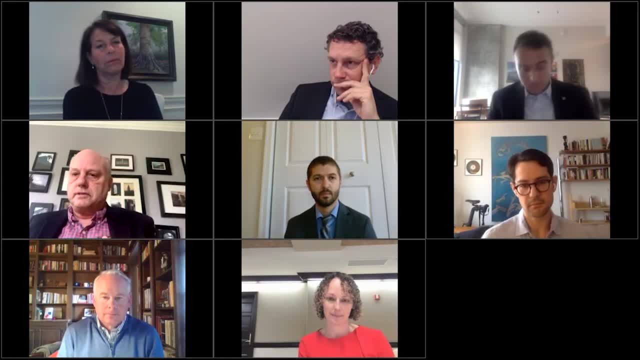 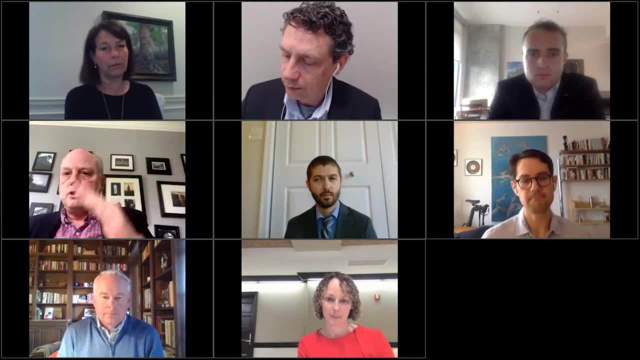 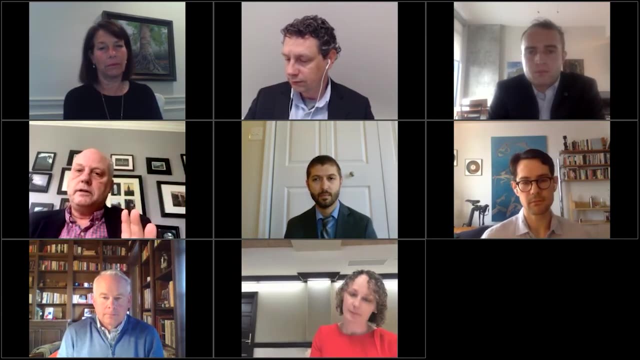 saying: Riley right is to think about your board in a business-like way. don't think of, don't separate E for employee from E for employee for compliance and EESG. don't do that with environmental and remember that for your company, something where you could hurt society might be different than another company and that 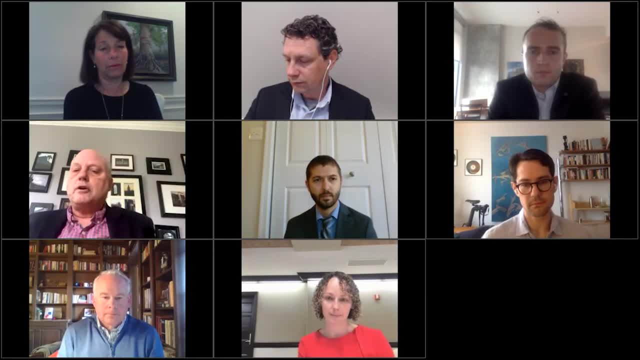 you really have to think about. I think it's a way, Riley, we're also thinking about how companies are good citizens and it's how they affect the world in their stakeholders and that if you apply that good business judgment to that, you're going to be able to also you. you know you can identify expertise. you're. 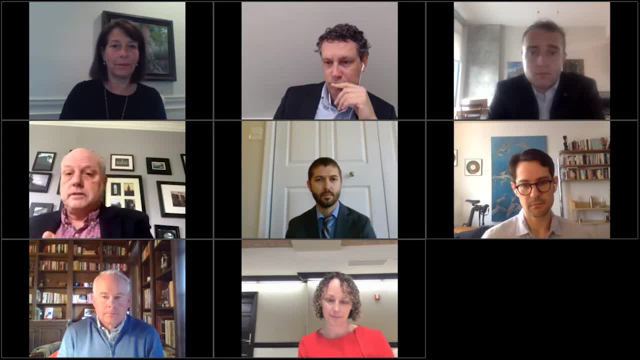 gonna want on the board and, by the way, you can find more women and minorities to do some of these things because in some of the sectors of the world, like the regulatory world or the military, people who know supply chain, who know human resources, who know 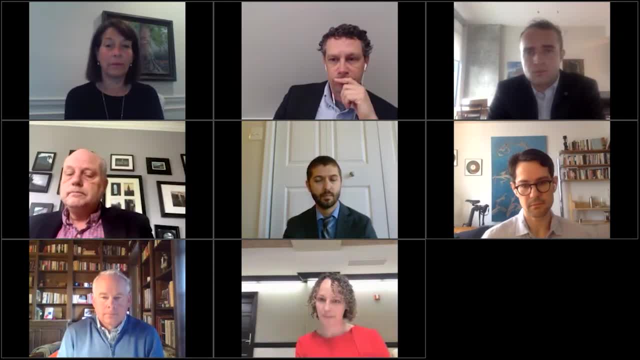 safety. it's a more diverse group, you can do it And functionally you'll be more effective. So it's a way of thinking right, Riley, of bringing a business-like approach to this, And it's a way of thinking about it where you think about how you affect the world, And that's. 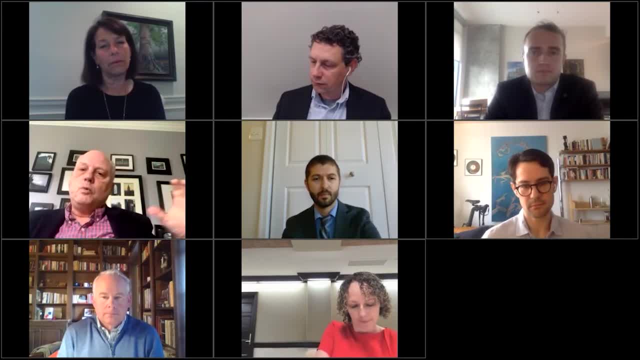 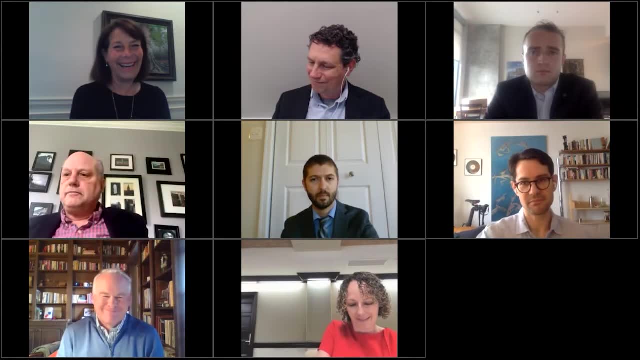 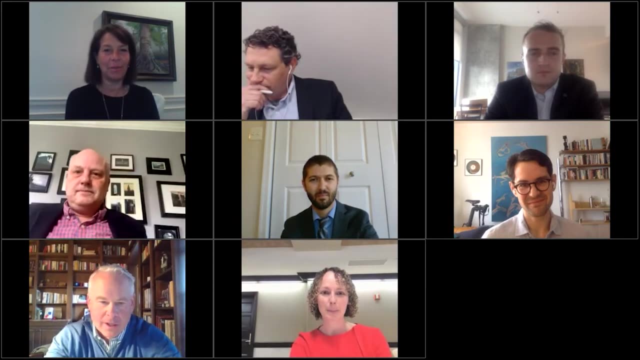 what drives you know your thinking, more than just reacting to external things. So that's a little bit of overview, And now I think we are right at 1135.. So I know you guys are amazing staying on schedule And obviously this is very thought-provoking because questions are 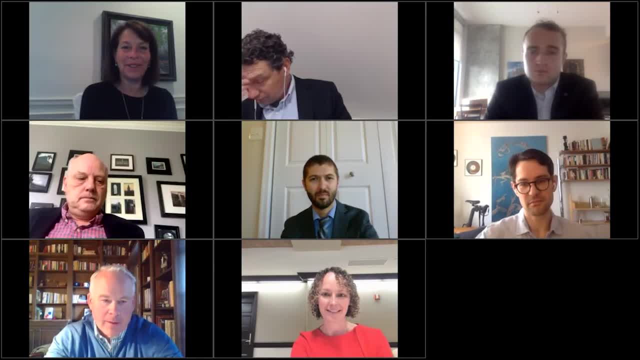 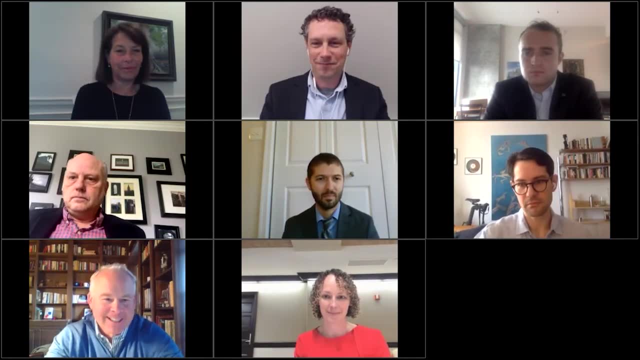 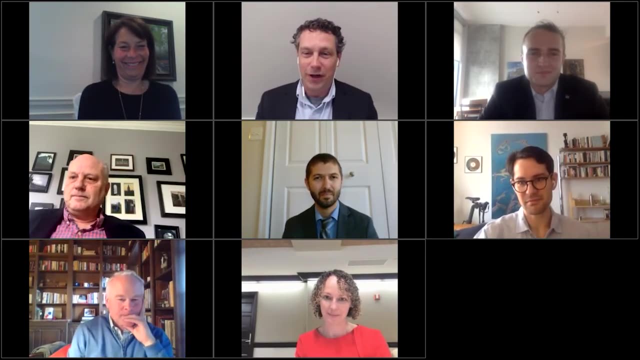 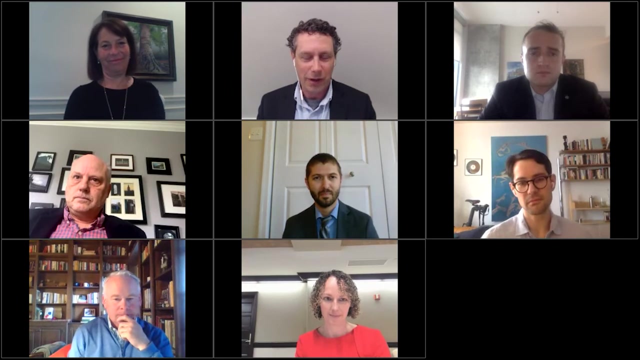 pouring in Great questions. I think we will turn first to Jonas for comments. You can imagine what the Strine courtroom must have been like watching this. Well, first, thank you very much And I really appreciate the author's thoughtfulness and forthrightness in sort of putting together this paper And really 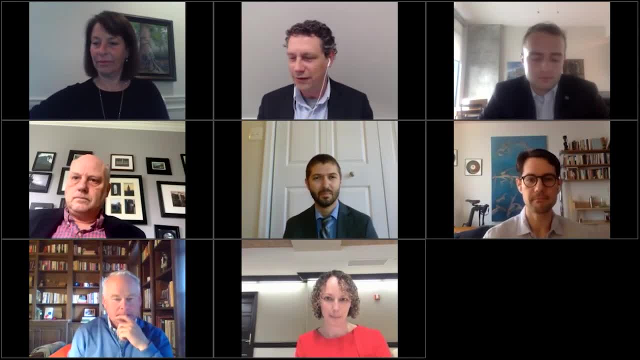 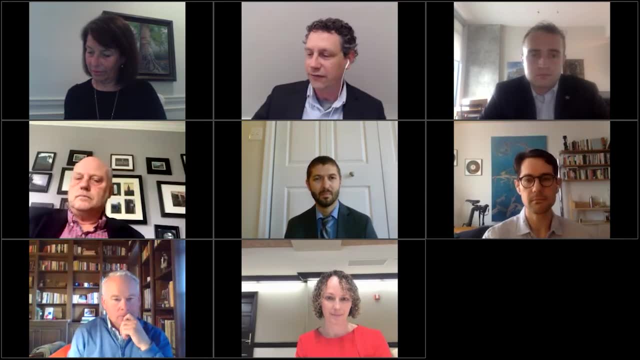 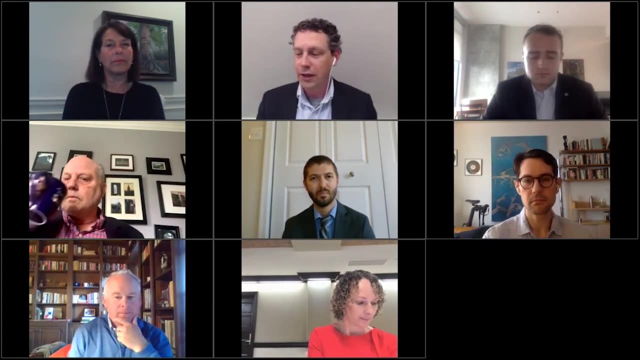 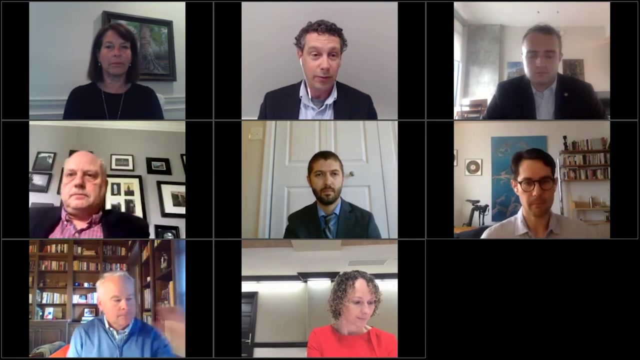 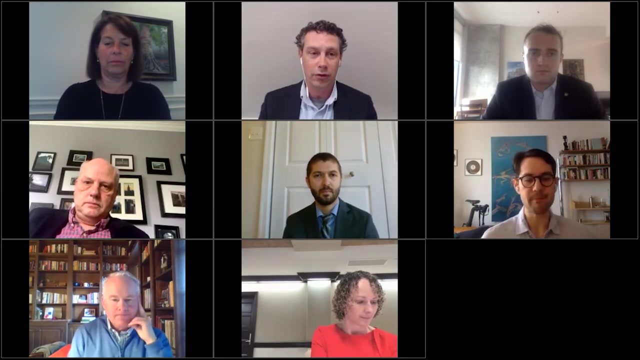 I do find it very thought-provoking And thank you for the opportunity to provide my thoughts and perspectives on this. I guess I would just say a few things at the top as a way of context for my own particular question. Thank you for your comments, And the first is that Trillium Asset Management- and I'll talk a little bit about who we are- is not representative of investors more broadly. You know, the investors of the world come in many shapes and stripes And actually that's sort of the beauty of it, you know, is that we have a marketplace with a lot of different risk profiles, a lot of different goals, a lot of different philosophies of investment And we have our own particular approach. 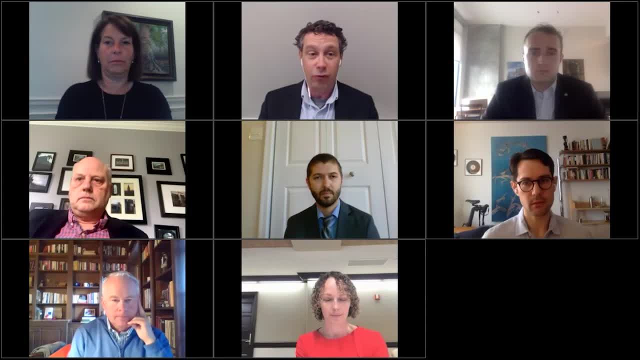 Trillium has been around for 40 years. We're actually in our 40th anniversary And we manage about $5.6 billion in assets. We do that through direct accounts with institutions and individuals, but also through a series of mutual funds. We also- and I should probably say this at the top as well- that two years ago we were acquired by a large global Australian financial services firm, Perpetual. 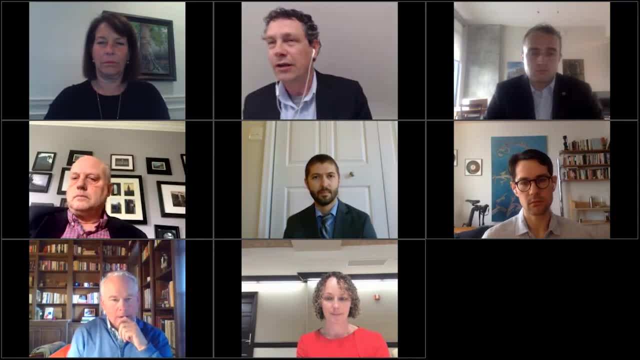 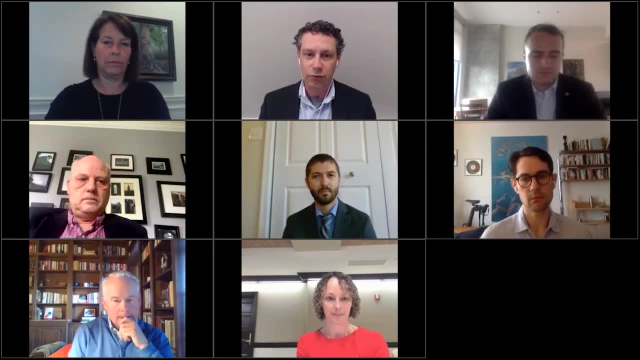 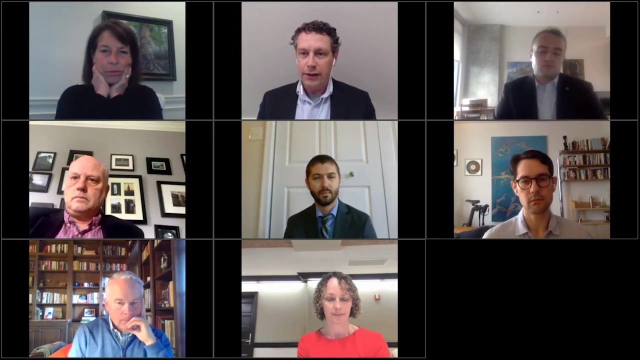 Perpetual Limited. But our history actually, I think, provides some distinctions that I think are probably useful to draw out here when thinking about these questions and the questions raised in the piece, And that is the distinction between ESG or EESG and SRI, And I think Leo sort of mentioned this sort of earlier that you know, socially responsible investing was sort of the precursor. 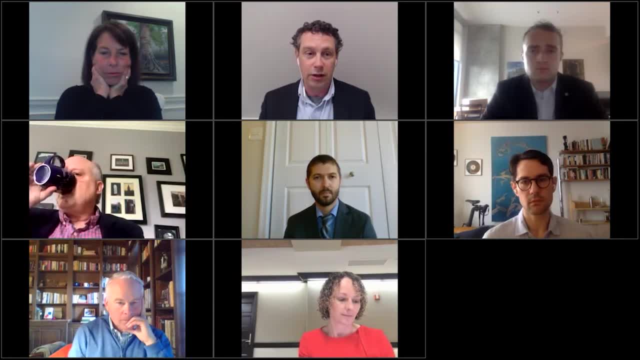 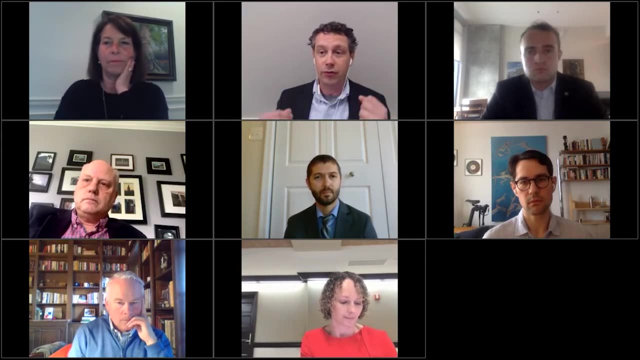 And to some extent, that's perhaps true that you can look at it as sort of an evolution, But I think, at the end of the day, that's actually not where we have found ourselves, that the field of investment as to you know, whether you call it responsible investing or socially responsible investing, or ESG investing or impact investing- has actually become quite nuanced and stratified into a lot of different pieces. 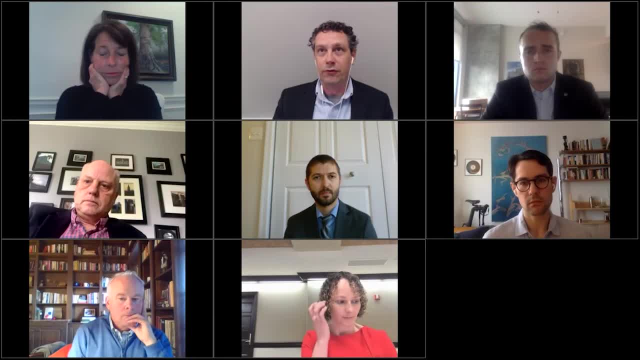 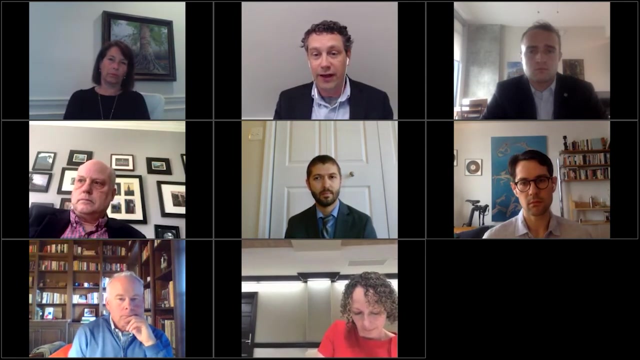 And that they're, you know, one way to sort of draw the lines, And I think that's a distinction that's becoming increasingly important, And that's a distinction that's becoming increasingly important, And that's a distinction that's becoming increasingly important. 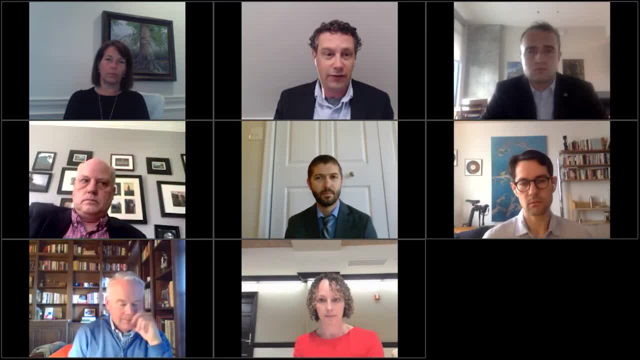 And actually we're seeing a lot more discussion of that in current events and actually seeing how companies and investors are reacting to events in Russia and the Ukraine and where our material decisions being made versus where values decisions being made. So I think that might just sort of be one sort of initial observation on the paper is I think that distinction between those two roughly speaking investment philosophies is something that I think could be drawn out more. 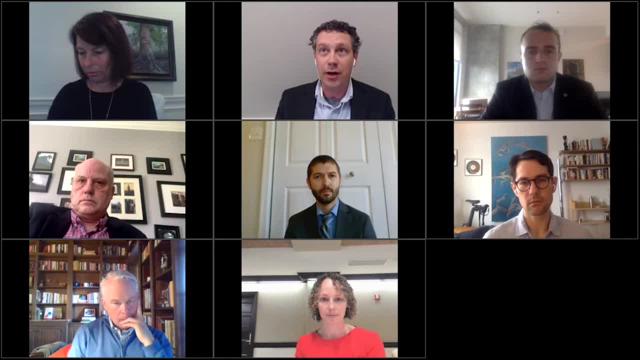 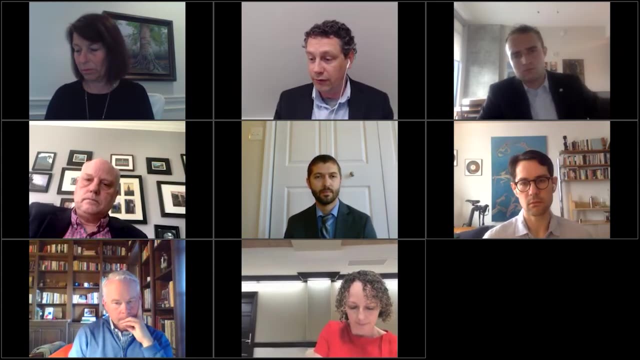 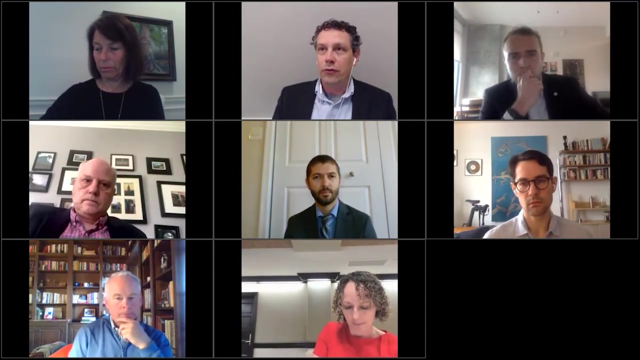 And I think that's a distinction that's becoming increasingly important. So I think that's a distinction that's becoming increasingly important. I should probably pause here and say: I'm the chief advocacy officer. What we do is we invest in companies that we are very happy to be investing in. 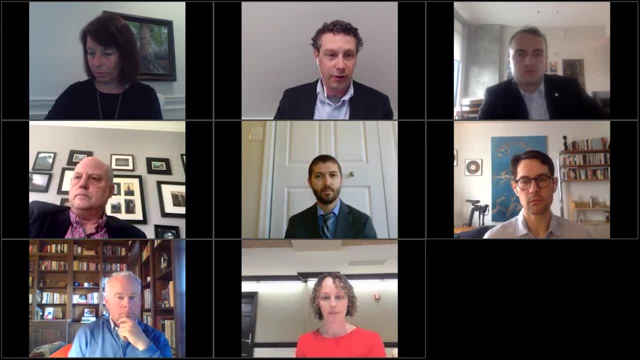 because of the way they treat the environment, their social impacts, their governance structures. But every company can do better, And every company has opportunities to avoid backsliding or to become a leader, And so what I do in my team is engage those companies. 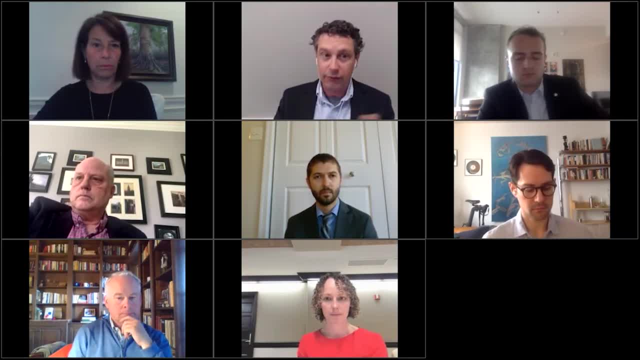 that we hold, that we are happy to be holding for ESG reasons and for SRI reasons, but to get them to take further steps. And we have a long history of using all the different tools of shareholder rights, whether that's shareholder proposals or whether that is organizing other investors. 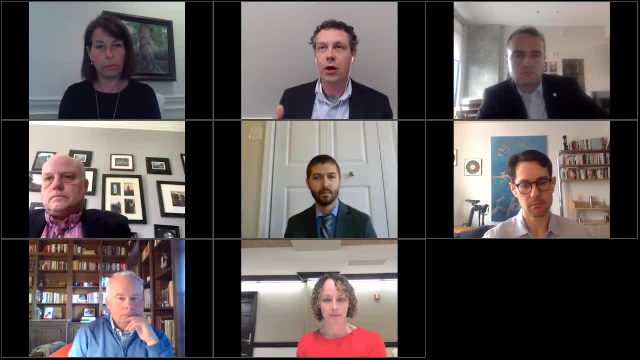 or whether it's meeting directly with companies and engaging them in conversations, or helping foster the public conversation through op-eds or other public actions to influence the direction that companies take on these environmental, social and governance and employee issues. One example of this, going all the way back. 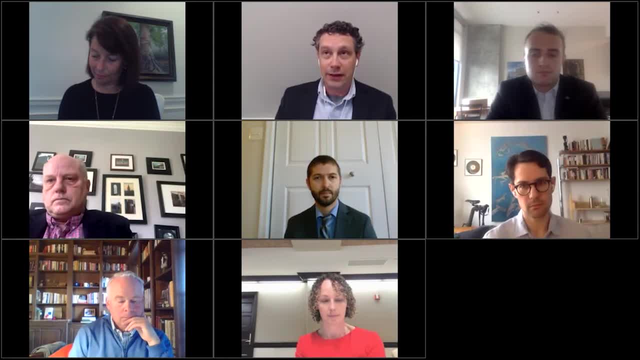 to our inception, or almost all the way back to our inception- actually back to the 90s- is that we started, and other investors as well- going to companies to ask them simply to promise not to fire their workers for being gay for who they loved. 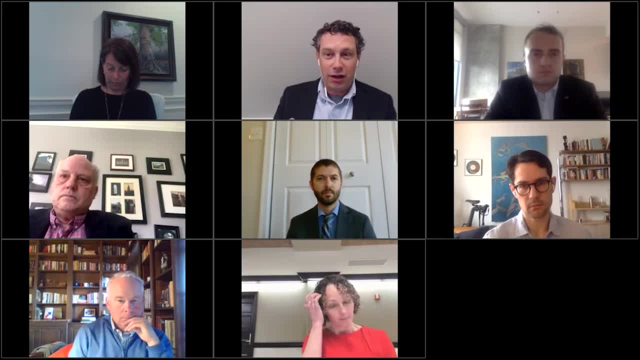 And in the 90s when we did that, companies would look at us like we had 10 heads. They thought that was totally insane. They did not know what we were talking about And in the worst cases they would be like: 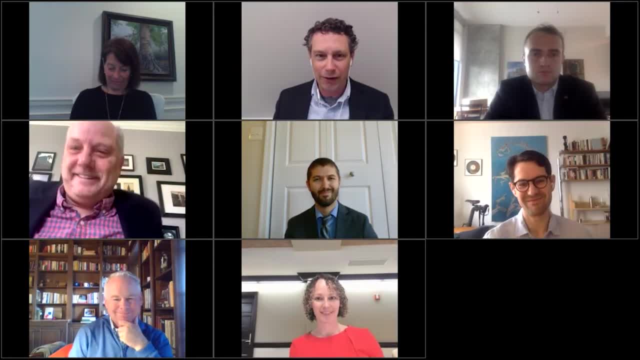 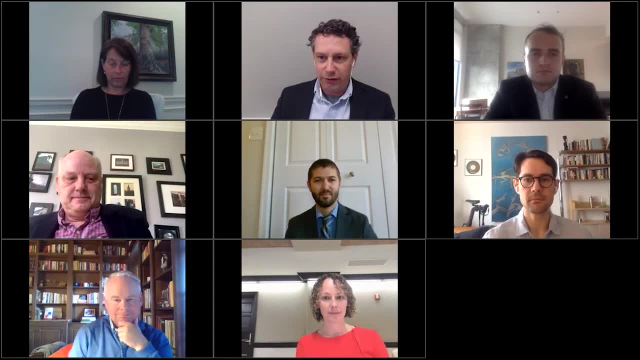 well, we don't have any gay employees. What are you talking about? Why would this be a matter of concern And we weren't? And we weren't doing it with a body of evidence behind us that this is a materially important issue. 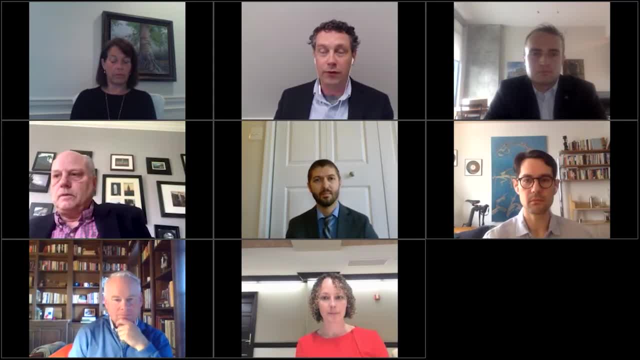 that there is evidence that a company like this is going to outperform in terms of their stock performance or even other financial metrics, But it was the right thing to do. It was something that was consistent with our values and that we thought were going to be consistent. 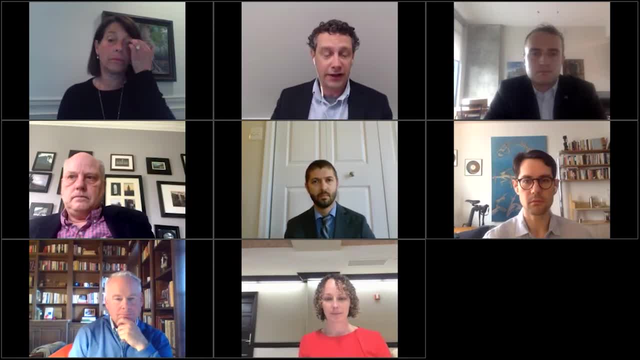 with the company's values And over the years, over the decades, we got more and more companies to make that commitment to integrate sexual orientation into their EEO-1 policies and eventually getting gender identity and gender expression into those policies and to the point where, eventually, we 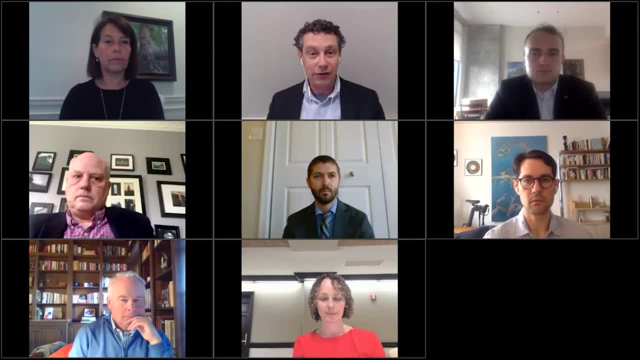 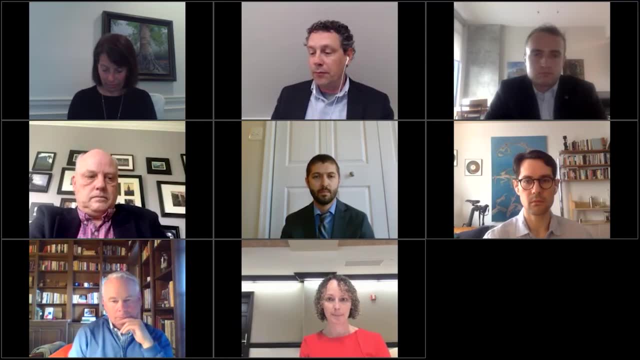 didn't need to do that because the interpretation of federal law changed and said that actually gender identity and sexual orientation are protected. But I guess the important piece of this is that I think there's a large group of investors that are going to be advocating at companies for these issues, that 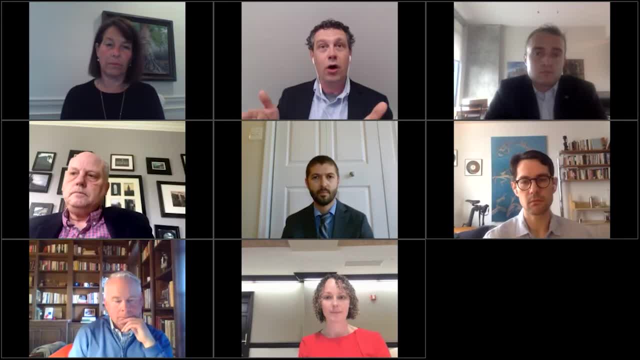 may not fit neatly within either financial argument or that there is anything compliance related for them to deal with directly. At the time, if you were going to be in compliance with your EEO-1 policies and EEO law, you could fire people. 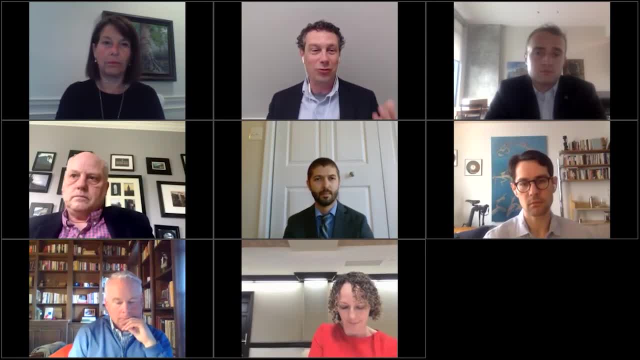 for being gay. all you wanted. You weren't going to be violating the law, You weren't going to be getting in trouble from a compliance point of view, But nevertheless it was the wrong thing to do And this is continuing to be the case that there's 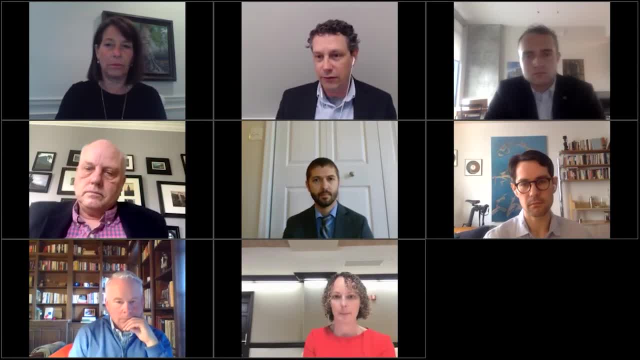 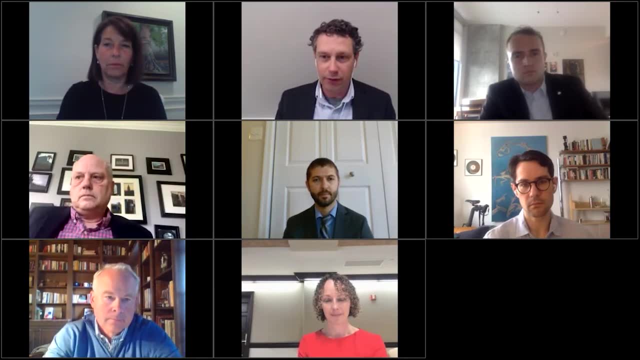 a group of investors that are sort of on that vanguard, that are looking at these issues That aren't necessarily going to be compliance related, aren't necessarily going to be material related. A couple other points here, And do I have two minutes left. 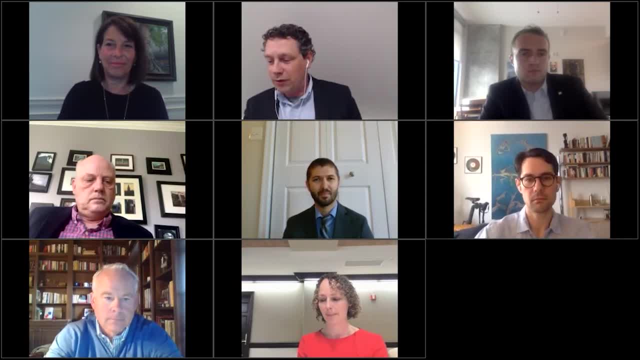 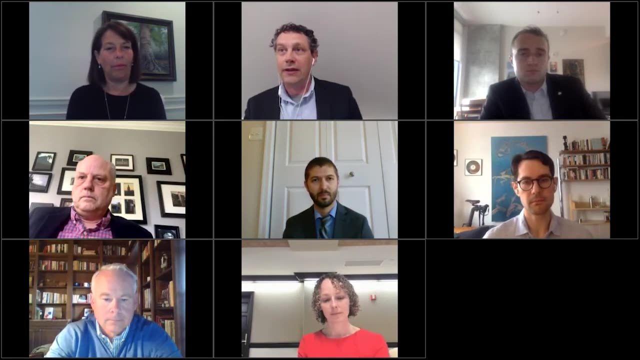 OK, I will very quickly go through these. One is that I really appreciated how the paper is sort of re-centering around the human element and being other regarding, I think, as the phrase was being used in the paper- And I think that's critical to the conversation. 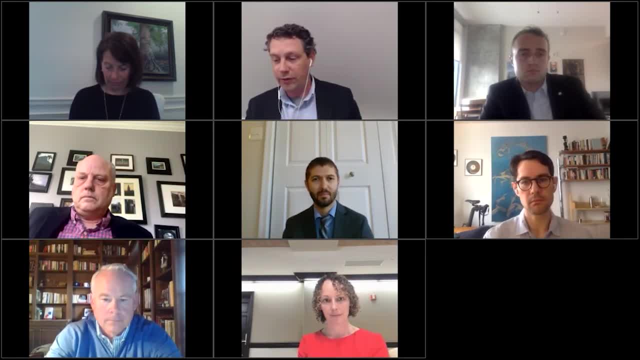 that we're having right now And I really appreciate that it was building so much of the argument around that. I also actually really appreciated in the piece in footnote 95, the discussion about signaling. There's a general effort these days to sort of say signaling. 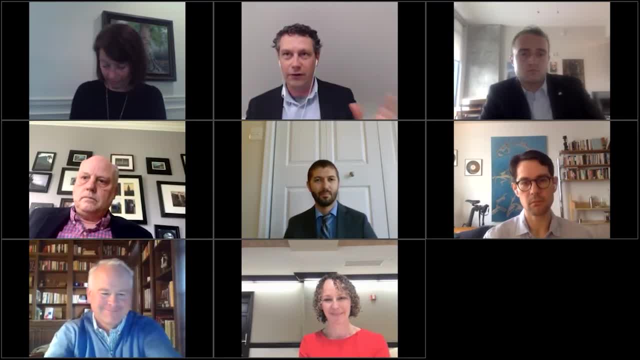 is a bad thing That companies are sort of just waving their hands and talking about something important but not actually doing something important, And I actually think that's totally wrong. Human beings are signaling machines. That's what we do to each other is. 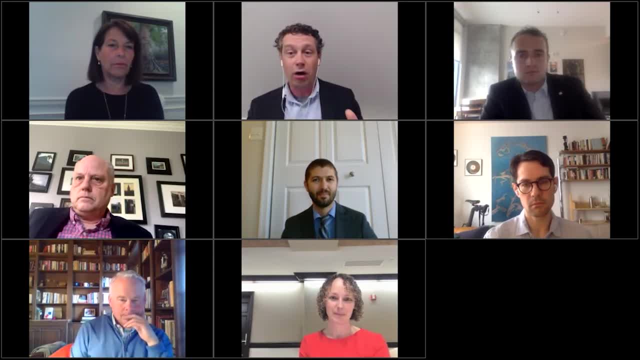 that we signal what is appropriate and what is inappropriate, And markets are all about signaling. Market signal is vitally important to conveying to companies what they should be doing and not doing, And so I really did appreciate the paper picking up on that point. 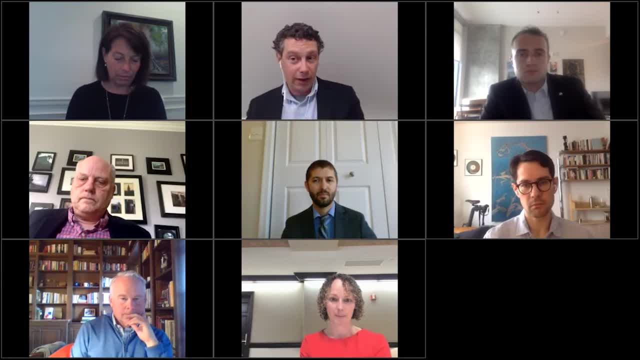 I just sort of want to underscore that signaling does need to be backed up by substance, but the act of signaling is actually incredibly important, And that's something I think that we in the legal community probably should be thinking about a little bit more. 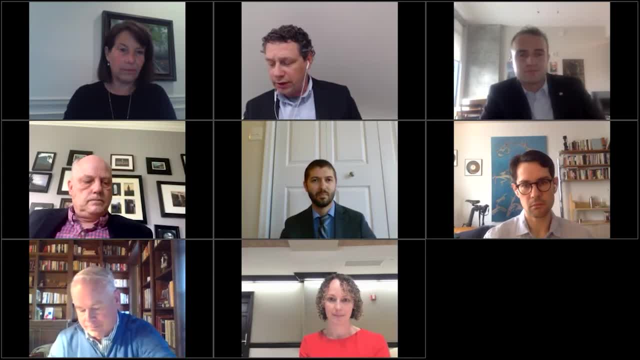 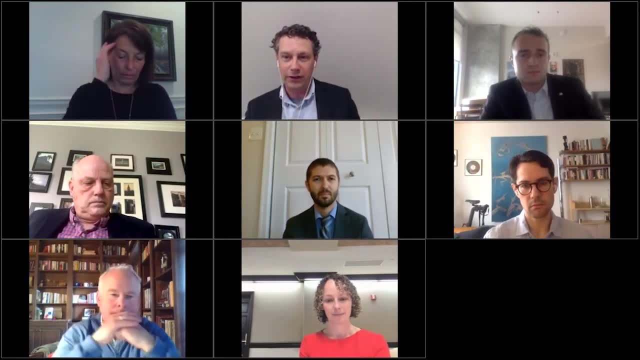 Last but not least, just to make it very quick here- is that this question about where to house ESG social responsible responsibilities in the board structure has been something that I've thought about for a long time, And I really do appreciate that and I 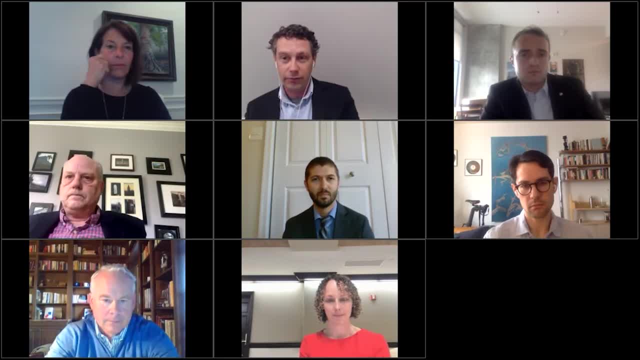 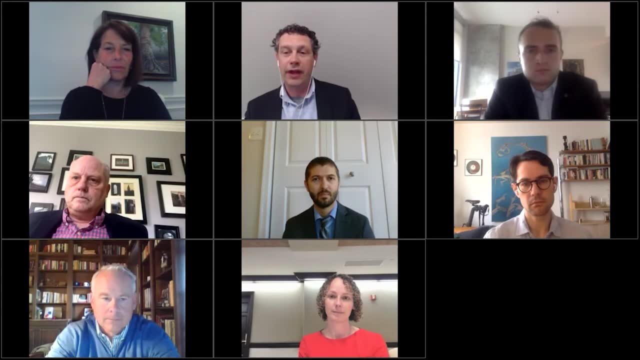 found the paper very persuasive that you shouldn't create a silo for that, or some people would say the ESG ghetto. For a long time I've actually been persuaded that it was helpful. It was helpful to have a single committee like that. 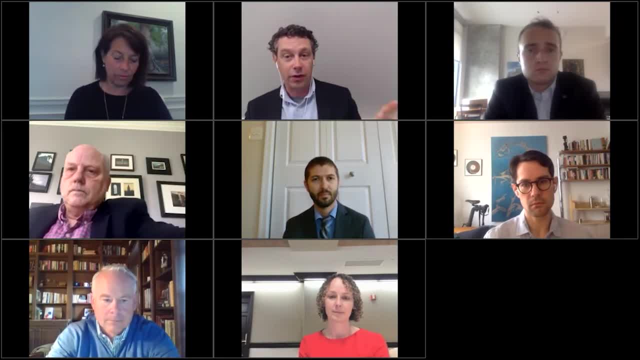 Microsoft, I think, was a good example. They have a committee that is very much focused on the public policy aspects of the company and that came out of the antitrust troubles that they dealt with in the late 90s and early aughts. 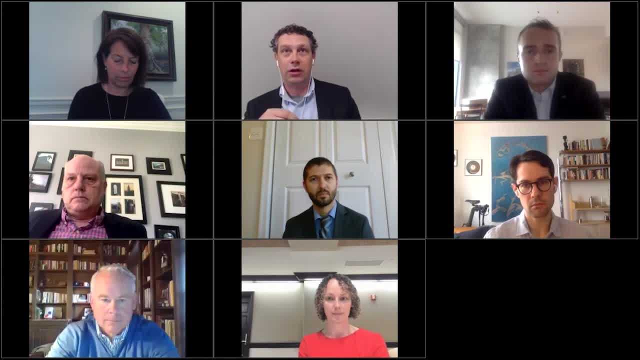 And I thought for a long time that the company managed, contrary to all the way that other tech companies managed- the pressures that they were feeling around the advances of technology and the relationship to society, that they managed that process much better than, say, Google or Alphabet or Apple. 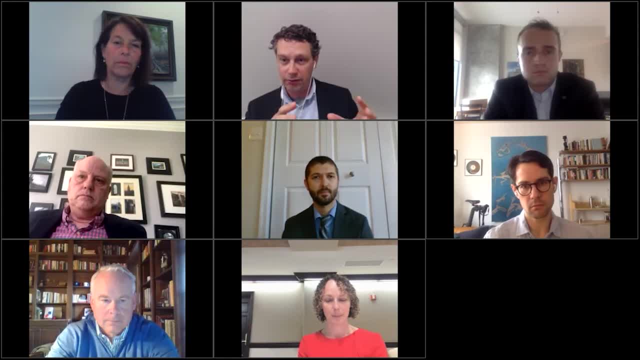 Because they had that dedicated committee to the topic. But I do find this paper quite persuasive that while maybe Microsoft is the exception to prove the rule, that really we do need to see these issues not be ghettoized, not to be siloed, but actually to permeate. 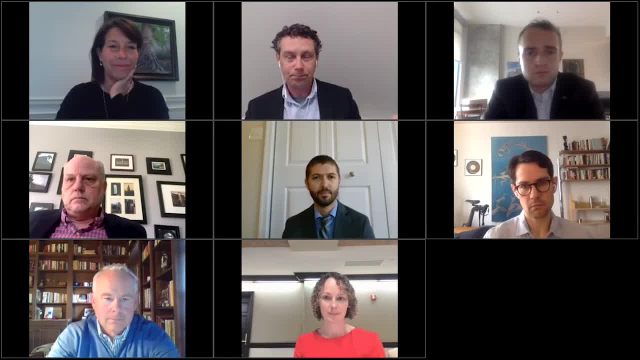 through the governance structure. So I very much appreciate that fleshing out of that idea and sort of tying it back to Caremark, And I think that is probably my time and I will stop there. But that's great. Yeah, thank you so much. 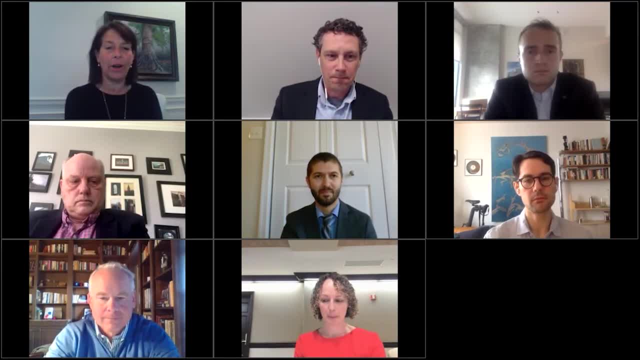 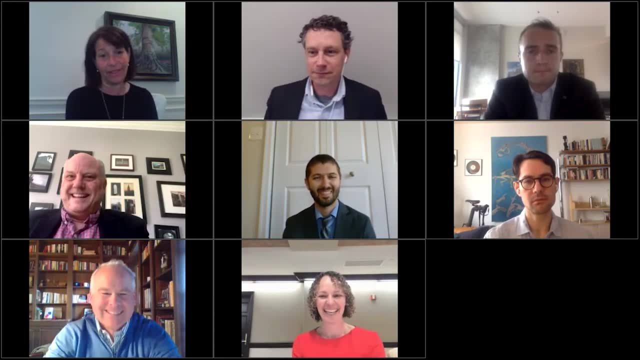 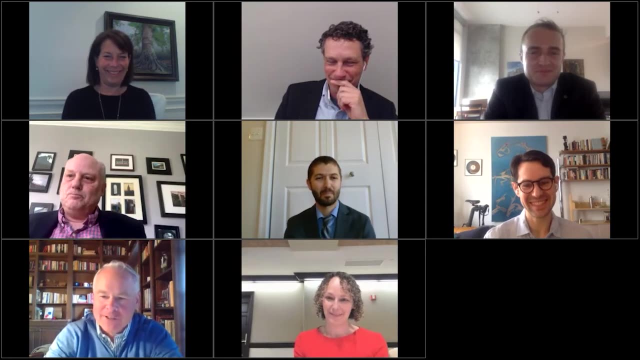 Really really interesting perspective And we're going to go to Margaret or Maggie next. And he has set the bar high because he cited footnote 95. So I hope that you read this as carefully as Jones did. I know from Maggie's guest lecture in my class. 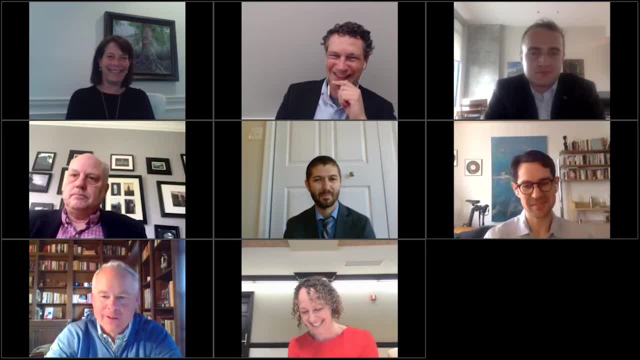 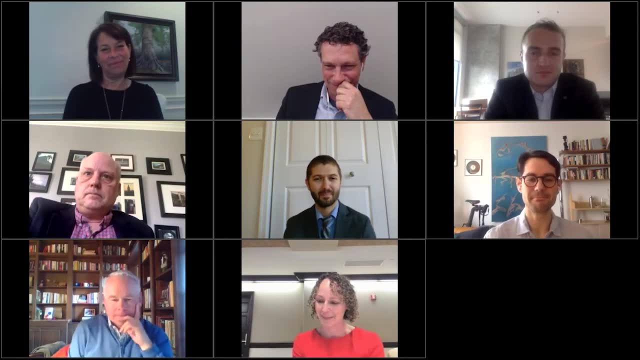 that we're going to hear a similar level of detail. It's really impressive, the group of commentators we've assembled here Now. you have set the bar way too high, Mike, But thanks everyone for having me. I'm sorry for sliding in at just the last minute here. 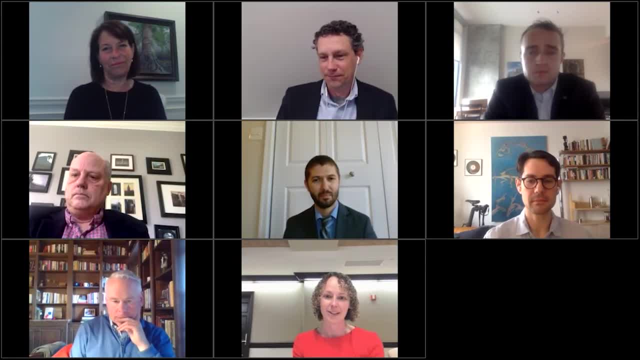 So I really want to position my comments in the context of the events of the past week that have been really significant for those of us in the climate and corporate governance worlds. I have spent most of my career as an environmental litigator and then as a climate change lawyer. 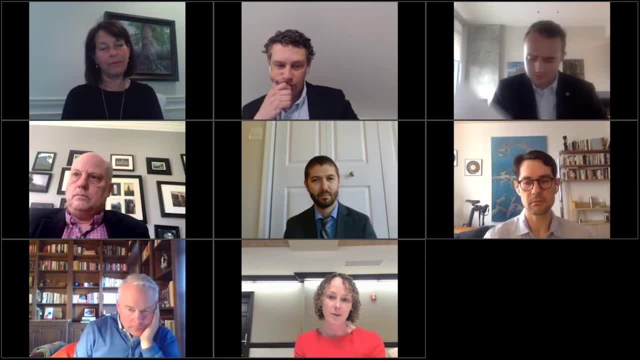 And over the last few years, a lot of that has really involved working very closely with both public and privately held companies and thinking about how should you build your climate governance. So this question of do you put a single climate expert on your board and let them sit in the corner? 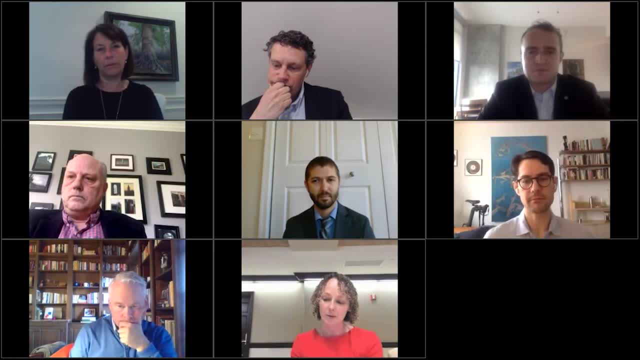 How do you think about where they belong? And so I'm going to spend a few minutes talking about some of the proposed requirements in the SEC's climate disclosure rule that came out this week, Because I thought that one of the things I would really love to hear from the authors on here. 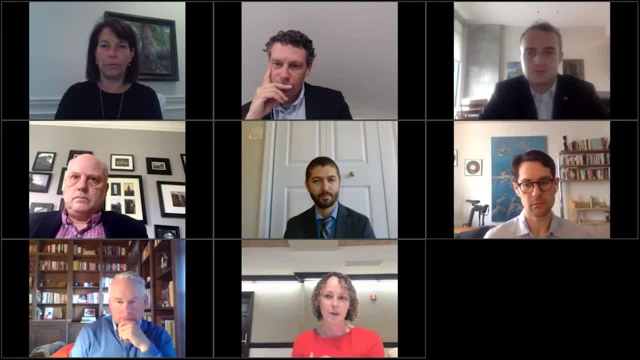 is your thoughts on this potential move into a more regulatory approach to ESG and how ESG disclosures might happen, particularly in the climate space, and what that might mean for the consequences for governance? Because I will just say up front, I think that it could potentially. 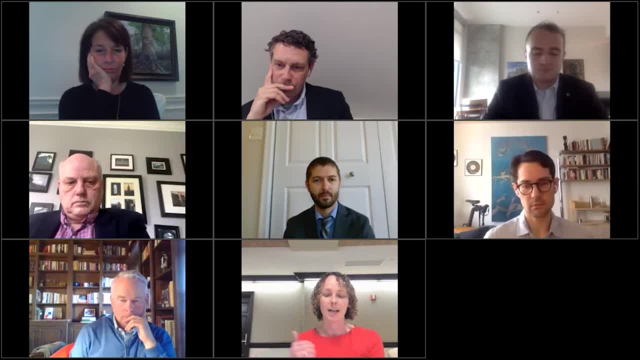 go in a couple of different ways. You could see sort of a very reactive like: oh my god. that means we now need a special committee that's really devoted to thinking about these very challenging things. But it may also- and I would argue it should- 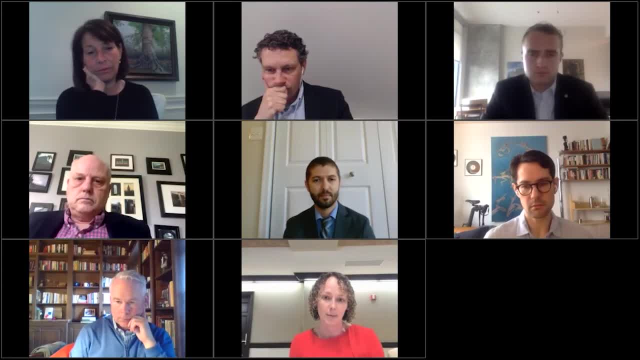 lead to a more reflective approach, similar to what you are advocating for in your paper, where companies are really being more thoughtful about the various you know things that are going on around the world, And so I think that's something that I would love to hear. 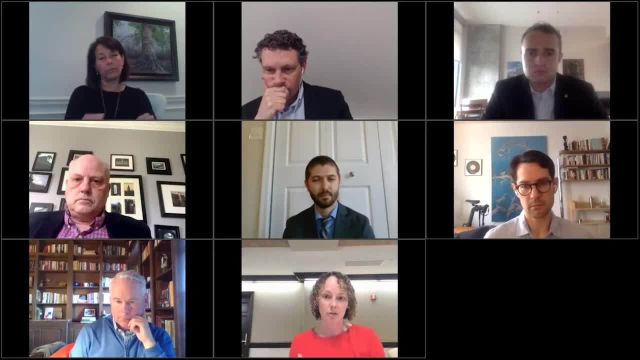 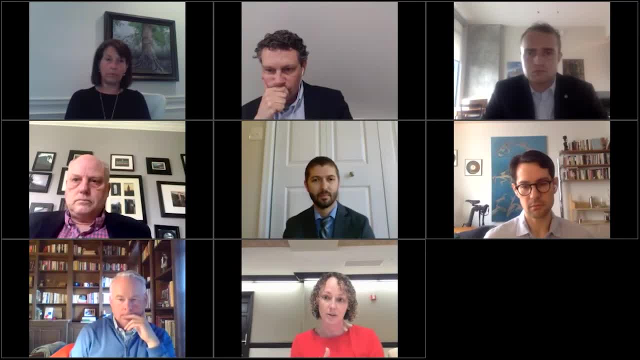 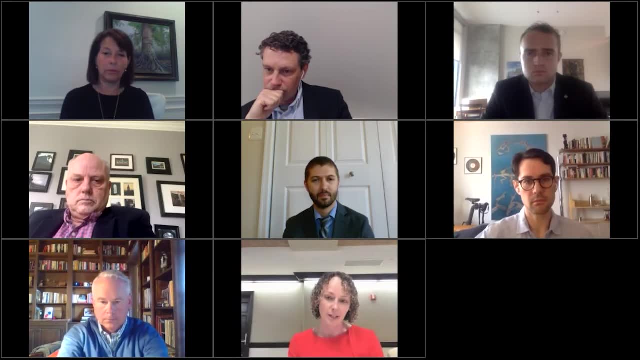 and how those permeate through the business and what that means for management and supervision. So just very briefly, for background for our audience, The SEC issued a Proposed Rule on Climate Disclosures on Monday. It is open for comment until either May 20th or 30 days. 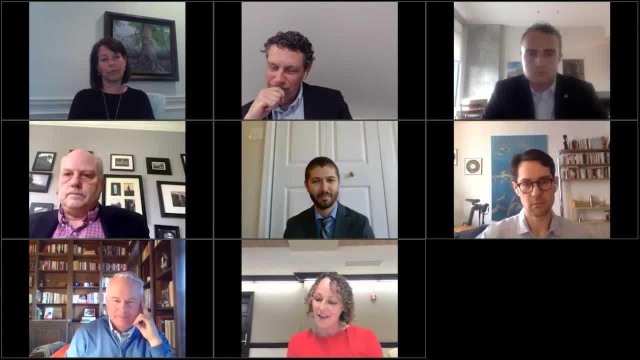 after it is published in the Federal Register, whichever is later. The rule is functionally going to propose to modify both regulations and regulations to provide a more visual picture: SK and Regulation SX. So that means both qualitative disclosures about climate risks and, potentially, notes to financials about your climate risks. In terms of governance, the rule. 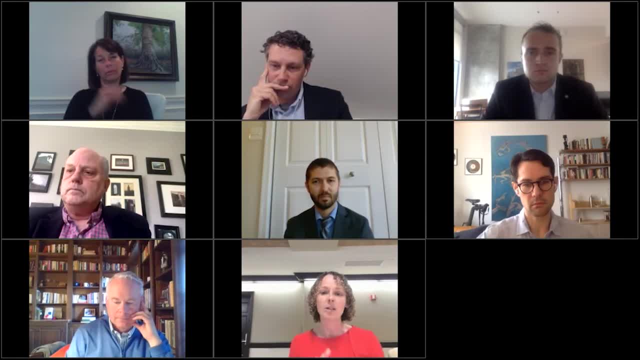 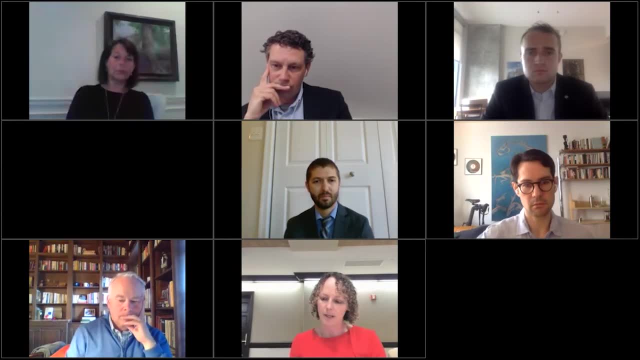 is based on the Task Force for Climate-Related Financial Disclosures, but it's looking for a number of very granular things. Among them: how your board members and committees of the board engage in climate oversight. who on the board has expertise in climate risk. how the board 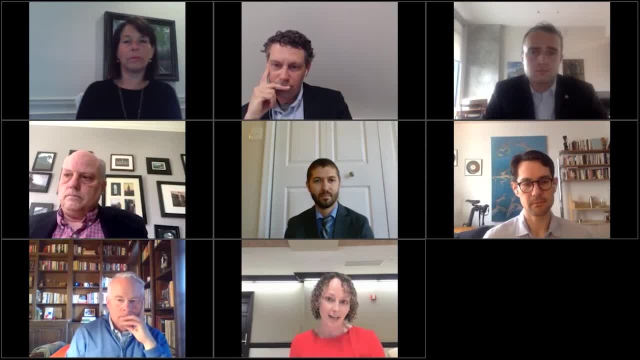 considers climate risks and how they impact strategy, and whether and how the board sets climate targets or goals. There are additionally a number of enumerated requirements for management oversight of climate that are not as granular as the board ones. The rule would also look to have: 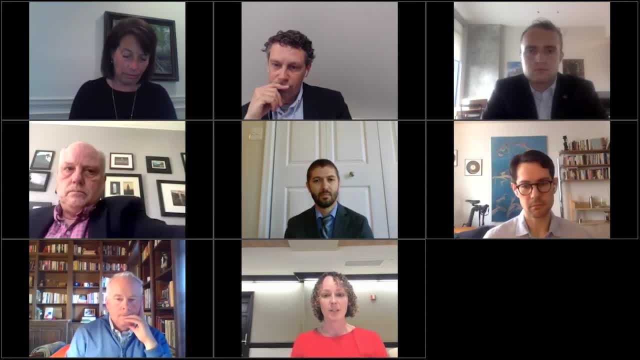 scope one and scope two, greenhouse gas emissions. So that is, direct emissions from your activities- if you are an airline and you fly airplanes, the emissions coming out of the plane when you fly them, and indirect emissions from energy consumption. So the power. 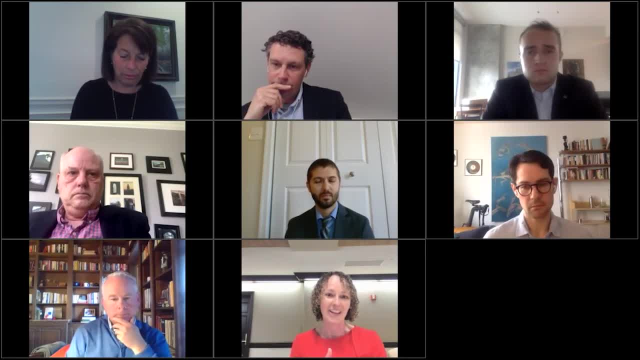 that's going to keep all our laptops running so we can be on this Zoom. And then for certain companies it will also require the disclosure of scope three emissions. So that would be emissions resulting from your supply chain, both upstream. So if I'm a power plant and I'm buying natural gas, 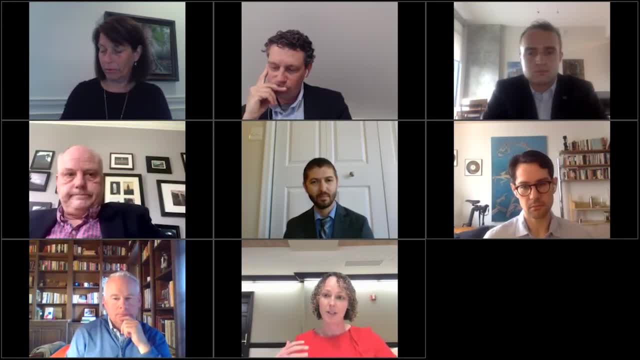 all the methane that may have been released when the gas is being produced and downstream right. If I am a car manufacturer, the emissions that come from me selling the cars to people and then putting gasoline in those cars and driving them around will be reportable. 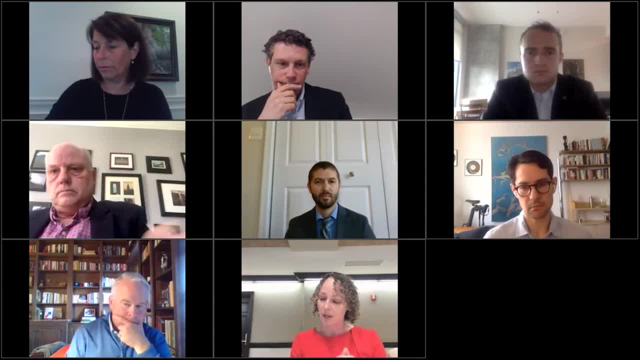 for the board members and the board members of the board. So that's going to be a really important rule for some companies And those emission requirements are going to be subject to assurance for scope one and scope two And those will be subject to the Commission's existing 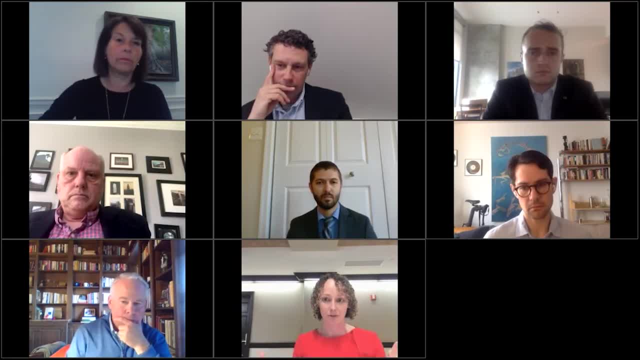 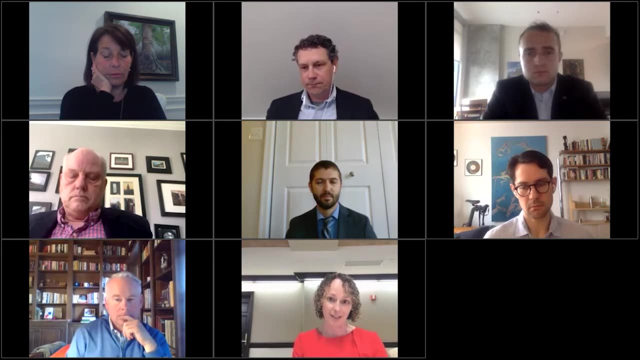 disclosure, controls and procedures. So we have a whole bunch of stuff that, as the authors have rightly noted, has often been done in silos that don't look a lot like our traditional governance silos that all of a sudden is getting swept into securities reporting if this rule is finalized, as 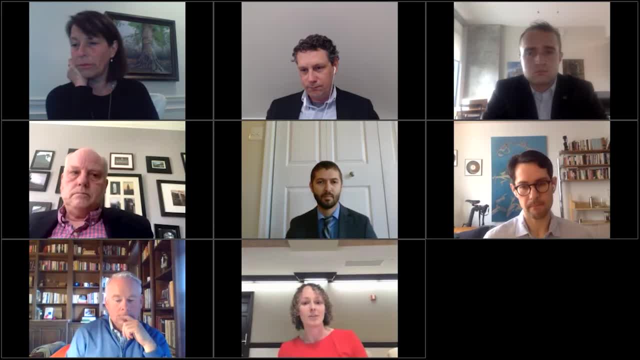 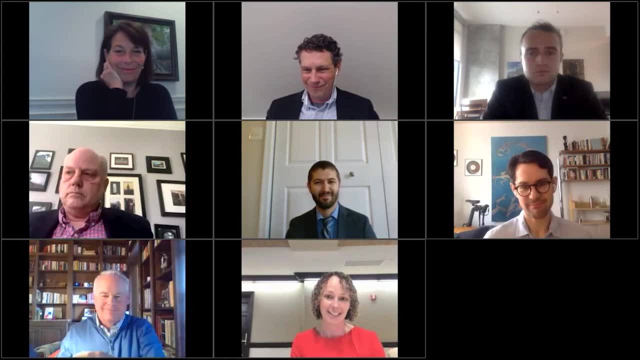 proposed, And I think that raises a number of really fundamental questions. I'm sure I'm not the only person on this phone who has spent most of their week on the phone with panicked clients about this, And there are just a couple of bigger picture things that I really wanted to raise here. 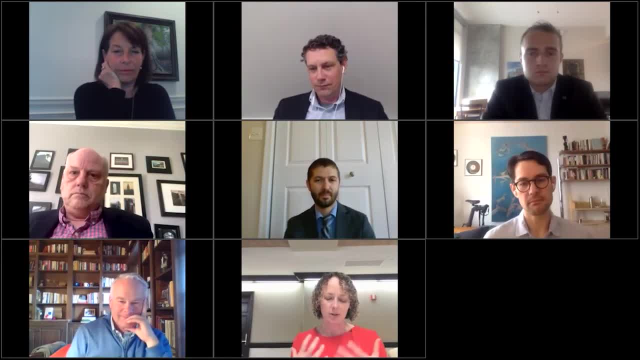 The first is: I was really intrigued by the paper's suggestion that we need another E in ESG. right, I am a climate person by training, going back a very long way, But I think we have been living in an era where climate while an incredibly significant part of the world's climate policy. 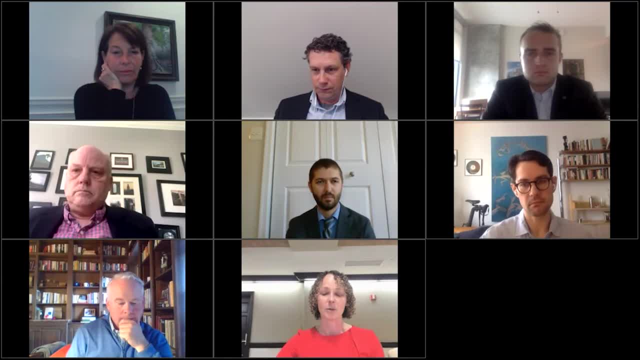 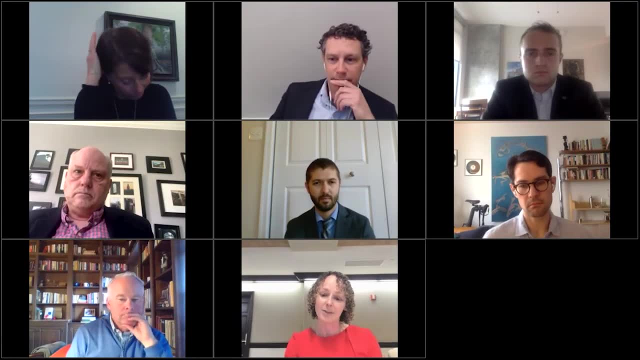 significant societal issue that we need to address has in many ways swallowed the rest of ESG. Right, And you see that even a little bit in this proposal, right, This is a proposal about climate change And then kind of at the back it's like, oh hey, but if you have metrics around water, 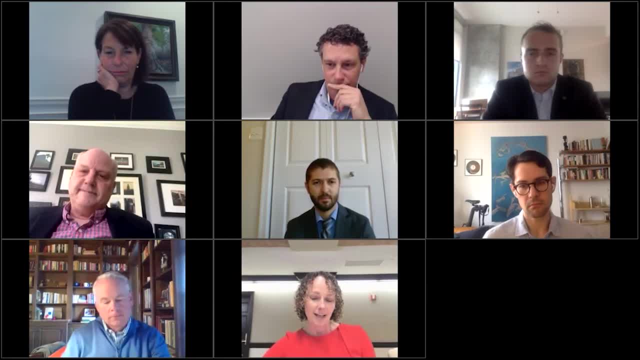 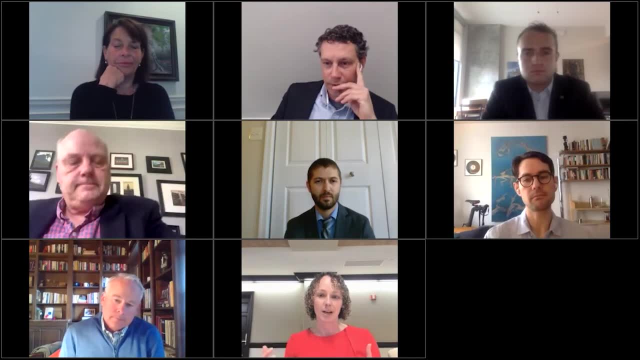 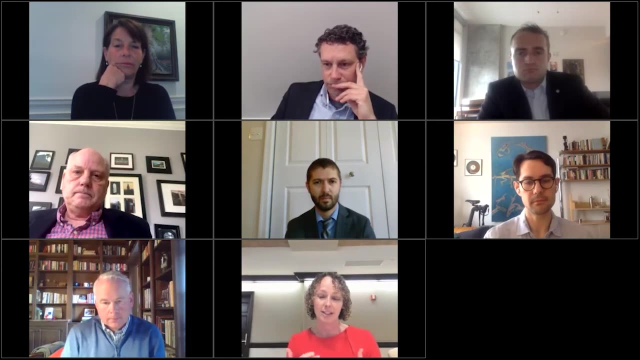 we think maybe those are disclosable here too, And I think that has some important consequences for how we think about governing this suite of risks that have traditionally been financial but emerge into financial significance, And I'd be interested to hear from the authors their thoughts on, essentially, whether a rule like 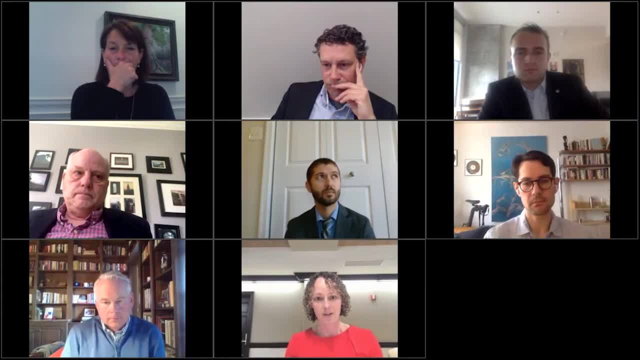 this puts way too much of a thumb on the scale towards one ESG issue that is certainly strategically important for some issuers but is not going to be the most significant one for all of them, And particularly in light of, I think, if you compare this proposal to the way that 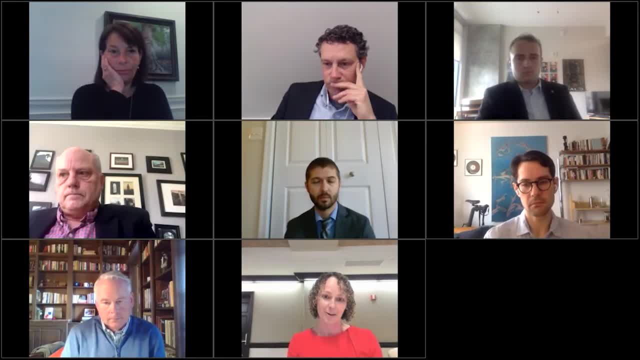 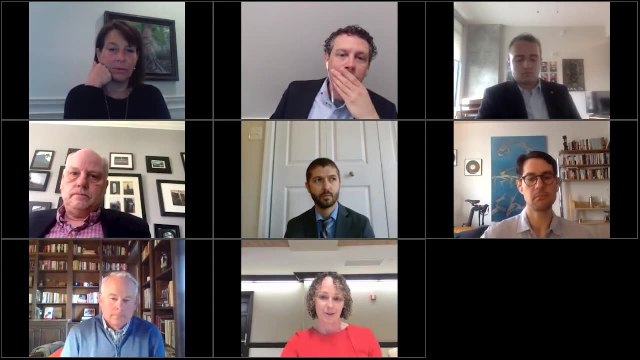 for example, the commission dealt with the human capital management rule last year. right Implicit in how the human capital management rule came out and what this rule looks like is a bit of signaling from the commission that right now they care a lot more about companies investing a lot more in climate. It's not clear to me that that should be the 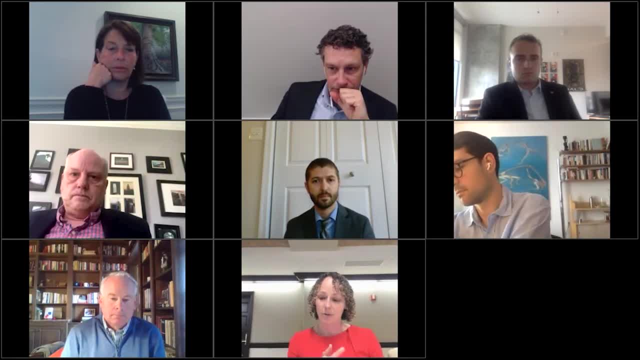 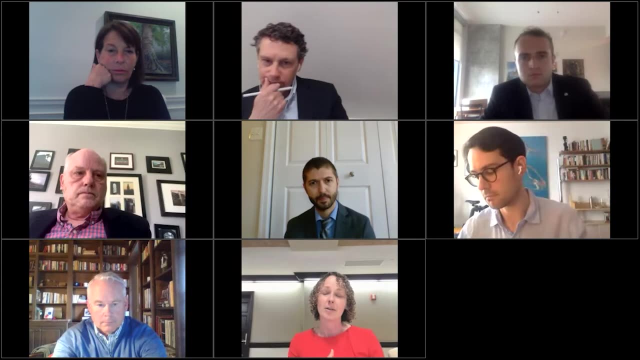 policy preference, that it's the correct policy preference or that it's really the best approach for all companies. The other thing that I think is going to be really interesting here is this question of how do you think about how you organize yourself? We had had a lot of conversations with 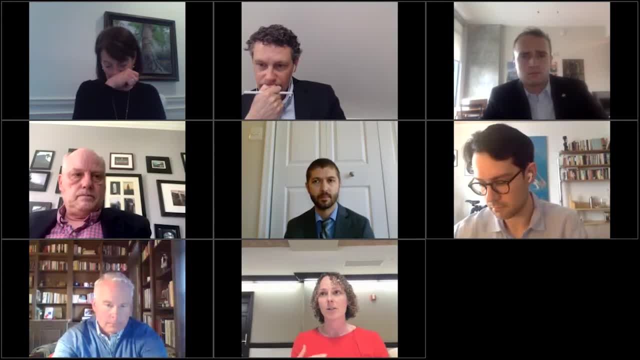 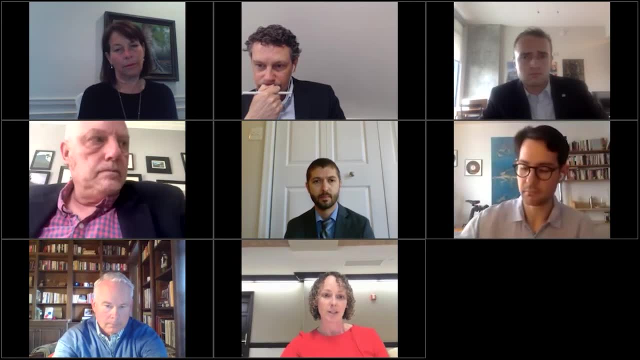 clients, even before this rule came out, thinking about things like: well, gosh, when you go, look at big institutional asset managers are talking about how they think about climate and the things they want to vote on. They're starting to say things like: well, if you get a climate proposal, we want. 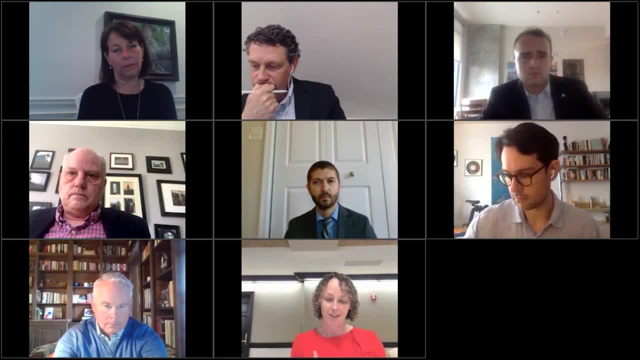 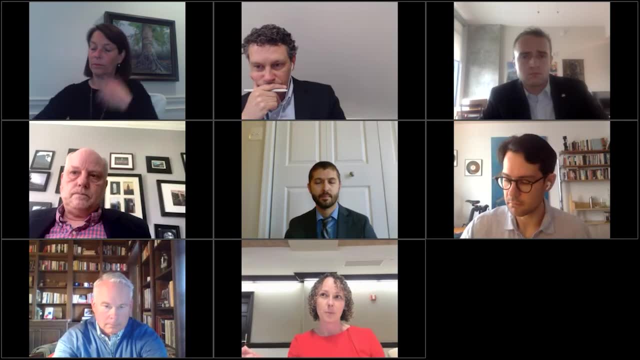 to understand. do you have executive comp that's linked to climate, right? Do you end up looking for very specific policies that, when you looked at them, arguably did belong under existing core committees of the board, right That maybe that's a comp function, And I think that one of the really 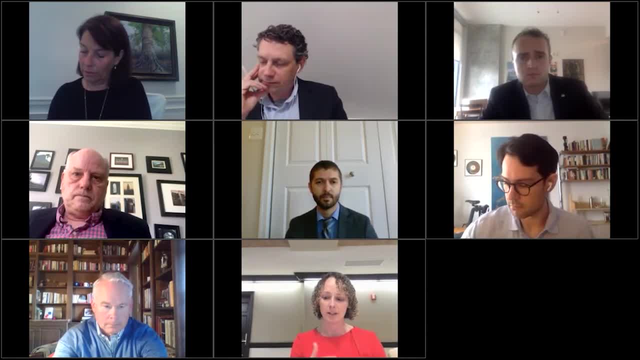 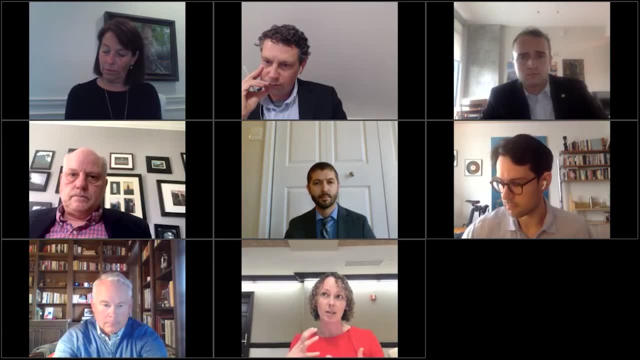 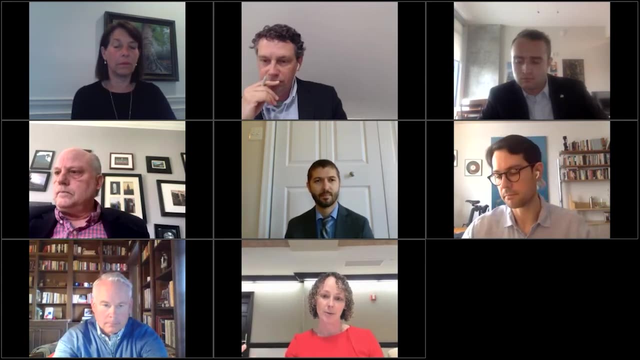 interesting things coming out of this particular rule. all of this is going to go under securities reporting if the rule is finalized as proposed. is this question of: have you suddenly double or triple burdened your audit committee, Because very traditionally much of this work would have come through audit. But as the paper rightly 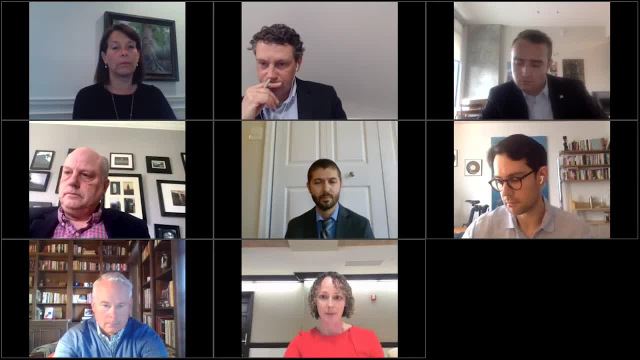 points out, the folks on audit committees are typically financial experts. They're not going to be experts in greenhouse gas accounting, But I think it'll be interesting to see how corporations deal with that. And how are you going to deal with the blowback? 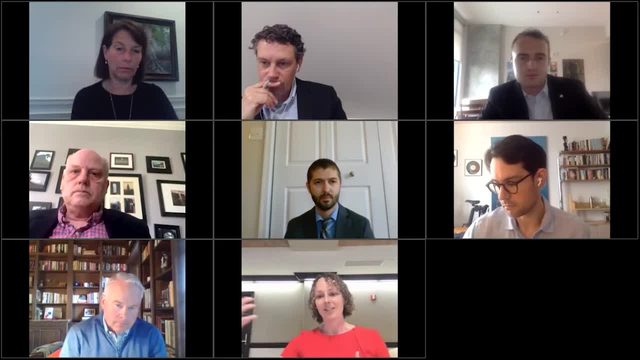 from someone's got to understand that greenhouse gas data, understand how it's been audited and assured, and then bring it back over into. so what does that mean about what notes I need for my financials? And I know I have just two minutes here, So I'll give you all a very specific example- 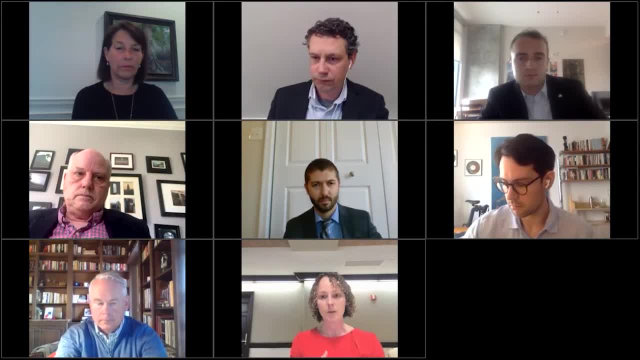 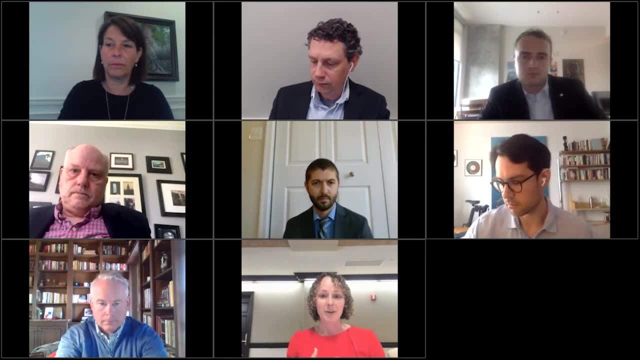 of this where I think it's a challenge. So I work with a lot of companies who have long lived assets And one of the things they need to report in their financials is their asset retirement obligations. And starting about a year and a half ago, because I'm physical climate risk person at heart, I 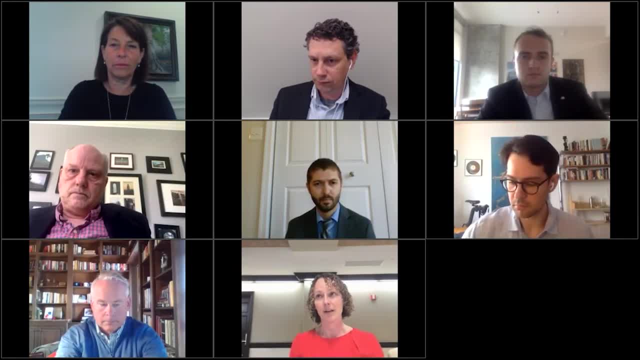 started saying to my clients: Hey, gosh, you know, when you estimate your ARL, do you think about whether the refinery that's in there is going to potentially go underwater due to sea level rise at the end of its life? Because I'm 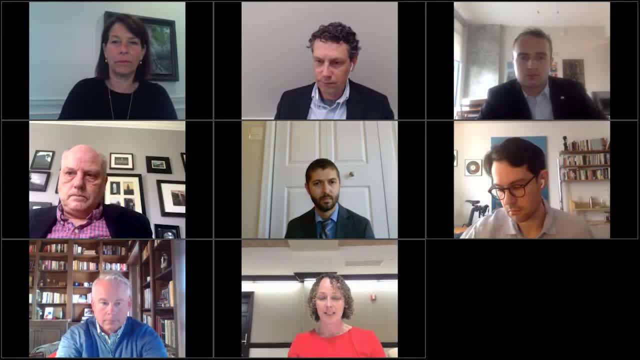 looking at the sea level rise projections for where it is. I'm looking at your useful life projections, And these two things do not match up to me. So have you thought about whether you need a piece in that probabilistic expectation of what it's going to cost a third party to remediate the 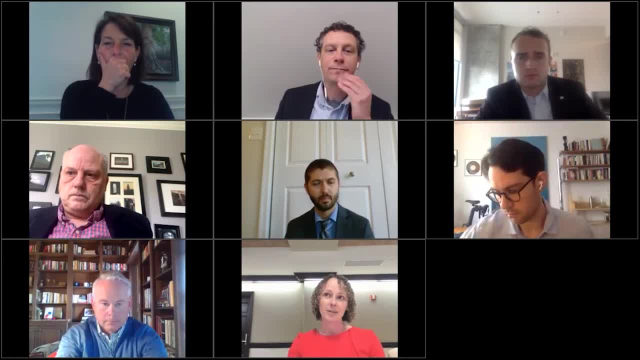 site, which is how you calculate your asset retirement obligation. that basically accounts for the asset retention and the cost of that asset. So if I have to be like you know, I've been thinking about this for months and I'm looking at how I can get my assets to go underwater. 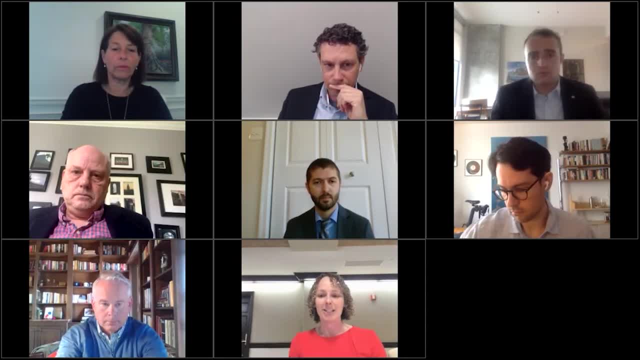 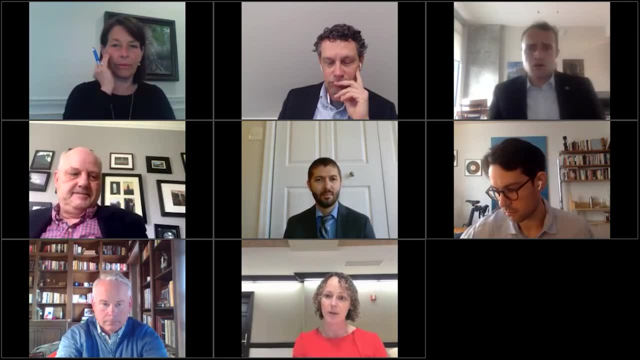 or maybe I can't, just, you know, pave this over and assume that the contaminated soil is never going to get anywhere. And in fact I have to prepare for this piece of land to be completely submerged and deal with the impacts that are coming from that, And none of you will be surprised to know. 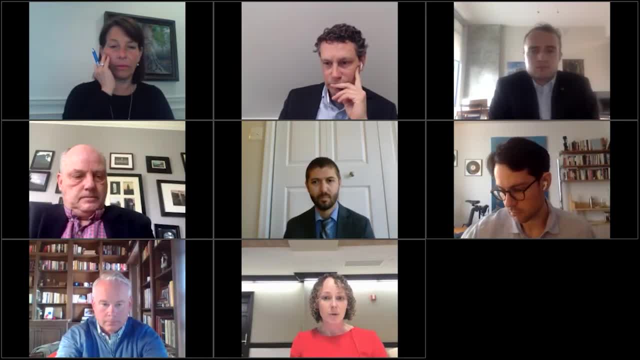 that's the kind of thing that typically has made clients headache, heads explode. Because to really get at that right, what you need is you need accountants who are expert in thinking about those kinds of economic estimation. make a probabilistic judgment of like: do we think this is likely? If so, how likely? How do 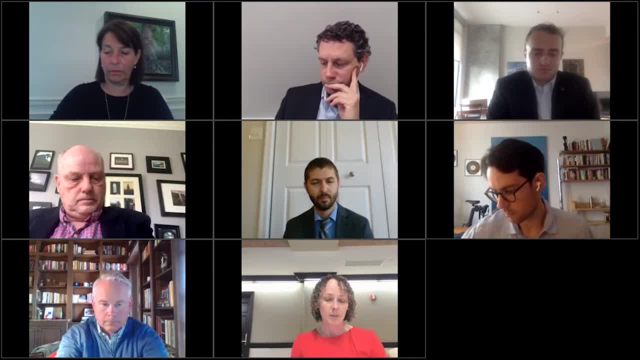 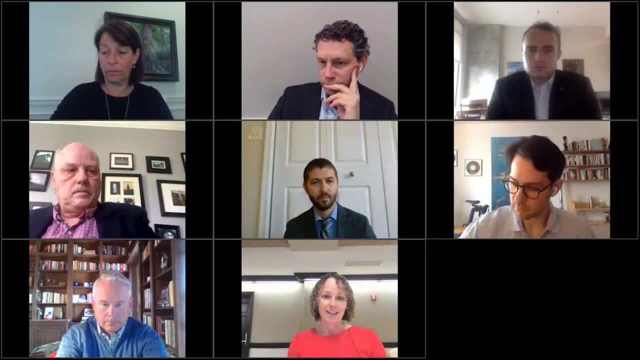 we weight that against the other potential outcomes. And then you need to engage the business people, the client, because for clients with certain types of long-lived assets, those AROs are a very significant part of the financial statements And so you know, I think, where that 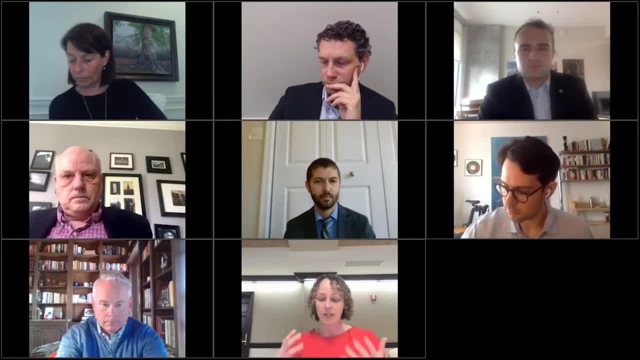 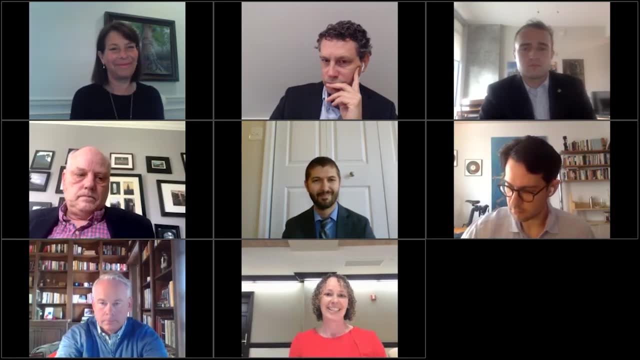 leaves you is that we're kind of in this brave new world where you do need a lot of different types of expertise that may need to be positioned in different ways to make this all work, And I will stop there and hand it back to Linda. Hey, thanks so much for those thoughtful comments and 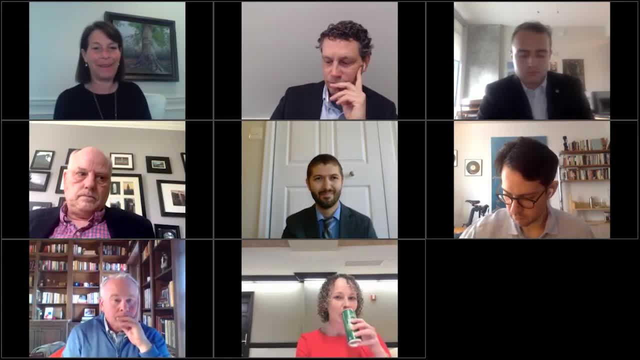 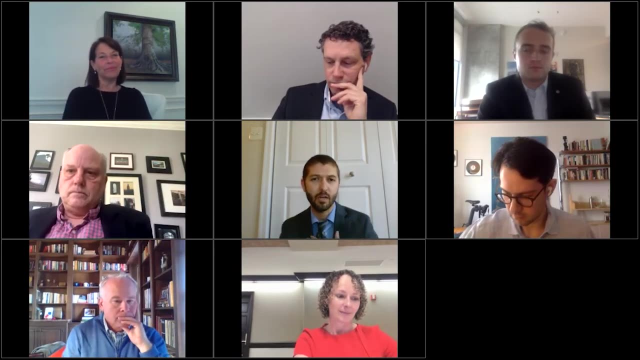 for also commenting on the very recent development, because I know people have been thinking about that quite a bit this week. We are going to go to our final commenter and that is Todd Over to you. Great Thank you, Linda, And thanks everyone. I'm Todd Phillips, Director of Financial Regulation. 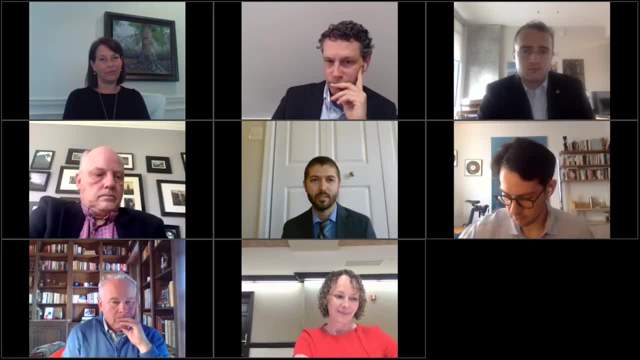 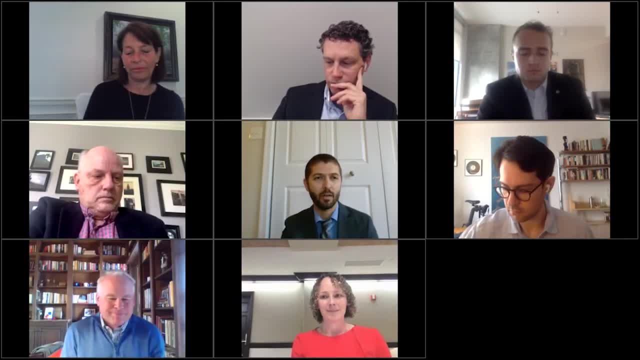 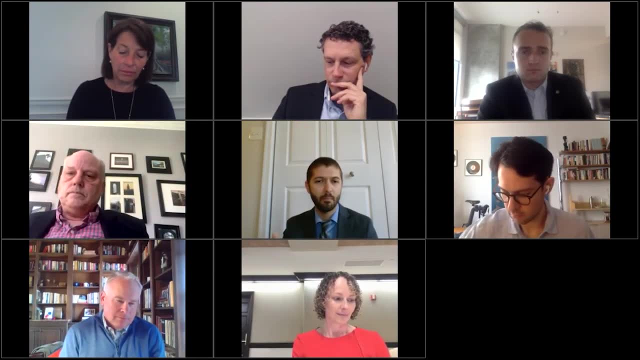 of course I have a lot of thoughts and opinions I express on my own and not of my employer. I had a list of you know things I wanted to say, but Margaret's talk there just made me think that I want to throw something else in The climate rule that the SEC just proposed, You know. 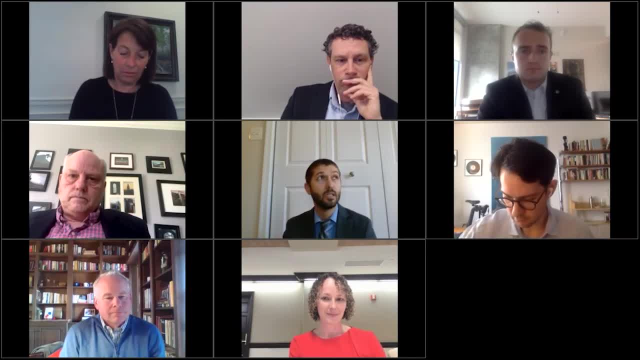 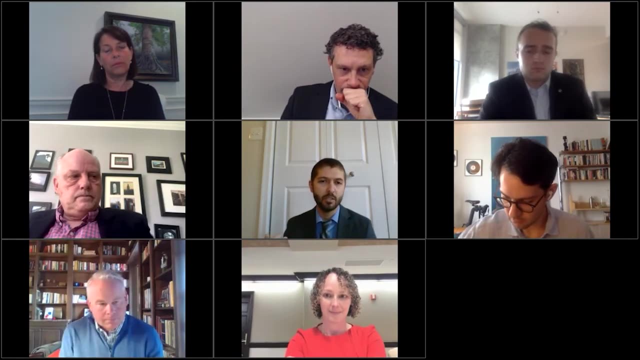 I think that the reason I think the SEC proposed something about climate and not about other parts of EESG is that this is really something that investors have been clamoring for, and not just investors, but also asset managers, people who advise investors. 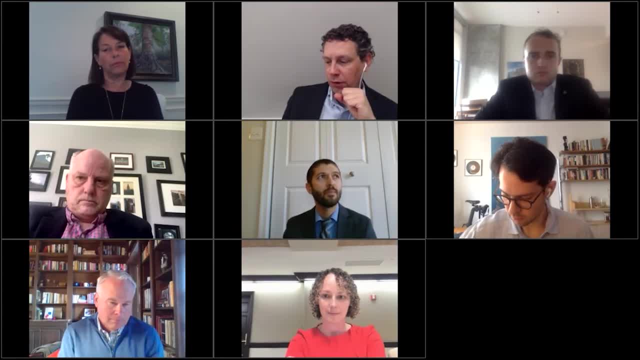 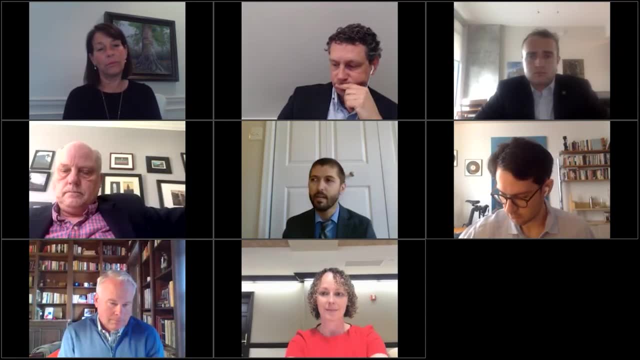 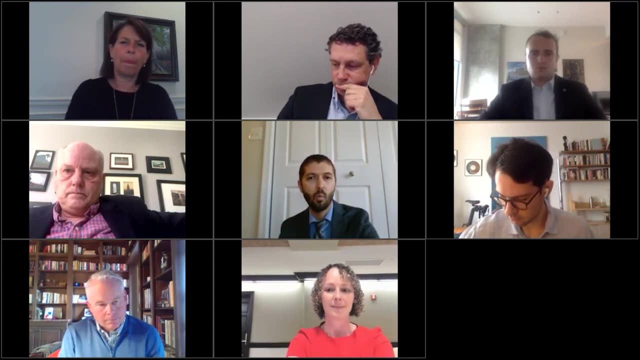 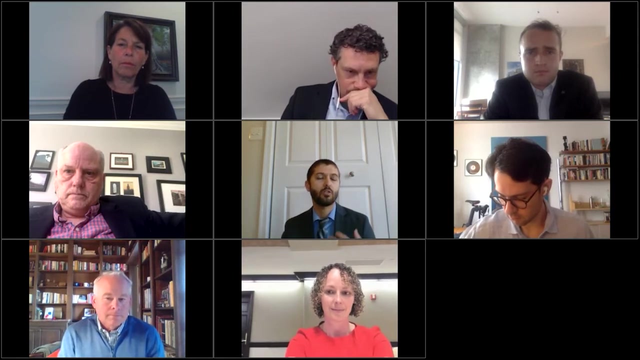 This is just something that they really want, and the SEC is giving it to them, And I think that that leads me to what I did want to talk about with regards to the piece was. I think that, while the piece makes an important contribution to corporate governance literature, bringing it into Caremark. 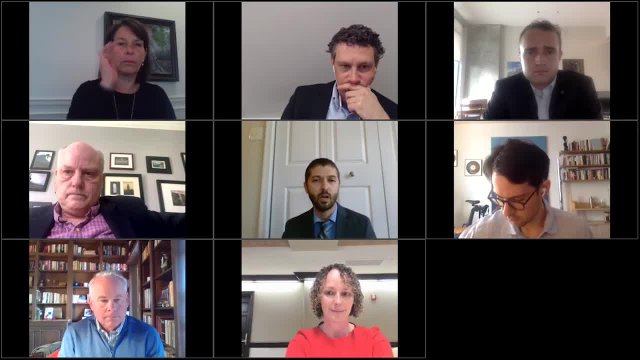 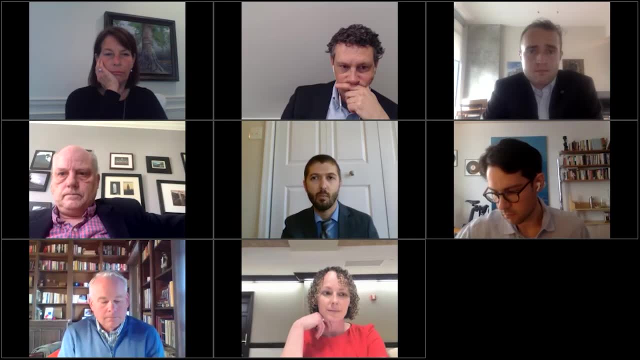 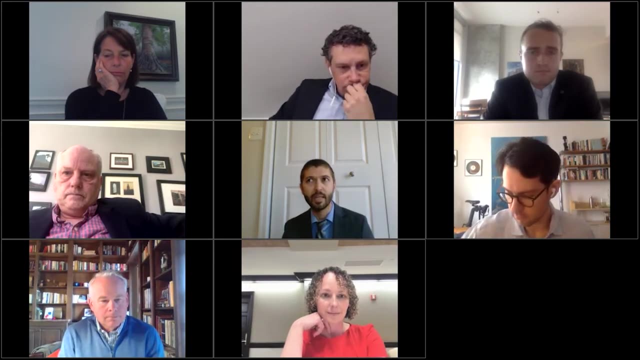 I think the practical takeaway at least I saw was that board directors really need to be involved with their ESG. One thing that it's my sense that ESG and EESG is something that is mostly done at the management level and lower, because it is something that companies think they have to do. 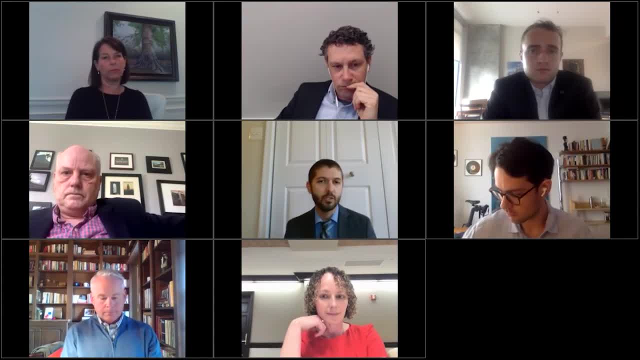 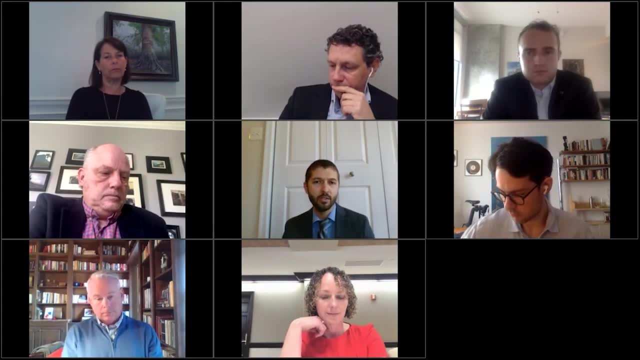 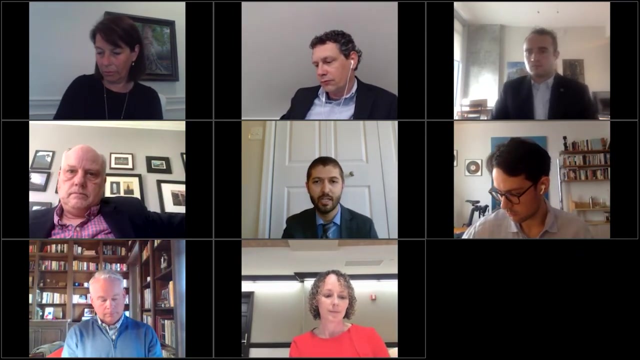 But it's clear that investors are clamoring for this type of information so they can make informed investing decisions, And the directors- who are the directors, Shareholders, representatives on corporations- need to do what the investors want them to do, which is to think about ESG and EESG matters. 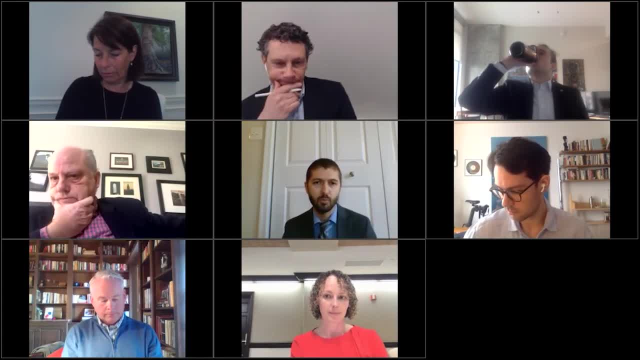 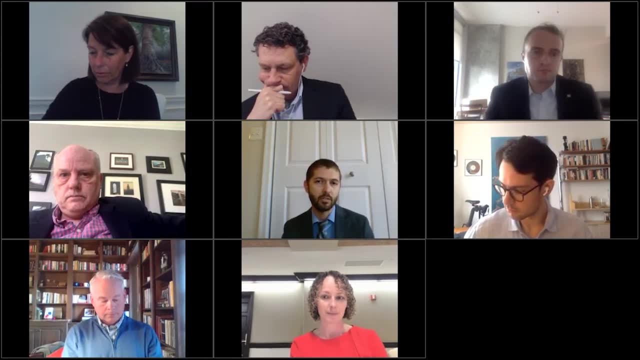 There was a 2019 letter from Business Roundtable and other companies, signed by the CEOs of some of America's largest corporations, saying that they made a fundamental commitment to all of our stakeholders, including customers, employees, suppliers, communities and shareholders. 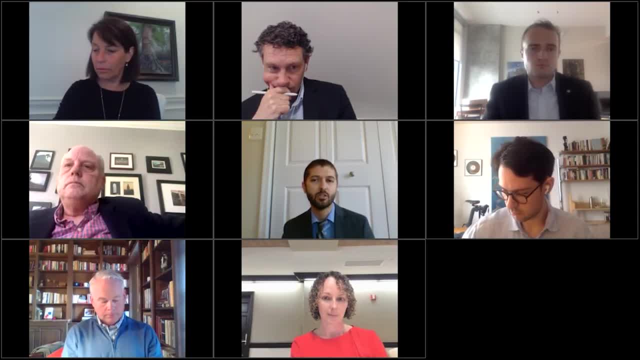 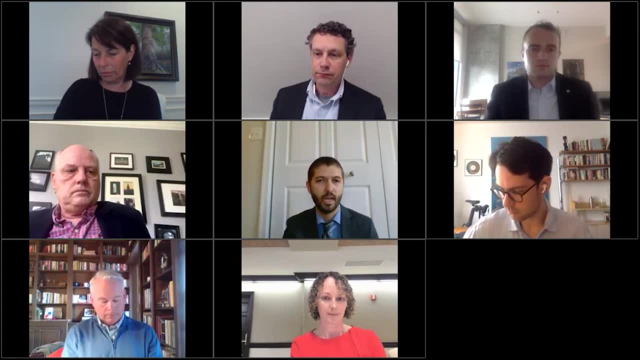 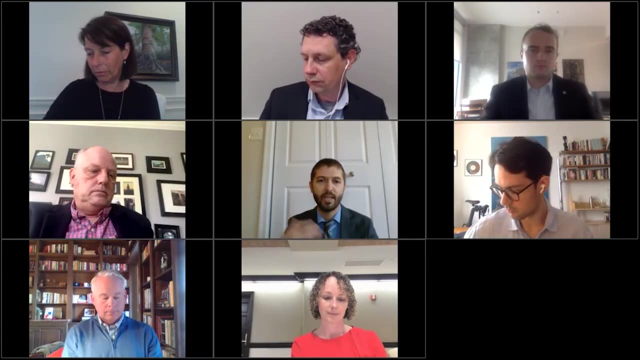 And the most significant criticism here is that it's just reducing CEOs responsibility to shareholders, not increasing their responsibility to workers or society or anyone else, And because shareholders clearly do want this information or do want to invest in companies with this type of activity. 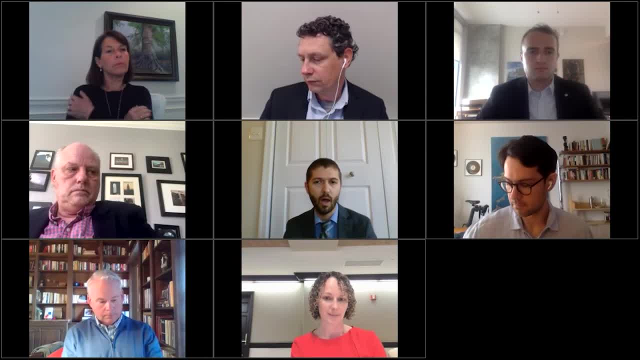 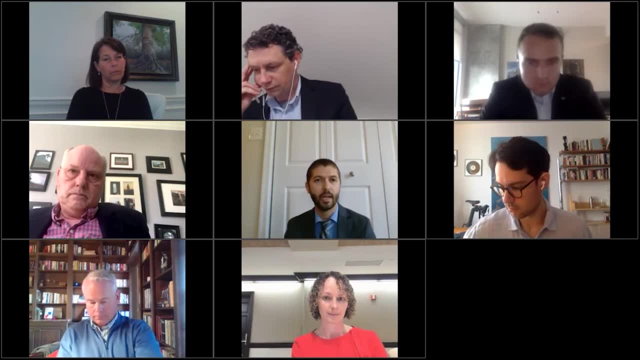 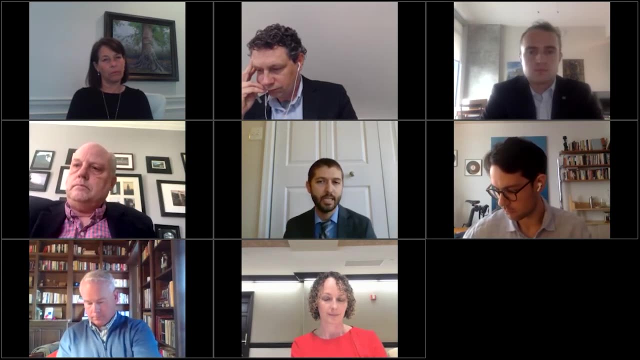 ESG funds total roughly $8 trillion, And that's a significant amount of dollars worldwide. with inflows growing, It's clear that directors need to be taking this into account and playing a role in ensuring that their companies are taking ESG seriously And it's not just sloganeering or greenwashing or something like that. 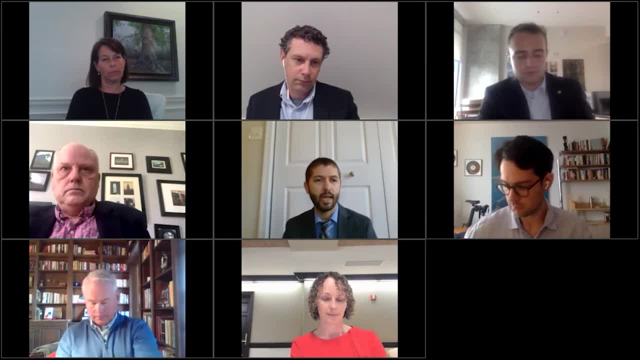 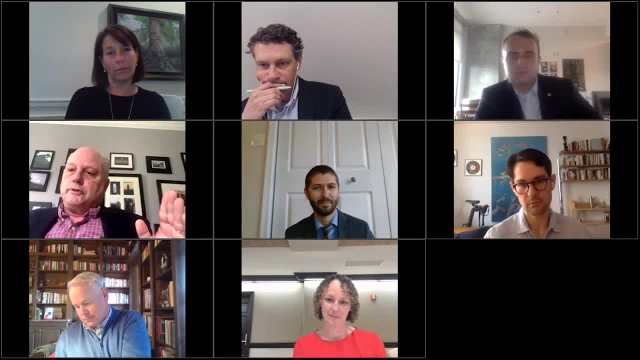 So I think that that is one of the big things that we need to do. So I think that that is one of the big things that we need to do and then you can measure. but we have papers as well on these things and I think, in terms of thinking about the environmental thing, I'd say these: 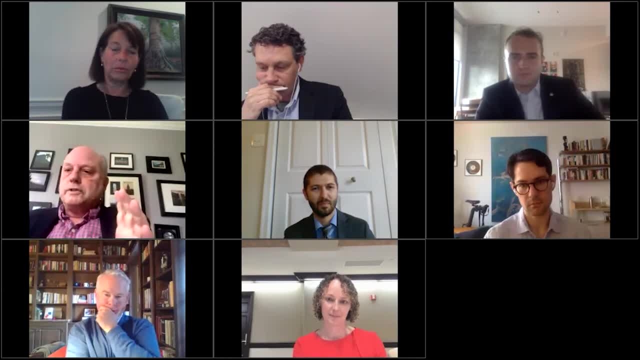 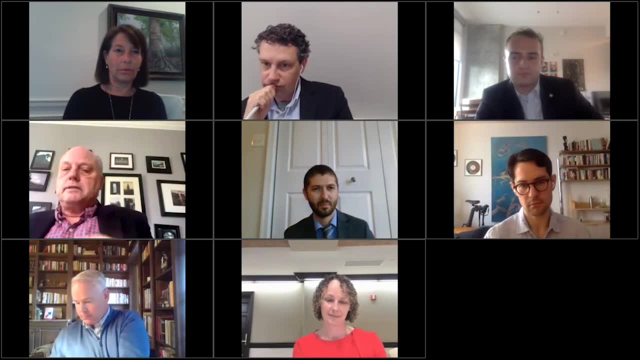 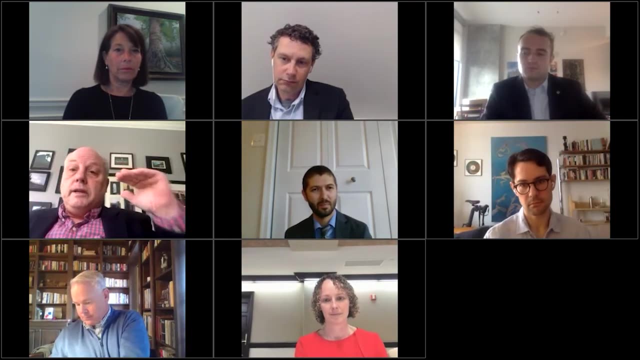 environments. take a look at the paper on on workforce and then apply it to how you're thinking about particular companies and- and we're we're giving right Riley- a way of thinking about this that's focused on this. Jonas, this is the one thing that I think we would like to see heterodox not be about. we need our 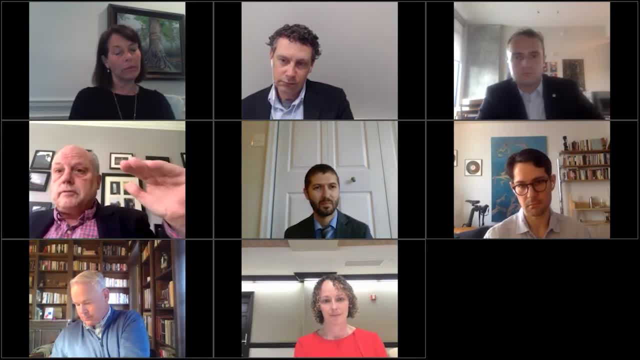 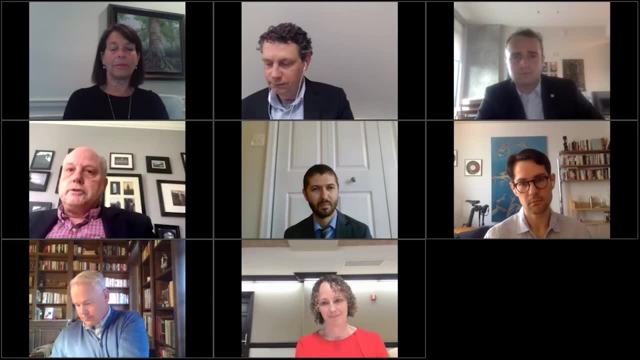 market economy companies. to make money the right way, they do have to be profitable, but the right way is making money net of externalities. if you don't externalize your harm to your workers or consumers or your environment and to the communities in which you do business, that is what is going to maximize the 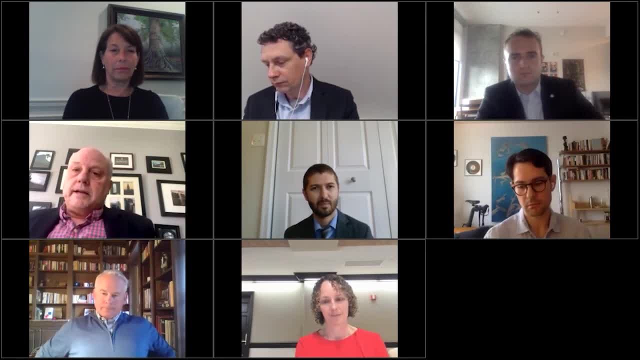 productivity and quality in the American economy. it's going to maximize the economic and well-being of all investors, because our portfolio includes the taxes we pay and that also includes things like shifting. frankly, the more risky you make companies and you just shift value, you make money. that way, we're not going to be able to get any more money to. 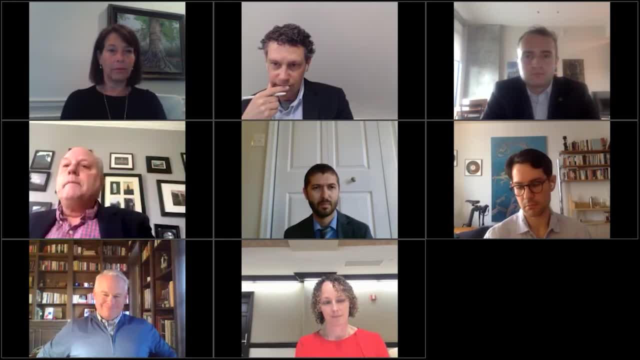 equity holders away from debt holders. well, guess what most investors have to are prudently invested in debt securities. most, except for the top percent, most of us- we get to save for retirement and invest is attributable to our job. so thinking about that and organizing our corporate governance, 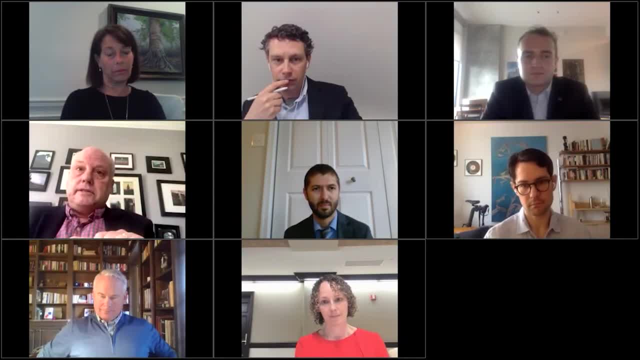 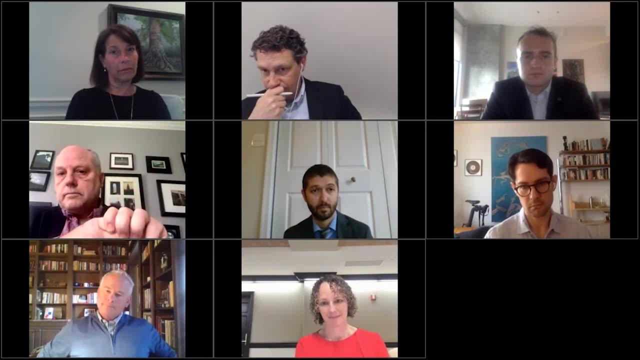 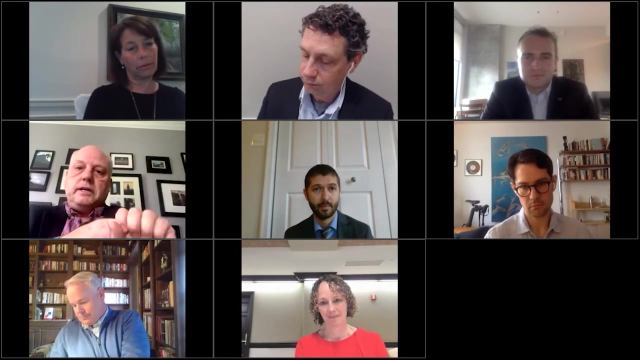 system right. Riley, about making money the right way is important, but this is complex. and to the SEC proposal, just give you a couple quick concerns. I'm very divide. It will not improve the climate to take high cash flow producing businesses and simply force them to go private and to avoid the hoo-ha. That will not help anything. The SEC has. 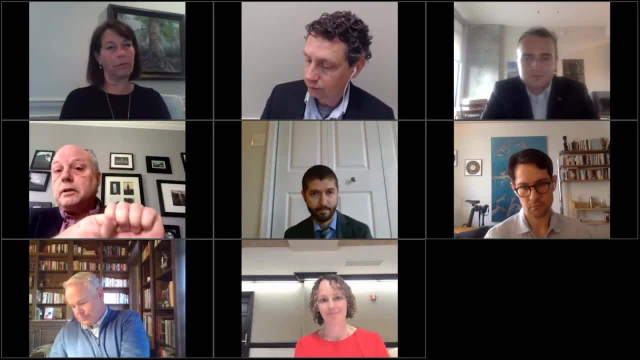 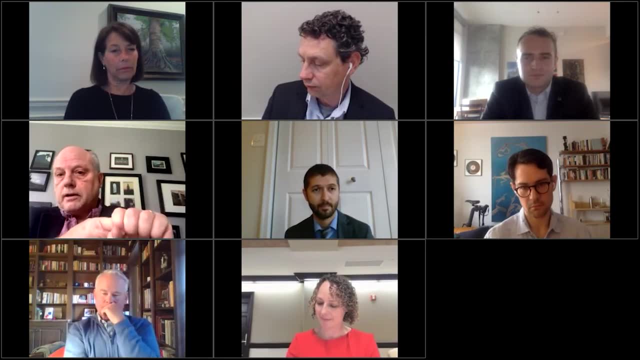 facilitated through exemptions, the growth of huge private companies, and there ought to be a level playing field, And I am pushing Congress to do this and I propose that a billion or more in revenues, whether you're public or private, you actually have to file the same double ESG things. 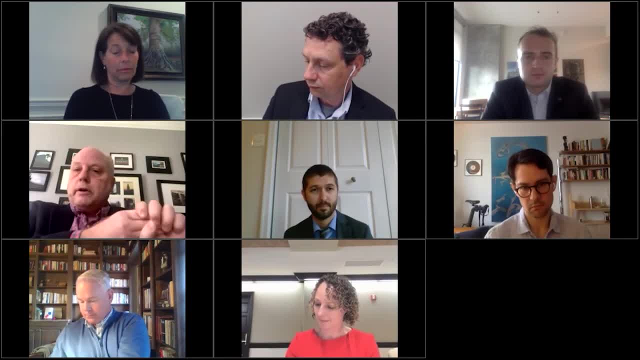 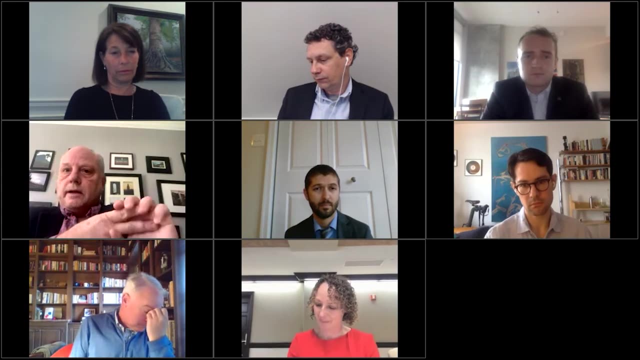 They could do a form double ESG. The point about companies focusing on what's most salient applies to this rule. I think it would be a lot better to be honest if we picked 35% of the industries that were high salience and phased it in by industry. I think it is really silly to have 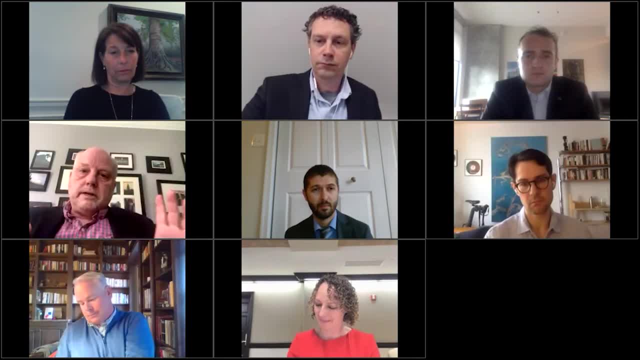 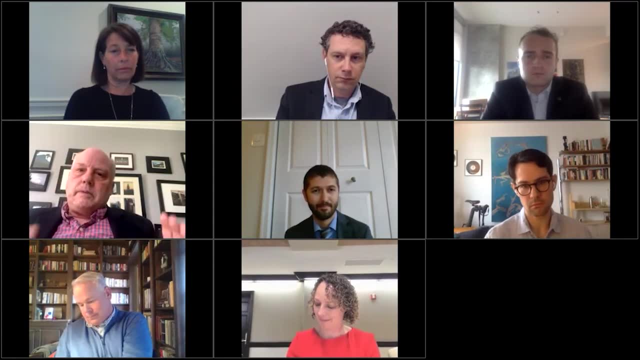 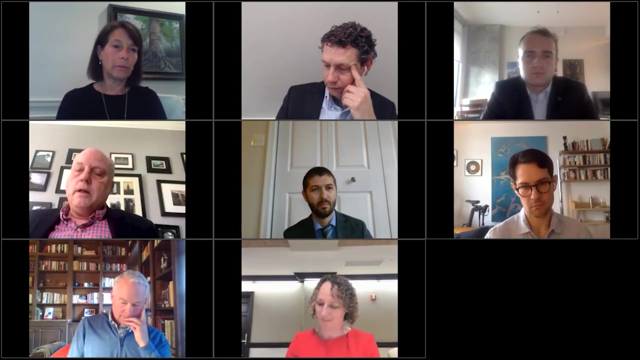 scope three. The so-called break on scope three is by size of issuer, not by industry. You know, by covering 30% of the industries well in climate and focusing on education and implementation and not enforcement in the first wave, you can probably have 90% of the impact that you want By taking- I'll pick a- 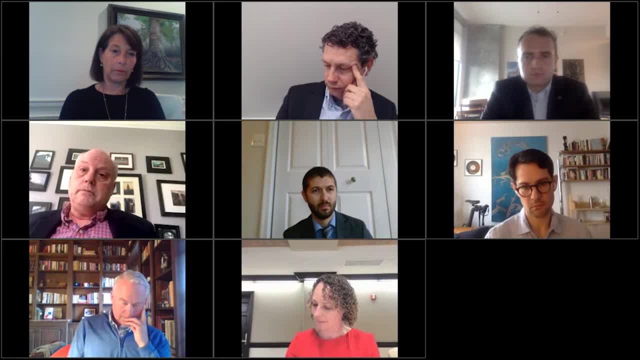 company that I think has pretty good double ESG values, at least I perceive it- to Two companies. JP Morgan, really good employer in our state, Pays people well Involved in charities Salesforce. We really want them worried about scope three. 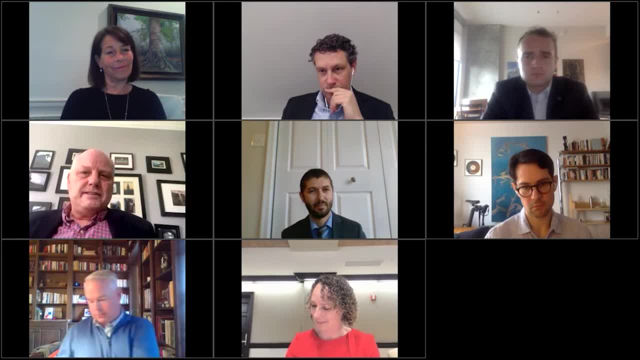 emissions. I'm not saying they don't have double ESG concerns, but is that really where we want to focus it? And are we going to make this a private right of action where plaintiffs, lawyers, can play games with this? Because when you do choose, and this is when the SEC chooses to focus- 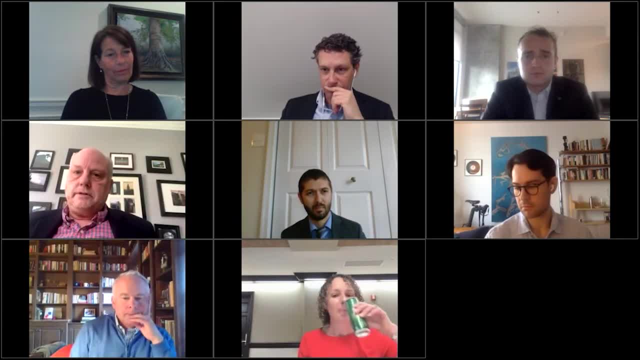 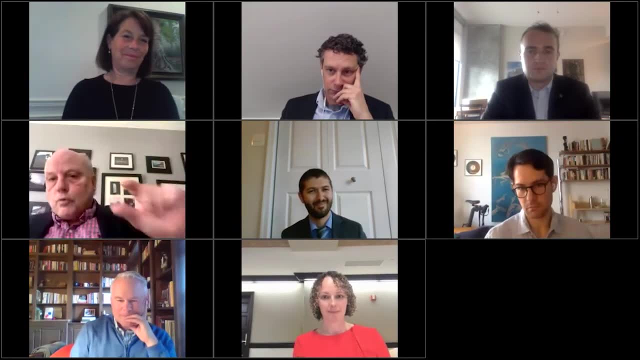 on something having to be disclosed. it does subordinate other things And they are choosing, and I'm a Democrat and Joe Biden's a hero of mine. The workforce should go forward with climate, not in isolation, And I could come up with sensible metrics around workforce. 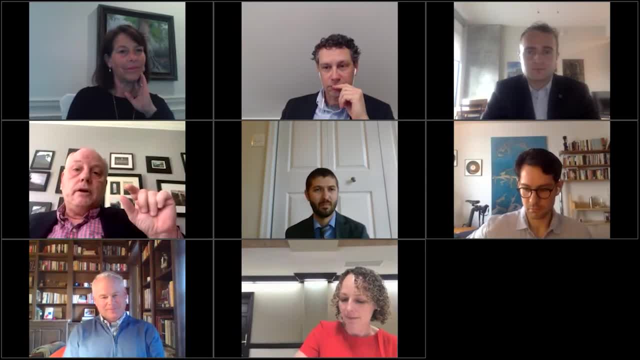 very easily. that could be implemented by business much more immediately and with less controversy. And the other thing we better admit is: sometimes you need the legitimacy of congressional action And the double materiality question is being grappled with in other parts of the world. And 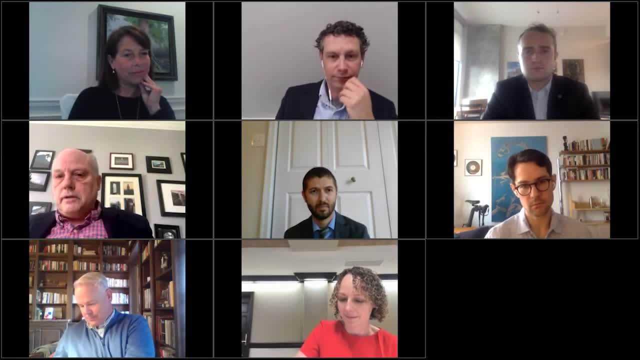 the reality is we're going to have to do something about it. And the reality is we're going to have to do something about it. And the reality is we're going to have to do something about it. And the reason we're talking about climate is not just because of equity investors. And, if we allow it, 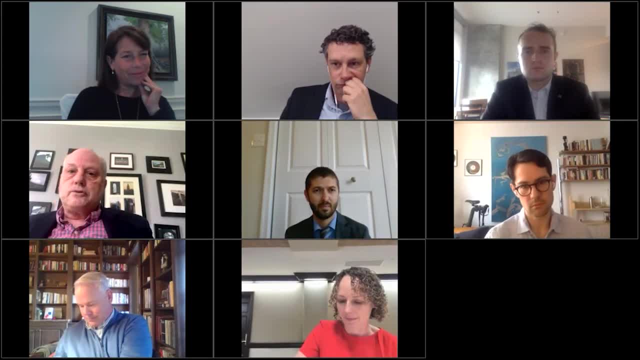 to be driven just by them. it'll be a perversion of public policy, And that's true for other environmental and workforce issues. And so I'm a fan of Orwell Orwellian. Orwell was not. Orwell was a straightforward, candid person, And I think what we're saying is: there has to be a real look. 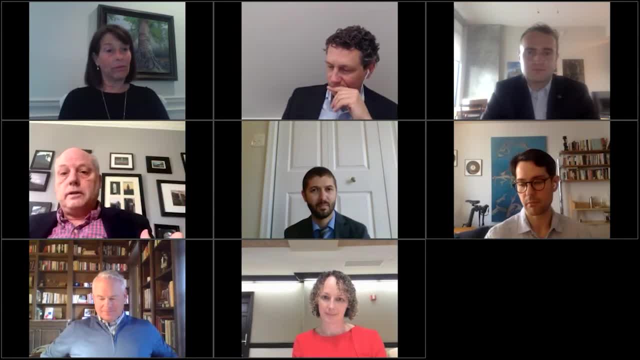 at what companies can actually do and what's the viable way of doing it, And we're a long way from that. But this power, I think we're trying to give you a real look at what companies can actually do, And we're trying to give you a real look at what companies can actually do, And I think that's. 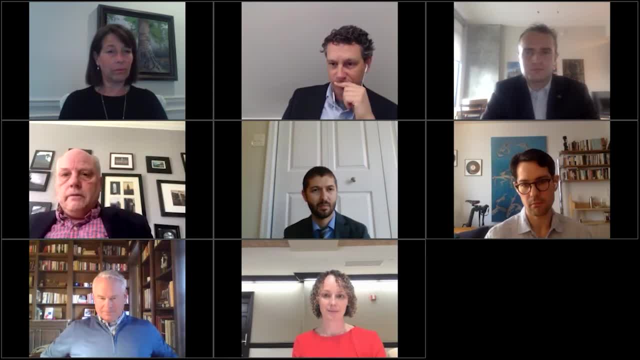 a way of thinking in a business-like way that would help these companies more effectively get to where we want along. But I think there also has to be constructive feedback from the environmental community to the SEC that if you don't make this practical for companies, 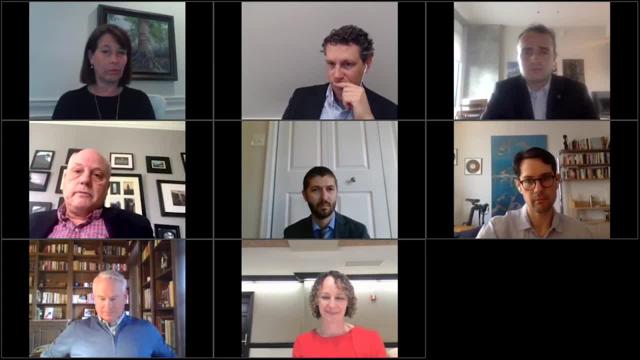 if you make companies do stupid things when they actually have other risks that are more important and you don't focus on the sectors that are key. first help them. focus on help them, not beating them up. Nobody knows exactly how to do scope. 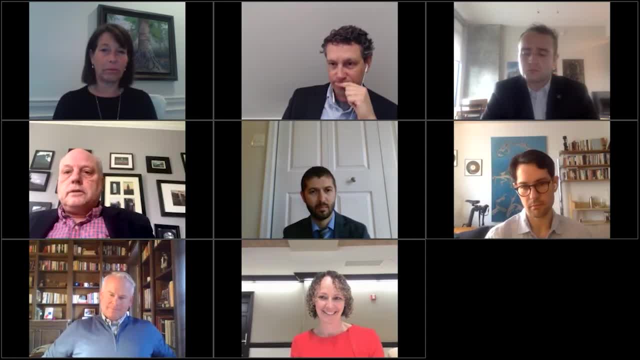 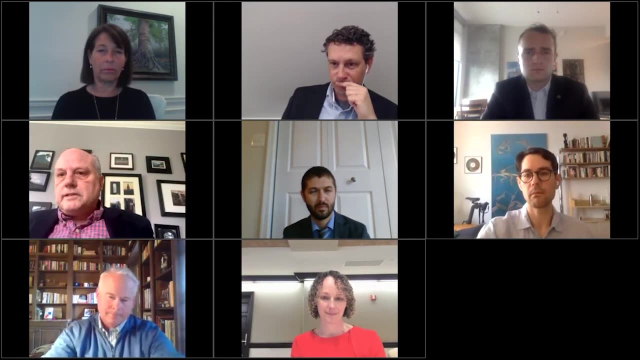 three, even as to the most salient. so what are you supposed to do if you're a bank, when companies are the sum total, environmentally, of just having their individual employees all together at work and, frankly, that calls out for carbon pricing other government action as being more of the? 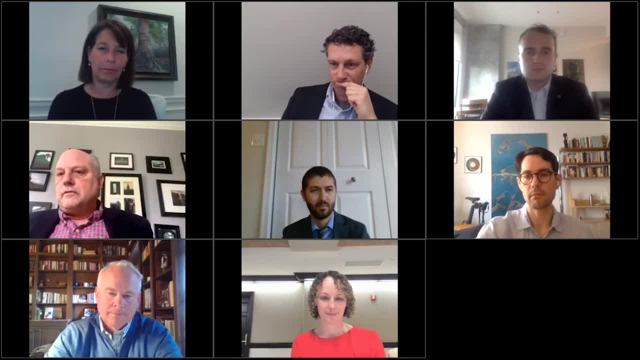 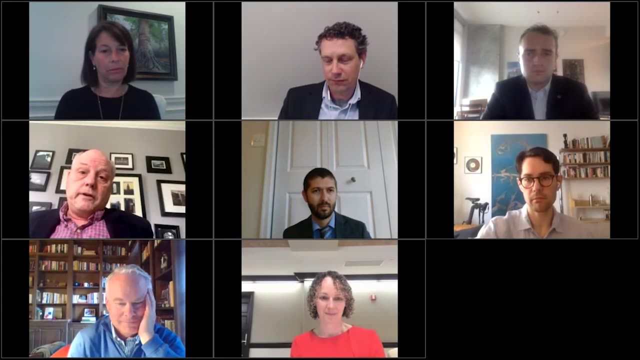 focus. so i worry, jonas, you know, to be honest, that by for investors, by being very diffuse- you're actually for values driven investors like you. you're not going to get as far as if you encourage the sec to actually focus on where it matters and and not to forget that for other 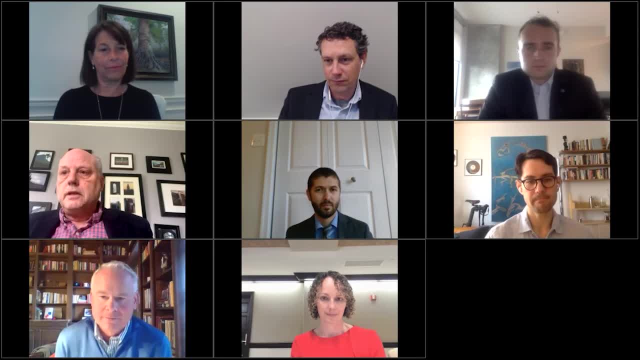 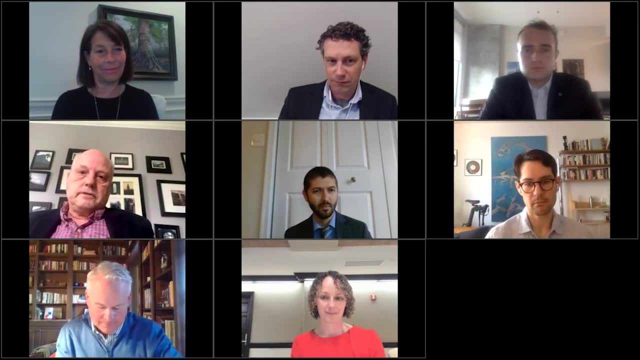 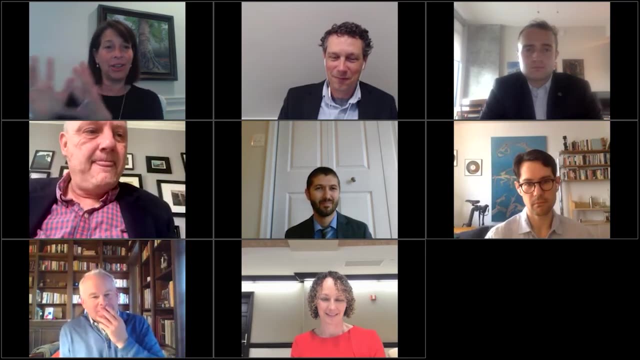 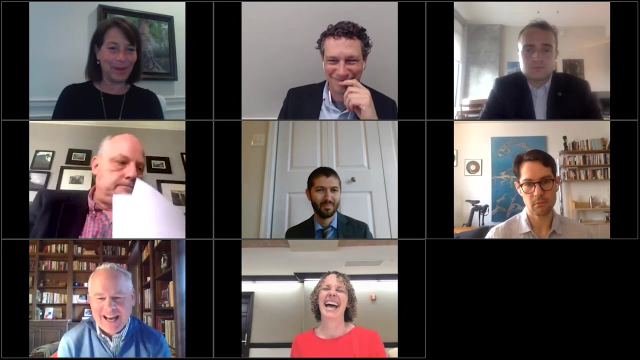 companies, there are equally compelling social considerations that they should be addressing and that if you force them down this path, it may not be the best allocation of social resources. so i think one more fascinating, and i i want to get to student question audience question, but i have a feeling my co-host, mike vandenberg, is aching to make a comment, so we'll. 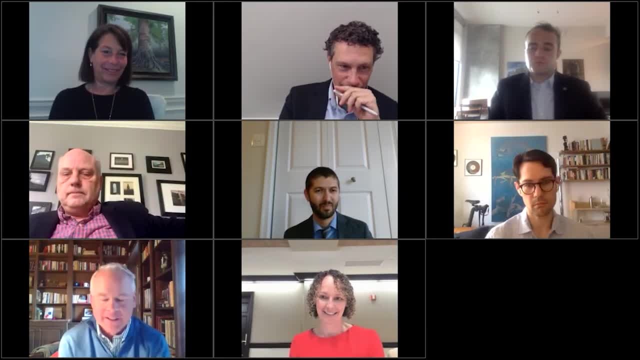 i was on. uh, i love this paper. i pushed for it internally, i was with you all until that last uh soliloquy from uh, from the chief, as riley says. and there, there we. there, we depart, and i understand where you're coming from, but i really do think a couple of things. number one, if anybody, on this: 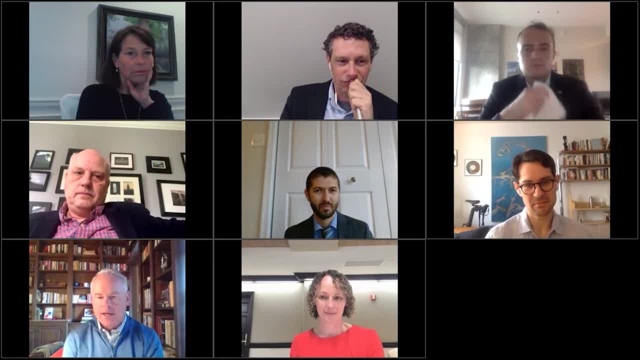 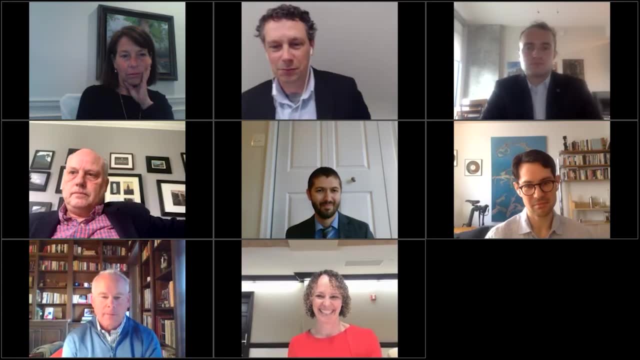 call, or anyone you know thinks that climate change isn't a dominant issue, even for companies that are selling ice cream. please contact me and let me set you up with the physicist who's the co-author on my book, which is called beyond politics: because climate change is going to affect us for 500. 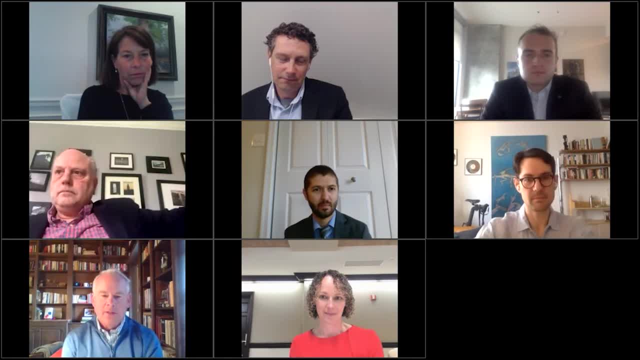 generations and, and so if you care about your employees, the number one thing you can do is avoid catastrophic climate change. number one if you care about environmental justice, if you're on the left, number one thing you can do to help the most disadvantaged people today is to avoid the 500. 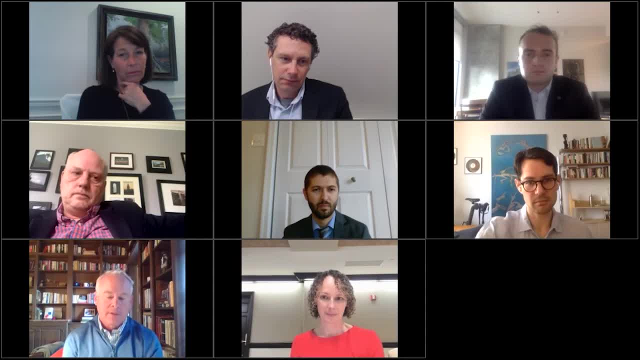 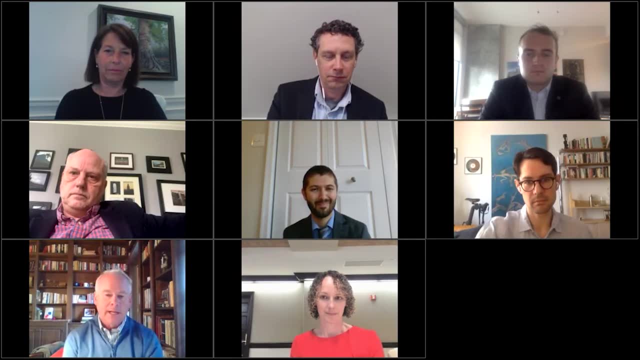 generations of their offspring from being suffering from catastrophic climate change. if you have any doubt about that, please contact me. we'll set up a workshop. what we do typically in my classes at vanderbilt is we bring out all the best skeptics ideas and all the students go get them. we put them up on the board and we have as long a discussion as we need. 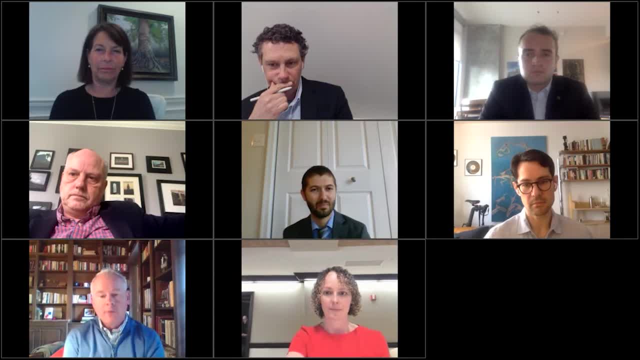 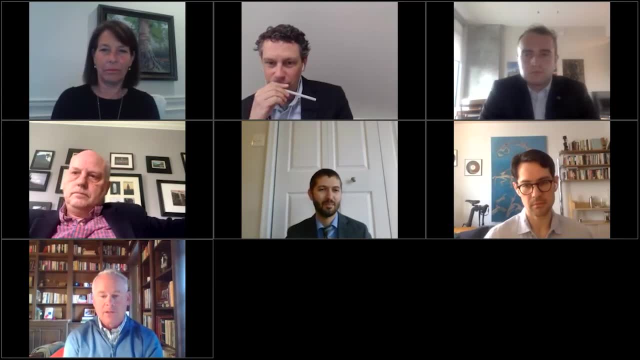 with the physicist to walk through what's happening. so i'm with you completely on a lot of the pragmatic parts of this. i- i was a partner, lakeland lockins- i represented investment banks. i've done hundreds of disclosures so i'm not a- you know, sort of a, a green advocate, but i- i think we are in a 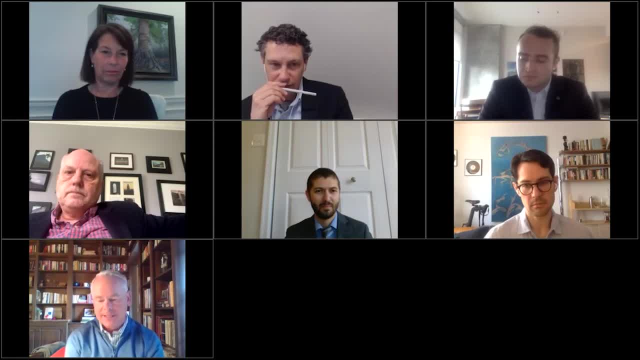 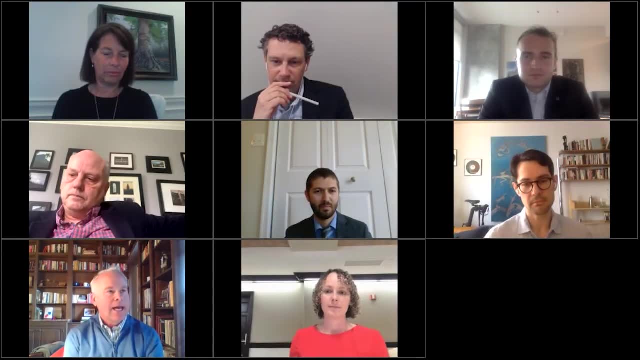 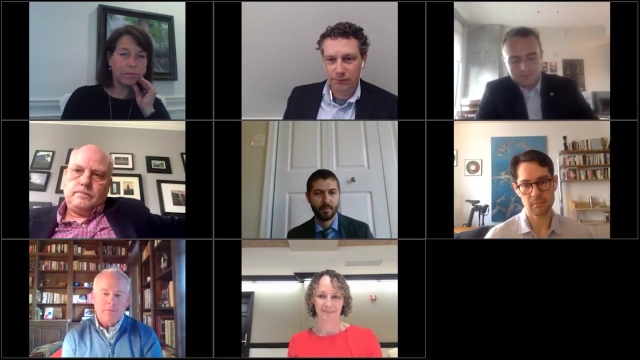 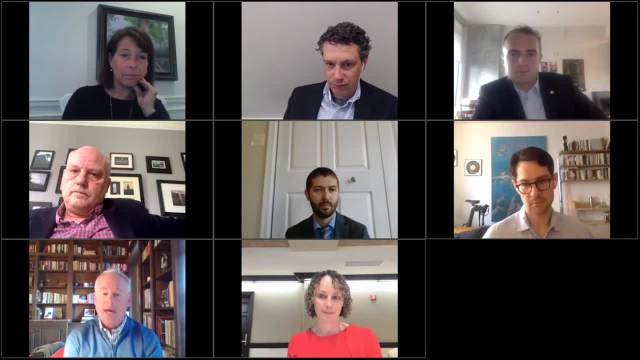 chief of staff from 1993 to 1995. have we gotten the carbon tax? no, uh. have we had a major pollution control statute in the last 30 years? no, we have not. so sitting around waiting for a perfect solution, i think, is a mistake for companies, which makes me wonder whether we should engage a little. 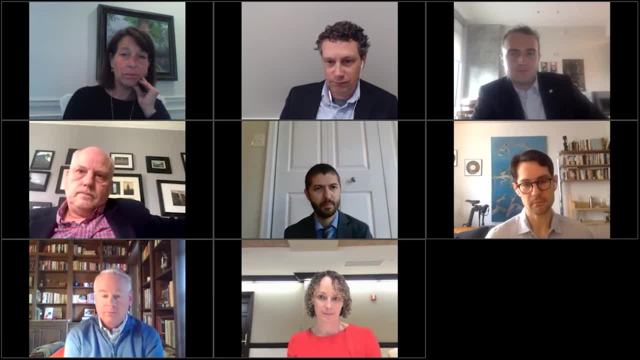 bit as a group with the notion of common owner or universal ownership. i'd be really interested in the reactions of everybody on the call to john coffee's written about this, madison condon and others. what do you think about that is? is that, is that adult? i wasn't smart enough to write. 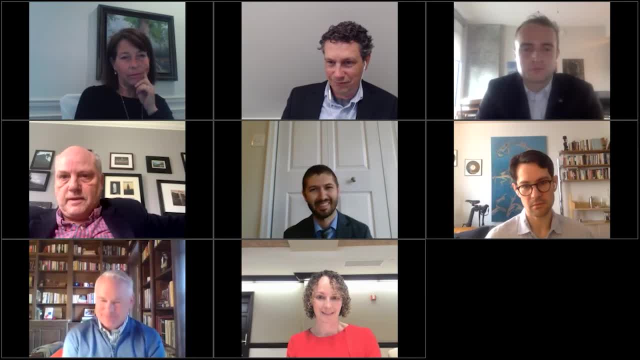 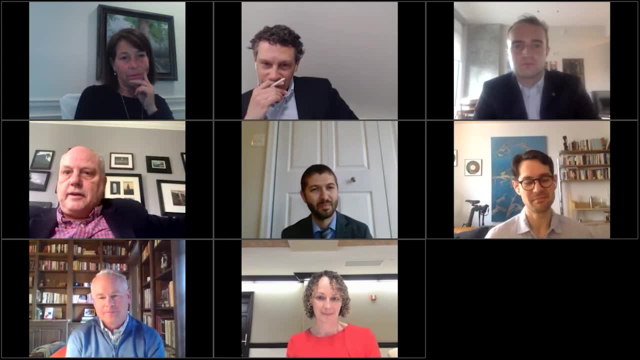 about it as a universal owner. i've been writing about it the entire century. i mean i love it. i really do, which is one reason i mean is when i say: focusing on growth, net of externalities. right, that's what you're saying. exactly what i mean. 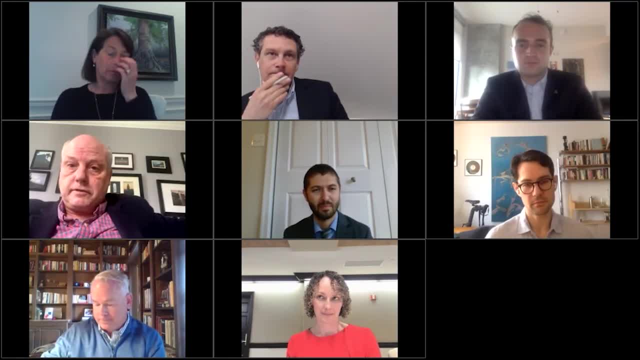 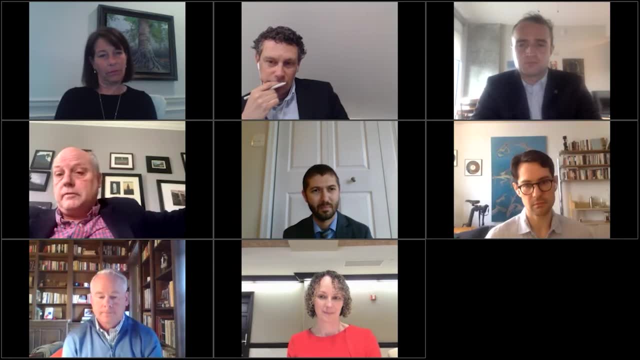 and my only point: i i believe unscientifically that billions of people spewing carbon and methane into the, into the air over 100 years, i believe unscientifically that that is likely to have a huge impact and has had a huge impact on our climate. so i don't underestimate the change. 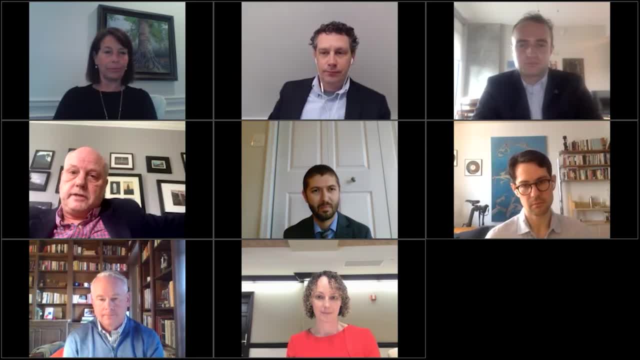 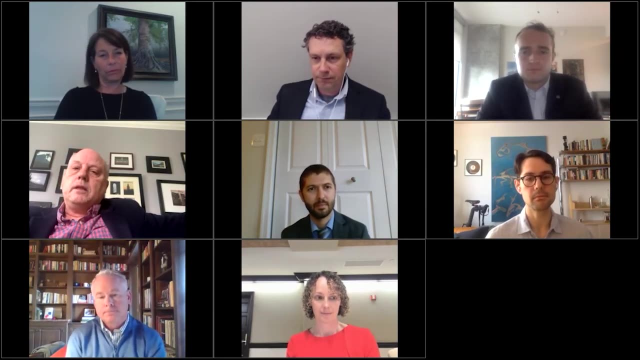 i want to address it. what i'm saying, michael, is in terms of phasing it. sometimes, the more that there are companies and industries where you can uniquely focus on them have the most impact. it may make sense to start there. the more companies look like, frankly, the sum total of us as individuals just at work. it may be that we want to not burden. 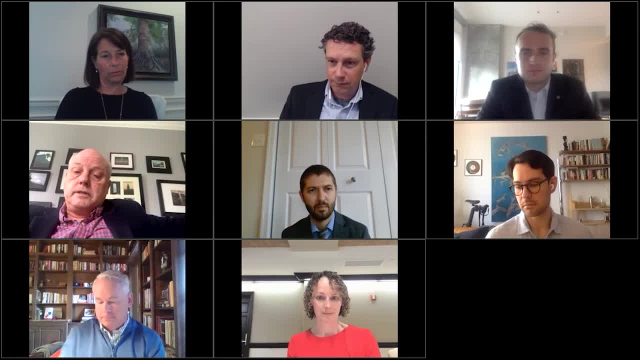 everybody but do something well. i believe in big government honestly, but smart big government and diffuse poorly thought out public policy. that will get challenged, if we do it that way, by members of the business community because, as you know, michael, part of why we got none of these. 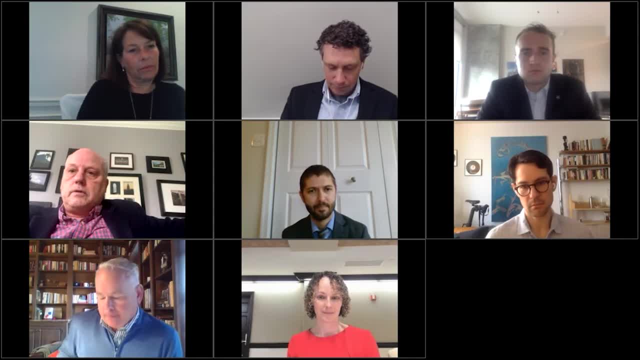 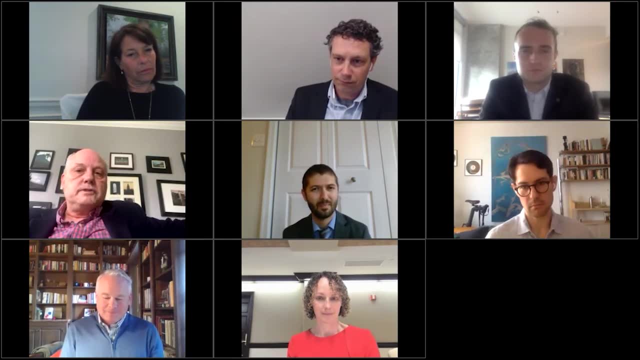 investments that we make money禁尽 as stock market of materials. some the stocks. just陳 cheers us out. never thought we'd be making as little as we did last year. that's where we have a huge impact on our economy, so i'm hoping to. הא� sounds like you understand. well, i don't. 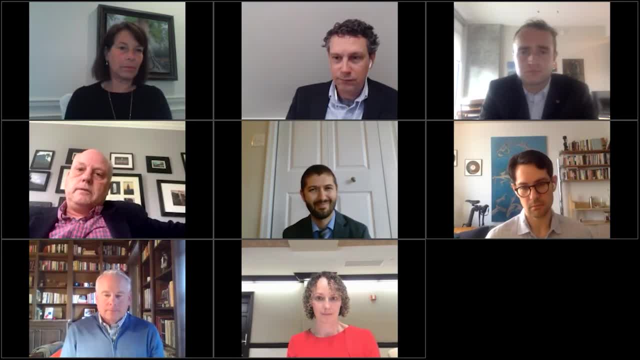 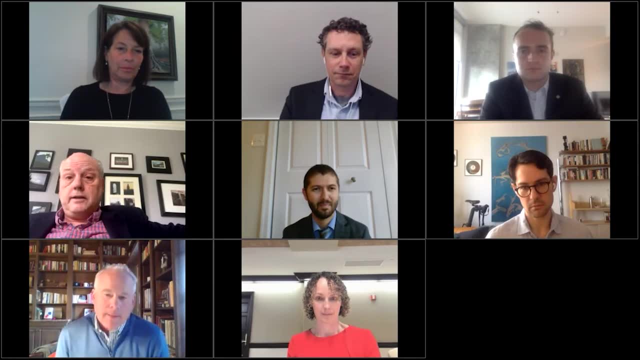 care of how big a big thing it is- $100 billion- right, i'm just like, okay, let me get this right, i'm gonna go III do the same thing: $100 million to save gas costs. i've got to deep think. i'm really going to have how to do that. so, michael, so it couldn't be too long today. i think digital innovation and digital economy have helped. so I think for that iki, carbon action, the 19th century job was impact office in Valve. 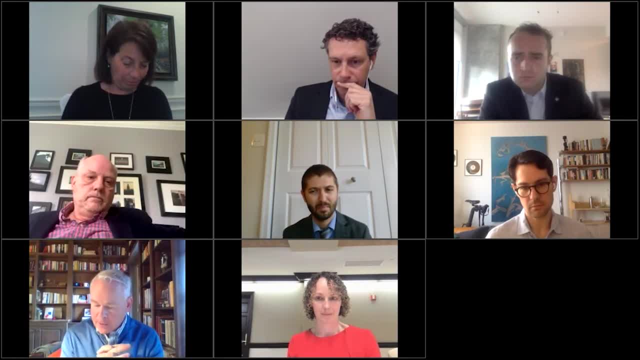 So I think we're very closely aligned on that. But I filed some comments with the SEC. I have a paper coming out any day now which suggests that when I look at the way the SEC conceptualizes what the risks of climate change are- and we tend to talk about risk, but opportunities are things investors care about too- 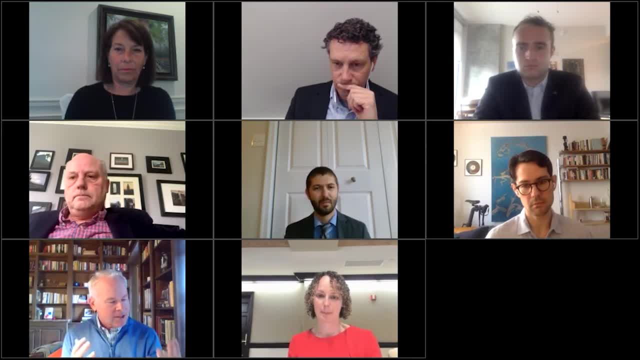 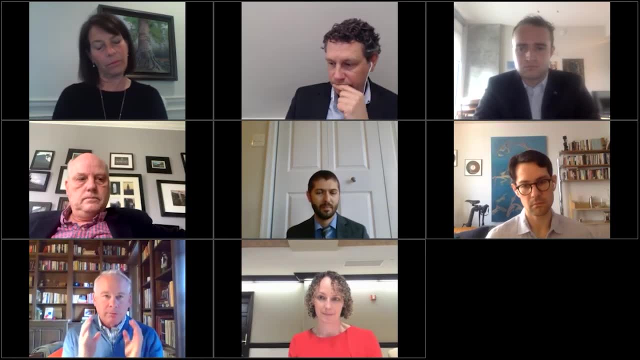 It's odd that we don't talk more about that, But the idea is physical risks- on the one hand, your docks will go underwater and the other is transition risk- And my concern is that much of the real risk that companies are facing are private governance risks. 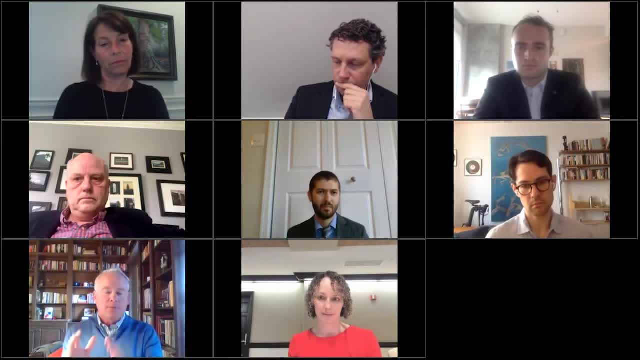 It is that your supply chain. I have a paper that's about to come out that says that 80% of the largest firms in seven large global sectors are imposing environmental requirements through supply chains right now. But that's not a regulatory risk, which is the way the SEC, I think, conceives of a transition risk. 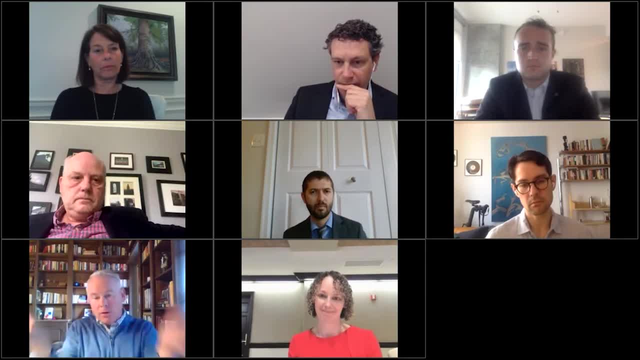 And it's not a pure market risk, It's something in between, And I think all of you all. one of the things I love about this paper and all the commentary is: you all get that. You're working with that. You're working with that every day. 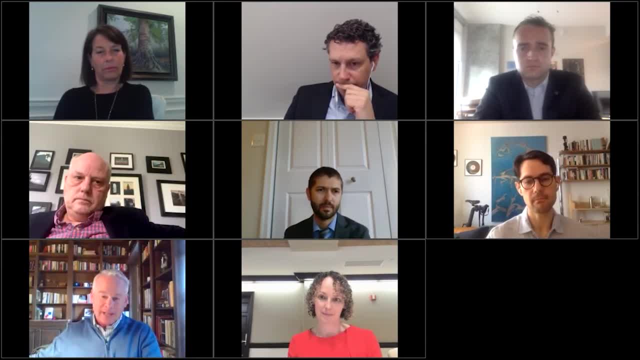 But if you actually look at the 2010 SEC guidance- and I haven't fully gotten through the hundreds of pages of the new one, but I don't see that conceptualization of the risk being captured earlier. Maybe, Maggie, you've really gone through it. 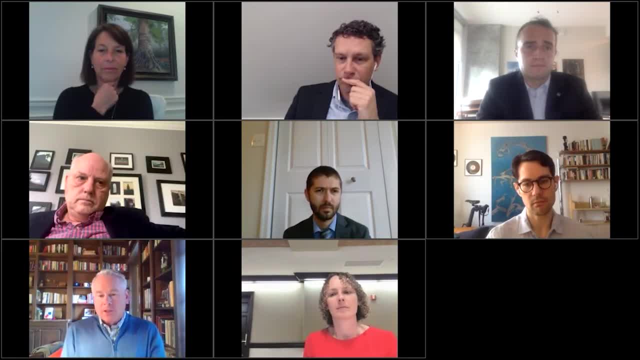 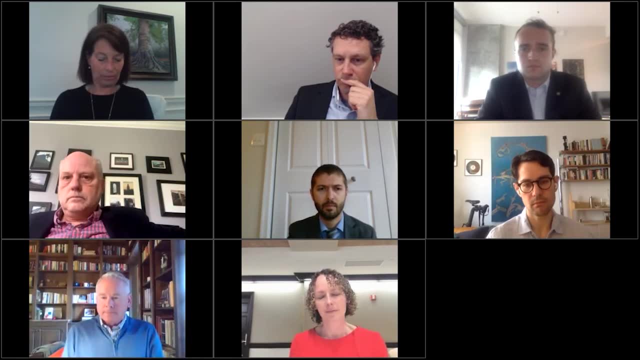 Maybe you see it more coming out in this version. I tried to get them through comments to do more of that, but I get a sense that we're all still functioning in an old sort of pure market or pure government regulatory area. but we're in a different zone now. 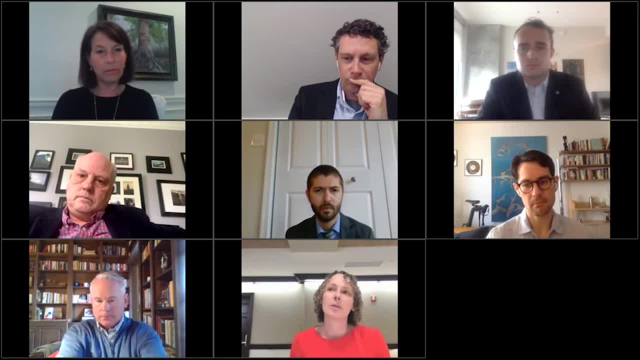 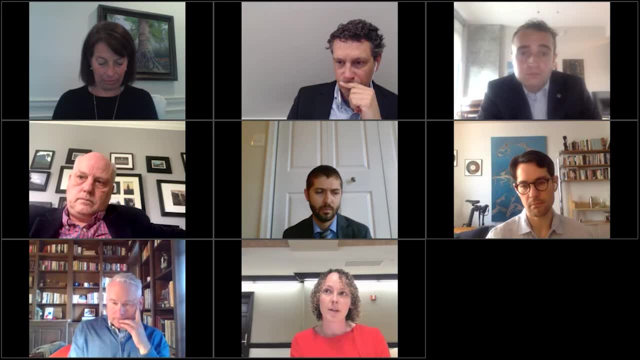 Yeah, I think, Mike. just to respond specifically on the issue, The proposal- I think that you're right in a lot of ways. I think that there is a bit of a sense of, if we push more on better governance, disclosure and more granularity about how you spot risks, that maybe we will, as an ancillary benefit of that, get some of these other disclosures. 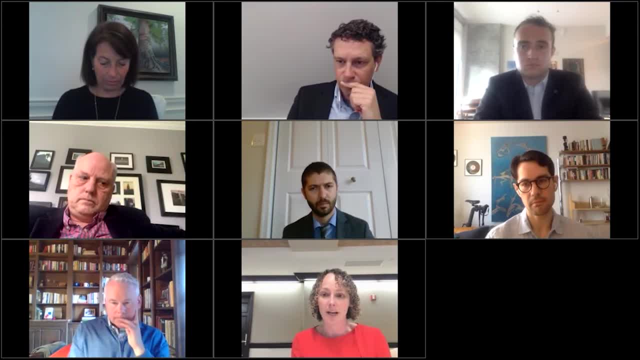 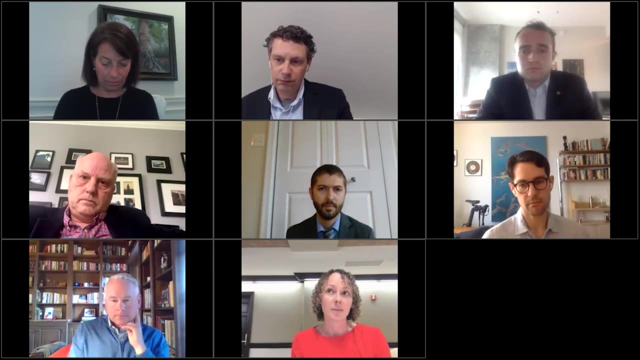 But I think that the private governance element of how this all happens is really where it's going to be in a lot of ways for corporations, right That even with just a proposal, We are already seeing lots of companies asking a lot of hard questions about how do, how do I shape my conduct or report on my conduct so that, when this rule is effective as to me, I can comply with it. 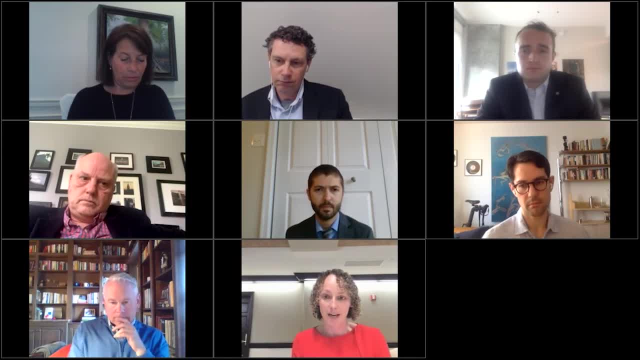 And I think to the good point that was raised about private companies. right, Some private companies are going to say, oh, this doesn't apply to me. But some are going to say, I might want to sell myself someday, I might want to IPO. 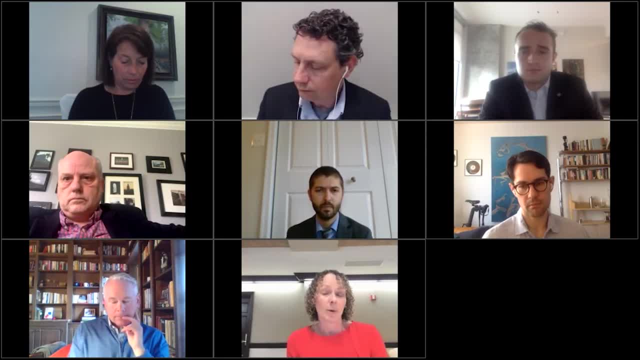 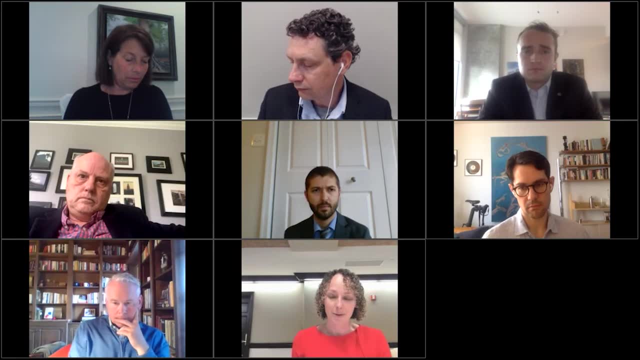 And how do I think about that? Or I might be the upstream oil and gas supplier, Just somebody who is subject to this rule. Or maybe I want JP Morgan to underwrite a bond for me and they're going to be subject to this and they're going to need to then report what they've done in their underwriting as part of their scope. three emissions: 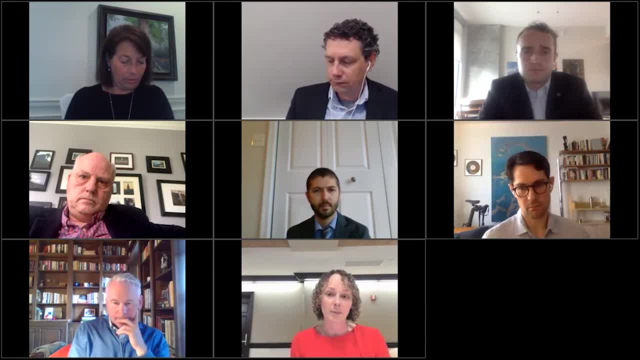 And so I think the private governance part is really fundamental and is perhaps not coming through as clearly in what the commission has proposed, And I don't know if that's because of a lack of appreciation for it or just because that's a really hard thing to get at. 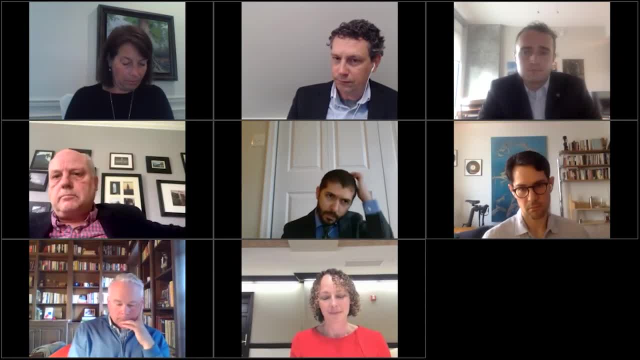 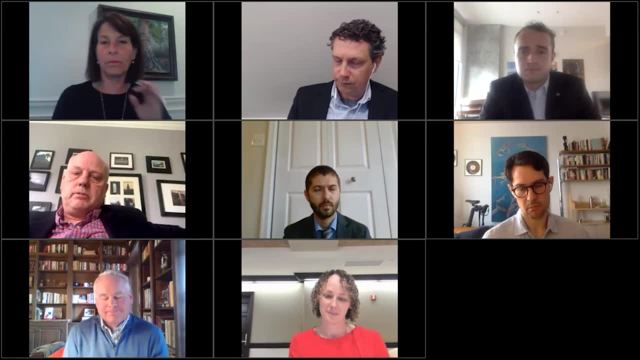 But again, Maggie, though there's always going to be- I mean companies, I'm sorry, but there are companies that make money the wrong way throughout history, and that's not going to change, And there needs to be a level playing field. 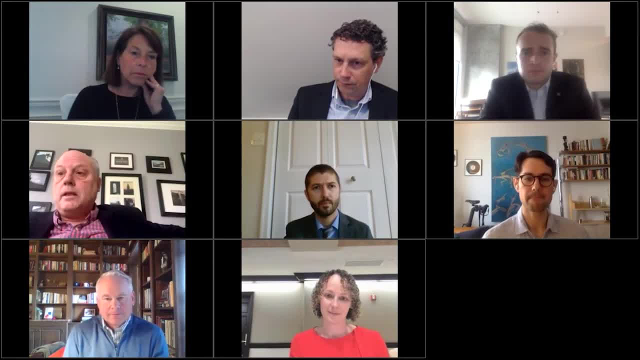 And all I'm saying is by not addressing the rise of private companies at the SEC is just going to imbalance it even more. You have to address it And most of those companies use SEC exemptions to raise capital. The other point I think we make- you know- I thought Mike made a great point about climate- is Ukraine and Russia. 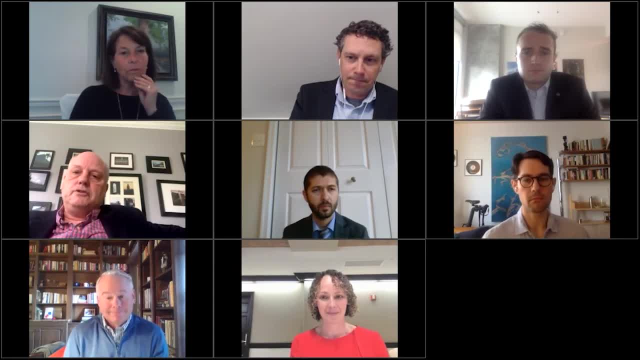 Had we focused on genuine, sensible energy independence and addressing clean energy 20 years or 25 years ago, as we should have, we'd be in a much better position, And now we find ourselves in the confounding place of using dirty energy and having an argument for dirty energy because of national security, when it's actually the opposite. 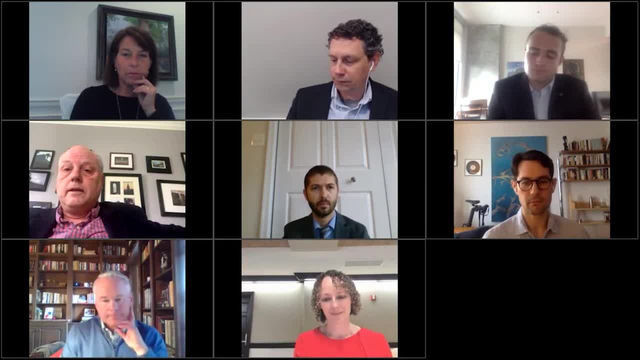 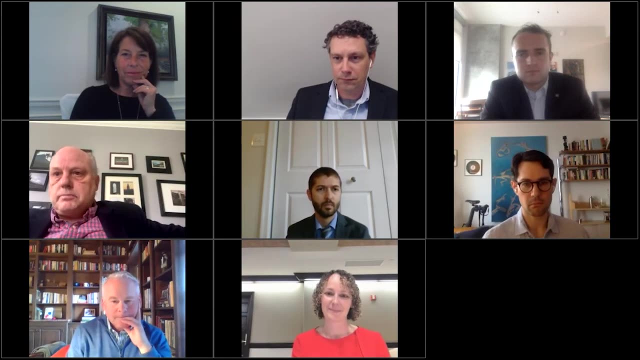 I thought Mike's point also about jobs and opportunity for the American and for the OECD nations through innovation is something We do. But here's the point. a point about businesses: Where are they? on President Biden's effort to finish the climate change investment package? 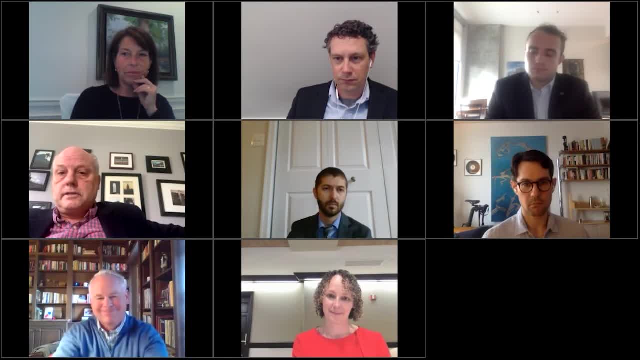 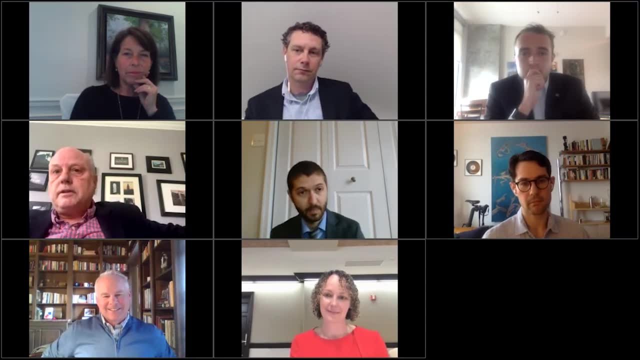 I blame my own party for three and a half trillion dollars of diffuse nonsense. If you called Build Back Better the infrastructure bill, that makes a lot more sense to the American people. And if you do the poor part of climate that's still left, that's an adjunct to that. 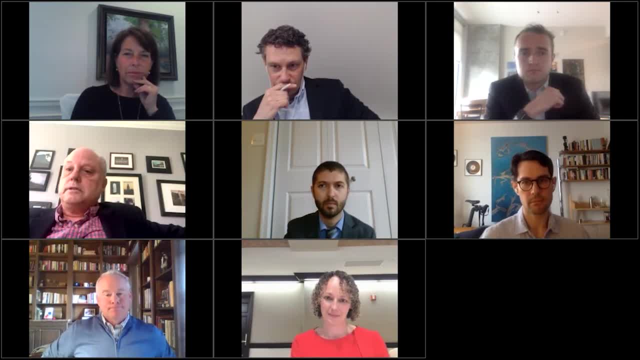 But where are the businesses that we're talking about? Maggie and Jonas and Elizabeth and Todd, Where are they? Where are they on that? Because don't tell me about your disclosures if you're not going to support the process, And it takes time. 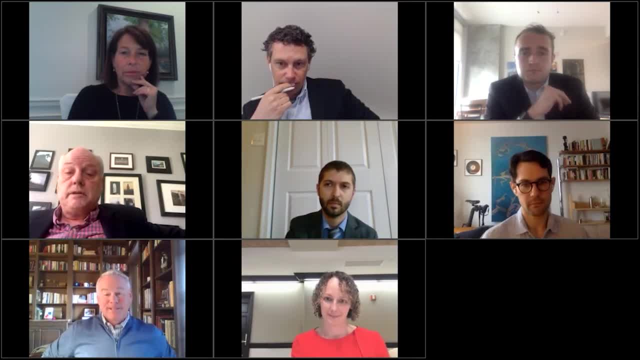 I mean, there was a hydrofluorocarbon ban done during the Trump administration And it's because of our senior senator in Delaware, who's a Democrat, who worked his butt off like an old time senator to get- and he gave credit to crazy people to get it passed. 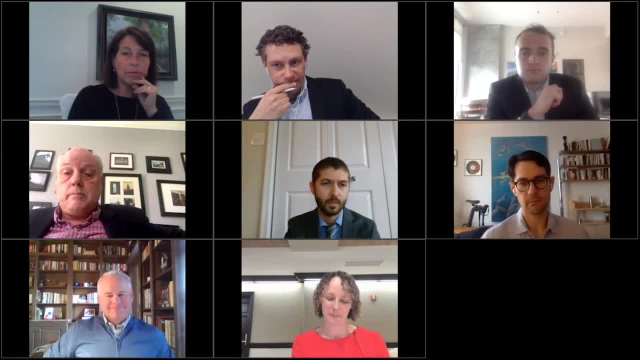 But he had the Environmental Defense Fund and the BRT do it. But it takes time. But business could get the Biden package done If they use their voice and frankly, where are they and how have investors hold them accountable? I think that's a key thing. 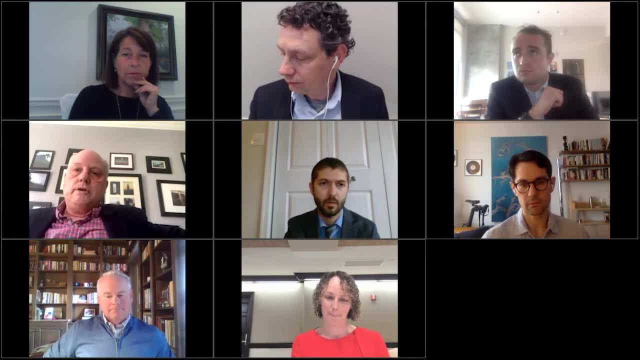 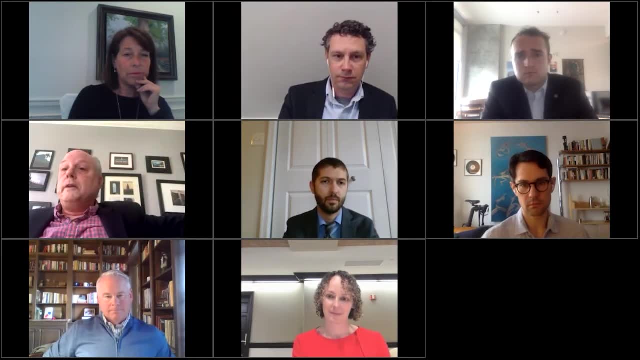 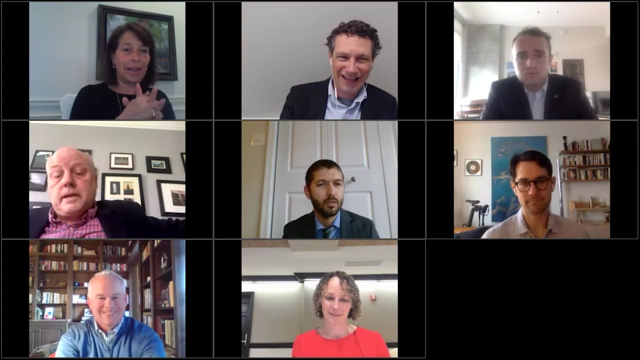 And that's why it's a cycle of disclosure as well, where I think, Jonas, you're entitled to know all along the dimensions of corporate impact, what they're doing and whether it really aligns with what they're saying, Because I don't hear a zombie from K Street going to finish the climate change package. 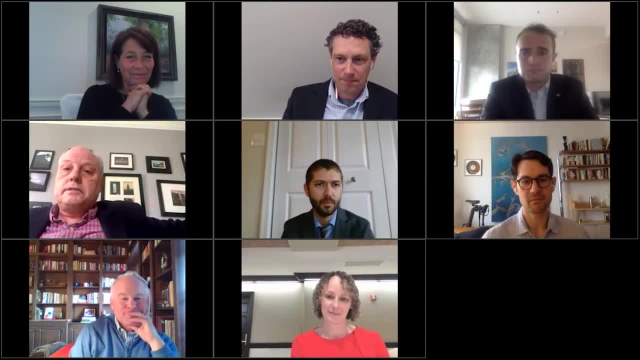 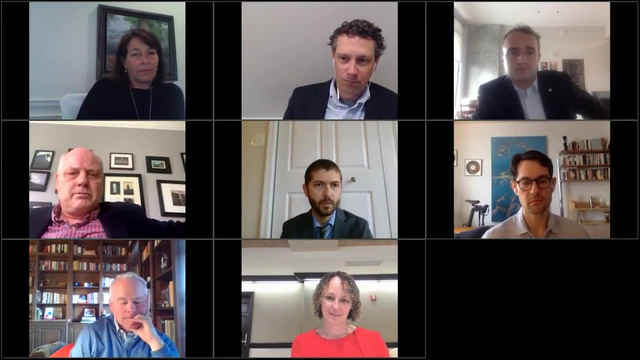 And even frankly saying to some people in my party: yes, we understand the need for more child care. That was kind of put on the table late in 2020.. And you didn't really read the primary results. This climate thing is really important. 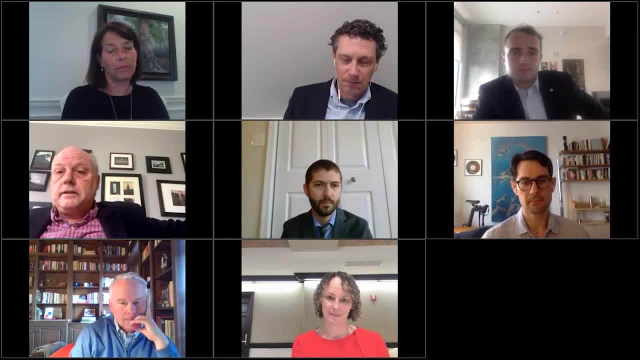 It really does relate to jobs And, by the way, Joe Manchin might get it if you put another hundred billion into the climate with the transitional thing for the industries, And it focused on the parts of the country that generate oil And there was a specific focus on the workers and communities. 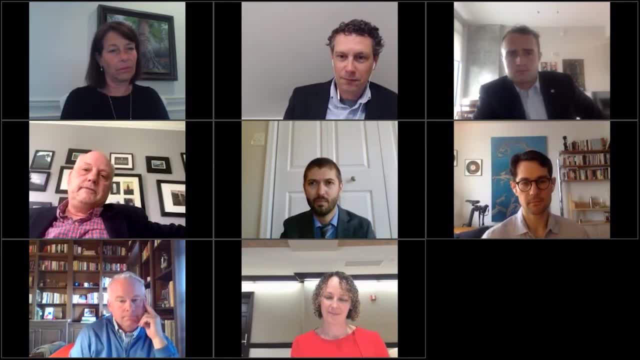 You know, That's the kind of thing where I'd love to see the business community, instead of putting out another sustainability report, have their own march on Washington. This should not be a partisan issue. It's good for the economy, But that's real stuff. 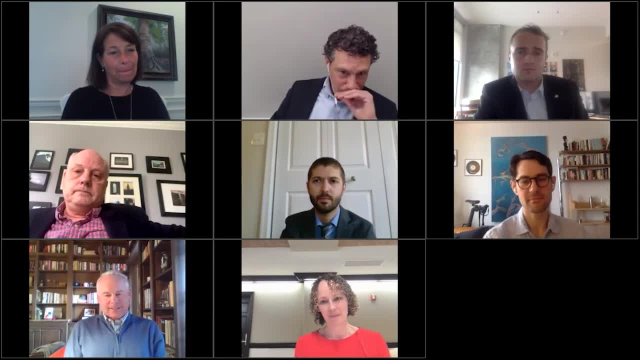 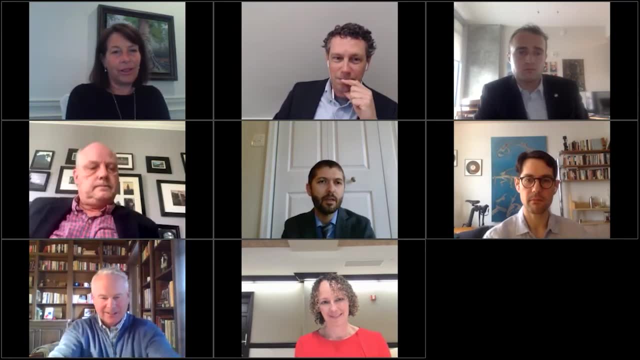 And this system has to deal with that. Jonas or Todd, do you want to jump in Because we're going to run out of time. I want to make sure you can engage. Yeah, I'd like to jump in and say: you know, I agree with everything. 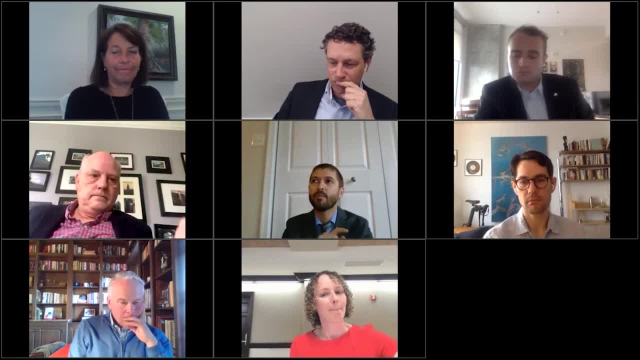 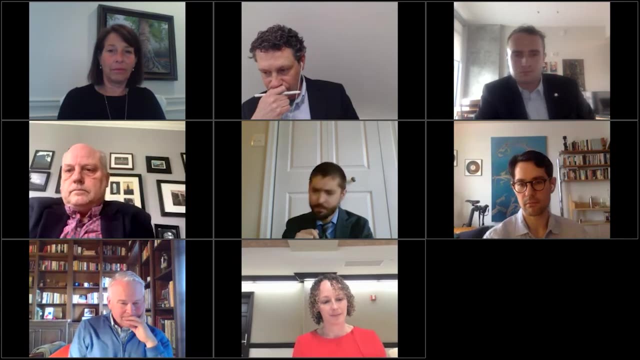 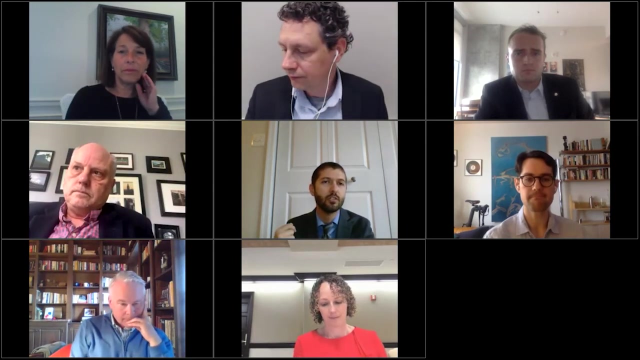 Chief Justice, I think we're facing an issue here in law in that, you know, Congress is not going to enact new regulatory statutes anytime soon And I think that, to the extent the agencies want to work on these issues, to the extent that investors are calling for climate disclosures, the SEC has to work within its existing 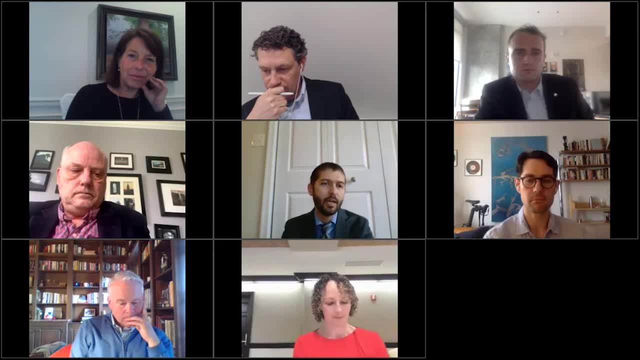 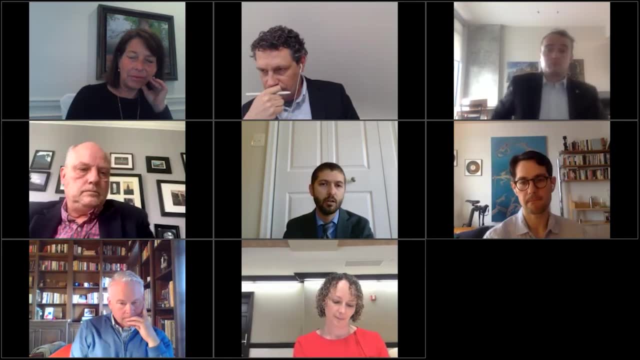 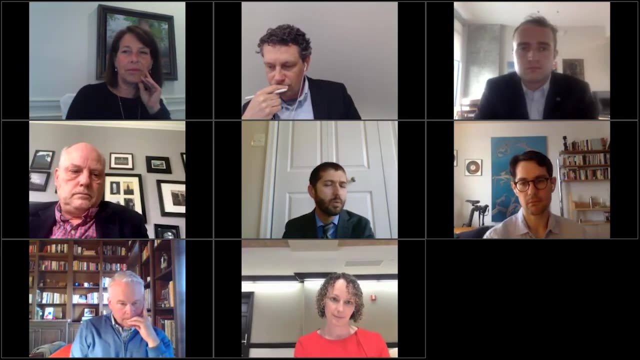 Statutory framework to get there, And I think that this climate disclosure rule is one thing that will help us get there. I think that there are a lot of other things on the SEC's unified agenda. There is at least one proposed rulemaking, if not more, talking about closing private market loopholes. 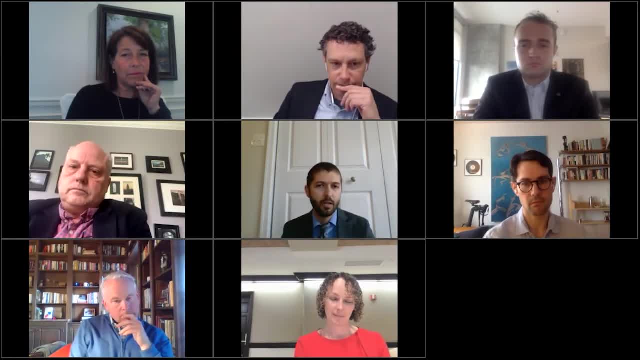 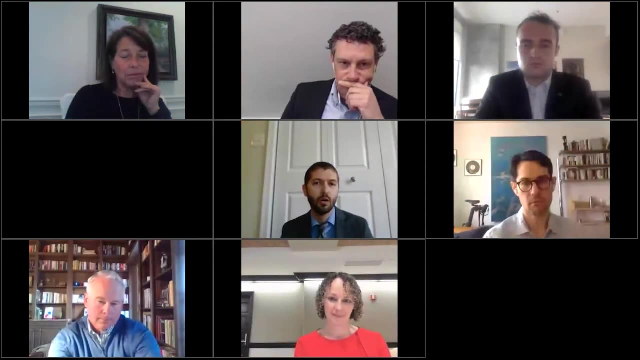 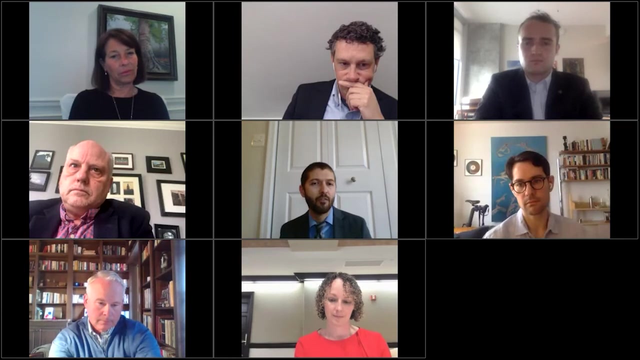 There are just a lot of things here that we're talking about, And I think it's It's a process that just has to be worked into the Securities Act and the Securities Exchange Act. I mean, the fact is that there are people who are on the other side of this rule, who are claiming that the SEC is taking up the mantle of climate regulation and is trying to declare: you know what companies have to or cannot do regarding climate emissions. 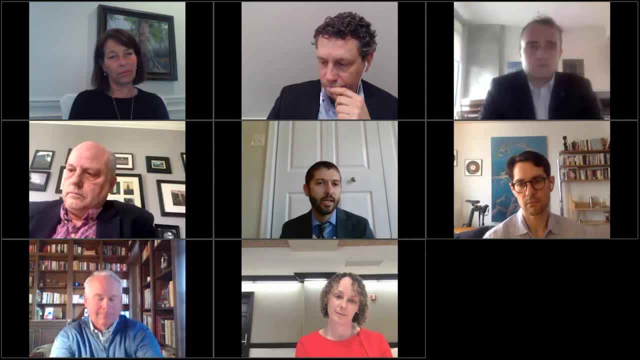 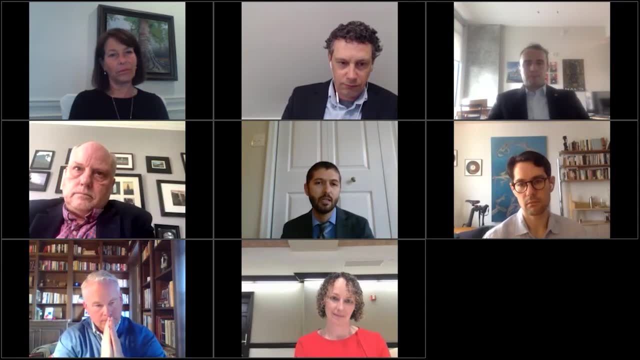 And One. I mean not only is that not what the SEC is doing here, but it's that side trying to take down this rule. that really is about what investors want and need and is core to the legal mandate that the SEC created in the 30s. 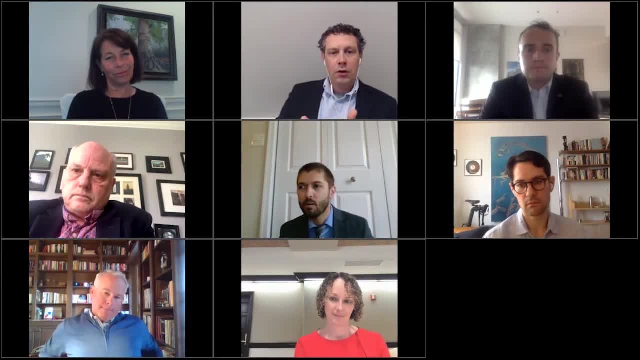 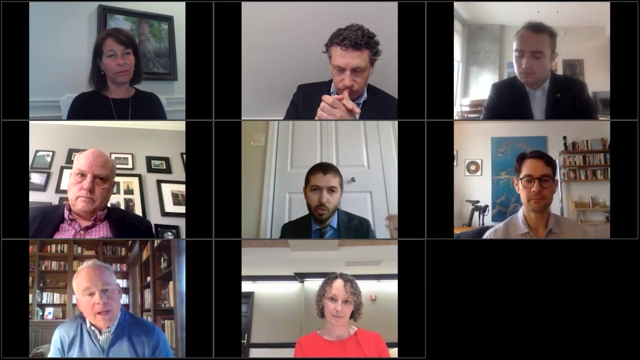 I think that there are just a lot, of, a lot of issues here with double ESG and You know, To the extent we we can push Congress to enact new statutes, great. but beyond that, Regulators need to work within their existing authority and I think that's they're doing what they can do with limited resources. 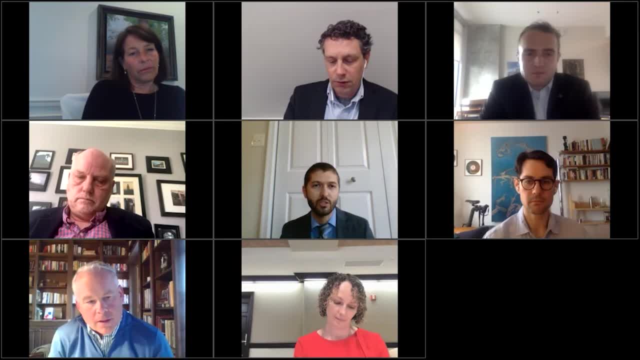 And it takes, I think, folks like all of us trying to push Gary Gensler to move the SEC in a quicker direction on a lot of the issues that we care about. Something I would say is that if I were the SEC chief of staff right now, 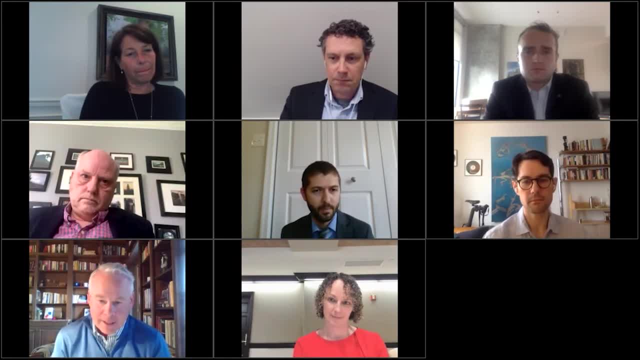 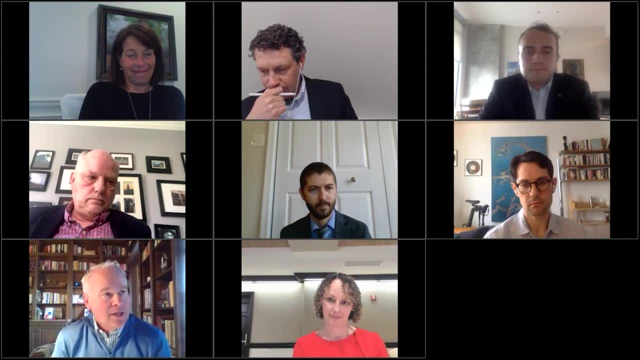 What I would be doing is, and Maggie, putting the pedal to the metal on getting this thing out the door, because the longer it will pass, I think, the more opposition builds. as well as that, you know you can expect appropriations riders down the road. 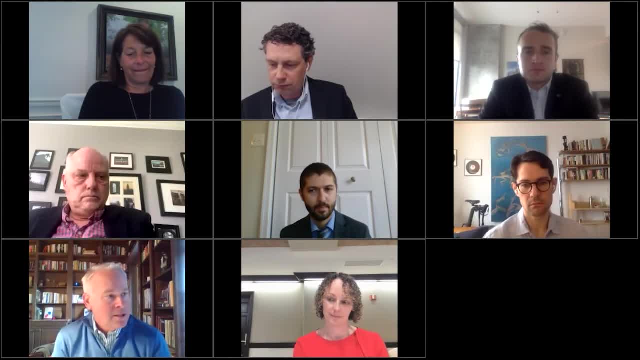 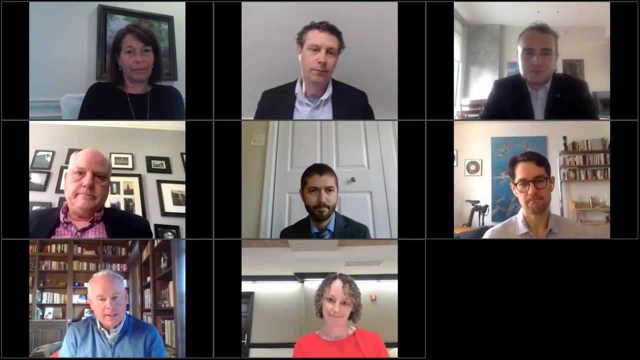 And I think it'll be fascinating to see when this finally gets to the Supremes. if it does, whether the major questions doctrine eats this alive, like it will, you know, the Clean Air Act, Section 111 regulations. I think there's a lot of risk out there. 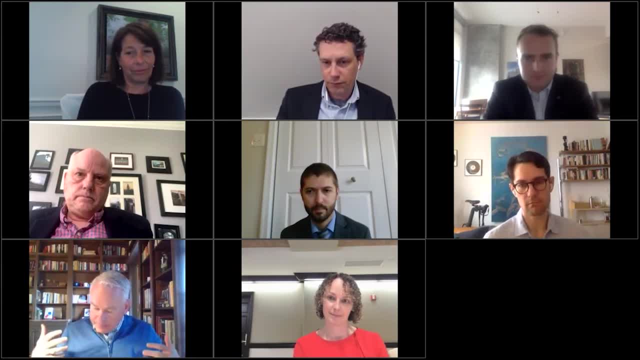 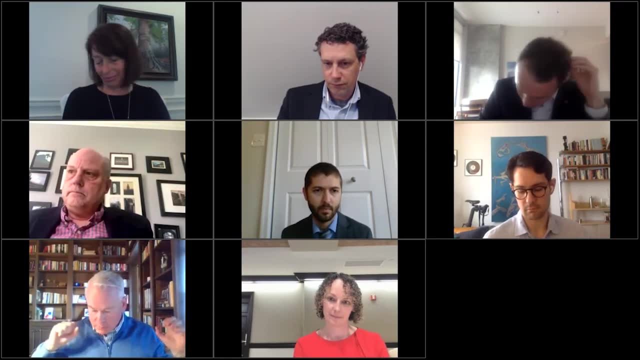 Which is one reason why I keep coming back to the idea that You know again if I'm at JP Morgan right now, even if the school goes away. CDP has requirements. there are lots of pressure you're getting from shareholders. 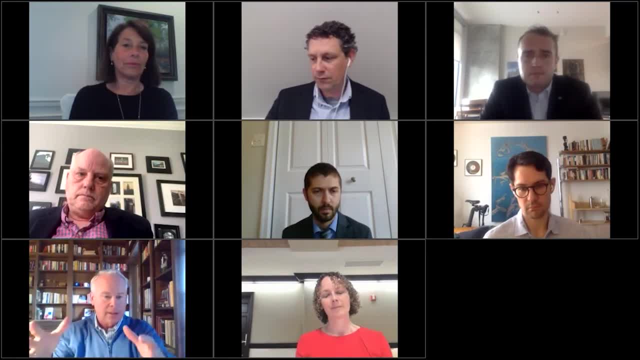 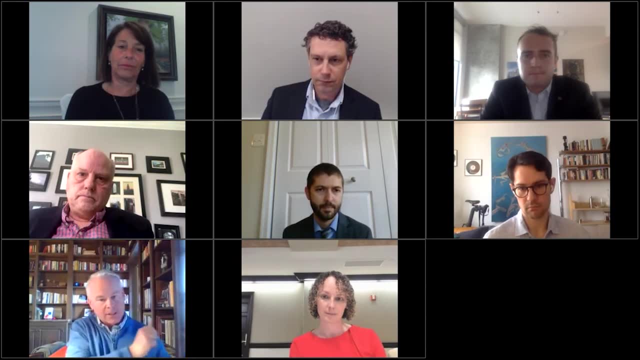 So there's a whole private set of things that are going to continue right now, even if this rule doesn't succeed, which is a reason why I think we have to make sure we don't put all of our eggs in, assuming it's going to be public regulatory options or not. 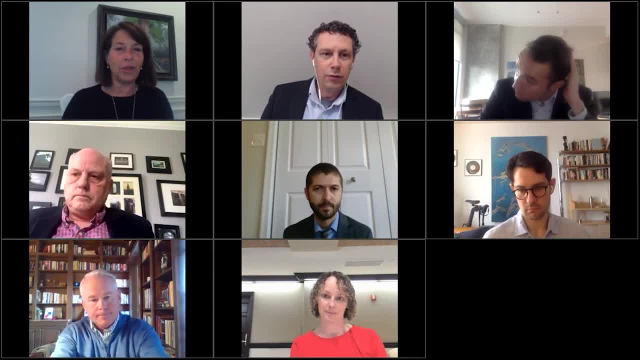 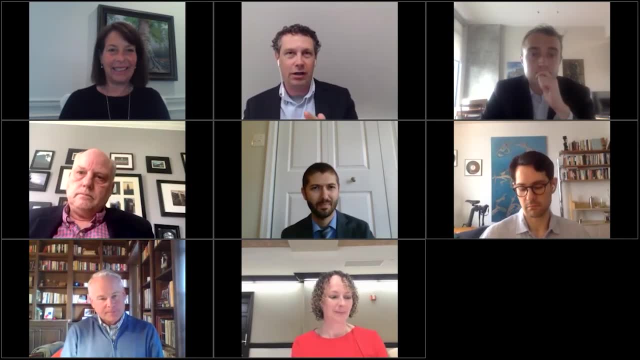 Not that I don't wish we would have them. Jonas, did you want to say one last thing? We're basically out of time. I'll just make one last point, One really quick comment. I appreciate this conversation And a lot of what we've been talking about here, I think, is really sort of about power and where the power resides and how the power is expressed. 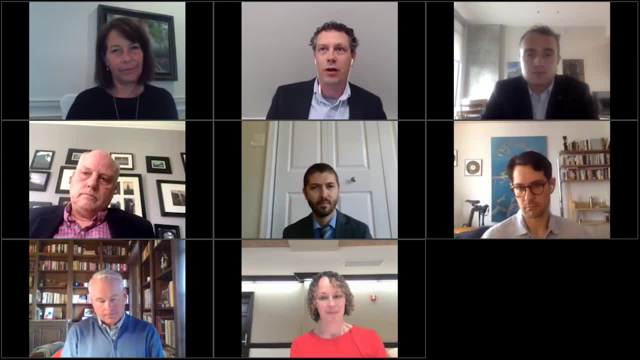 One thing, and maybe this sort of pulls a lot of it together. One of the things that I really liked about the paper and that we haven't really gotten into here is the human element, in the sense of what companies are doing right now is not only motivated by the regulatory environment, not only defined by the physical risks that are happening, but their employees. 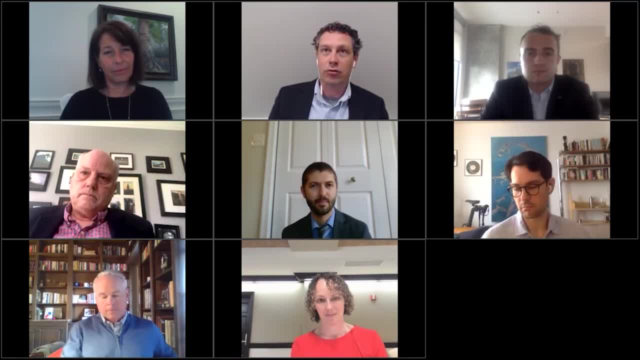 The generation of employees that they are competitive for. right now. It's incredibly demanding, And one of the things that this paper does that I think is really important is it talks about the role of reputation. It talks about the role of embarrassment and shame for CEOs and managers and boards of directors. 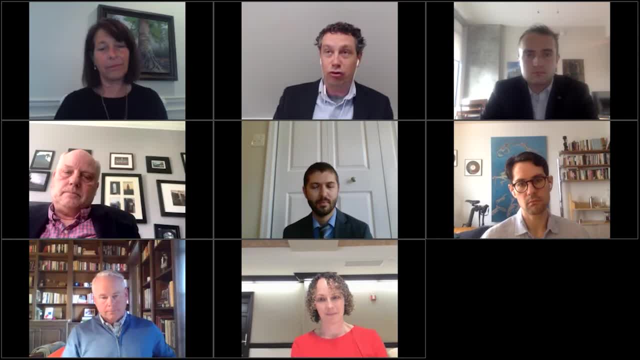 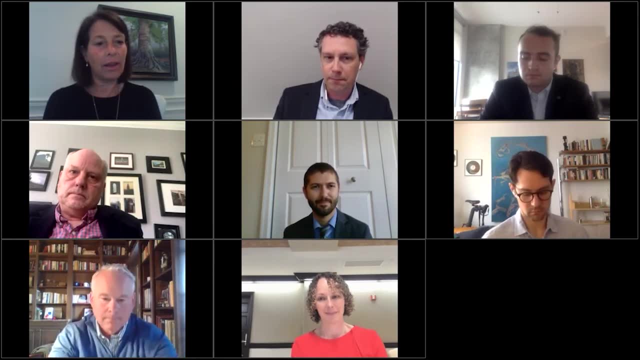 And that human element within the companies, I think is a really important driver of a lot of what we're talking about right now. that we probably haven't touched on And I just sort of wanted to pin up there. Yeah, Okay, We're basically out of time. 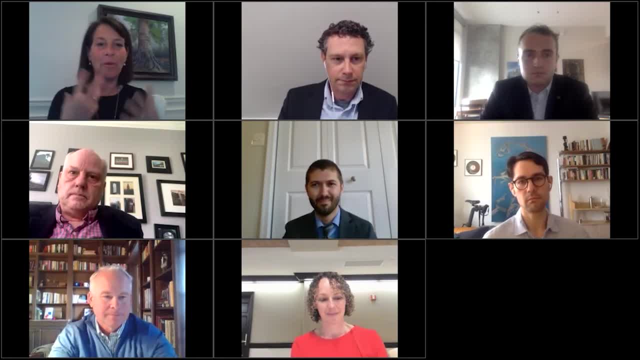 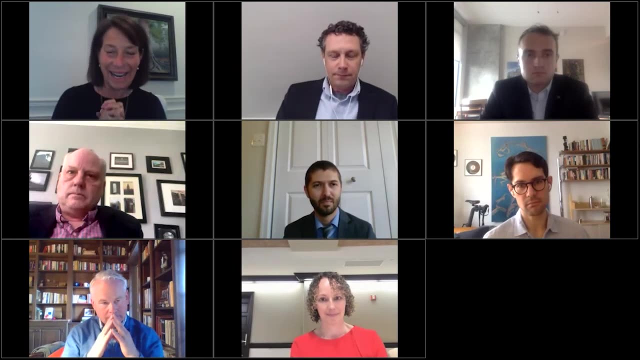 And I'm sorry we didn't get to audio Audience questions. I just felt like this is probably one of the first really robust conversations about these recent developments. and just an exceptional panel. I'm going to offer on your behalf that if somebody put a question in the question box and they really would like to get an answer to that question, just put it in there again and I will direct it and hopefully, offline, some of our panelists will be willing to respond. 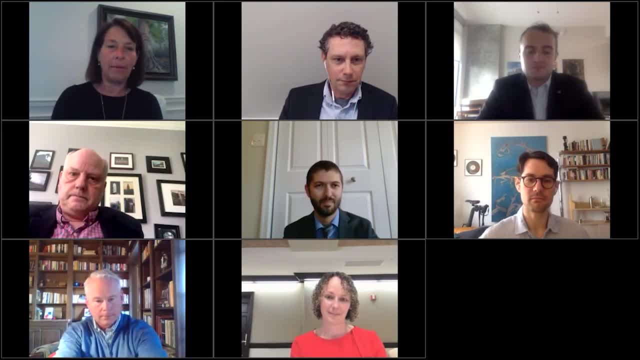 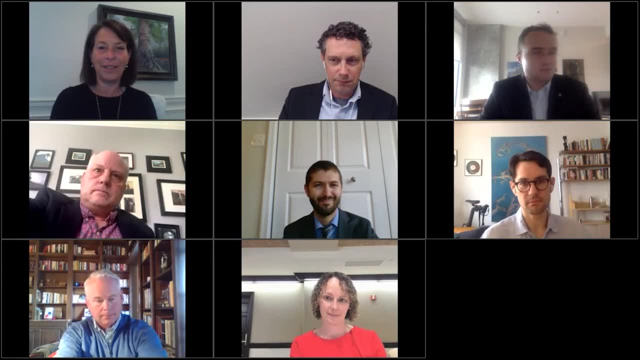 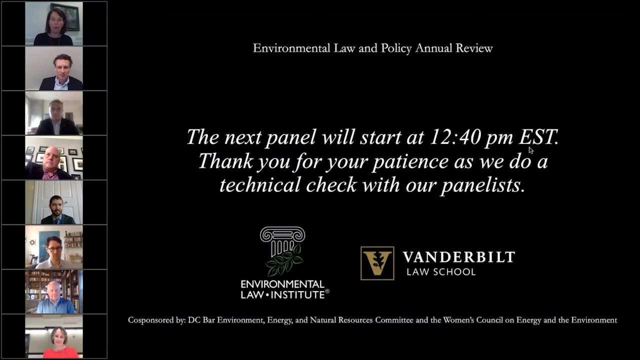 So thank you for a wonderful discussion. We're going to Take a basically a 10 minute break. Once again, we apologize. you will be able to hear us doing the tech check, but we will reconvene in about 10 minutes to talk about our third and last panel on rethinking great governance for the climate change era. 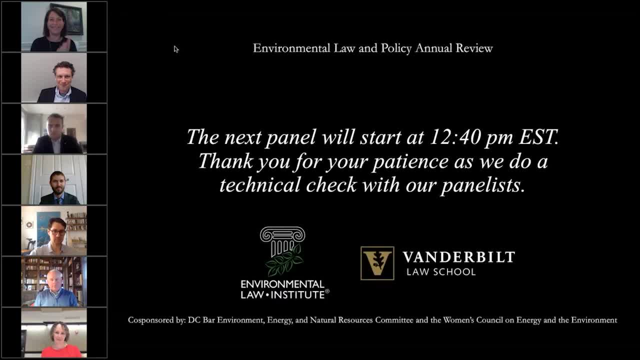 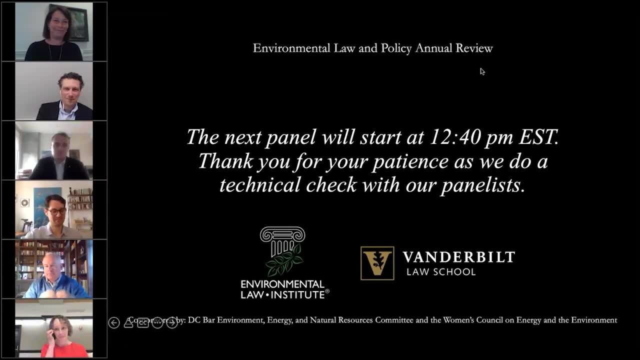 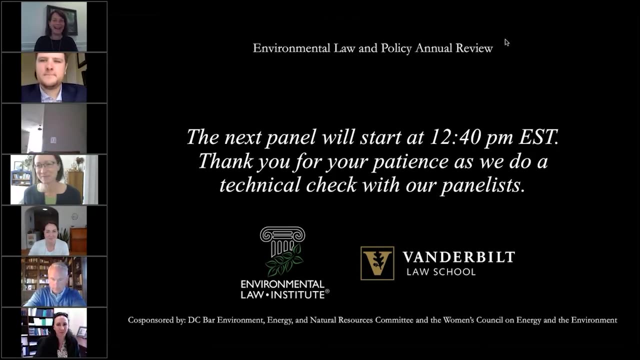 And again, thank you so much for a fantastic discussion. Yes, thank you. That was a terrific discussion, Great paper. Thank you everybody. Thank you so much, Thank you, Thank you, Thank you All right, Well, welcome back everyone to our third and last panel of the day. 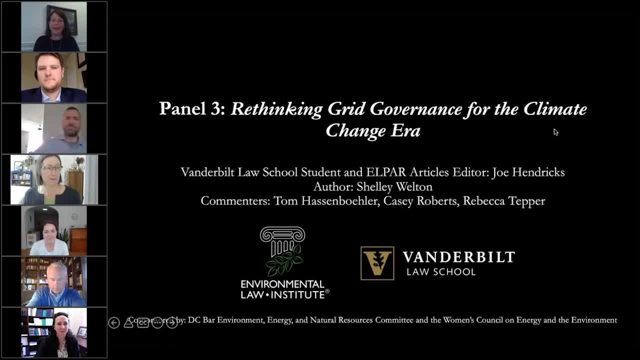 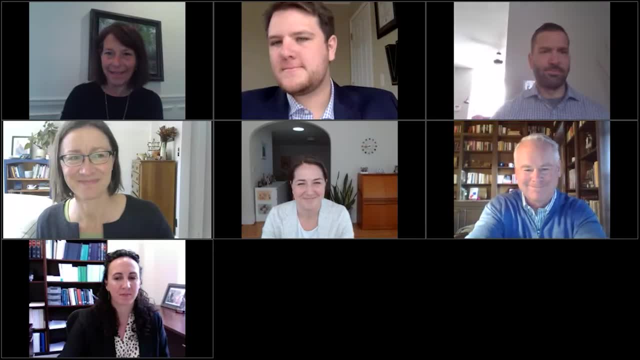 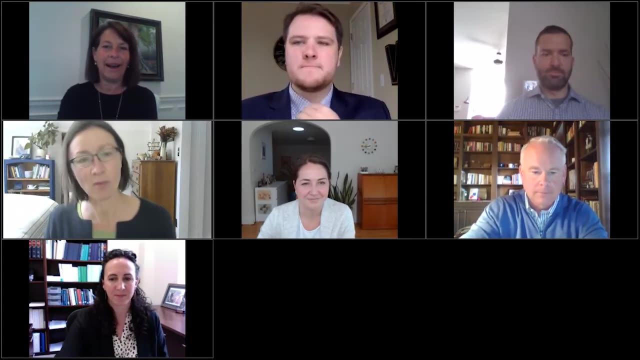 Before we start our panel, I want to introduce our new Environmental Law Institute president, Jordan Diamond, who has joined us since our last LPARC conference, and, as many of you know, Scott Fulton has moved to President Emeritus, so he'll fortunately still be working with us. 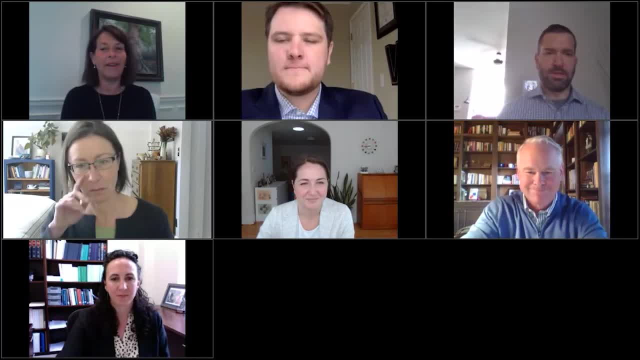 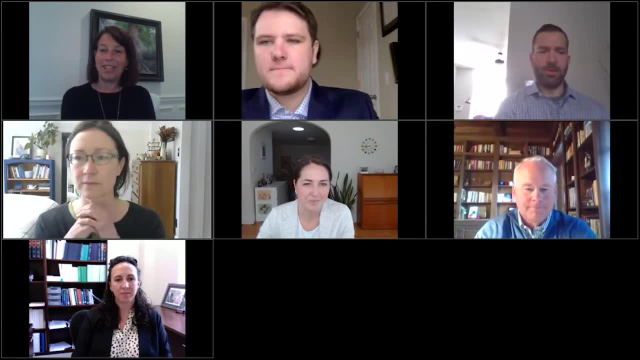 But we're so excited to have Jordan. She joins ELI from UC Berkeley, where she was the executive director of the Center for Law, Energy and Environment, And she is also a former ELI attorney, so she's come full circle and we're just so excited to have her back. 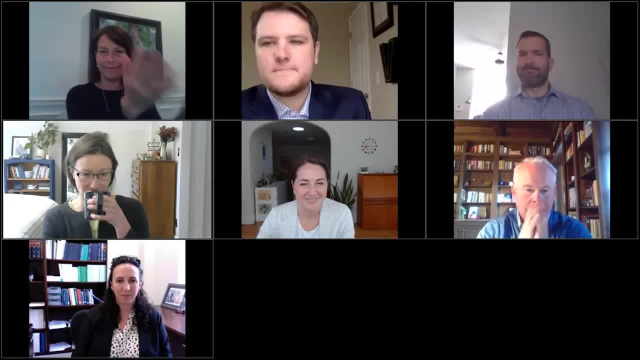 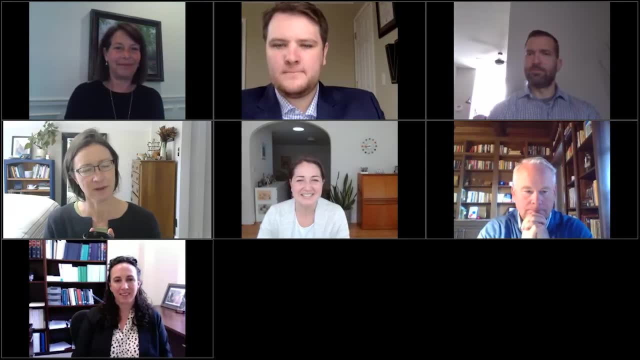 And I just wanted to hand it over to her for just a minute to say welcome and let you say a few words before we jump into the panel. Thank you, Linda. It's wonderful to be here And of course, it's nice to virtually meet all the vampires. 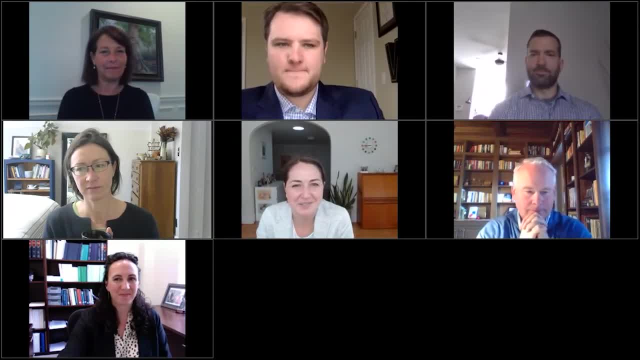 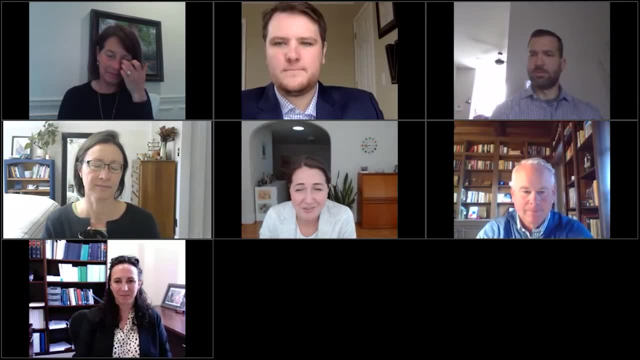 Thank you. Thank you And all the Vanderbilt students who are doing such a great job of introducing the panels today and did such a tremendous job from the outset of picking these articles with, of course, instructors and, of course, with our terrific LPARC advisory committee. 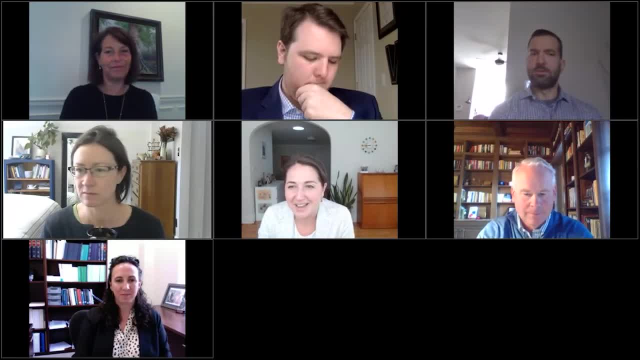 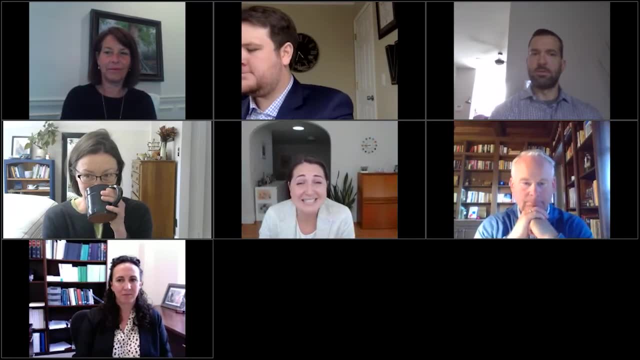 In the interest of time, as Linda said, I will keep this extremely brief. I simply wanted to take a moment to personally and personally welcome everybody to the final panel session of the day and express my sincere hope that we are back together in person next year. 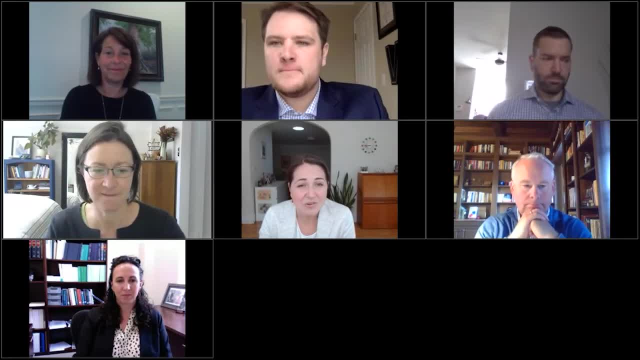 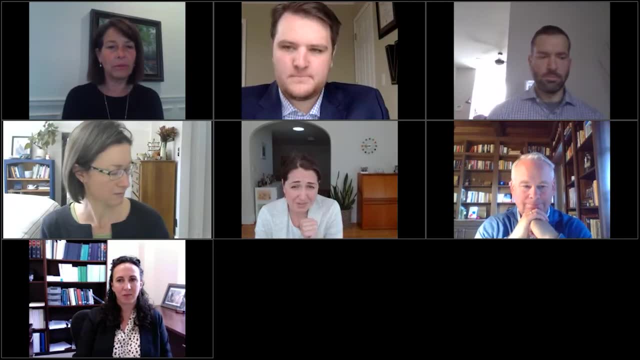 It's a particular joy to welcome everyone to this panel, which is focused on such an incredibly important topic and really the cutting edge of where we need to move forward, Stepping back. I also wanted to offer one additional note, Although- and this is a conference as a whole- 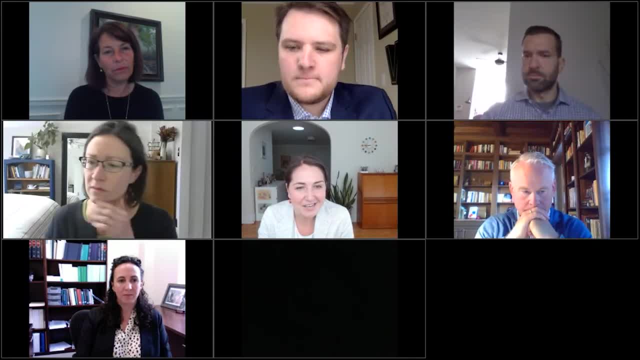 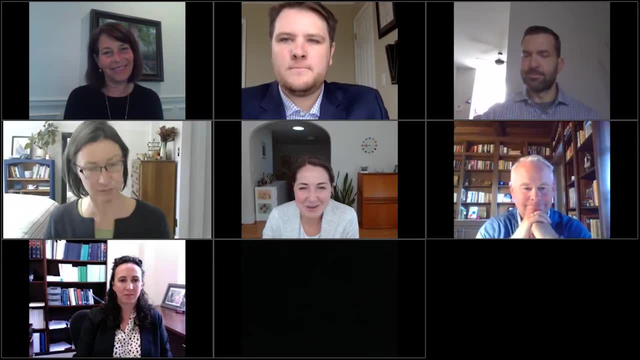 although I have only recently returned to ELI after an eight year hiatus at UC Berkeley, I have kept track of LPAR over the years, And that's because of the immense value I place on bringing ideas from the academy to policy makers and to practitioners. 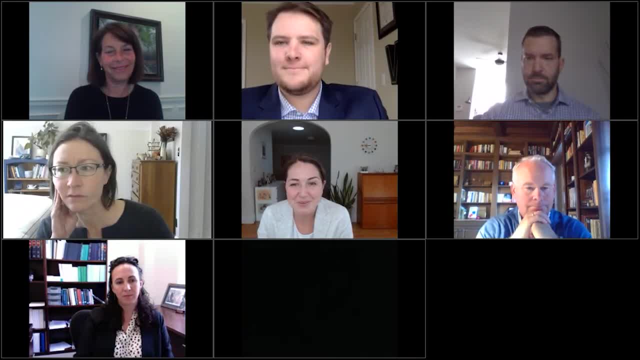 Because while we otherwise, we do in fact know that busy lawyers don't always have time to peruse law journals, Although I feel traitorous saying that because I met Casey Roberts when she was my editor-in-chief at the Law Journal at UC Berkeley. 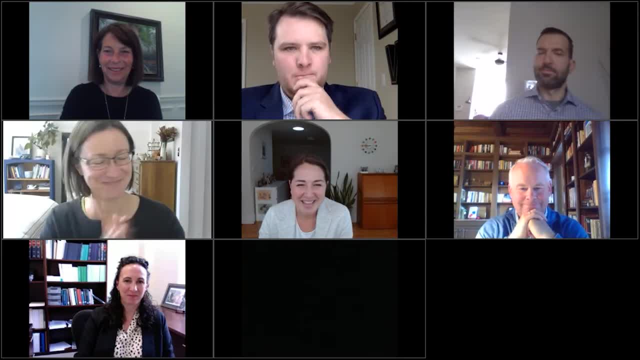 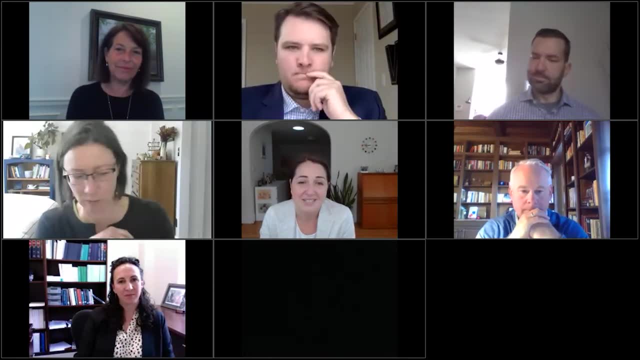 Casey, that was not true. we were working together, obviously. But in general LPAR has been such an outstanding 14 year partnership with Vanderbilt Law School which we hope will take us far into the future. So with that I will stop hogging the microphone. 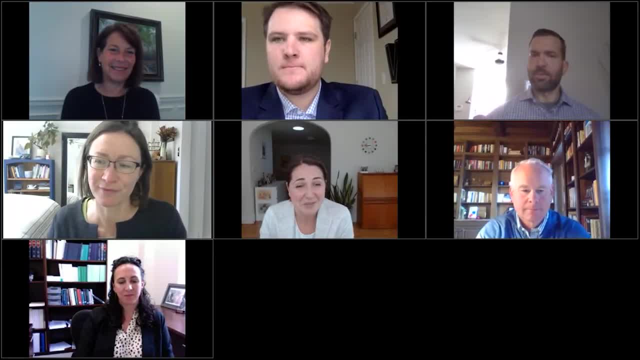 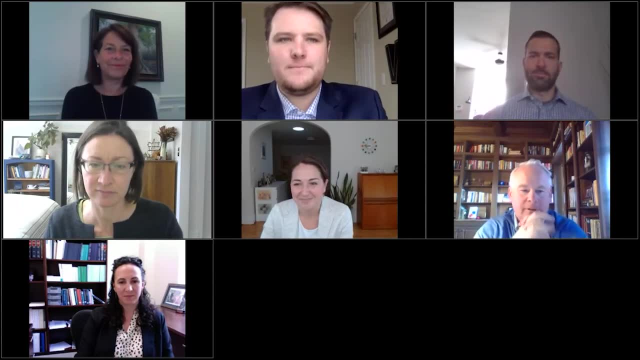 and simply extend my thanks to all of you for joining us today. We look forward to the conversation Back to you, Amanda, Thank you so much. We really appreciate your effort. Jordan, Glad you're joining us. Well, I'm going to hand it over now. 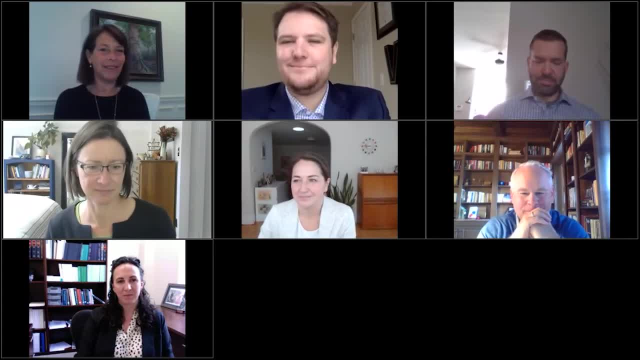 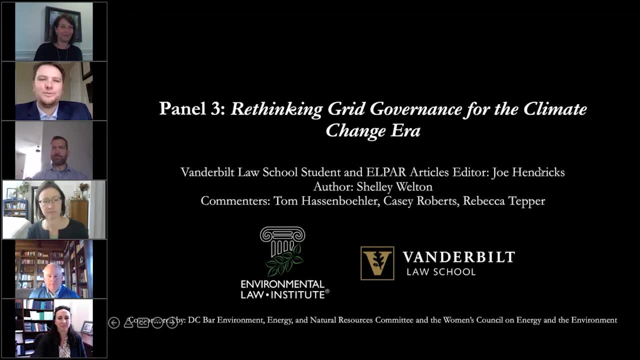 to third year law student, Joe Hendricks, to introduce our fantastic panel. Thanks, Professor. My name is Joe Hendricks. I'm a 3L at Vanderbilt Law School and an articles editor for LPAR. I'm here to introduce our third article. 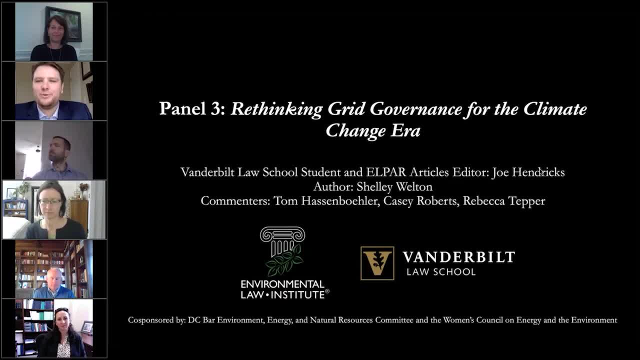 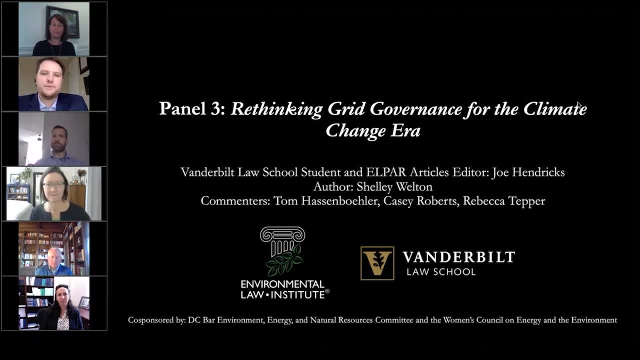 Rethinking Grid Governance for the Climate Change Era by Professor Shelly Welton. Professor Welton is an associate professor at the University of South Carolina School of Law and the incoming Presidential Distinguished Professor of Law and Energy Policy at the University of Pennsylvania. 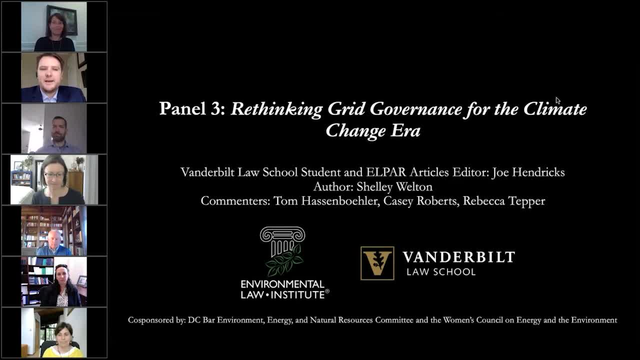 beginning summer of 2022.. Prior to academia, she was the deputy director of Columbia Law School's Sabin Center on Climate Change Law. We also have three panelists with us today. First is Casey Roberts, In her position as a senior attorney at the Sierra Club. 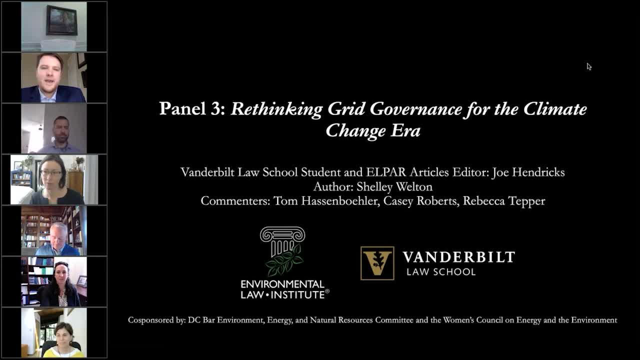 Casey advocates before state public utility regulators and at FERC for policies that protect consumers and allow full and fair competition by renewable energy, energy storage and demand side resources. Before she joined Sierra Club in 2011,, Casey was a fellow at the Natural Resources Defense Council. 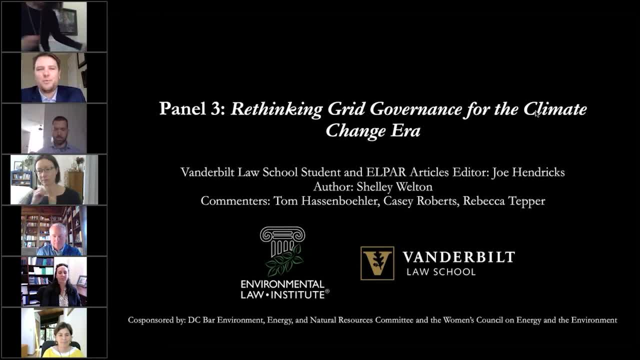 and at Altshuler-Burzen LLP. Casey received her BA from Rice University in biology and public policy and her JD from the University of California, Berkeley, where she was the editor-in-chief of Ecology Law. Quarterly Following law school, she clerked for Judge James Parker. 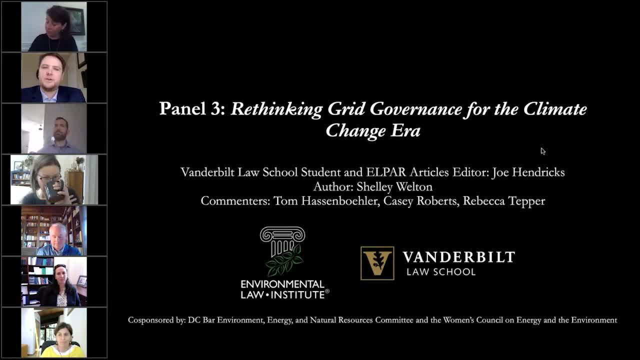 in the District of New Mexico and Judge Diana Murphy on the Eighth Circuit Court of Appeals. Our second panelist is Tom Hassenbohler. Tom is a partner with Coefficient, a mission-based strategic consultancy focused on advancing public policy and market solutions. 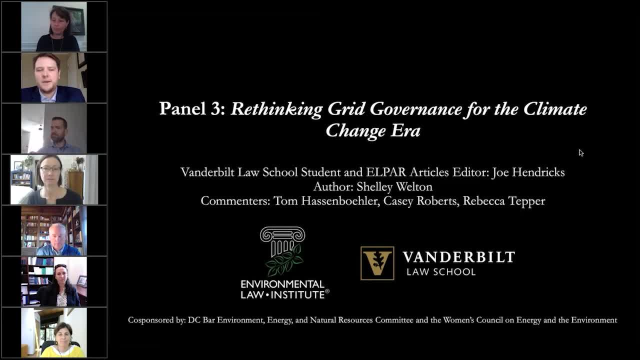 in the energy and environmental sectors in Washington DC. From 2013 to 2017,, he served as the Chief Counsel for Energy and Environment at the US House Committee on Energy and Commerce Before his role in the US House. 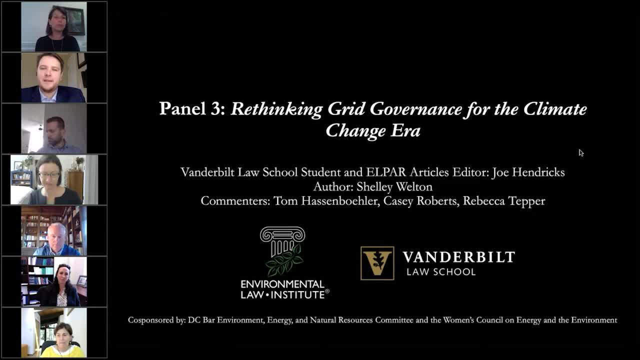 he worked in the private sector as the Vice President of Policy Development and Legislative Affairs for America's Natural Gas Alliance. Tom's earlier experience was in the Senate as Counsel for the Committee on Environment and Public Works. A native of New Orleans, Tom received both his undergraduate 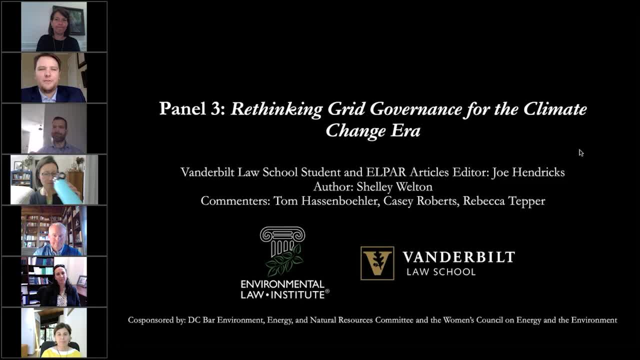 and JD degrees from Louisiana State University. Our final panelist is Rebecca Hassenbohler. As the Chief of the Energy and Environment Bureau in the Massachusetts Attorney General's Office, Rebecca serves as the Attorney General's Chief Advisor on Energy and Environmental Law and Policy. 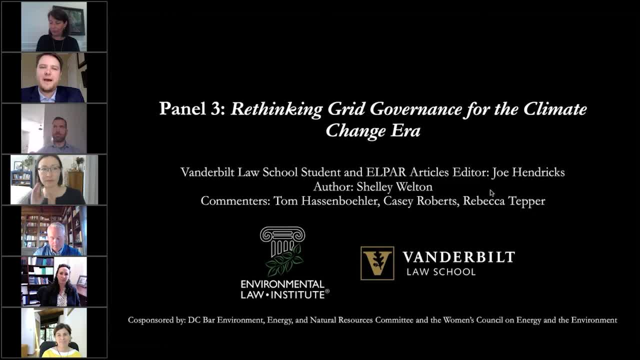 Prior to joining the Attorney General's Office, Rebecca was the General Counsel to the Massachusetts Department of Public Utilities, DPU. Prior to the DPU, Rebecca served as the Director of the Massachusetts Energy Facilities Citing Board, Before joining the state in 2009,. 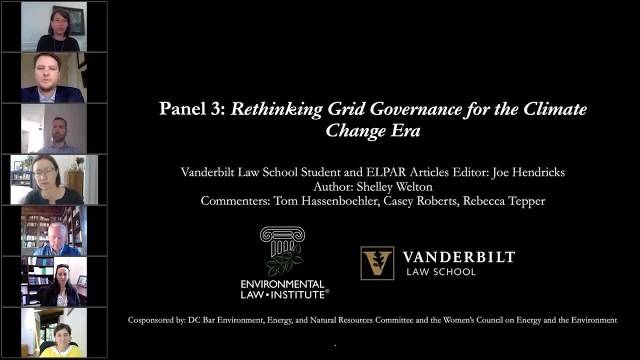 Rebecca had 15 years of experience in the private sector, representing developers throughout the Northeast in siting, permitting, financing and contracting of renewable distributed generation and conventional energy facilities. Rebecca is a magna cum laude graduate of Boston University Law School and received her Bachelor of Arts. 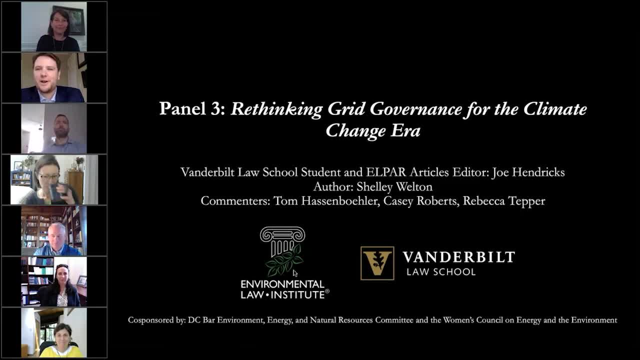 from the University of Wisconsin-Madison. I'll now hand it back to Professor Bragan. Great, thank you, Joe. An incredible panel and we're just gonna jump right in and hand it over to Professor Welton Shelly. you might take about 15 minutes. 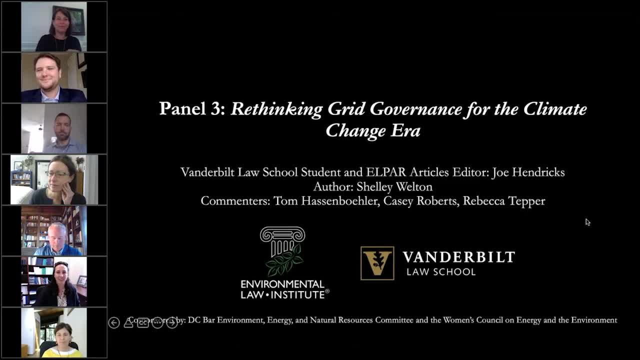 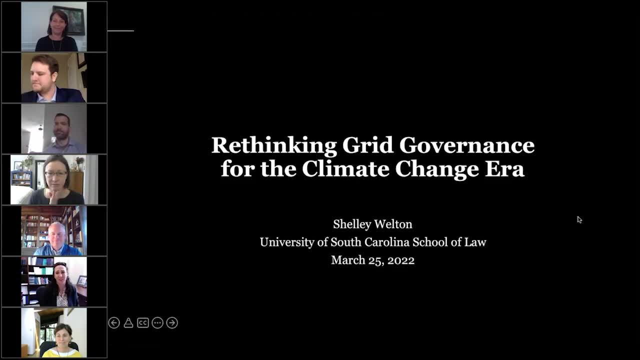 and tell everyone about your article. Great. I wanna just start by echoing lots of the thanks to ELI and Vanderbilt, to the students who I know worked so hard to pull all this off, and to my commentators. thank you so much, Casey and Rebecca and Tom, for taking the time. 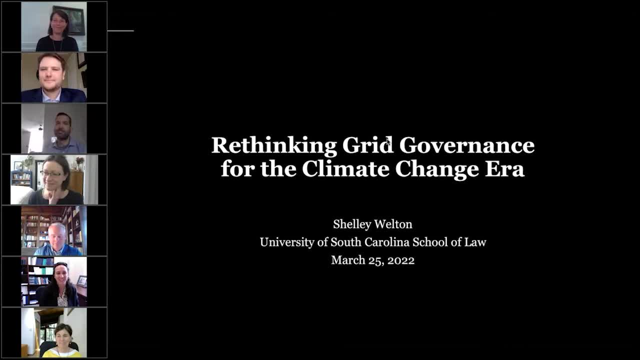 to engage this article and really talk about some of its ideas. it means a lot, So I thought I would start my presentation with just a little bit of good climate news, which always we are in need of. So let's see if I can get this to advance. 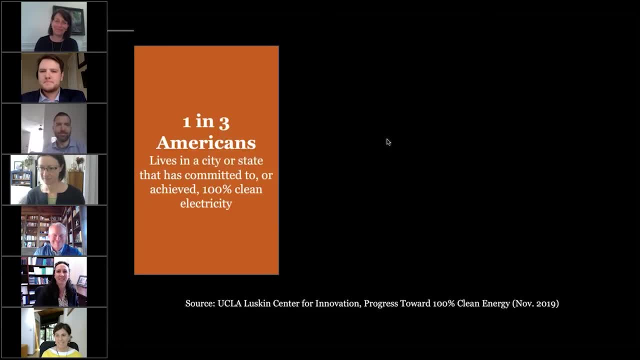 I can't make it advance. There we go. okay, Somebody's making it advance. So here's the good news: One in three Americans now live in a city or a state that has either committed to or achieved 100% clean electricity. 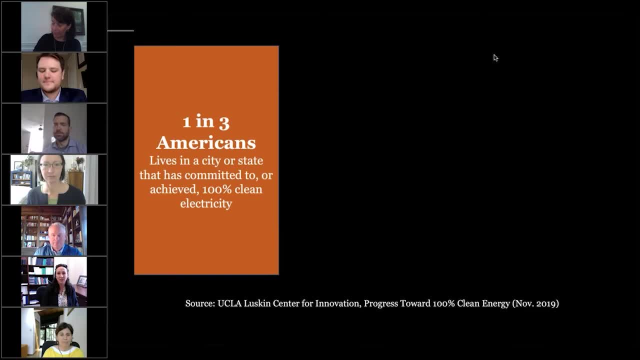 That is not a small number. That's a number from the end of 2019, from a study out of UCLA's Luskin Center, If you look at a timeline which maybe somebody can put up for me. Shelly, I'm happy to try again or I can do it. 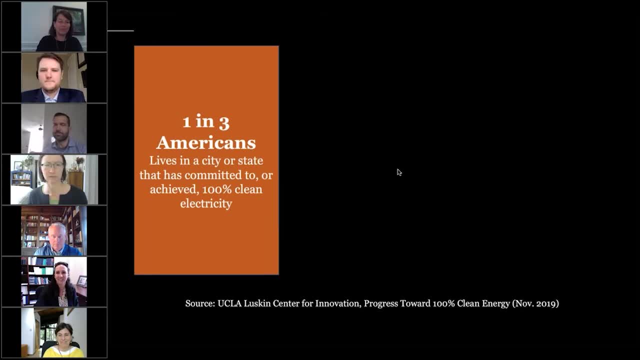 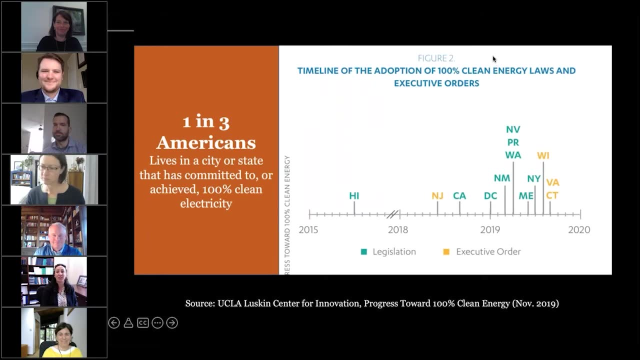 Here, try one more time. Okay, I got nothing still. Okay, all right, Heather, it's all yours. There we go. thank you so much. Okay, if you look at a timeline, this is a trend that's been significantly accelerating. 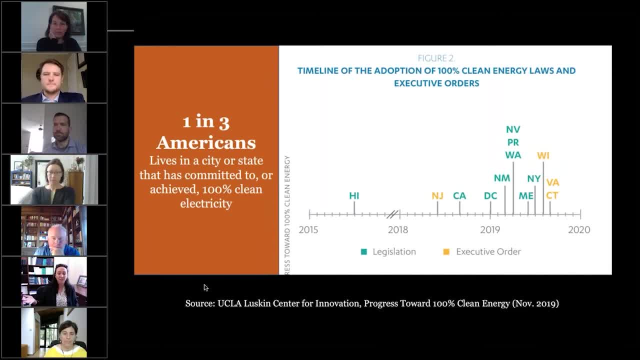 It accelerated a lot, even during the Trump administration, And I'm really thrilled by these numbers because I think it aligns with a lot of my past work and a lot of theories suggesting that democratic engagement and energy policy may actually ultimately help build a more durable national movement. 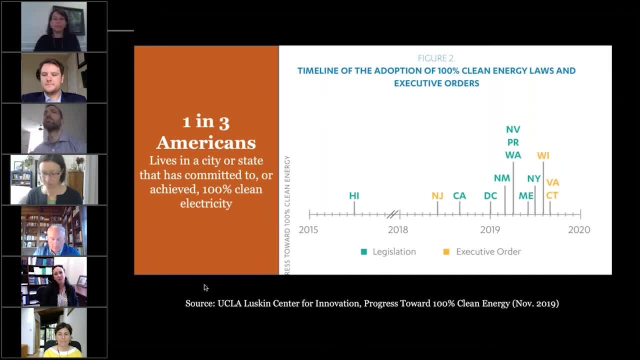 in support of robust action on climate change And under this growing democratic support that we see here, you see companies that are wise to the fact that, at least publicly, they need to display some recognition and acceptance of climate change. You even have the big Southern utilities. 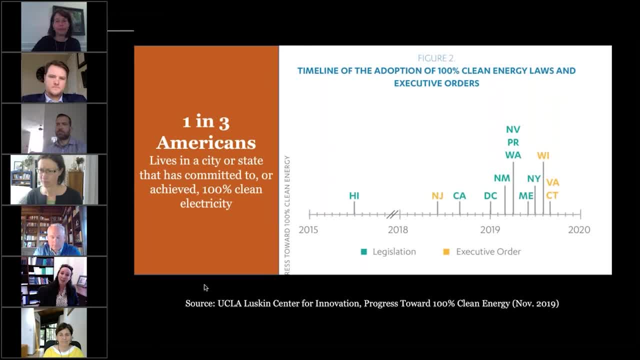 now making net zero pledges, But at the same time, what I argue in this paper is that they're shunting some of their resistance to more technocratic, less scrutinized corners of energy policy, including, as I'm gonna discuss today, grid governance. 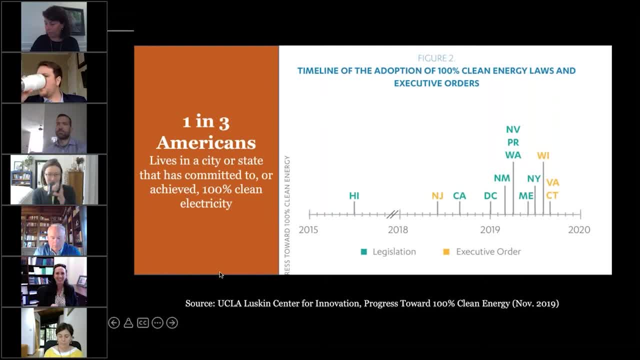 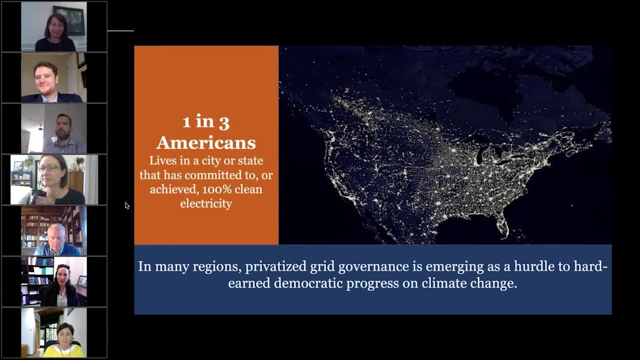 So, Heather, can you hit animate twice please? Yes, great. So the main argument that I wanna make today is that I want us all to be paying attention to climate change and I want us all to be paying a lot more attention to this sort of hyper-technical world of grid governance. 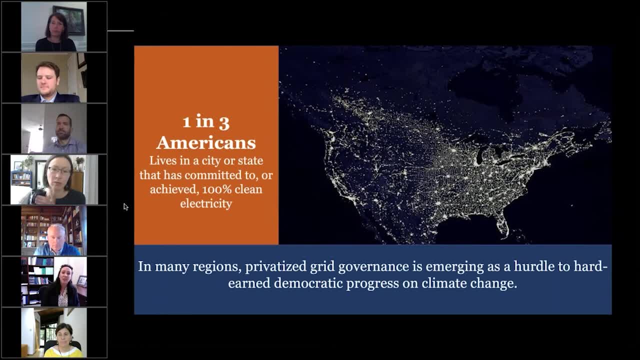 because in many regions, as I argue in this piece, privatized grid governance is emerging as a hurdle to hard-earned democratic progress on climate change, And so I was moved to write this piece by this kind of sense of mounting frustration that there aren't adequate mechanisms of accountability. 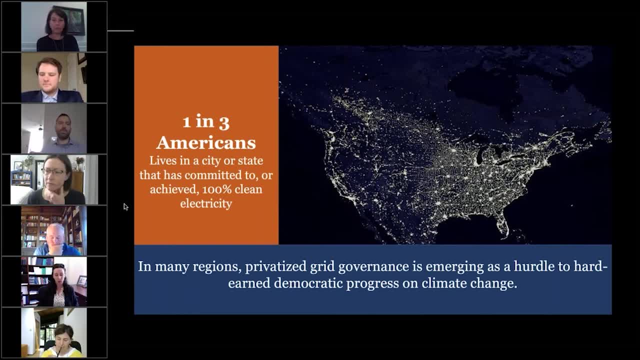 to make private grid governors respect democratically determined climate change policies, And so I'll build through the presentation to a series of suggestions about how we might increase the accountability of grid governance to the public interest. First, though, I have two pieces of background to cover. 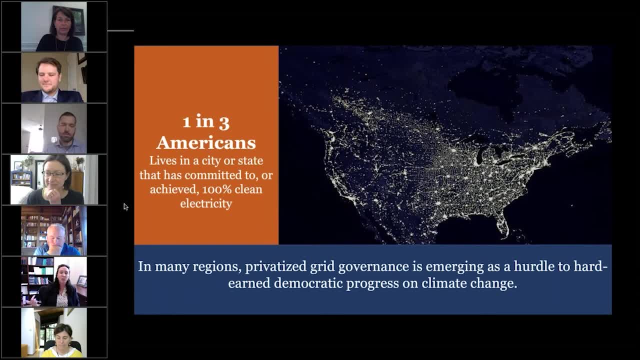 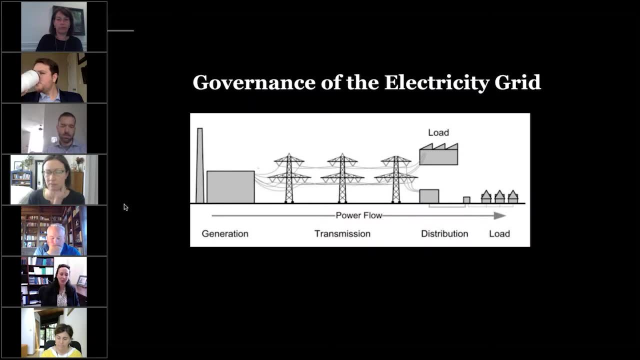 And the first is how the grid is governed. The second is why the electricity system matters so much for climate change. Okay, next slide. So, in terms of how the grid is governed, there's basically three parts to the electricity system that most people that feel the need to tune in for this. 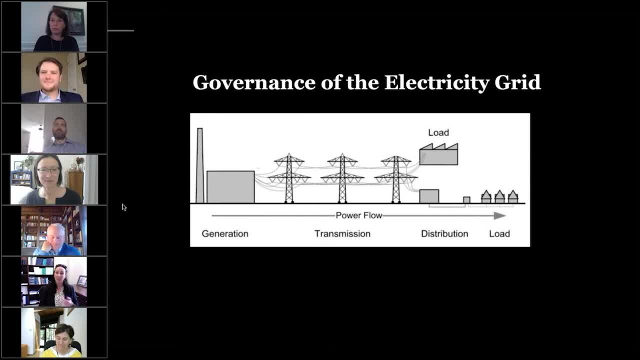 probably already know about, There's generation, making the electricity, transmission, moving it, and distribution, delivering it from utilities to customers, And in the US, the key law that establishes authority over the electricity system is the Federal Power Act of 1935.. 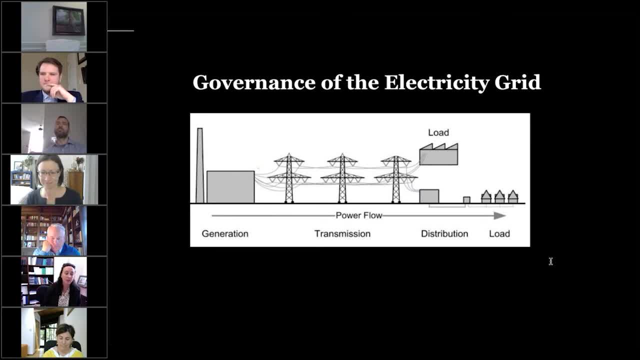 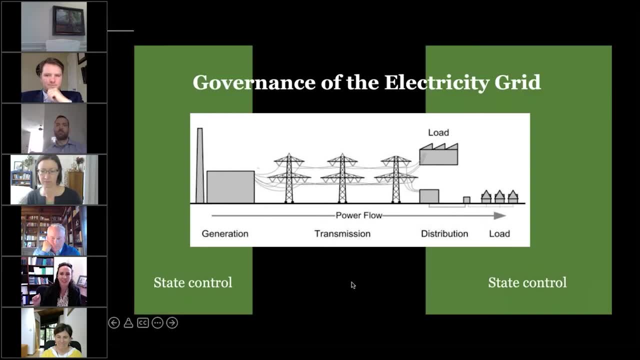 It grants states control over generation and sales and delivery to end-use customers. Heather, will you animate twice to make the green areas come up? Yep, so these areas state control. And then it grants federal control control to FERC, the Federal Energy Regulatory Commission. 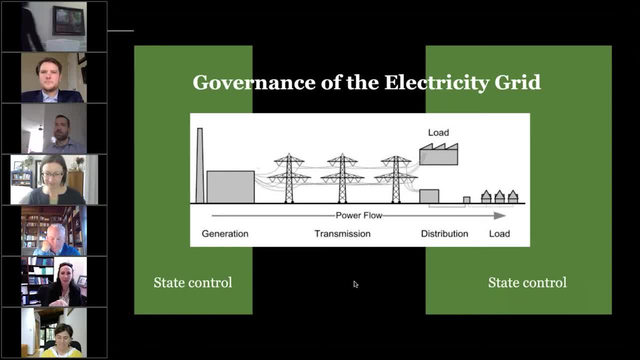 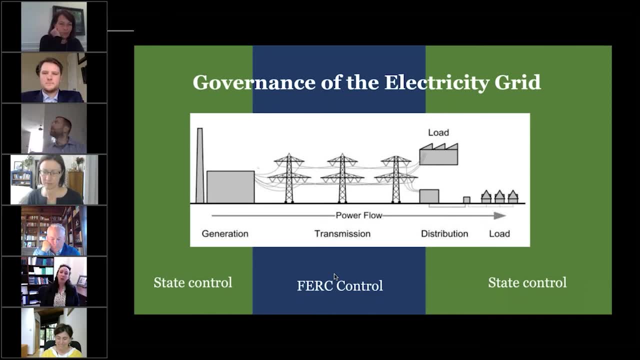 over interstate sales and transmission. So basically, the part that Heather's gonna make blue right now, Yeah, and FERC's job in particular is to ensure that all utilities charge just and reasonable rates for the services that it regulates. Now, traditionally, all of these grid functions. 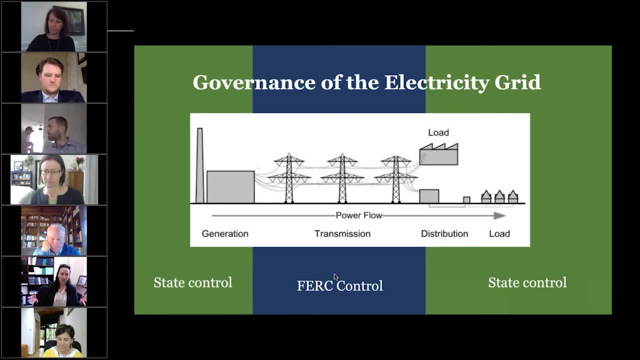 were performed by these individual, vertically integrated utilities that owned the entire system in a single monopoly service territory. But as part of the digital grid, the deregulatory initiatives of the late 20th century, ownership of these resources began to be split apart and many more sales started to occur between utilities. 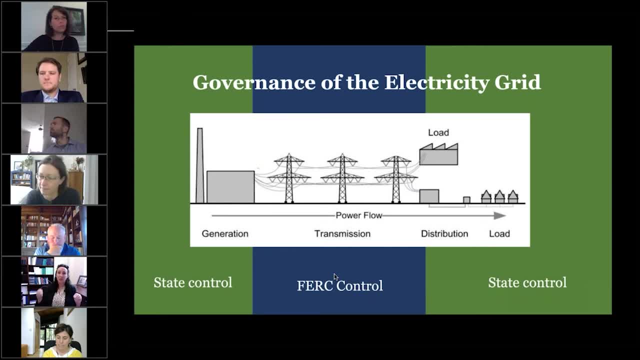 That created the possibility for lots more price discrimination. Basically, utilities would charge other people more to access their lines than they would charge themselves, And so FERC increasingly intervened to ensure non-discriminatory access to the grid. And in the end, I'm gonna make a long story short. 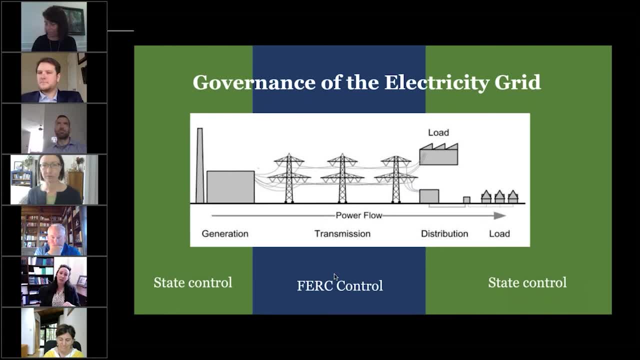 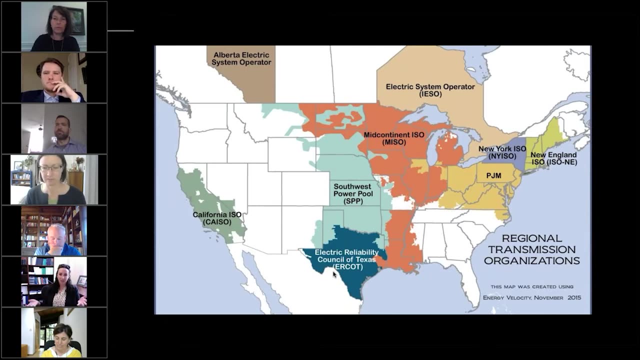 and just say in 2000,. FERC asked all utilities to either create or join what are called Regional Transmission Organizations, or RTOs, to run the grid. Next slide, please. So most regions did what FERC asked. 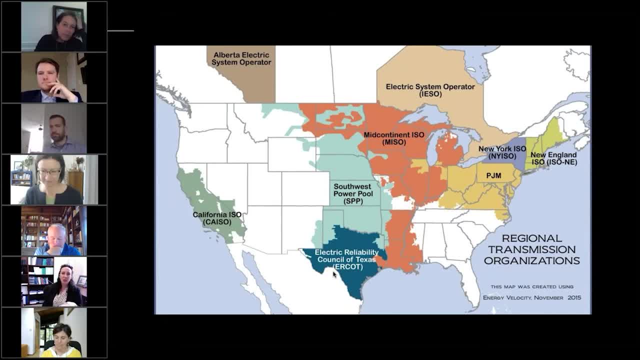 You can see here a map of the RTOs that have formed. A few regions took a big pass on FERC's idea- those areas that are in white. There's some interesting comparisons to make between the areas that didn't join an RTO at all. 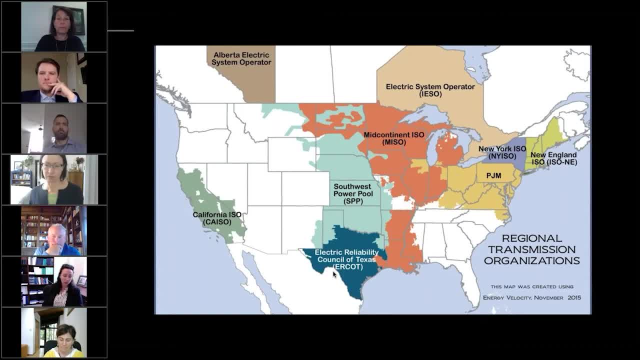 and those that did. I have a different project that's looking at some of those issues, But for now I really want to focus on the two-thirds of the country, as measured by population, that ended up with this RTO structure. I want to focus here primarily. 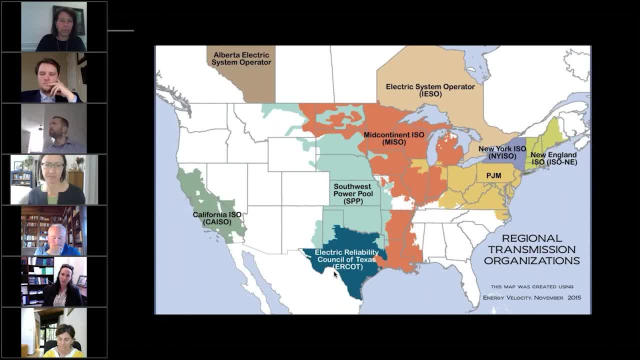 because pretty much everyone agrees that if we're gonna achieve decarbonization we need more regional grid cooperation. And in regions that did create these RTOs, these organizations perform several really important functions. They manage the transmission grid, which means they set rules to make sure. 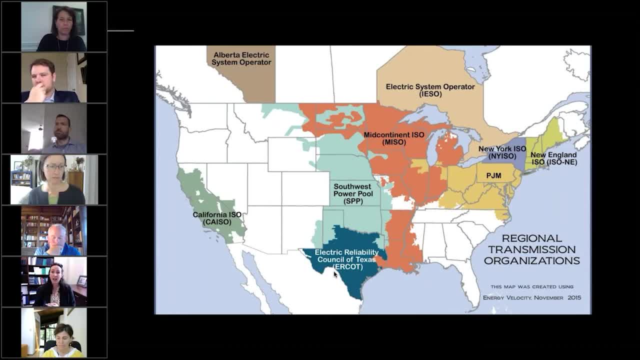 that everyone has fair access, gets compensated appropriately, and they plan and they pay for new transmission infrastructure And they also run a series of markets, including, most centrally, markets for electricity, where generators bid in and utilities buy whatever they need to serve their customers. 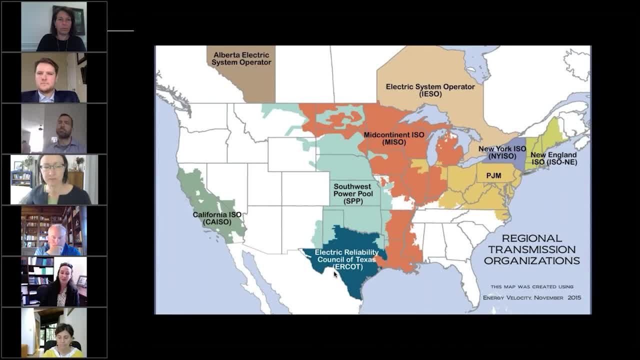 Which means that these RTOs also have to establish rules and policies regarding how energy gets priced and regarding eligibility to participate in these markets. So how do they set these rules? There are a lot of regional divergences here that I'm not gonna go into. 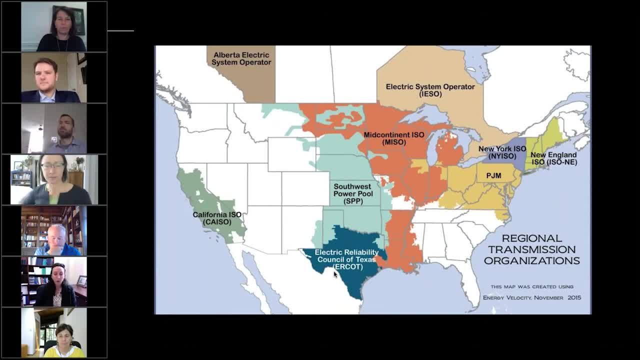 Uniquely, California created its RTO, which is called CAISO as functionally like a state agency. So there's no members, there's a state-appointed board and they make their rules through pretty classic notice and comment rulemaking. 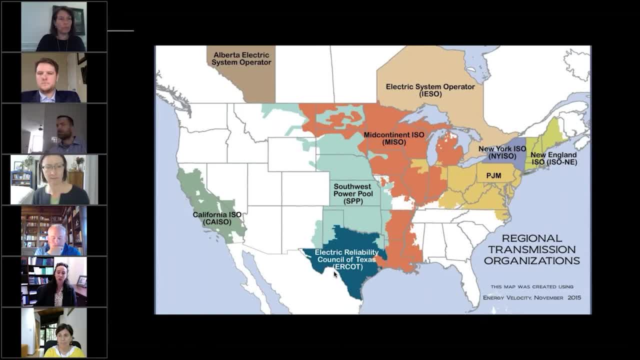 The rest of the RTOs, though, are far more privatized in their structure, So I view that they have many of the hallmarks of new governance or reinventing government theory that was in vogue in the late 90s, when these entities came into being. 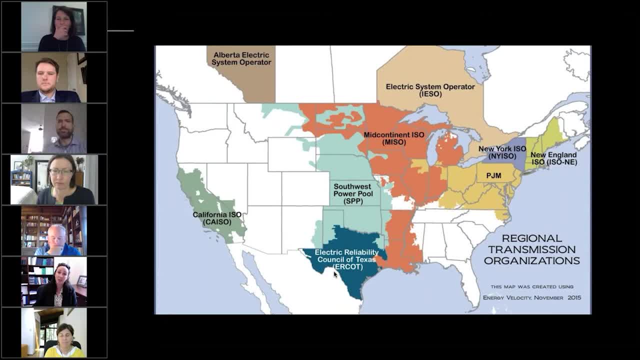 These are not-for-profit voluntary members. these are membership clubs that utilities can choose to join if they want to. They're overseen by board of directors that can't have any financial interests in any members, although they typically are industry insiders, And the rules are established primarily. 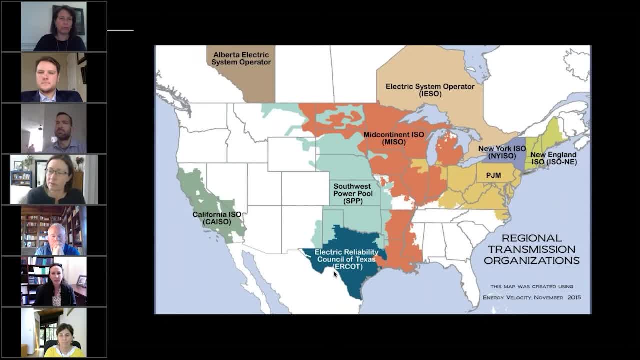 through membership voting processes. So I just wanna give you a flavor of what this looks like in one RTO PJM, which is the largest RTO Heather, will you hit animate maybe twice? Yeah, they use this process in PJM called. 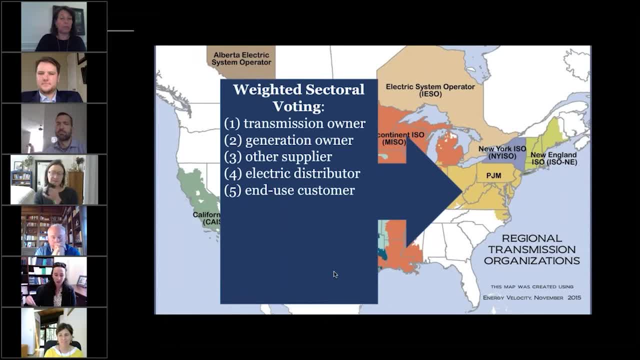 weighted sectoral voting, So each of these five sectors gets 20% of the vote and a proposal has to get a super majority in order to make it through to the board. Heather, will you animate please? And then in all regions for some issues. 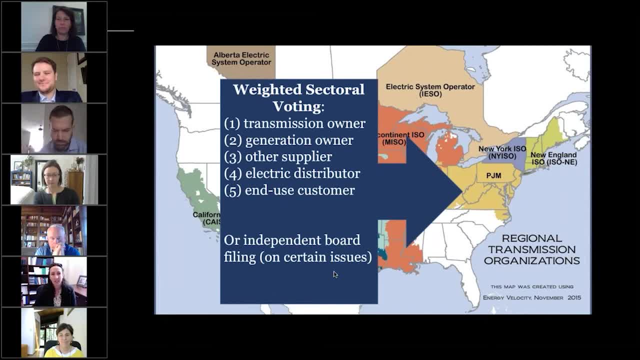 the board can independently approve. for some issues they actually have to get through the membership voting process. So I'll just say I can see why RTOs made a fair amount of sense to FERC in the late 1990s. The industry was kind of tripping. 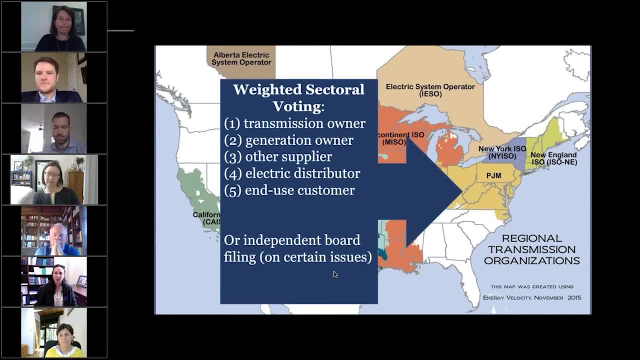 chugging along. There were limited political pressures to change sources of electricity and they seemed like they just needed some rules for reciprocal fair dealing about how to manage the grid. However, in the decades since, there's emerged a definite clash between this privatized 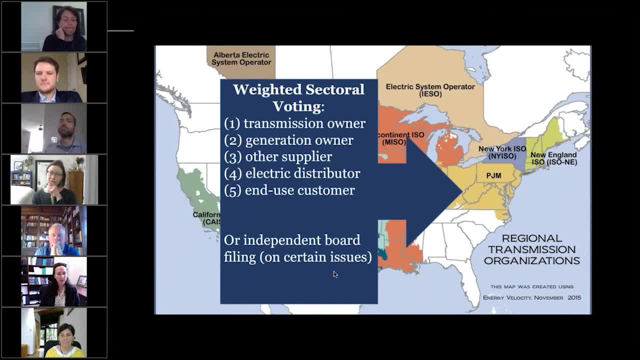 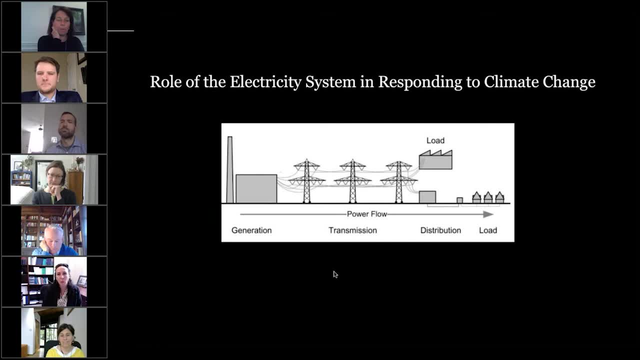 model of grid governance and the climate change challenge. So that brings me to a little bit of background on decarbonization and the grid Next slide. So I want to just talk for a minute about why the grid matters so much for climate change. We're at a critical juncture for responding to 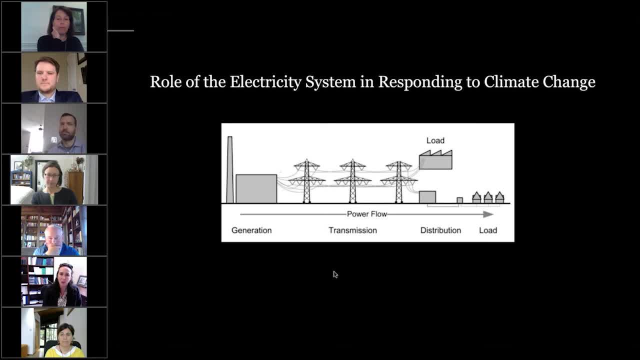 this problem. If we're going to have a plausible shot at keeping warming to non-catastrophic levels, which is still going to pretend catastrophe for plenty of people- leading scientists suggest that over the next 15 years or so, we need to take the electricity system. Heather, will you animate? 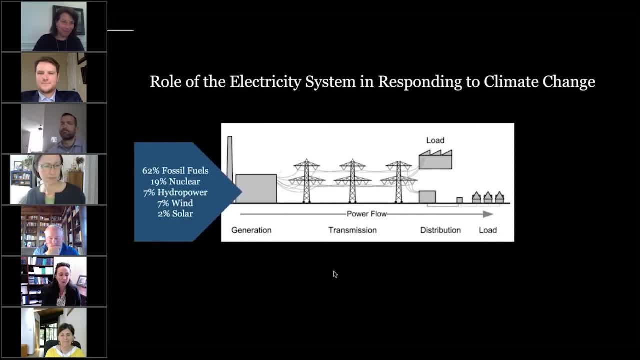 please from over 60 percent fossil fuels to zero percent fossil fuels, at least if we don't have any substantial energy. So we need to take the electricity system and we need to take the services of energy companies. that will also have some substantial advances in carbon capture and 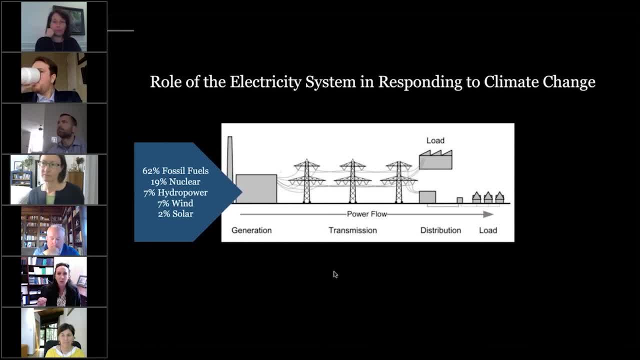 storage, And that's a fact we see reflected in all of those state 100 percent clean energy mandates. States understand what we need to be doing here. Some states do. At the same time, the system needs to integrate a host of new technologies on what's traditionally been thought of as the demand side. 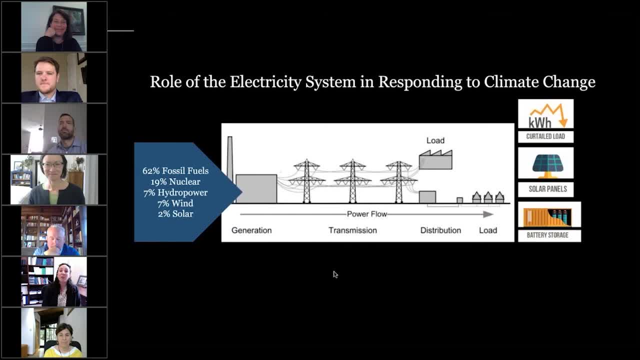 of the system. So, Heather, can you hit four times please? So we need to integrate resources like energy efficiency and demand response, lowering total demand, like small-scale renewable energy- most notably rooftop solar battery storage technologies, which are really increasing substantially their presence on the grid, and electric vehicles. These electric vehicles 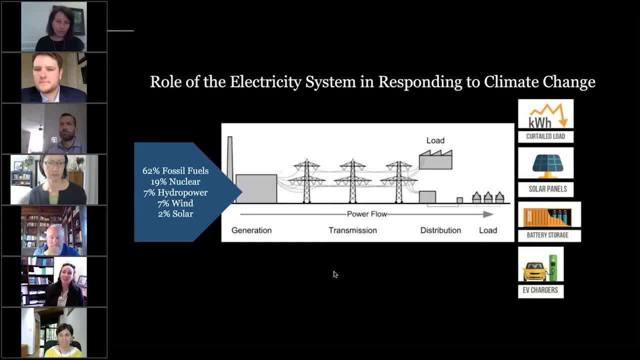 are particularly important and challenging because pretty much everyone agrees that one of the key ways we're going to clean up the transportation sector is to move to electric vehicles, which means that if everyone's plugging their cars in at the same time that we take this, 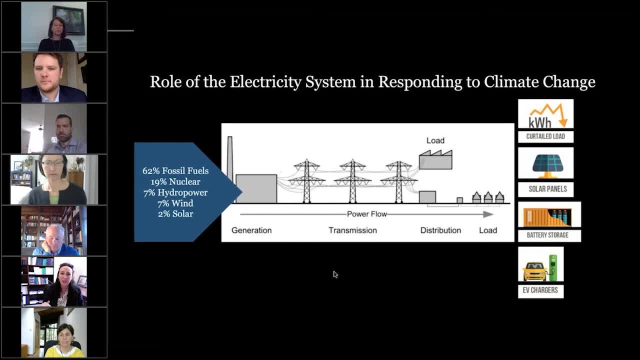 system down to 0% dirty energy, we have to basically- most people think- at least double the size of the grid. So it's a huge challenge that lies ahead and critically important for basically decarbonizing across the economy. So my goal in this project was to forge this link. 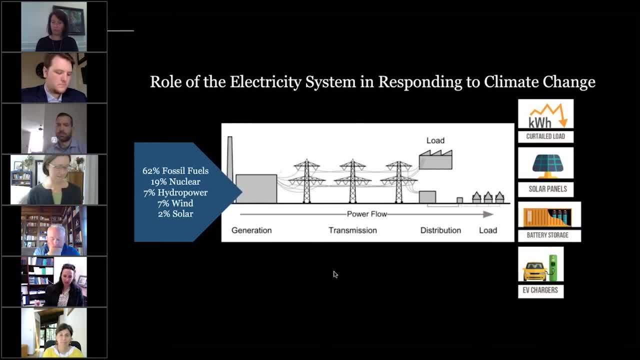 between grid governance and climate change. A lot of scholars are thinking hard about this decarbonization challenge, but there just hasn't been a lot of discussion To date linking decarbonization as a substantive challenge to the governance of the energy system. 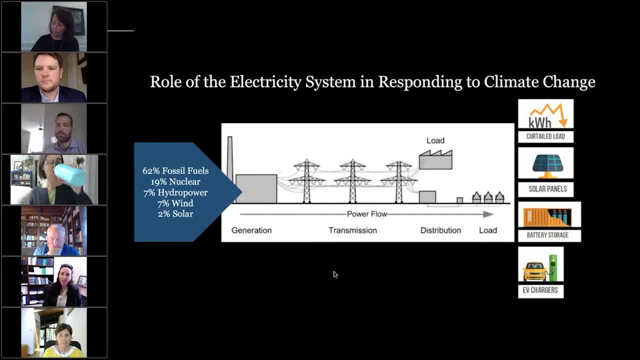 even though pretty much everyone agrees that RTOs are going to have to play a key role in facilitating this transition- And I should just note that as a theoretical matter, there really shouldn't be any clash here- RTOs describe themselves as policy takers in charge of making 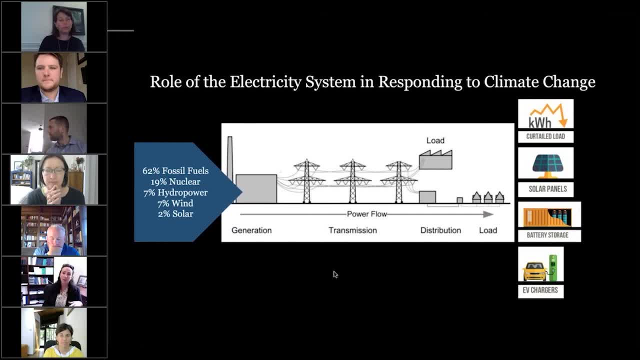 their markets run in light of whatever policy priorities state and federal regulators adopt. But what I suggest in the paper is that's not really how things are going in the era of climate change. So in my project I set out to trace the many ways in which RTOs, as grid governors, are writing rules that disfavor. 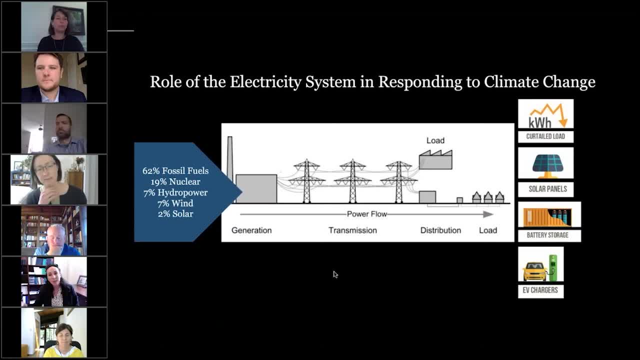 clean energy and favor traditional resources. One set of challenges that I call the heel-dragging challenges really involve a lot of the new resources that are cropping up on that traditional demand side of the system. Here RTOs need to amend their market rules to allow these resources. 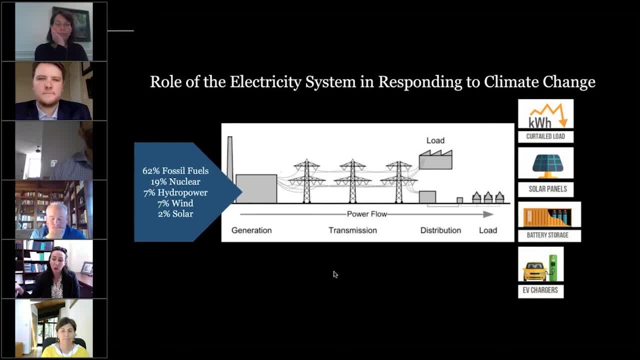 that have characteristics that look pretty different from, say, like a large coal plant, to compete in their markets, But they've been extremely slow to do so, even though a lot of evidence suggests that they would save consumers a considerable amount of money by moving on these issues, And that's because these technologies often threaten the 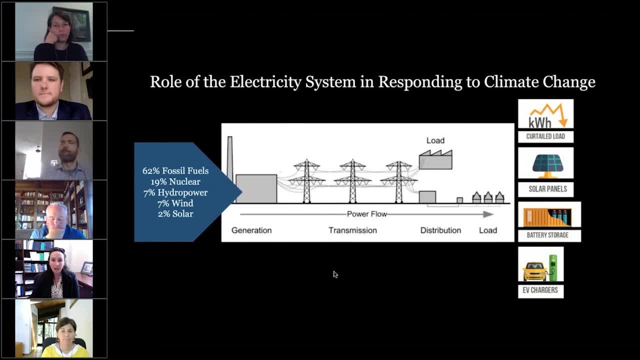 bottom line of incumbent transmission and generation resources, who make their money off of building more supply-side infrastructure. Now, on the supply side of the equation, many incumbent generators within RTOs are none too pleased that states are mandating the aggressive adoption of renewable energy. I think I 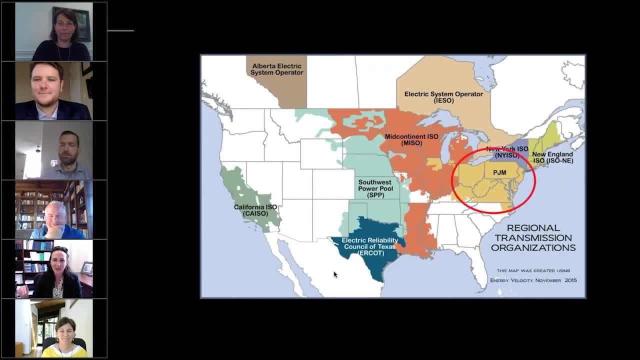 have animation here too. No, just kidding, I don't. Okay. Okay, So states are mandating the aggressive adoption of clean energy which, of course, by adding supply, is going to drive down prices in RTO markets. This is a particular threat to companies with a substantial amount of natural 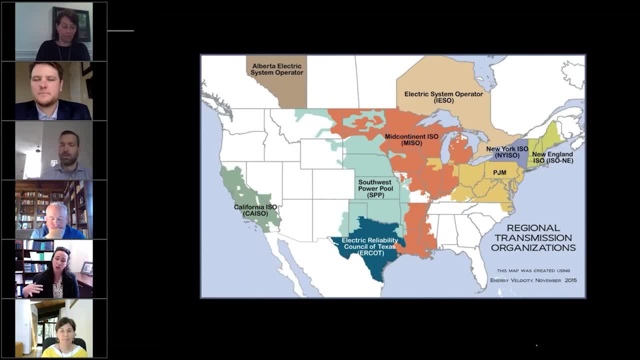 gas resources who've made pretty recent and long-lived infrastructure investments that they're afraid aren't going to take off in the long run if renewables continue their pretty dramatic ascent. So in the past few years this has become a particular problem in two eastern RTOs. Heather, will you hit animate twice? 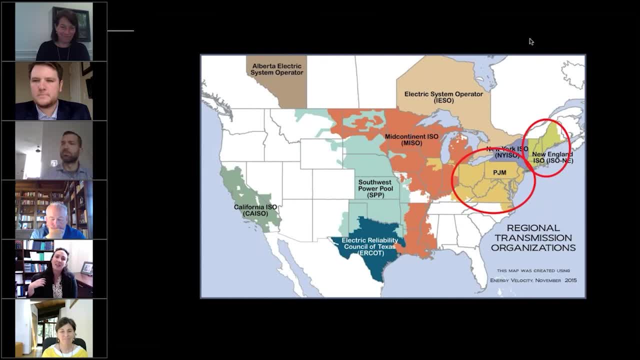 please PJM again and ISO New England. So in these two RTOs incumbent suppliers pushed a series of complex rule changes- and I'm not going to go into the details of in their markets, which essentially made it a lot harder for renewable energy that was supported by state policies to 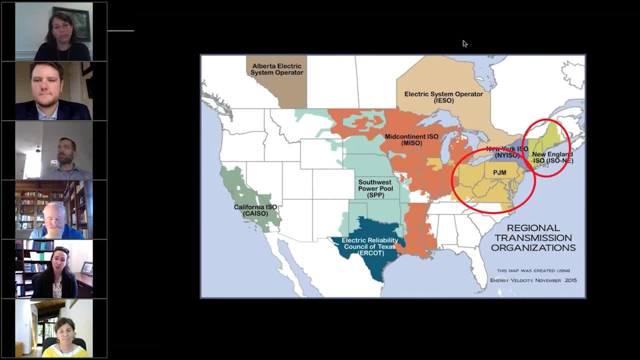 compete with fossil fuels and supply and capacity in these regions. PJM has since walked back this reform. New England still has a legacy of theirs. Now, these changes actually failed to get supermajority support in either of the regions' voting processes, but they came close in both And states in both regions pleaded with. 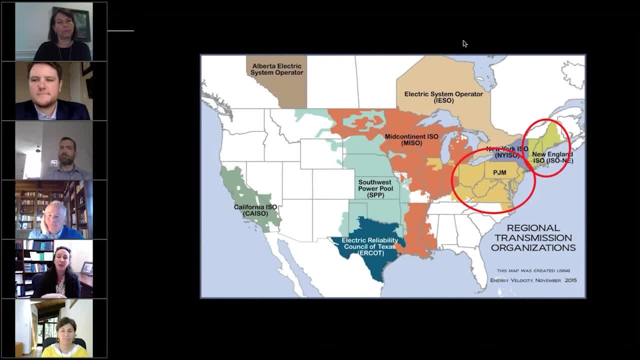 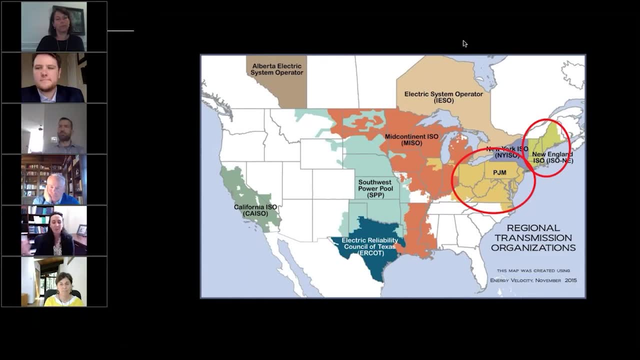 the RTO boards not to undermine their clean energy policies, but the boards filed the changes nevertheless And FERC, under the Trump administration, accepted these revisions on misguided reform but were basically grounded in investor confidence. The result is that private RTO 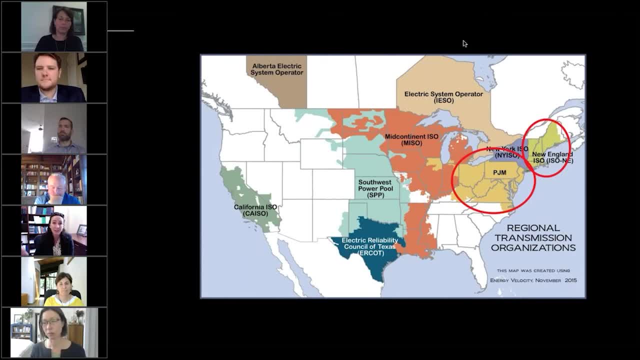 governance processes succeeded in causing consumers to pay probably at least tens of millions of dollars for unneeded polluting fossil fuel generation that states definitely did not want investors to be confident in building. Now a lot of commentators have recognized the perversity of these reforms, not least FERC Commissioner Glick- now Chair Glick- who wrote: 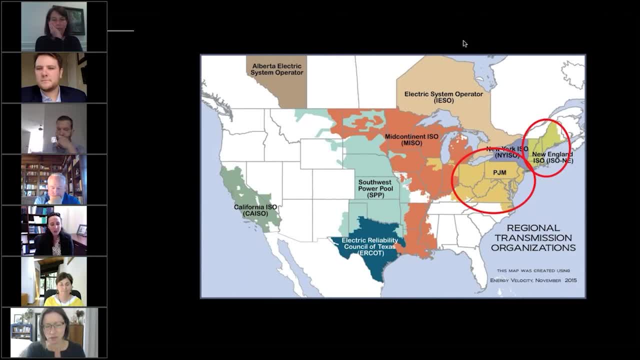 scathing dissents from both the RTOs and the RTOs themselves. Now, the RTOs and the RTOs themselves, as well as the RTOs themselves, did not get the same amount of press coverage. So, Heather. 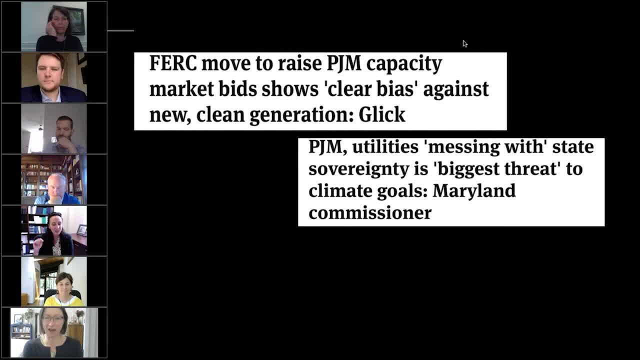 will you put up two more clicks please? So here's two headlines. The first is the December 20th 2019 headline from Chairman Glick. The second is from a Maryland commissioner, basically saying that these reforms were messing with state sovereignty. So it's not like they. 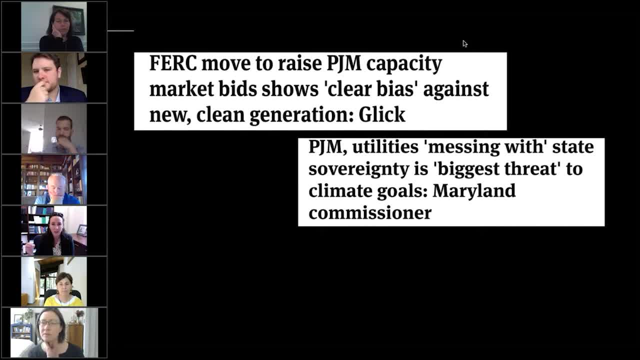 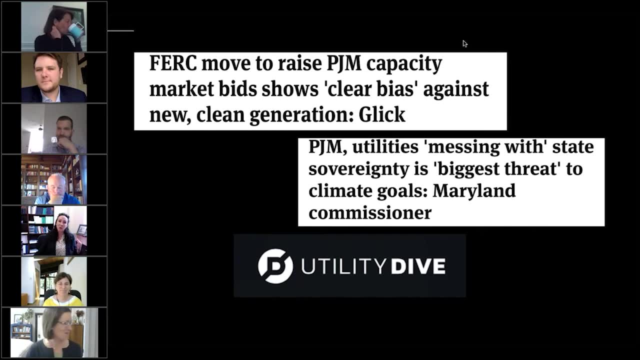 didn't go unnoticed, but here's the most prominent publication that covered these in detail. Can you animate please? I love Utility Dive, Great trade publication, but it's not exactly mainstream media, right. So I think this is a perfect example of a reform that has major impacts. 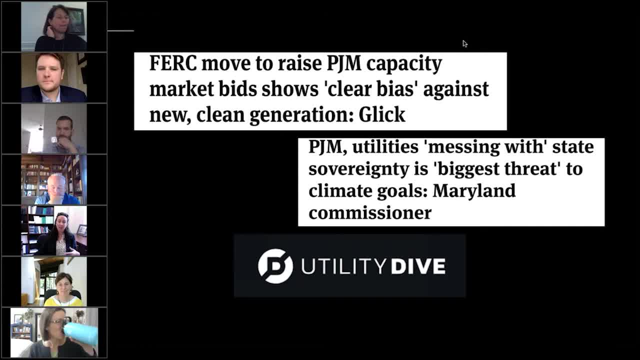 on the clean energy transition happening behind the scenes in these private processes, out of the media spotlight, but with the same effect as a lot of the Trump administration's more public pronouncements about trying to save fossil fuels. So I could point to a bunch of other examples. 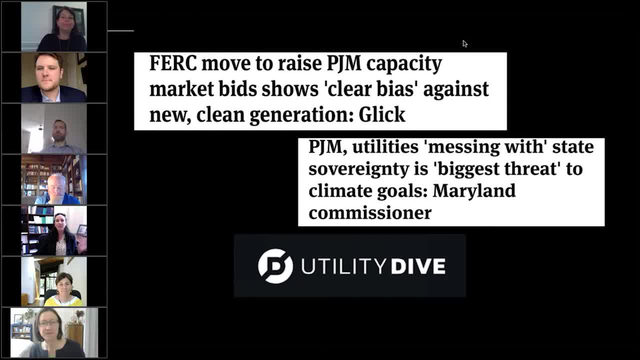 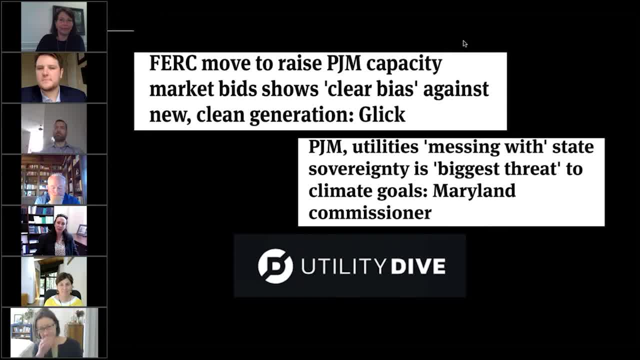 So, as these examples help to illustrate, privatized grid governance is emerging as a threat to progress on clean energy. Whether proposals proceed or fail to proceed through RTO's democratic voting process, or they get passed on by the board after having failed these processes, there's a substantial 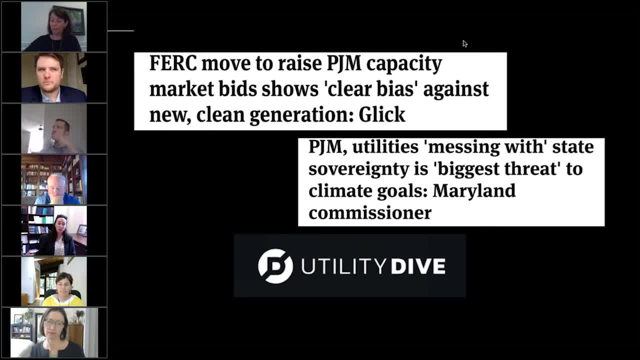 gap in democratic legitimacy and public accountability in RTO governance. The companies that are heard out there, especially outside of law, have started to sort of catalog this, and the main solution proposed to date has been to reform stakeholder processes within RTO's themselves. 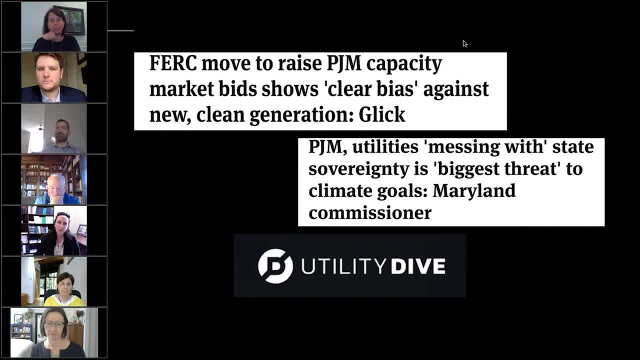 I think this is a totally good idea. I would love to see it happened, but what it ended saying in the piece is that I think this is probably too anemic of a solution in the long run. right, The problem here is that private governance by incumbent industry members just doesn't. 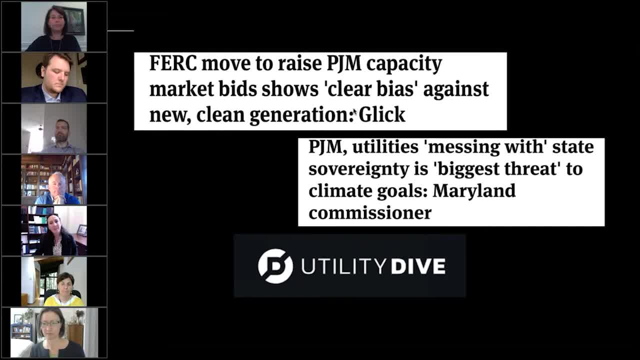 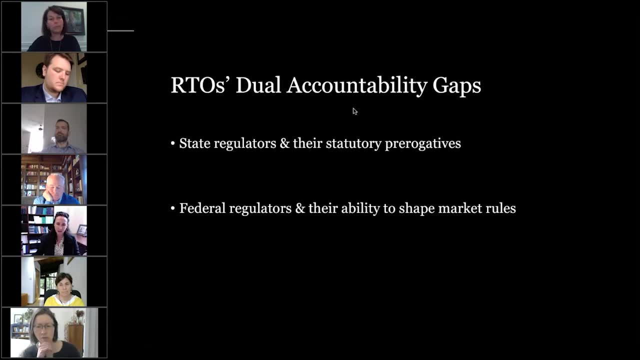 really make sense needs to transform. So, as I see it, the problem with RTOs is really one of two public-private accountability gaps- Heather, next slide, please- One between states and RTOs and one between FERC and RTOs. So I'll just say a word about each of these and then offer a few suggestions. 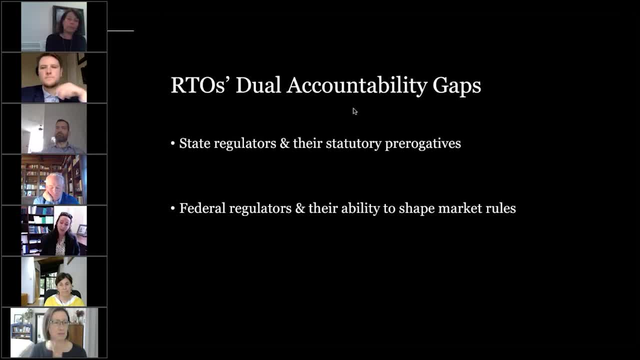 So states, by statute, have control over their generation mix, but RTOs are often not working as partners to help them exercise that control, And in part that's because states themselves have very little voice within RTOs, Although regional state committees exist in every RTO. 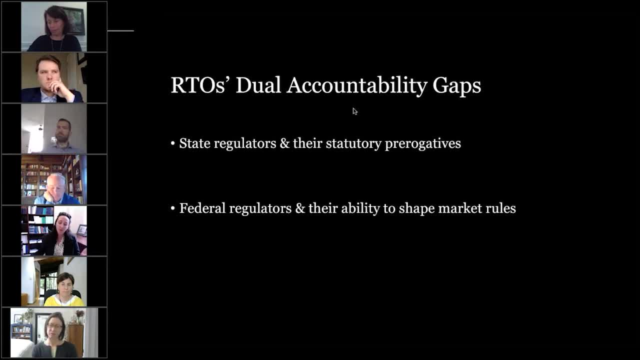 they typically are relegated to kind of a weak advisory role. Second accountability gap is between FERC and RTOs. So one fair argument here might be that FERC approved all of the changes that I'm complaining about. It's FERC's fault And in part, I do think particularly under the 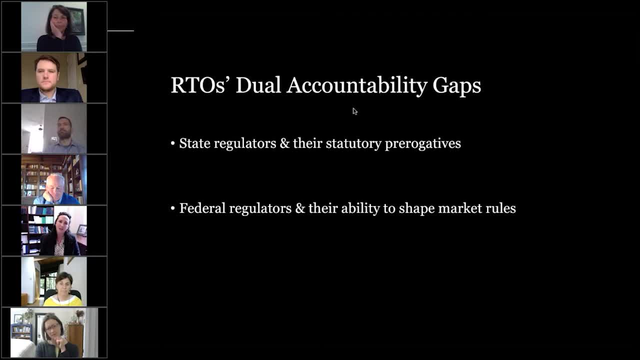 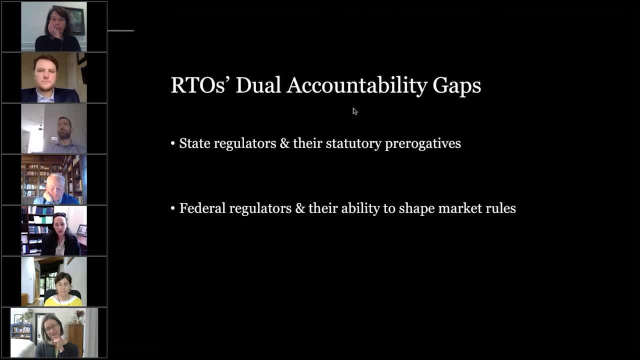 a much more politicized, But I actually think the private structure of RTOs facilitates this kind of accountability gap across administrations, And that's because when FERC created RTOs, it was using this old statute, So it's used its old authority to regulate these as normal. 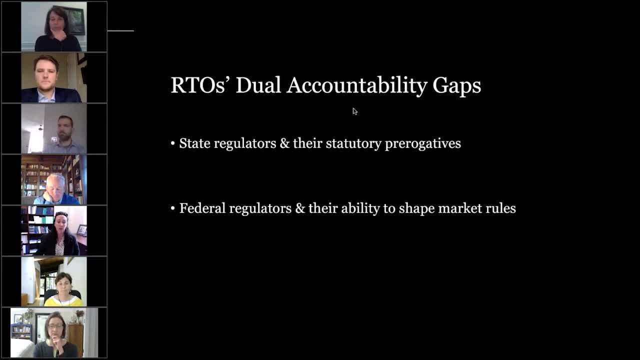 public utilities under the act. And what the law tells FERC is that it has to be passive and reactive in this role and can only force changes in practices if current practices are entirely outside the zone of reasonableness. That's a framework that looks. 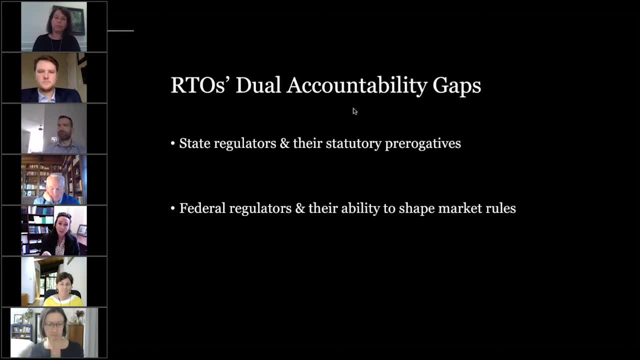 really different from the typical way that agencies operate right. The Chevron framework typically lets agencies pick their preferred policy solution and requires courts to defer. This is really a much more cabined role for the regulator that we've created in the current legal framework. That makes it hard for FERC to force beneficial changes, even when the agency wants. 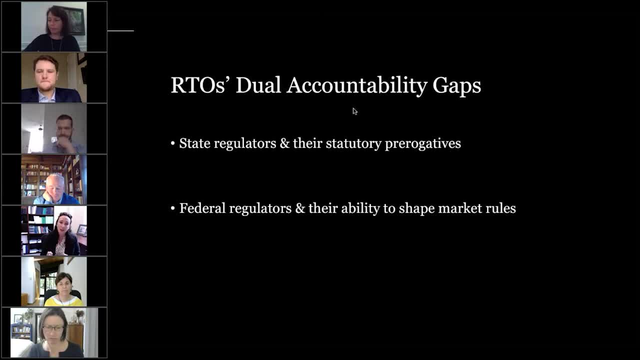 to be proactive And it gives commissioners that are sympathetic to incumbent interests a lot of cover to sort of passively and reactively accept biased rule revisions. So that brings me to a couple ideas for solutions. There's a lot of excitement about the powers that a Biden FERC 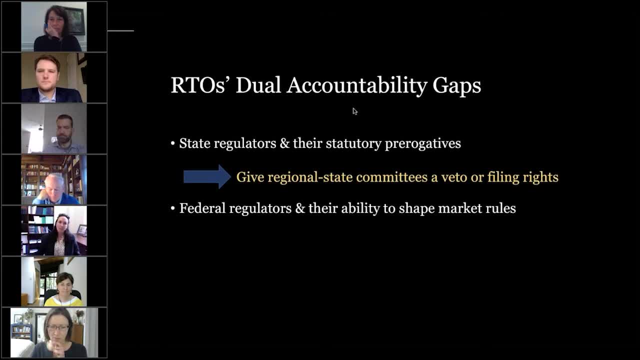 might have to fight climate change, And the commission's already making some really good strides on substantive reforms in this regard. But one of the key reasons that I engaged in this project was to make the case that governance reforms, even though they're tedious and less sexy. 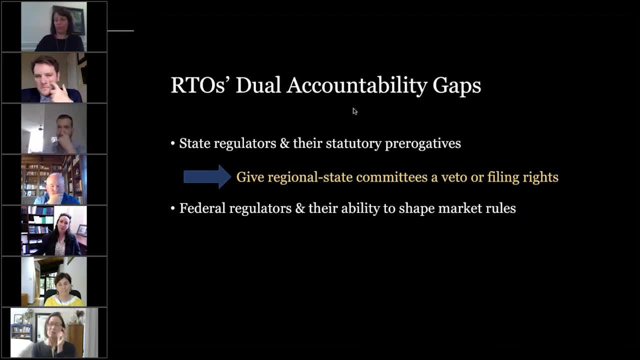 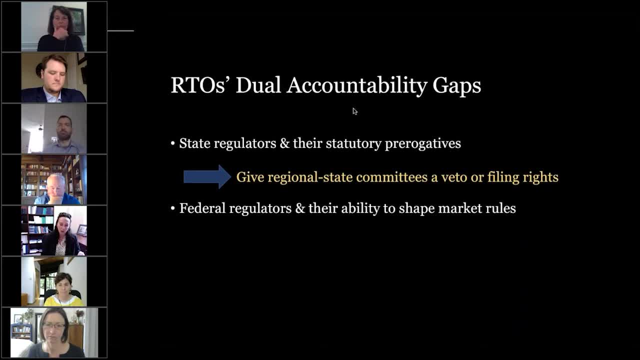 though, is because renewable energy requires a more integrated grid. we cannot just unwind. We've got to figure out a way to make better RTOs, So one option that I've put up here is to give states more control in RTO rulemaking, So a regional state committee could be given a more 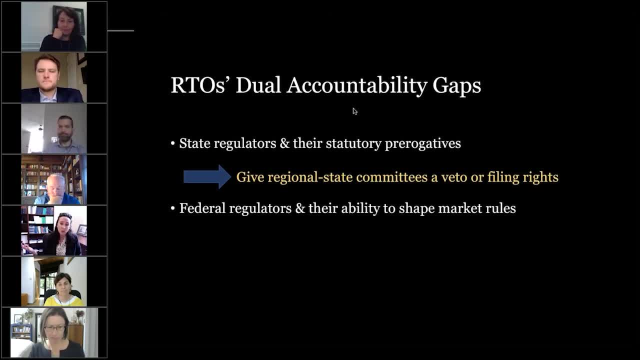 robust role in the process of making sure that we have a more robust rulemaking. So I want to highlight just two options that I've put up here. One is having a federal government vetting process, such as maybe a veto point over proposals that implicate state interests. 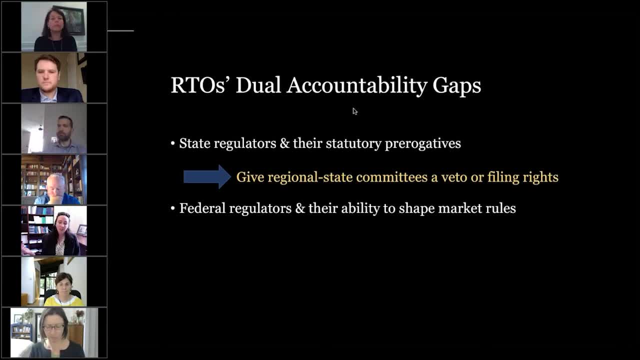 or a right to file computing proposals with FERC. Second policy option- animation- is to stop regulating RTOs as plain old vanilla utilities and recognize them as policymaking bodies, either through a statutory rewrite to give FERC more direct authority, or through FERC deciding to exercise some of its muscle and spend some political capital and 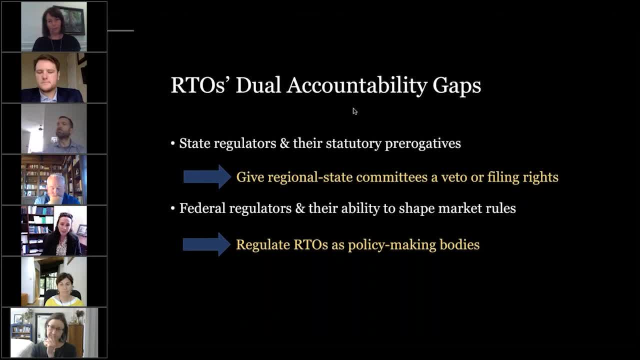 declare that RTOs are unethical, And I think that's a great way to highlight the role of RTOs. governance, as presently conceived, is not producing just and reasonable rates. Finally, I'll just throw out a more radical option that I talked about in the paper, which 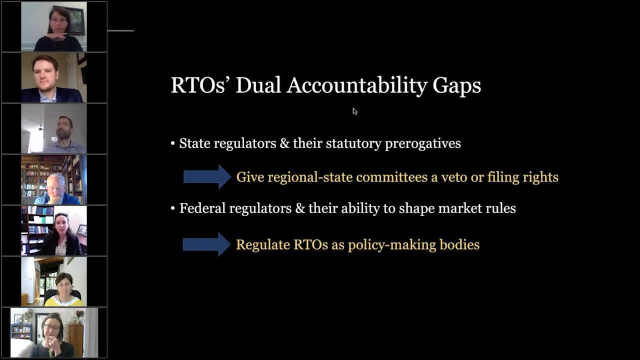 is to consider a more thoroughly public grid. right, You could have public ownership of the grid. You could have agency control over these decisions instead of a private governance model. That would bring the system on a national level closer to the California model, which 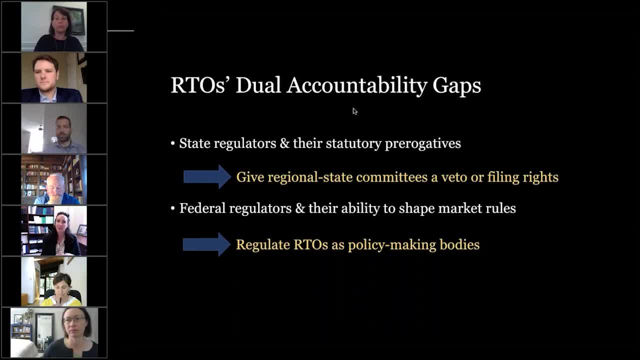 California reports has been pretty important in helping that state achieve robust decarbonization. Now I don't think this final public solution is likely to happen, but we do think it's important to put it out there as a framing point, which is that this system really needs. 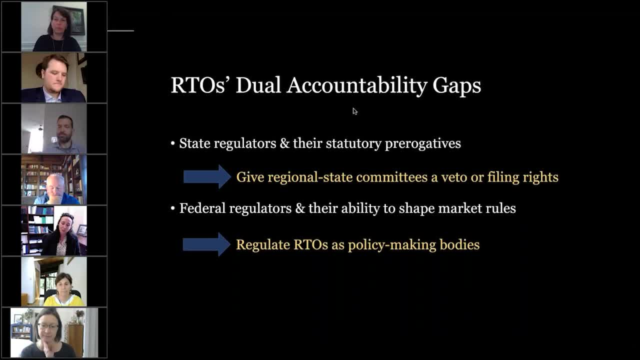 to be made to work for the public in the service of democratically established goals that we have for the future of the grid. So I'll leave it there, Thanks, and I really look forward to your comments. Thank you so much, Shelly. 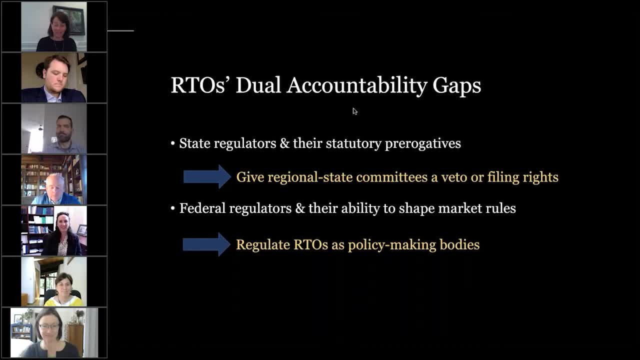 I learned a lot from your article. We had a really interesting discussion in class about it and I just want to say you've totally raised the bar for me On the slides. that animation thing is very cool and I am definitely going to try to. 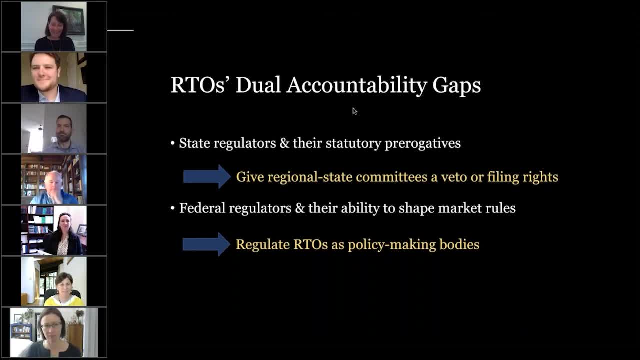 do that now, probably not with as much success. I want to remind everyone that the slides will be posted on the ELI LPAR website and also remind everyone to send questions in now. Don't wait till the end, Just put them in the question box. 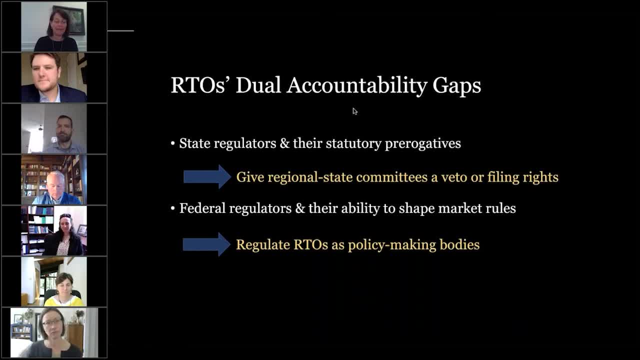 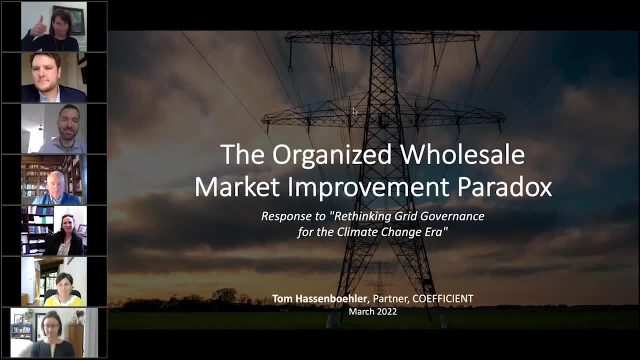 And I think with that we're going to go to our first commenter. Tom, take it away. Okay, Can everybody hear? Can you hear me? Yes, Thank you so much, Shelly and Linda. It's great to be here. 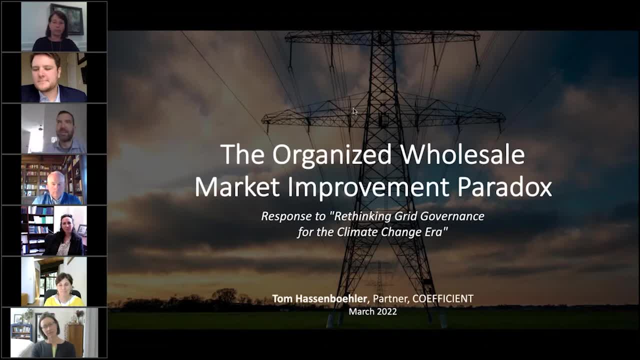 One of the first things I wanted to comment on is just A appreciating how very readable your article is. That's one of the main challenges for this complex topic: just getting people to want to understand and pay attention to the big picture and what's at stake here. 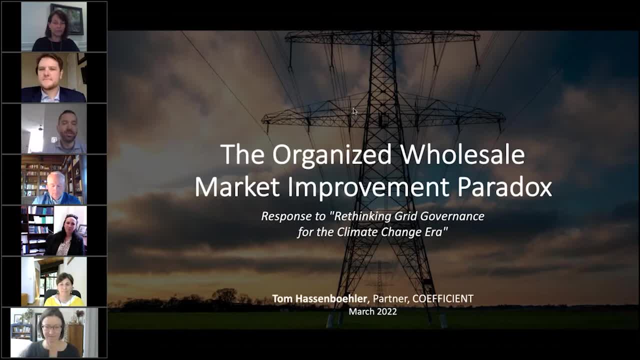 And I think you've done that very nicely. I mean kudos for translating the challenges and the opportunities of our RTOs into something very readable and interesting. So that's just the first kind of comment. To cut right to it, I'm going to make three points that follow just brief introductory. 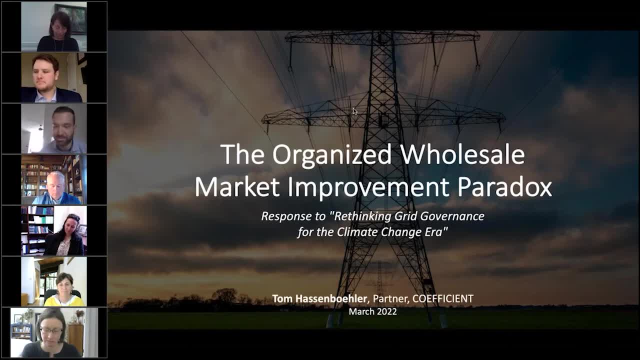 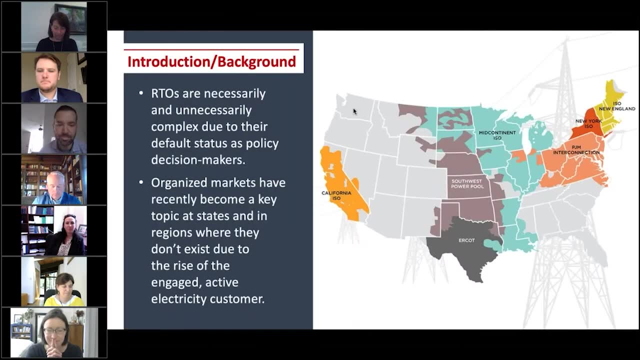 remarks and then move it- and I'll be brief and to the point- And the first and only thing: move to the next slide there. So I'm a late appreciator and supporter of RTOs and what they've achieved over the last. 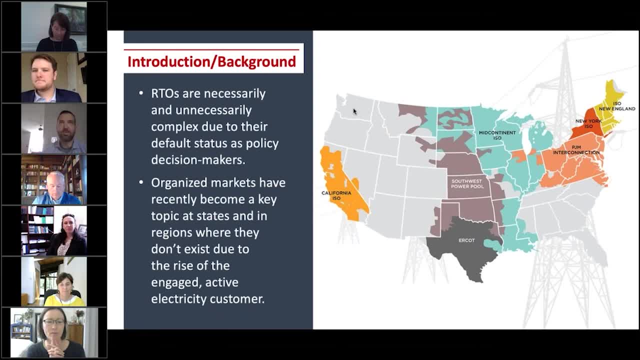 two decades I really, Despite working on Capitol Hill for several years in my early career. it wasn't until my second stint on the Hill, when I came up as chief counsel, that I even really understood what an RTO did, and that should be a little bit unnerving to people. 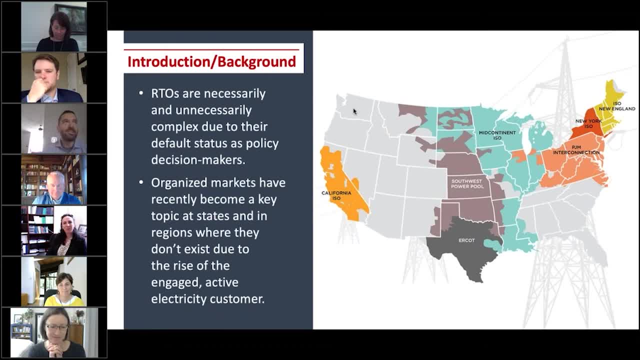 Frankly, it's because this problem and this topic has been really relegated to the FERC experts, the electricity practitioners. A lot of people view it as overly cumbersome, complicated, problematic And they just don't want to engage. And that's a problem. 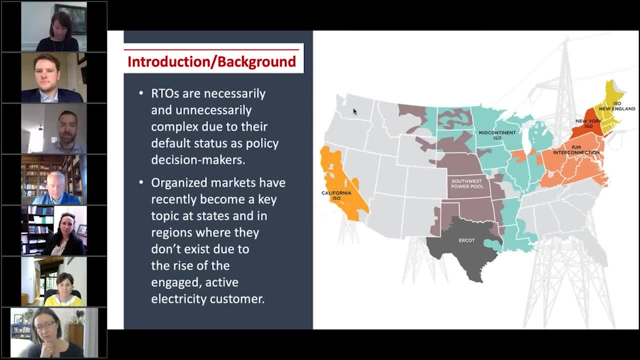 It's a problem because, as I think Shelly rightly points out, this matters on so many levels and it's so vitally important to the future of climate policy, energy policy, security, resiliency- everything that we should care about as a nation. 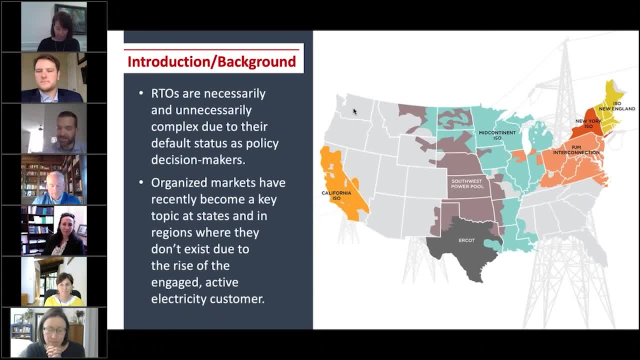 My second kind of Congress used to care. actually, And it was before my time And I think a lot of you are aware- in the late 90s and 2000s, Congress was actively debating these topics. right, You had several bills in the late 90s. 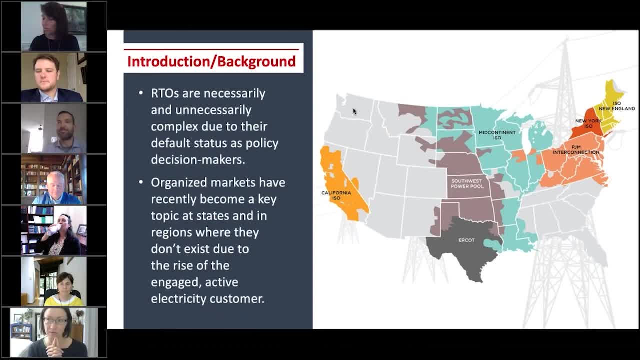 You had of course the fallout from Enron, which kind of stopped and slowed down the rush to competition in the United States Congress and kind of froze everything where it is today. And then we started focusing as a nation on climate policy, The Clean Air Act policy, environmental policy shifted away from electricity policy. 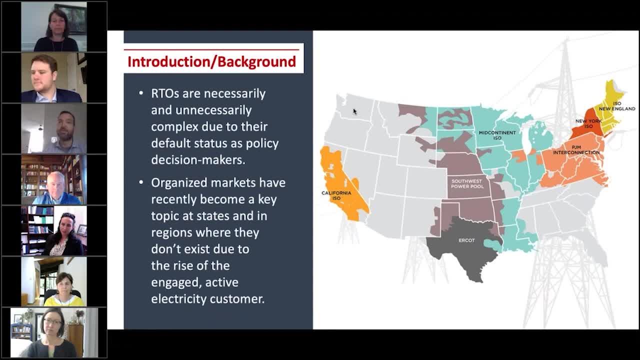 And we didn't really. We lost about a decade of focus on the Hill. My second stint on the career, I did start a series of hearings that I'm very proud of and I encourage you guys who are interested to look at- called Powering America in the. 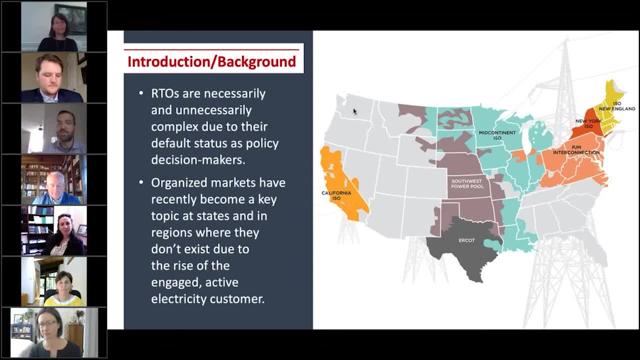 House Energy and Commerce Committee. The hearings ran for two years and they were. What's interesting about it is that they were done completely on the Hill. They were done completely bipartisan. We had the Republicans and Democrats jointly set up the themes, the topics, the witnesses. 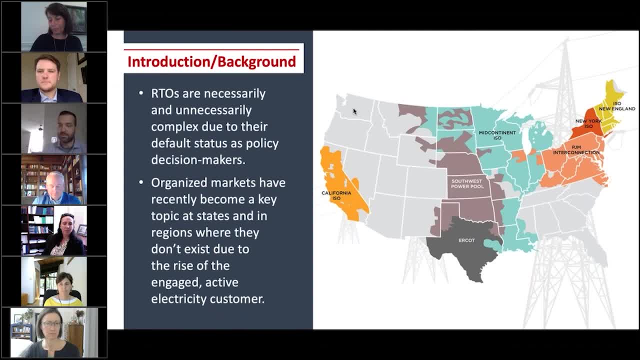 And we did just a series of exploratory hearings on kind of the current status of wholesale markets and their challenges, their opportunities. One of my favorite hearings from that series was one called Consumer-Oriented Perspectives on Improving the Nation's Organized Markets. 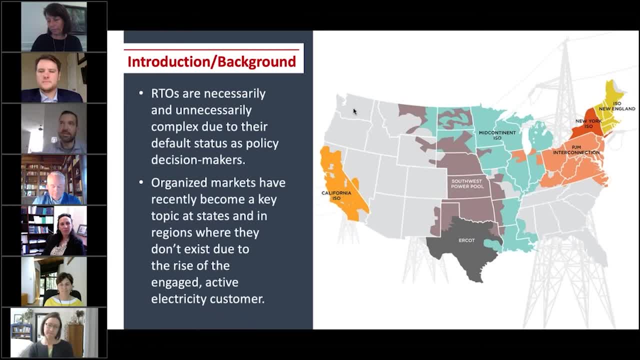 It was kind of the first- It was done in 2015,- but it was the first way And it kind of It kind of inspired my career now- where we brought together kind of the 21st century electricity customer, a big tent evolution from consumer advocates to large industrial. 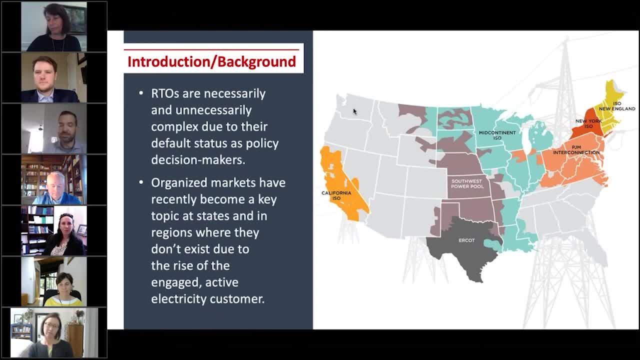 and tech customers to the more active, climate-conscious consumer who really wants to secure clean and increasingly localized electrons. Those active customers were just really not part of the equation two decades ago, when RTOs were first evolving into their current space. It was set up as a platform. 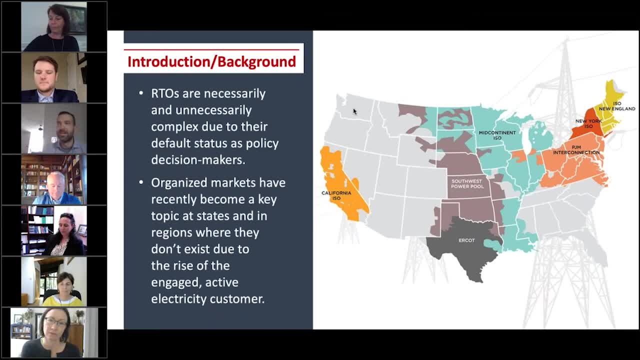 It was set up as a platform. It was a platform for transmission owners and generators to trade and to dispatch in real time and increase economic efficiency, which all of those things made a ton of sense and they were moving in that direction anyway. But now, as the electricity industry evolves, RTOs have become a topic at the state and 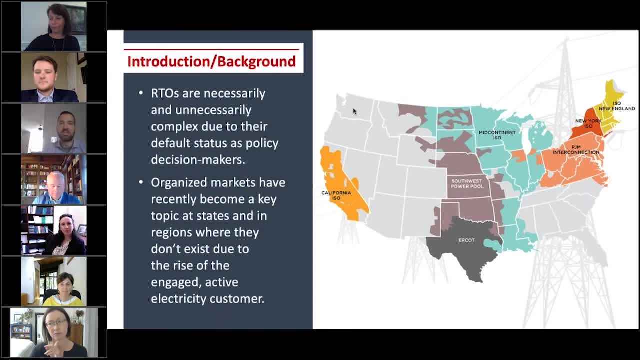 in the regional level again, and that's in no small base. It's no coincidence that it's also paralleling with the rise of this new active electricity customer, And so as part of that- I think you know, Shelly- your article correctly points out: 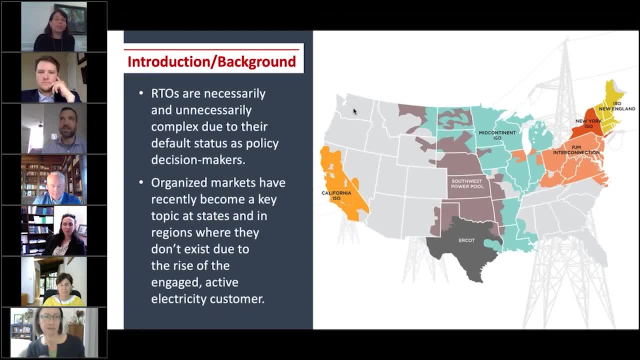 a lot of the flaws and a lot of the challenges and challenges the reader to think a little more comprehensively about ways to improve upon their existing structure. And that rethink really comes at a critical time and opportunity as new configurations of RTOs are actually being considered in those white regions of the country in the Southeast. 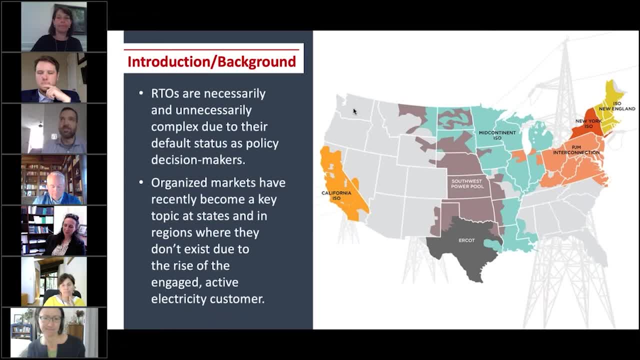 and in the West, And as more engaged efforts are happening in the existing infrastructure and as new RTOs are actually being considered in those white regions of the country in the Southeast and in the West, And as more engaged efforts are happening in the existing infrastructure. 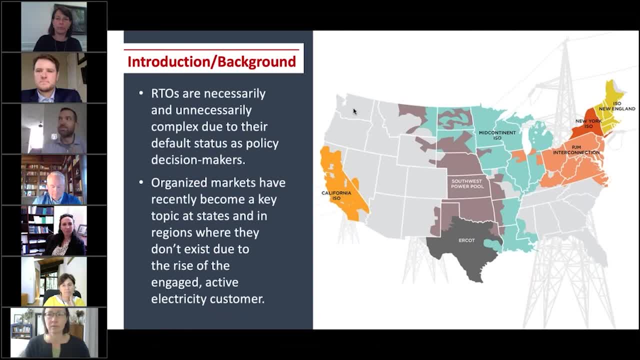 And as more engaged efforts are happening in the existing infrastructure, They're not quite building RTOs, but kind of at a crossroads. there's been a continued release of academic lip of their articles about how RTOs are being transformed and what 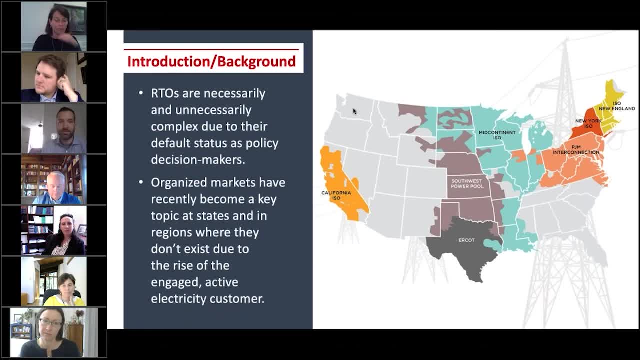 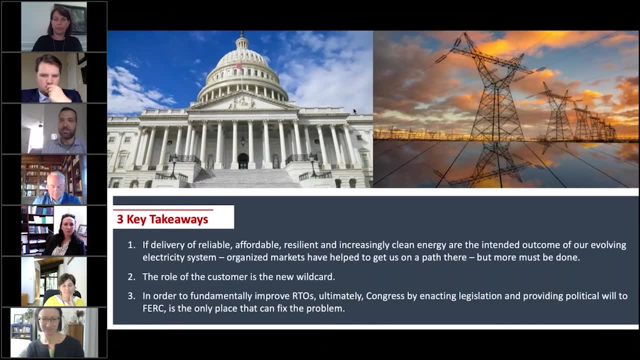 needs to happen, And so I guess we can move to my three points now, which are on the next slide. They're pretty simple, but I think they kind of underpin Shelly's bottom lines here. Exactly, Right, Yeah. 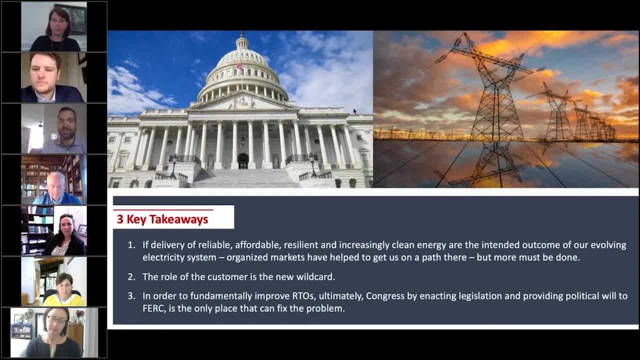 incumbent uh operators who aren't necessarily inclined to push the envelope on technology innovation and change. i think there's been a growing resistance to um keeping the rto model as a as a path for um, this country to kind of build its platform for the future um. i think a 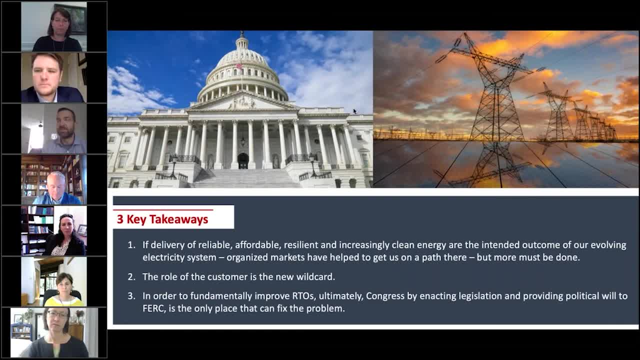 lot. most of the stakeholders um you know, while there's some disagreement in some regions of the country, still um are looking towards improving and and making the rto experience better. so if, if, ultimately delivery and reliable, affordable, resilient and clean are our intended outcomes. i think you know congress has spoken in the past supporting competition and wanting to continue to. 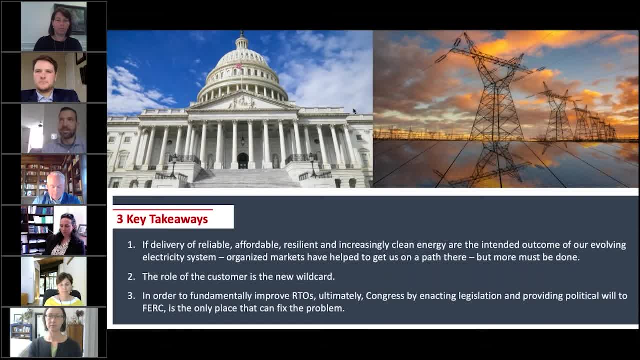 promote it. but i think everyone is in agreement that more must be done to get us there, and markets are far from perfect. they're they are. they are a construct more than a platform for a perfection. everybody wants to get something out of a market that's different, and hence we have a lot of 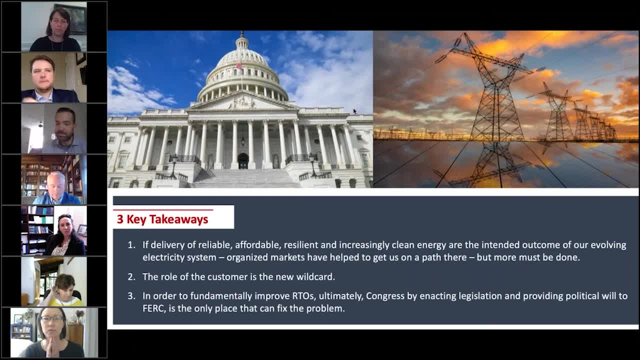 um, you know, problems with how we manage this and and put this together: um, the role of the customer really is the new wild card. you know, exacerbating these developments is you got technology change that outstrip the pace of regulatory and institutional adoption. um, you know, the customers. 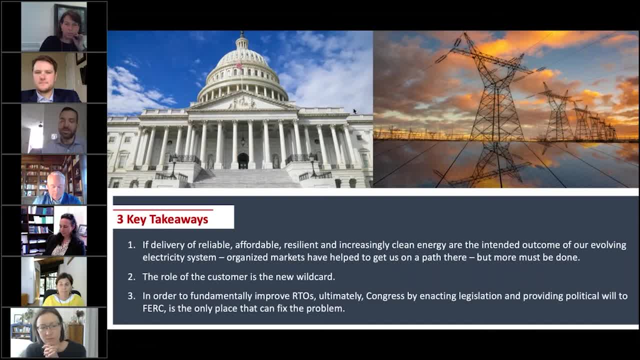 of the rto is one thing was never really supposed to be the customers in the traditional sense. you know, when we look at customers, meaning customers, industrial customers to a residential customer, you know we've done assessments of um, consumer advocates and other customers who don't feel like. 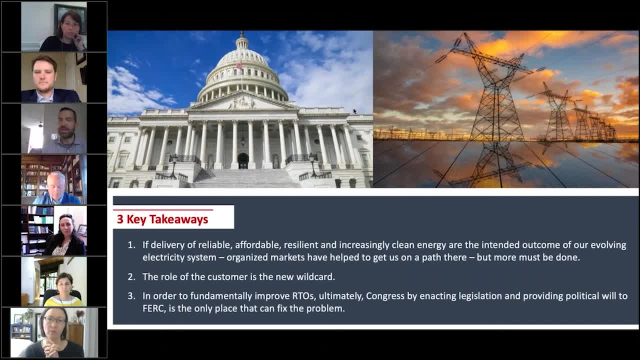 they are the customers of the rts. they ultimately were set up as the transmission arms and i think that's a different paradigm that is shifting fast. as an active, climate conscious customer- whether you're a large tech company who wants to build on-site generation and have 24: 7 clean to a 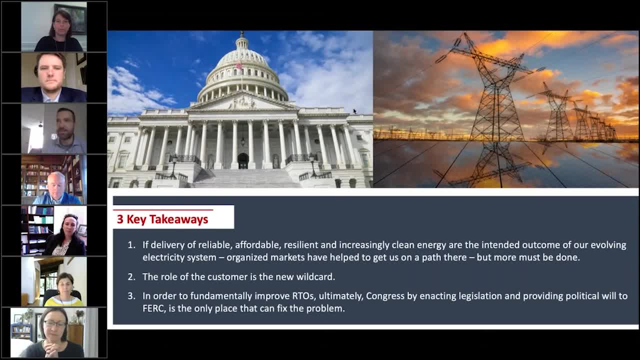 residential customer or municipality who wants to accelerate the transition to clean and, frankly, the- you know, local monopoly utility is not delivering the goods. these platforms are ways to have a functioning market that can actually, um, you know, speed up the process and accelerate the transition, which is why 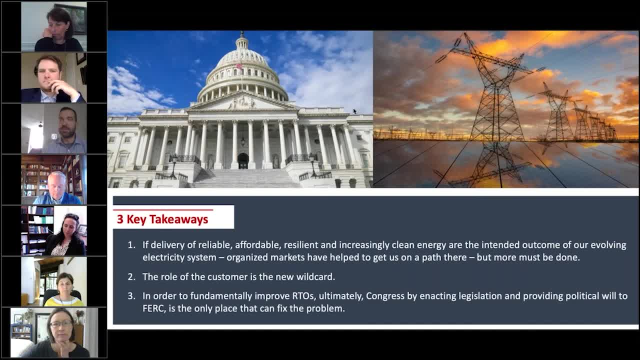 you know, as i think shelley correctly says, most academic stakeholders and clean energy advocates have put their weight behind um, pushing towards an rto and expanding rtos and improving them. so. but all these forces together really have created an extremely difficult confluence of challenges to really harness, govern even the best functioning. 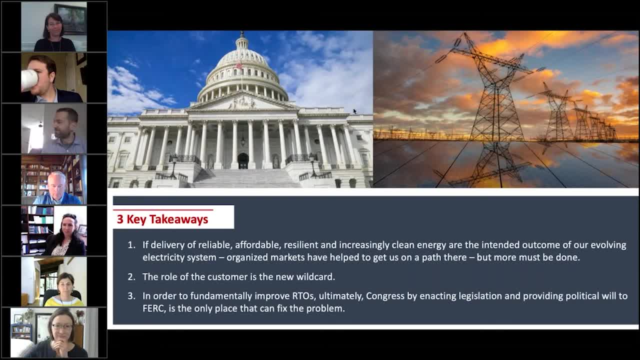 market systems and that's what's going to take. all right problem, those um. that necessitates even more. the final point about congress, and you know obviously i'm going to be a little biased towards congress because most people roll their eyes and say, yeah right, you know, congress is. 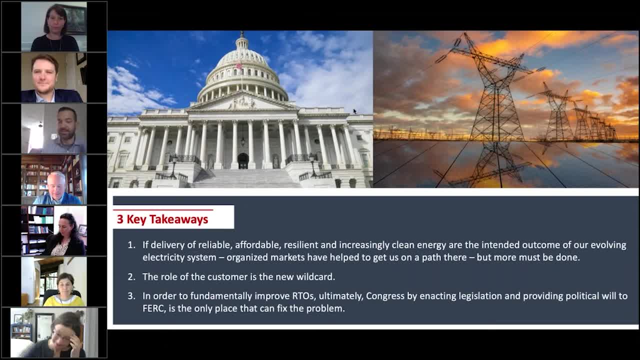 never going to do anything. i i'm going to argue that congress is ultimately the only place that can fix this problem, like we are in a state where, um, you know, there is no real um, the black boxes that were left to fill voids over the, you know, over the last several years because of a lack of 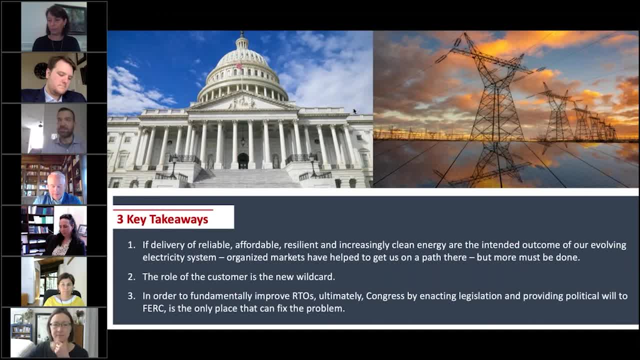 regulatory and political will have just continued to compound on each other over the last two decades to the place where, you know, firk doesn't have even an aggressive perk. you know, chairman click certainly has been aggressive on several things and is supportive of markets. um, there needs to be a greater political will to move the needle on this. 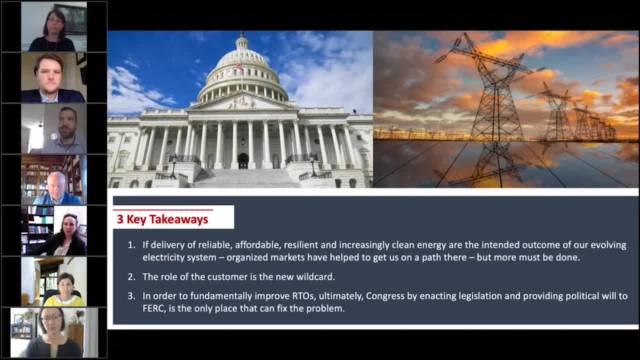 and without that we're going to be stuck with some, you know, uh, next to best, uh, you know solutions that are going to be kind of burbling up from the bottom up. you know, my argument is, the top down really is the only way to do this. now, that doesn't mean we roll over the states and that doesn't mean 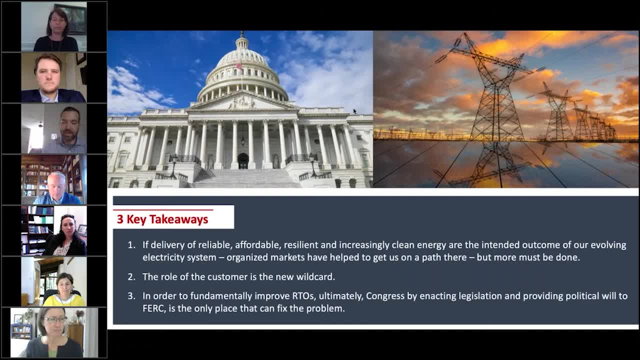 we, the states, are not, not part of this equation. um, i think that the main, one of the main points is that, you know, similar to the highway system, the states need to be part of the players here and we must think bigger about where the status quo has left us. 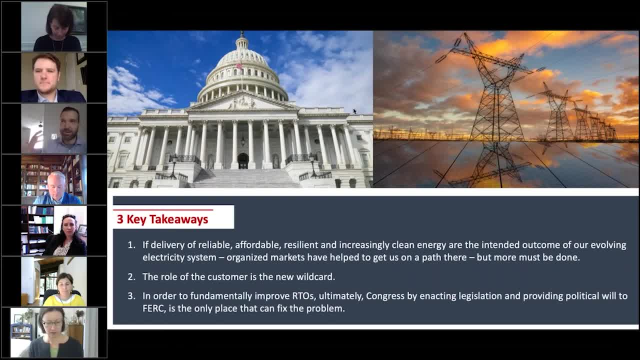 um, you know we're in these regional sandboxes. there's partly due to the physics of the grid, that's partly due to state versus state regional conflict. we have to think about how the grid- you know that was built in a different era- should run more like the interstate system, with 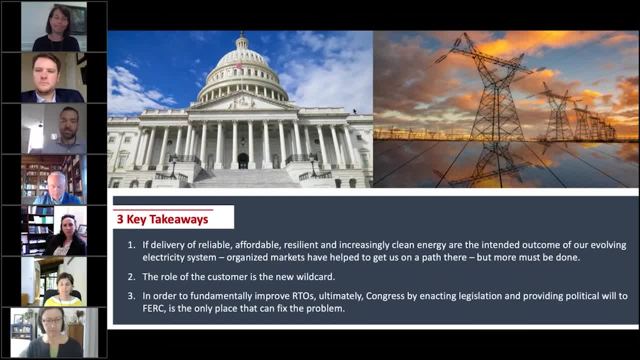 the free flow of electrons across state lines and increasingly being generated behind the meter, across traditional jurisdictional boundaries, is really going to change the paradigm for the future and that really the only place to debate that is is congress. uh, you know, congress is vested with the- you know, often forgotten interstate commerce authority that. 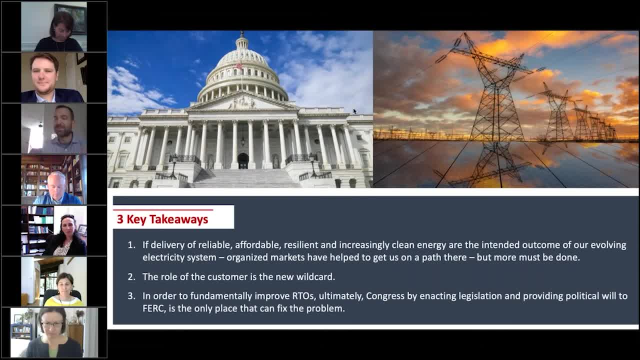 does allow for the creation of the federal power act in the first place. and, uh, you know, and, and i think, with the sensitivities towards states right now, there is a lot, rightfully so, there is a lot of hesitation to tackle some of these things, which is why 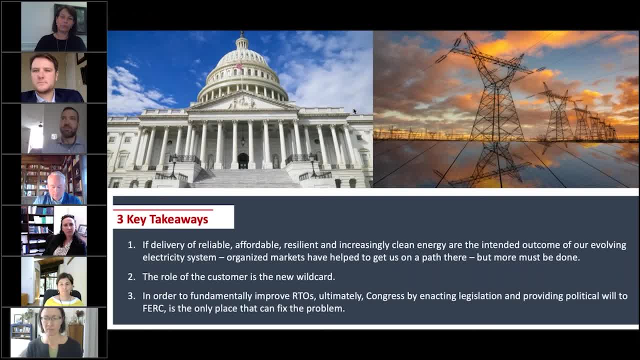 some of the suggestions that are emerging in congress- just to close- are very promising. the good work that we did at the committee five years ago hasn't been lost. in fact, you know there's several uh folks in congress currently that want to continue the uh shift and move towards just um. 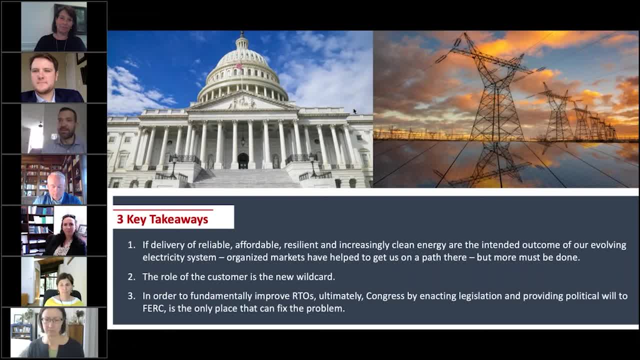 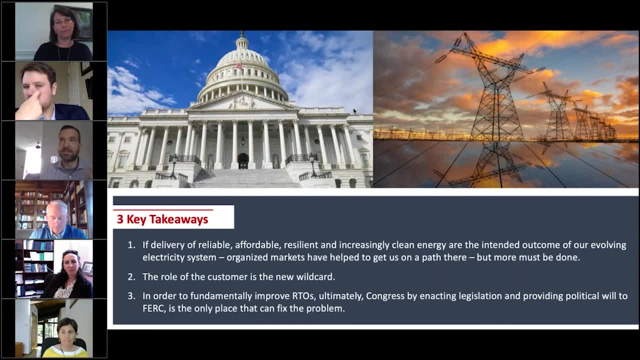 solutions. uh, senator markey has just recently introduced a bill that takes a comprehensive look at some of the um solutions for the grid of the future. one of them very relevant to this and we've worked on, is setting up a faq style advisory committee, like taking these issues outside of. 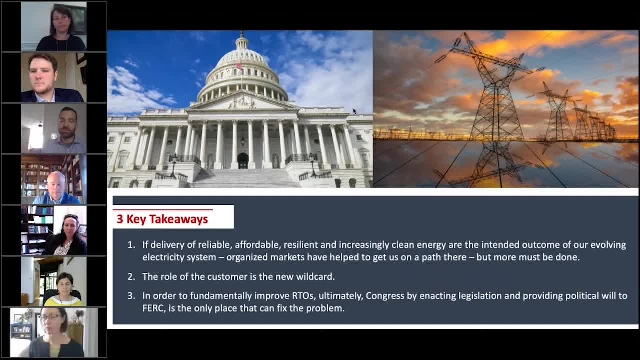 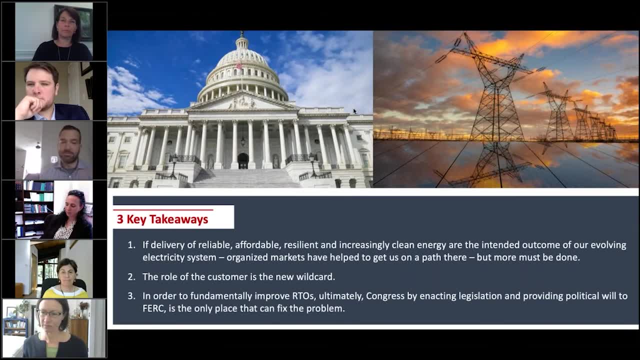 brook outside of the rtos and developing a very comprehensive approach to think about some of these solutions and opportunities that shelley um posted in her very you know, good, you know article, you know, ranging from technical fixes to capacity market to you know, should the rtos be completely. 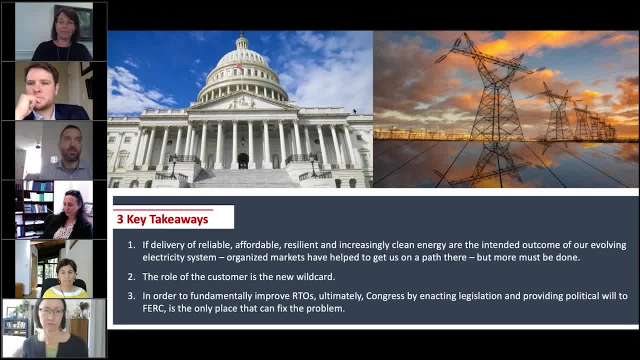 rethought as public institutions. i mean, you know, all of those kind of things could be on the table in that kind of setting. that is not part of a current, you know, FERC technical conference there are. there are some other opportunities for FERC to look at this. order 719 is a very commonly cited 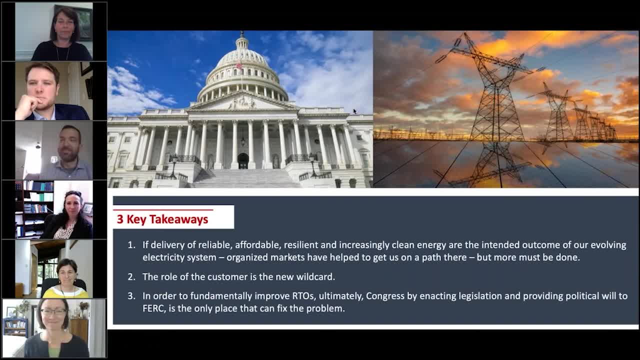 order that i know casey knows well. it will probably mention um that we we have been working on too, and there are some emerging efforts in the house representatives to uh, look, get FERC to revisit that order, which was the last time that FERC took a comprehensive look at stakeholder. 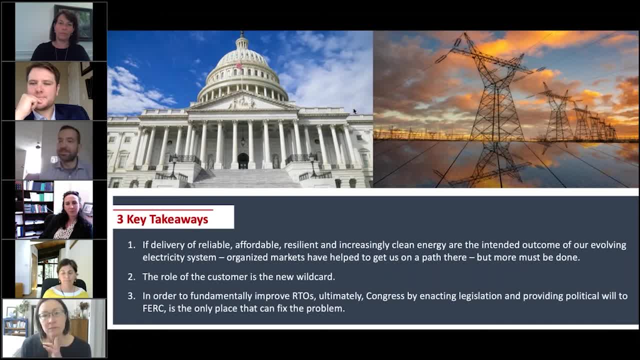 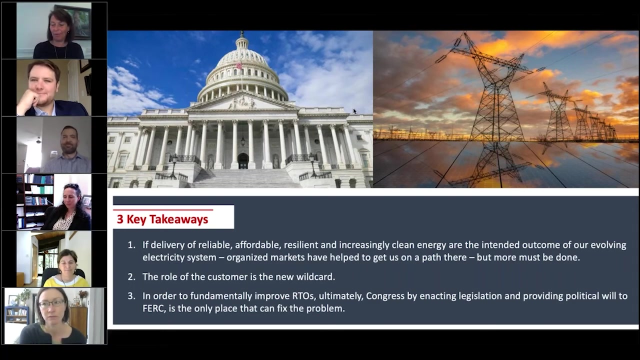 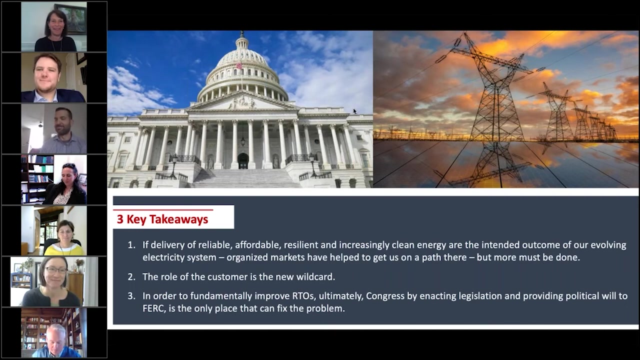 reforms at the rtos. so everybody's focused, let me guess, i guess, on all on here. 47, point two, this is q and h, so But it did help me fondly remember the days when there was bipartisan oversight hearings and bipartisan fact-finding hearings. 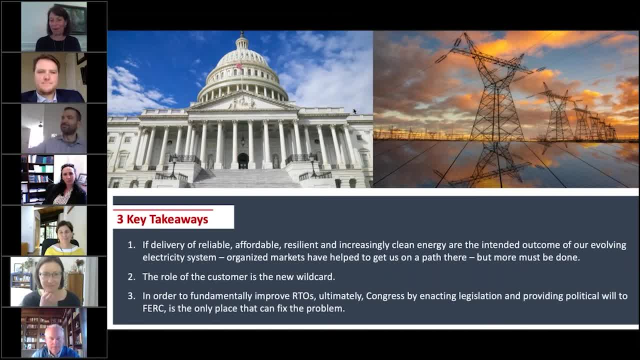 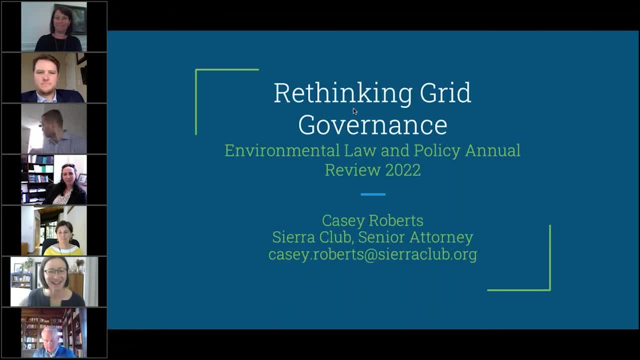 And I'm glad that you have some optimism about moving forward. So, Casey, you are up next. Okay, great. Thank you so much to Environmental Law Institute for inviting me to participate in this and to the folks at the Vanderbilt Journal for their support as well. 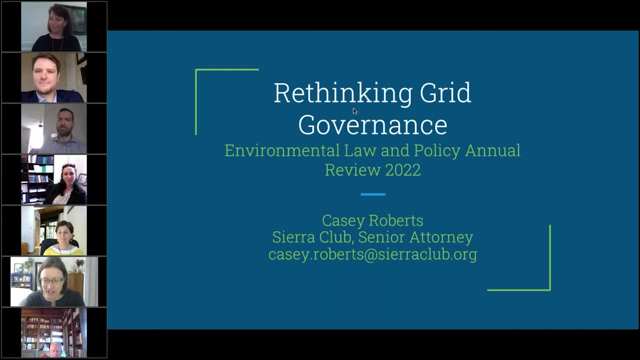 Really appreciate the opportunity. As a practitioner, it is incredibly helpful to have someone pull together all the big ideas that you've pondered before having to shove them down to deal with the next big filing deadline. So I am really, really excited to see Professor Welton's article. 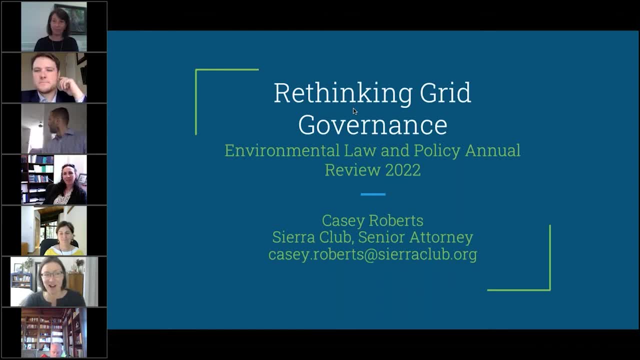 It was actually sent to me by a state legislator who I have been in some discussion with on these issues. So just to reassure folks thinking that maybe law review articles don't have an impact or get attention, this one really speaks to the moment at hand and I think that that shows. 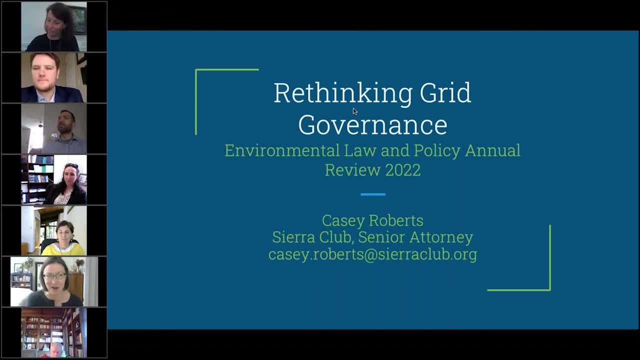 Before I get into all that, I actually want to take a moment to personally congratulate Jordan Diamond on becoming president of Environmental Law Institute. As Jordan mentioned in her intro, she and I were on the Ecology Law Quarterly Board together, And that was more years ago than I would like to admit, but I remember well what an effective 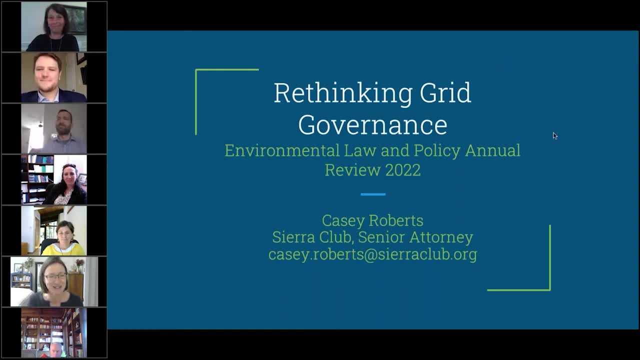 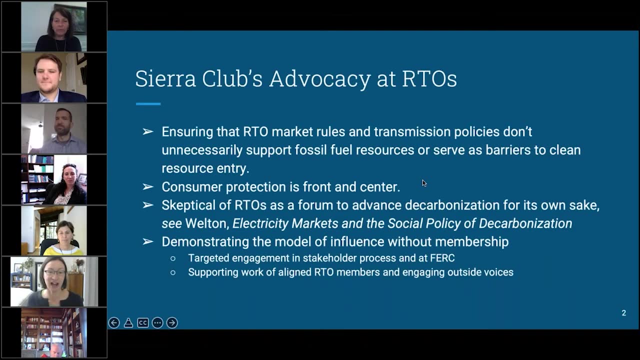 and fun team member Jordan was. So I know ELI is in excellent hands, So could you advance to the next slide please? I would like to start out with a little bit of a description of Sierra Club's advocacy at regional transmission organizations. 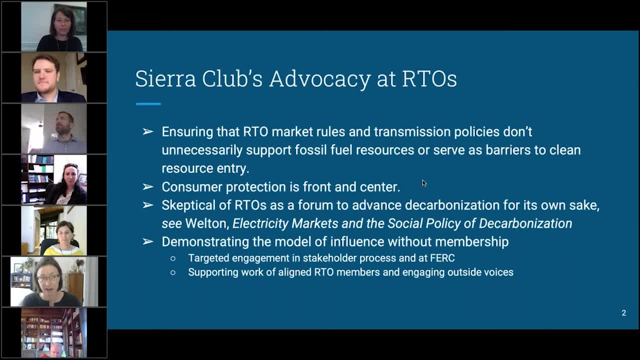 So I'm a senior attorney at Sierra Club. I've been there for about 10 years, working on RTOs and FERC for five to six years of that, And I think that this would just give a little bit of perspective on my comments today. 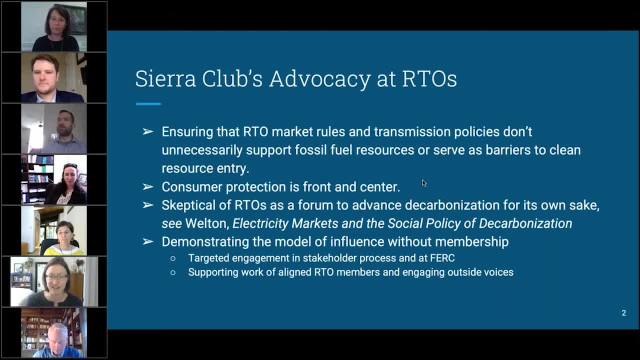 Okay, So first, one of our objectives is to ensure that RTO market rules and transmission policies don't unnecessarily support fossil fuel resources or serve as barriers to clean resource entry, And in advancing that, consumer protection is always front and center. Obviously, the affordability of electric service is a significant issue in our country, and 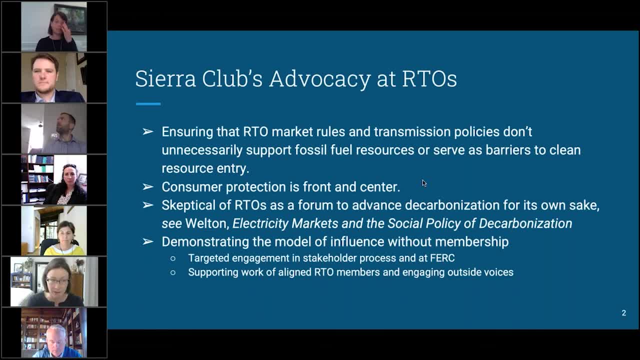 it's very important to organizations like Sierra Club and many of the others who we work with in the RTO space that decarbonization not proceed Okay, But we have to recognize that there is a fashion that the consumer is tractor, as they are at the expense of consumers, and that the efficiency that markets can bring when 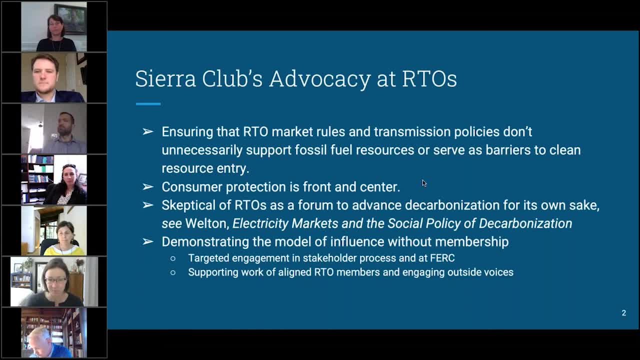 they are allowed to actually be truly competitive is really significant to consumer protection. Sierra Club is also skeptical of RTOs as a forum to advance decarbonization for its own sake, And on this I really highly recommend another of Professor Welton's articles: Electricity. 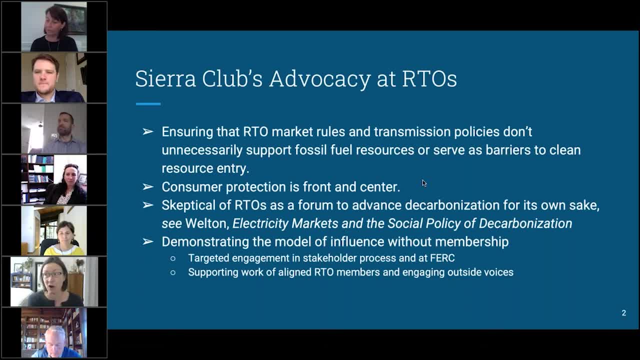 Markets and the Social Policy of Decarbonization, which really helpfully explores sort of the issue of decarbonizing And on this I really highly recommend another of Professor Welton's articles- Electricity RTOs versus states and other more electorally accountable entities as forums for advancing. 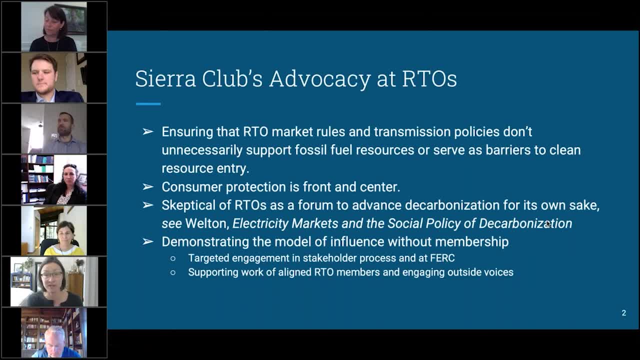 de-carbonization, given the many sort of objectives and broader values that are important in those policies. So that article very accurately describes some of the questions and concerns that we have and has really guided our approach to RTOs, taking them much more on their existing. 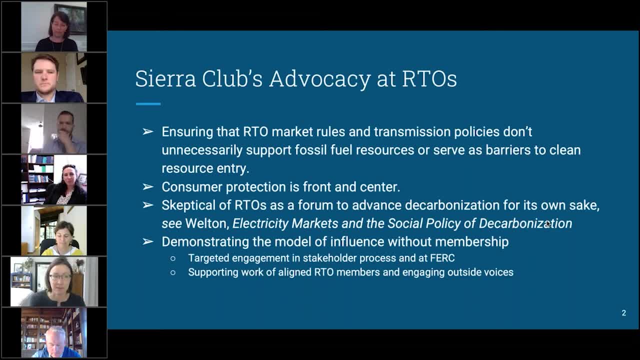 terms about market access and transmission planning, for example. Finally, I'll note that our advocacy in this space is sort of attempting to demonstrate a model of RTO influence without membership. So we are not a member of any RTO, but we do participate in stakeholder processes to 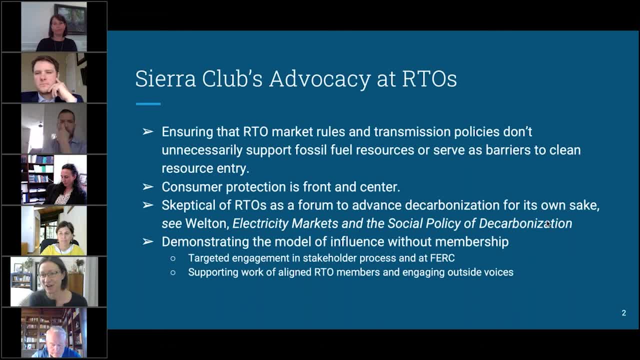 varying degrees. Obviously, bandwidth is an enormous consideration there, but so we have targeted engagement in stakeholder processes and then at FERC and in the federal courts, and we work to support the efforts of sort of aligned RTO members And also to bring in outside voices and draw attention to what's happening in these spaces. 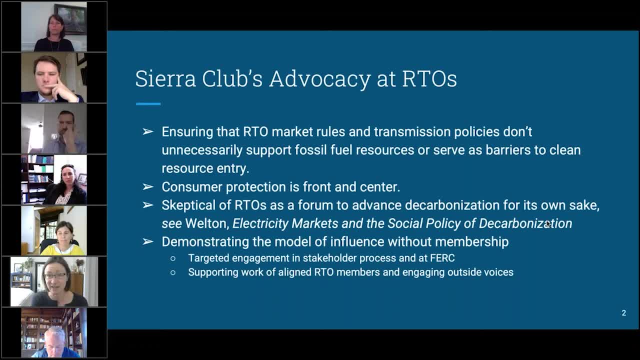 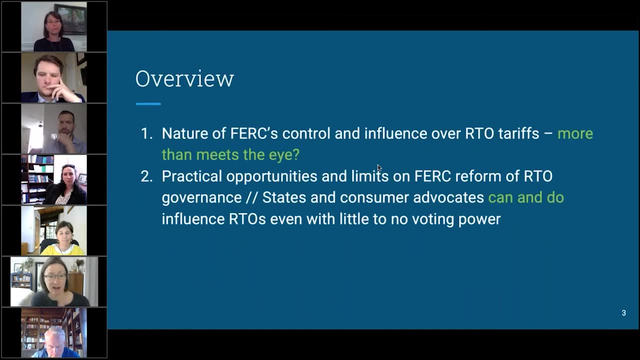 in a way that we hope can influence the outcomes. And you'll see that these strategies kind of reflect some of the recommendations or hopes that I have for how we can move ahead in RTO governance. So next slide, please. So the two main points that I want to make here today are- and hopefully, things we can. 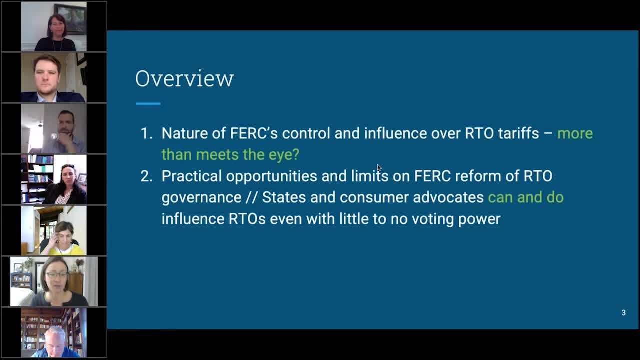 explore in the discussion later. So first I want to offer some more context on how FERC influences RTOs. I think here I disagree just a little bit with Professor Welton's article that FERC's authority is too limited to serve as a meaningful check on RTOs. 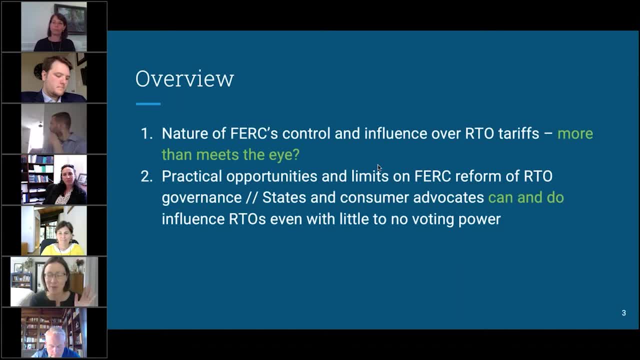 There's a bit more to it and I just want to add my perspective so that folks don't come away too dim of view of FERC's authority, because I think there's maybe more than meets the eye there. Second, I completely agree with Professor Welton that consumers and states need a bigger 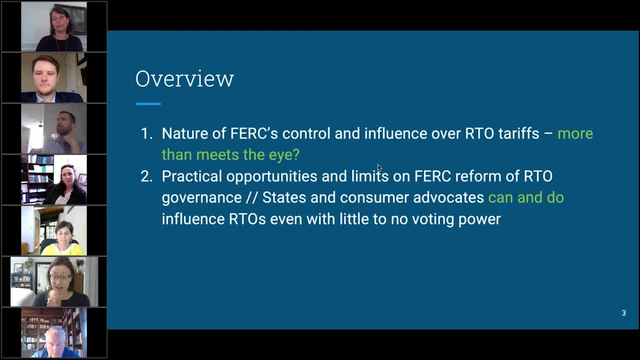 voice in RTO governance. I also see challenges to achieving that. So, in the spirit of yes, and I offer a few near-term, perhaps slightly less ambitious ideas for increasing the power of those voices in the meantime, while hopefully, as Tom says, 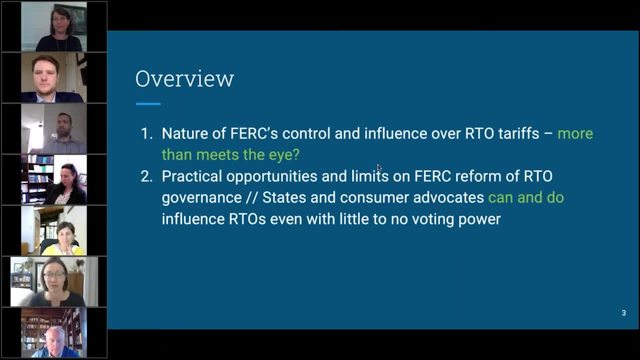 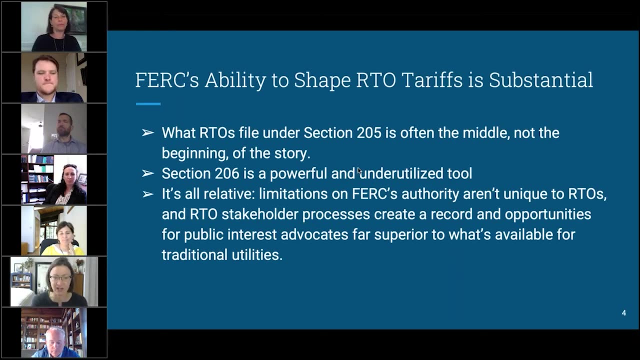 we can eventually get Congress to act to bring about deeper reform in RTO governance and how they interact with their various regulatory authorities. So next slide, please Thanks. So in my view, FERC's ability to shape RTO tariffs is substantial, even if under Section. 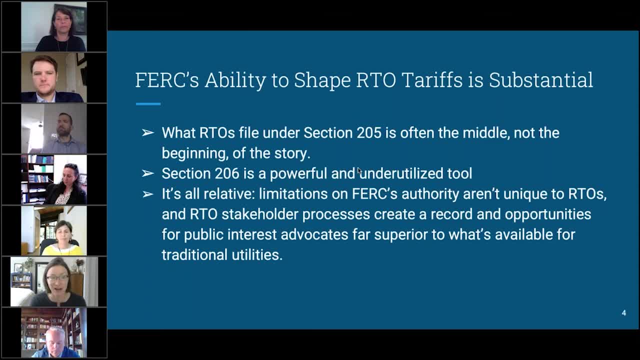 205, FERC is mostly limited to a sort of yes, no answer up down vote on what the utility files First. in my experience, many RTO Section 205 filings, especially on big issues, are shaped by conversations with commissioners and staff. 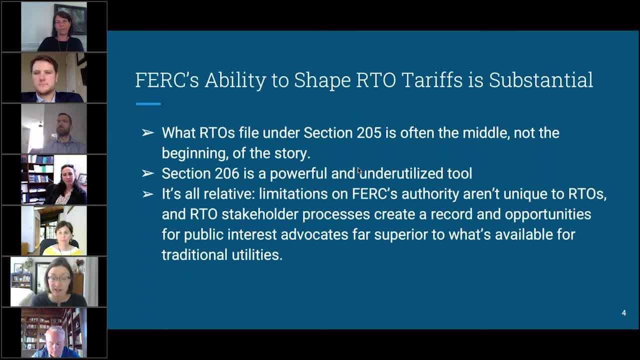 These may be public conversations, as in a technical conference, or private ones, which frequently happen in the lead-up to a filing. So I think that what the RTOs are filing under Section 205 is often the middle and not the beginning of the story. 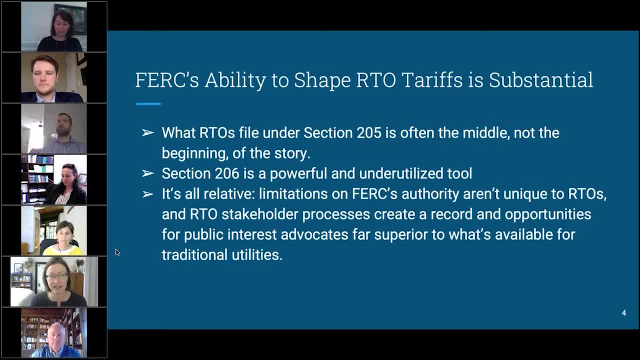 FERC has actually had influence on the utility's thinking and how they're weighing their different member perspectives. leading up to that, RTOs don't want to have their filings rejected and we'll try to develop more information about issues are concerning to FERC, or what kinds of analysis FERC has indicated it might. 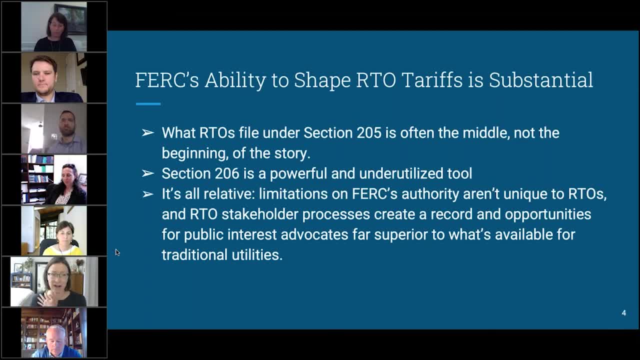 want to see that sort of thing, So yeah, So that's kind of maybe a less obvious way that FERC is able to influence what the RTOs are doing. Also, while FERC can take a deferential-like stance under Section 205 and find that a wide 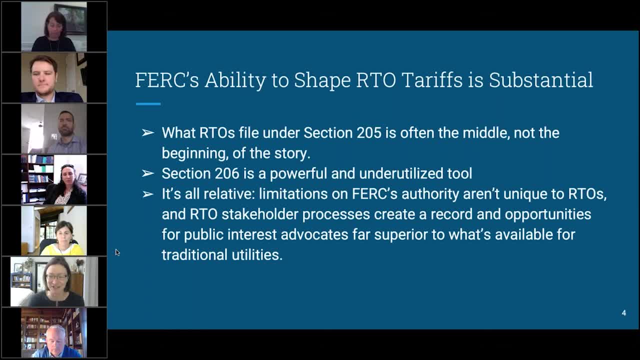 range of proposals are just and reasonable. it definitely doesn't have to do so. FERC rejects RTO Section 205 filings all the time and I don't think the problem is that FERC lacks sufficient authority to keep RTOs in check simply because it can't modify those. 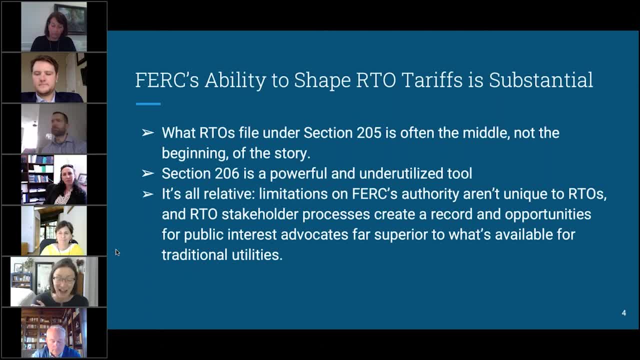 filings. So things certainly might get done more efficiently if FERC did have the authority to modify RTO filings. but I think that where FERC can you know, either a record is created by stakeholders or through FERC's own investigation. notwithstanding that sort of passive and reactive stance, it 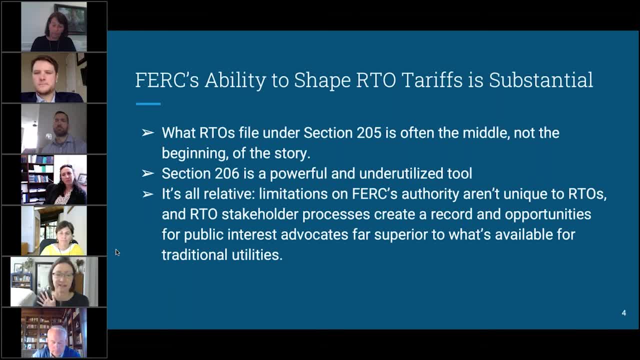 really can push back on those 205 filings. Which also brings us to Section 206 of the Federal Power Act, where FERC does have direct authority to make things happen. Okay, Professor Welton notes in her article it can be ponderous and more legally risky, for 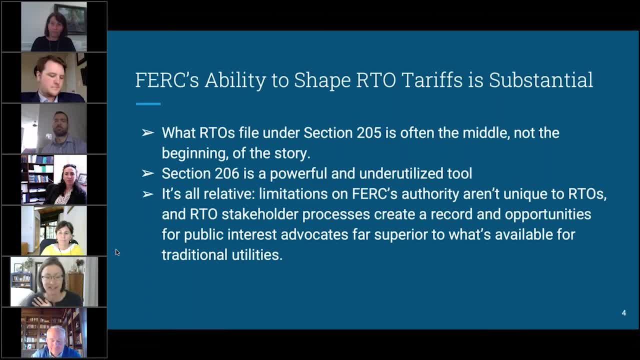 FERC to act under Section 206, because it must show that the status quo is not just and reasonable, rather than simply showing it has a better idea about how to do things. I certainly agree with this, but I also don't think we should discount the authority that. 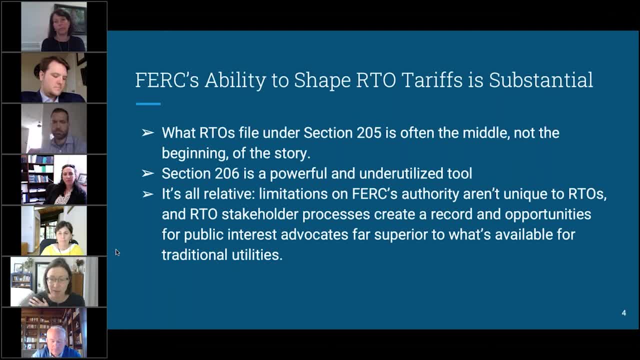 FERC has under Section 206.. The article discusses a couple of examples of FERC using this authority in recent years to open up RTO markets to energy storage distributed energy resource access. Of course, the full benefits of those orders have yet to be seen. 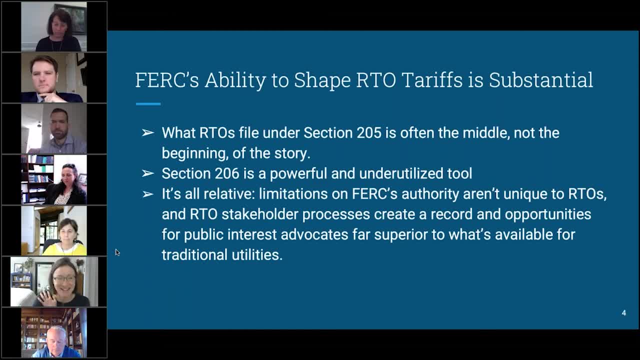 And of course, 206 can be used for some unfortunate- at least to see our club- ends, such as the orders that FERC has did put out in the PJM context regarding the minimum offer price rule, which we do not have to go into details of that just yet. 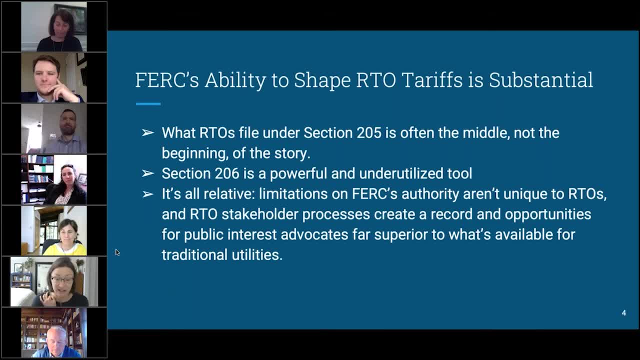 So, for better or worse, FERC has the authority to get RTOs moving in certain directions if it really wants to and if it's careful to develop a solid record. Okay, And my final point here on this slide is that these limitations on FERC's authority aren't 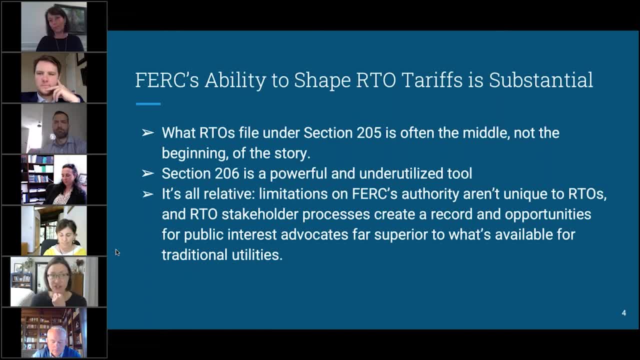 unique to RTOs And Professor Welton just talks a little bit about the evolution of RTOs from the sort of prior traditional utility model This sort of reactive and then barriers to acting under Section 206 is how FERC interacts with all utilities. 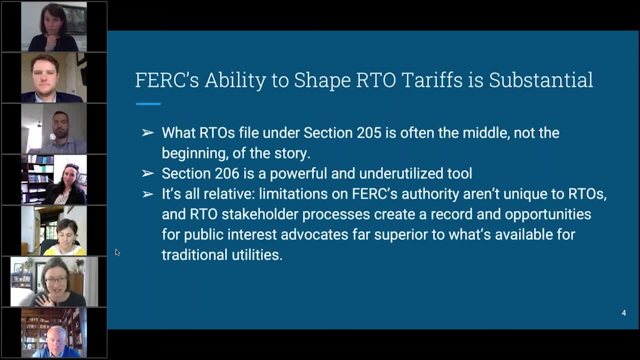 And I think that the situation is actually a lot better when it comes to RTOs than these other utilities. The stakeholder process, as flawed as it is, does force some transparency or some analysis and, at the very least, gives advocates a heads up to start building a case against a utilities. 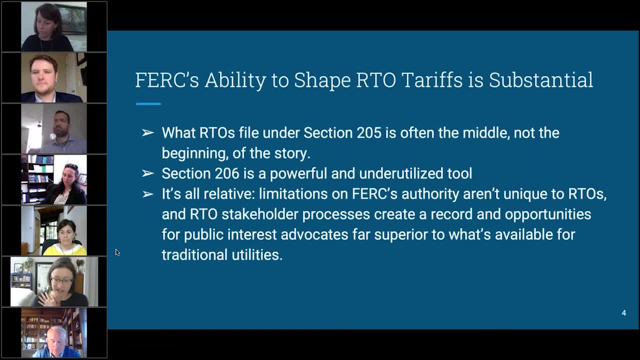 filing. So this improves advocates' ability to hold utilities and FERC accountable. I don't want to overstate the case here. RTO governance matters a lot but I'll come back to this point later because I think that even short and deep governance reform FERC could. 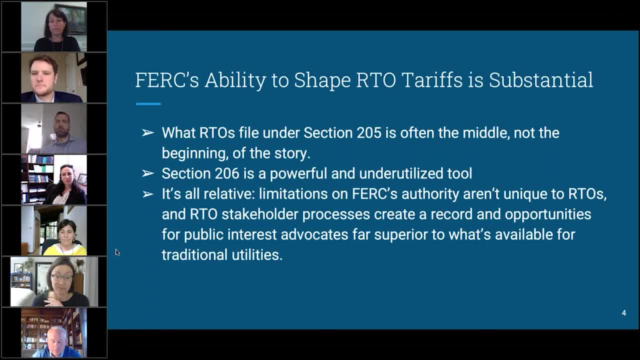 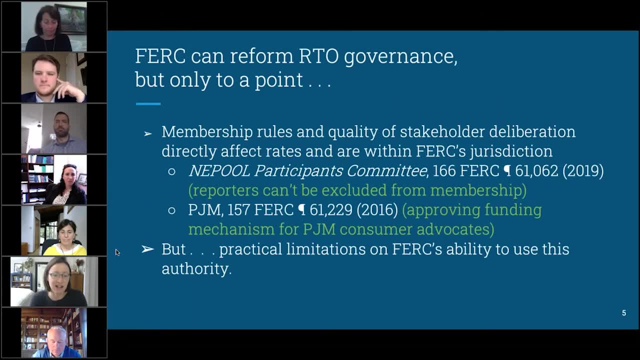 take some actions that would significantly improve the quality and transparency of the stakeholder process. Next slide, please. The next concept I wanted to react to that comes up in Professor Welton's article is what FERC can actually do on governance. The article discusses the CAISO case where FERC's efforts to shape the CAISO board were. 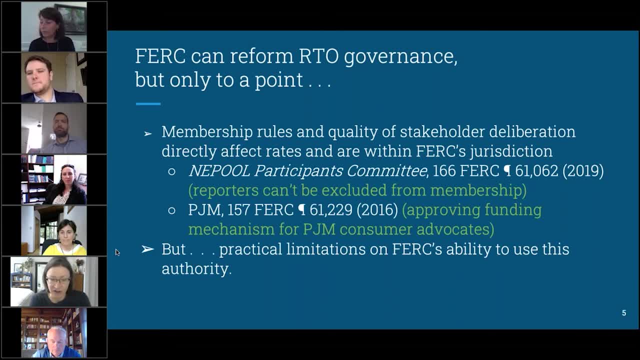 rebuffed by the Ninth Circuit. Okay, But there are a few other cases that are significant in my world that I wanted to bring up that, I think, suggest some potential paths forward. One of these is this NEPOLE Participants Committee case from 2019, where NEPOLE actually sought. 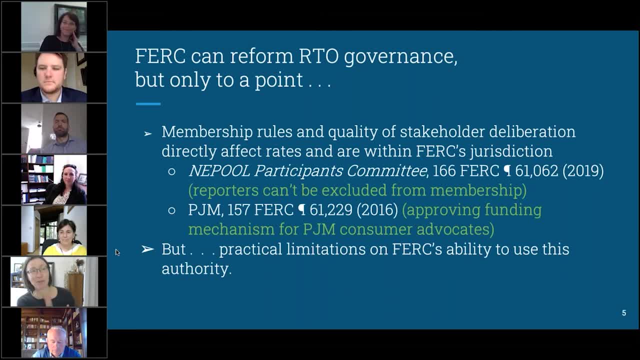 to change. Sorry. NEPOLE is the governance stakeholder body for ISO New England and they sought to change their market rules, their membership rules, to prevent a reporter from becoming a member. FERC rejected this and in doing so, reiterated that it does have jurisdiction to. 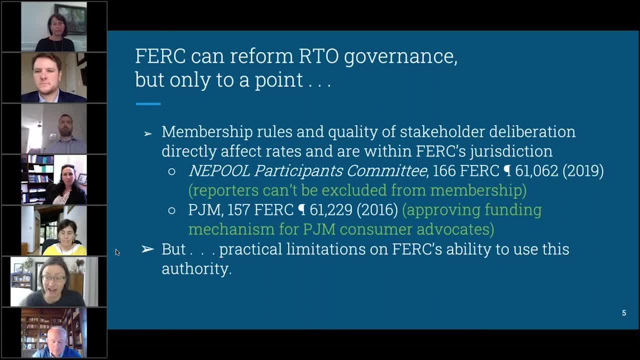 With respect to membership, and it said that because membership directly affects commission jurisdictional rates, A prior order that I also think is helpful relates to This. one comes out of PJM, and in this order FERC approved a terra filing that would grant 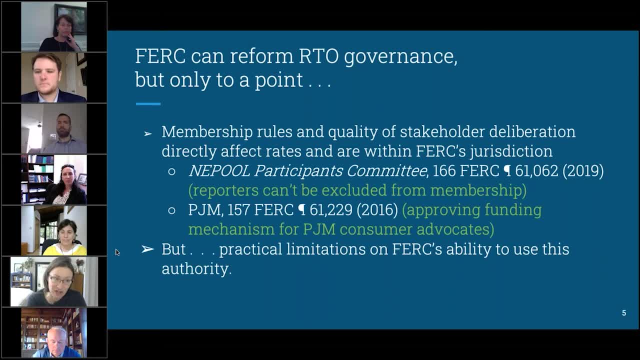 funding, a funding mechanism for the PJM consumer advocate body known as PJM. Okay, So it's the Consumer Advocates of PJM States, or CAPS, And here FERC said and clarified, really, that stakeholder input is an essential element. 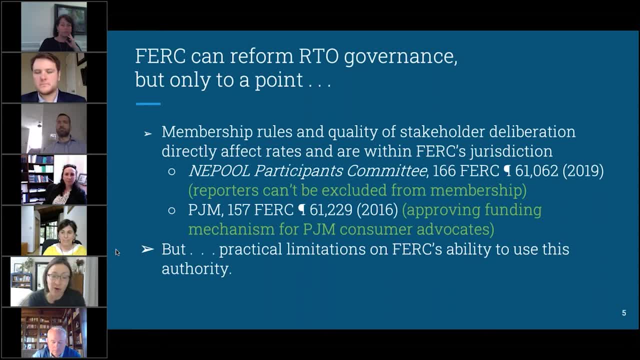 of just and reasonable rates coming out of RTOs and commented quite a bit on the quality of stakeholder deliberation and the stakeholder process in terms of what rates come to FERC. So these two examples might make your imagination run wild. 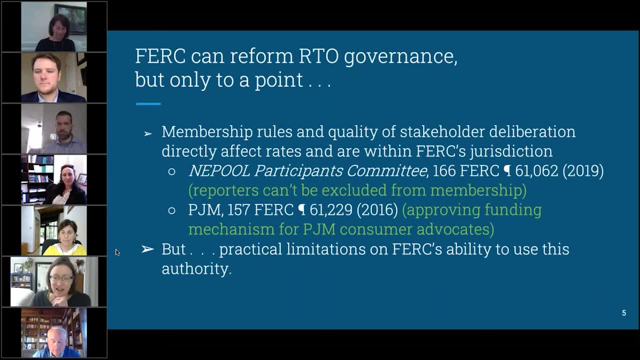 Okay, I was gonna say- and I think I'm gonna leave it for you, but I think it's important to be realistic- that there are practical limitations on FERC's ability to use its authority over governance in the stakeholder process, And this is because, with just a few important exceptions, RTO membership is voluntary. on: 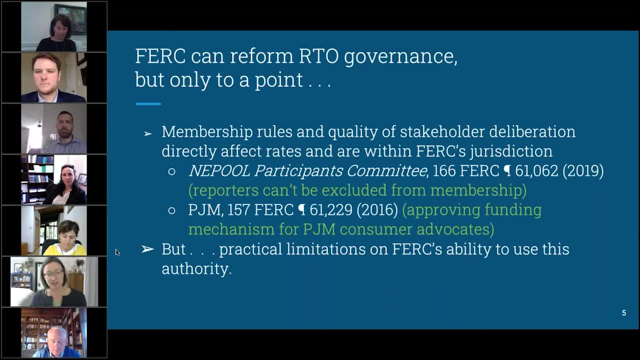 the part of transmission organizations. So there's only so much FERC can do to push on this without making it unattractive for transmission owners to be members of RTOs, And that's why, as Tom was suggesting, I think some congressional action on this point would. 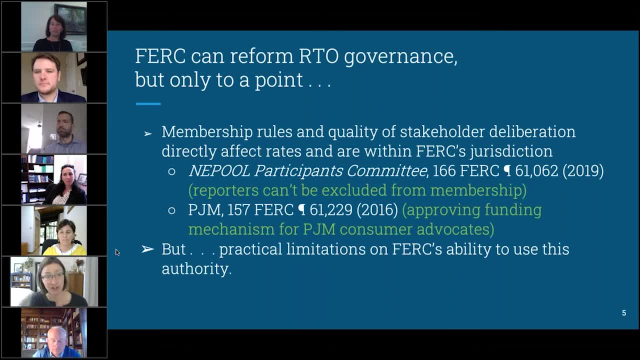 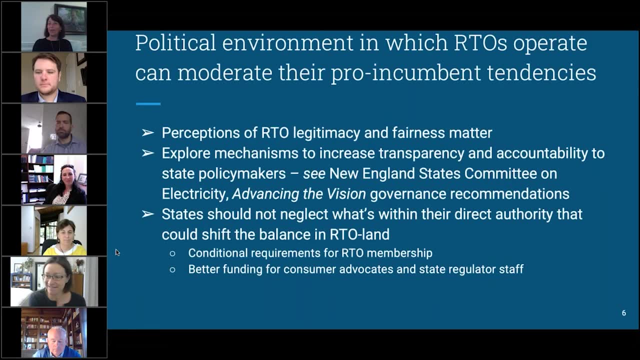 be really helpful to sort of strengthen FERC's hand vis-a-vis the RTOs and governance. All right, Next slide, please, Okay. So I also think it's important to note that the political environment in which RTOs operate can moderate their pro-incumbent tendencies, which are well-detailed in Professor Welton's 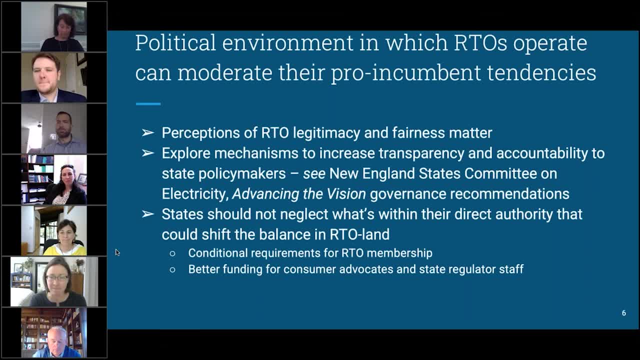 articles, unfortunately So. first is that RTOs are very sensitive to perceptions of their fairness and independence and legitimacy, despite the maybe most prominent articles on this PJM controversy being published in Utility Dive. as Professor Welton was noting, I think there's many changes. 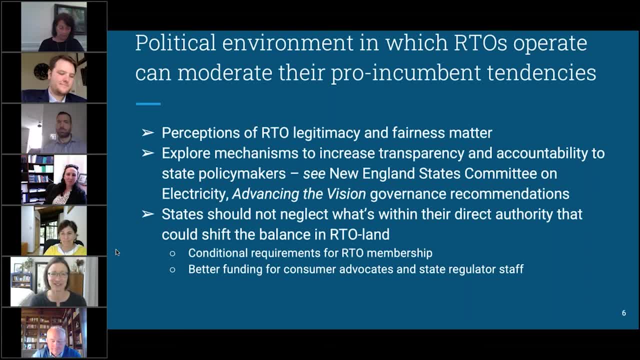 There's many channels, both you know through the trade press and other types of communications, in which RTOs do feel public pressure when they take an action that's widely viewed as unfair And to the extent that an RTO becomes perceived by FERC or its membership as favoring one. 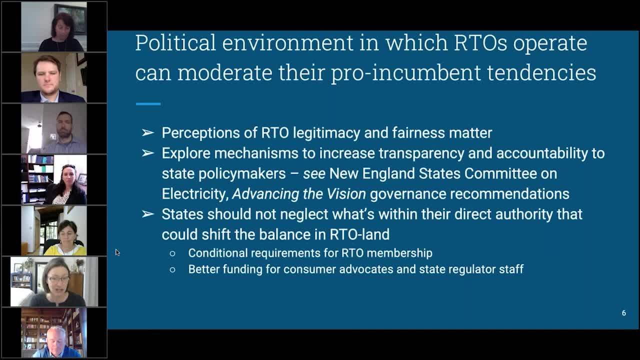 membership sector over another or not being truly independent, as they're supposed to be. it makes their job a lot harder. It's harder for them to get filings approved at FERC. The stakeholder processes are more difficult, So I think that's important. 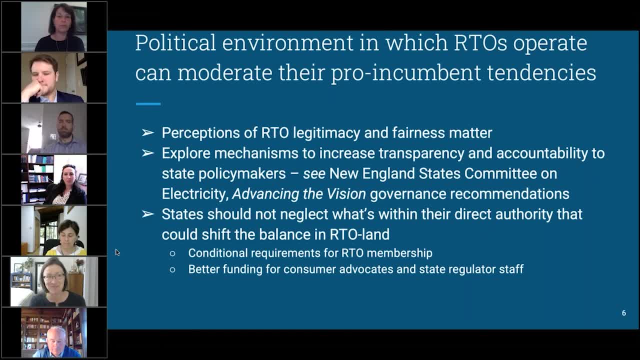 They're more contentious, And I think all of these things do help to encourage RTOs to try to balance things out in the stakeholder process. Of course, you know voting weights in a you know sort of sector-weighted situation. 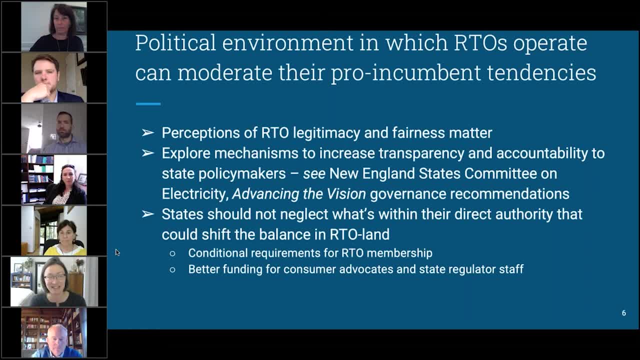 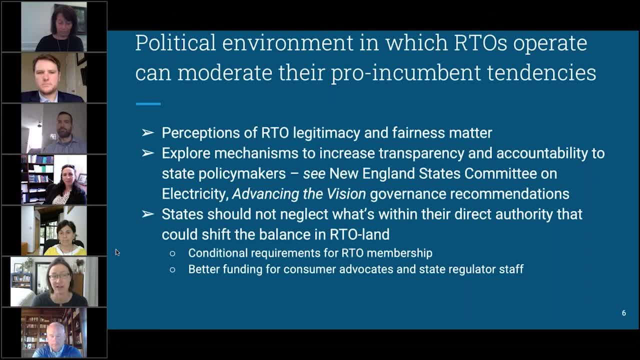 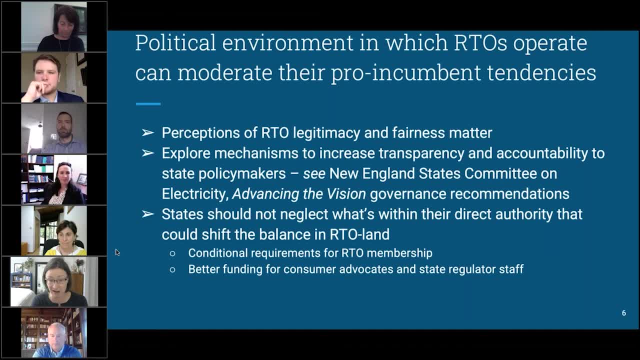 And I actually recommend. the New England State's Committee on Electricity, or NASCO, published a report- I think it was last year- called Advancing the Vision And it makes a couple of really interesting governance recommendations- recommendations about requiring the IS New England board to 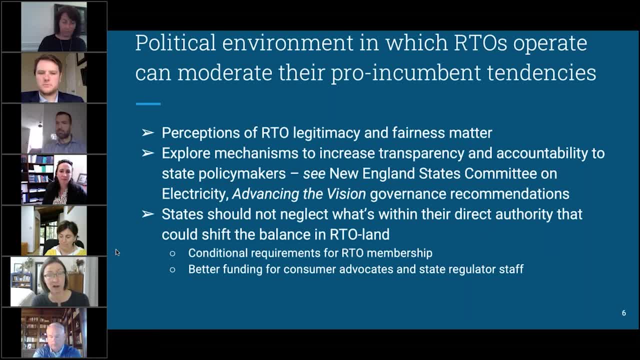 sort of state its reasons for rejecting the position advanced by a majority of NESCO state members and otherwise just sort of increasing the Transparency and accountability around actions that the board takes that are contrary to state interests. So obviously this is far short of something like giving the state a veto right. 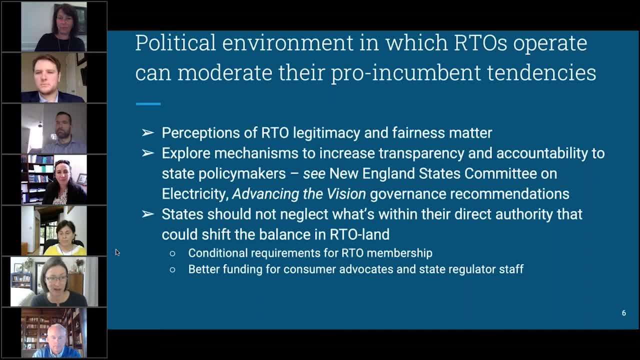 but I think it reflects that even Some sort of incremental improvements on transparency can really help to make it harder for RTOs to outright reject really well considered positions of their state members. Casey, this is all so awesome, but we're running out of time. 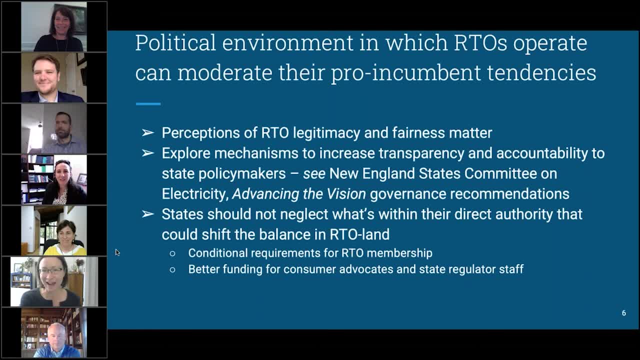 I want to make sure everyone gets a chance. Yep, Yeah, my bad, My bad. Um, I'll just leave it this. the last bullet is the last thing I'm going to say, Which is just that I also think states should explore What may be within their direct authority to improve sort of funding and capabilities of consumer advocates. 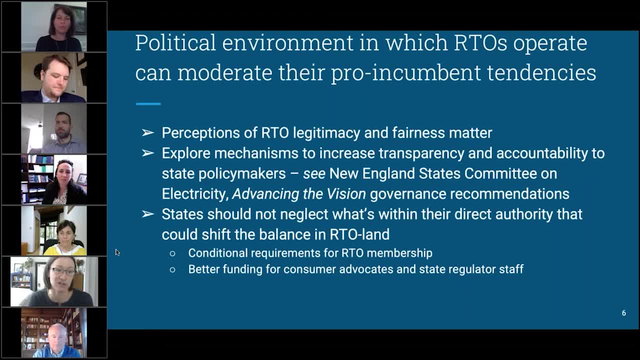 environmental Agencies that are advocating before the RTOs to try to help shift that balance as well. So it's not only things that FERC or the RTOs could do to level the playing field, but things that the states themselves Could do. so apologies for going over, I'm really excited. 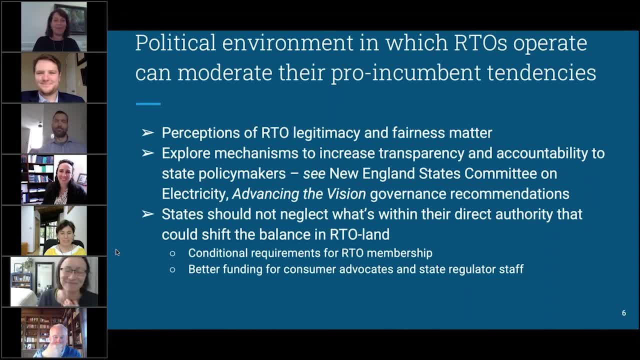 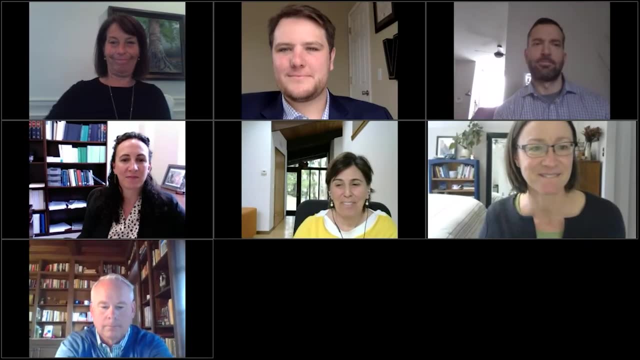 It's all I mean. so much great information. I wish I wish these panels were a little bit longer, actually. So let's turn now to our last but definitely not least commenter, Rebecca, and remind you So: thanks so much. um, it's so good to see everyone and 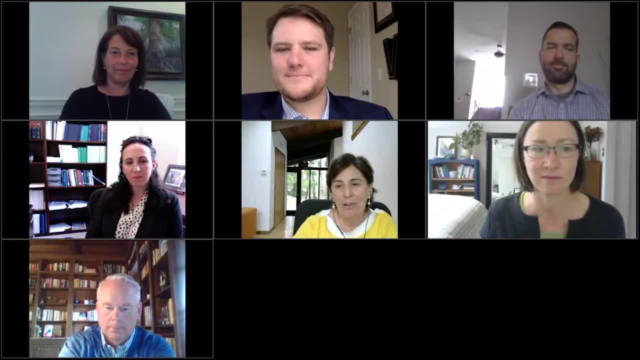 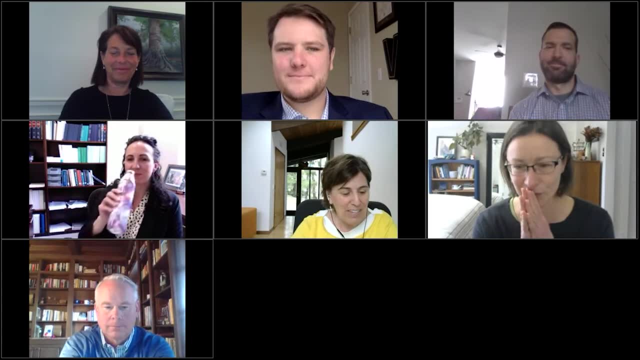 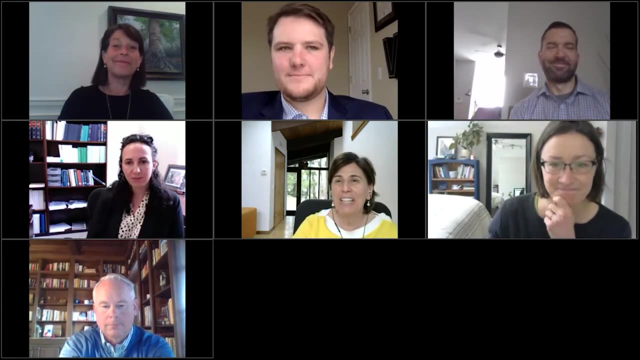 I have to say I too will give a plug for the law review articles, because I too wait for them and read them, and a plug for those Congressional hearings which I think I actually was part of And it distresses me a little because I feel like the same arguments I was making five years ago. 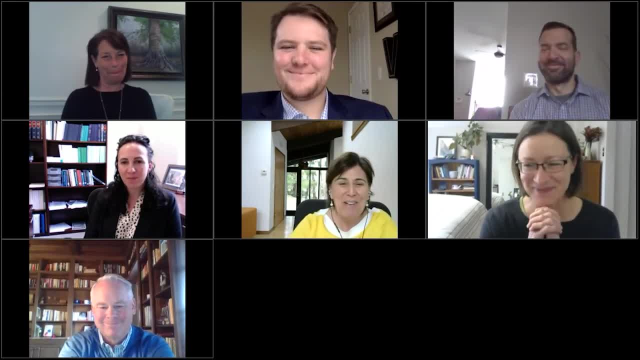 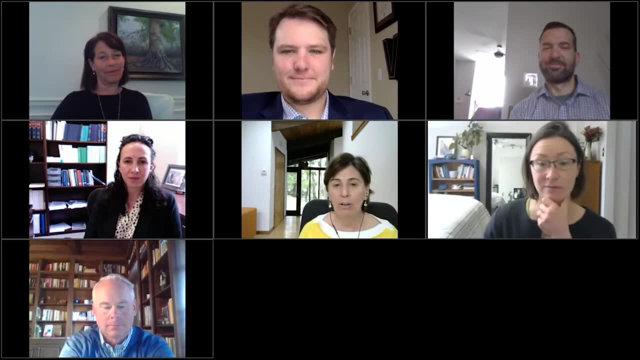 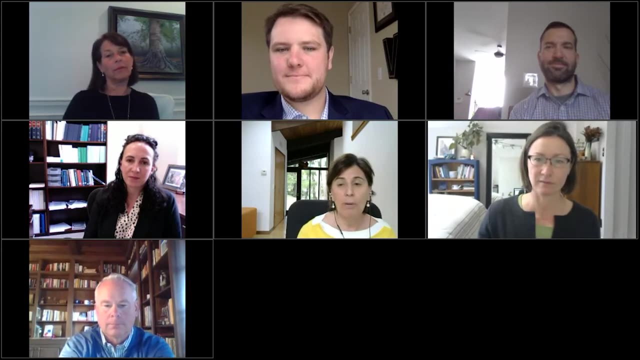 I might be making today, which is a little discouraging, but, um, you know, I'm here, I think, to talk about consumers and particularly about consumer advocates, and I think most people know that that most states have consumer advocates that are particularly Designated to represent customers at public universities. 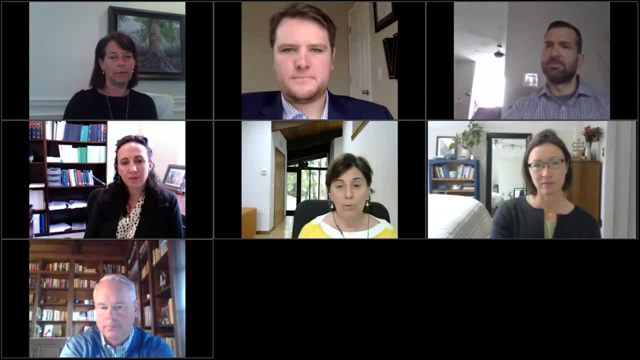 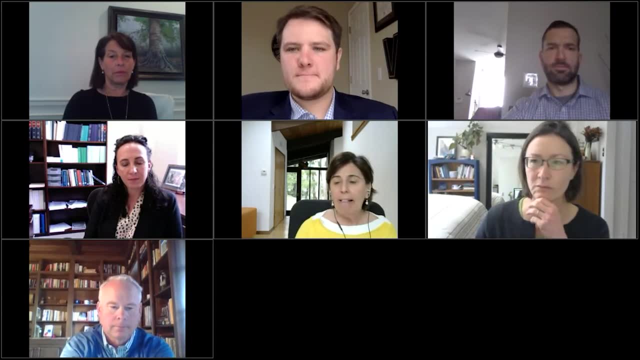 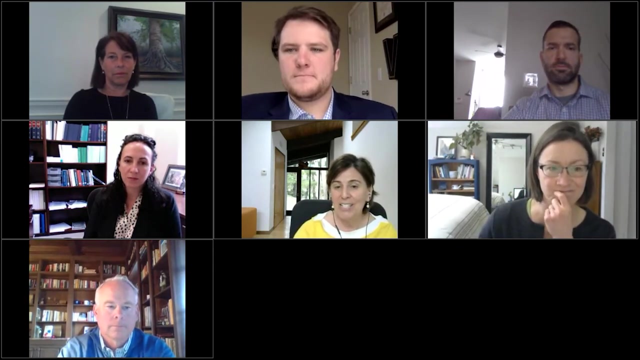 utility commissions and also Most of them have the authority to also represent customers at it, like places like the RTO and FERC. and You know, as professor Welton notes, FERC has recognized that. you know that what happens at RTOs is important for customers and 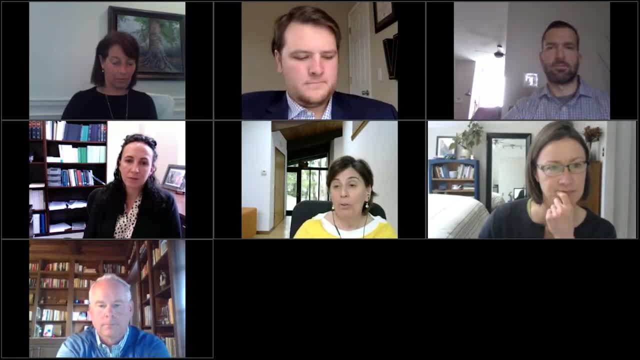 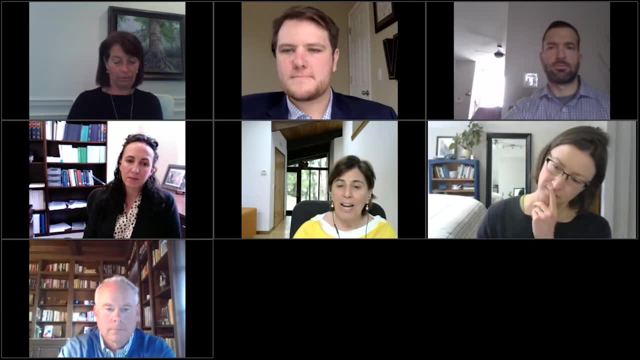 specifically, has talked about the need to give voice to the people and the businesses who ultimately pay for electricity. You know, I think, that RTOs right now, I think more than ever, as you guys have mentioned- are setting rules that really impact our clean energy future. 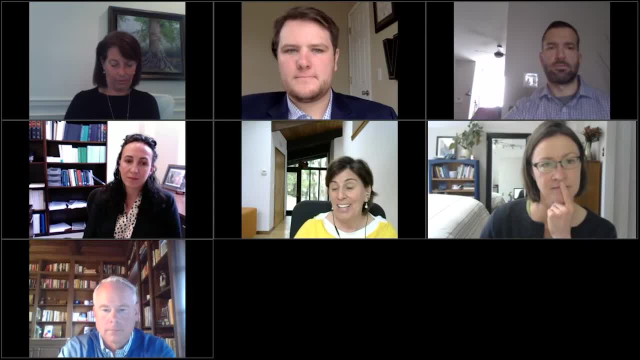 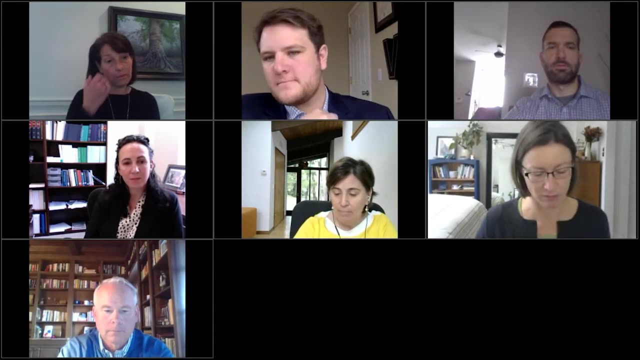 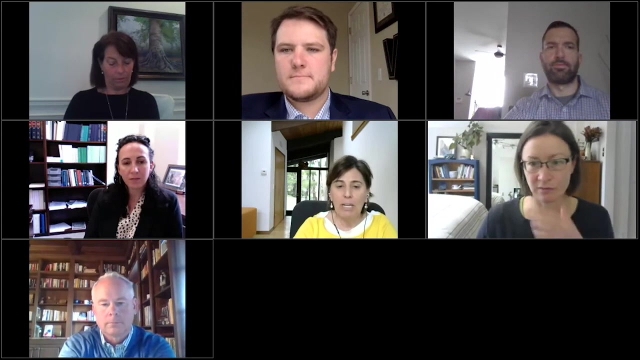 They decide, as we've talked about, who in the wholesale electricity markets gets who gets to participate in those markets. They, they decide things that directly impact utilities bills. So So I will tell you, as somebody who has appeared at our ISO New England and RTOs before there, right now is not a meaningful opportunity for customer participation and decision-making. 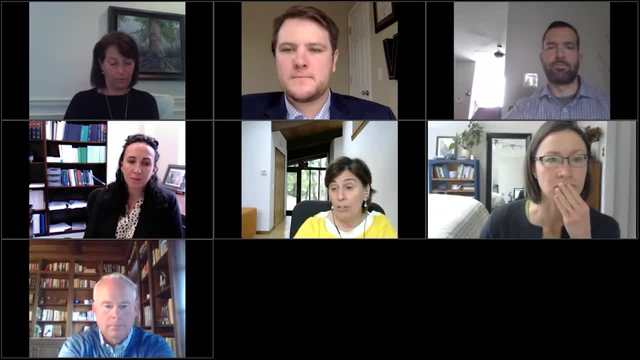 Nor is there the necessary transparency to to democratize access. It's, it's just not. it's not there In New England I can give you a little bit of example. We have two sort of main avenues that people think are important for customer Participation, and the first one is what we call the consumer liaison group. 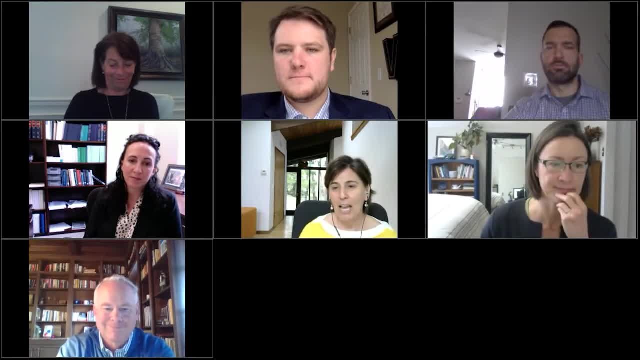 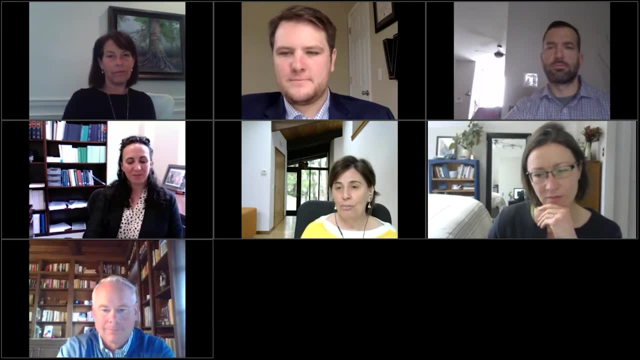 And I've had the honor of being the head of that group for a very long time and I- but I will tell you what it is and what it isn't. and What it is is primarily an educational forum for customers to come to meetings and hear from ISO New England. 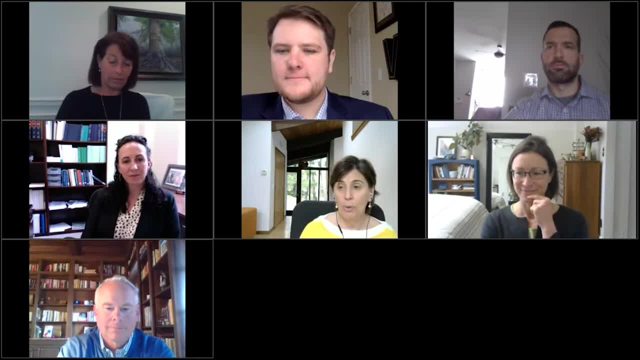 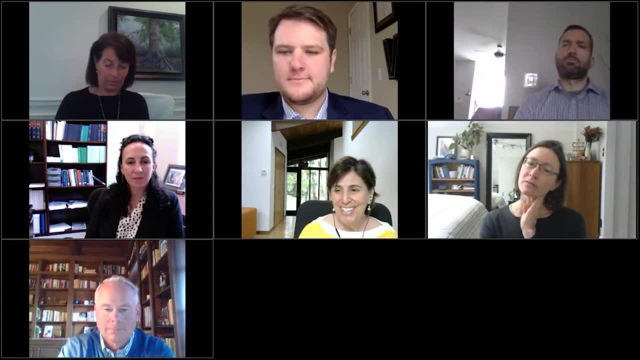 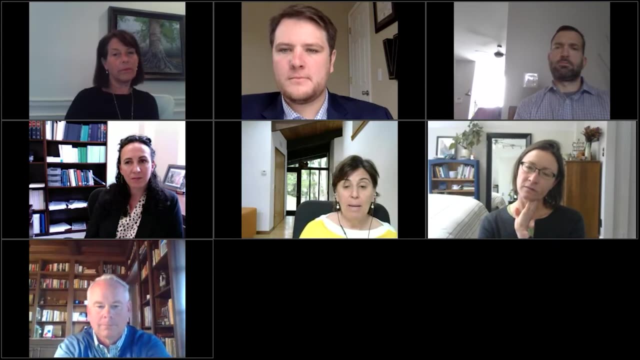 And hear from the high-level officials at ISO New England and have an opportunity to learn about what's going on there and ask questions. But it does not serve as any kind of decision-making body or influence on ISO's decision-making. And if you want to actually have some kind of decision-making authority, 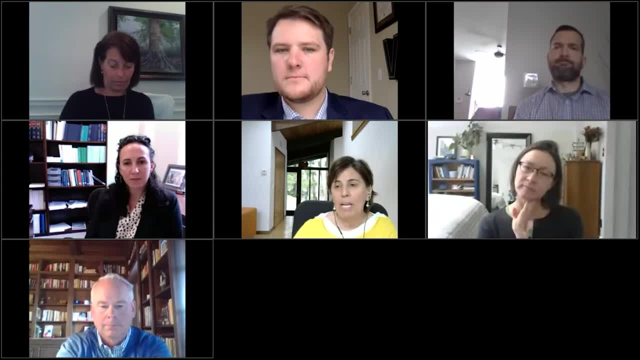 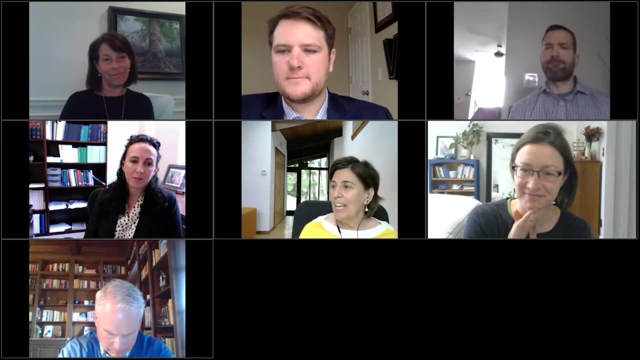 You have to join the stakeholder process, which means you have to become a member of the stakeholder process, which means you need to pay, and It means that That you're good if you really want to be a real participant. as Professor Weldon noted, there are hundreds of meetings a year, hundreds, And between the 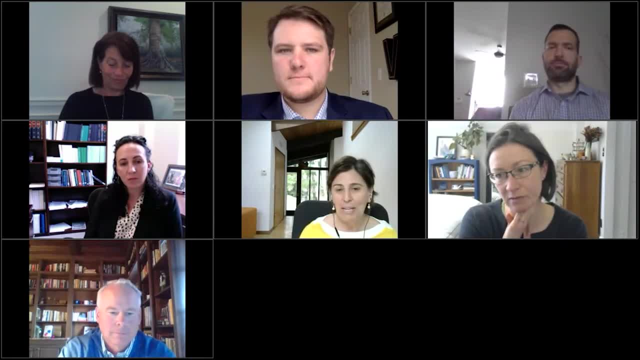 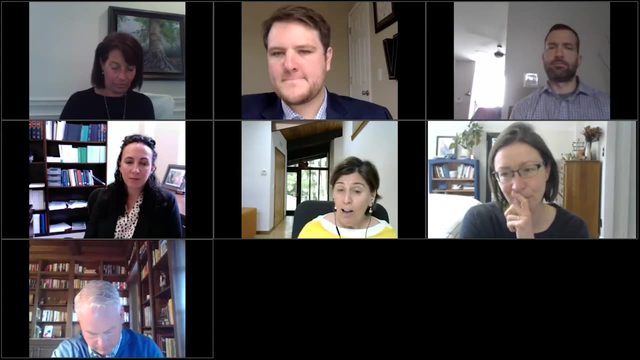 subcommittees and the committees and the participant committee. it's a process that is complicated and expensive and time consuming And I think if you're a regular person, you're not doing that And if you're a consumer advocate, like we are, my office devotes. I'm trying to think. 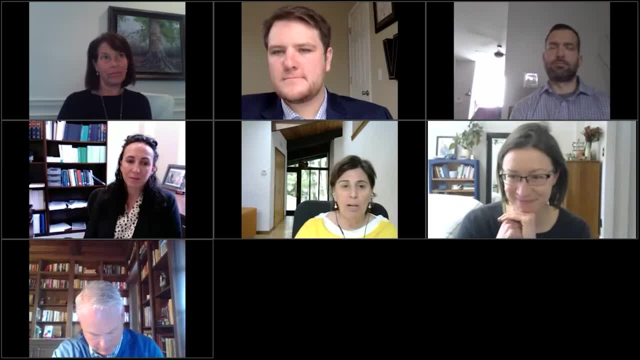 we devote a lot of people. We have a lawyer and an analyst who work full time on RTO matters And we have two lawyers who spend time on FERC And we have two more lawyers who help with the consumer liaison group. But most states don't consumer advocates. they just can't afford to. 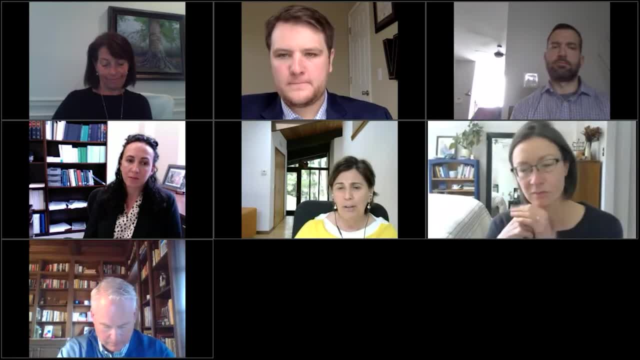 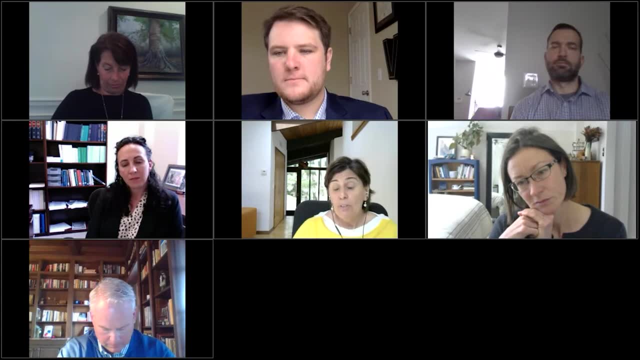 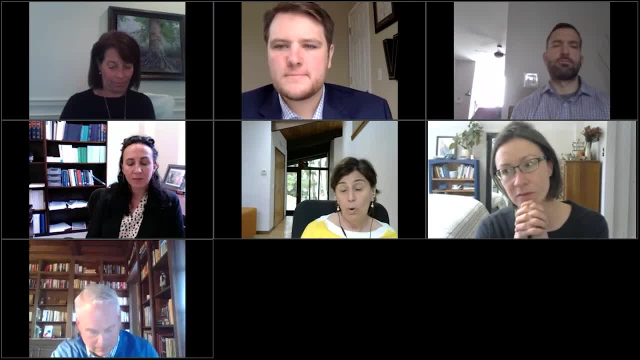 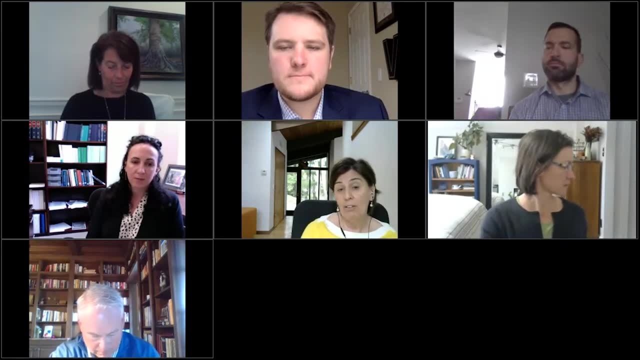 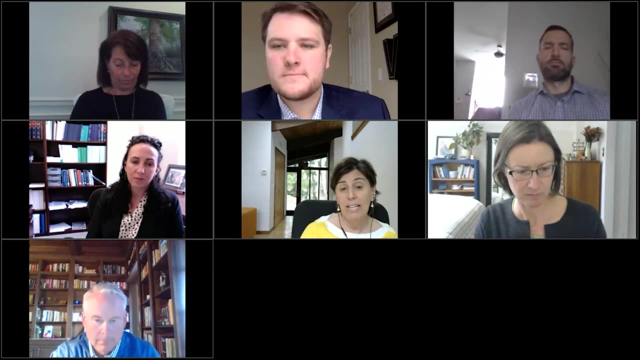 mechanisms we put in place back when we did order 719- i mean, the consumer liaison group in new england was the result of order 719- but what we have found is that there is not meaningful participation by the people who ultimately use electricity, or consumer advocates second um and 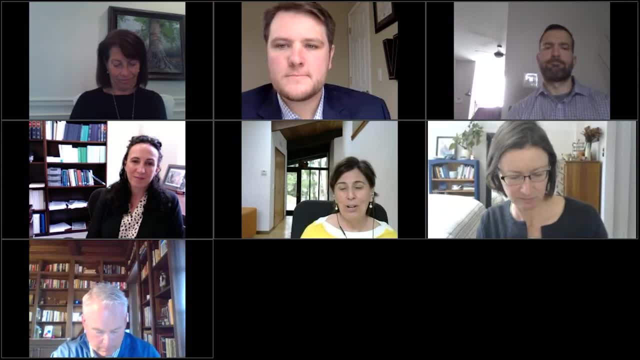 this is- i've been my rallying cry for a long time, so i can't forget it- which is, i think that if we establish some kind of stable funding mechanism that enables consumer advocates to fully participate in the rto process, in the stakeholder process, i think that that would be helpful there. 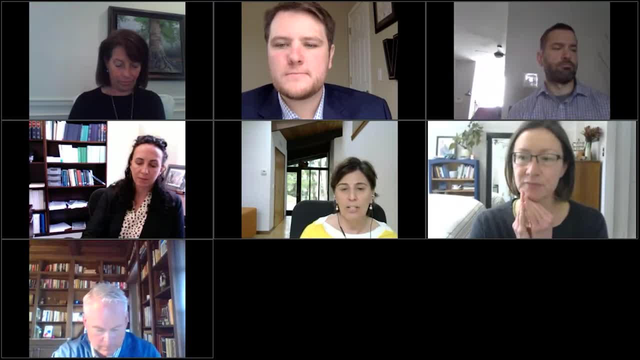 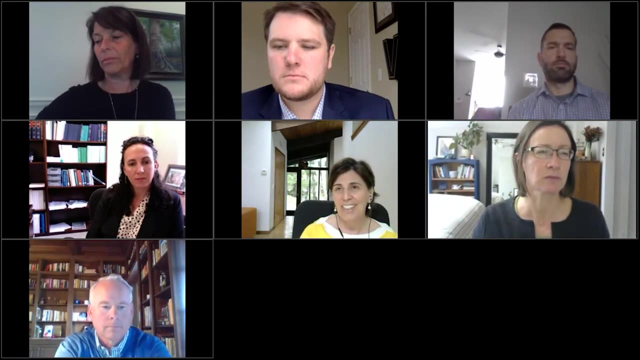 is one um example of that that's in pjm and it's called the consumer advocates of the pjm, states caps, and they actively participate, help help state consumer advocates participate in the stakeholder process and they're funded through a small part of the fur tariff and um i think. i think if we 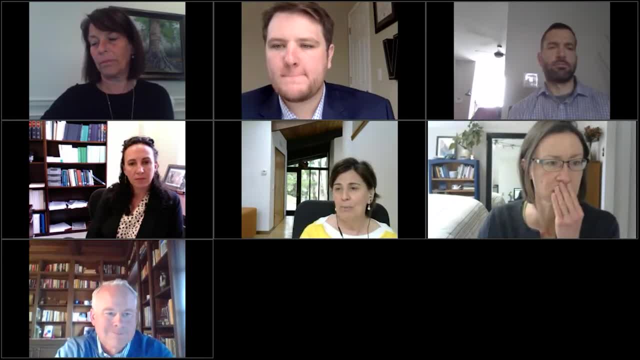 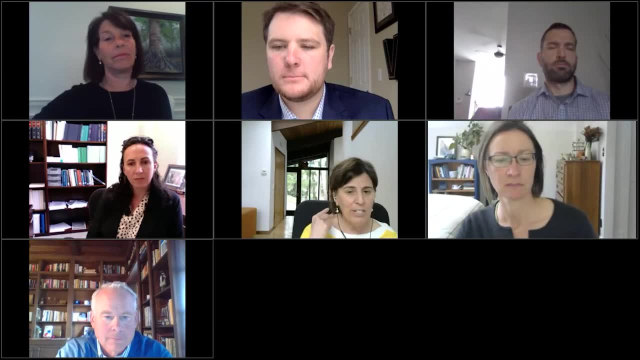 had a little bit more time to think about that. i think that would be helpful, and i think that's one in new england. new england would be like a penny on customers bills to fund something like that very small um. the other thing i think is important is that we haven't talked about today is 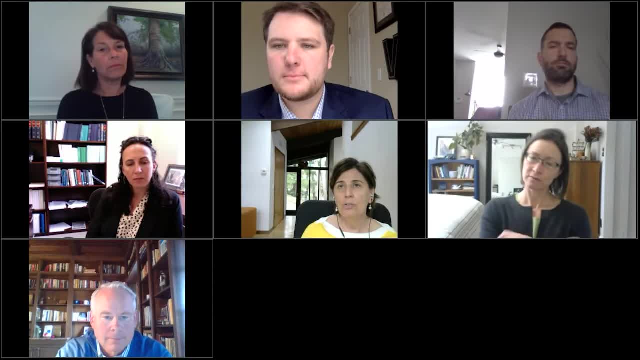 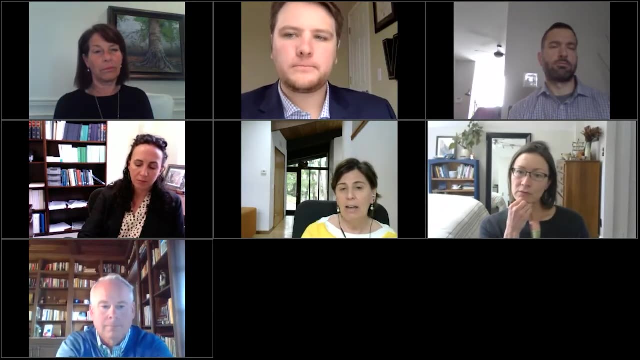 um that that isos and rtos should be required to consider costs in their decision making and provide cost impact analysis on major proposals and the reasonable alternatives offered by others. and if that analysis was performed early in the process, which it very rarely is, that would increase. 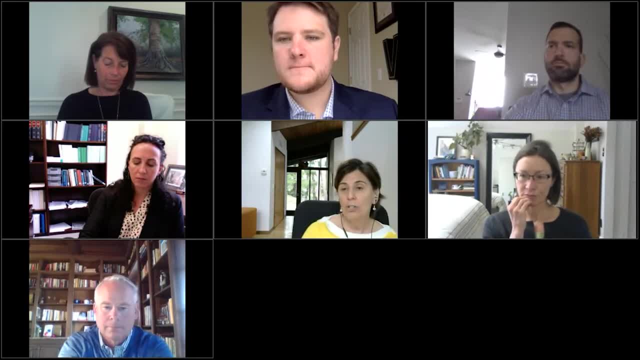 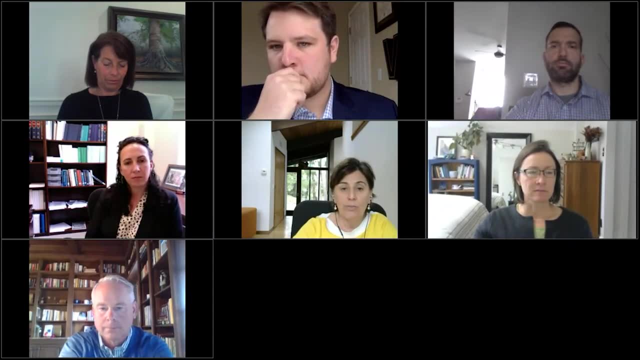 transparency and provide consumers with access to the cost information that's the most relevant to them. um, in our state, transmission generation accounts for sixty percent of a customer's bill. that's it's a lot of the bill, and cost considerations are one way that a customer's 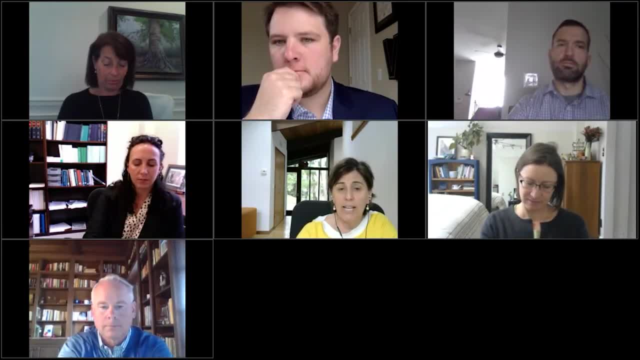 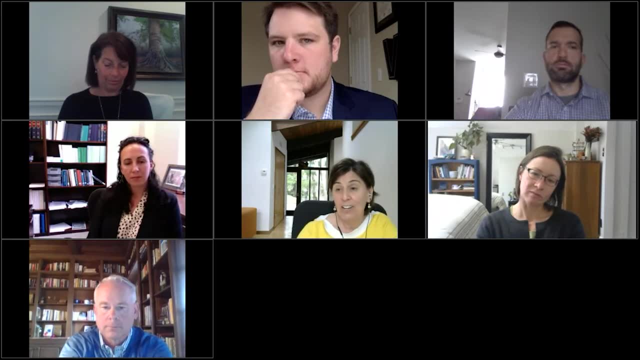 cost can be thought about um in the decision making process. i can tell you i never hear anyone talk about how much this is going to affect somebody's bill. i mean in an rto. it's just not what people think about um. i think i mentioned earlier we could increase, we could increase. 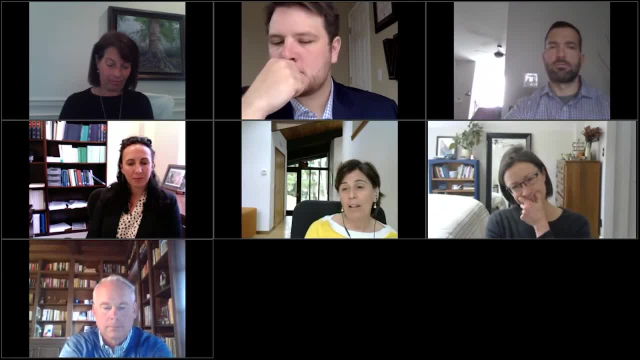 communication between rto board and consumers. um, one of the ways that we have been advocating for- and i think we we have been somewhat successful- is to have at least one member of the board have experience in consumer issues and or have a board member who is designated as sort of the 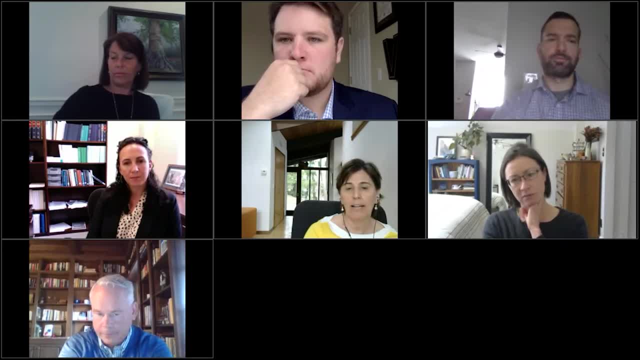 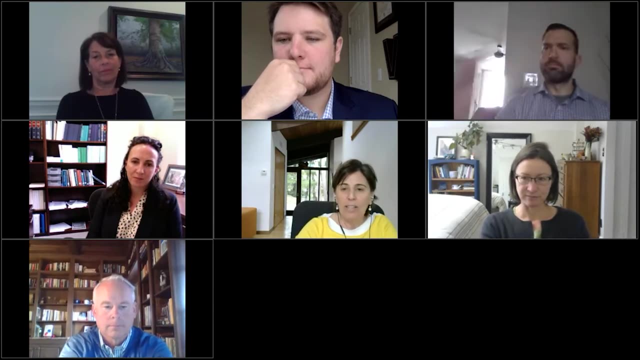 consumer liaison board member dela. you know, does it liaison? the last thing i want to do is a pitch to all of us, um, which is that we all also need to be educators if we're going to ask the public to get on board with a lot of new transmission and renewable. 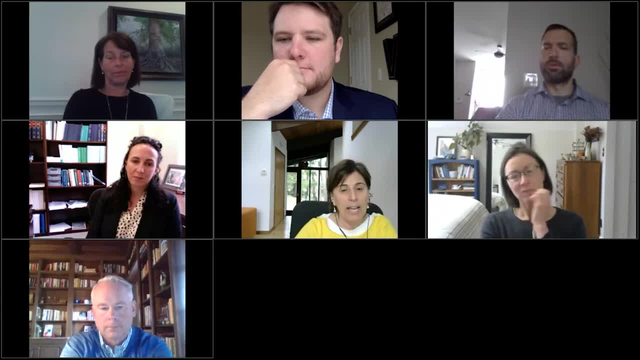 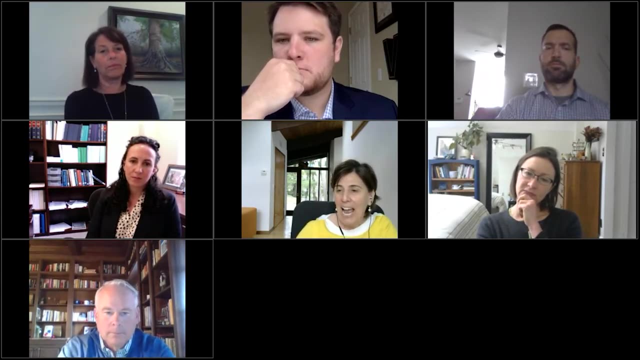 build out and you know we're going to need their input and we're going to need the support not just of the traditional stakeholders. we're going to need a broader public buy-in, including grassroots organizations, academics, elected to all those. everyone is going to have to be informed and be an active public on these matters because otherwise we're not going to. 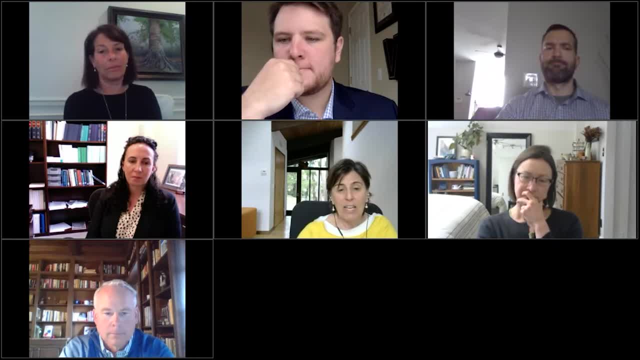 get anything built um, and i think consumer advocates like my office can play a big role in that. um last a couple years ago we launched an educational campaign specifically about iso new england um and to sort of enhance knowledge um in this state about what it is and why it matters. 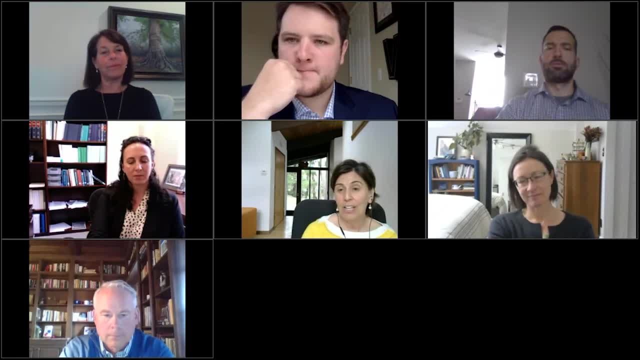 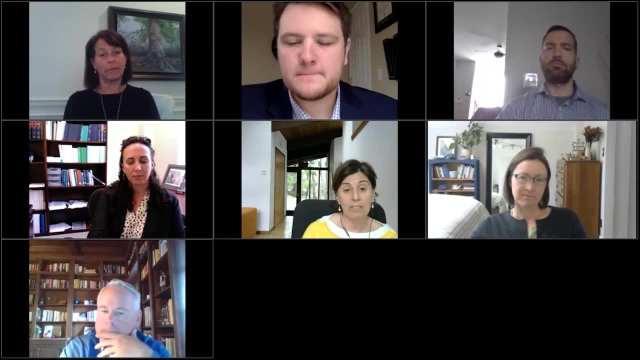 and we, we, uh, we released two videos that we put on um, that we put on facebook and twitter, um, basically explaining the issues, um, for people who aren't, you know, seeped in this stuff, and i was told when we were doing the videos, it has to be that a fourth grader could understand it. 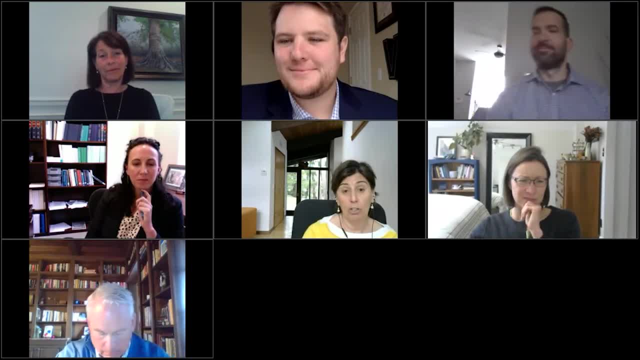 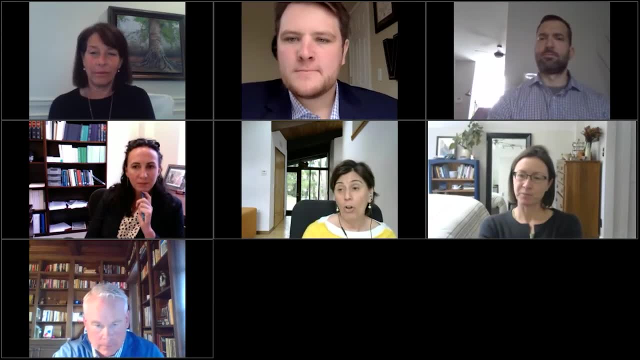 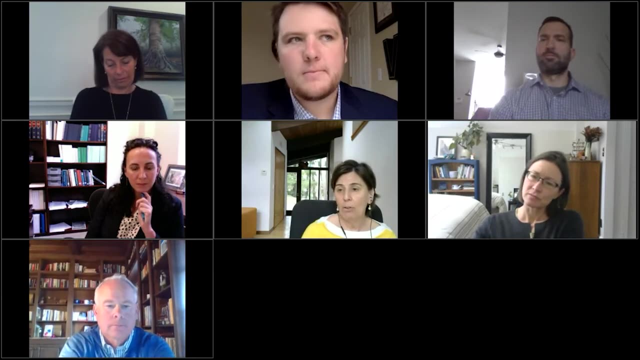 and that's what we did, um, and we had a lot of people watch it, and what we did was we followed that up with a day-long teach-in that was attended by about 300 people. that talked about people in my office. each person got an uh assignment and about 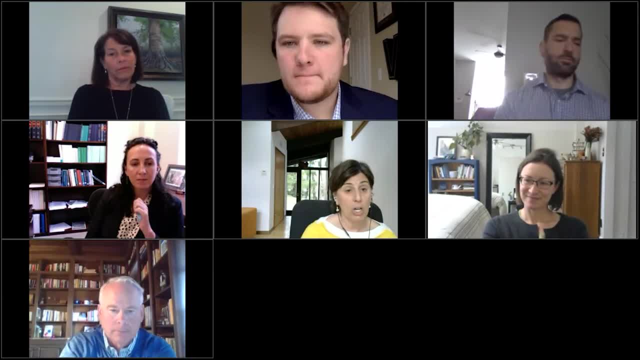 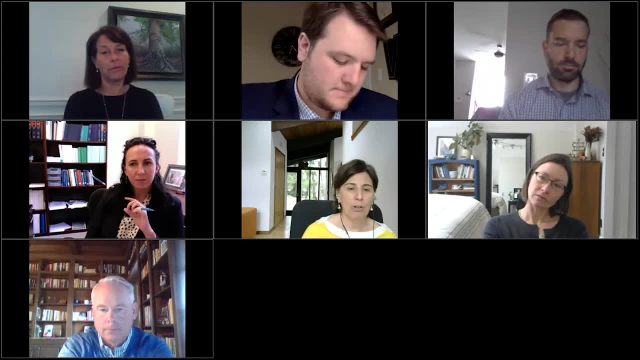 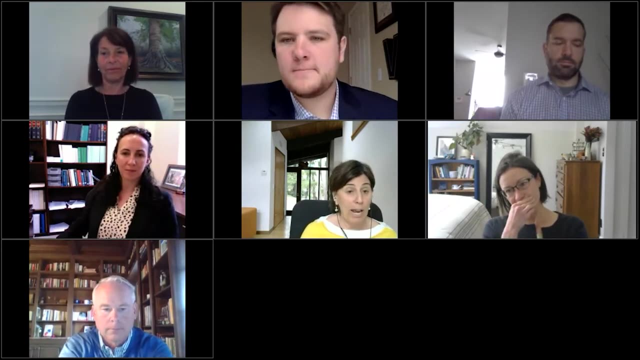 about iso new england and they, they gave, they taught about it. um, it's just too important what's going on in those rtos to leave to a group of industry insiders. we really do need to level the playing field by providing, providing consumer advocates with the tools that they need to meaningfully participate. 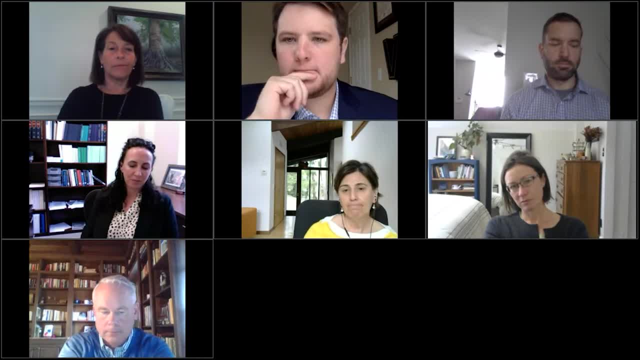 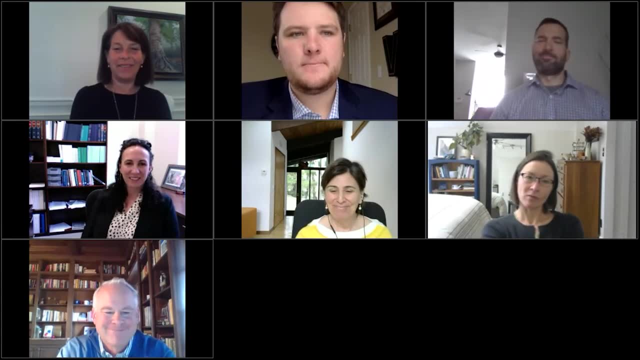 and to bring in a broader group of voices. that's all i have. is that it? that's great. okay, i have some follow-up questions on that as well, but i want to give shelly a chance just to respond to the comments that she's heard. maybe take five. 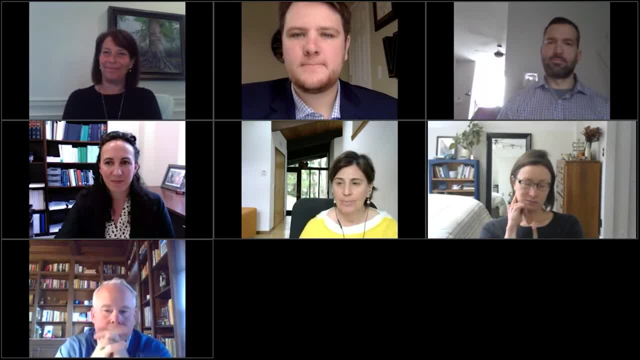 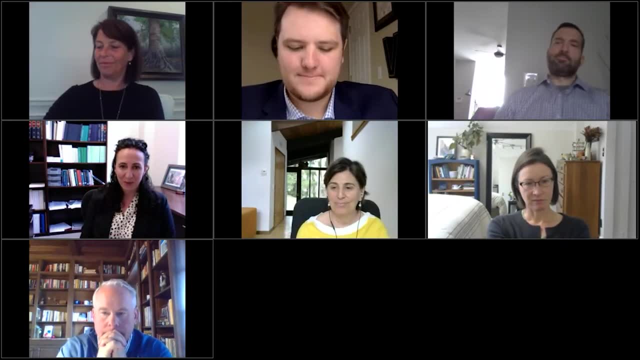 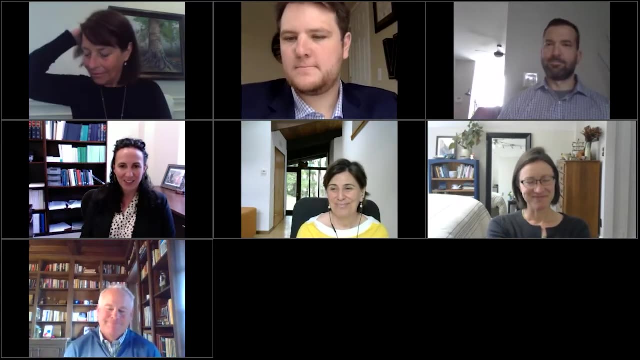 minutes and then we'll take a couple of questions and wrap up. that sounds great. thank you all so much for engaging so hopefully, with the project. it really means a lot to me. um, it's like very energizing for going forward with this kind of work to hear that it's kind of making the rounds like it. 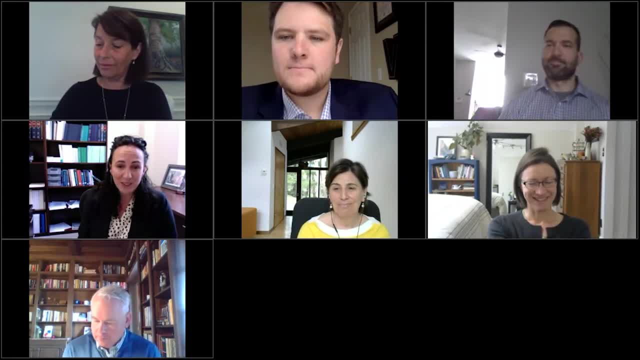 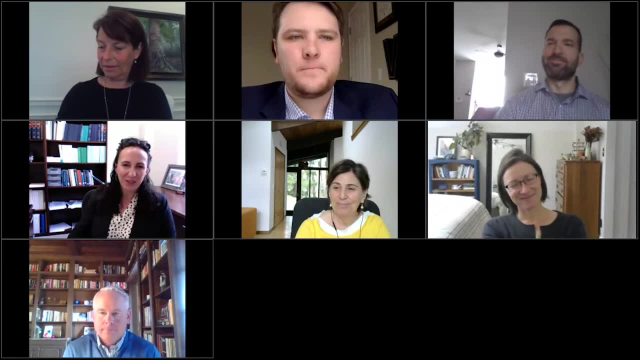 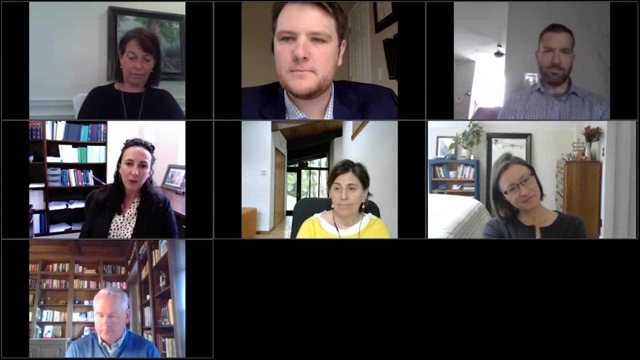 it. i i think often that i'm writing into a black void, and so this is like the best thing that could happen to me, so i really, really appreciate it. um, i just jotted down a few things that i thought might be like interesting places to go with this um one. i'll say i really do like i feel like i've. 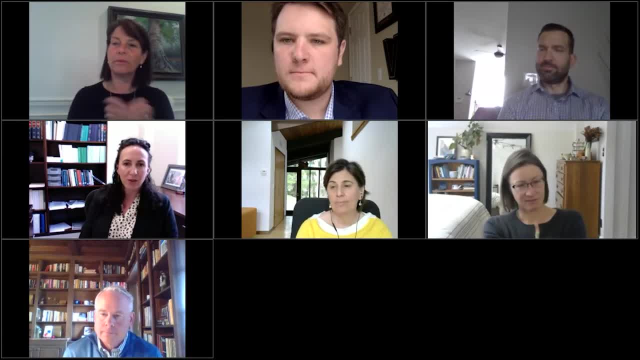 fully appreciate the points that rtos are better than non-rtos in terms of a space in which to hatch out these challenges. um, i guess part of why i was moved to do this project, though, is that, like, i feel like that is offered as a defense a lot of times for rtos. 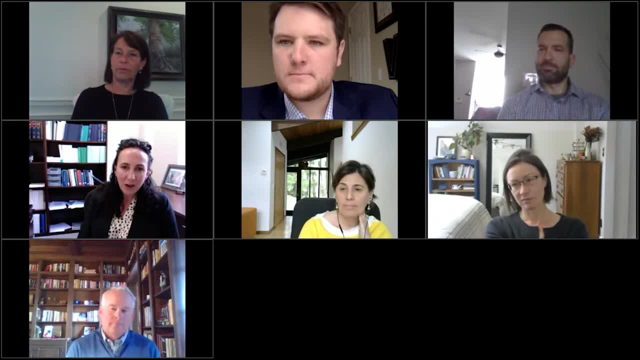 and like sure you could say we're doing better than the south, but like that's not much of a defense right, like that's a very sort of low bar, and so i guess part of what i want to do is really push rtos to be the best version of themselves, in no small part because i do think, if 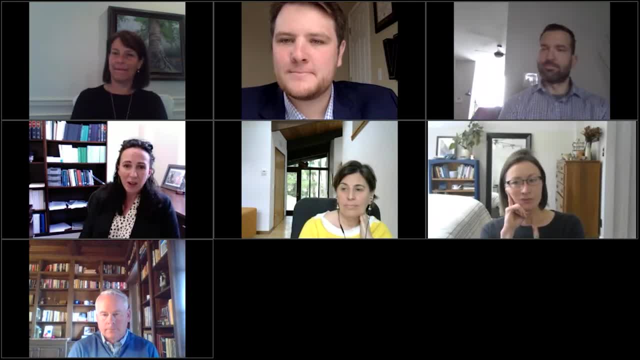 we want to get all these regions on board with rtos. the governance questions are actually huge here. right like the challenge of making a bigger western rto has been dominated by governance concerns, the southeastern proposal, um, anemic though it is, is like the south's version of doing. 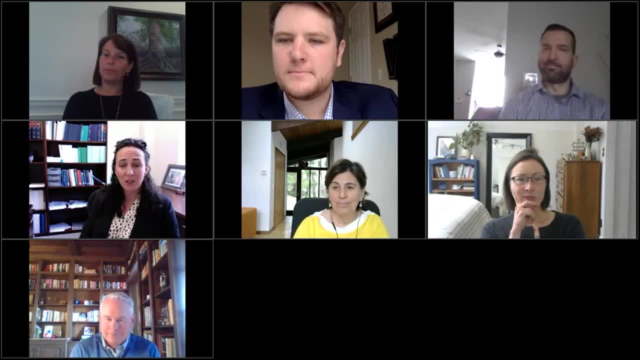 rto governance that they can stomach right, like i do think governance issues are going to be front and center to getting broader buy-in to markets as a solution. um, so you know, i think i think this is i really appreciate sort of like the nuanced conversation that we're diving into about how exactly to do that. um, tom, i think you're. 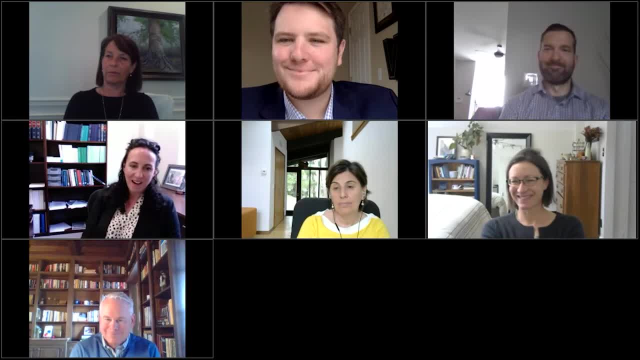 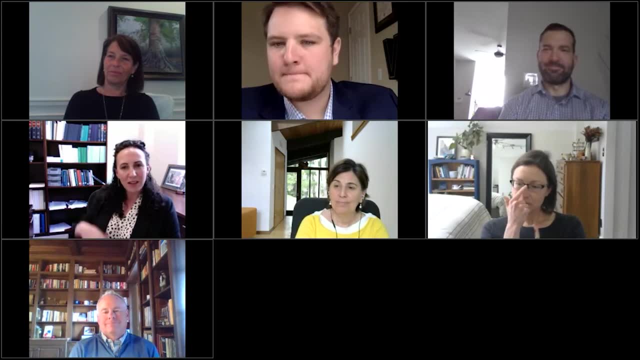 right. i really would like congress to do this too. um, i think the charge act is interesting. the question that i have about charge that i would love to hear your thoughts on. so i've also, contemporaneously with this project, i've been doing a project on the south and why they didn't. 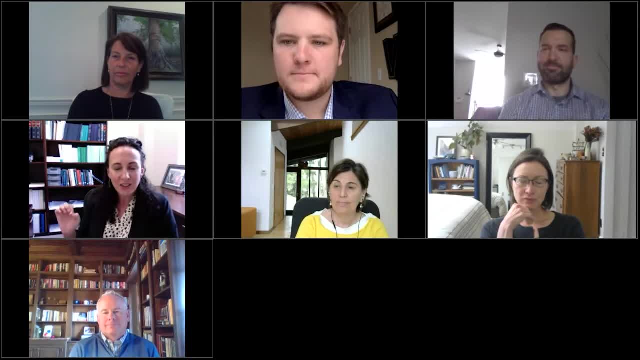 have a standard model and sort of the story behind that. the key thing that the southern states all did was they formed essentially an advisory committee to study the problem, and that's where the problem went to die. so i guess my question with the advisory committee is: do you really think it has the teeth that that it needs to do what we need to do, or is it like? 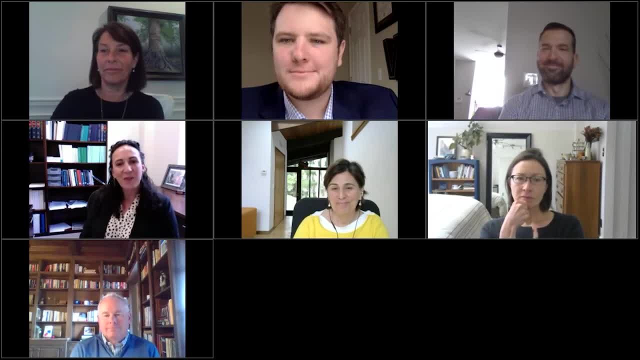 really sending the problem to die. um, and you know then. one other question for the broader group is: i have really wrestled with the question of whether or not FERC should just use its authority to say it has the power to require rto membership and do it. if you made rtos mandatory and then you 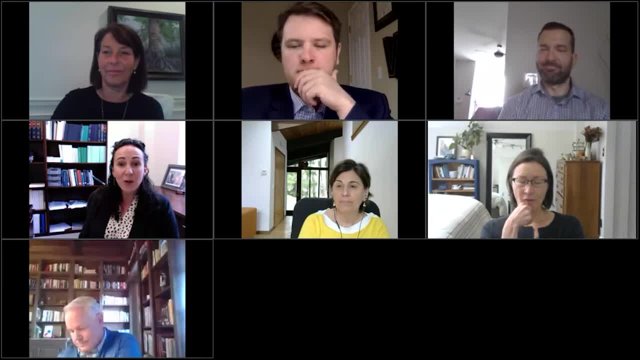 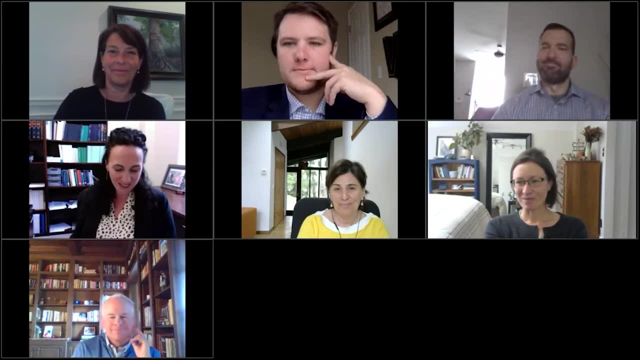 did rto reform, utilities couldn't walk anymore. now i know that this is like both politically and legally explosive, but i wonder what your thoughts are about it if we can't get it through congress. um, and then casey, i really appreciated your points about sort of like soft power in rto. 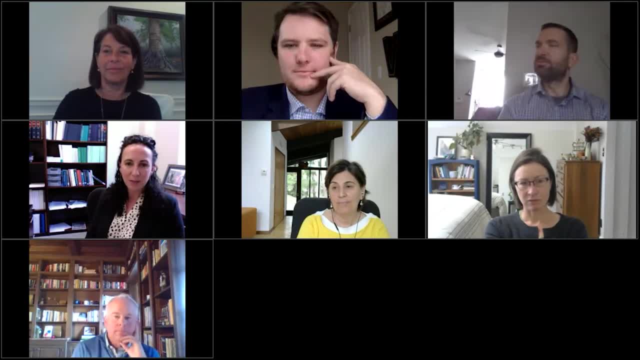 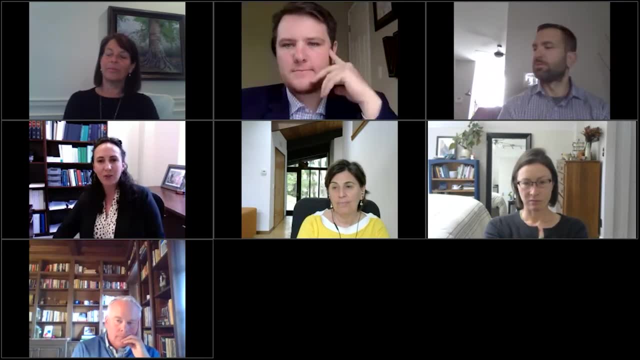 i think as a as an academic especially, it's been a long time since i was on the inside of rto stakeholder processes and i don't see the soft power at work as much, and so, as i've gone through this project, i've had a lot of interesting conversations about how the power is greater. 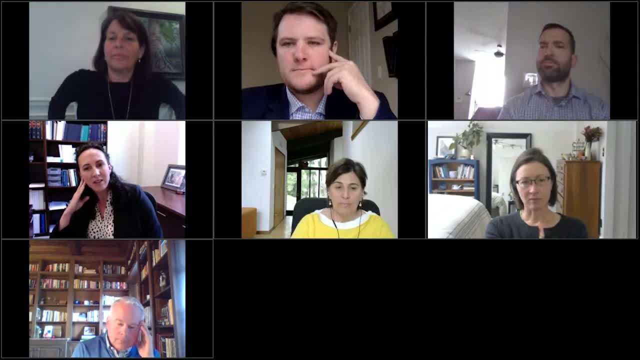 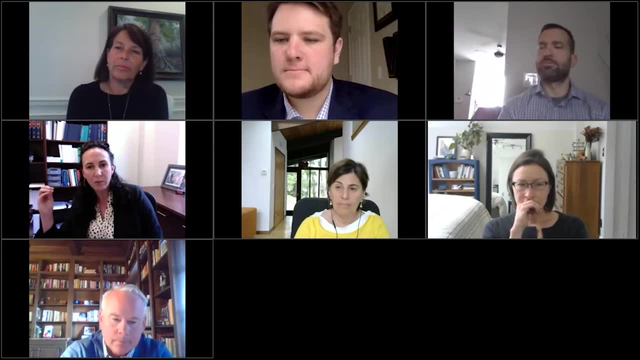 than it would look like. if you're looking at overarching frameworks, i guess the one thing that i would say is that, you know, i think it's imperfectly theorized, but there is a clear relationship between hard power and soft power, like the more hard power you have, the more. 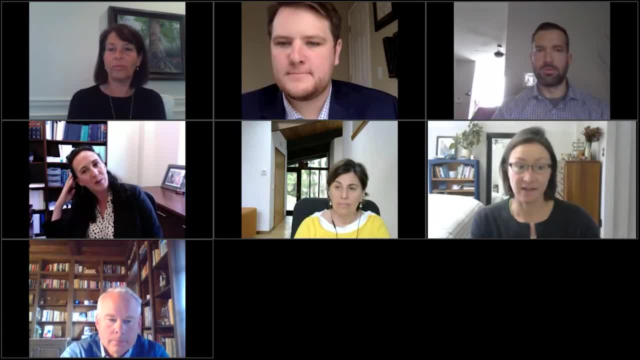 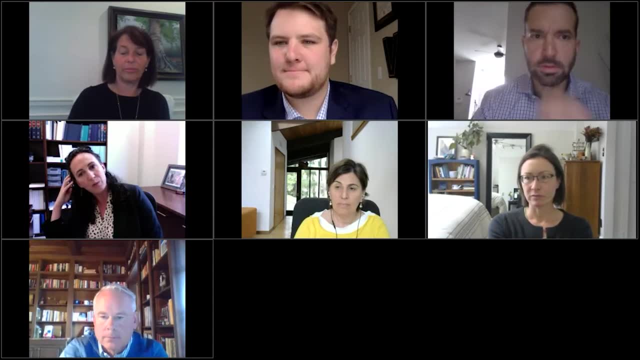 soft power you get to push solutions, and so, like i you know, i don't want to um be insensitive to the ways in which this process can move within its bounds. but i also think moving the bounds changes the relationship of sort of like how soft power can work in the system too. 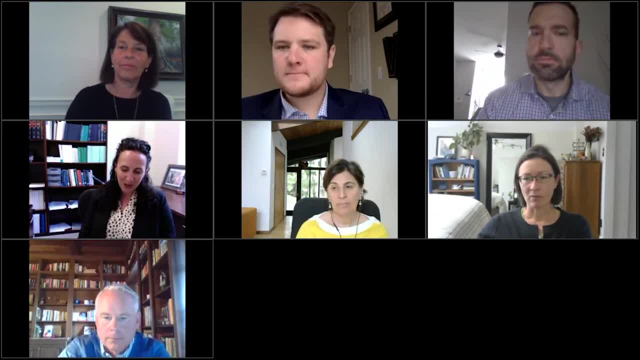 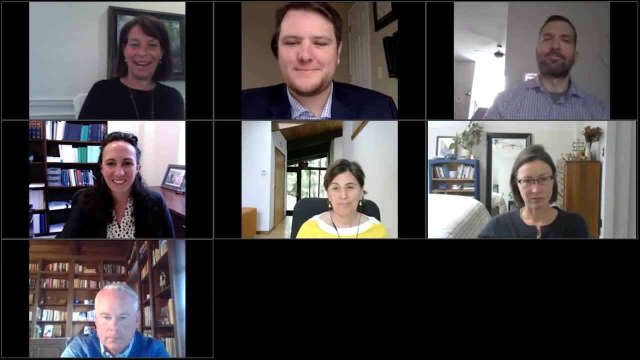 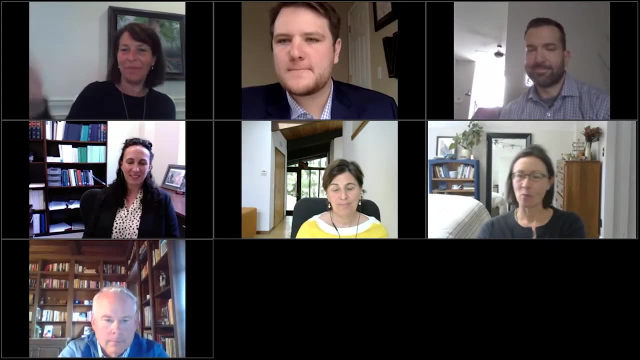 um, so i'm curious what your thoughts are about that. um, okay, i think that's about it for now. let's leave it there. i think some of this dialogue may have to happen offline. after, after the panel, um tom, uh, or well, any of you, do you want to jump in response real quick to shelly, and then we'll. 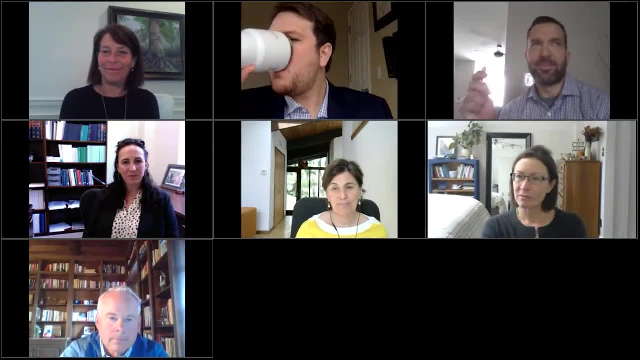 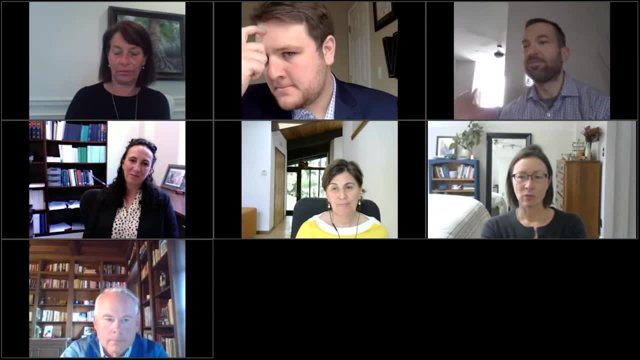 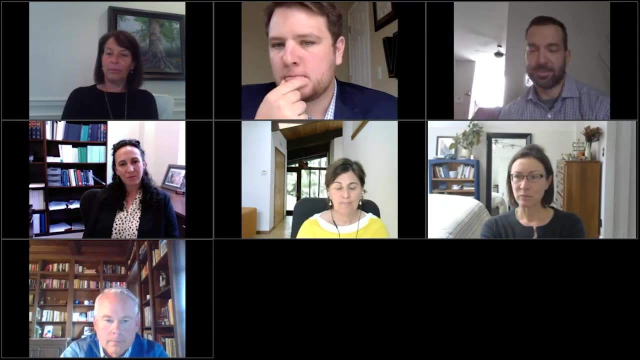 go to a question from joe. yeah, i can be super fast. number one: um rto mandate has risen again. when recent the clean future act, there was a provision um, and some of that has been informed by the committee's history. you know, energy and commerce, as i said, had a lot more kind of push. 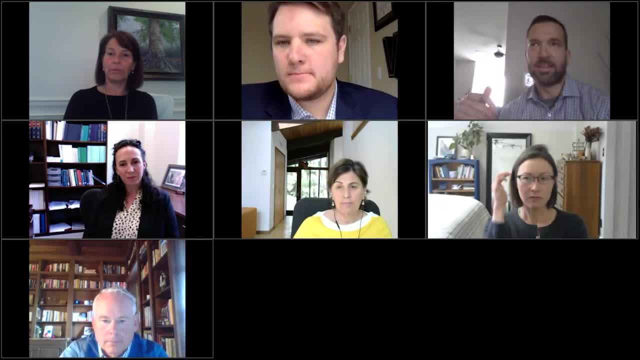 it obviously did not go anywhere, neither did that piece of legislation, but i think there are several um in congress who think that that's the only way to really kind of push the envelope on this. it is gonna. it is a hard, exclusive topic to address, but it's out there. 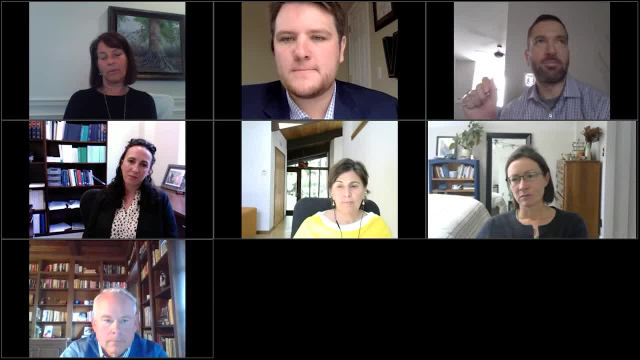 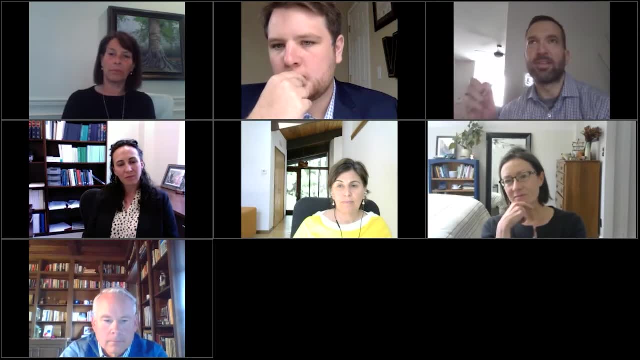 still um. the other piece on the advisory committee i think would be as a standalone item. i concur that it's not necessarily a good. you know it's not going to solve all the world's problems. i think the idea is to help take this topic out, elevate the role and the complexity of the problem, bring 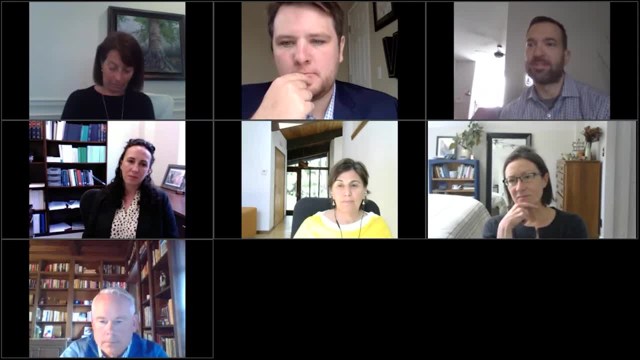 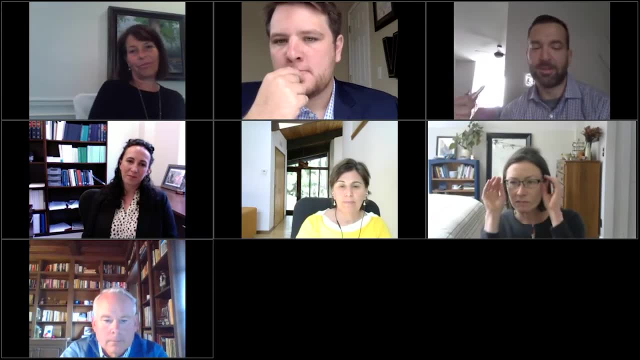 more attention to it and couple that with actual next steps. that would be enforceable, so that would have to be there. unlike a, you know, just a scapegoat, this would have to be coupled with something else, and this is where the pieces of that marky bill ultimately get the idea to break some of those pieces up, find more. 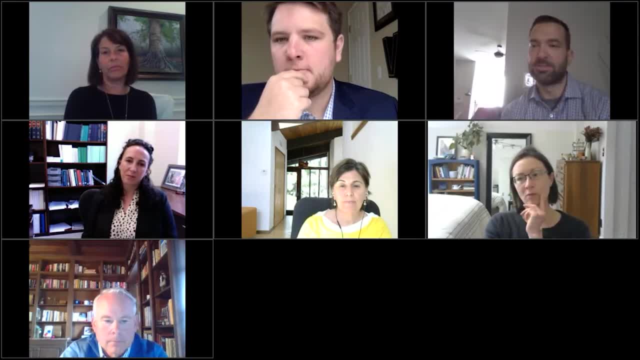 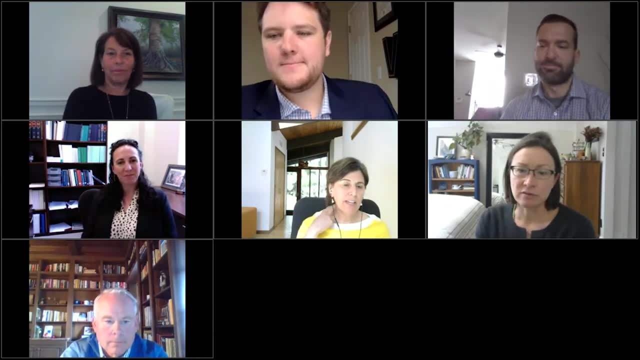 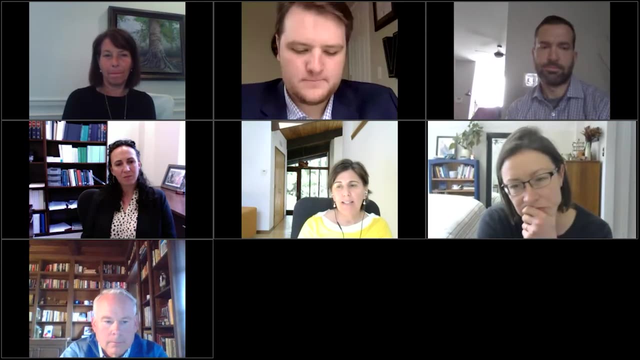 bipartisan support and then move some of that as standalone pieces. so there's some more in the works behind the scenes on that. yeah, can i just turn one quick thing on the? on the other issue about the soft power, i actually have real concerns about the RTOs board and staff having acting as policymakers rather than regulators or 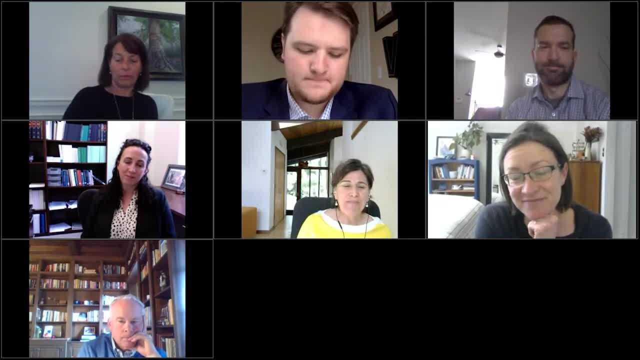 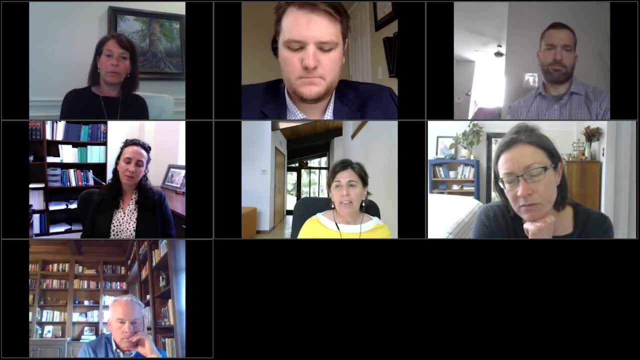 whatever they really are. utilities, I guess, is what they are legally. But there's, there's a lot of. I think Casey's right. they care a lot about what people think And they come up with their ideas and then they're out pitching them. You know they are talking. 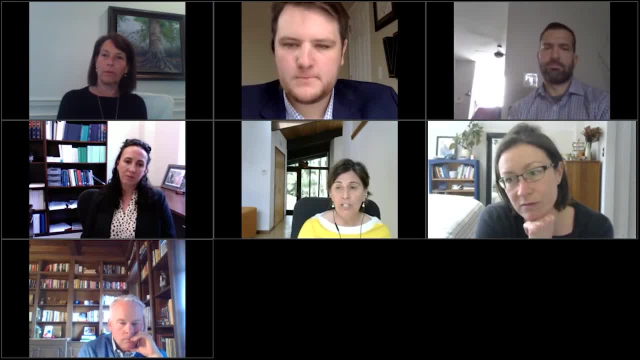 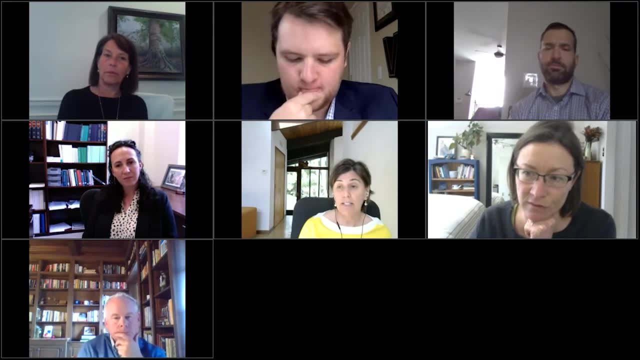 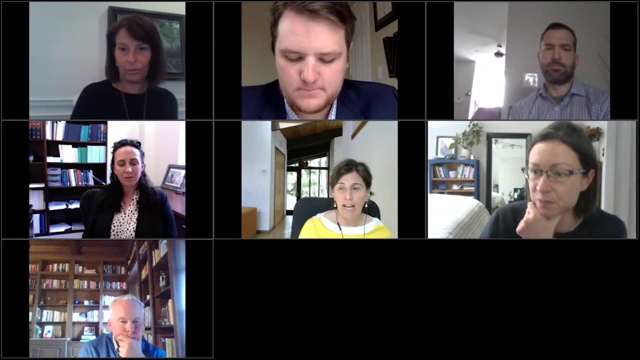 to reporters, they are at conferences and they are pitching their ideas And even if it's, even if the stakeholder process isn't necessarily along the same lines, and they do go to FERC before their filings and they talk to FERC about their filings and FERC. 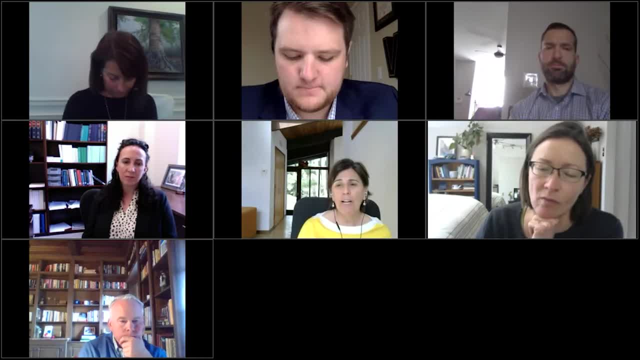 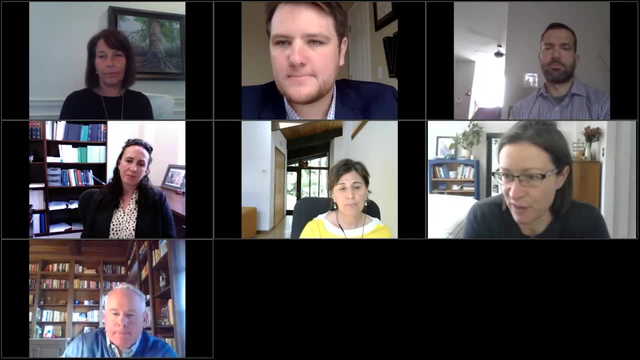 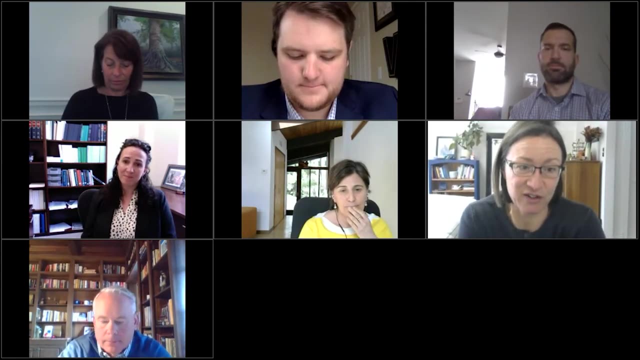 gives them a lot of deference. So I worry about that. Yeah, I wanted to add on the, the RTO members. I think that's a really important membership mandatory versus voluntary thing. But there are states that have mandates for their transmission to be members of RTOs right, Ohio and Virginia. 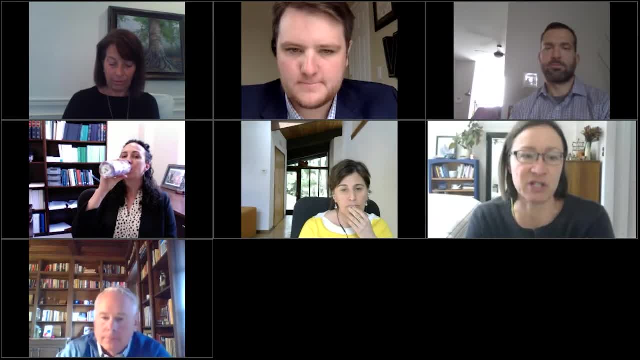 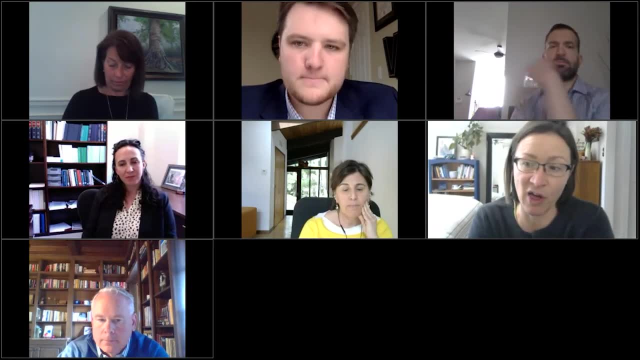 come to mind, and most of those were put in place sort of during restructuring, Um, and I think that would be an interesting thing for states to look at going forward, And it pains me to say that as somebody who has more recently advocated for states to leave RTOs. 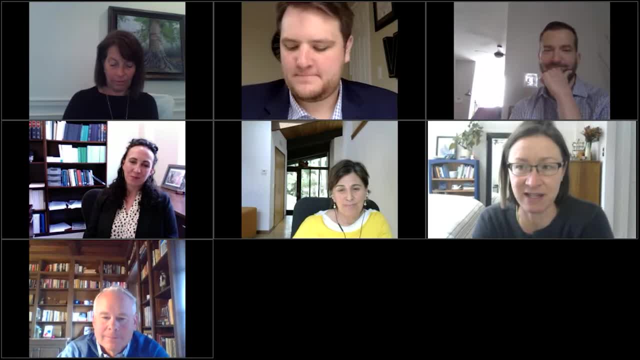 or to have their- you know, transmissioners leave RTOs because of things like these capacity market rules that are so important And I think that's a really important thing for states to look at, because these things are so adverse to state interests. So I would 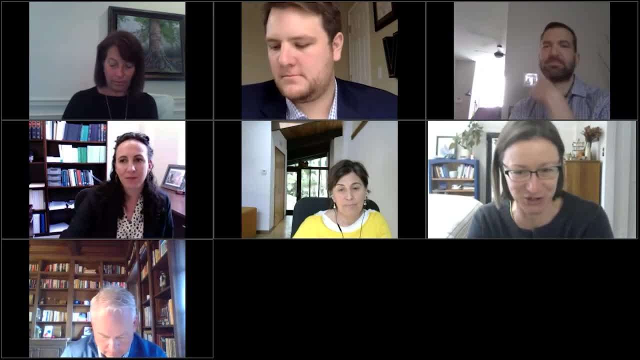 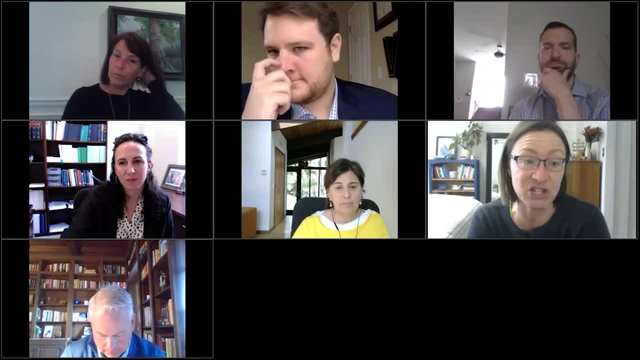 say, I would encourage states to explore that as a sort of conditional requirement of something was sort of continued oversight as opposed to a one time you must be a member. but I think states can really change that balance of power, Um, and that that that might be. 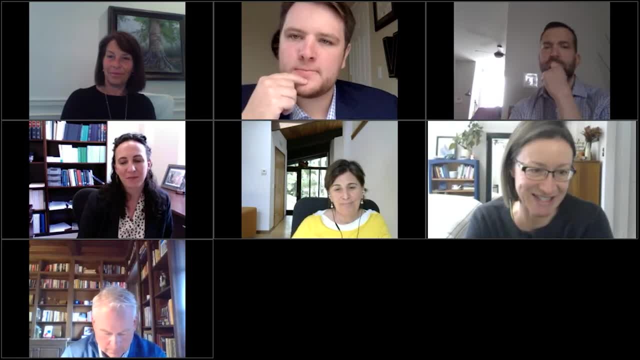 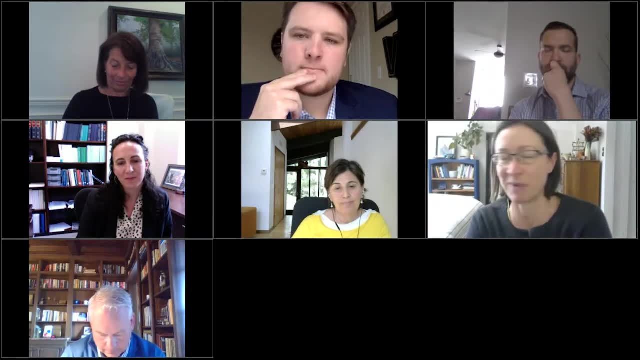 helpful to pursue. So, And on the soft power issue, Yeah, I don't want to overstate kind of what can be achieved simply through, you know, well informed and resource consumer advocates helping to shape the agenda or get media attention right, like that's no substitute in the 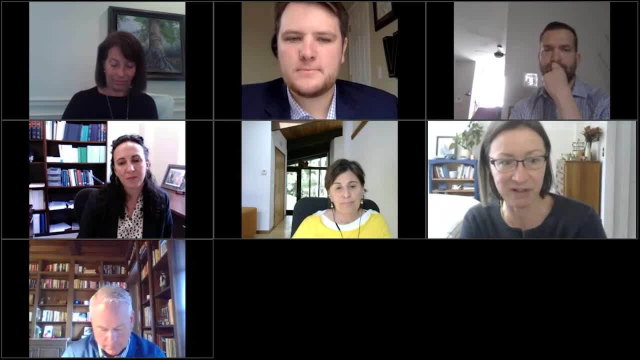 end for sort of voting power or, you know, some ability to directly influence section 205 rights. but i think that in the meantime it can, by expanding the capability and drawing more attention to the issues, it could make it easier to get to that step of getting congress to act. 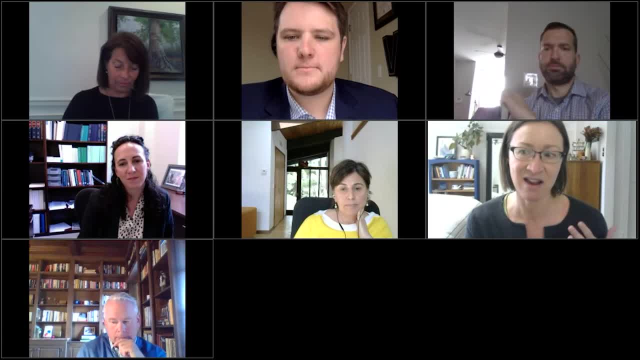 on it because you've sort of demonstrated how important these things are and how much more effective and, um, effectively- those processes operate when consumer views are incorporated at the beginning, instead of just having to raise objections at the end. so i suggest it is like: uh, maybe a step that will help us to get to deeper reforms, as opposed to an end in itself. so 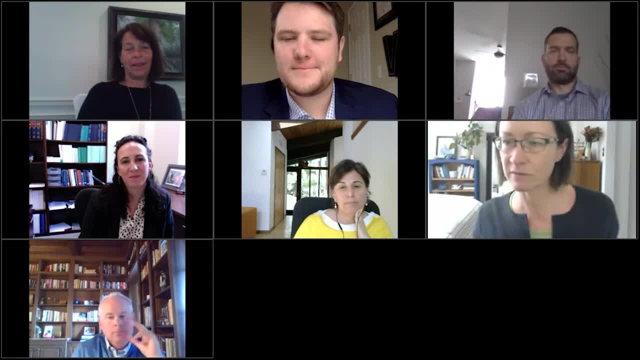 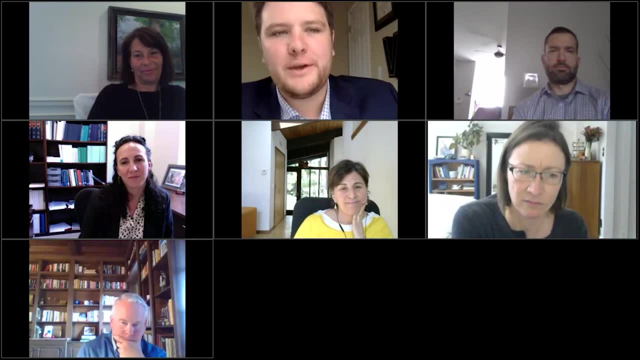 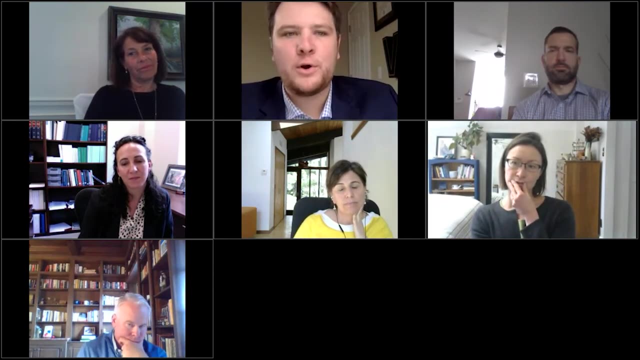 yeah, uh, thank you all. joe, do you want to ask the uh panel a question? sure, yeah, this would be primarily, i guess, for professor walton, but then anyone else who wants to jump in. um, but the article discusses multiple pathways to better grid governance, including paring back rto authority, increasing regulatory oversight, better policing. 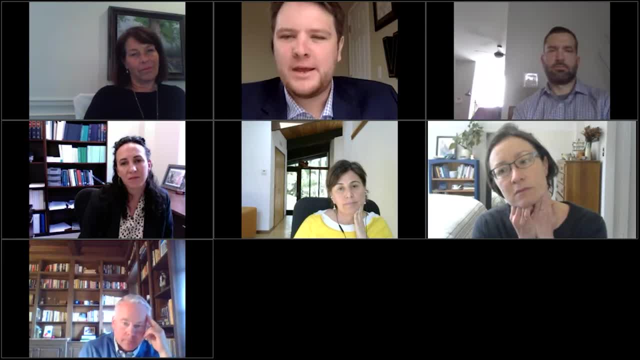 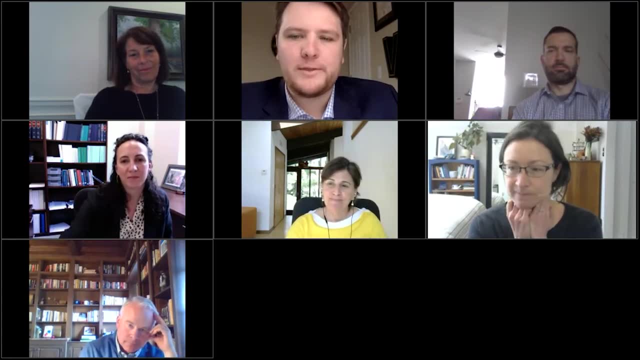 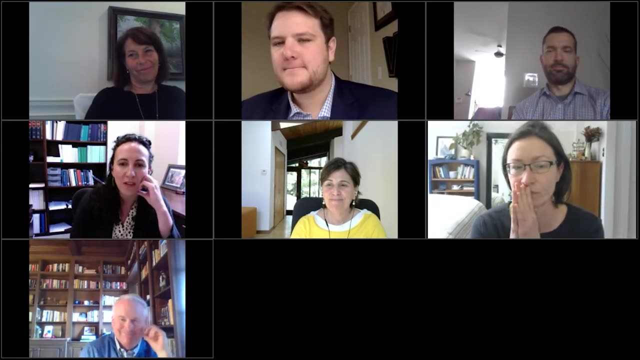 sectoral corporate power and considering a public option of these potential solutions, what's the most feasible in the current climate and could provide the most immediate benefit of reforming the electricity sector? yeah, you know, joe, i really appreciate that question because i think we have focused almost. 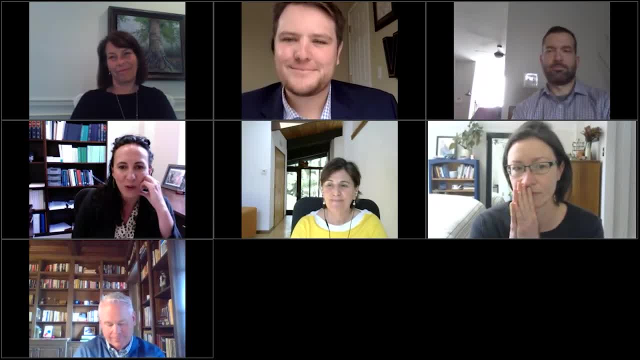 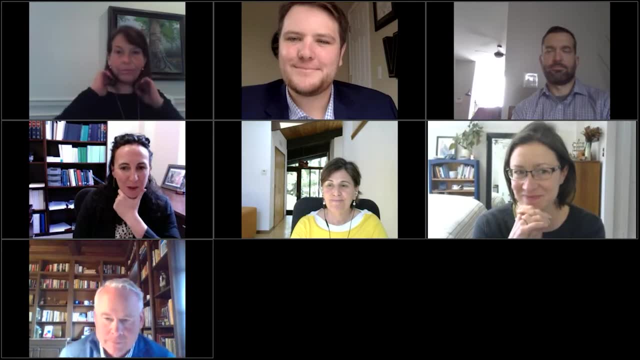 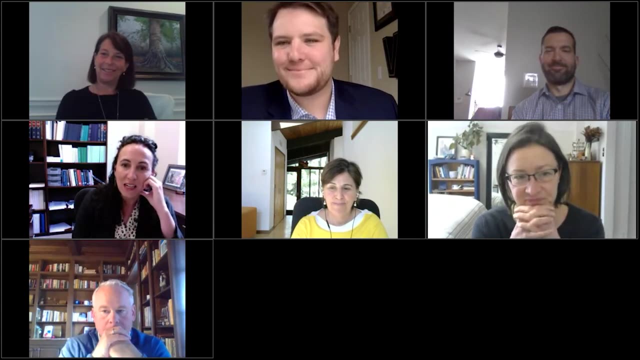 exclusively on. what is it? option two, right, which is like oversight mechanisms for rtos, and very little on the other option, um, which i think probably is an answer to your question in and of itself, that we've all sort of honed in there, um. but i'll just say: look, i do think 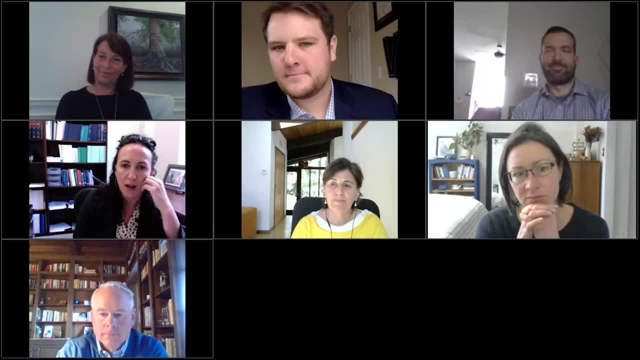 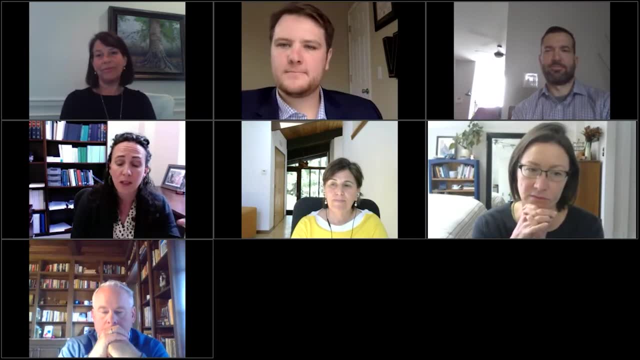 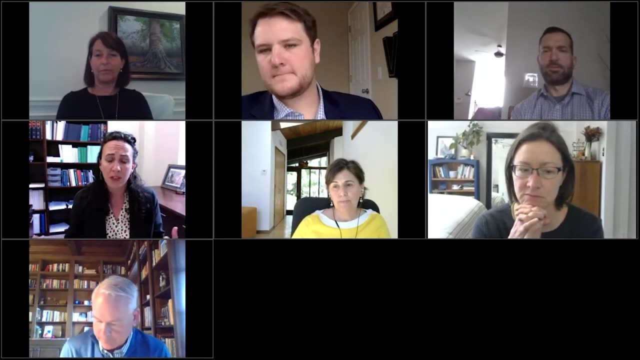 one of the things that came up when states were um particularly upset with the eastern rtos and were threatening exit was: maybe you don't do a full exit, maybe you do a partial exit and sort of claw back some of the authority that rto has taken. but you actually really want most notably authority. 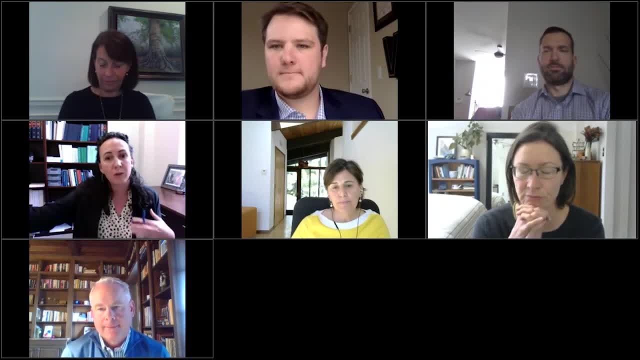 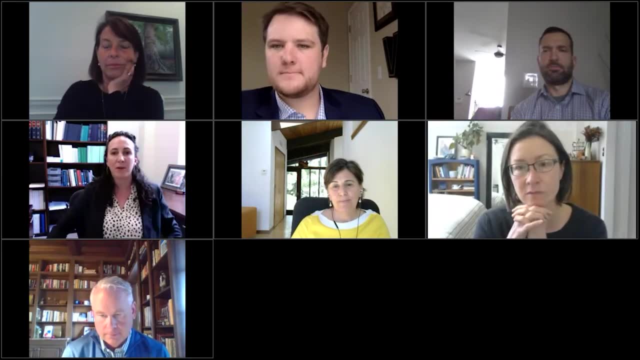 over resource adequacy or like: what resources should we be building in the future and how do we decide what resources those are? i don't think that's a totally implausible pathway to go down going forward, but i think it's probably less likely than sort of playing in the land of reform. 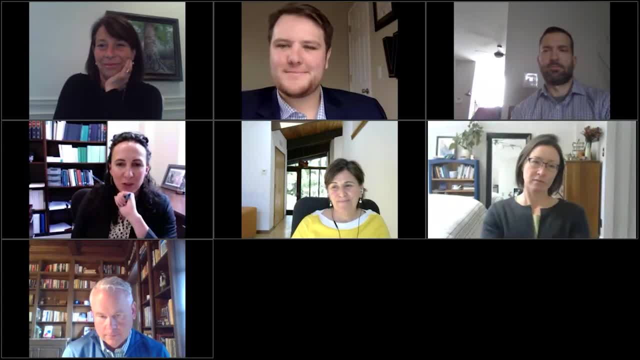 i will, though, just put a plug for thinking more about sectoral consolidation as we think about these issues, right like. i think that these topics are. these topics aren't talked about enough together, but it's so striking to me that, in the 1990s, at 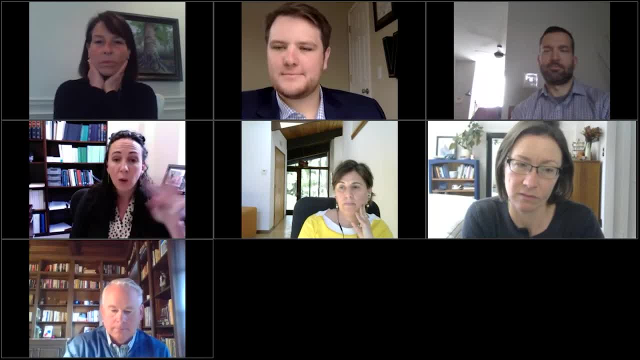 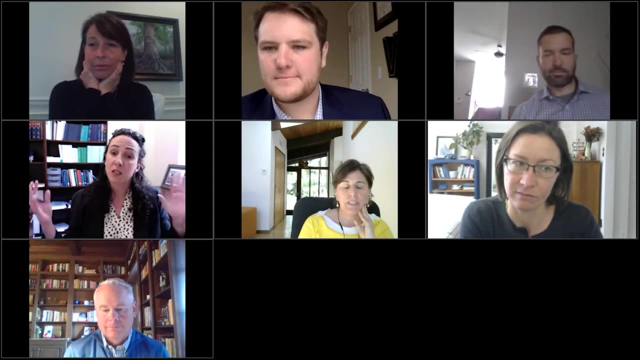 the exact same time, that congress was like, hey look, we can deregulate this sector because, look, competition, right, competition's going to solve our problems. you'll have, you know, the industry checking the industry, we've got generators that are going to be separate from utilities, and so look like. 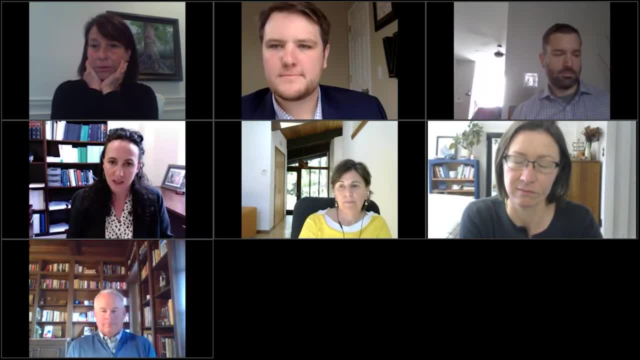 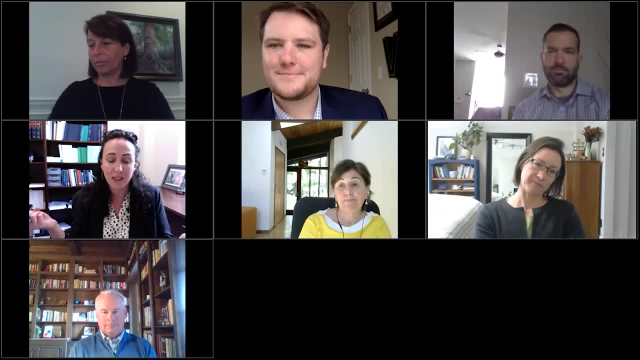 let's use competition to drive low prices in this sector. that's happening on the one hand, and on the other, they're lifting the prohibitions on utility mergers that have been in place for most of the 20th century, and so you see massive consolidations happening. so, like the theory of what's supposed to, 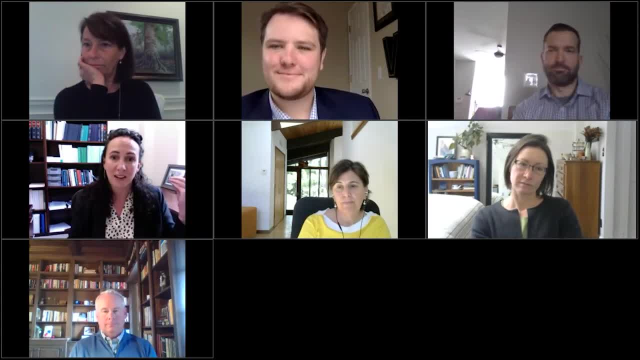 be checking us today. competition has actually evaporated at the same time, and so like maybe FERC should be going back and thinking about its merger policy, maybe congress should also be, and i think congress actually has some appetite right now for thinking about, um, the woes of massive 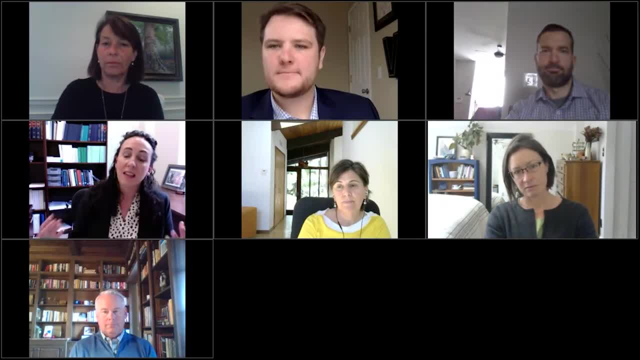 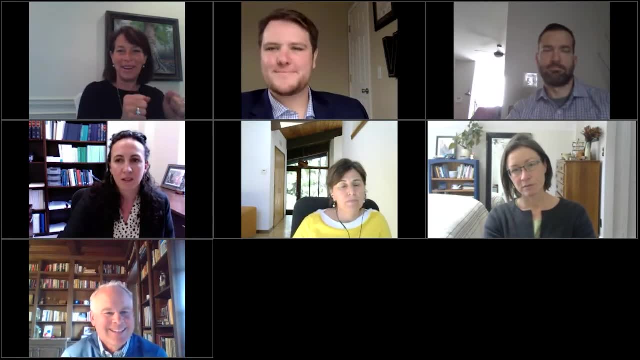 inflation, which obviously is never going to come. but i would say, trust me, the business structure of what's happening in that sector is really important. you know, i think it's, you know it's going to get better for everyone. but i think the thing that's really important to think about is 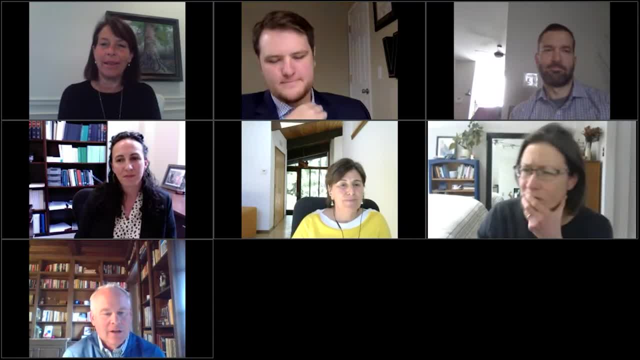 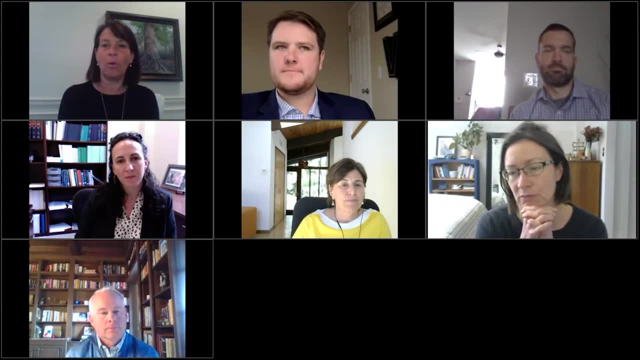 um, is this? um, you know why is this happening? i think this is one of the reasons why we're having this kind of shift in the industry, where, cuz you know, people think that what's happening isn't as good a thing, and i think we're going back into the digital mold of where on the internet. 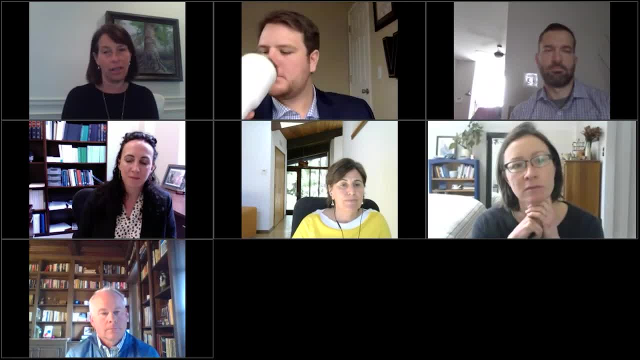 in terms of, uh, you know the, the politics are not the same, but that there's a lot of stuff happening at the same time, and it's very- it's very interesting to see where you take that, and even for people who work in this area, right? 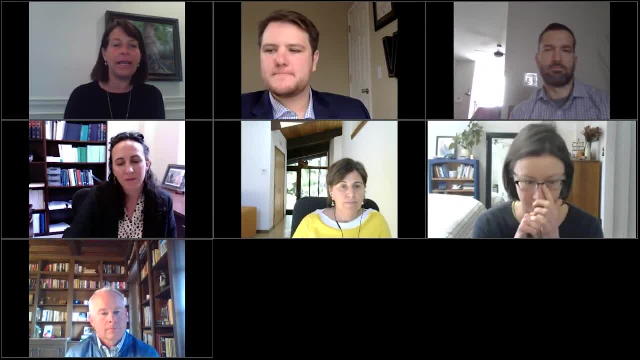 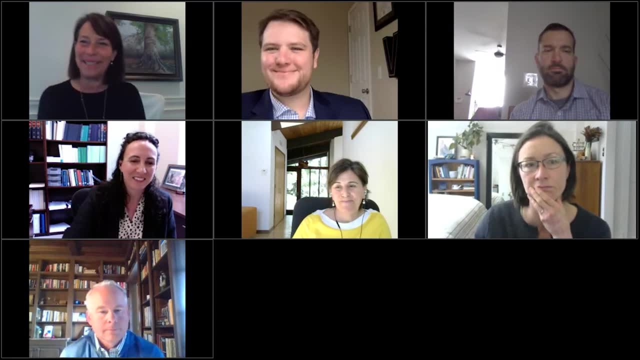 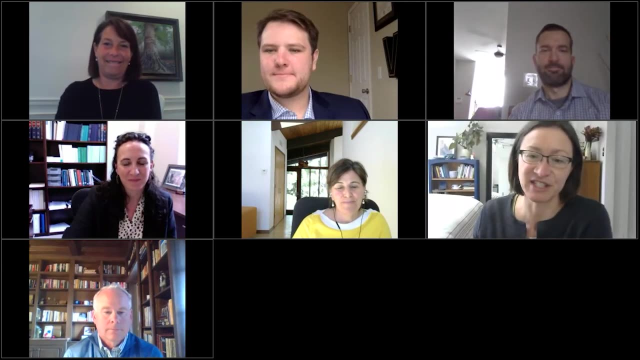 So, Rebecca, you offered a few ideas of things you guys are doing. If there's anything you want to add, great, Would love anyone else's perspective and maybe like in 30 seconds each, so we can wrap up on time, I'll just say the video. 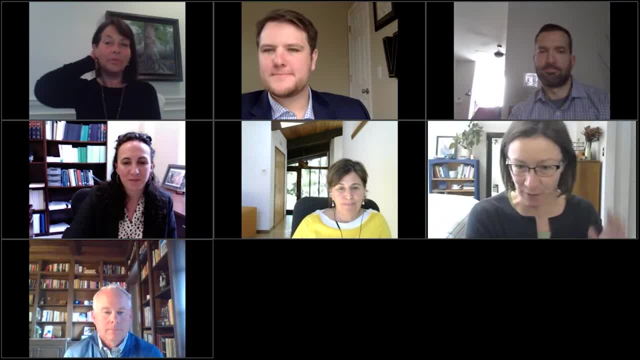 that the Massachusetts Attorney General's office put together in that teaching were amazing And I forward them to people all the time as like a quick explainer. So thank you so much for doing that. I do think better resourced consumer advocates and other sort of state entities. 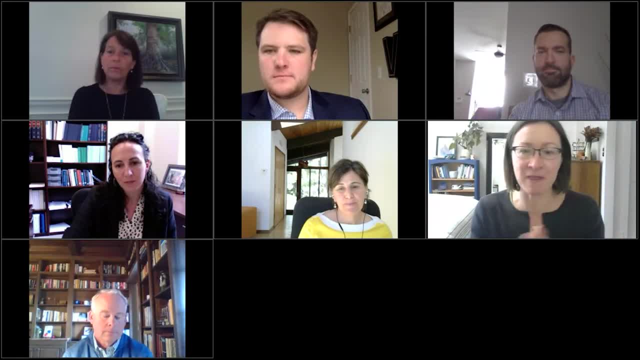 they can not only engage in the stakeholder process more effectively, but then they can be those messengers to the public. Most consumer advocate offices have like one person covering all these meetings and probably some state rate cases too. They don't have any time left to serve. 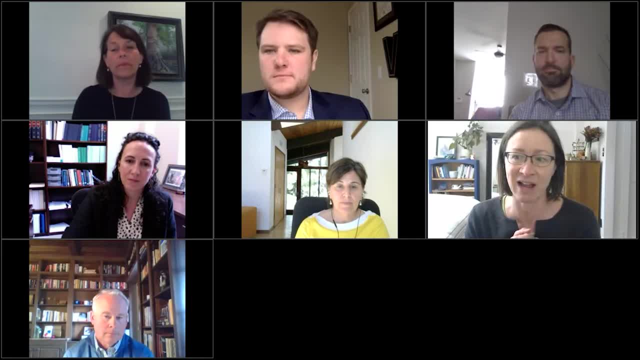 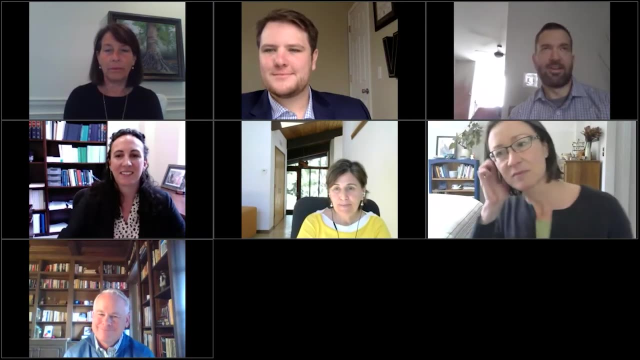 as that kind of public liaison role, And so I would say that's the one thing. It's better resourcing all of those offices so they can help to take that message to the public. Oh, go ahead, Tom. No, I concur. 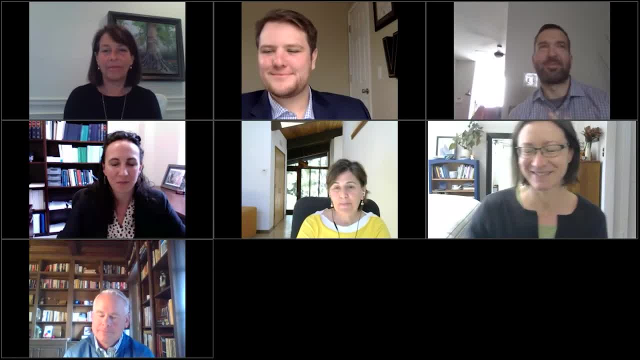 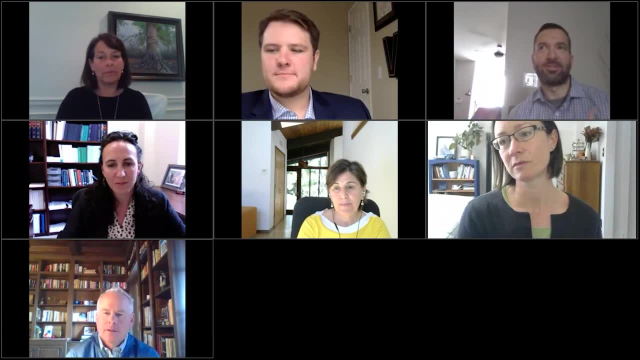 I don't really have anything other than like communicate. you know active customers, you know the enlightened climate, conscious consumer. If you can sort of mirror the opportunity between the retail wholesale side, I think there's one way to get them to care a little more. 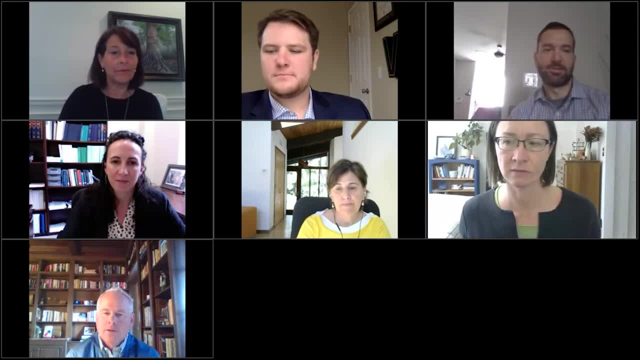 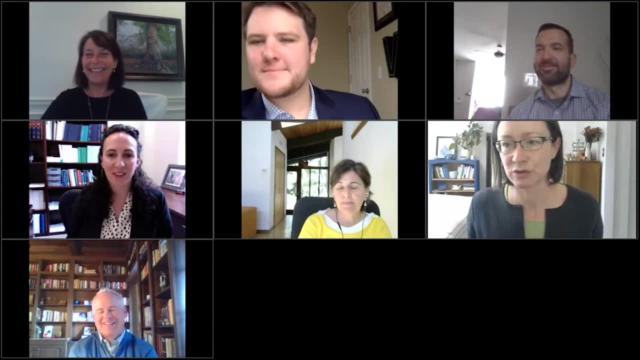 So that's my big picture observation. Rebecca, did you have one other thing you wanted to say? No, that's right. Hey, I'll throw one more thing out there that I think everybody should be paying attention to going forward, which is that, in addition, 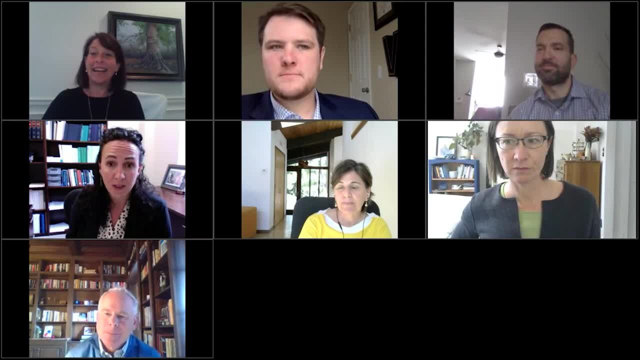 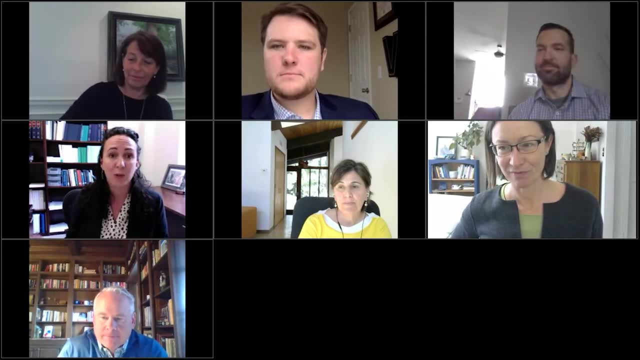 to everything else going on at FERC. they're right now charged with creating this office of public participation. It is a feared experiment by Congress. They have to do it, but the idea is to do exactly this, exactly what Linda's suggesting. 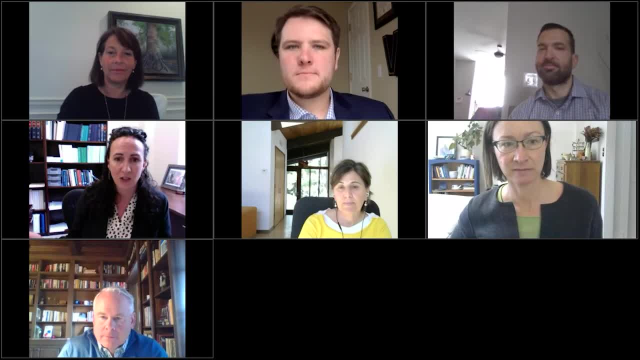 is figure out a way to engage publics that have not presently been engaging at FERC. It is going to be a huge lift. I don't think they've figured out exactly what it looks like yet, but I think it's going to be a really interesting experiment. 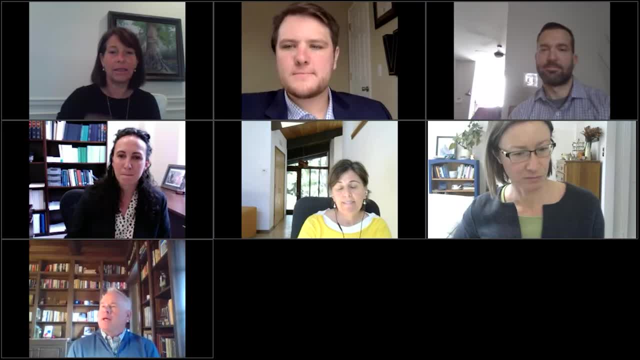 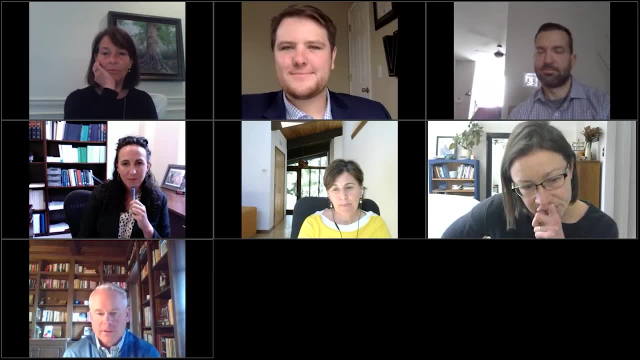 in how you do this. I wonder, too, whether, if we're really thinking about democratizing the energy system, whether we need to think a little more broadly about what's truly in consumers' interests. You know, and this is going to challenge everybody- 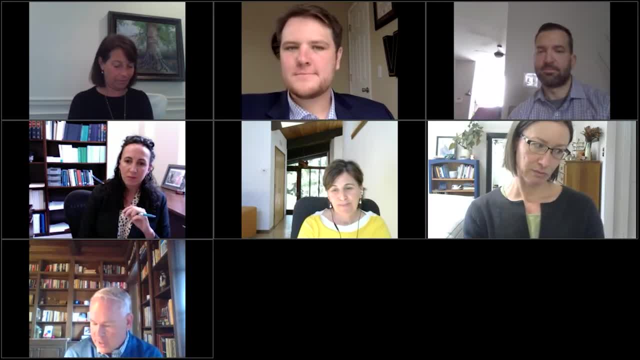 because it's a really nice thing to be able to say is is decarbonization. Decarbonization should not proceed at the expense of customers And I know, Casey, you said that that's sort of a fundamental point and I see that everywhere. 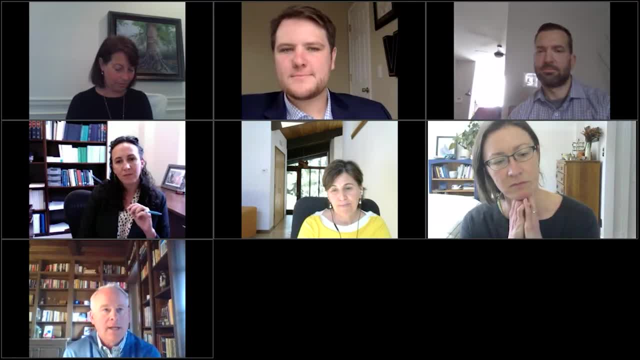 But what we saw in the last panel is something we're seeing much more broadly in society, which is that it's in shareholders' interest to get a little less return in order to avoid catastrophic climate change. So I wonder, as they build a public office, 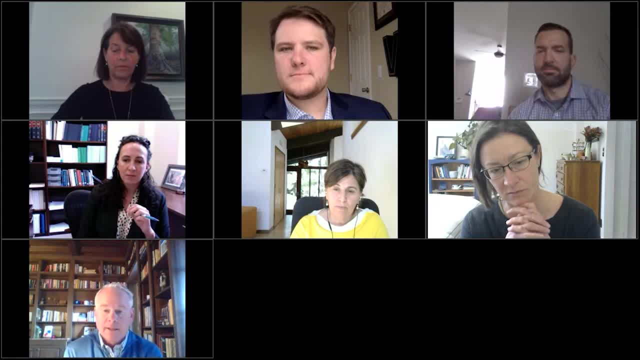 within FERC for public participation. is that going to be a good thing or a bad thing? And that in part depends on whether we help shape the way we think about what's truly in people's long-term interest, And it's not what it was 30 years ago. 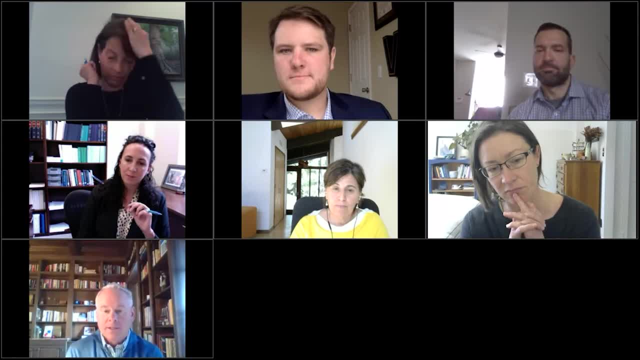 when paying less for power is a good thing, necessarily. If that happens and it creates 500 generations of elevated sea levels, that will most seriously affect those who are most disadvantaged. that's not in customers' interests. So I'm interested in whether part of what needs to be done 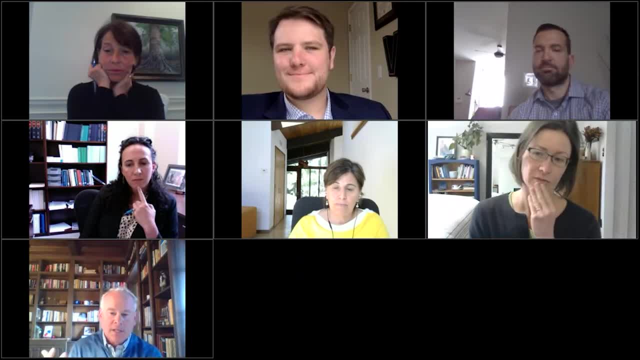 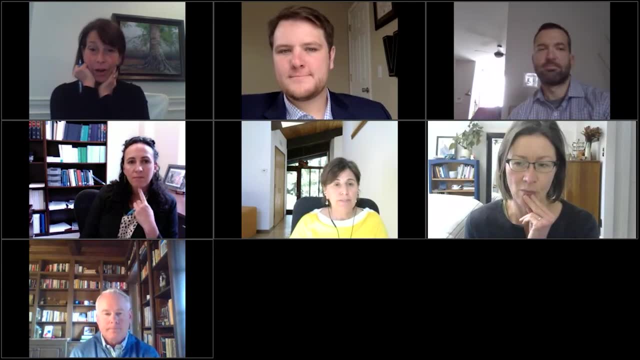 is not just simple access to the system but a reconceptualization of what we really mean by the democratic interest of the population we're serving. And on that provocative note, it's going to be a comment, not a question, because unfortunately we are out of time. 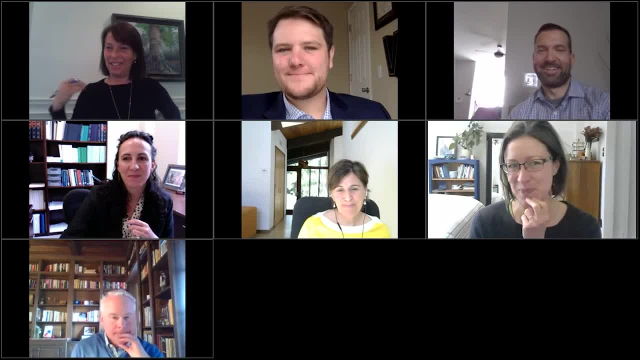 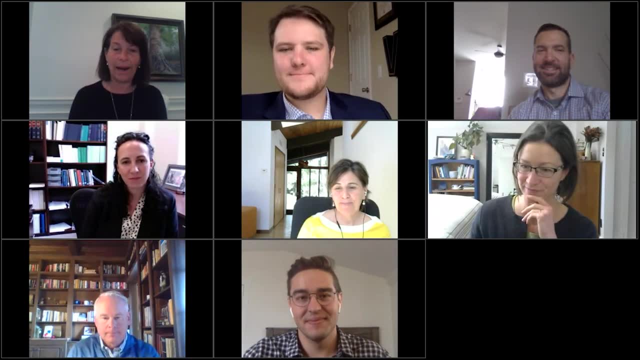 And we do have a third-year law student, Conor Feidel, who's just going to wrap things up for us today. This has been a fantastic discussion. All of these panels have been, I think, just great today. Thank you so very much for participating. 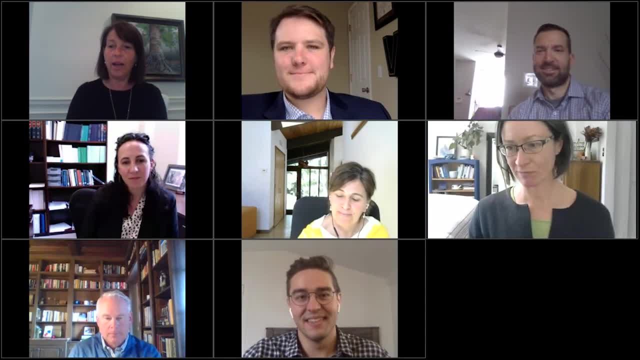 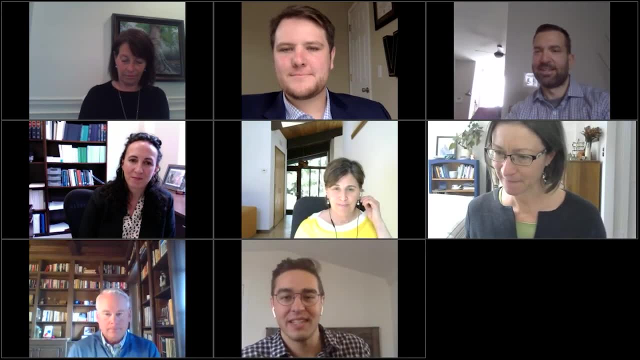 for the sophisticated level of discussion. And Conor, wrap us up. Yeah, echoing what Professor Bregan said. thank you guys so much. That was a really engaging and interesting panel And I know I learned a lot, so I'm sure everyone had a really good time. 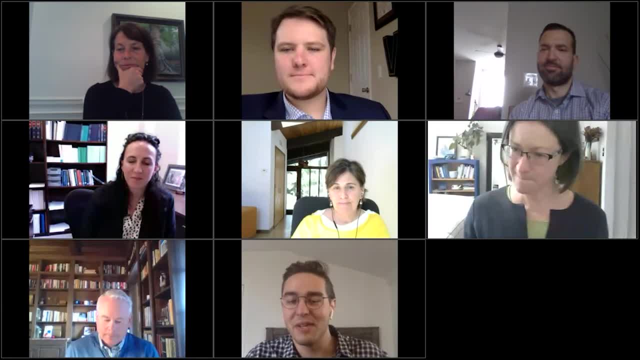 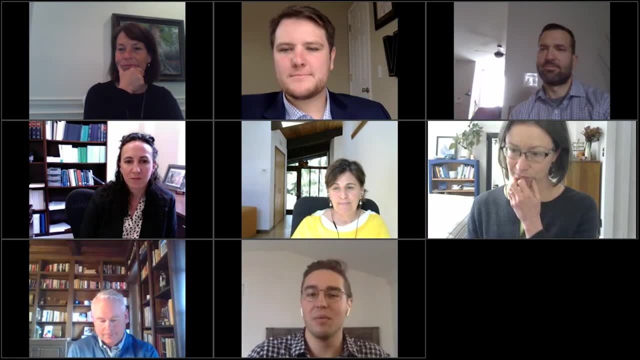 As Professor Bregan said, I'm Conor Feidel. I'm a 3L here at Vanderbilt Law School. I'm also the executive editor of LPAR. I would like to start today by congratulating the authors selected for this year's LPAR publication. 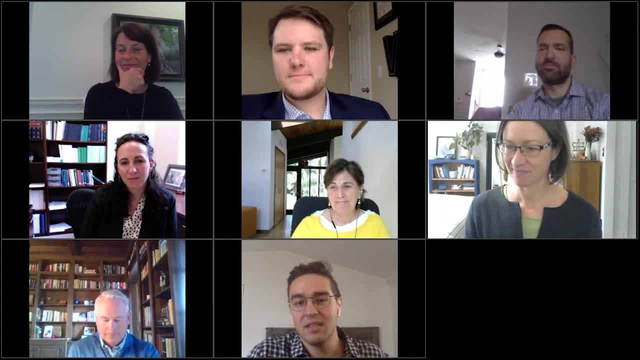 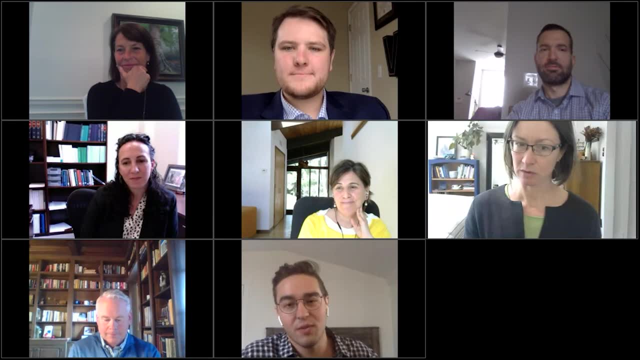 We sort through hundreds of articles, and the three that we discussed today are the ones that stood out to us most as proposing the most feasible creative, impact and persuasive policy proposals. So thank you all for your very important work and congratulations. I would also like to thank all of the panelists. 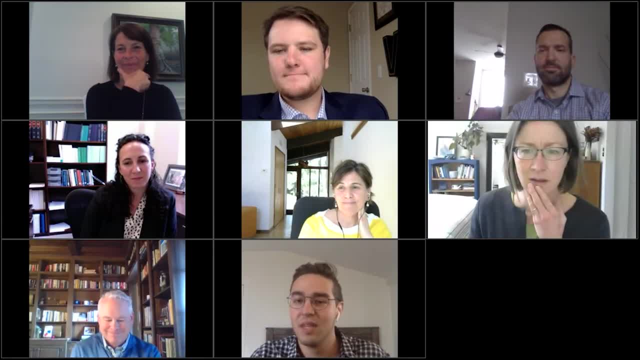 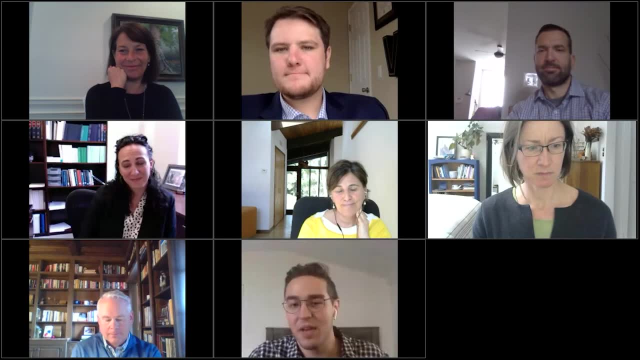 We selected these articles because we don't want them stuck in an academic vacuum. Your efforts made this possible and we are really grateful for your voices and for your time. Thank you also to the members of LPAR who coordinated this event, especially Catherine Denny, our symposium editor. 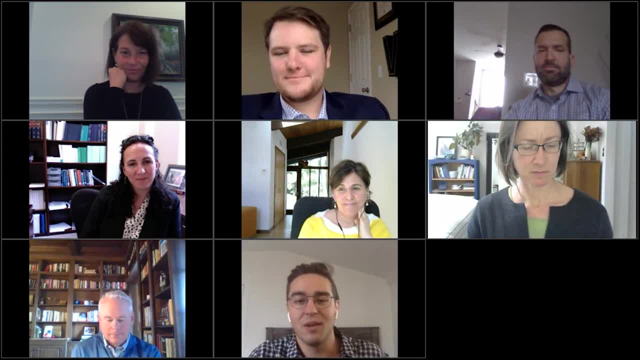 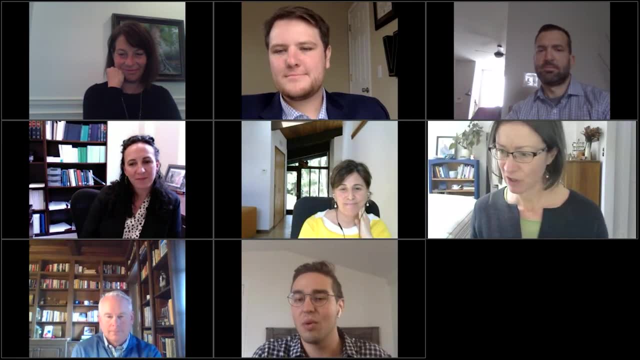 We couldn't have done it without you, Catherine, so thank you so much. I would also be remiss if I did not thank Heather Ludeke, research associate at ELI, Victoria Dorward, academic and educational support program coordinator here at Vanderbilt Law School. 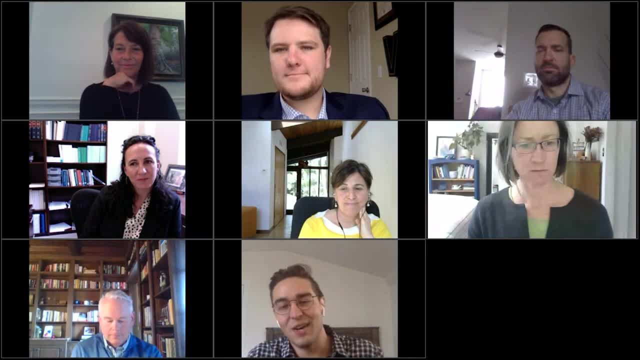 Each have been absolutely integral over the past year, and I know I am not speaking for just myself, but we would have gotten lost many times without their help. Most importantly, though, I would like to thank Professors Bregan and Vandenberg. 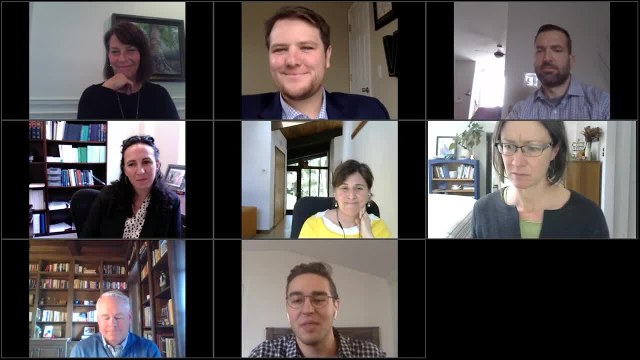 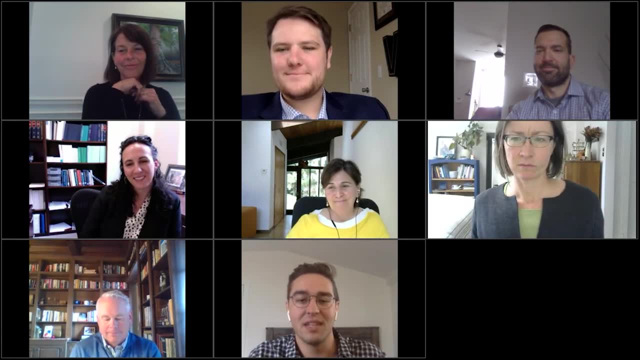 They are our guides and our fearless leaders, and none of this would be possible without your support, your guidance, your knowledge and, especially, your passion. We have learned so much from you both and have all been given an amazing experience, unlike anything else in law school. 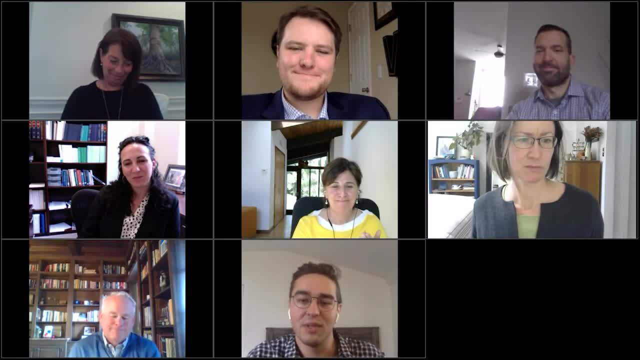 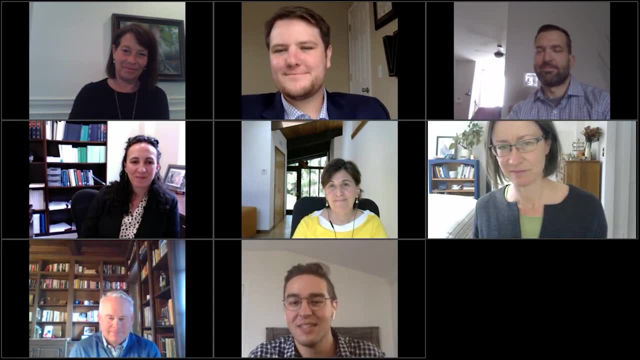 So thank you both so much. Lastly, I would like to thank everyone who attended today's conference. I know that being glued to your computer screen can be exhausting, even after two years of practice, So thank you to anyone who joined us all day. 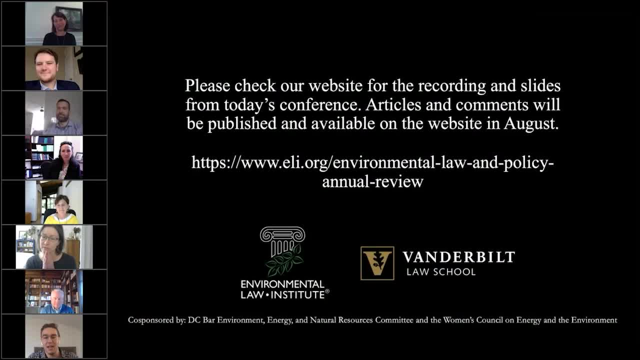 If you'd like to access any of this recording, it will be available on the ELI website within the next few weeks. The articles and their related comments will also be available in August on the ELI website as well as in the August edition. 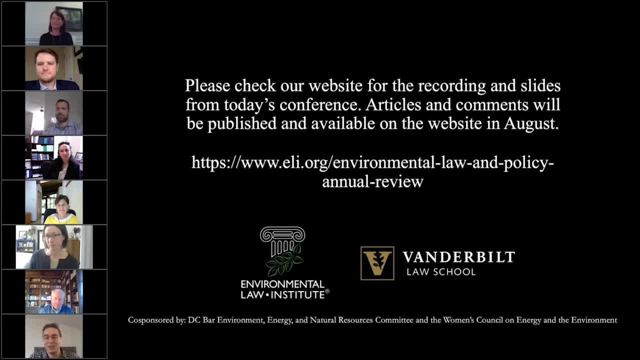 of ELI's Environmental Law Report, And thank you all so much. I know I had a great time and I hope you all did too. Thanks again, everyone.